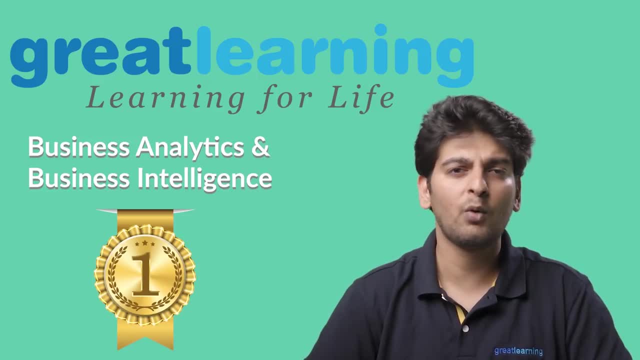 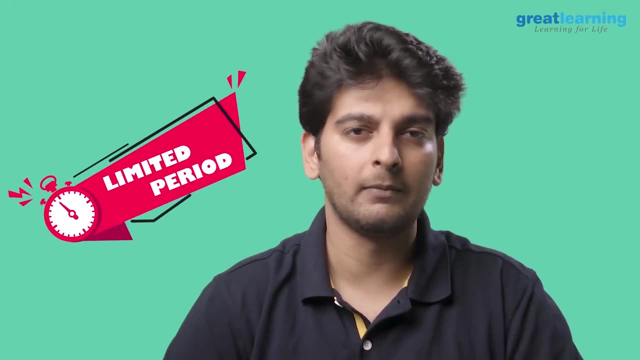 and business intelligence course, which has been made possible by Dr Abhinanda Sarkar. Dr Abhinanda Sarkar has been ranked number one analytics program consecutively for the past five years. This tutorial will be on YouTube for only a limited period of time so that learners across. 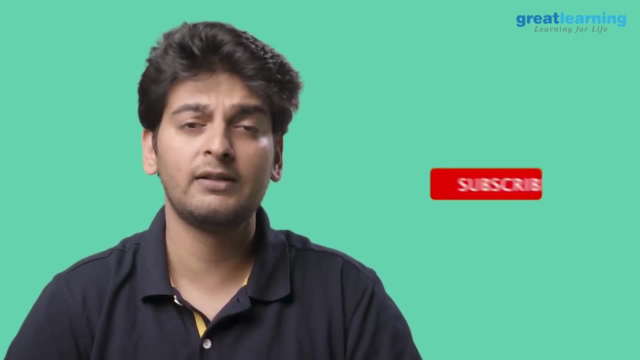 the world can have access to high quality content, So please do subscribe to great learning's YouTube channel and share the video with your peers so that everyone can learn from the best. Now, without further delay, let's have a quick glance at the agenda. We'll start. 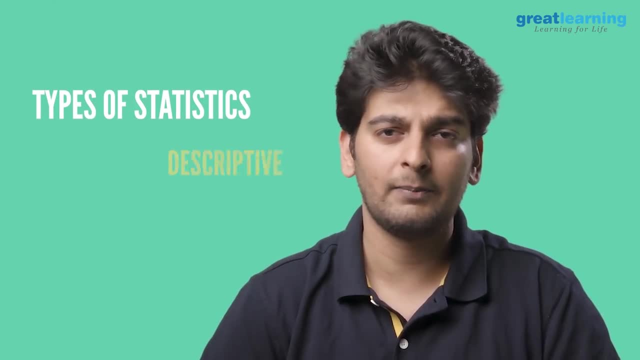 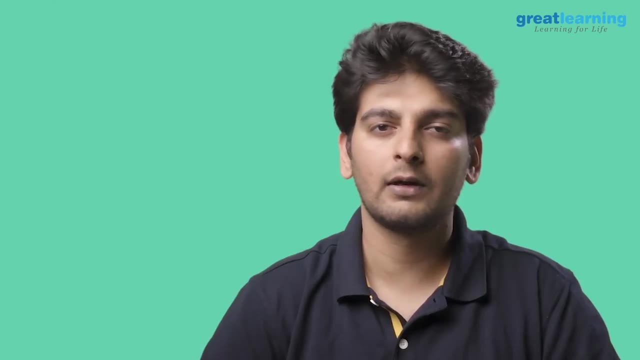 off by understanding the types of statistics, which are descriptive, predictive and prescriptive. Then we'll understand what exactly is time series forecasting. After that, we'll look at the components of time series, which are trend, seasonality and irregularity, Following which we'll 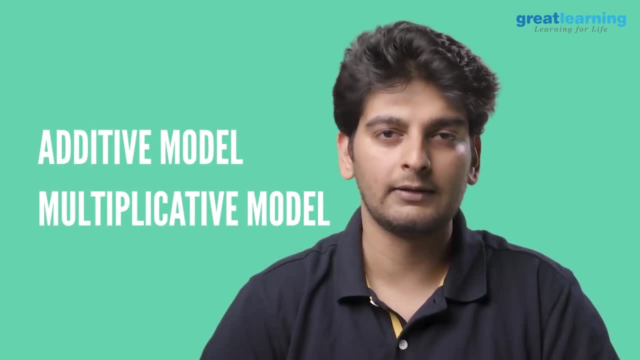 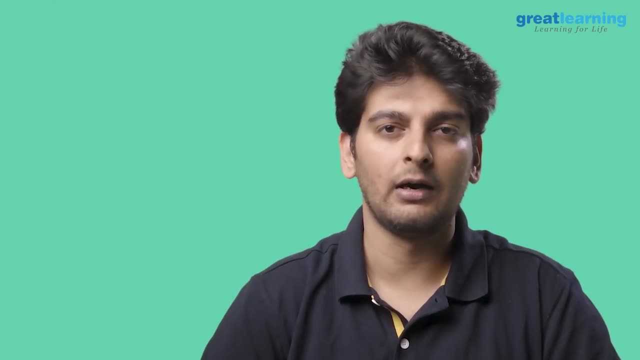 look at the additive model and multiplicative model in time series Going ahead. we'll look at some of the measures of forecast accuracy. Finally, we'll work with two forecasting methods, which are random walk with drift and exponential smoothing. So let's start off with the session. 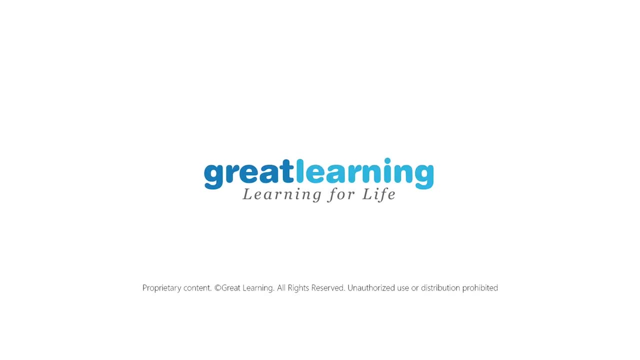 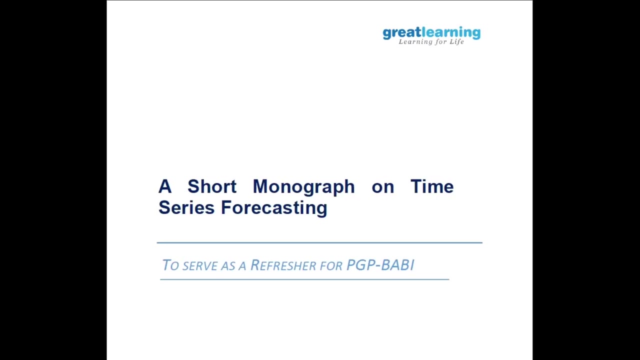 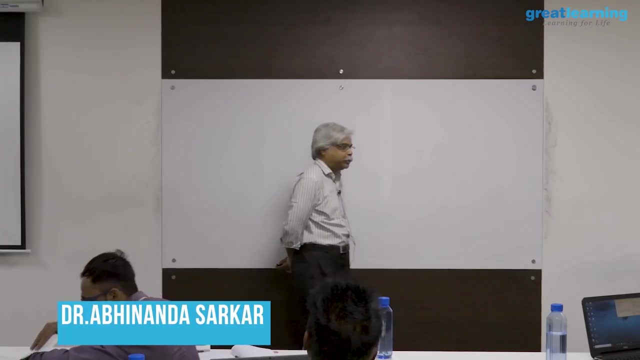 So let's start off with the session. So my name is Abhinanda Sarkar. I usually teach in the BABI programs for the first part of the statistics courses, So SMDM, advanced statistics, things like that. So I don't think you and I have 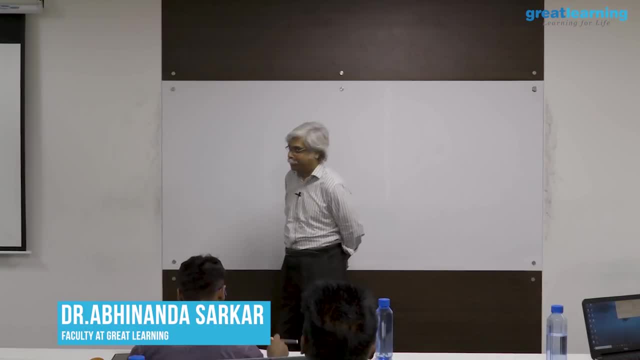 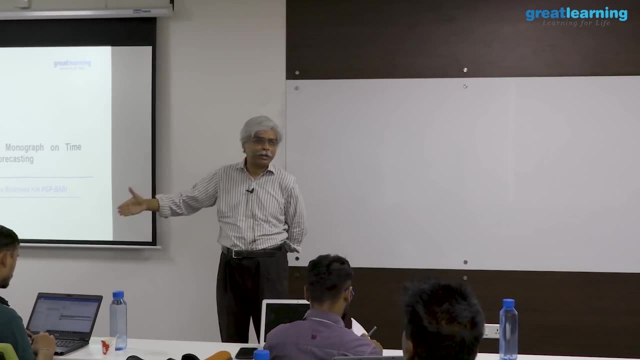 met right Very good. So now we'll be seeing too much of each other because what we're going to do is we're going to do all of time series in sort of one residency. So we're going to talk about time series, So we'll do four hours today, we'll do four hours tomorrow and we'll do four hours on. 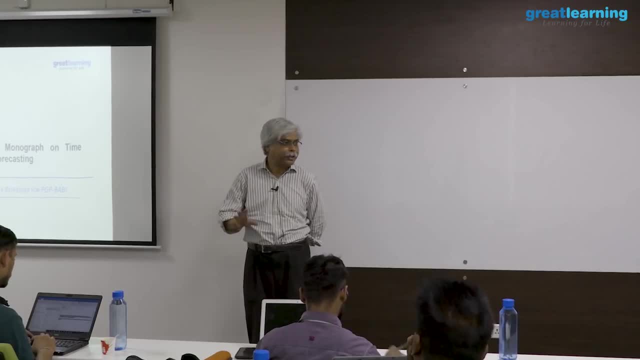 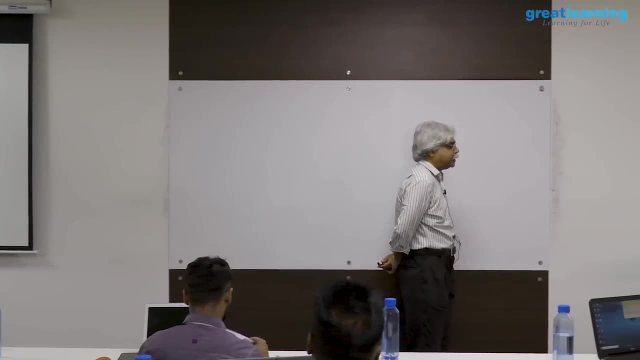 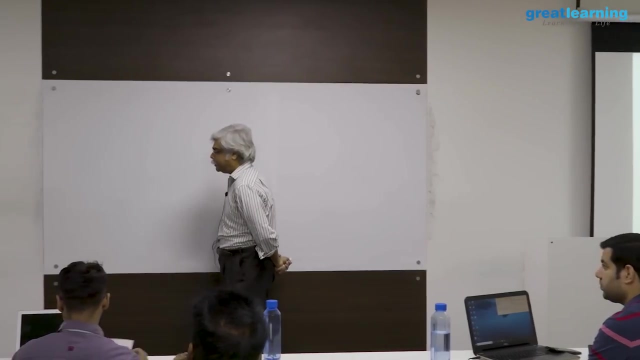 Sunday, And I think your afternoons are the same way, right, I think you're doing marketing in the same way, one in three. So it's a very simple residency, a little long, but I think both sides will be will be interesting to you. So whenever I've taught time series this: 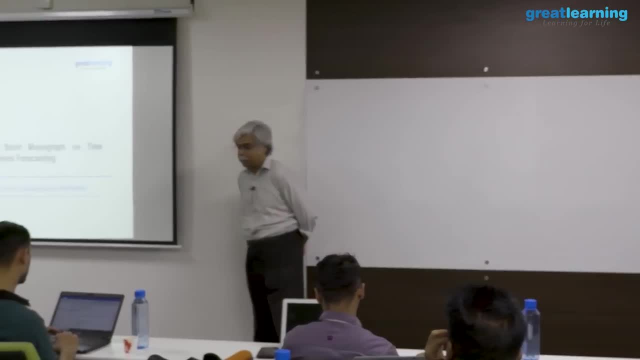 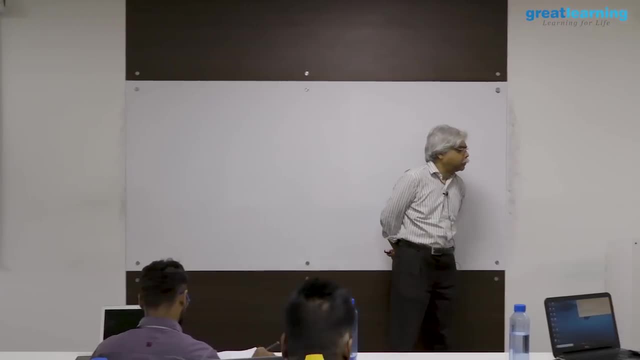 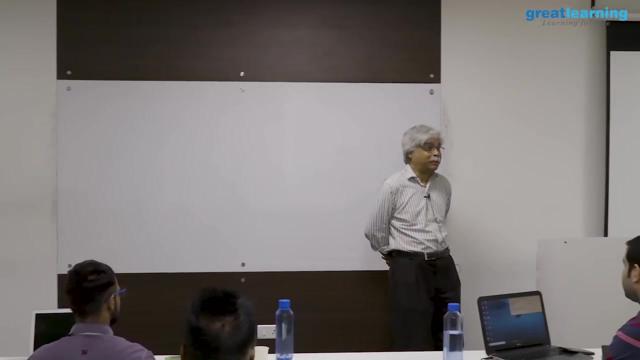 has gone a little differently for different groups. We can modify as we go along. There are sort of math sides to this that some batches are very interested in. There is the R side to it and the algorithm side to it that many people are interested in. 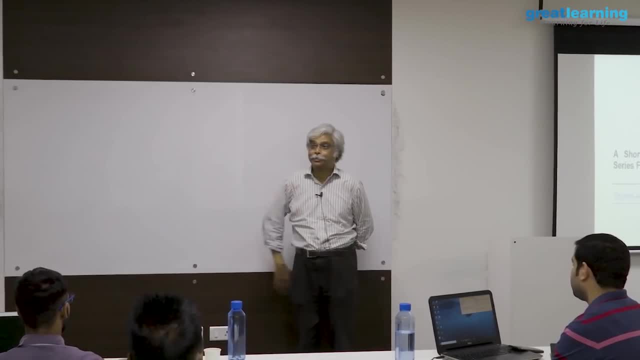 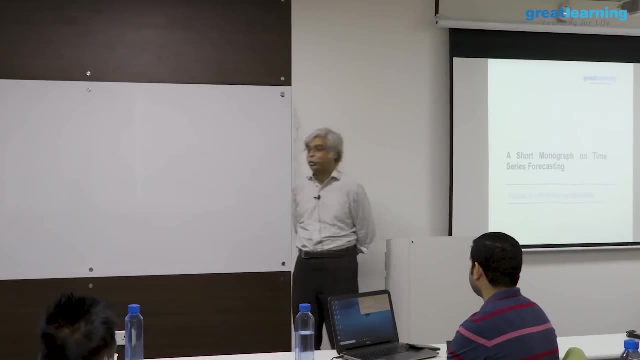 And then there's the business side to it, the applications and where all this goes that people are interested in. We'll see where your temperament lies, what you are passionate about, and we'll spend more time on it as we go along. So if we go slowly, then we'll kind. 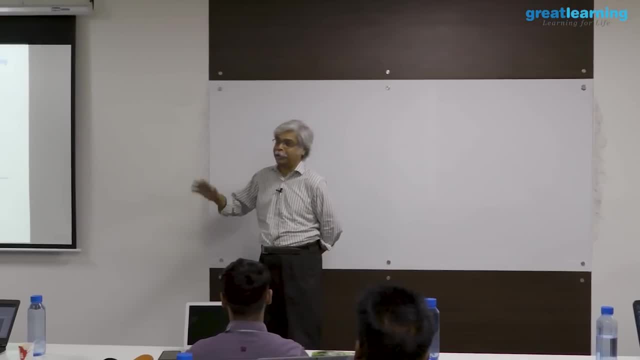 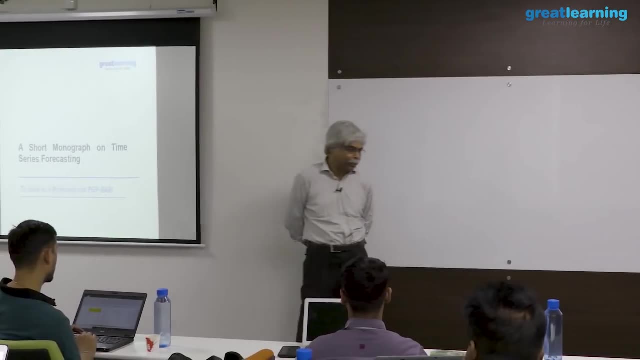 of cover the material. If we go too quickly, then that's okay. On Sunday we'll do some case studies and look at other data sets and you can try your hands out. So not to worry, we'll pace it as we go along and we'll see how it shapes up. Okay, tell me a little bit as to. 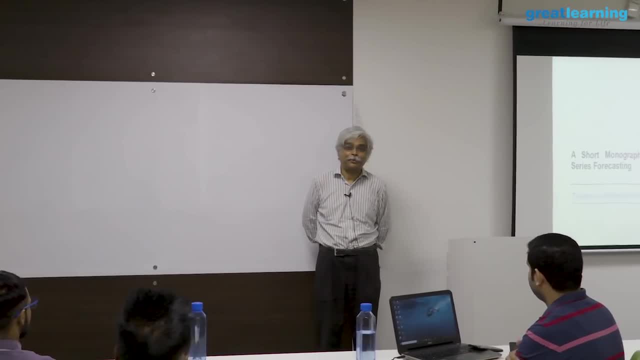 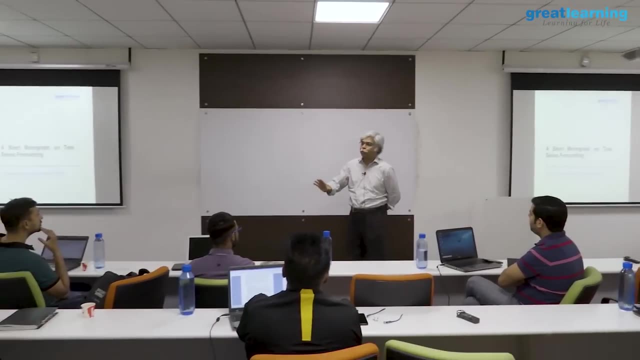 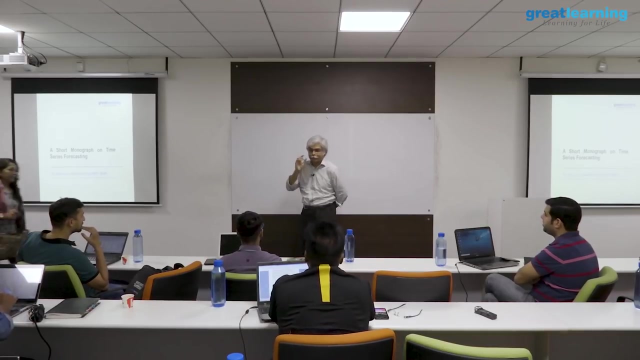 what you've been up to. So what happened in the last residency? What have you done so far? Predictive modeling: Predictive modeling is done, So you know. linear regression, linear regression, logistic regression, linear discriminant or discriminant analysis, LDA. 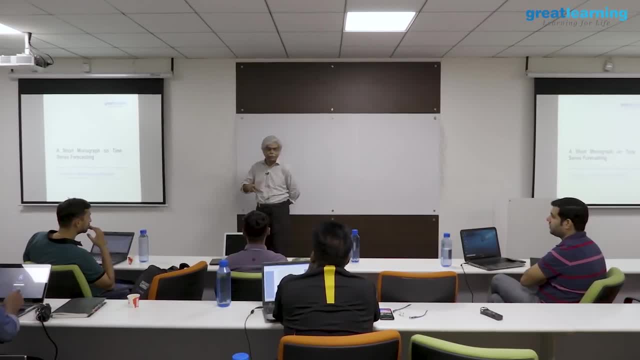 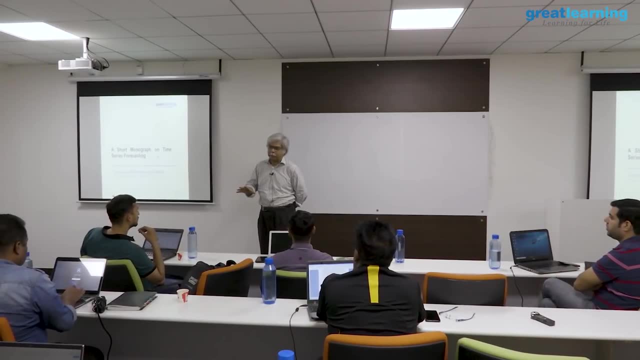 And that was last residency, That finish. last residency, PKV taught this one Gurmuchar, but he also taught conjunct analysis, So that that will be useful, I think, for the marketing research path. So that's a typical marketing technique. and on the data mining side, 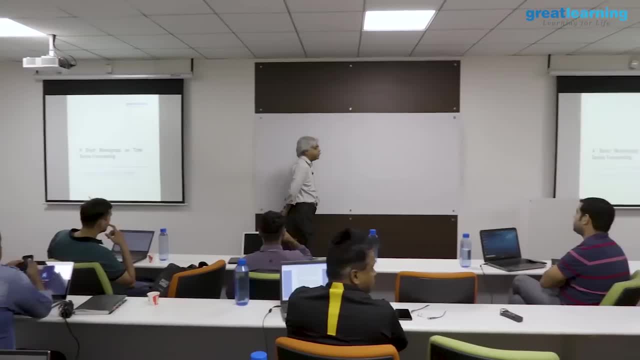 Random forests, neural networks, decision trees. So the idea of a training, design of data mining practices, forning user data. This is taken to a separate table and someamesu demo looked at other aspects of it, Looked at some of the maintenantwhy it was done, but anyremember more complex patterns for Speed score�, The. 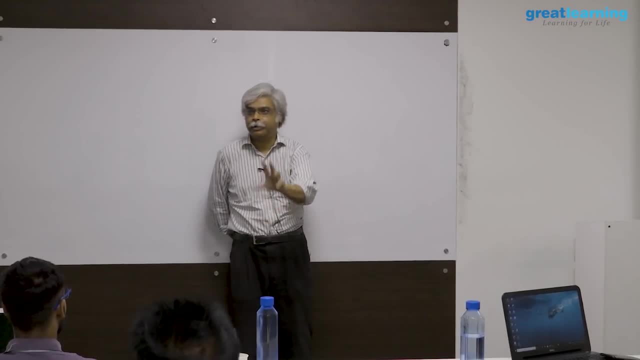 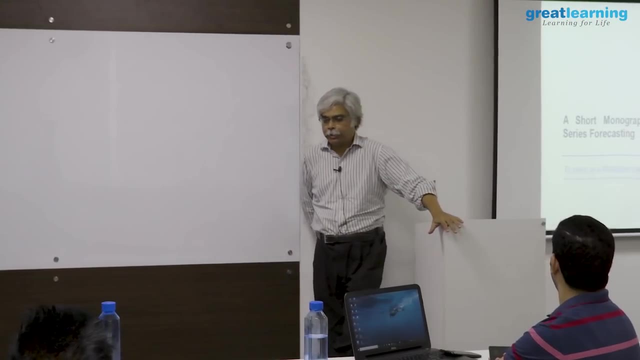 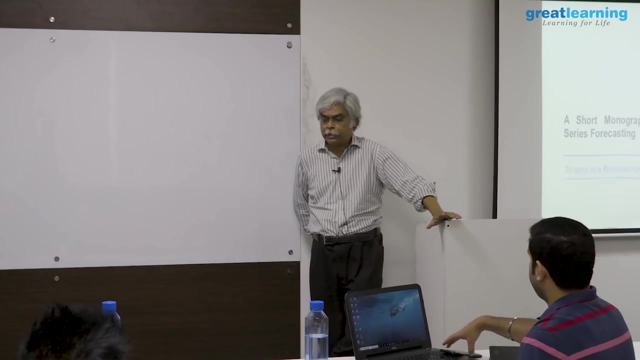 set test, set validation, said: all that has been all that, all that has been seen. okay, cross validation correct. so what? we'll be using some of that for for this module. so this is a module that follows up on the statistical side to it, in other words, the look and feel, for it will be a little bit statistical in its 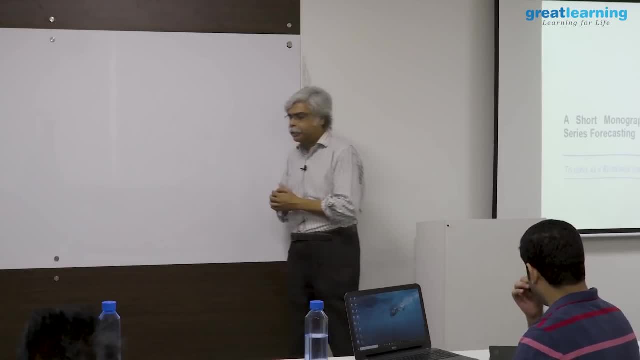 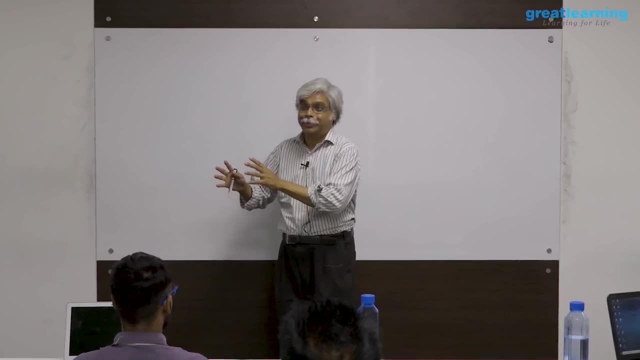 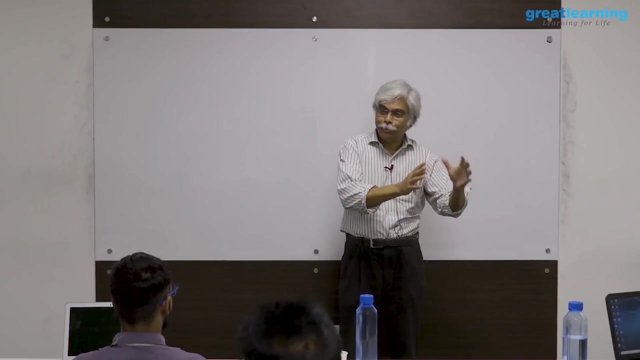 nature, particularly the second half, but the forecasting methods, as you will see will become, will be evaluated using machine learning, like holdout type methods. if I know the past, then I know the present. if, therefore, I know the present, then for I know the future, we'll take that idea and we'll build some test. 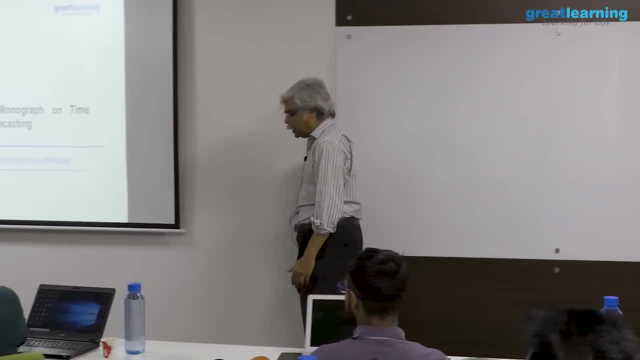 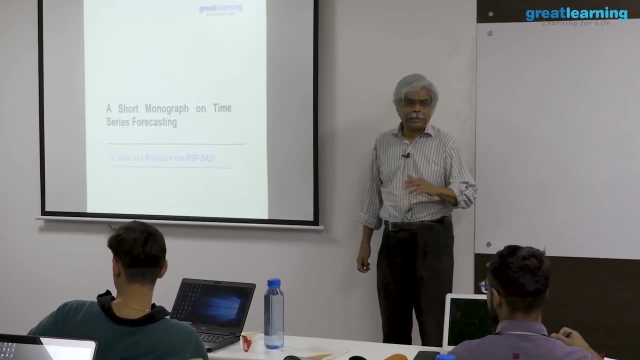 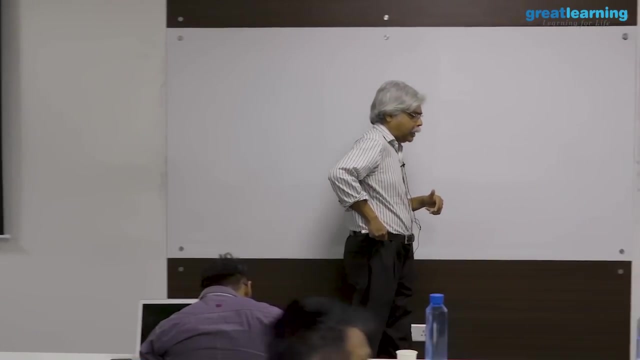 training principles around that and then what else. so none of the domain courses have happened. finance has not happened. this is the first one. this, this residency is the. this is the first one. this- this residency is the first one. this- this residency is the first one. this- this residency is the first one unsupervised. 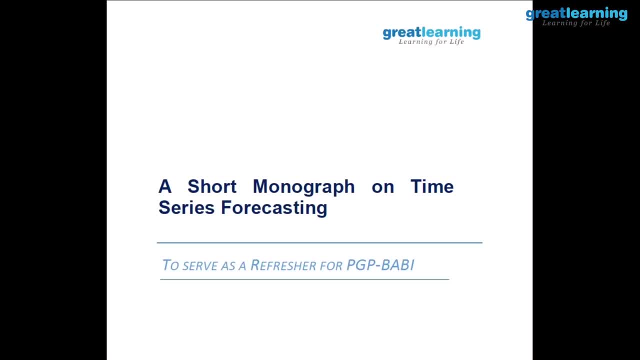 learning, clustering, clustering and things like that, k-means and stuff, stuff of that sort. that is an advanced statistics, which you have, which you have also done, analysis of variance- any major thing I'm missing. that's about it. right, I haven't taught all the modules, but but some such things. 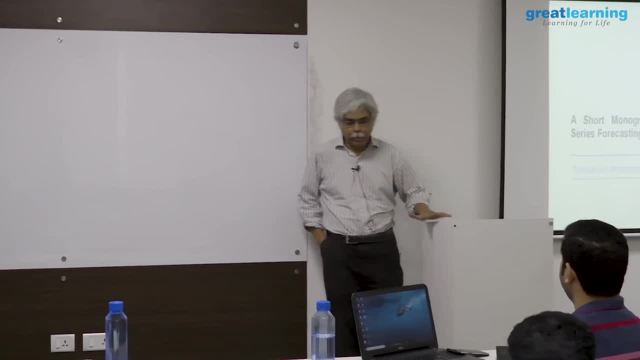 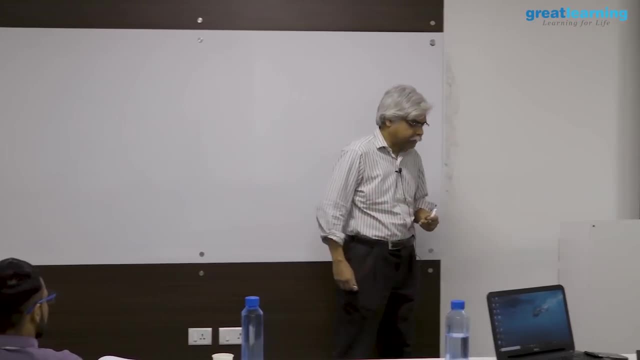 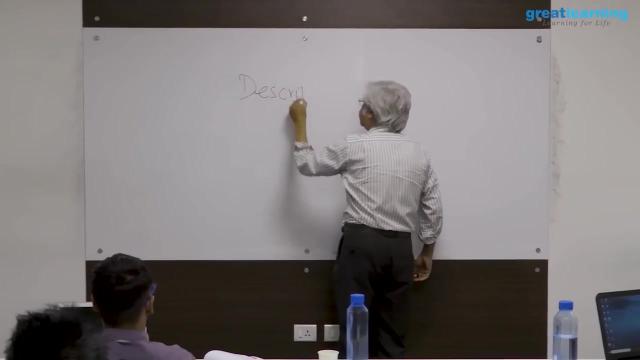 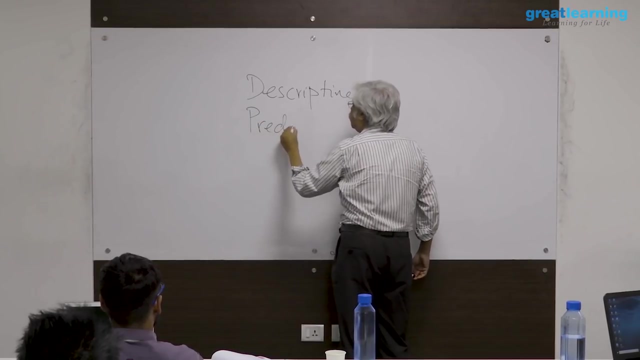 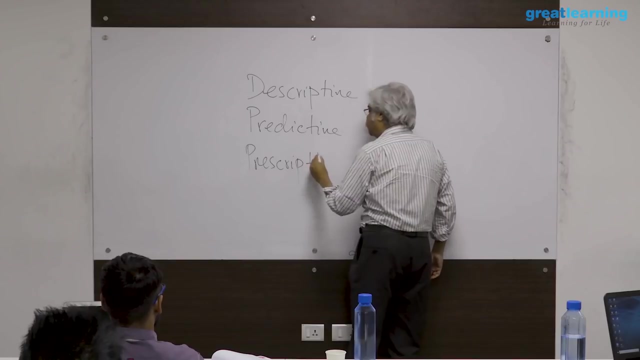 all right. so usually when an analytics session is done, it's often done using certain certain definitions, certain ideas. so some of the words that we often use, for example these things you may have seen already: descriptive, predictive and prescriptive. so there are other ifs as well, as you said, diagnostic. so these are the ways. 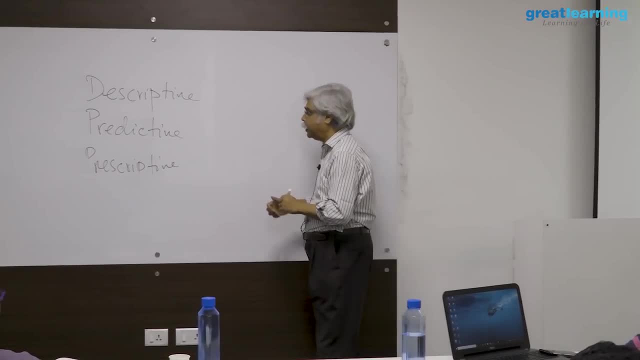 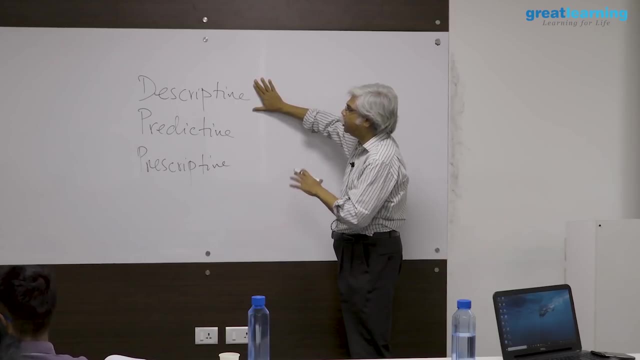 that is usually talked about, but there are other ways of doing it as well. the description is more about saying: here is the data and I'm simply going to tell you what it looks like. prediction means I need to be able to build a model on the data in order to 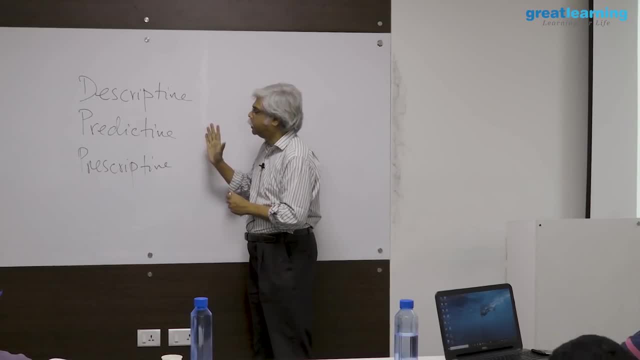 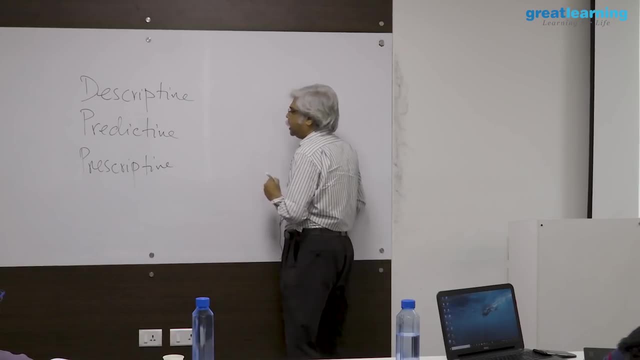 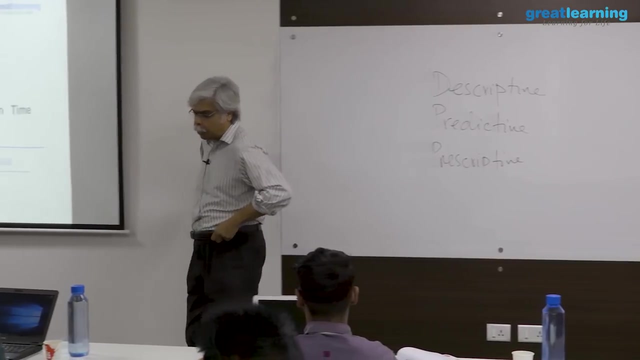 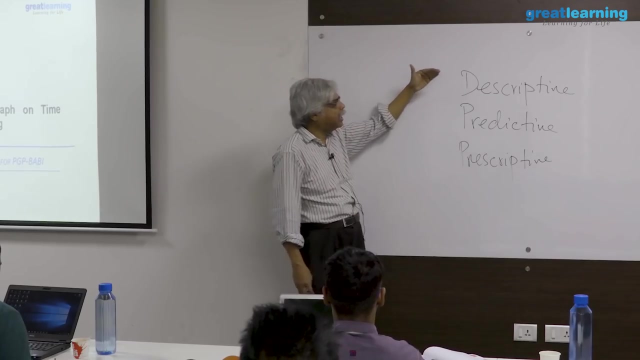 answer certain what-if type questions. what if my X becomes this, or what will happen in the future? prescription is roughly speaking, so what if this is what the prediction is? this for the description is: what actions should I take based on what I see? very roughly speaking description would be something like saying how many. 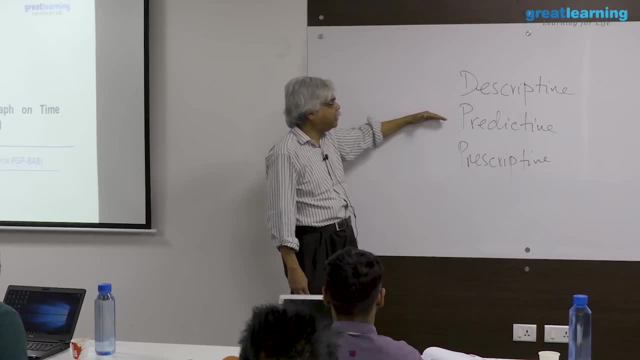 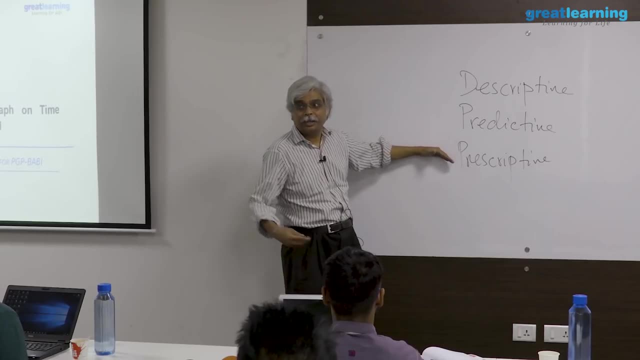 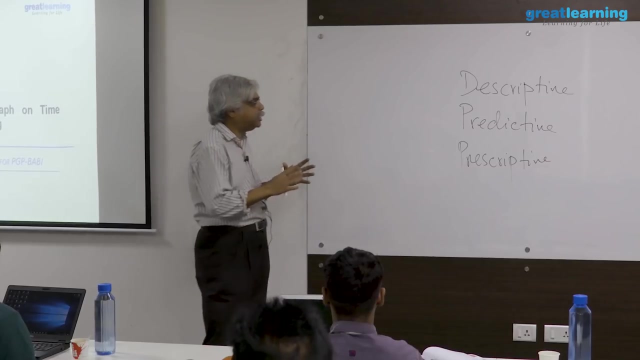 centuries has Virat Kohli scored? predictive is like how many will he score in the World Cup, and prescriptive would be: how do we get Virat Kohli to score more centuries, which is the business end of the problem, so to speak. some of this is, of course, description is mostly about the data itself. in other 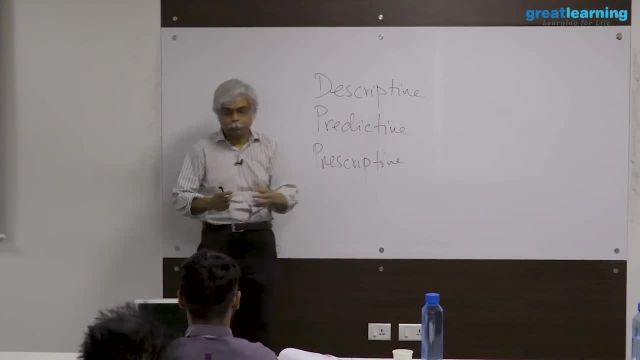 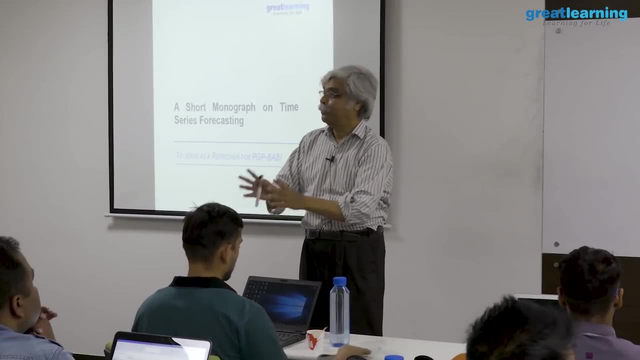 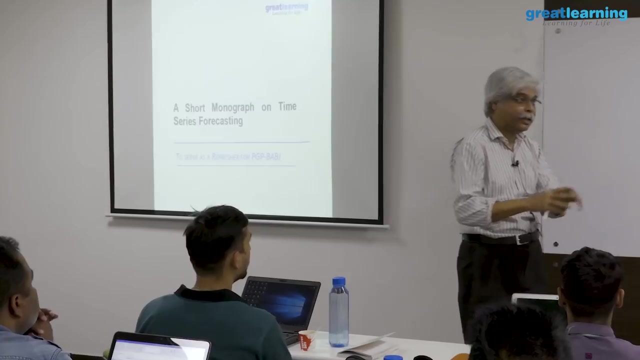 words. it looks at data and it simply says: I'm going to do some processing on the data- maybe visualization techniques, maybe database techniques- and say this: is it? quick info, for example, is good descriptive. IMDB, the movie database, is good descriptive. there's no model there, but it's a it's. you want some? 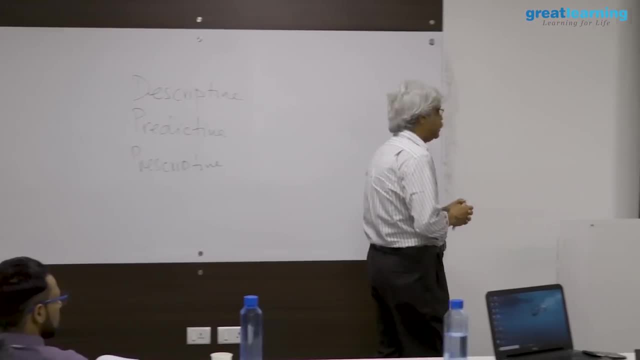 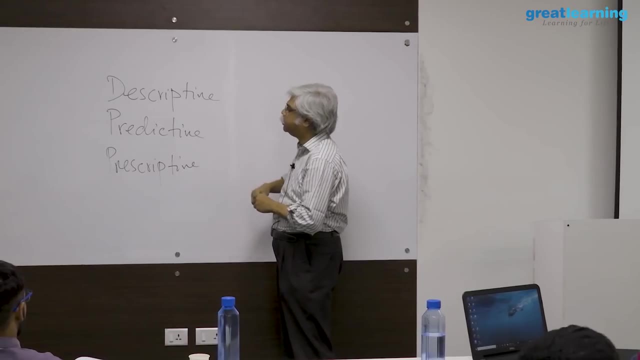 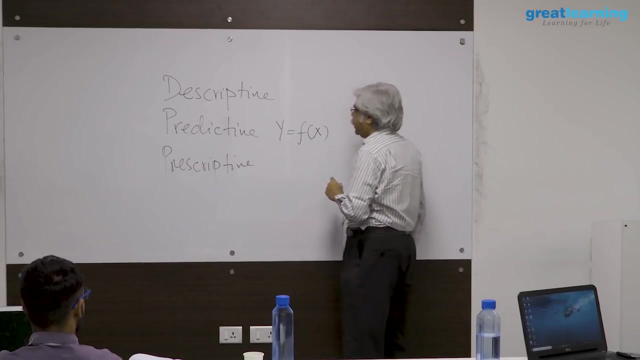 information about the movie. you'll get any information about them if you are here. it's a combination of working with the data and having a mathematical structure on it. so, for example, you often have equations. say Y is equal to FX. in this case, predictive means what predictive then says that if I give you 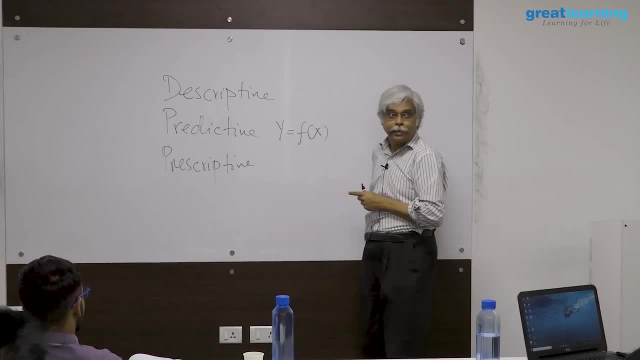 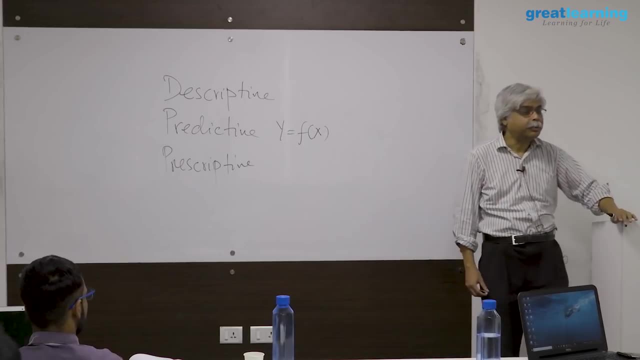 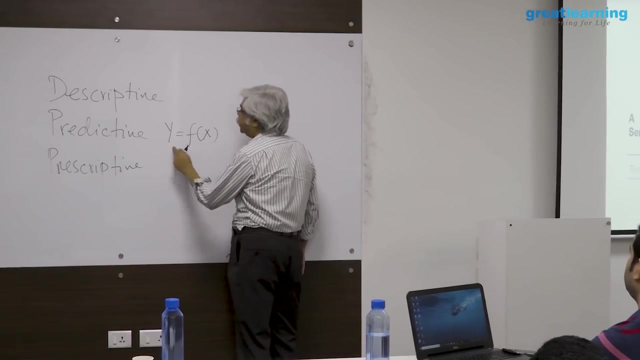 an X, you must give me a Y, which is what supervised learning essentially is all about. all the neural networks work, and all the regression work that you did was essentially dedicated to that. of course, that doesn't mean this is the only use of predictive. you can also have an equation that says Y is equal to FX, and you can also use it. 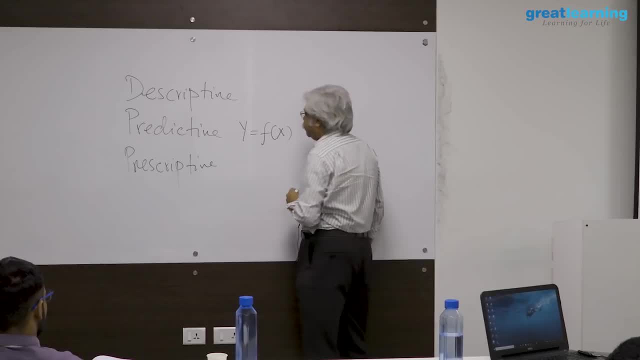 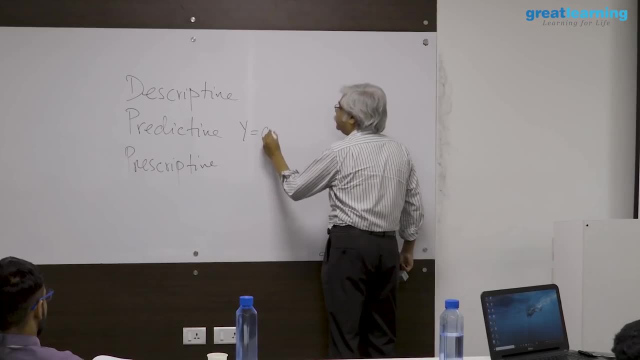 purely to describe. so, for example, you could say that, instead of Y is equal to A plus B X, I'm going to write a, going to write an actual equation for it. let's say, I'm going to write Y is equal to A plus B X, when this is a descriptive. 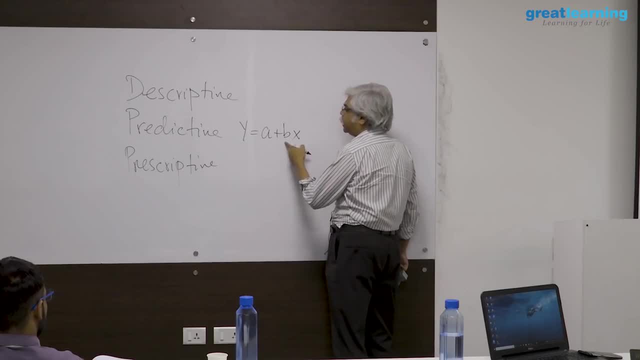 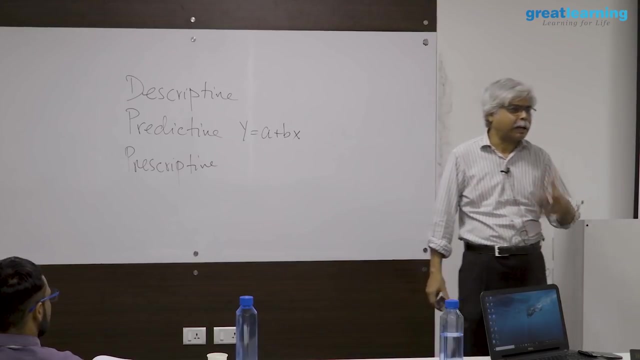 of data, then A and B means certain things. so, for example, what is B? B is: if X you increases by one unit, then Y increases by one unit, for example in marketing. you may do this and use things, use concepts of elasticity. if price goes up by one unit, what happens to sales? if price goes up by 1%, what happens to? 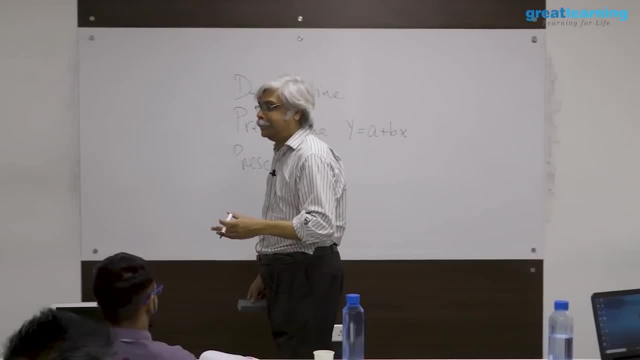 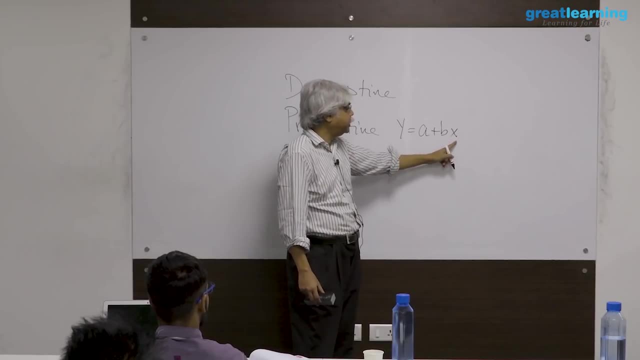 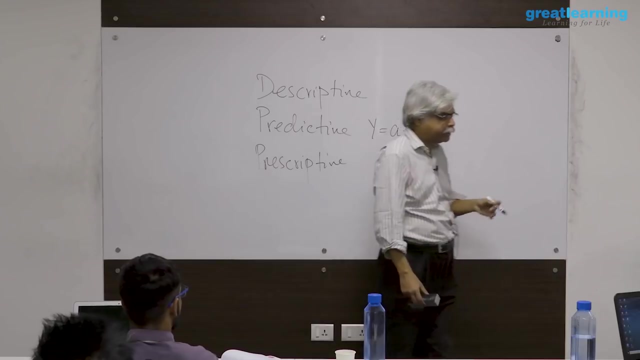 sales. that's usually called elasticity of demand. it's a description. another use of it could be to say that if you give me another price point, then what will be my sales? to use it to predict. if you want to use it to predict, then certain things have to go, have to be done with it. one basic principle of prediction is an idea. 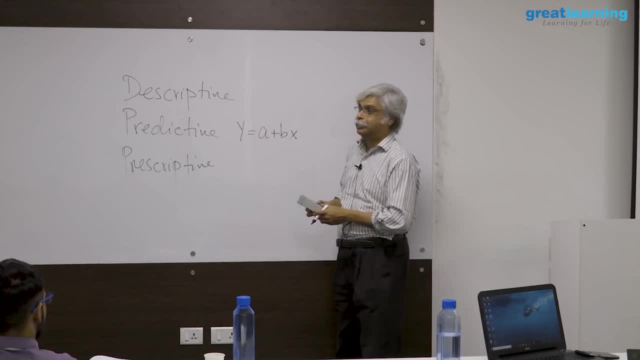 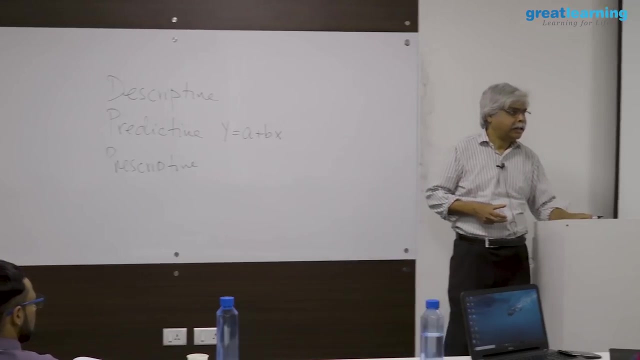 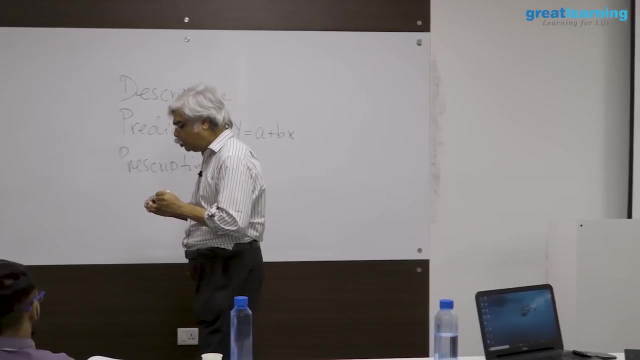 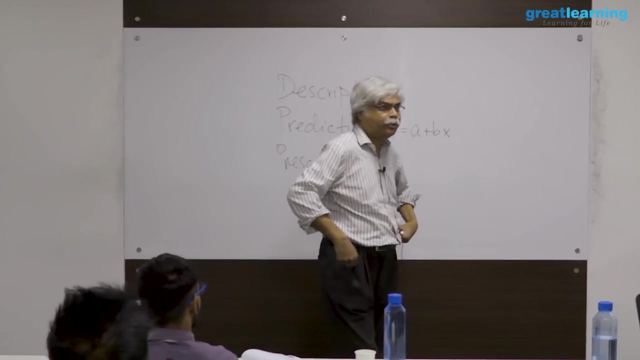 as to why is the prediction good or how good a prediction is. how do you answer that? performance on what? and then say what? train and test? there are many parameters around. why do you do that? okay, so what? what does your answer typically tell you what? what does? 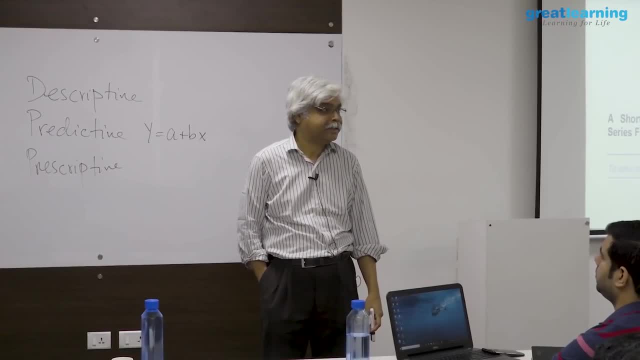 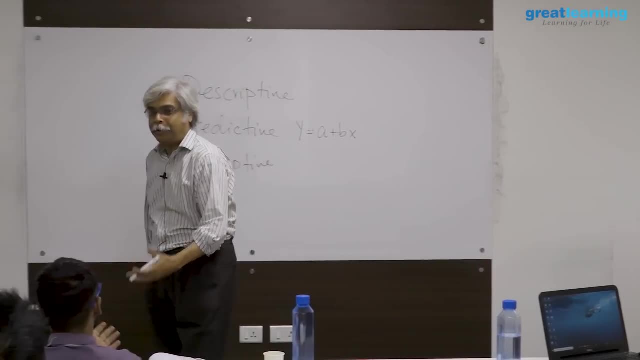 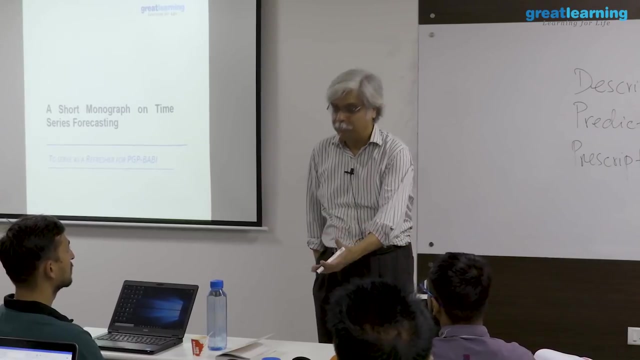 the. what does the result of a test training analysis look like? or when you do a cross-validation, what do you end up with? give me and give me a number. what is it? what does the number look like if it's a classification problem or if it's a percentage? wise percentage, true. 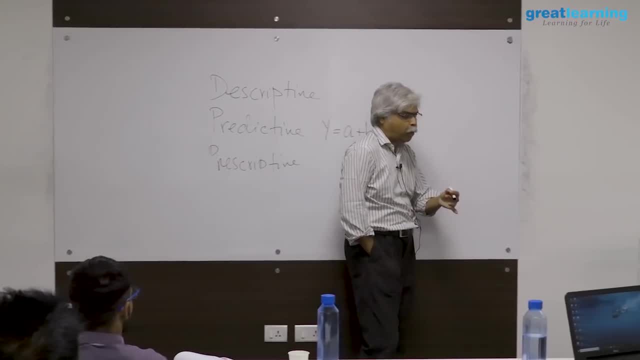 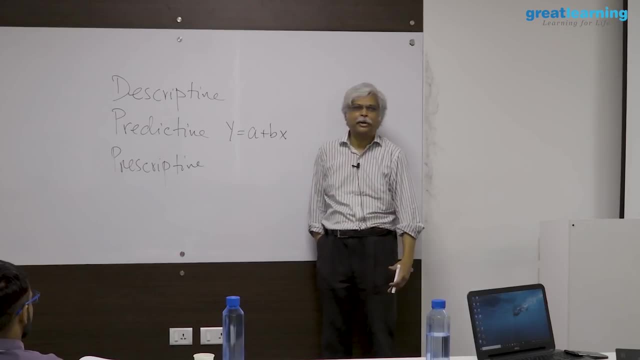 positives or true negatives, confusion for what? so let's say that your, your true positive or true negatives, your sensitivity, specificity, precision, recall what? if you call it, let's say it's 10%? oh well, not 10% is horrible, right? 90% the other way around. so 90%. let's say it's 90%, accurate. what did that tell you I? 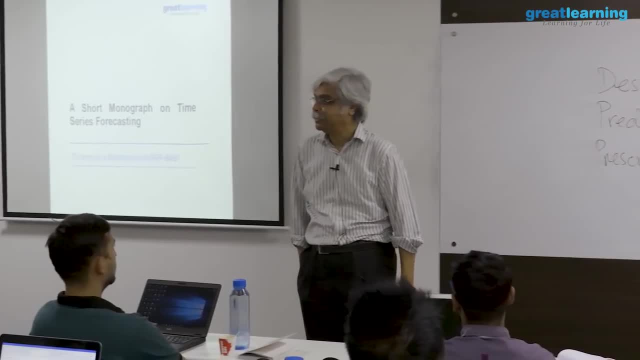 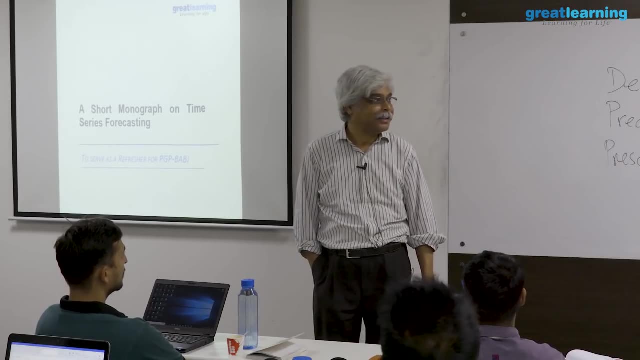 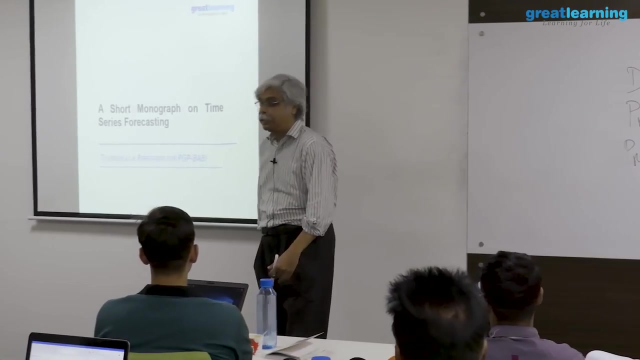 mean. 90% of the time I'll be okay. 90 percent time a prediction is correct. so I'll give you two interpretations. tell me whether each one of the right or whether both are right or neither is right. one is: give hundred people predict correctly, ninety of them will be right now. ninety of ninety. 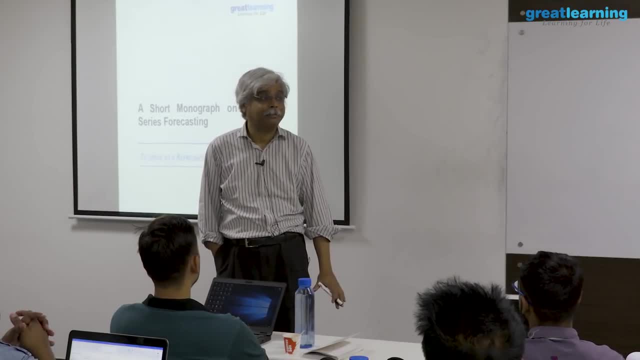 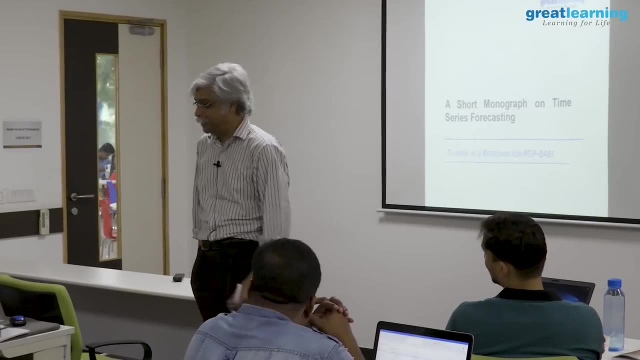 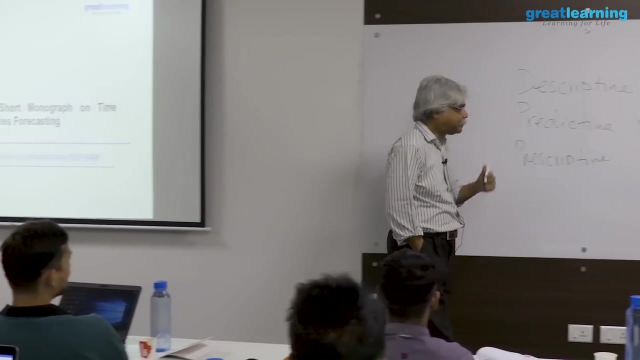 hundred people are predicting using your model. ninety of them will be correct. no, okay, one person uses your model. there's a 90 percent chance that he's correct. you like that one better? okay, all right, different people like different interpretations to it, but that's that's one way of doing it very, very good. now, how did you do it in? 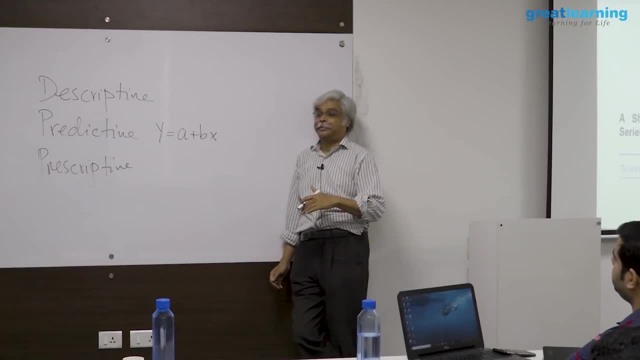 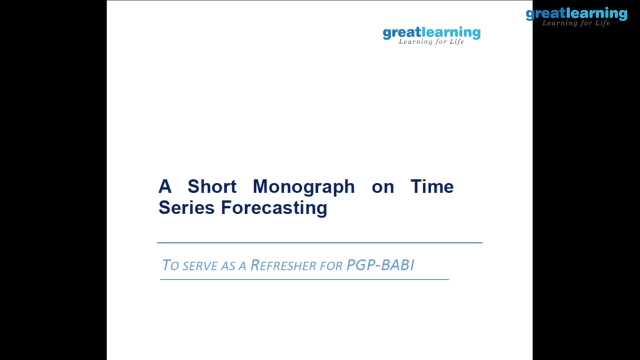 regression, linear regression. what did you do with the linear regression? you found an R square. what did that tell you? okay, so now, given a linear regression, what should I do? should I take out 70 percent of it and test it out on the remaining 30 percent and tell you the error, or should I use R square? okay, do. 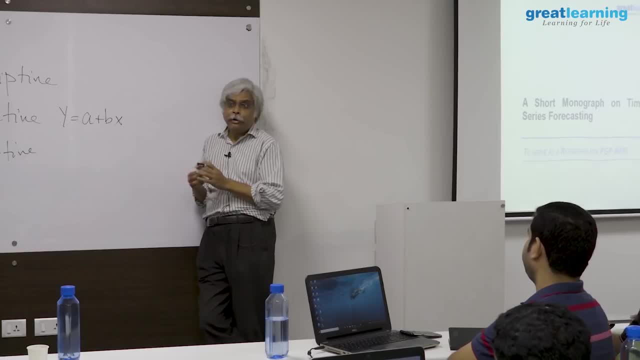 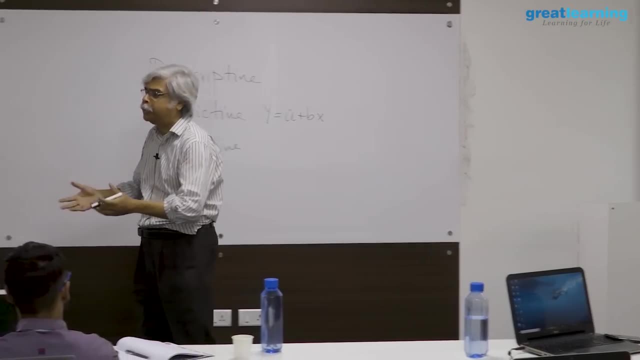 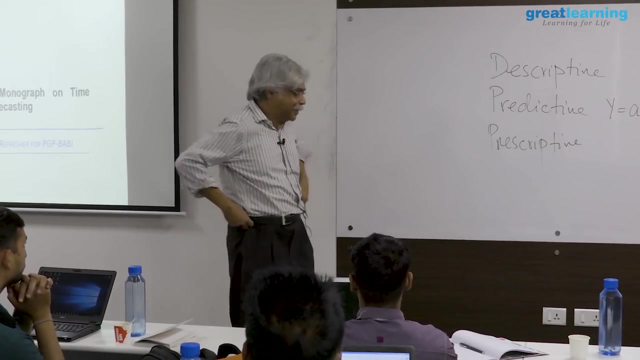 you do neural networks. did you calculate R square for neural networks? why not? why we're not interested in the percentage variation there? what is the difference between a linear regression and a neural network? that's a black box. so whenever there's a black box, there's no R square. ah, that's nice way of looking at it. so my experience is there in both very 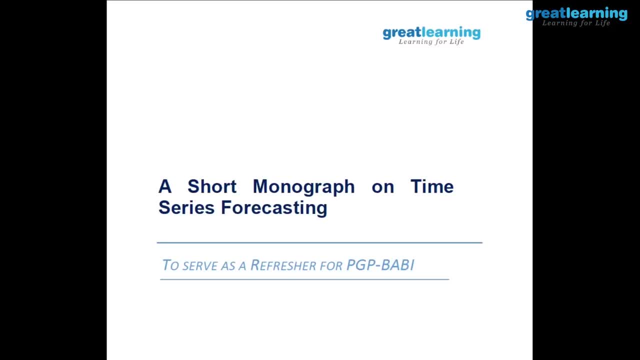 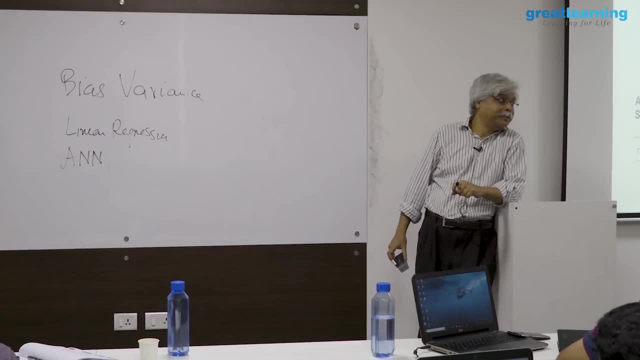 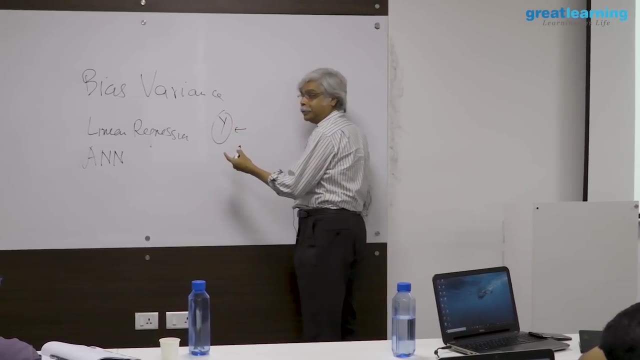 good linear regression goes after which one? that's a, that's a method, another method. let me ask you this: given Y and given X, let's say a continuous Y, give me an example of that, like of a continuous Y, a number sales, okay sales. and then let's say: this is: 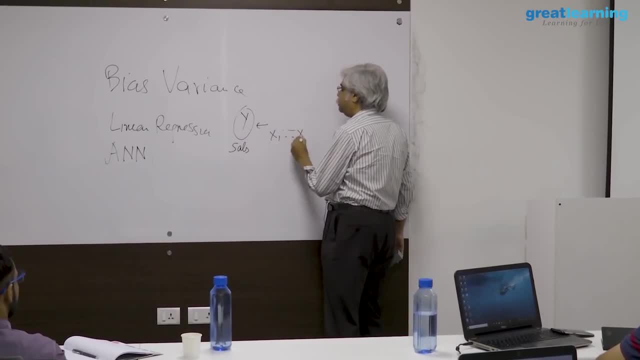 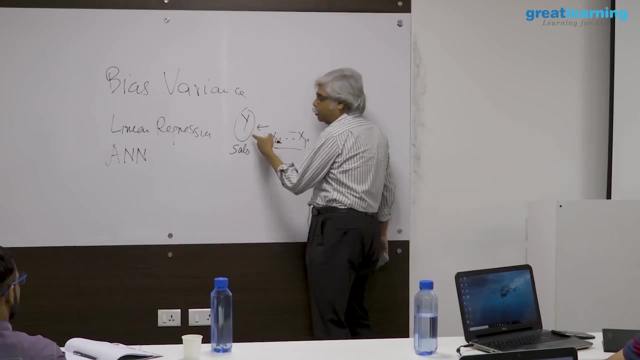 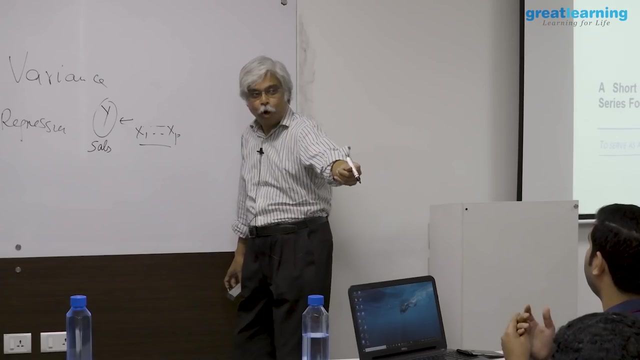 sales, and I have lots and lots of data here, say x 1 to X, P- whatever- I've got P, X's here correct. and you want to predict Y, what model would you use? and Y, and then what would you do with it? all right, so what you have done is essentially you. 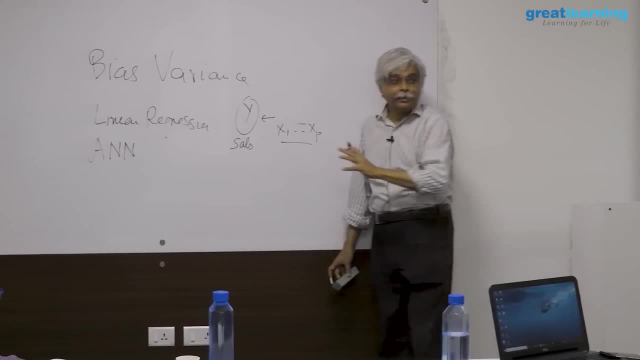 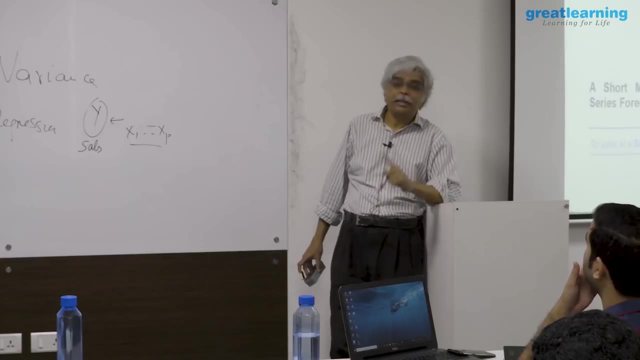 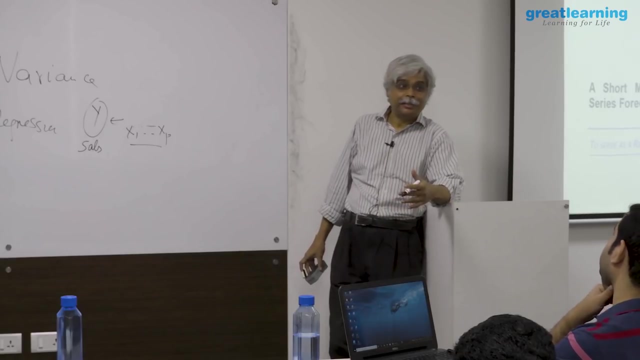 have told me that if it is a descriptive purpose, a can go for a linear regression because that that linear regression describes the thing you know understandable way. there's an equation, there are coefficients, there's a model, but if your purpose is to predict and not care about, 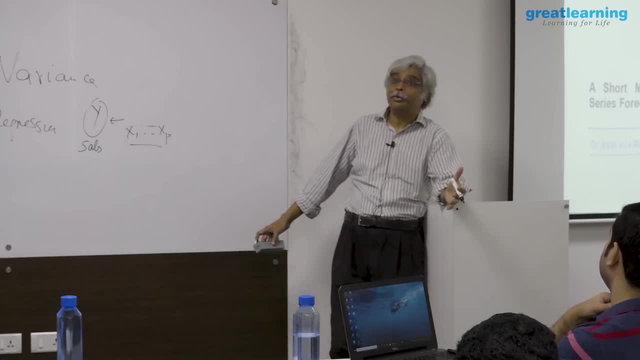 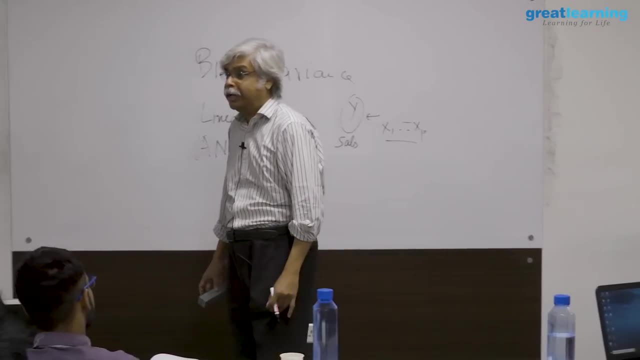 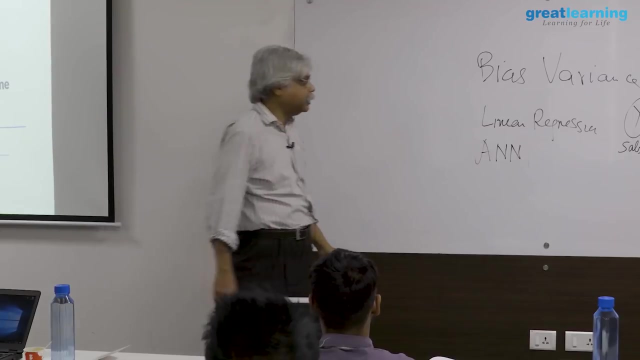 what's in the model, then maybe you can use a model that has no interpretation, no coefficients, no description associated with it, but all you're interested in is the prediction. you can, it's harder you can. I mean, yes, a neural network does effectively what a linear regression does. it's just that that the 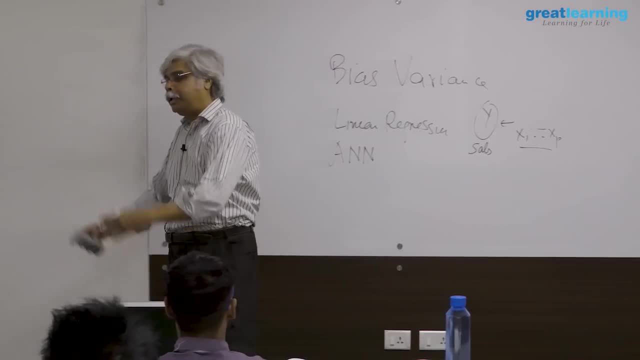 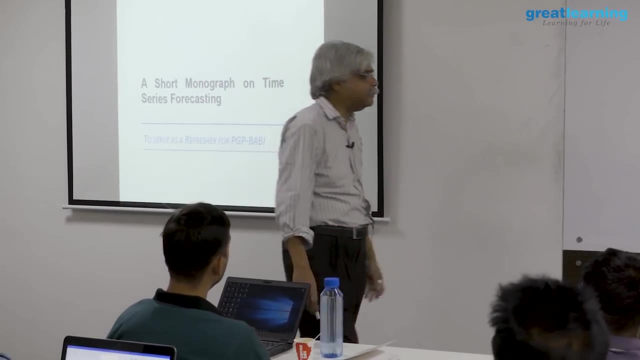 model is a lot more complicated. so there are many, many more parameters sitting there, the weights and the offsets and the biases, and and instead of having a something very simple like ordinary squares, you've got back propagation and. but a neural network is designed to do something a little bit more complicated than a linear regression, and that's why we're. 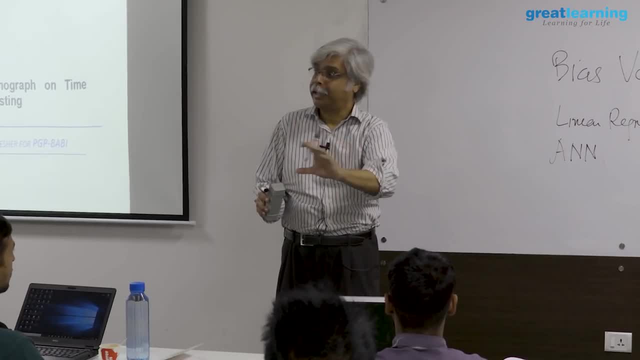 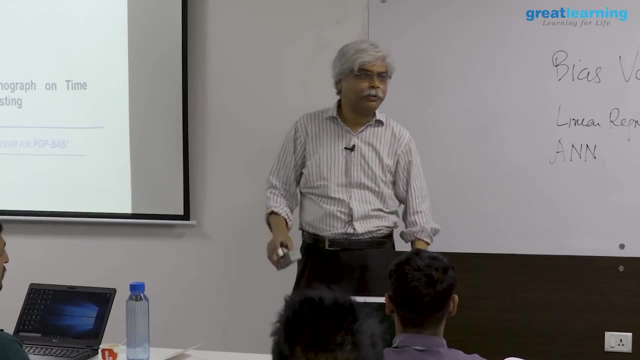 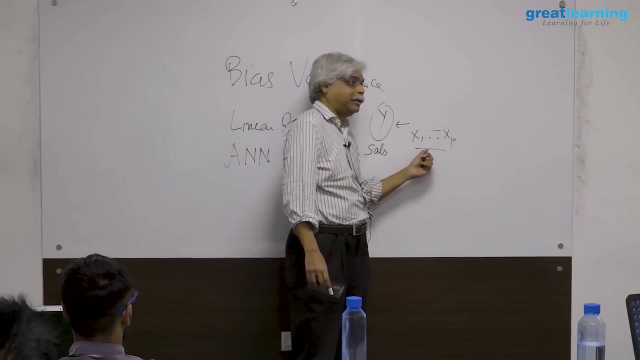 different. a neural network is designed to say that I will forecast and I don't care how right, and the quality of my model will be judged by only one thing: how well I have forecast. a linear regression is doing something a little different. a linear regression is doing- I'm going to give you an equation- what? 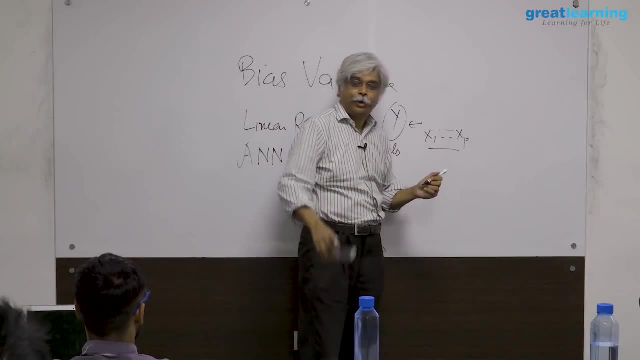 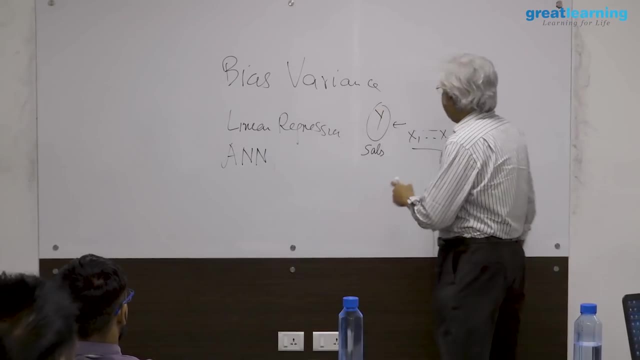 you do with that equation is your business. you can use it to describe. you can use it to forecast. you can use it to prescribe. you can say: if I want my sales to go up by ten percent, my prices should come down by how much you can use. 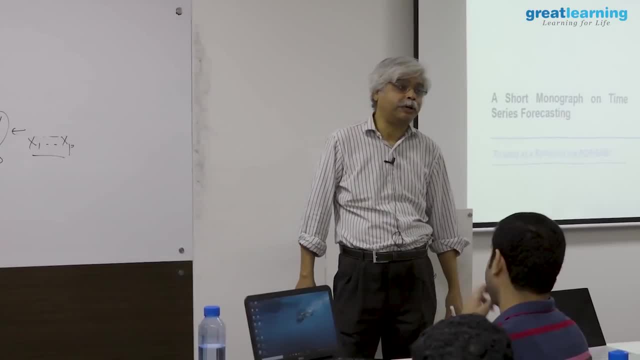 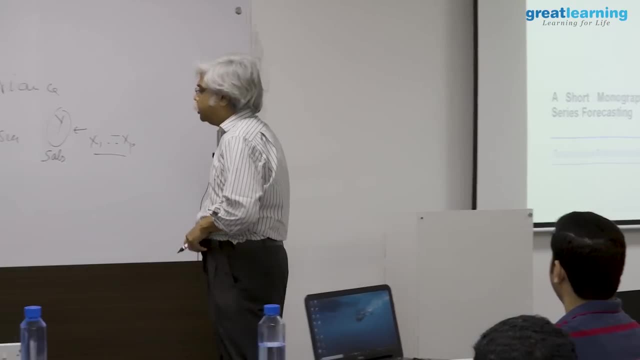 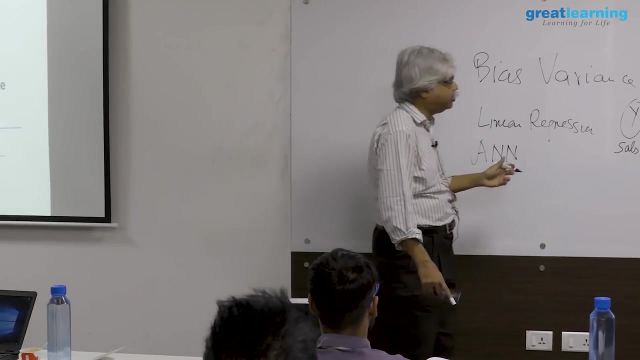 your coefficient to answer that question? that's a very hard question to answer for a neural network. it's not designed to answer a question like that, so they have different purposes. so this philosophy of modeling that you have been exposed to has different endpoints: the, the, the prediction. endpoints are the things that 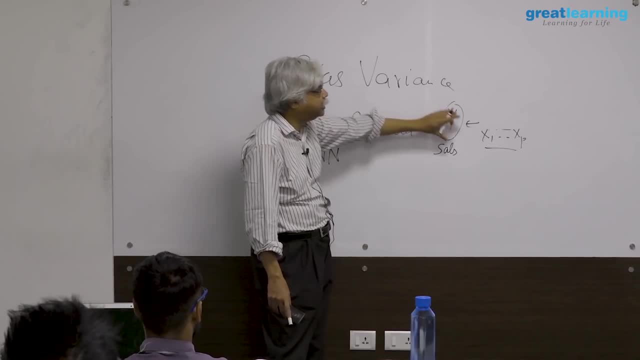 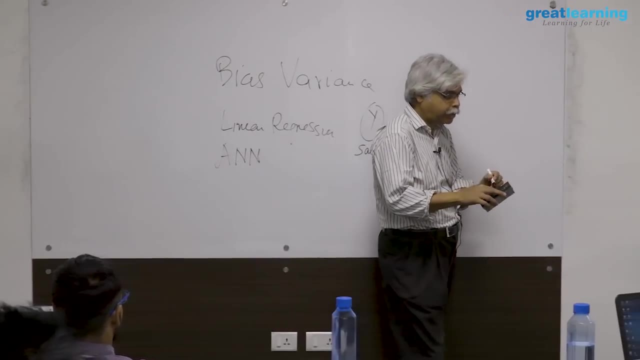 you can predict and it shouldn't be predicted. so this is what we hold true. energy is the end point is an endpoint, that is one of the possible end points of an analytical exercise, which is to say what happens in machine learning. that point of view is is central to the to the exercise, the machine is learned. 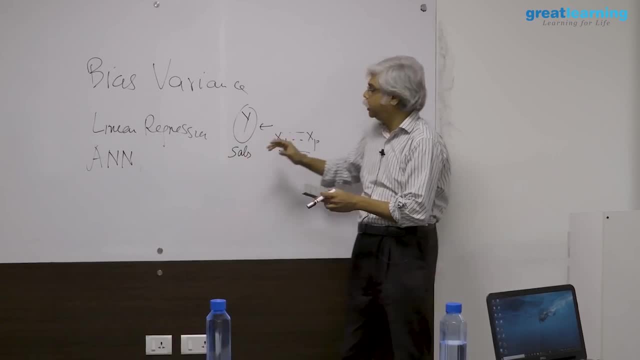 and you're trying to understand how has it learned and therefore use that learning for a new input. give me a new X and then tell me what this new Y is, to say how good that is. you now give it a new set of X's and understand how good. 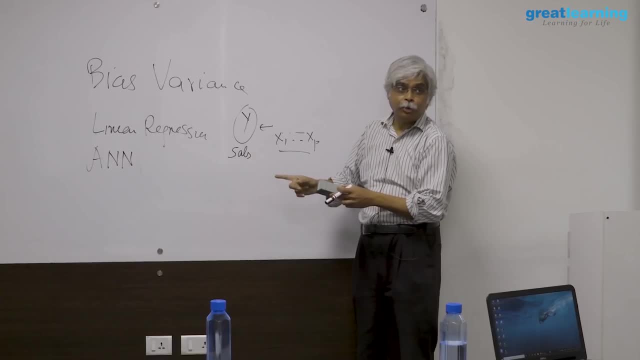 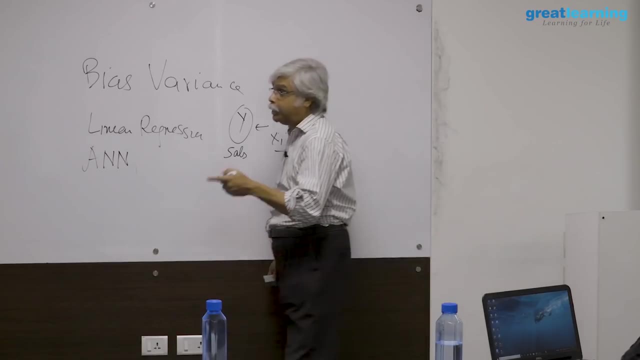 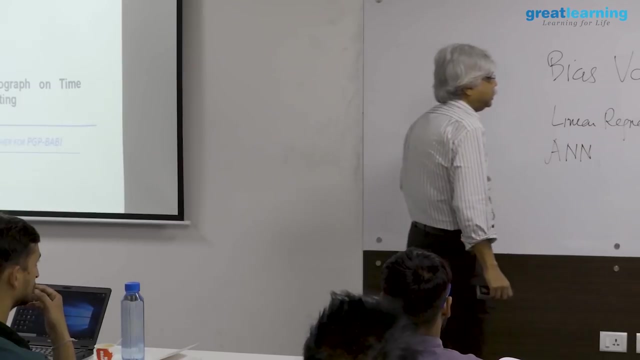 done the concept of overfitting. overfitting means what? it works very well for the trained data. that means it may or may not work very well for the test data lack. it doesn't generalize well, so that's the neural network challenges that premise by essentially saying, okay, if it doesn't do that very well, what I'm. 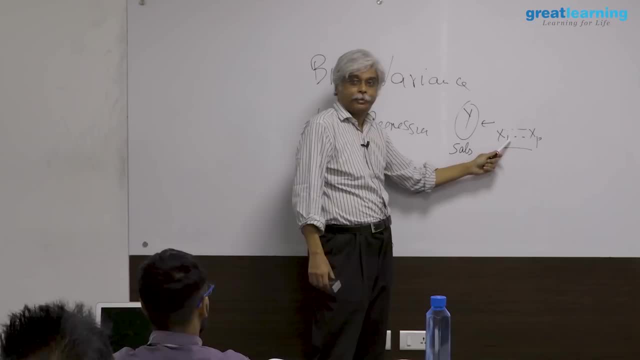 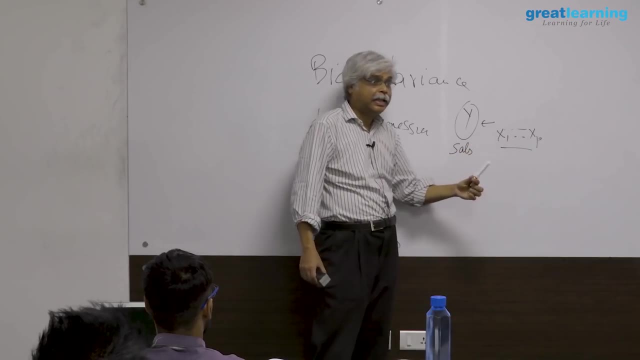 going to do is I'm going to take my data and I'm going to use it to generalize, so I'll take 30% of it out, pretend it doesn't exist, or 10% out, or whatever, and then predict it and then say that if a known part of the data can be predicted, 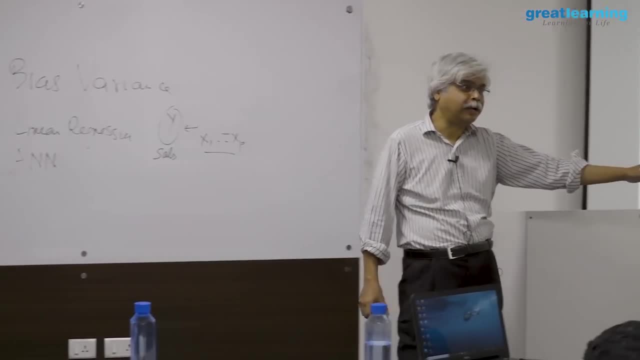 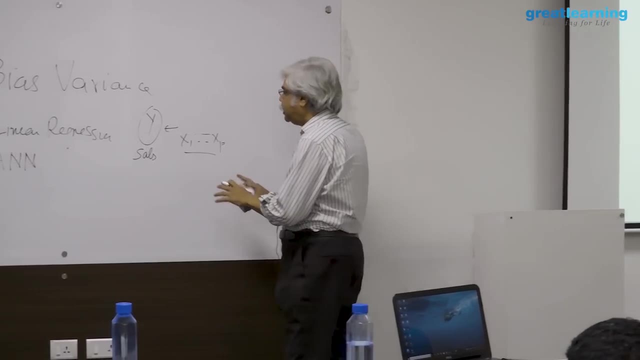 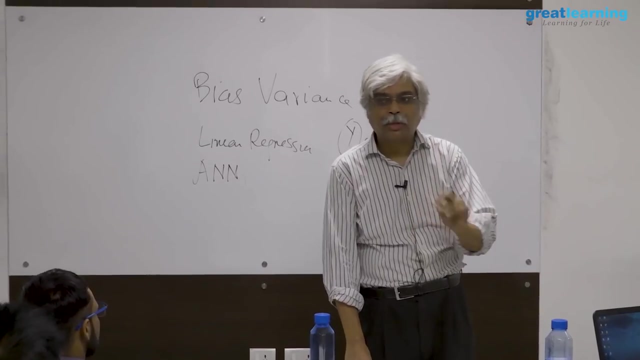 without the data. having seen it, then the unknown part of the data would- like I have hopes will be predicted. in other words, that's its purpose. now, how does a regression method or how does a statistical method deal with this problem of saying that it needs to work outside the data set that it is seeing? 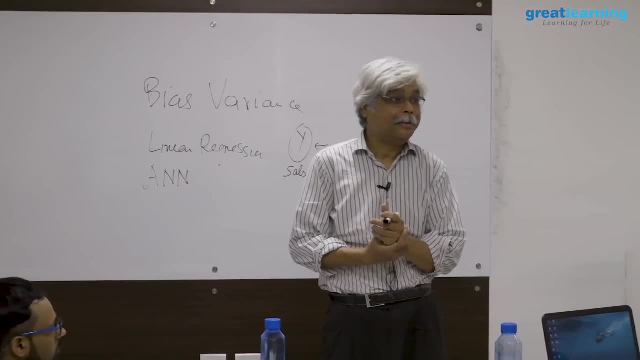 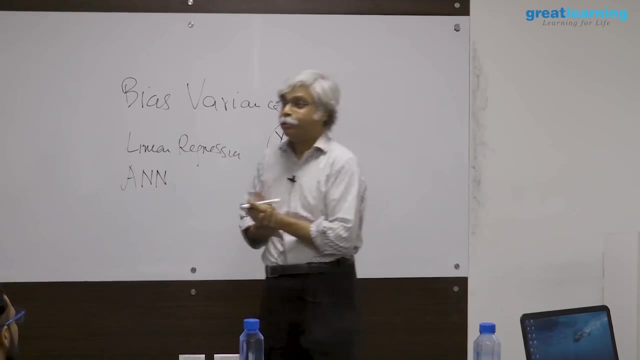 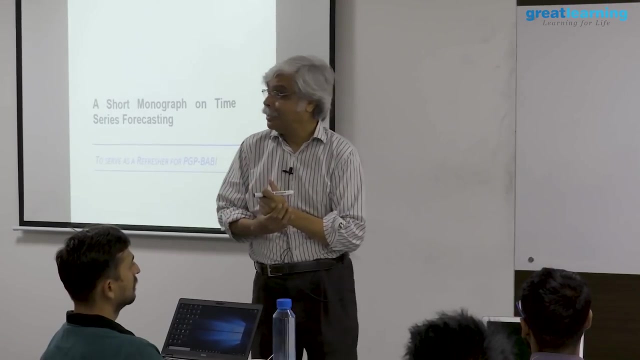 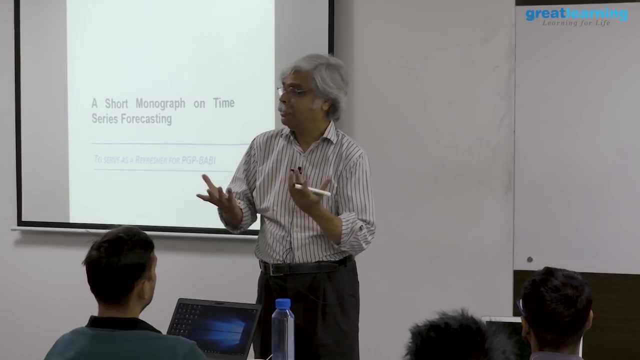 you, you do. did you do that in, say, say, ANOVA? did you do that in hypothesis testing? why not? if I'm analyzing data, I'm doing a hypothesis test. the same principle should apply, right? nobody cares about your data, they care about their data. so why? why wasn't it done there? it wasn't done there because the principle that is 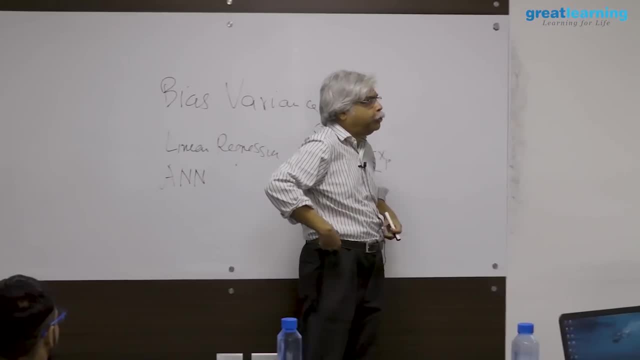 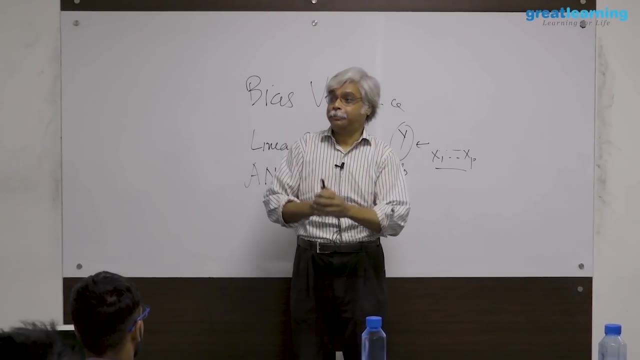 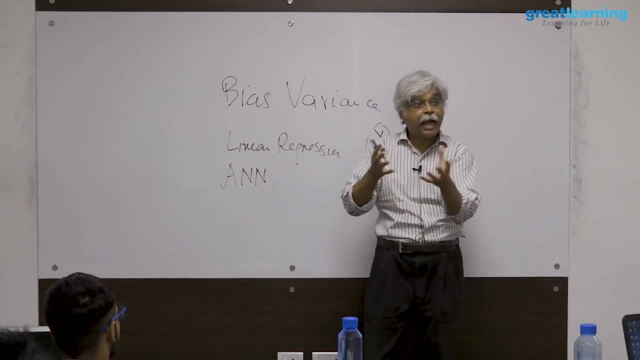 slightly different. the principle there says that, in order for it to work with your data, I am going to pretend that my data and your data have a common part. that common part is what we call the population. so you say there is a common population, from which I have a sample. 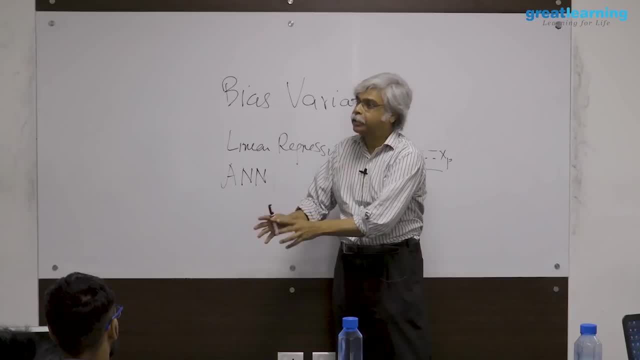 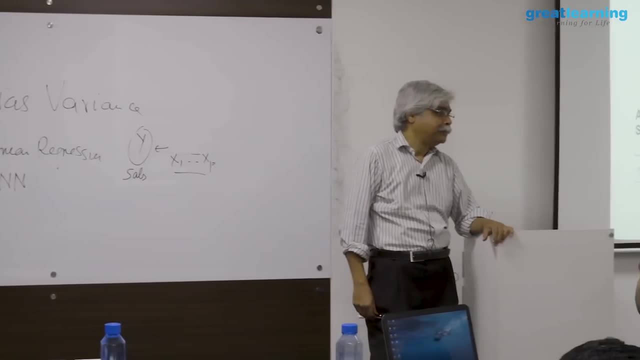 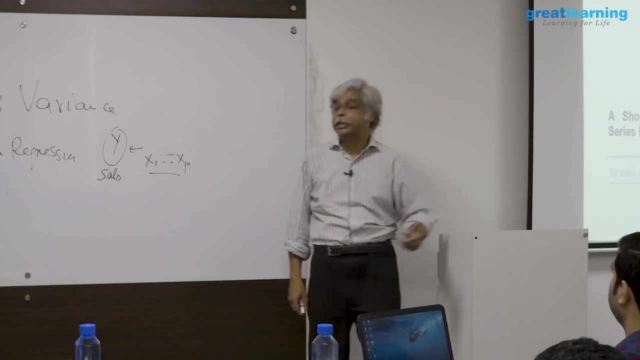 using my analysis, I will tell from my sample what it says about the population. that information you can now use for your purposes, which is a different idea. it's a different way of generalizing something, which is why, when you do statistics, you, you introduce the notion of a population. the population is the. 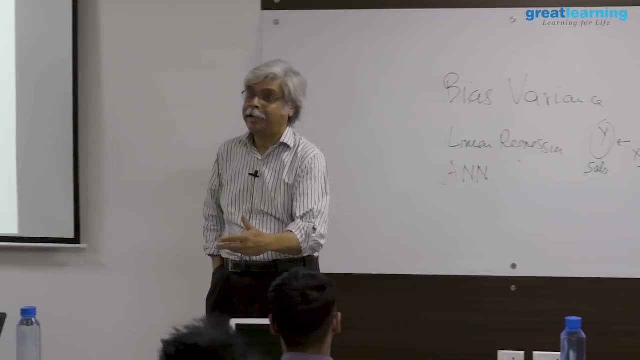 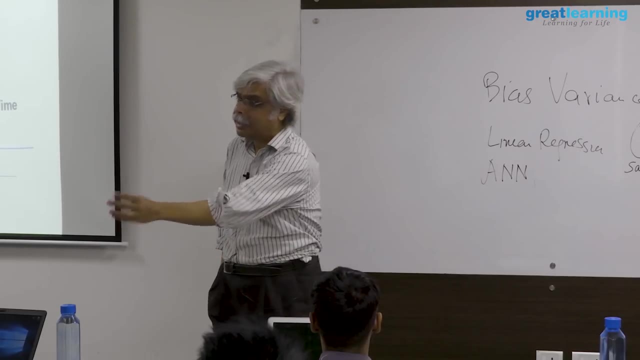 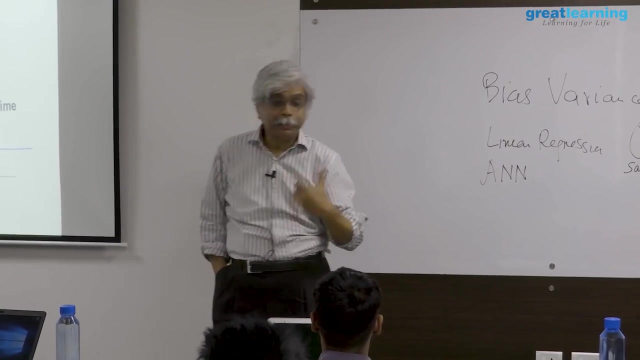 part that goes that that remains the same from data set to data set. it is the part that generalizes X bar, does not generalize mu does. X bar is a arithmetic calculation you are doing on your data set. that tells me nothing about my data set. what tells me something about my data set is the value. 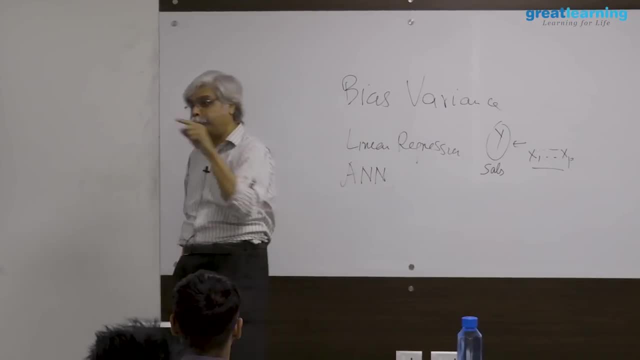 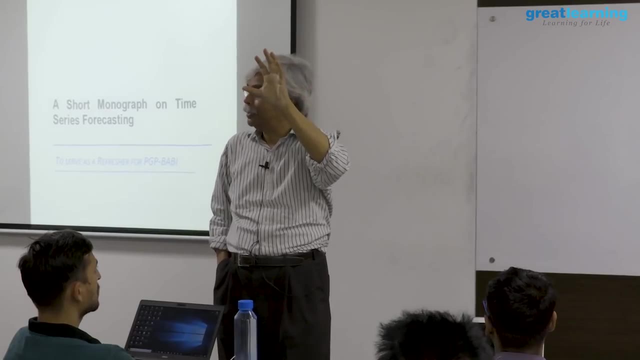 of mu, because the mu is the common to both of us. now the question becomes: what is your X bar? take, take about, tell about mu. from that I'll be able to say: therefore, if I see the mu, it is about this. hence you have to have standard errors, hence you have to have confidence intervals. 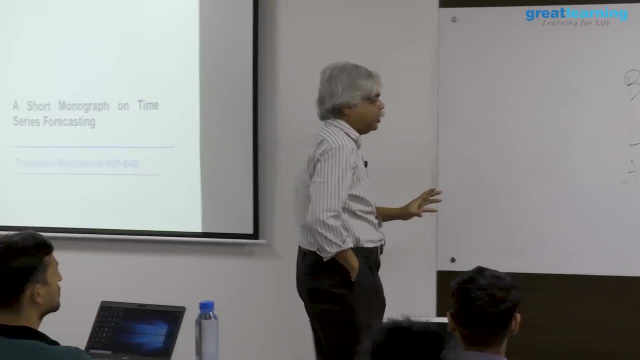 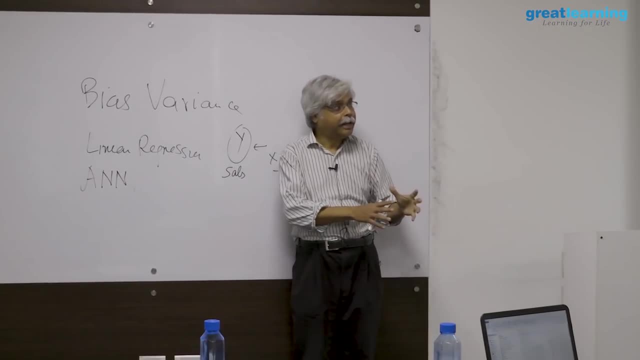 and things of that sort. so there are two tricks at play here. one is that one is a trick of out of sample learning, the test training idea that says that convince me by saying that it works out of the sample, and the other is the idea of a sample learning, of an ideal sample. I have a sample. I have an ideal sample. 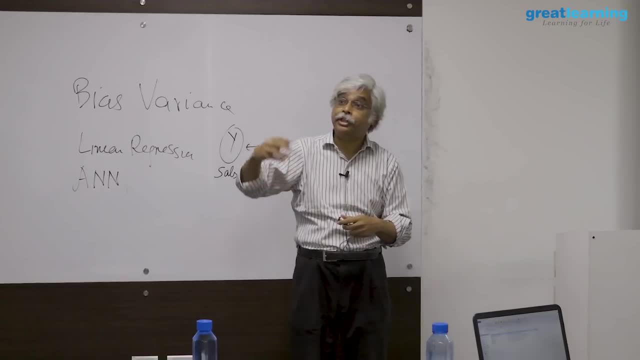 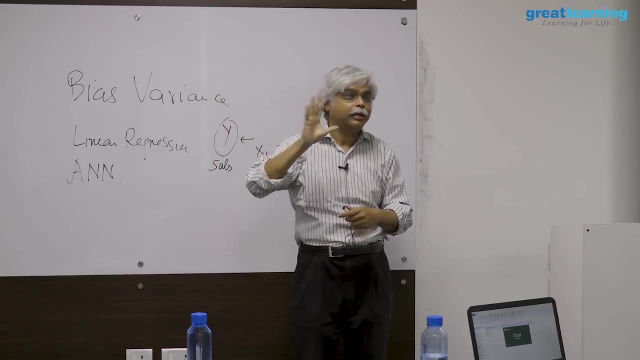 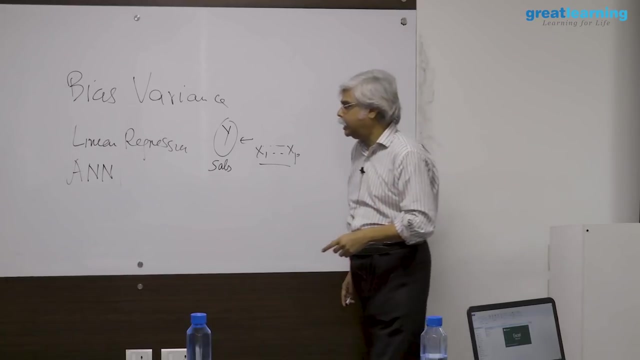 population, which is to say convince me by giving me an estimate of an unknown parameter, together with the uncertainty bars around it, and I'll be interested in that estimate. I'm not interested in your arithmetic number. so what we'll do for time series is that we'll take some of these ideas and we kind of extend them. 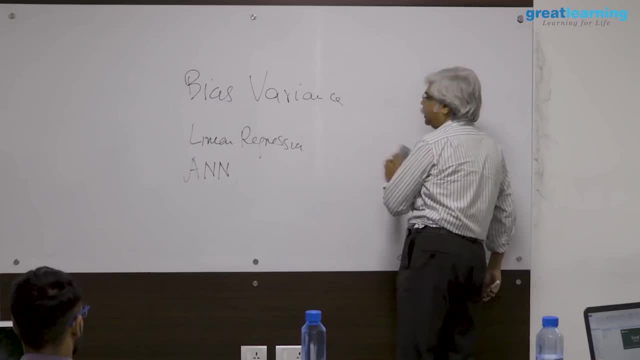 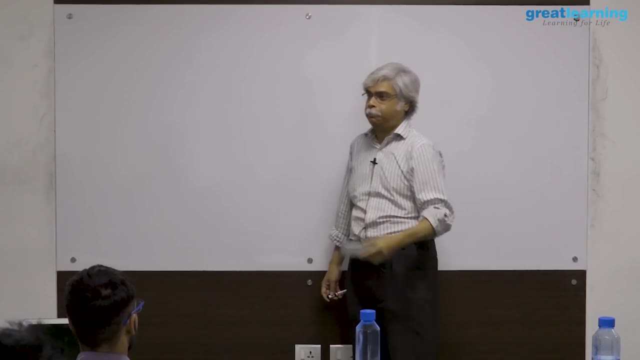 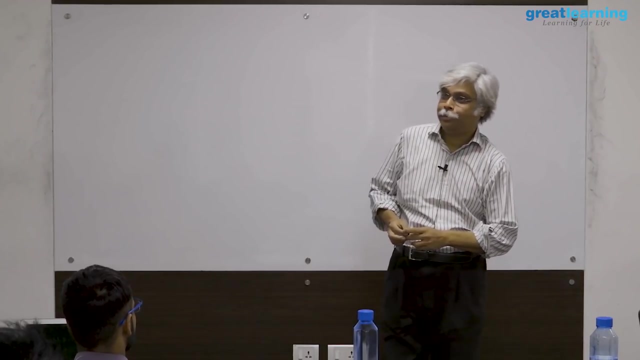 to a particular way of doing things, and that particular way of doing things says: is that. now I want to think of the problem of prediction in time. now, in English language, prediction and forecasting often mean the same thing in analytics. they don't. in analytics, prediction means what prediction means. 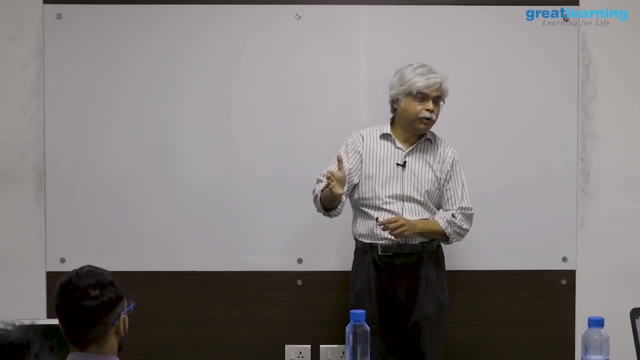 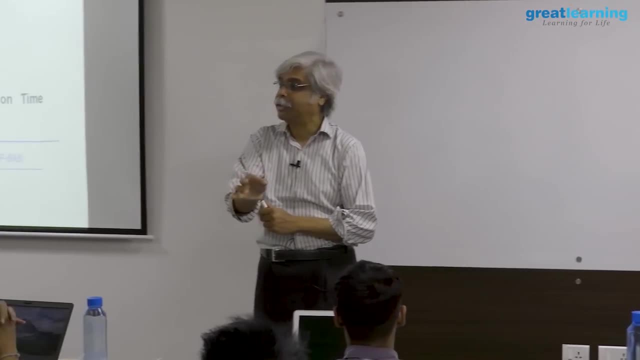 there's an equation of the type: Y is equal to FX. if I give you an X, predict the Y. forecasting means, if I've given you a series of observations- y1, y2, yn, tell me what yn plus 1 is and what yn plus 2 is. forecasting is about time. 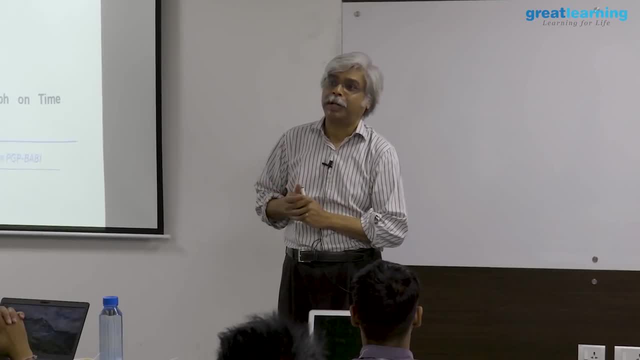 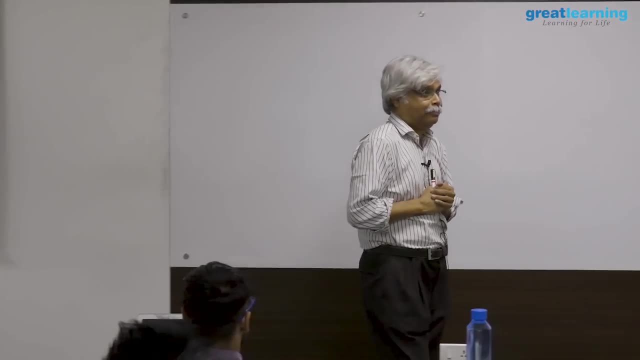 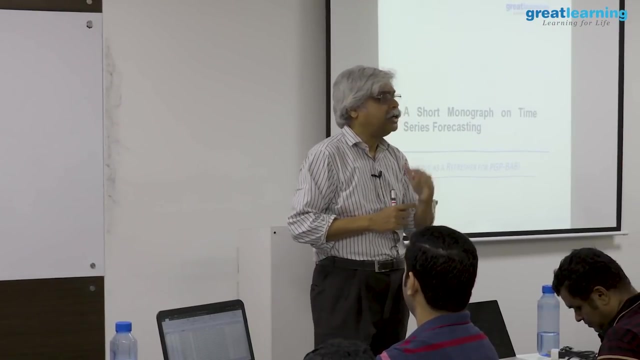 prediction may or may not be about time, and typically is not about time. so when people say predictive analytics, that doesn't necessarily mean that this time involved it could simply mean predict what will happen if my price goes down. forecasting is a little different. forecasting means tell me what my sales. 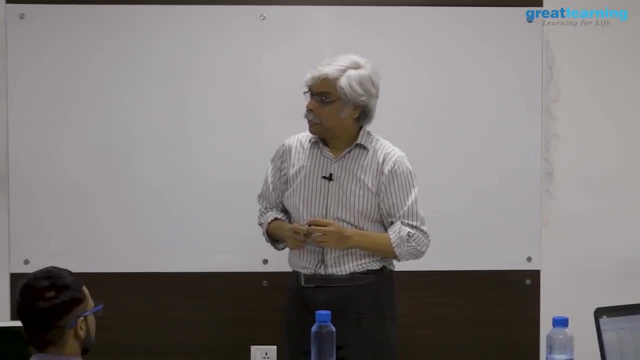 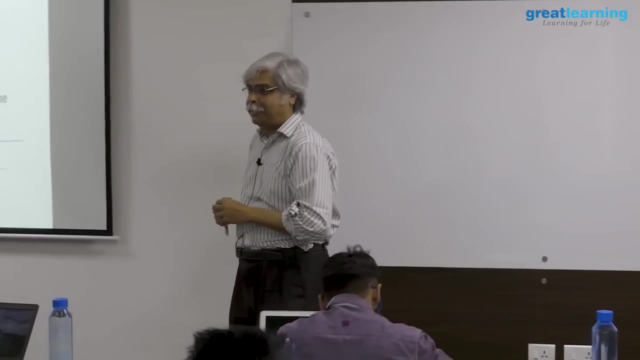 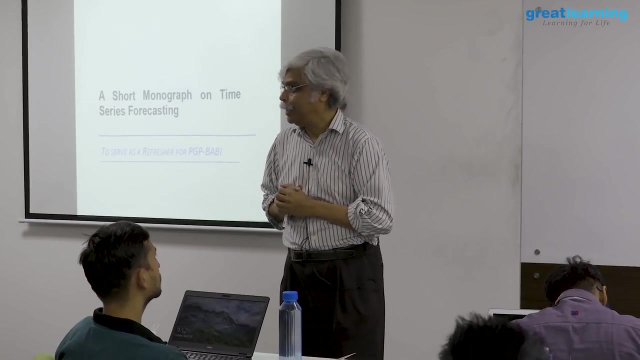 will be in the future. so the problem that we'll be dealing with today, tomorrow and the day after is the forecasting problem, not the prediction problem, and we'll be using prediction like methods to solve it. as you'll see, we'll borrow from the idea of regression to see how it works. 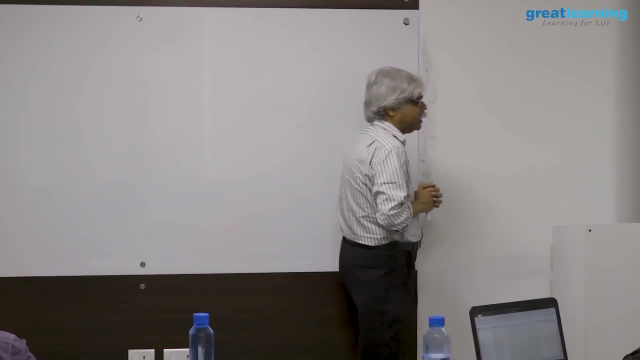 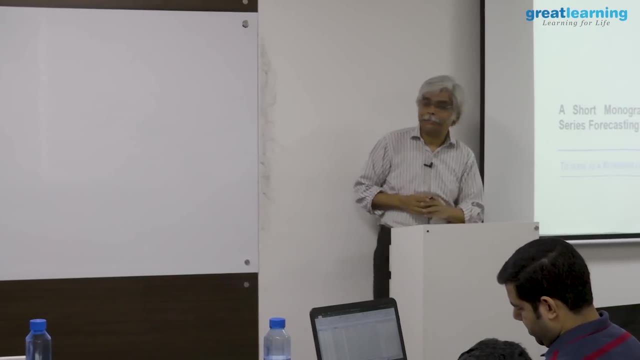 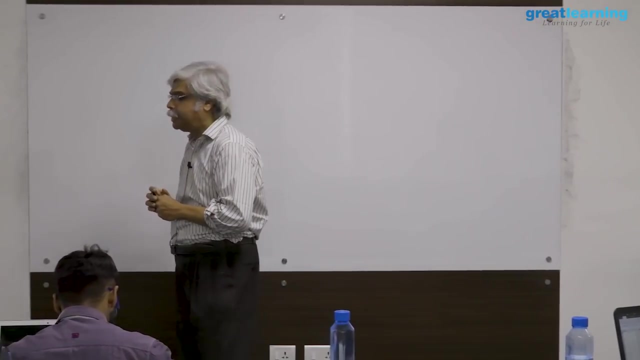 to see what kind of principles can be done. now there's a monograph that professor Basu, who teaches this course regularly and is sort of the standing faculty for this module, she, and certain members of the great learning staff have come up with this monograph. it's meant to tacware. according to some passeventi of analysis, gradin & cp1 follow up with this monograph. it's meant to some. 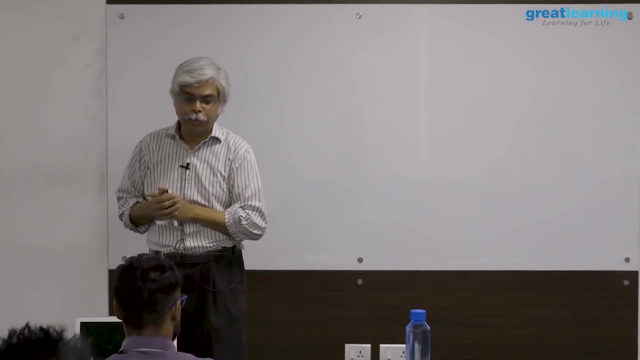 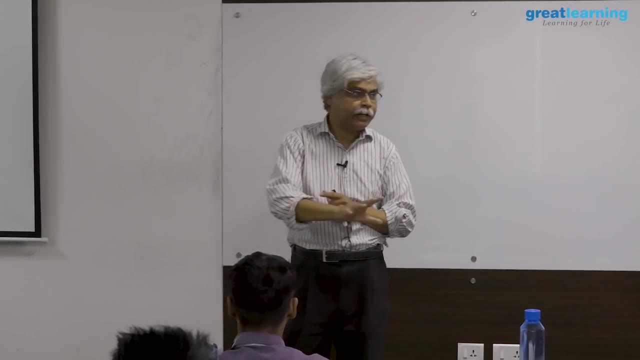 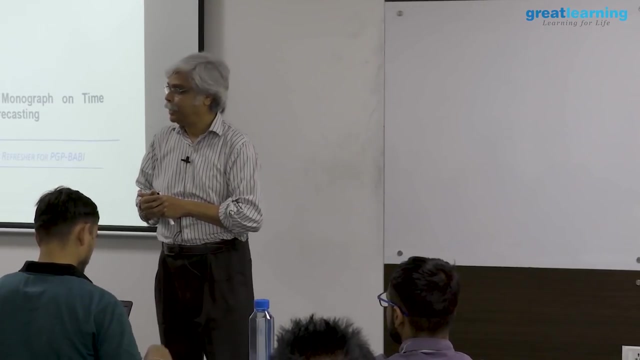 extent be a refresher, but we're going to use it as sort of the core material for the course. that should be available in your lms. there should be a data set also there, a tractor sales data set, which is sort of the the carrying example for this. it's an example that we kind of bring all 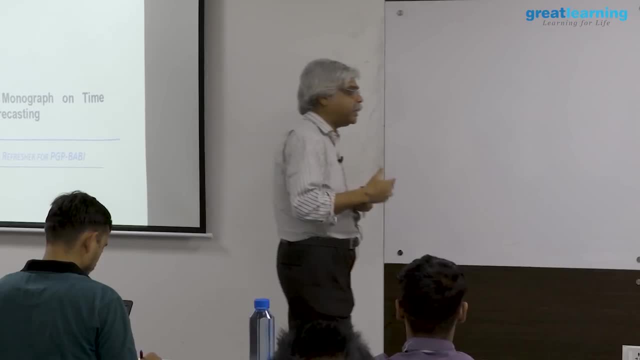 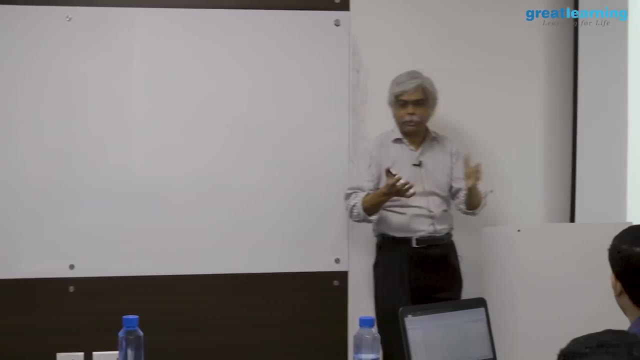 the juices out of, so, which means that, towards the end, we might need to take another example to see this. so what i'll request is that you download this file and the data that comes with it also on your machine, however you'd like to. however you'd like to access it, there are other data. 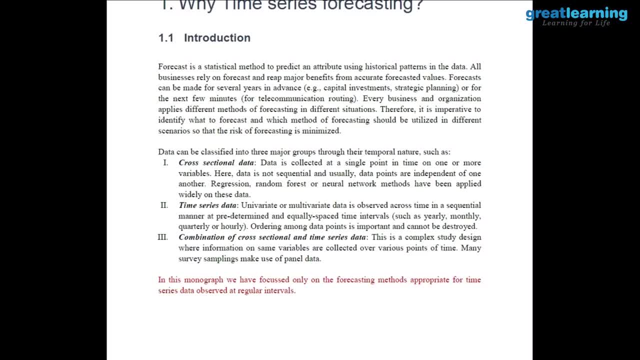 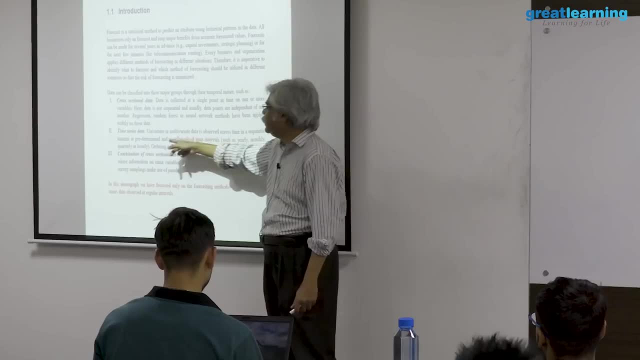 sets that we might load as time goes by. a little bit of an introduction to what this is, so i won't talk too much about this. i mean, it's fairly obvious. so a time series is a data in which the data is sequenced in time. it is observed in time in a sequential manner. 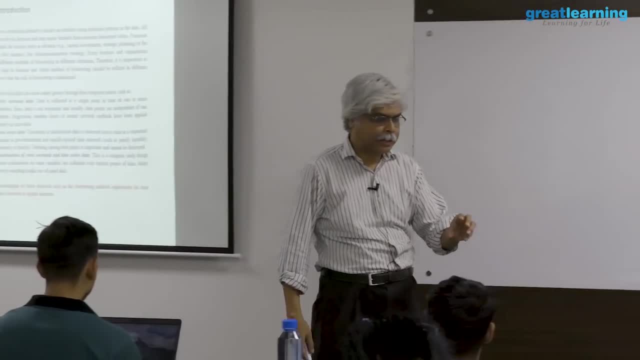 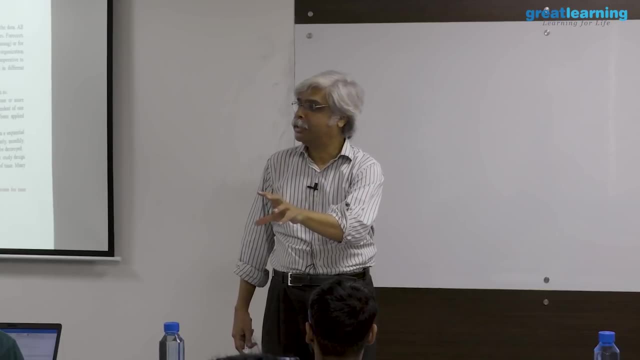 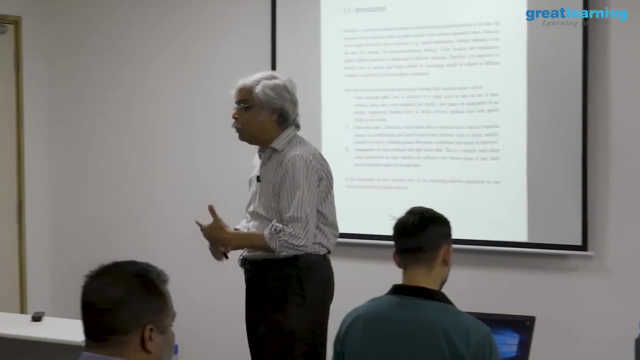 which means that the data arrives at you in a sense that this is before this. this is not true in a regression, a typical regression scenario, typical supervised learning scenario. in, say, a regression model, linear regression model, if the data comes to you in a different order, will you get the same answer? you'll get the same answer if the answer doesn't. 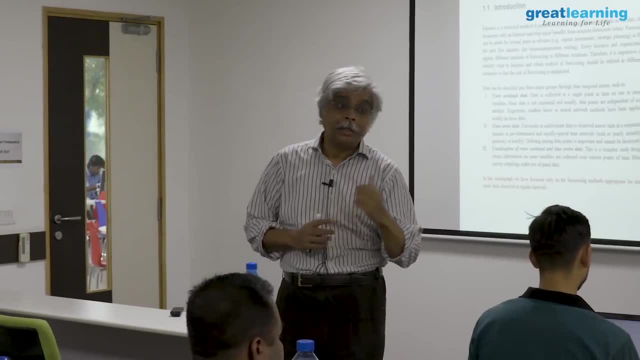 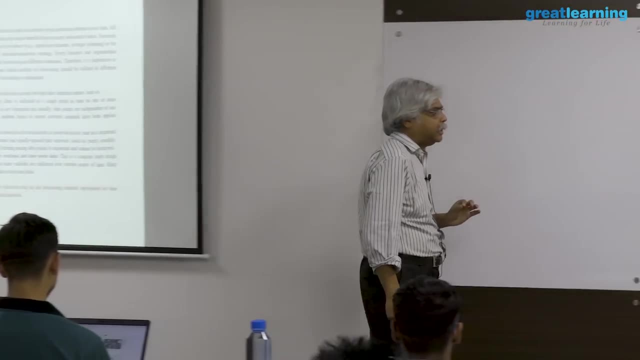 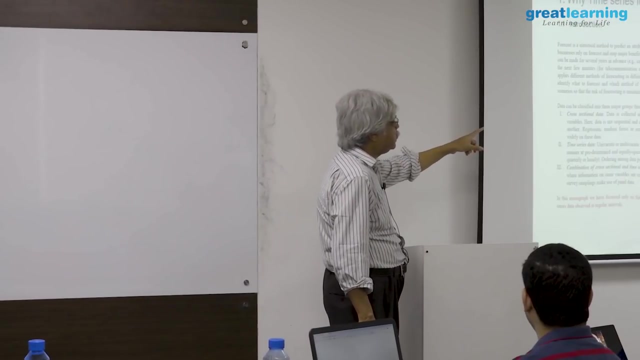 depend upon the order of the data. here it does, because the number is given to you in a certain specific sequence. now the sequence could be driven in hours, days, whatever it is, but that's the big difference now that does. that means sometimes that we often look at combinations of data that are of different. 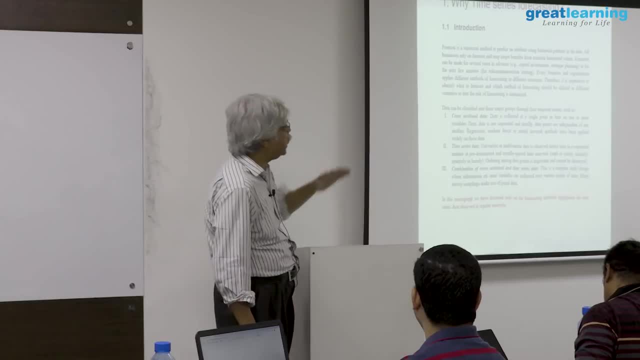 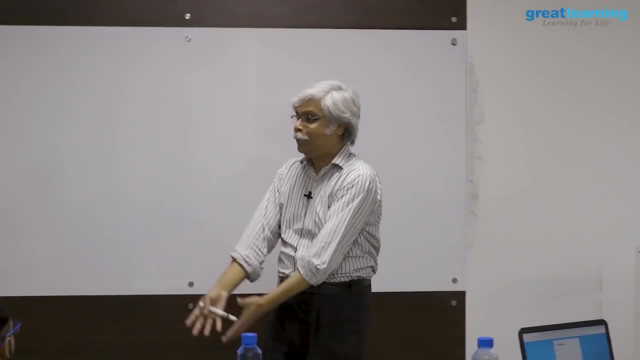 types. so, for example, it could contain data from different kinds of variables. in other words, a typical example of it would be: let's say that you're looking at stock prices. so you open a typical newspaper and you'll see lots and lots of stock prices. you can arrange those in time as well. 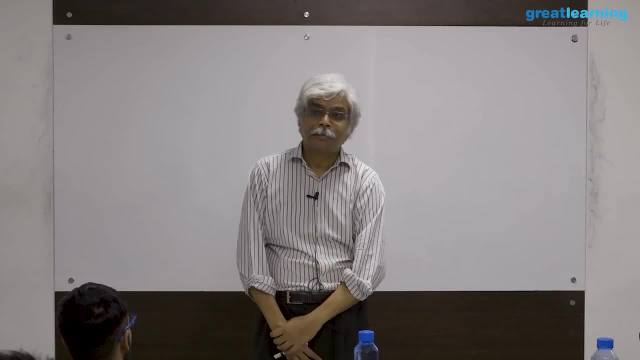 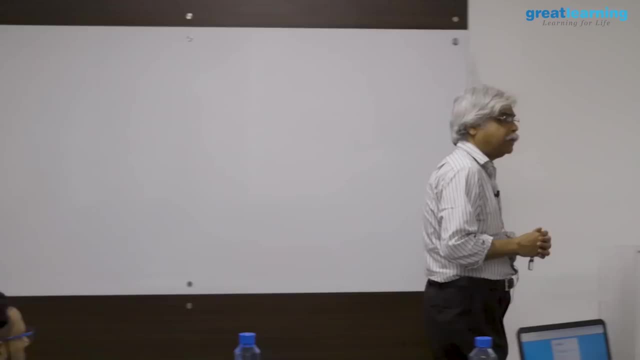 so you could look at, say, data from a bunch of stocks- let's say 50 stocks in the nifty- and you could follow them for a year. let's say you look at closing stock prices for a year- I don't know how many- that is say for weekdays, etc. you know 250 odd observations. 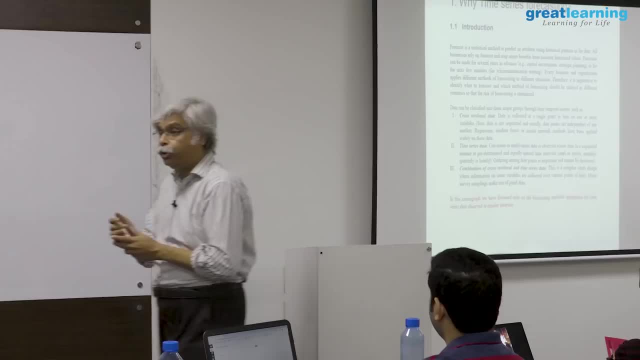 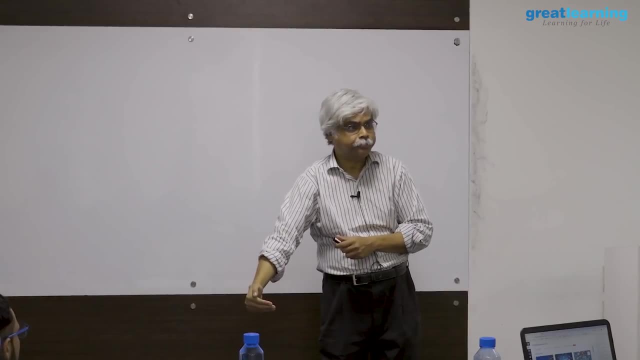 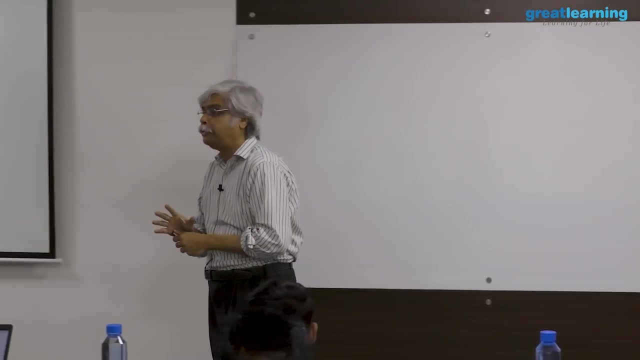 but you do it for about 30 to 50 stocks. now what do you see? you see a cross-section which is on a given day. you see all the stocks at the same time. you see a time series or, for example, you're seeing a video. if you are seeing a video, the cross-section version. 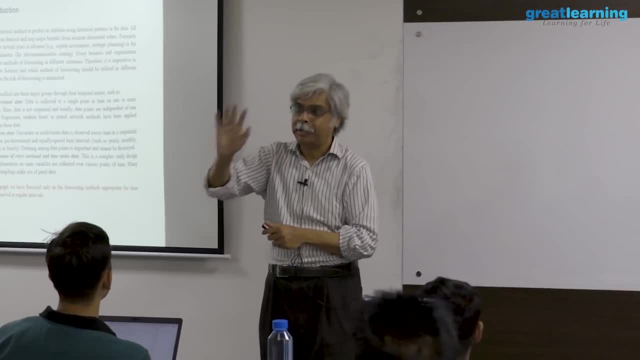 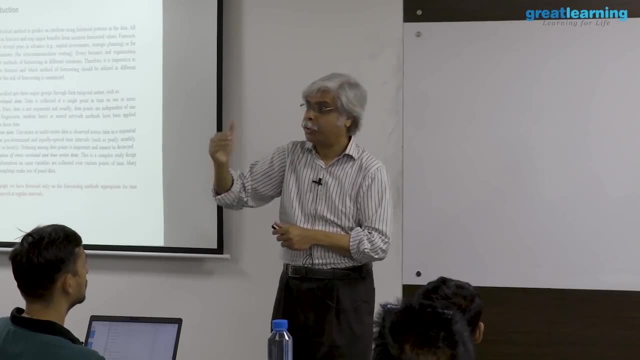 of the video is what the cross section version of the video is. at a given instant in time, there's a frame, so an image is the cross-section version of it. now, what's the time series version of it? the time series version of it is in time. there is a lots and lots of. 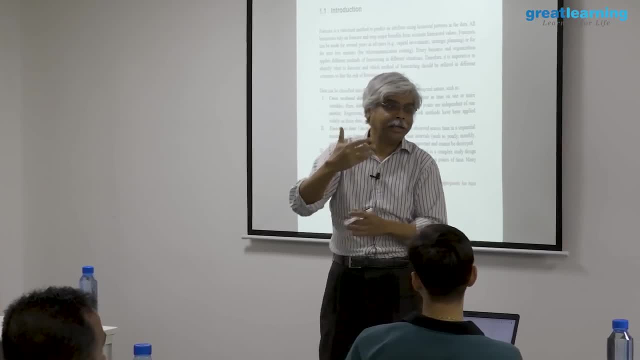 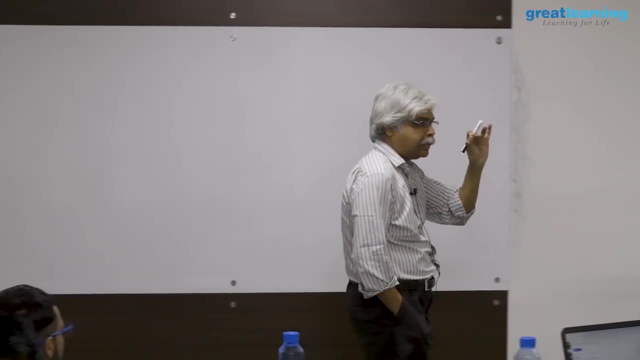 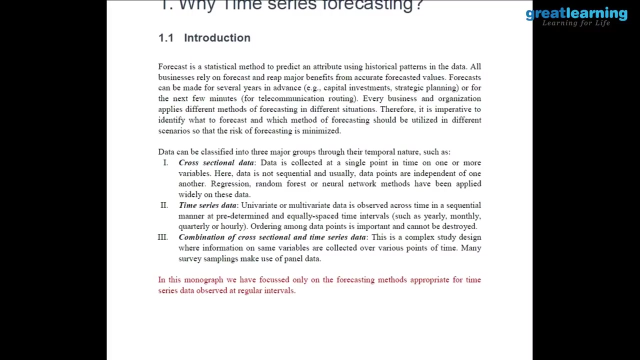 images that are running off one after the other, and in your eye they're rolling into into a movie. so, for example, if you look at, let's say, the, the technology of the, of the technology of the, of the software, how is that displaying this? that's displaying this, for example, pixel by pixel of voxel, by: 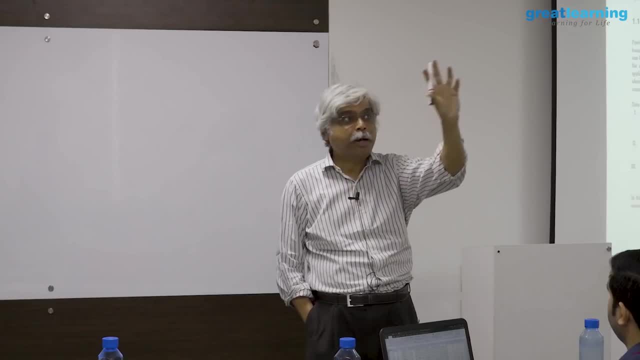 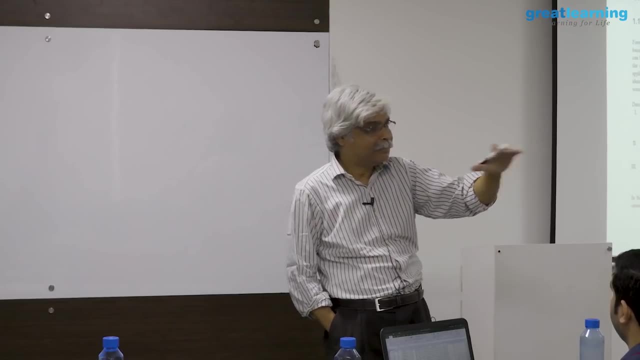 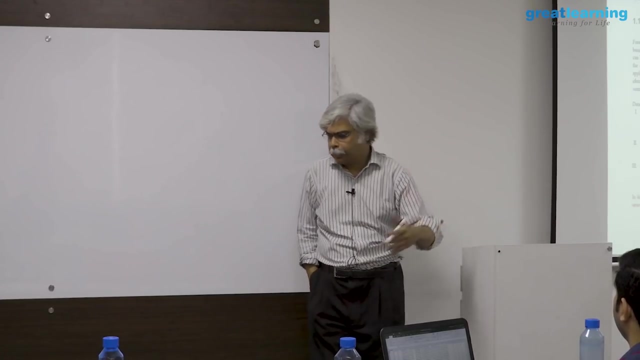 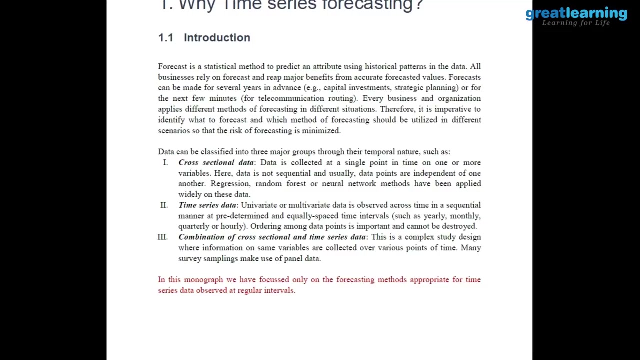 voxel, which means in a particular part, you're seeing one particular part of that video, but you're seeing it across time. so it's a combination of something cross-sectional and something time series, which is what a lot of data comes as data. that is, for example, sales data, data on you know your metabolism, your. 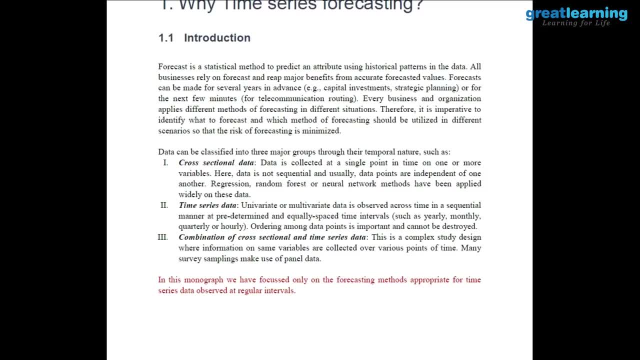 blood pressure, other records that you have. so full-blown time series data usually consists of both a time component as well as a series of variables that are at a given instant in time. at this point, I will say that in this monograph or in this series, we shall not be talking. 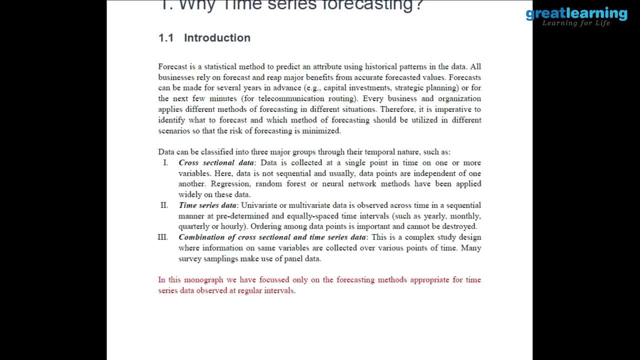 about cross-sectional data at all. the cross-sectional data part is something that you're already doing and towards the end, we might say that here's how you will combine these two ideas: the idea of variables being static in time, and then moving that across what we will be focusing on. 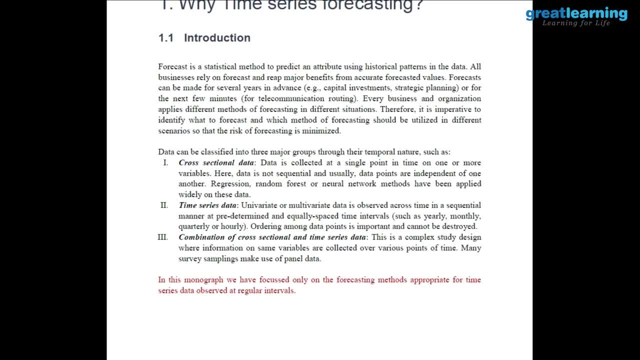 is only the time series component, so we'll be looking only at things that are moving in time. in particular, we'll be looking at only one series. so if you're looking at stock prices, only one stock price. if you're looking at sales, only one column of sales numbers. that's it. as I said, in the world out there, the data, 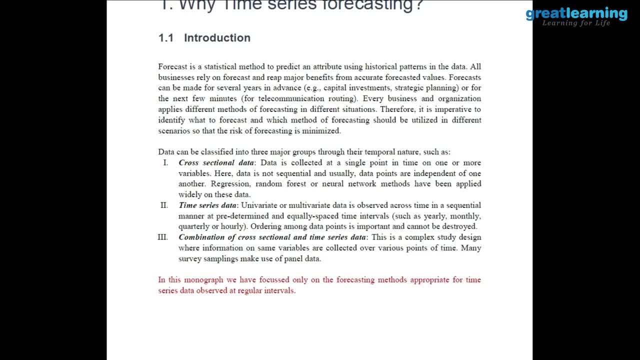 could come in many things. if you're looking at tractor sales, you're not just looking at tractor sales. you're looking at, for example, prices of tractors. you're looking at, say, competitor sales of tractors. you're looking at some kind of agricultural produce or whatever the tractor is used. 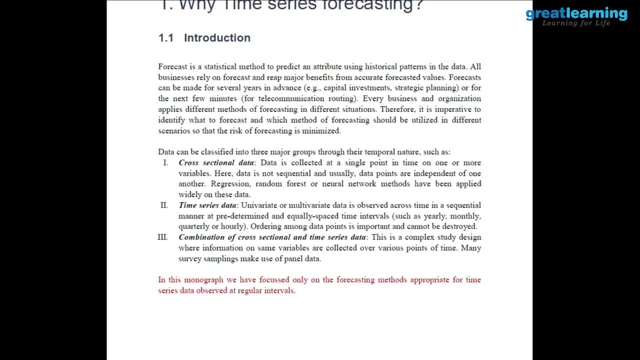 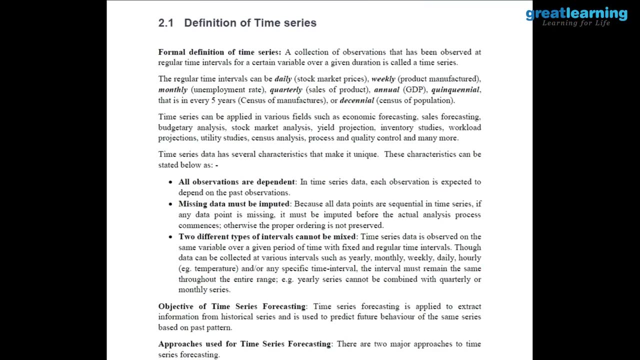 for maybe you're looking at fuel prices, right, maybe you're looking for prices of inputs, making those chapters, you could be looking at a number of things, but we'll simplify things and we look only at one series of numbers, only at one series of numbers. so, for example, you could be seeing data. 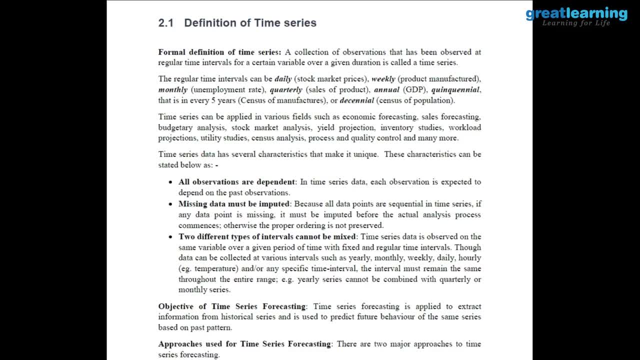 at different forms of what that series is. you could be seeing, for example, things that are oh, I don't know daily, like I was giving example, the stock market prices, weekly, things that are products that are manufactured monthly, let's say, an unemployment rate. some of these things are easy, some of these things are hard. 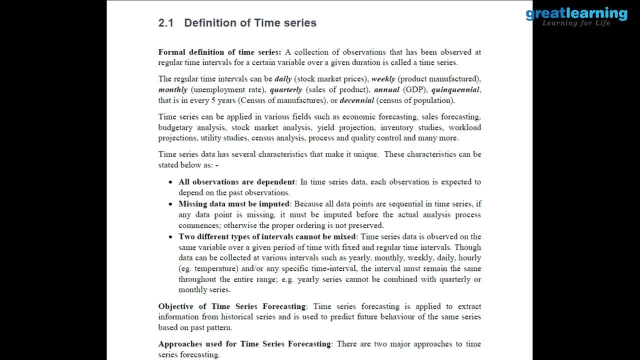 quarterly, quarterly sales of a product, annual gross domestic product of a country, census which are at more than one annual things. some of these are very easy to capture, some of these are automatically captured and some of these are not so very easy to capture. some of these are automatically captured. 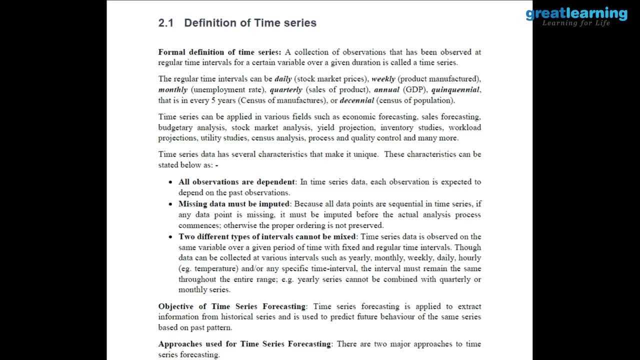 stock market prices are automatically captured. software in stock market exchanges are designed to generate that. you go to capital online, which is a website. the data is available to you. some of these are not so easy. so, for example, unemployment rate. the whole country is very bothered that we can't. 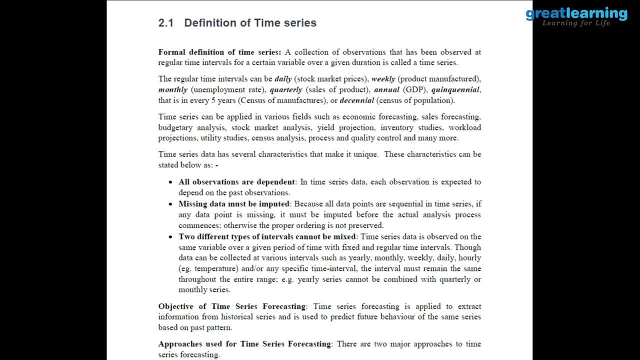 measure unemployment- not an easy thing to measure, depending on your definition of who is unemployed and what not. so some of these are definitionally issues like: how do you define an employment person, who is unemployed, who is unemployed? how would you if your analytics professionals or you're going 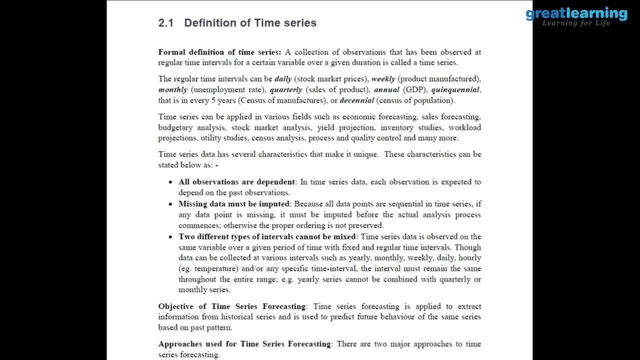 to be analytics professionals, or you are. if you are asked to calculate an unemployment rate, how would you go about doing it? salary purposes, so anyone who has a salary is employed. so someone who doesn't have a salary is unemployed. so if you haven't received a salary, 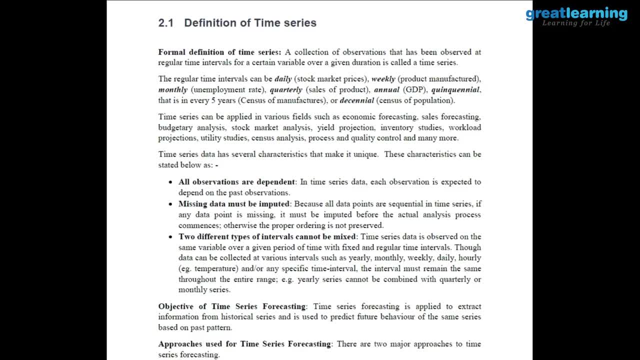 in three months. you're unemployed, salary lesser than so. here's a point. he has a. we don't knock it. so what would be your definition? my daughter is six and a half years old. right, we're trying to teach her money and we are giving her an. 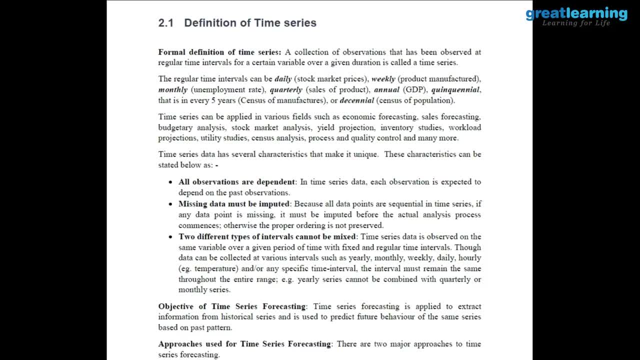 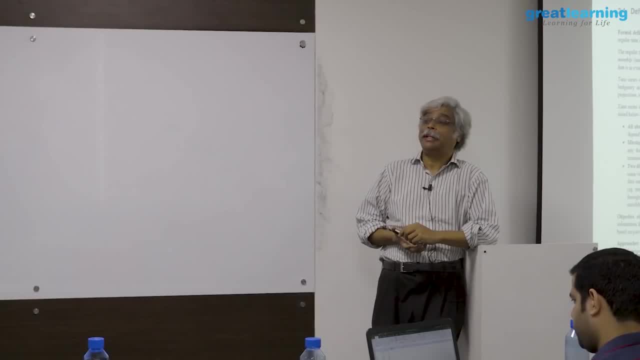 allowance of a budget of you know, five rupees every time we go shopping. so you decide what you want to buy. five rupee budget if you don't want to spend. if you don't want to spend the money, cool, you get it next week as well. rollover. 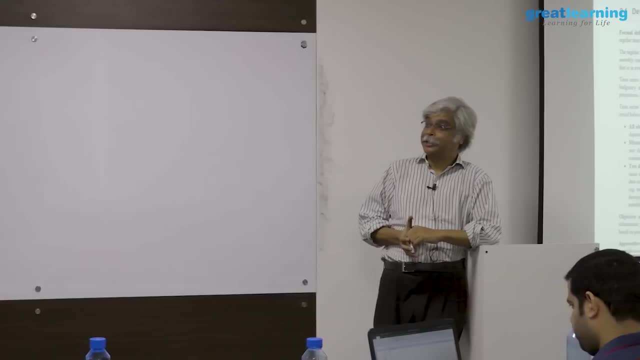 you want to buy something that's a thirty rupees, sixty rupees, etc. you've seen a nice little eraser or a toffee, etc. you figure out how many months or how many weeks you're not going to buy anything. you figure this out, right, she's. 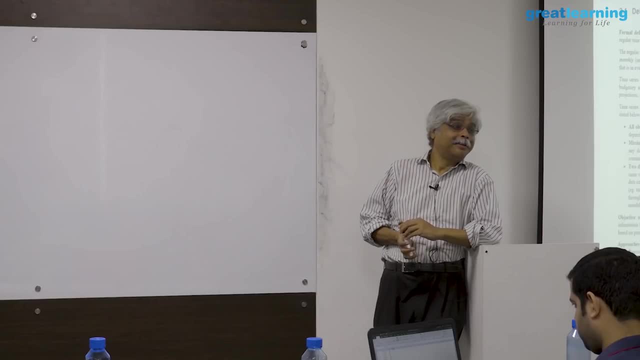 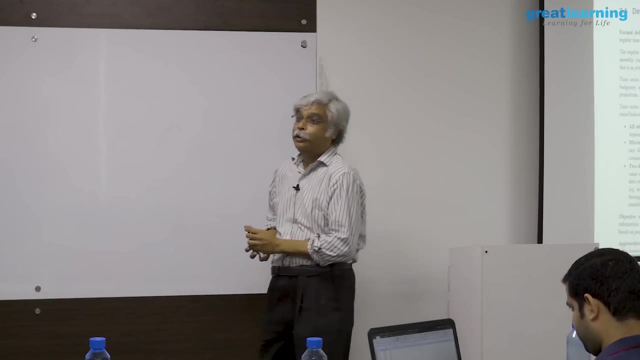 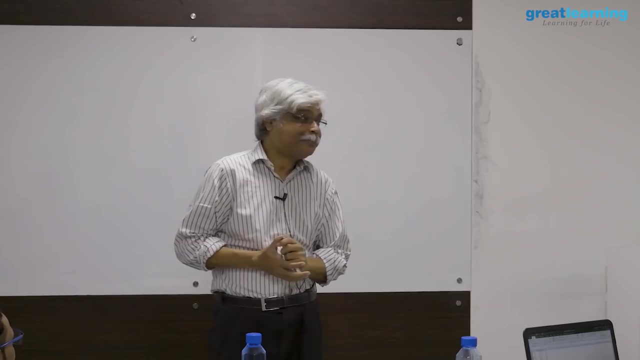 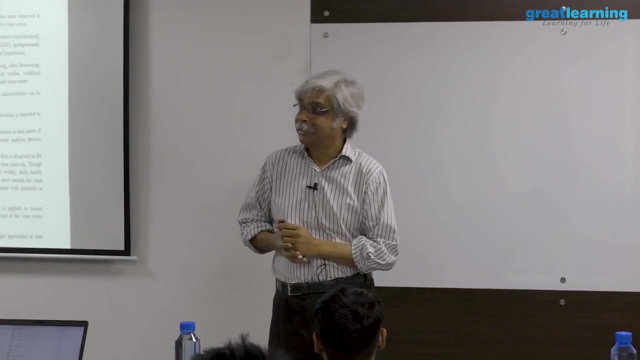 unemployed or employed? does she have an income? five rupees she employed. if you're calculating the unemployment rate of the of the country, where does she fall? things aren't that easy and serious people- people a lot more serious than you and me- haven't got this, gotten this right, so we're not going to get this right in this, in this class. my 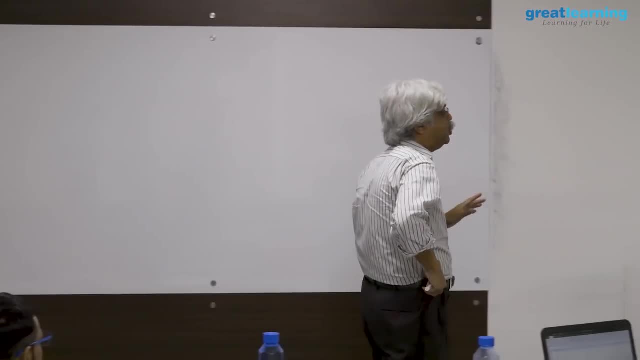 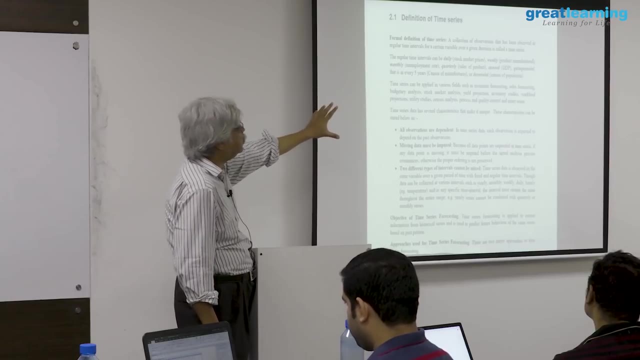 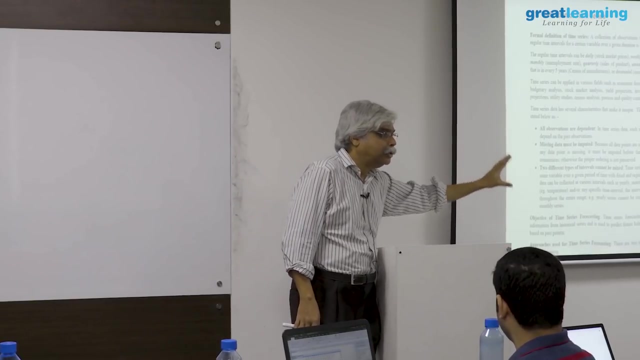 point being that there are some of these are very, very serious definitional issues. once those definition issues have been sorted out and you understand what this is, even for things that are in a business context, not just an economics context- sales of a product, right sales of a product- you know how to do that. 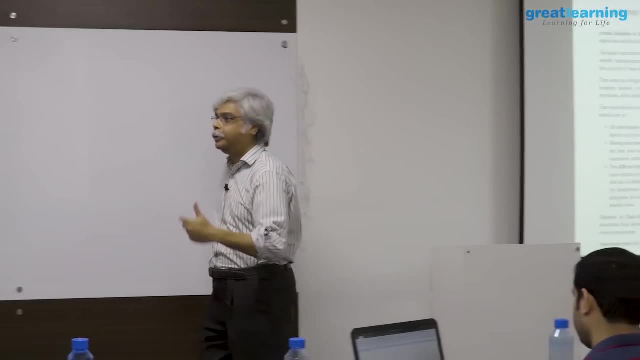 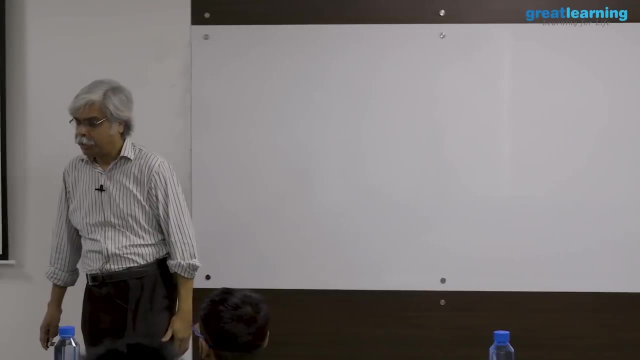 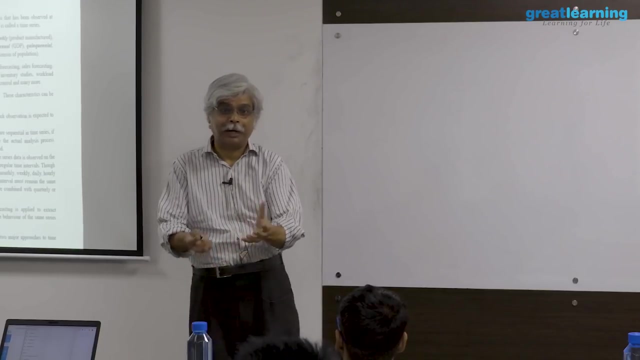 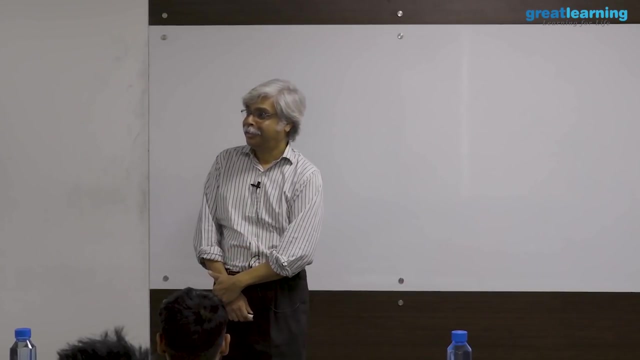 correct. let's say that you bought a house and you have what it using alone, correct? has it sale happened from the from the builders, first strength to the sailors? have, because the builder has received the money from the from the bank. from your perspective, as it happened, well, 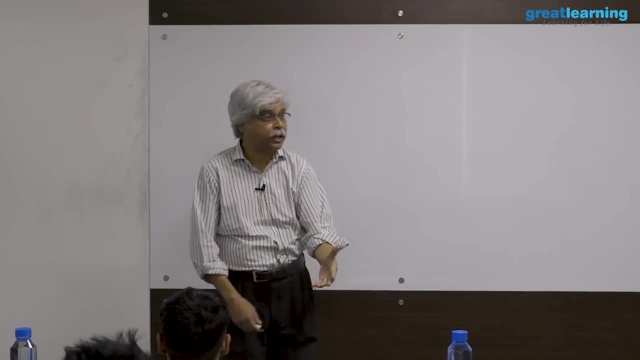 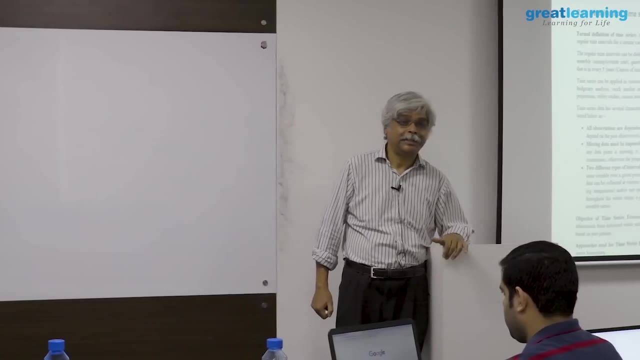 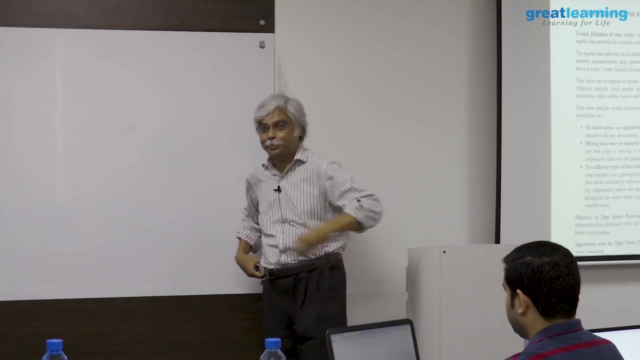 you're living in the house or in the apartment. presumably it has happened, or so. when do you account for us? when do you account for sales? any charred accountants here, accountant types? no, all right one. so how do you account for a sales? what if you're doing a bill of accounts for a company? when do you say? 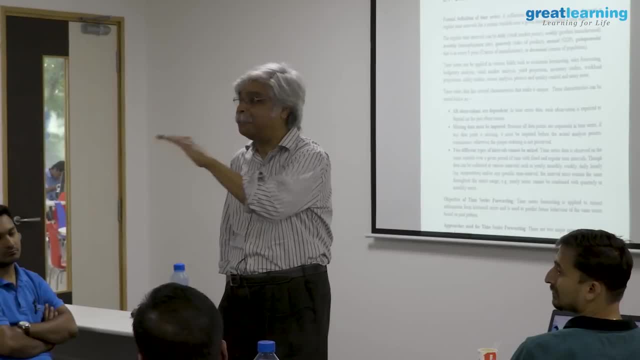 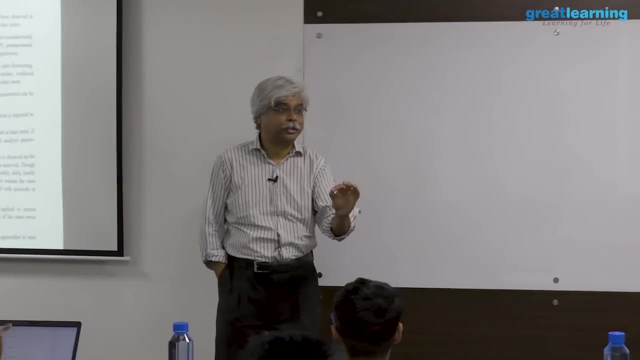 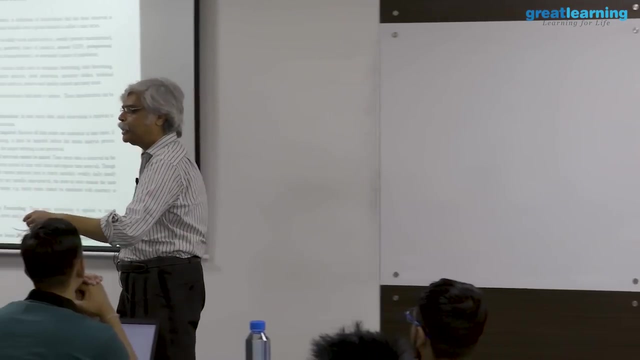 the sales has happened, at least always. so you've got some metrics that says that some something has to happen. so yes, it's also tricky sometimes- is defined as saying that the the product has to begin use in some way. that at least has to happen. then certain things has it been, so to speak, hasn't been delivered, so for 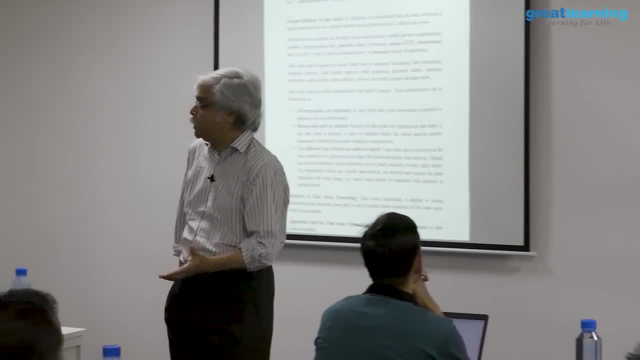 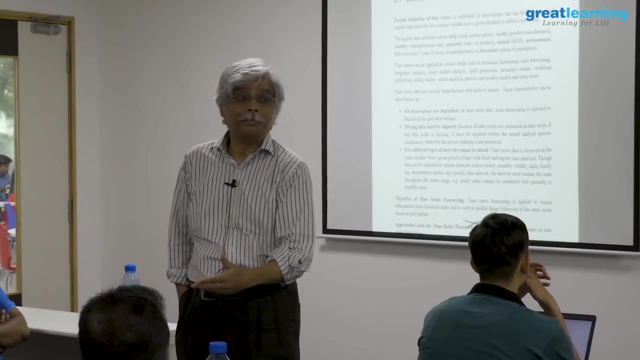 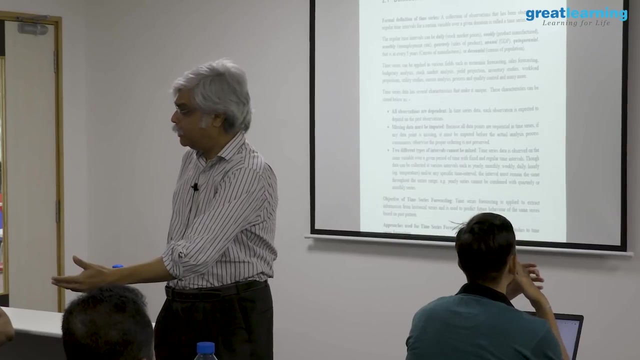 example, sales of a service. if you are, say, an IT service professional, has that sale happened? you're going to billable hours. how much have you sold? you've got a contract. that contract stipulates, say, two years of service. you have done say two months. you're built for two months. you've gotten. 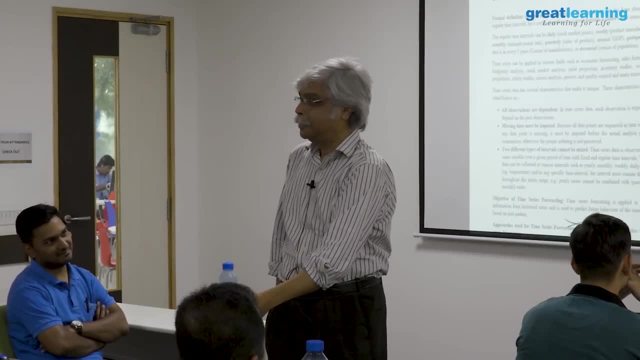 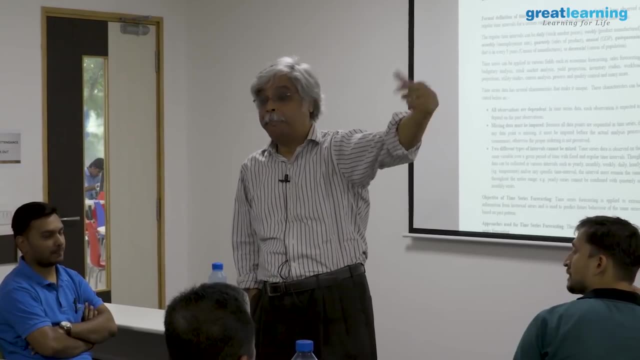 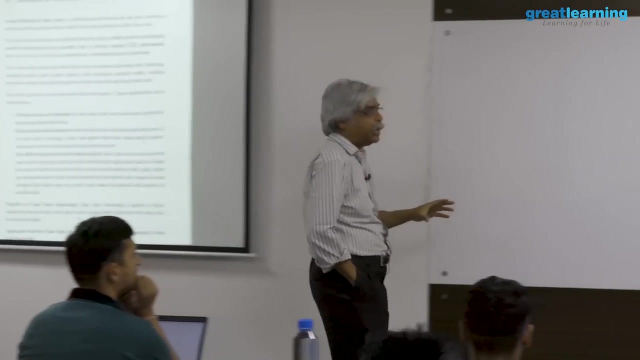 paid for two months, you've gotten paid for two months. you've gotten paid for two months. what got sold for two months only. you could argue that. but the contract, so to speak, or the pure whatever you want to call it, is for, let's say, two month period. so these are hard and very often what we often do in. 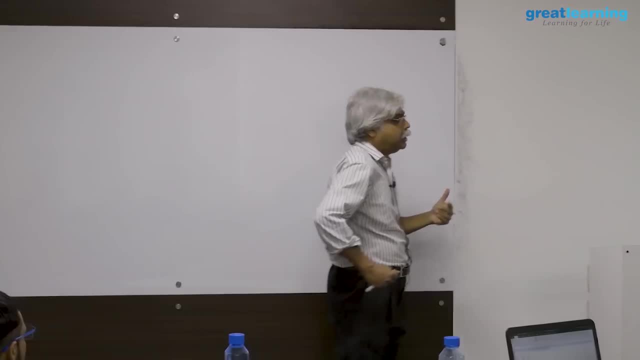 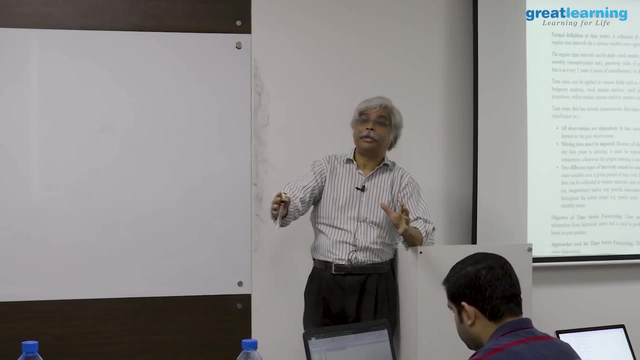 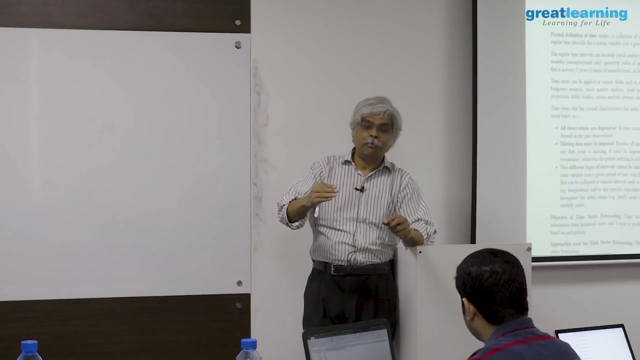 business, we, we resort to, in some way, management of that number in order to ensure that they conform to certain guidelines and certain metrics. otherwise, what happens is that you, you, you, you end up moving numbers around in order to meet certain business metrics. when do I account for the sale? how much do I depreciate on a product? how much do? 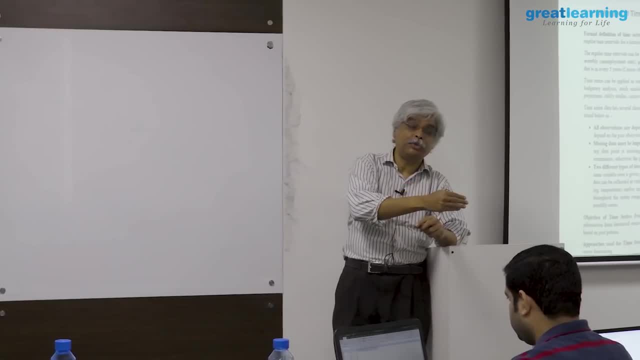 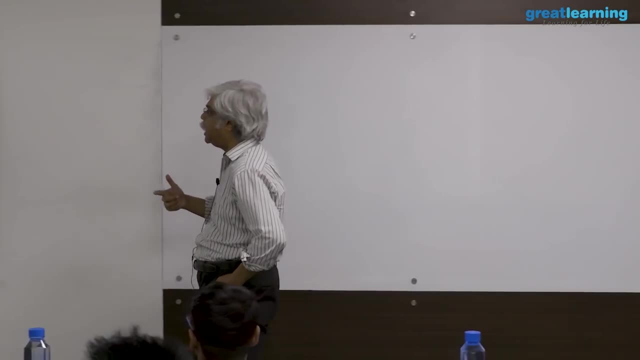 I keep on the books. how much do I keep off the books, so to speak? in other words, how much is future earnings, how much is all of that? so whenever you see a time series, there is this issue at the back of your head that says that where is this number coming from and what does it exactly mean? 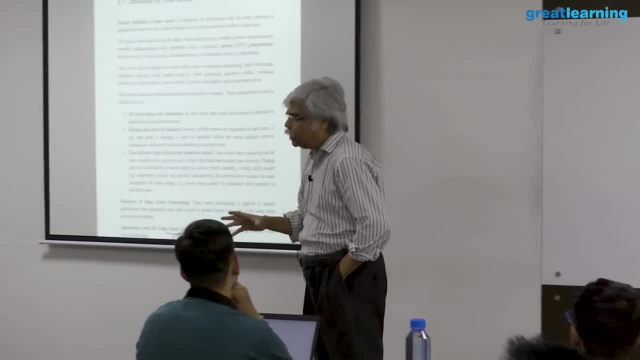 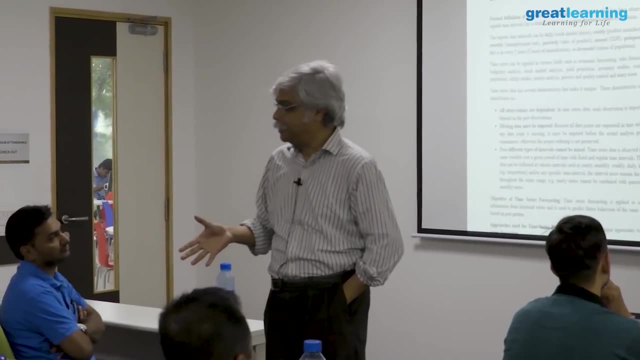 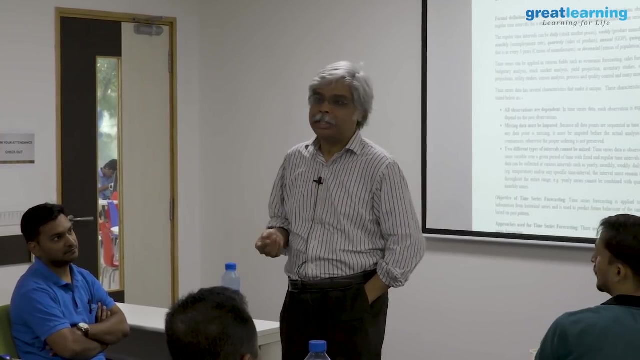 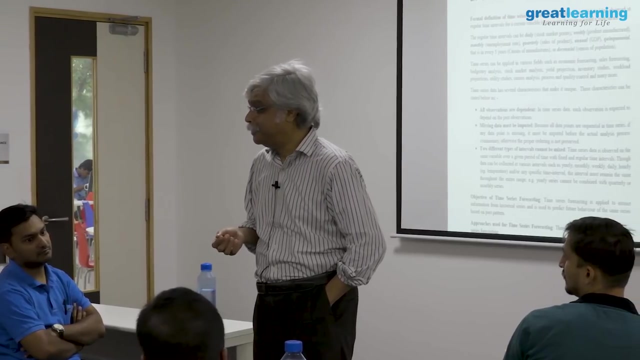 mean and how should I use it? it's not really important for the analytics itself, but it's important for understanding what the number means. for example, the census. what is the census? how often do we do the census? ten years? what question does it answer? population of what? India? when, when the census was? taken. how long does it take to do the census? one year. so it takes one year to do the census. what population is it measuring? little definitional issues here, right? so the census is designed to say that at, for example, they say the 31st December of 2001 or 2011 or somewhere. there is an estimate of the exact number. 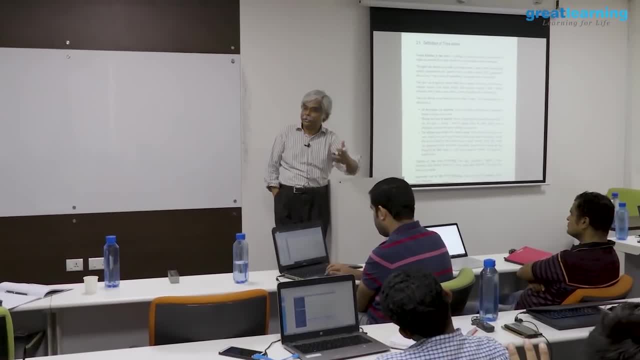 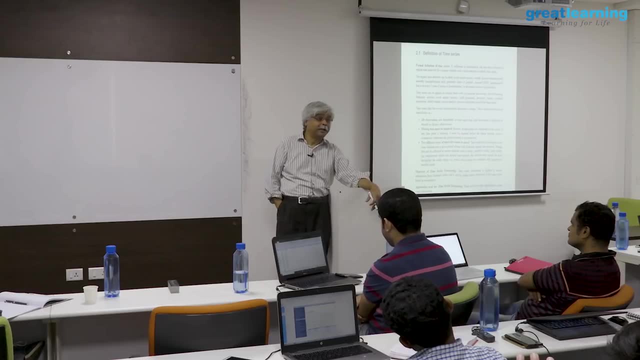 of people. that's there and if you see the census numbers, then you can- you know, these days, Google for it. I suppose you know these days, Google for it. I suppose it'll give you a number up to the nearest digits. this is the population of India up to the nearest person. it's not a round-off. now the population is it. obviously that the population is variable. it changes second by second. people are being born and people die in this country constantly, but you still need a definition to say that this is what the definition of the census is at 10 years. this is what the population of India is, so in the middle. 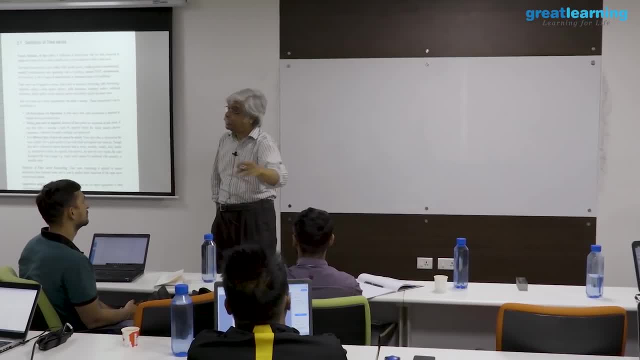 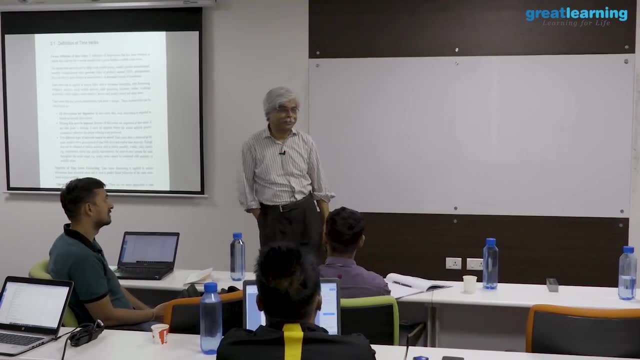 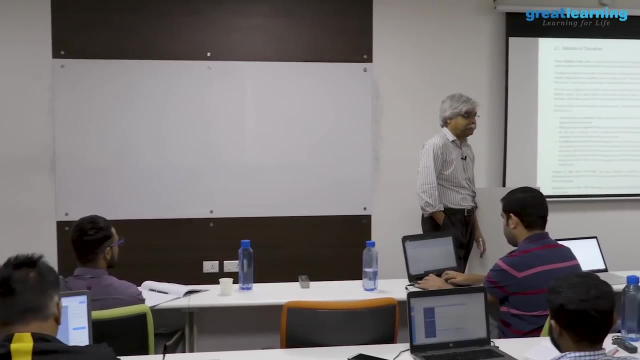 of, say, 2014 or 15. I will tell you to the nearest person what the population of India was at the end of 2011, which is a reasonable calculation to try and do. if I ask for what is the population today, that's a much harder question. and if I ask for the questions, and you can and you. 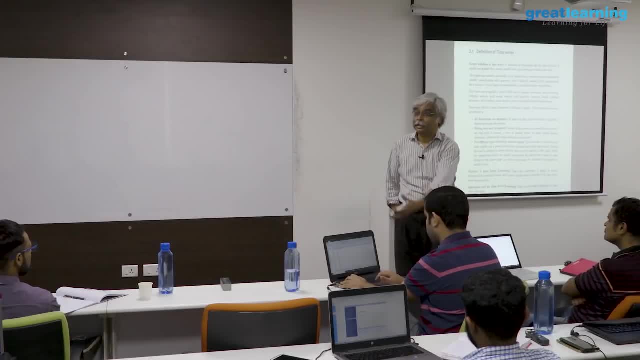 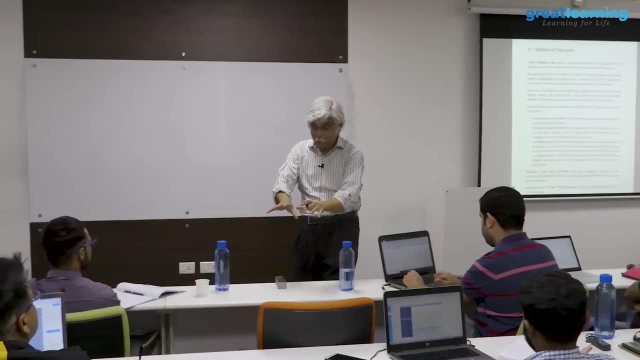 can look for that so you can say what is the population of India, what is the population of the world? there's a site that gives you that and that last digit keeps moving. it will constantly change because, naturally, you are staring at it right. as you're staring at it, the population of the world is is changing. 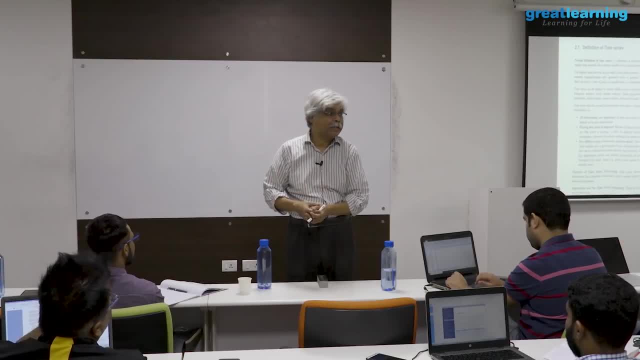 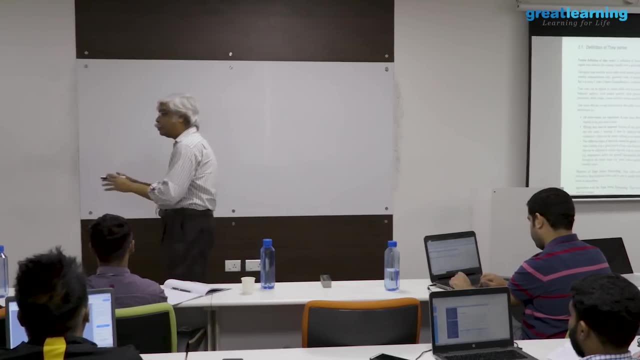 increasing up and down is, by and large, generally increasing. the number of people born every second is a little more than the number of people who are dying every second. and now let's suppose that I ask you a question. so what is going to be the? what is the projection of the population of the world, or the? 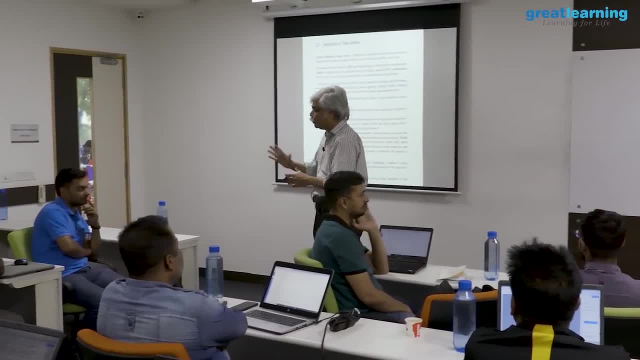 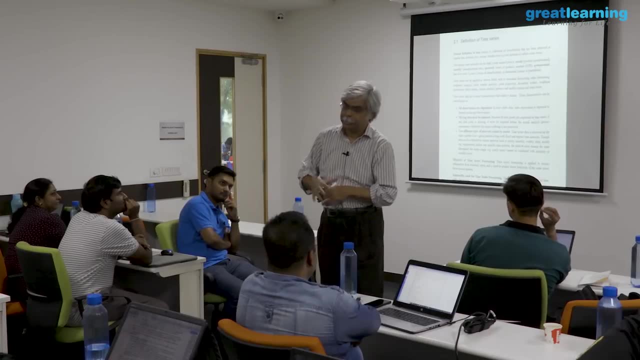 projection of the population of India, let's say, a year from now, which is the forecasting problem. this based on just one series. now, for us, that's going to be based on just one series. in practice, that's going to be based on a number of things. well, let's say, the population of 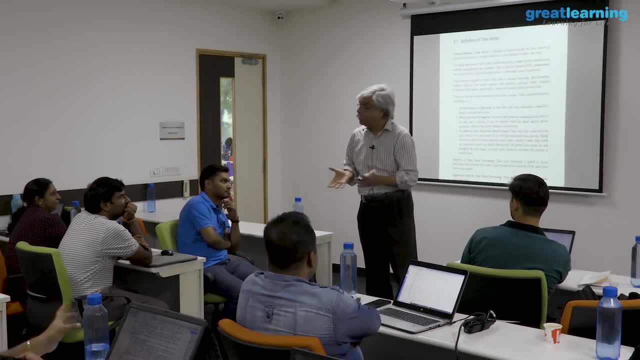 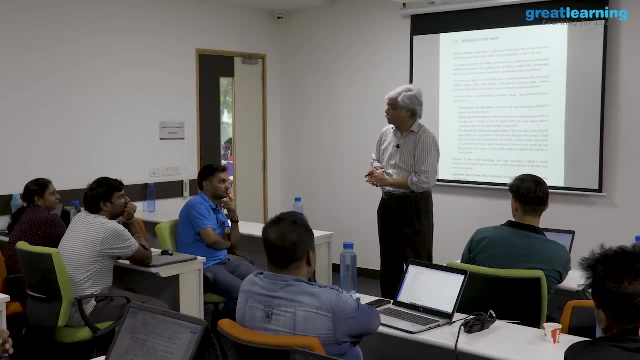 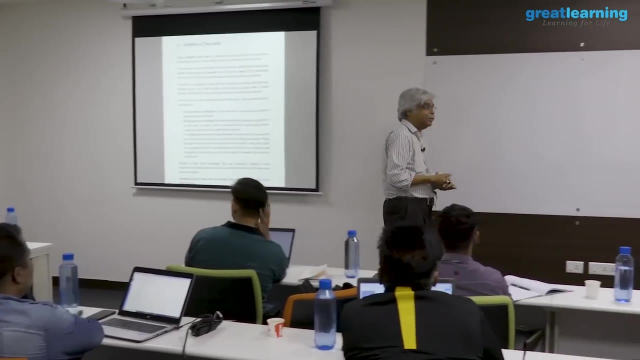 your companies. you work in companies. let's say that I want you to say how many people will your company have? well, let's say your HR team gives you this question. give me a forecast of the headcount at the end of the year, useful number to know budgeting purposes and all such kinds of things. now think about. 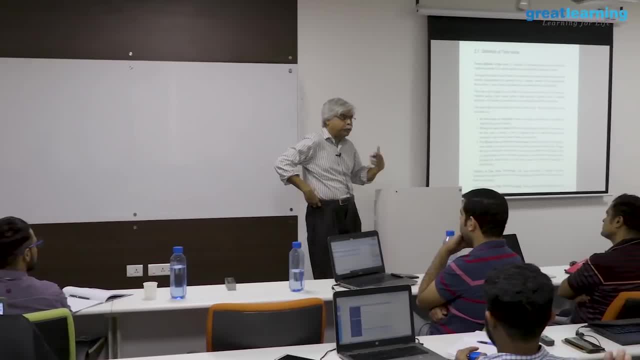 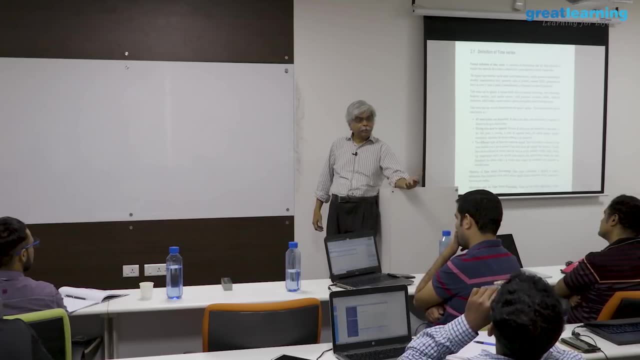 how you're going to go about doing that. what factors would would be going in? how would you do that? by the way, if someone asks you to say in your company what is the projected headcount at the end of this year? ah, that's that, in some ways, the 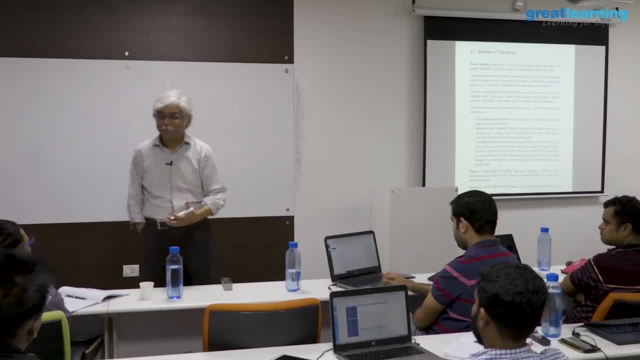 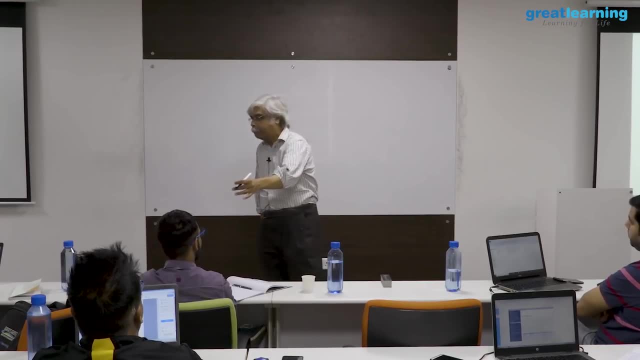 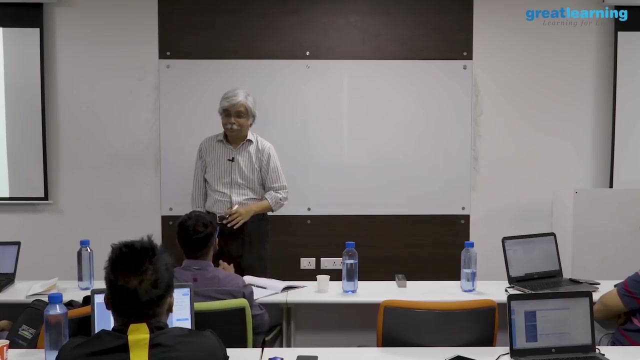 simplest way of doing it: net hires, as they say. net ads, net ads, huh. so how many people are coming in? how many people are going out in the past for the same series? in other words, you've converted into a pure time series problem. it'll be sequence. but more importantly than that, you're using of, you're using an. 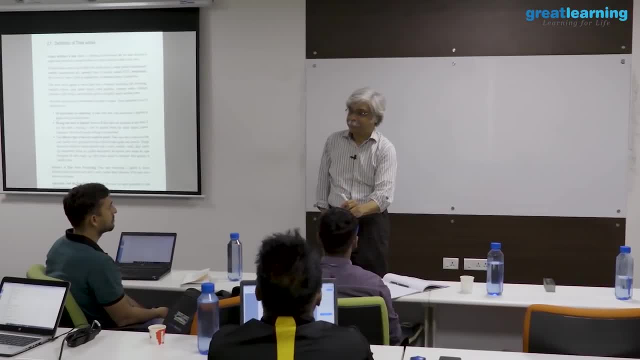 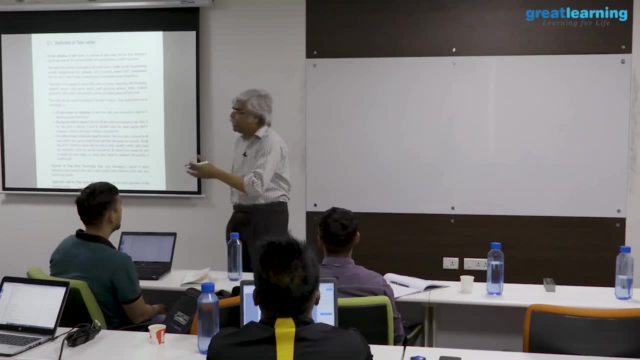 interesting idea. it says that this depends on many things, as you said. you gave me a 10 reason. it depends on on you know plans it depends on. it depends on many, see, but I say I don't care about all those many things. all those many things are already included in my data. they've all been factored into what has 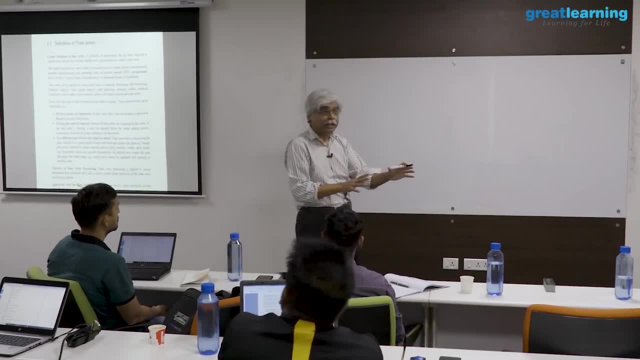 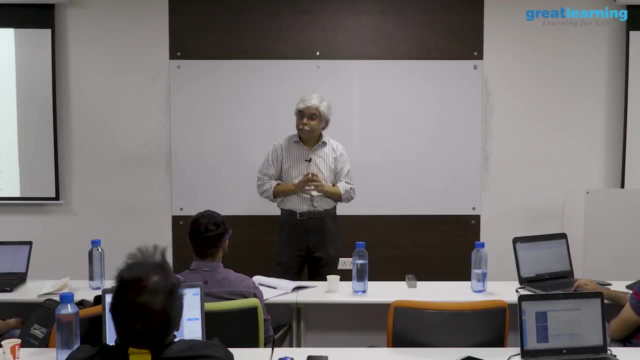 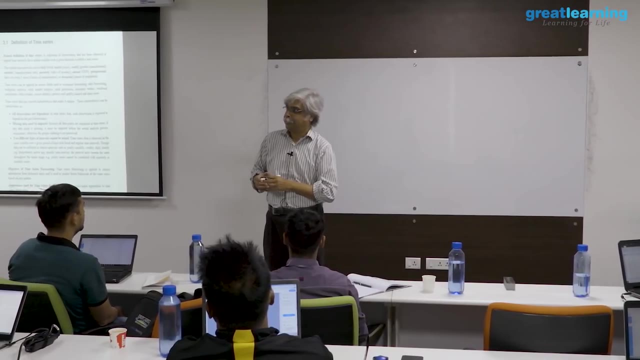 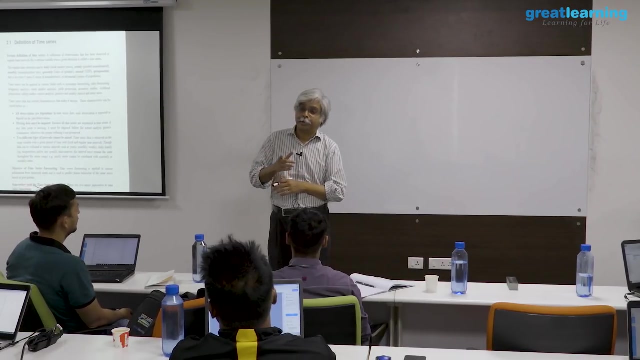 happened in the past. all I'll do is I'll figure out what this series looks like and then I'll project that series forward. now, this, this relies on it on an interesting idea, and the idea there is this: that the future looks like the past. now, if the future does not look like the past, what will you do now? here you're in. 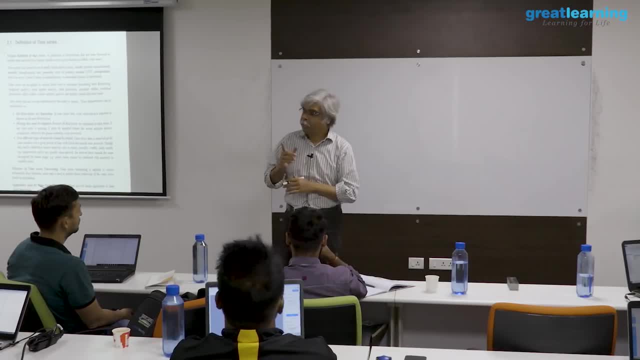 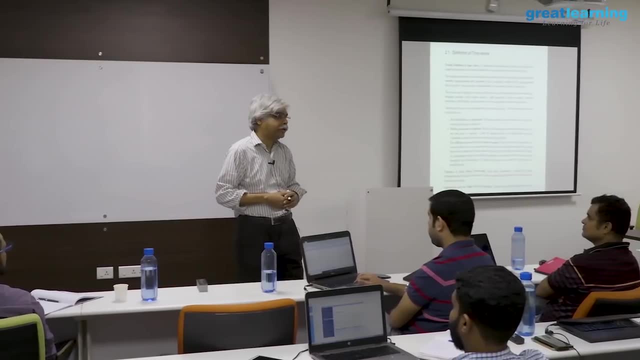 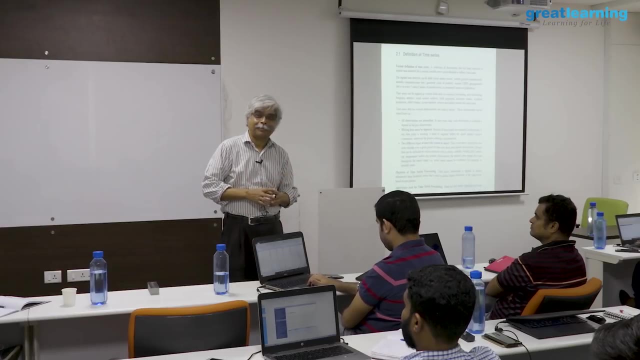 a fundamental difficulty because if you are a business analyst, then- and you are and you are in great learning to analyze data- the data involves only the past. the future has not happened. so now you're in a situation that your data may not be relevant, because the future is different from the past and the past is. 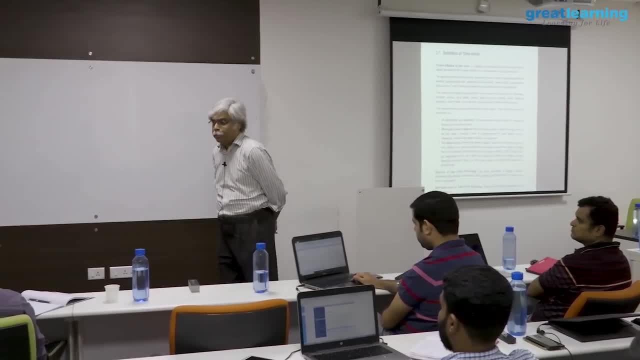 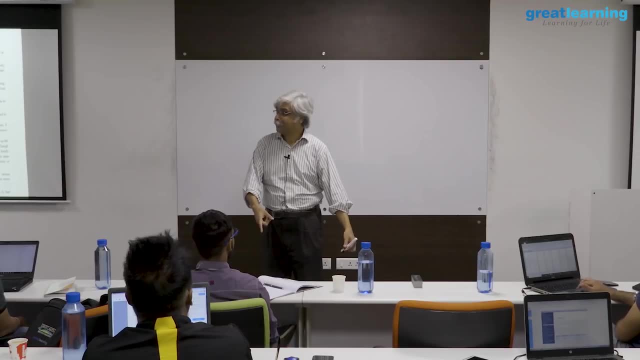 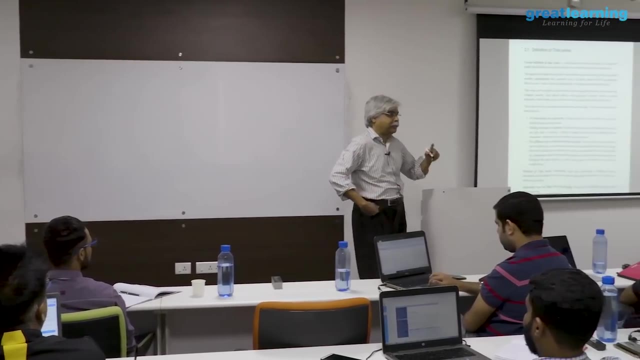 all that is available to you. the future is not available to you. the data is in the past, the question is in the future. you are sitting in the middle, so therefore, the the point is to be able to say: what about the past is going to be relevant in the future? what about the past is going to be relevant in the 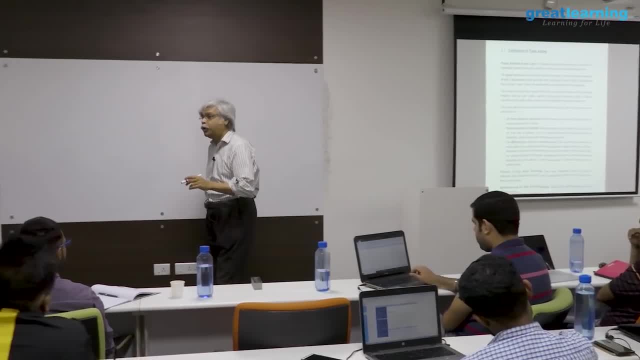 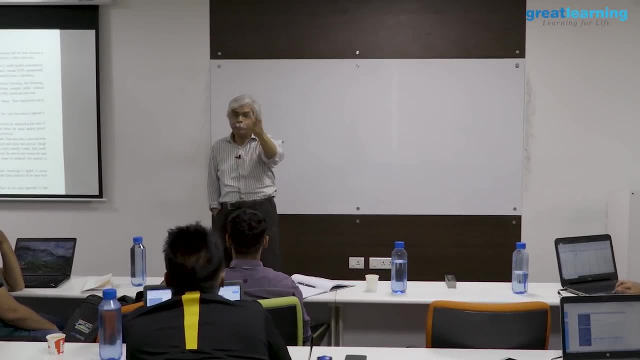 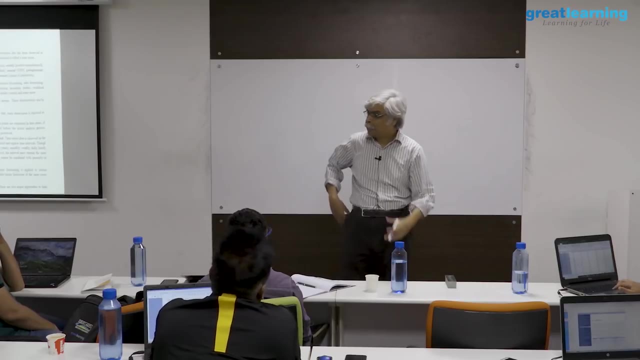 future, and there are multiple ways of doing that. for example, you could use the population idea to say there is a population from whom people were hired in the past and the population population from which people will be hired in the future. what can I say about that population and that? 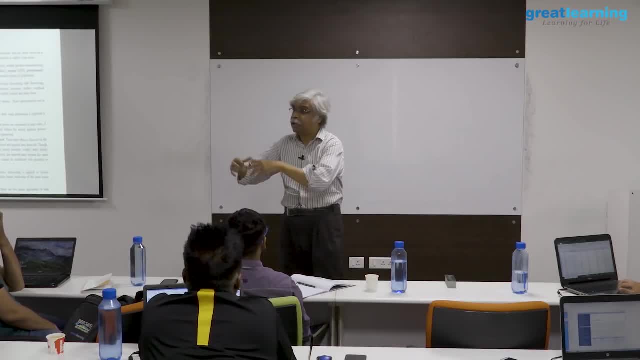 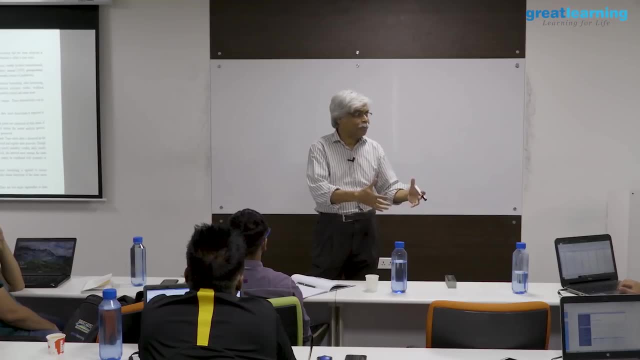 population is many characteristics. that population has demand characteristics, which means the labor pool people I'm hiring from. that population has supply characteristics, which is the managers, the people who are doing the hiring. but that population, I'm saying, is going to remain the same, and now there will be. 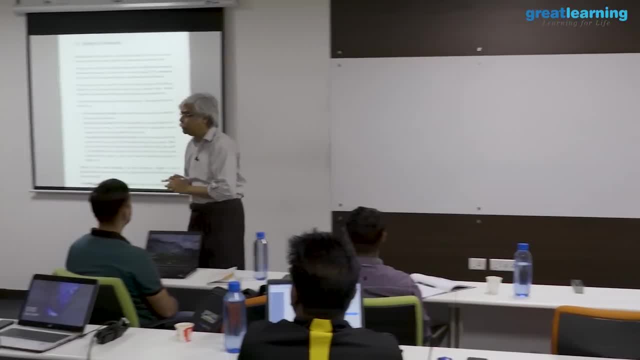 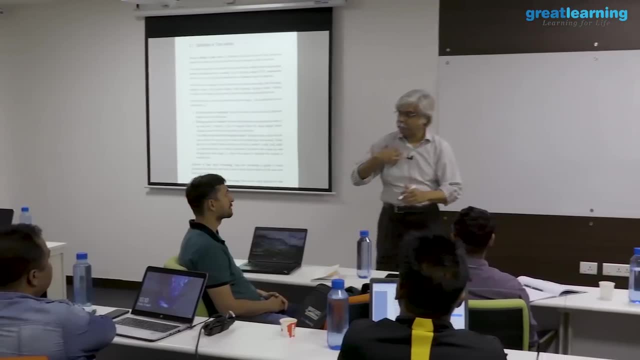 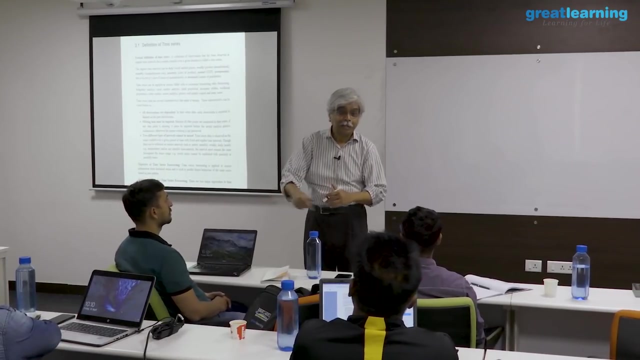 peculiarities that will differ. projects may differ, individual people may differ, motivation to leave may differ. he may leave for one reason, I may leave for one reason, he may leave for another reason. that's okay, but the attrition rate will remain the same. the individual attrition may differ and 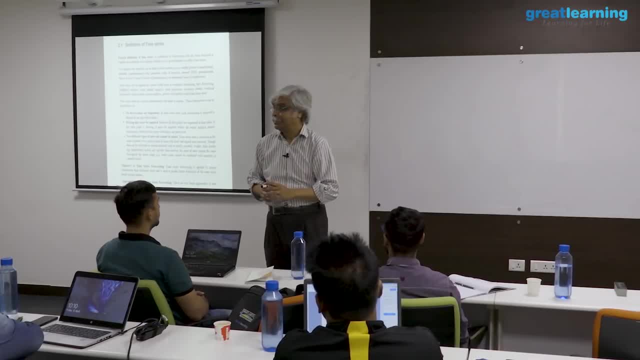 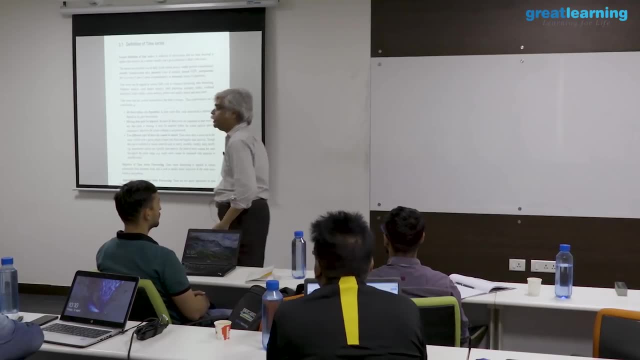 the way you predict that retribution may differ, but you may be willing to break the attrition. I don't care why people leave, but I'm going to assume that the rate at which they leave is going to be the same, so long as you allow me that I 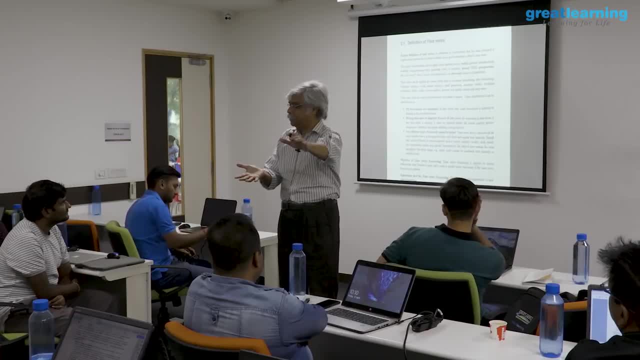 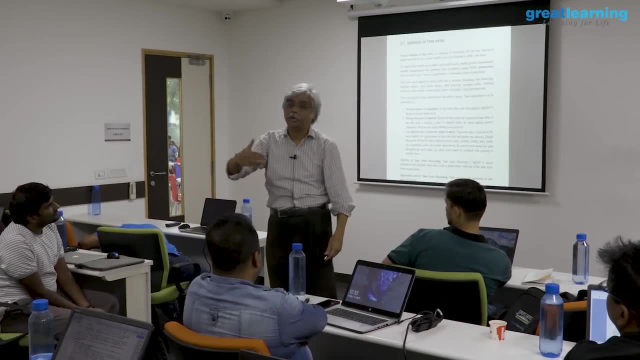 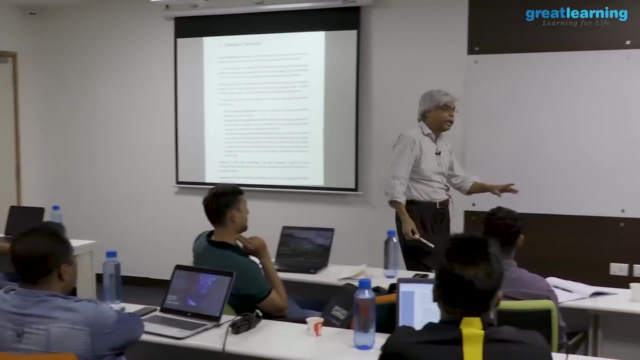 can project forward. if you challenge that now, I have a problem. now I have to say: okay, if I calculate the attrition rate, how do you think that attrition rate is going to change? and you say it's going to change. but I said, is it going to change like it? 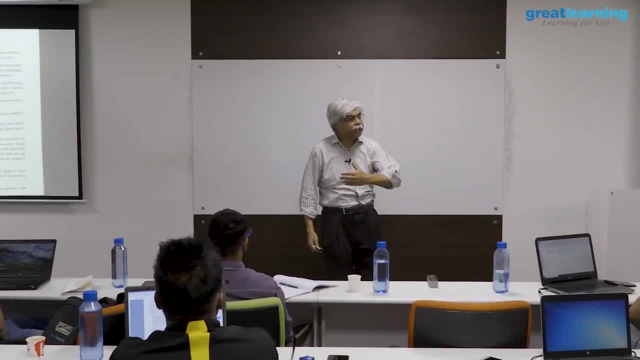 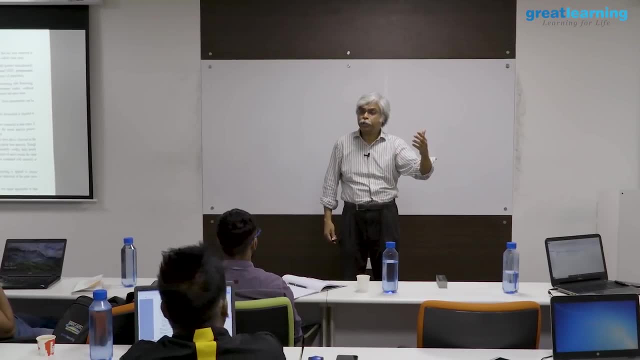 has changed before. so let's say, my attrition rate has been going up. so my attrition rate, let's say, was, you know, 12% and 14%, then 16%, and you may ask the question that if the future is going to be in the past, will it keep going up? and 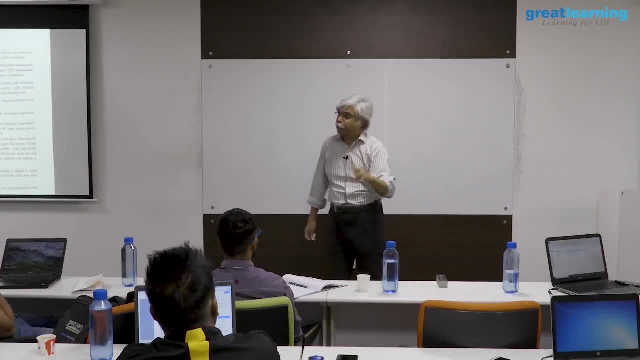 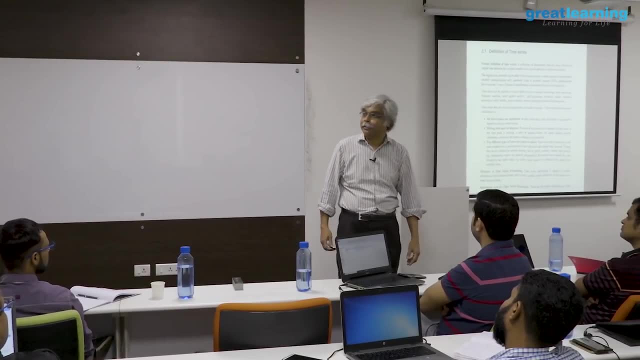 now management will say: no, no, no, no, no, no. now we have new CEO, new policy, attrition rate will not go up. we'll pay people a lot more. nobody's going to leave. very good, but now my trend has been disturbed. so the idea is to be able to 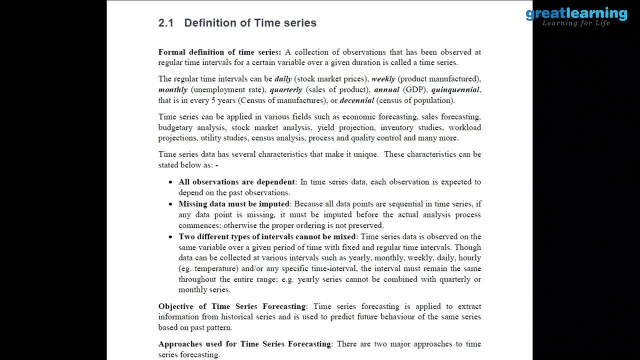 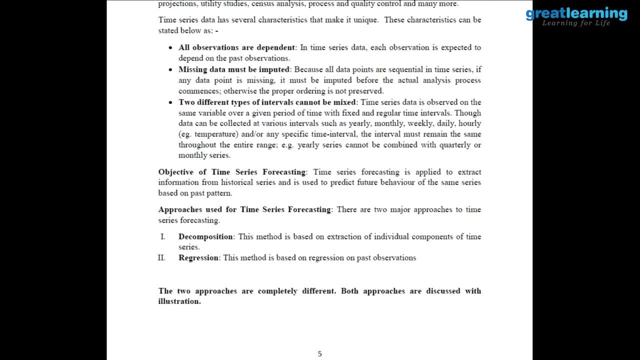 build different kinds of models to effectively solve this. now, the way this is solved is using two different styles of things, and we'll do both of these, and one of them is in some way called the decomposition method, which we'll do mostly today and a little bit of tomorrow, and the other is called the 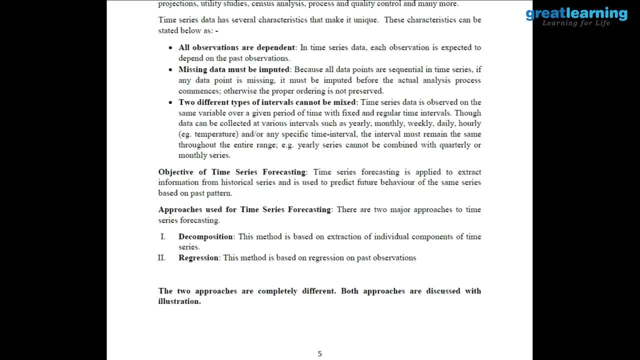 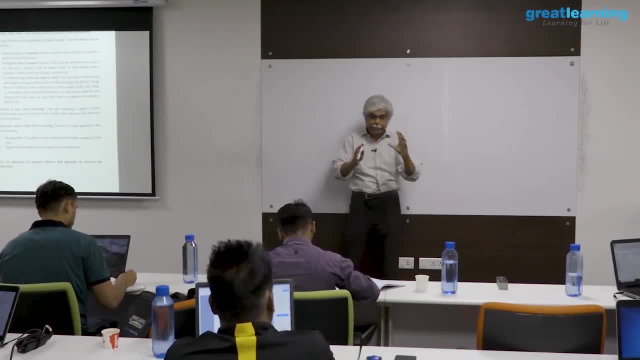 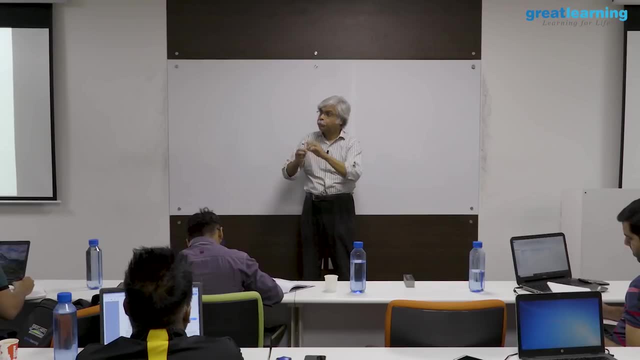 regression method. so the decomposition method essentially says this. it says that when you have seen a series of observations- let's say you've seen the sales- take that series and split it into certain parts. the first way I'm going to decompose it is saying that what part of the series projects into the future? and 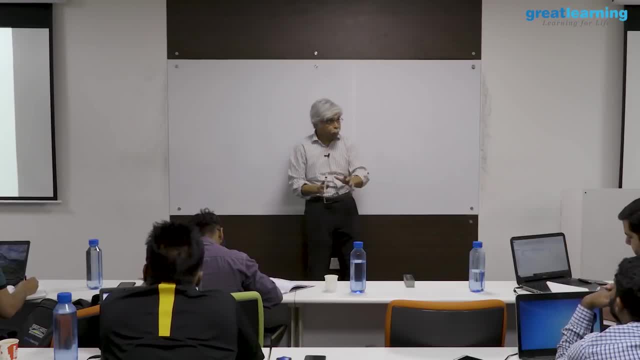 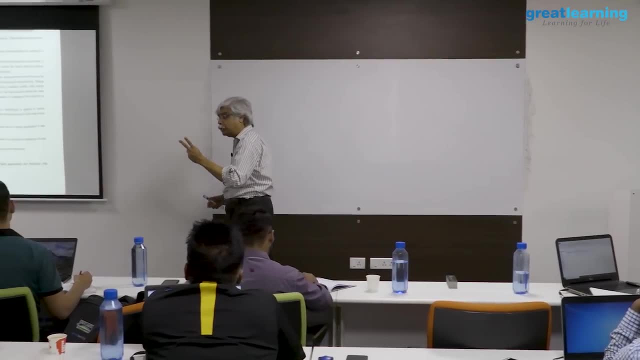 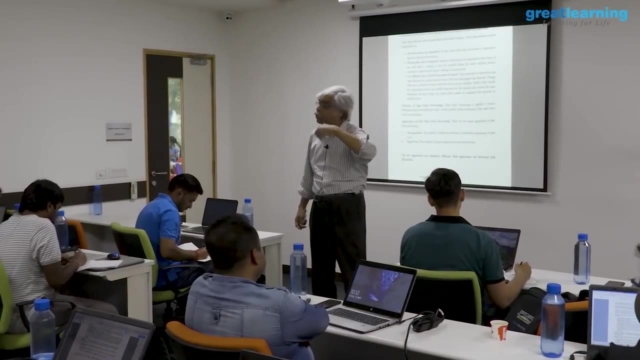 what part of it does not. in other words, what part of it, can I say, moves in the series and what part of it is not. that's the first decomposition. now, the part that can be forecast, the part that is systematic and not an error, is going to be useful in the forecast. 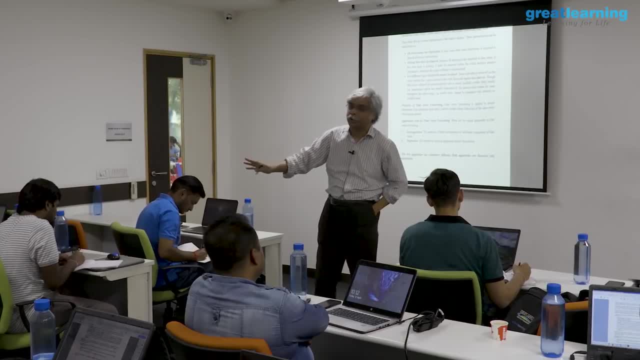 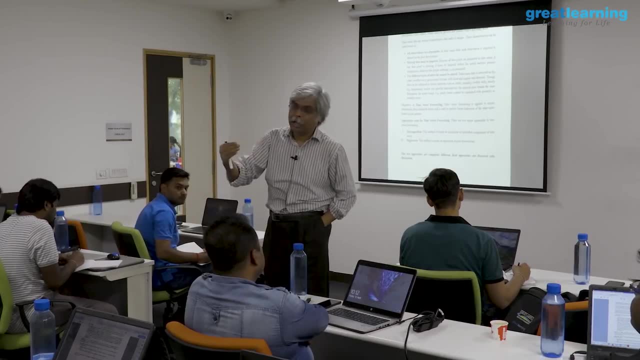 the part that is not systematic, like a random error I'm going to ignore. it's going to be like in your regression where you had: Y is equal to a plus B X plus epsilon in the forecast, your day plus B X. what happened in the forecast to the epsilon? 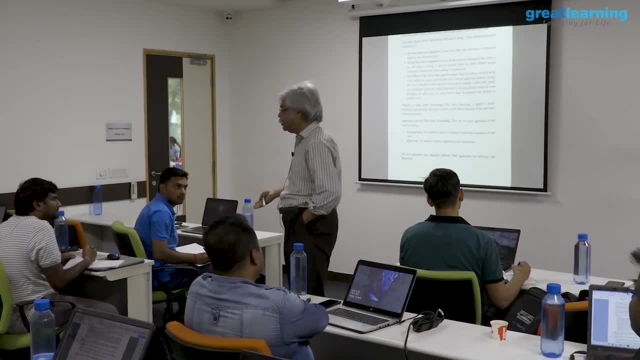 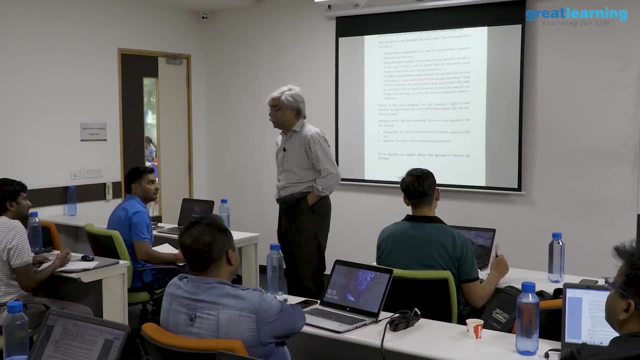 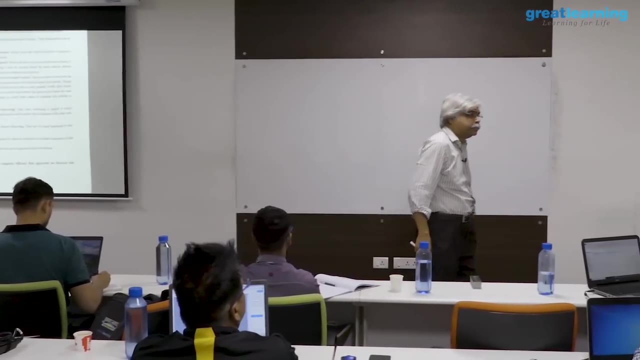 you ignored it. you ignored it. it was there in the data. it was in fact what is called a residual, but in your forecast you ignore the residual. why? because you said that the residual applies to this data set. it doesn't apply to the future data set. so when you forecast, you said Y is equal to a plus B, X with the new X. 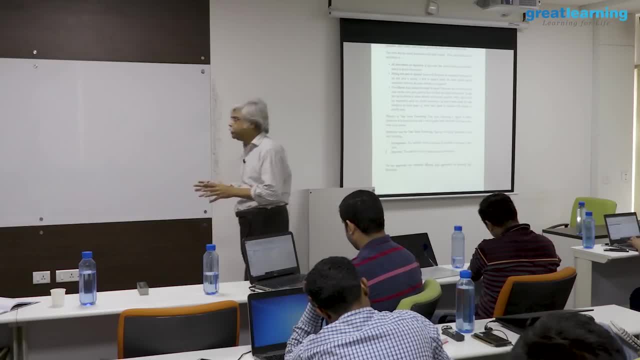 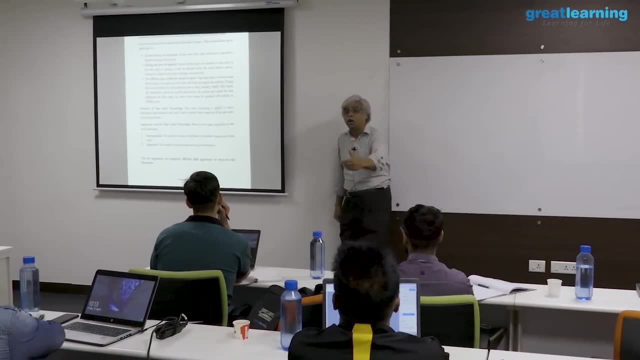 there was no attempt on the epsilon side. so decomposition decomposes the time series into four parts of the series and that's what you're going to do in the first teen- to two pieces: a part that is predictable and a part that is not predictable. the part that is predictable we'll use. the part that is not. 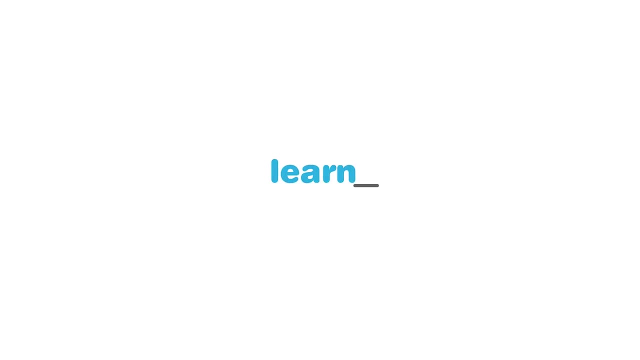 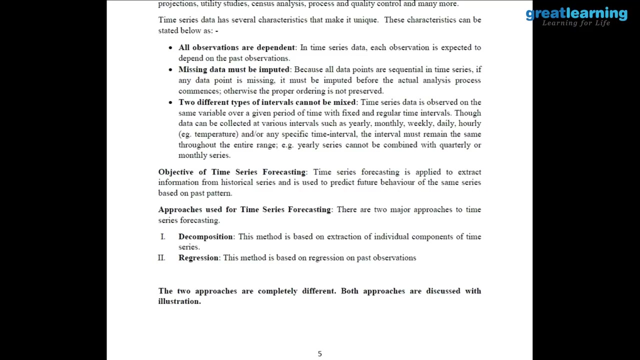 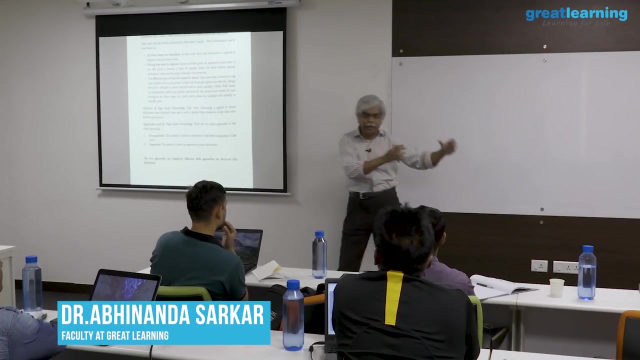 predictable, we will ignore. Oh you, Oh yes, absolutely, absolutely. that's a problem. but that's a problem not just any mean time series, that's a problem in all of analytics, which is the example I was giving in the, in other words, where you are going to predict, where you are going to project has. 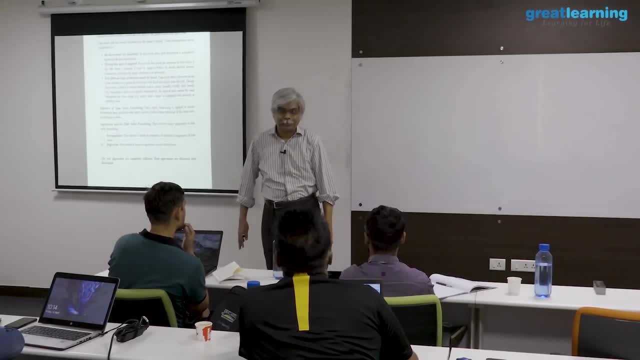 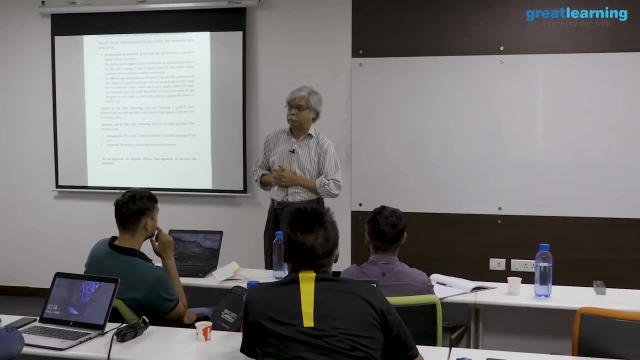 nothing to do with the data that you have. so let's say that you're trying to understand what's going to happen to jet Airways, correct now. what is the valid data for that? what data will you use in order to understand or predict what is going to? 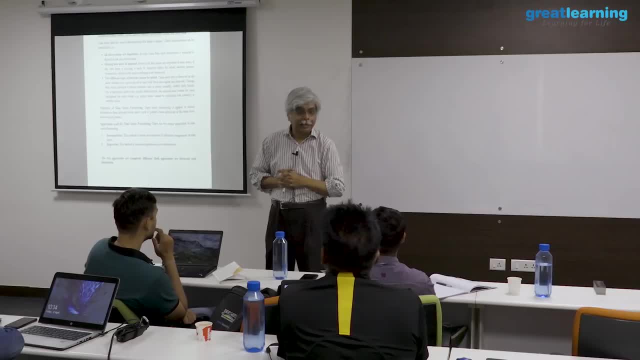 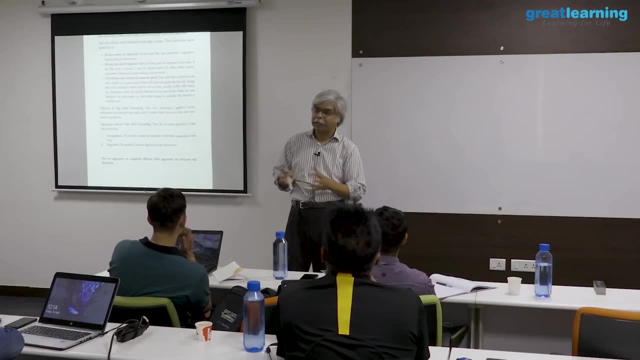 happen to jet Airways. so that is going to hit the problem. he's saying that the jet Airways of the past is not going to look anything like the jet Airways of the future. there are lots and lots of aircraft in the past- at 14 today, I think. 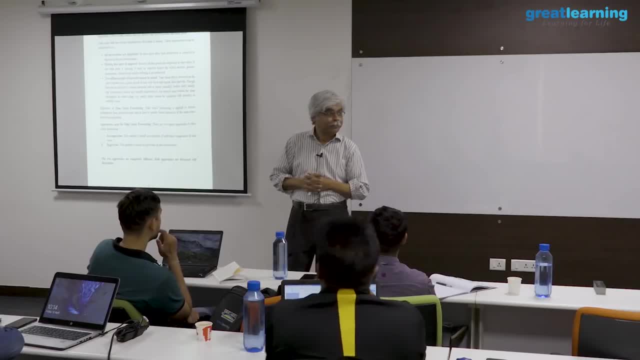 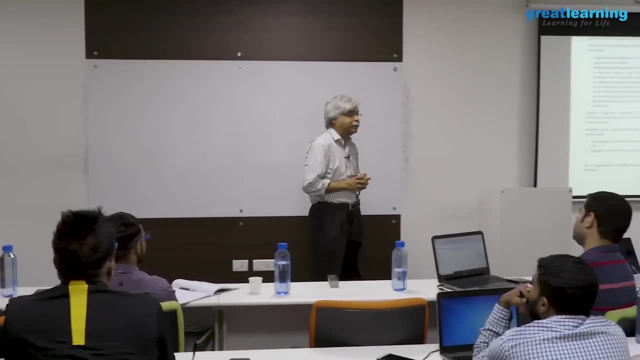 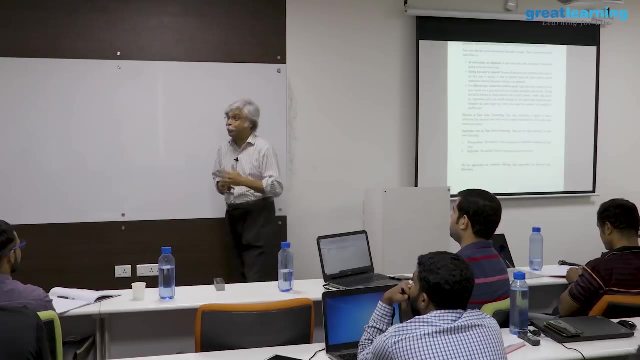 the newspapers were saying international flights are halted and things of that sort. right, I'm getting reminders from jet Airways saying your flight has been cancelled. I'm saying thank you for telling me. I had a flight. I didn't know I was booked on it. so well, I know now, and I now know that I have not booked. 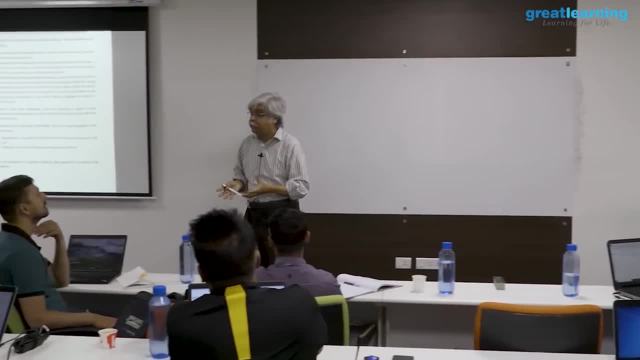 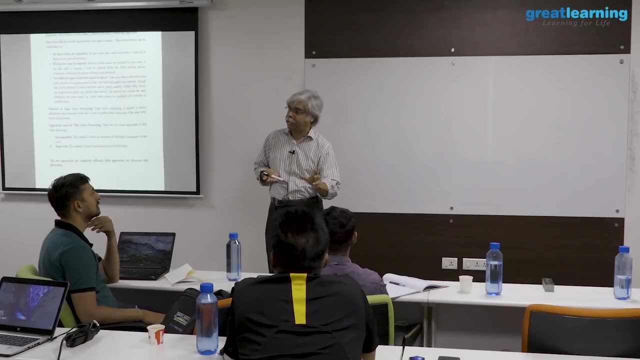 on it anyway. okay, good, so so is that the validator now? so so, or is it not? another argument could be that if I want to understand what is happening in a company that is going through this kind of a change, let me try and understand what happened to similar companies in the past that went through this kind of. 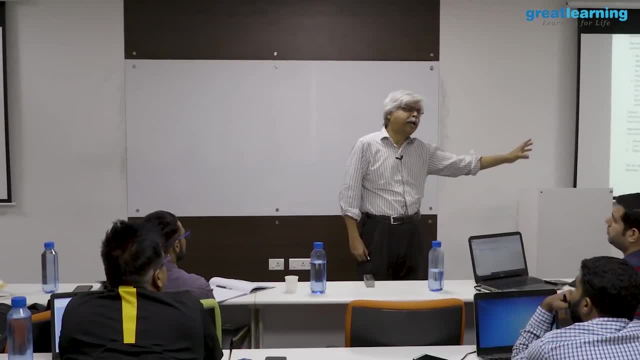 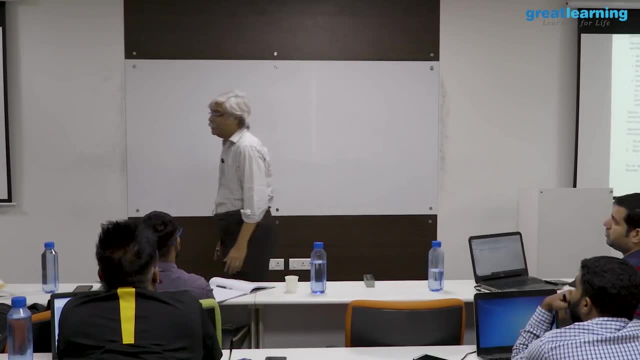 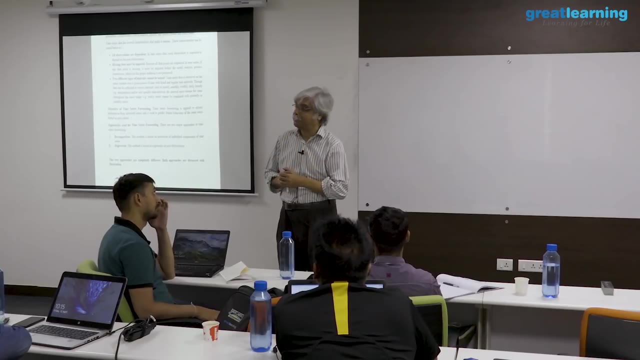 a situation. quite a few Airlines in the west of you know, some airline in North America and Alaskan airline, or one of those just left his passengers hanging in an airport. essentially, the airport shut down. a year ago. an airline shut down when the when his planes were in the air. so the pilot said, okay, we'll land you, not to. 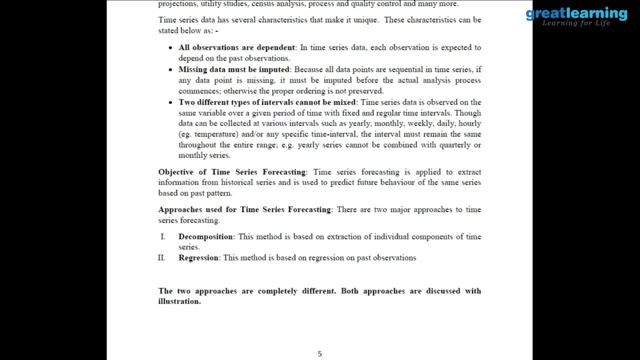 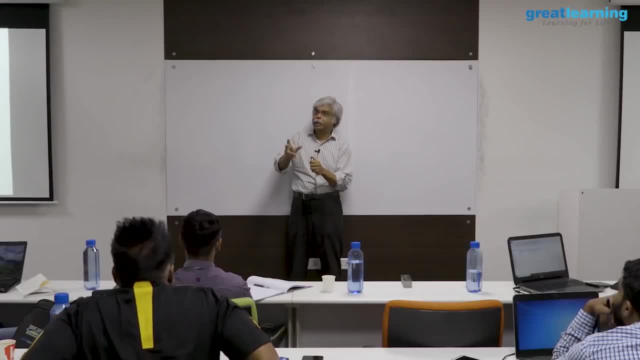 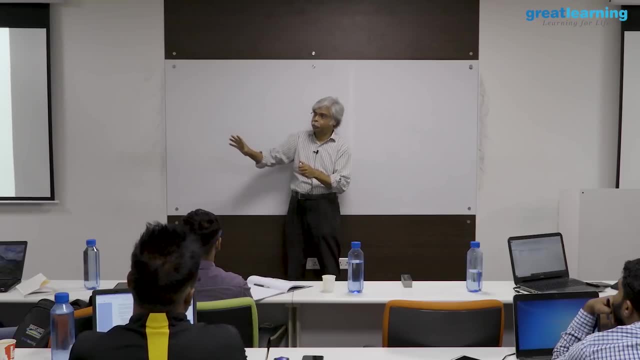 worry, I can't go anywhere, can I so? so there is data, but that data applies to. so the idea is what? the idea is? to say that if I want to get information about any situation, let me try and get information about similar situations and Kissinger whisper to me: if I want to go anywhere and get information about 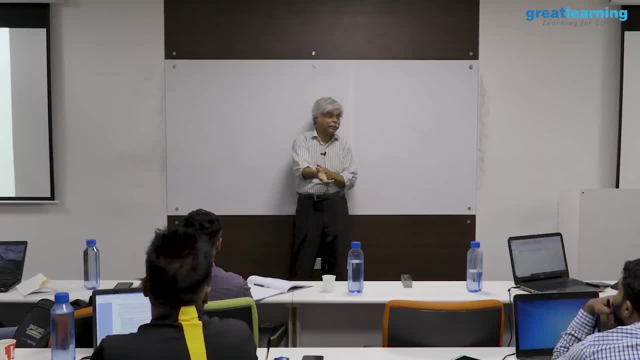 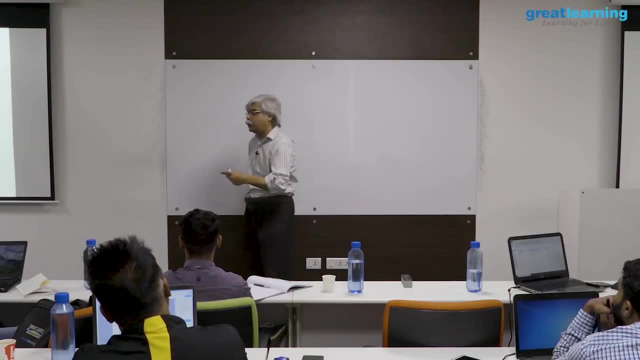 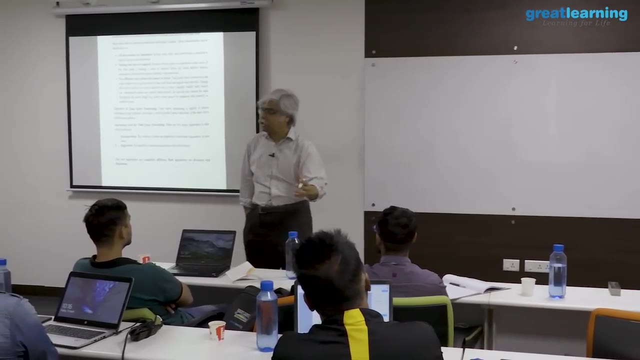 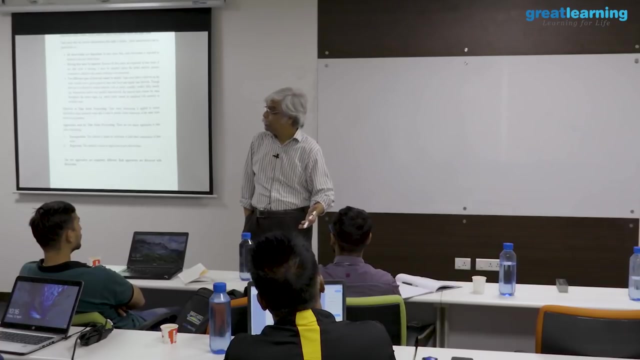 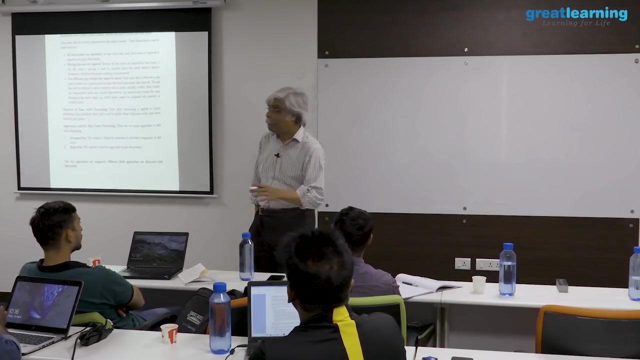 the same situation. someFRMD board, or maybe DC somewhere, will be a person sitting and setting a call from some village to somewhere�얼 vie, Esto es una La Casa T печерки No Bro. collapsing Airlines globally may be a better sample. is it an example of? 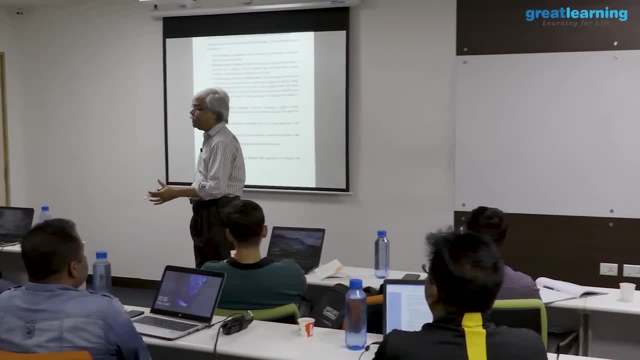 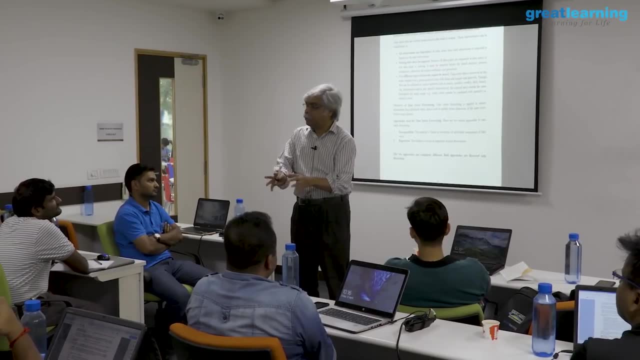 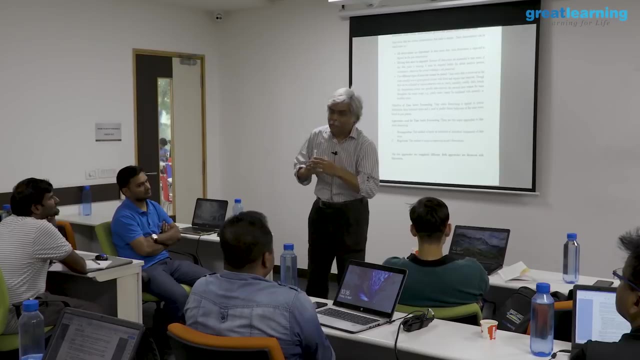 companies in India that are collapsing, maybe. so what we do is analyst is very often we play this game in saying that: if this is what I want to understand, where is this? where is the data on something that is similar? if nothing like that exists now, you're in trouble and essentially you have to make things. 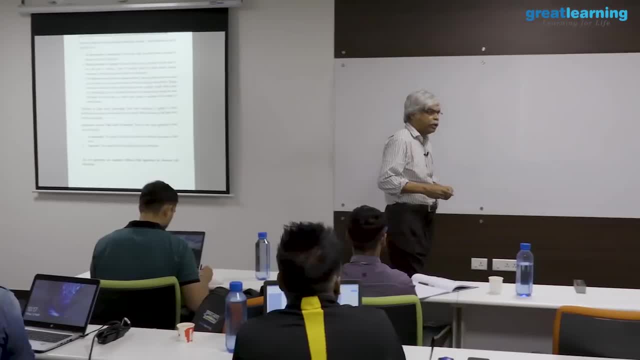 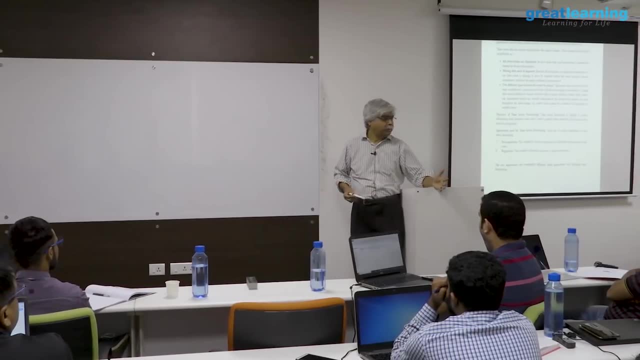 up we have to guess. or you build a pure mathematical model and you do some analytics on it. you optimize it, for example, and things of that sort. you build an equation, you've done optimization. so in optimization, for example, where do you get those numbers? you did a linear programming and mean. 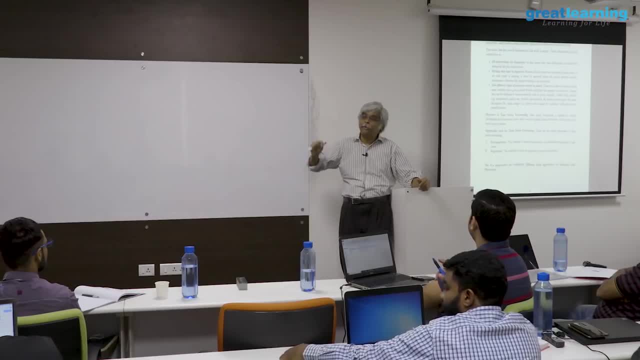 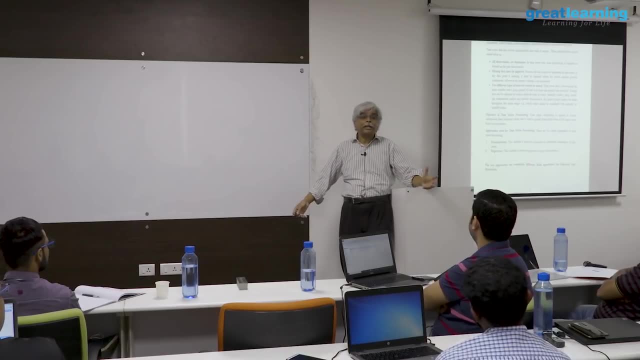 using solver and things like that. right, where did those input coefficients come from for the problems? you did those. so where did the? where did the number come from? when? where do? where did the right hand side of that constraint? where did the equations come from? from the business side? but how did? 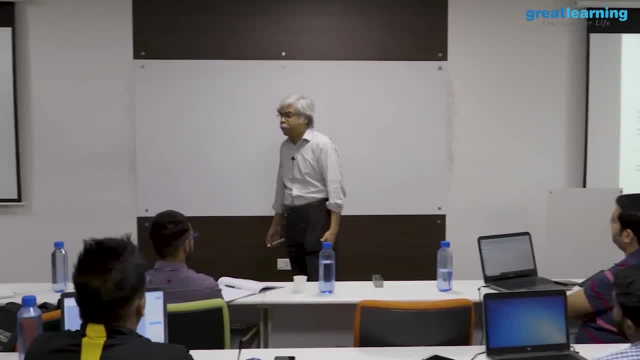 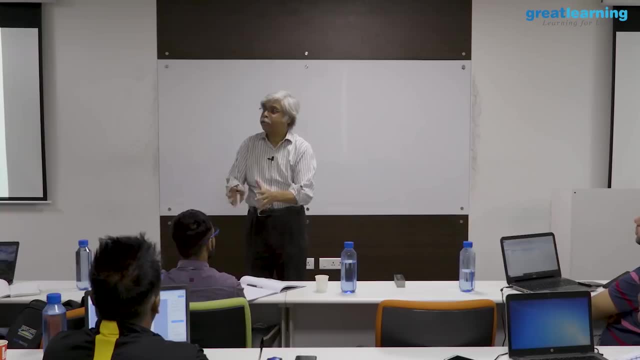 the business know? did they do some analytics to do that? did they make some assumptions? so, if there was no data at all, you sit and you make certain assumptions and say: this is it now in optimization? you did not, you did not think of that. but, for example, it could possibly be that the equations that 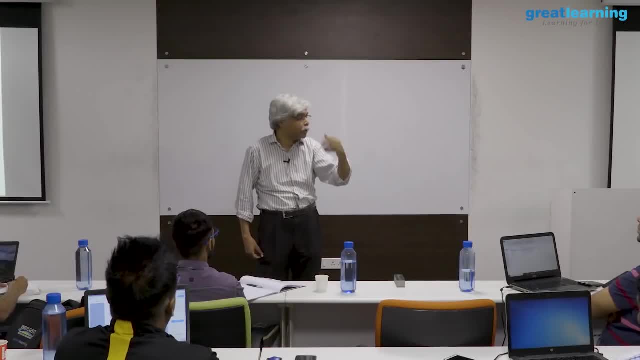 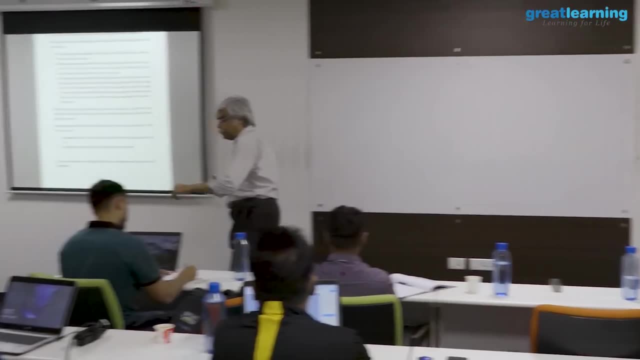 they're using are themselves sort of like linear regression coefficients or themselves projections, things that have gotten from the data. what is the cost? what is the cost of this input if you're, if you are going to use that to optimize, what is the relevant cost? the relevant cost is the cost that will. 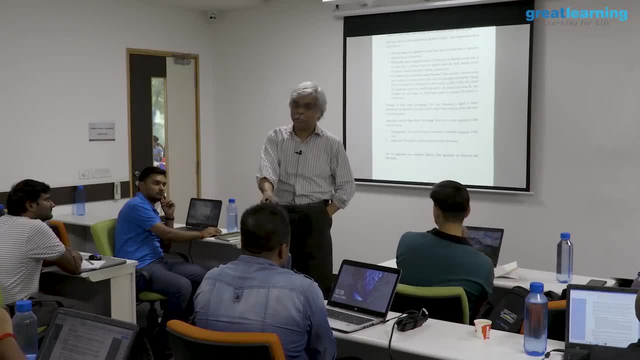 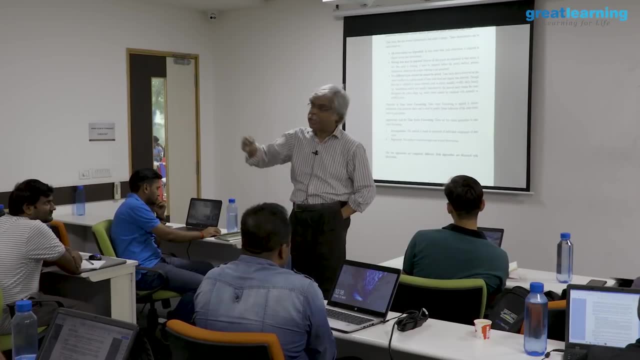 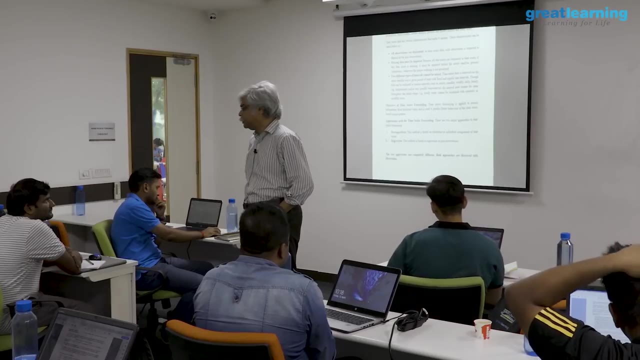 be in there in the future. but what is your data cost? your data cost is the cost that is there in the past. given cost in the past, what cost should you take to take as an input into the solver so as to optimize, let's say, your revenues or optimize your profits? that's going to be a projection of the cost, or? 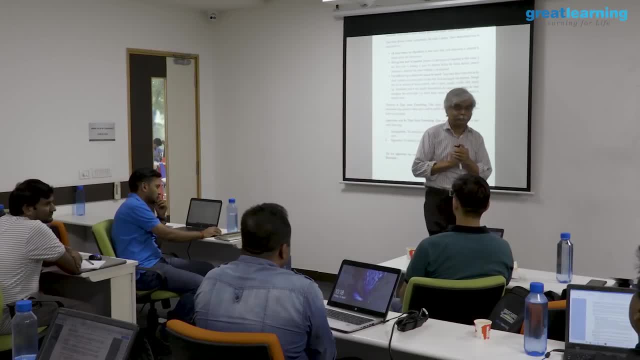 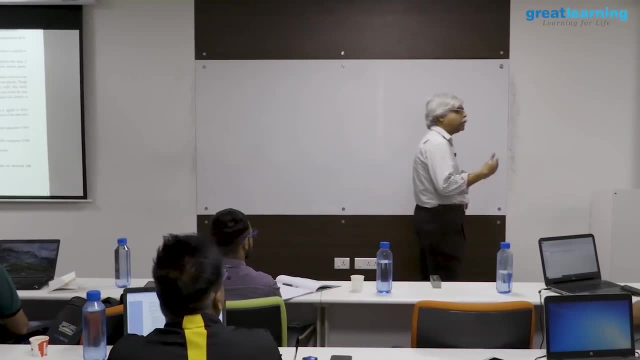 is going to be some model. if you could say: look, I've got no idea what this is. now you're in trouble. either you make up things as you go along- you know as you say- I'm going to assume that this is the case- or you start getting the data and you and you fill it in. you should read: 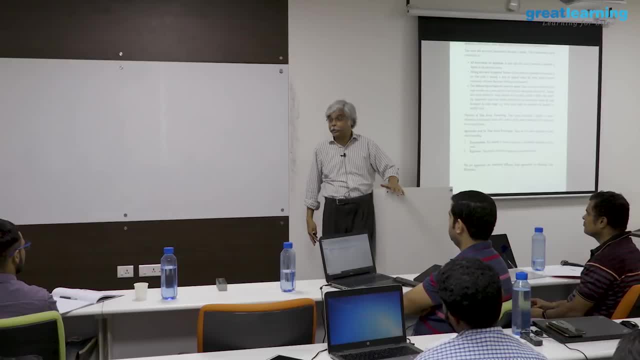 your books on by philosophers on this, I mean, makes a fascinating reading. that's saying that you know, you know humanity, so to speak. sometime around, maybe 2,500 years ago, whatever, people became conscious and people said that you know, we want to understand where we came from. we're looking up at the skies, we don't. 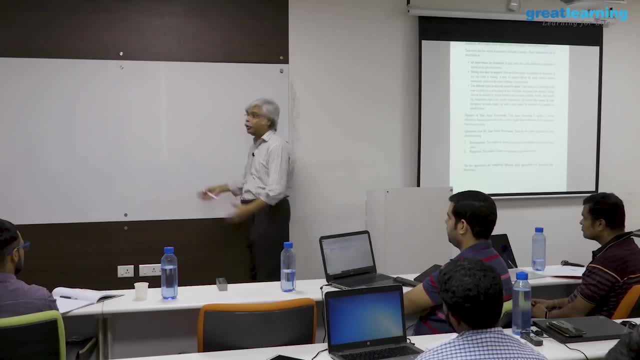 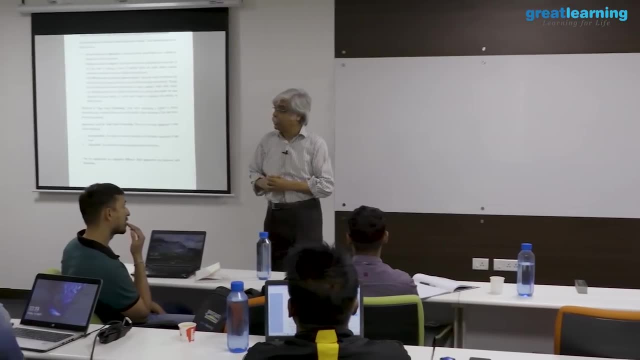 understand where it is. we're asking questions like: Who am I? why was I born? what do I do? what is my purpose in life? what is my purpose in life? what is my purpose in life? what are all these things moving around in the sky? are the animals the same as me? these are good questions to ask, but there was no data. 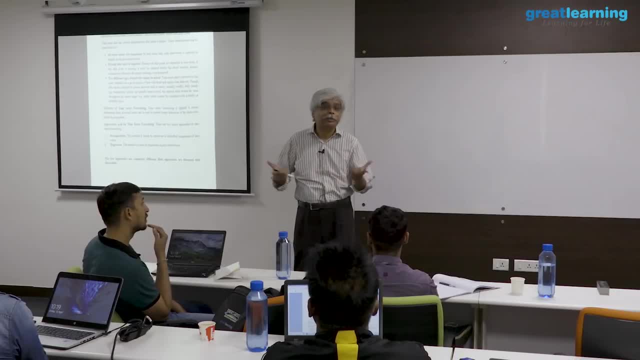 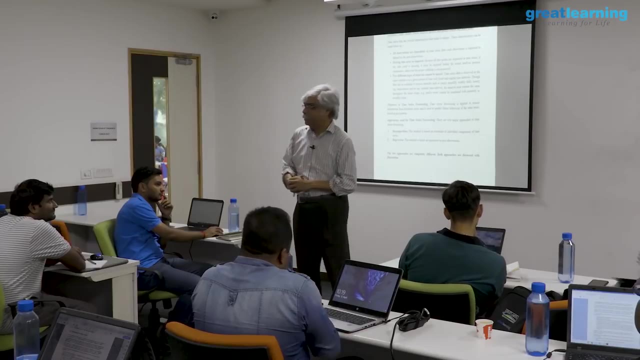 there was no information available to humans to answer these questions. so, in the opinion of many all over the world, religions got created because answers to these needed to be present. from a purely spiritual, from appears answer saying that: why is this happening? now I've got no date, I've got no way of knowing how. 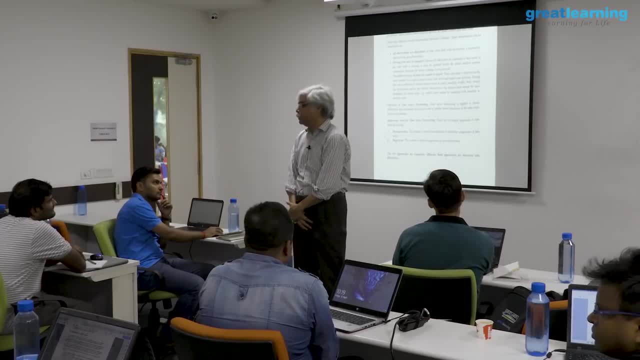 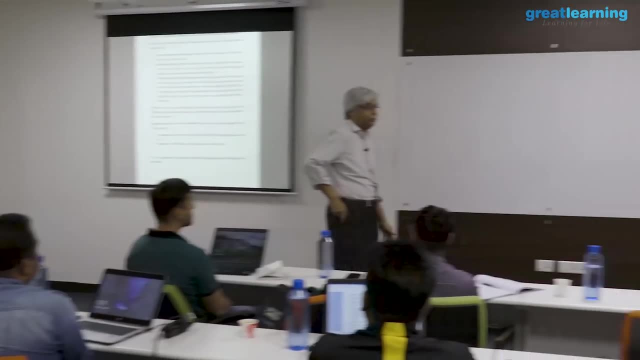 the universe was created. so let me make a hypothesis. let me say that this is how I was created and you do that, and then you, as the centuries went by, people figured out how to get data around it, so they got data around it and they got telescopes, and they got microscopes, and biology was created. and they say, oh, this. 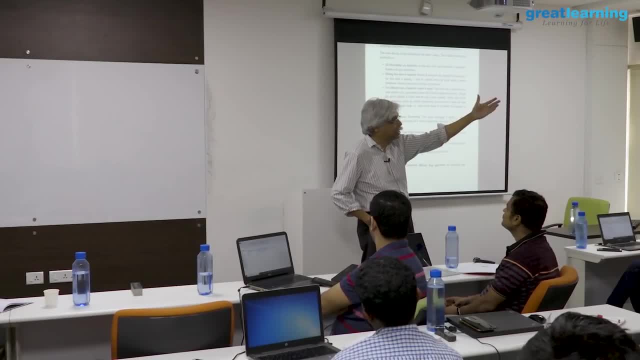 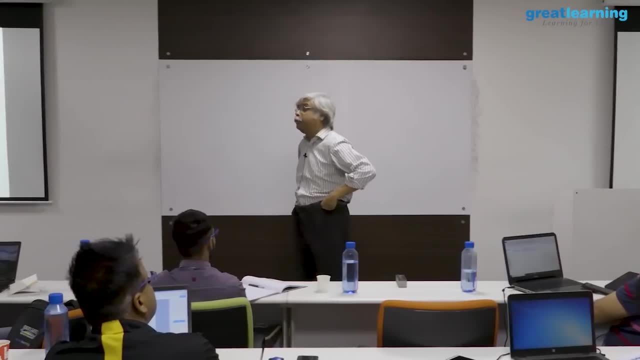 is what plants look like this, what animals look like. telescopes got created this, what the Sun looks like this, what the planets look like. slowly, people got data and they say so. this is probably what happened and people came up with theories of, of evolution, like you know, Darwin. others people came up with you. 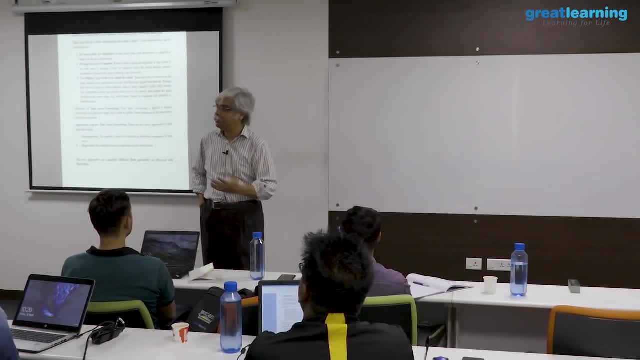 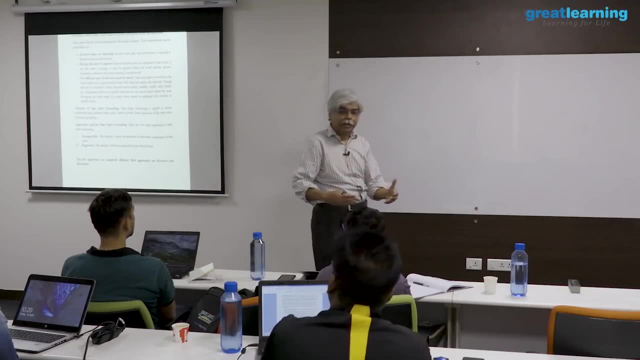 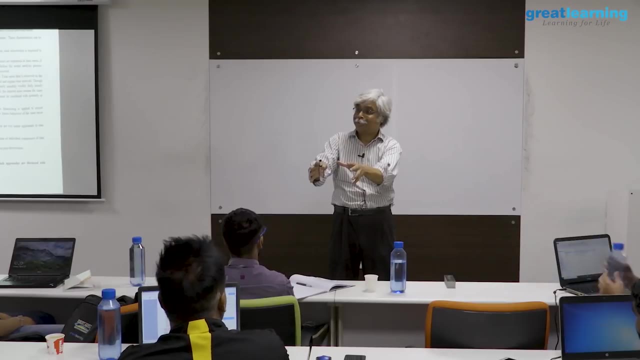 know theories of astronomy like Copernicus, and you know Bhaskaracharya and Aryabhatta and many others, and so slowly data started coming in and slowly science started getting created and you chipped away and you got the data and you say: now I have the data and I think this is true and many people believe that that 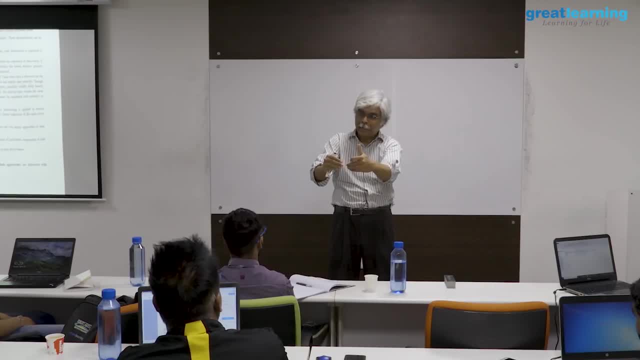 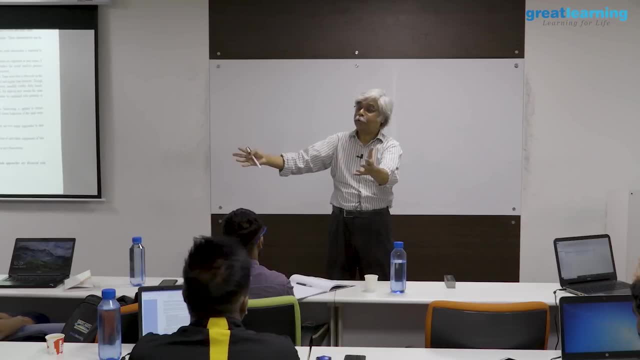 the way science operates is that you get the data and then you say: now I have evidence and now I'm going to remove my assumption with this evidence from the data, and but there are still things I don't understand and I don't know how to do that and I don't know how to do that, and 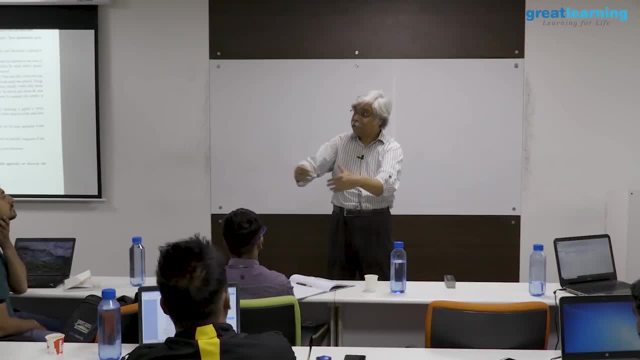 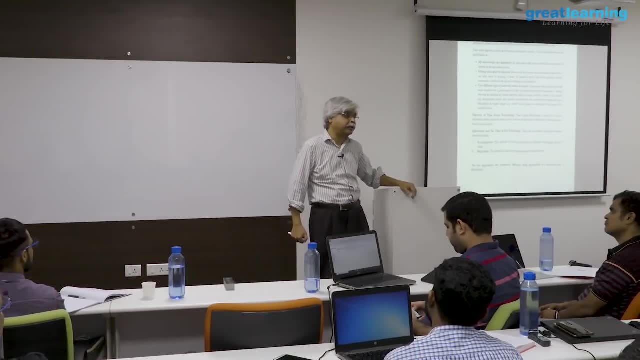 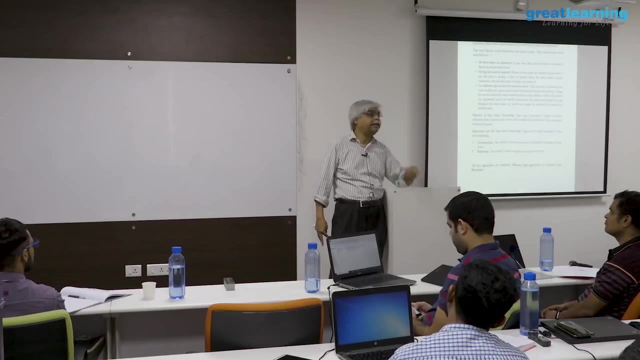 understand and let faith and religion remain there until I get enough evidence to say that I believe that this is not the case. and the analytical world. you end up doing something that is vaguely similar. if you, if you don't have any data whatsoever, then you make it up and as you start getting data, you start. 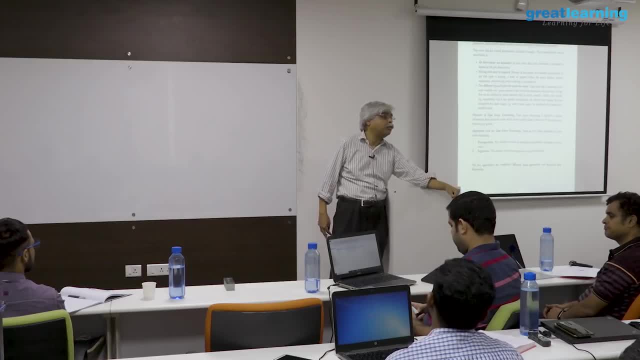 filling in those gap gaps. and you say, now, what should I do? not now, what should I do now, what should I do? and you get information around it, correct, if you don't have any data, you, you borrow it. how did you decide? you want to call it somewhere right, undergraduate degree. how did you decide? 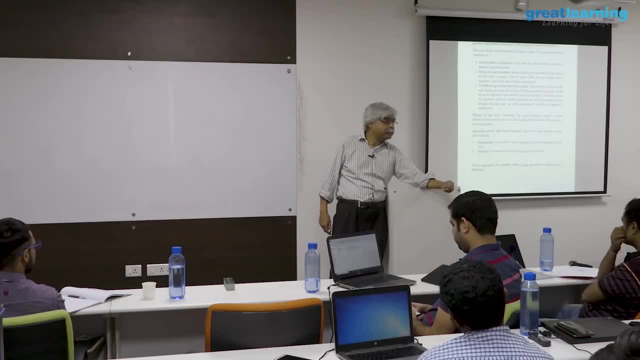 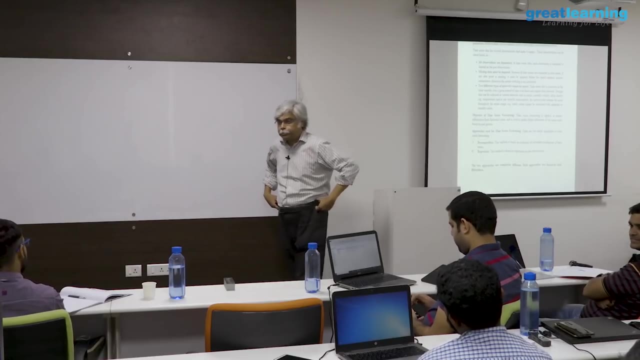 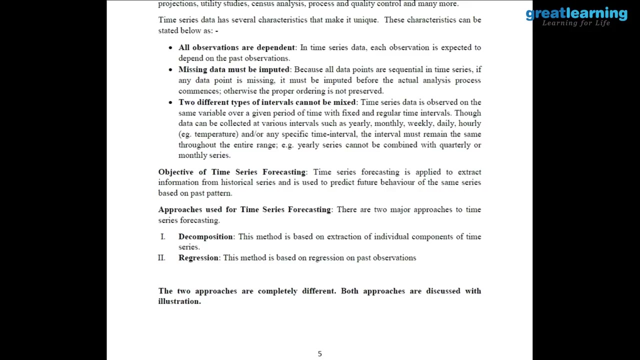 where to go first of all, did you decide where to go, or did someone else decide where you went? or your marks right? what did you do? you use your data to infer what, to infer where you can go, fair enough. so you use your data to say: the data says that this is where I want to be able. 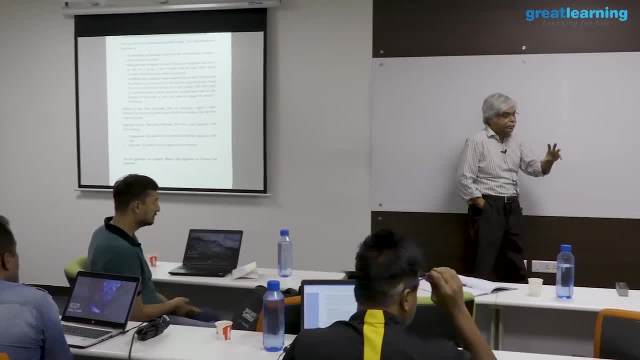 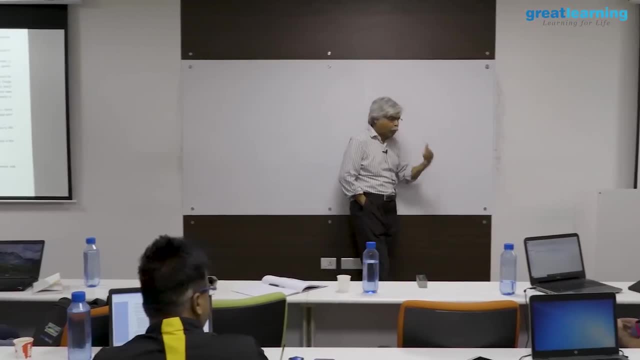 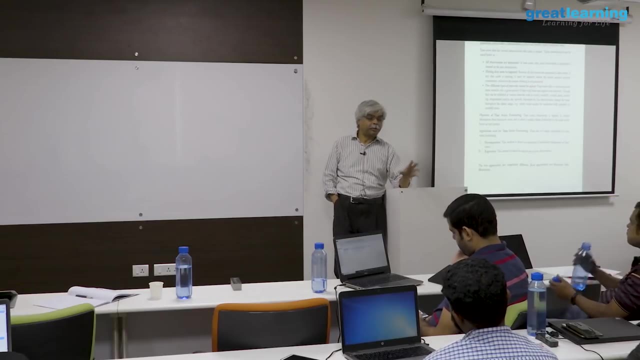 to go, or it might be that the data says that the best students do this once you are in there, then what did you do? so you made a database decision based on your performance to be able to do that, and then what you do, my point being that, as 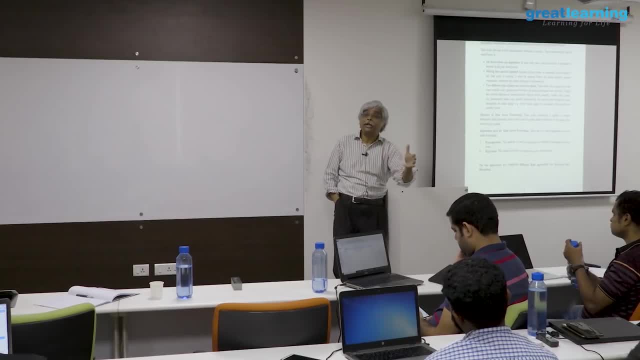 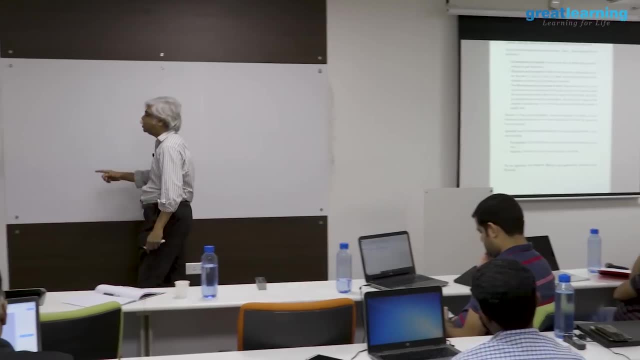 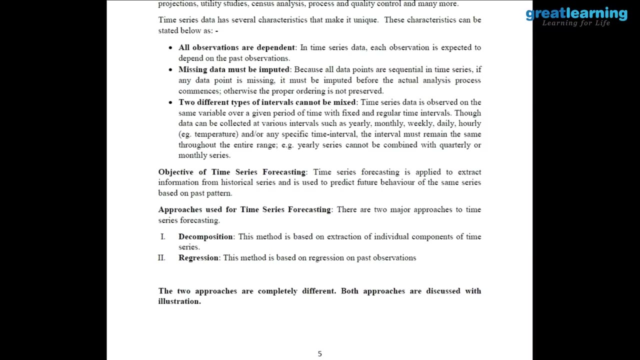 you got more and more information. you took more and more informed decisions as to what to do and every time around, to some extent, you use that information in order to be able to predict or forecast certain activities that you will do. you're standing on the road. you're standing on this road in front the taxi. 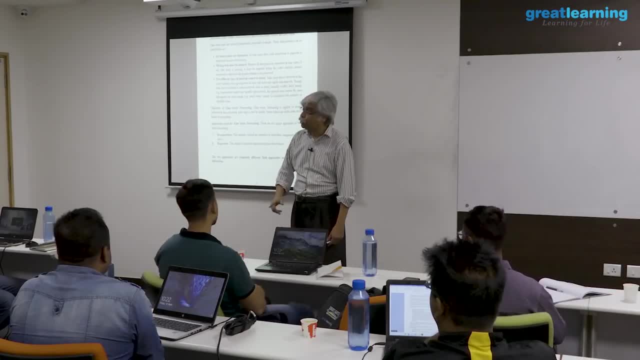 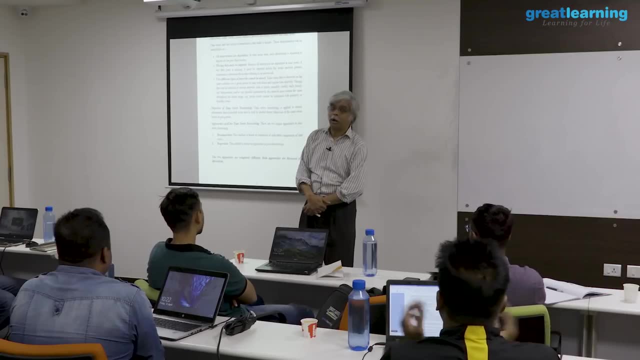 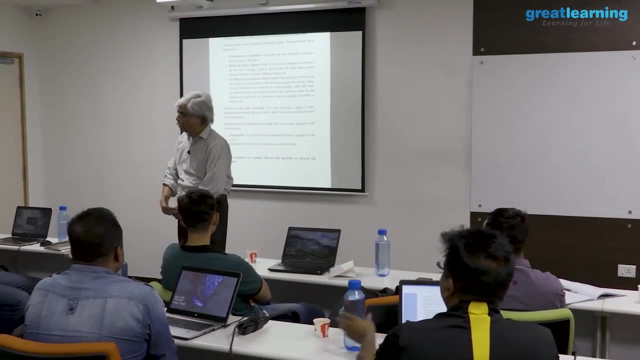 has dropped you off on the other side. you want to get here or you want to get home. do you cross the road? how do you decide whether to cross the road or not? based on what? based on the data. so a car is coming towards you, you're deciding to cross or not to cross. how are you making that decision? 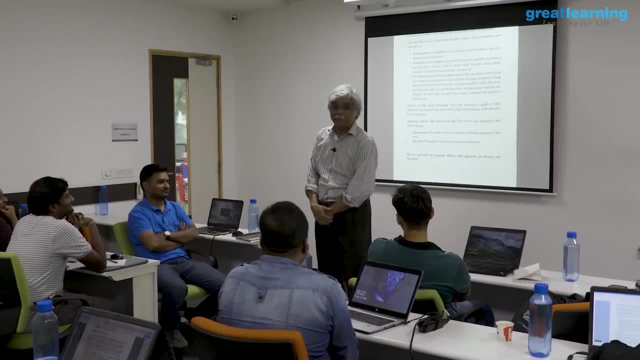 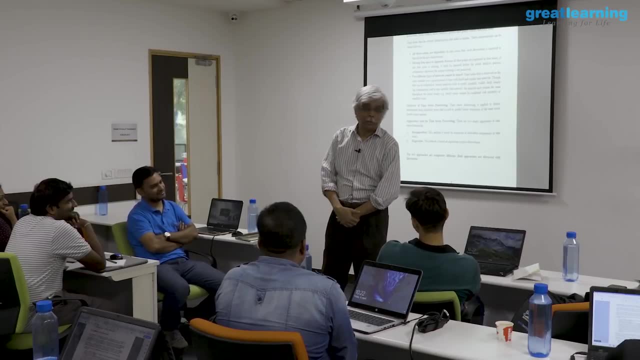 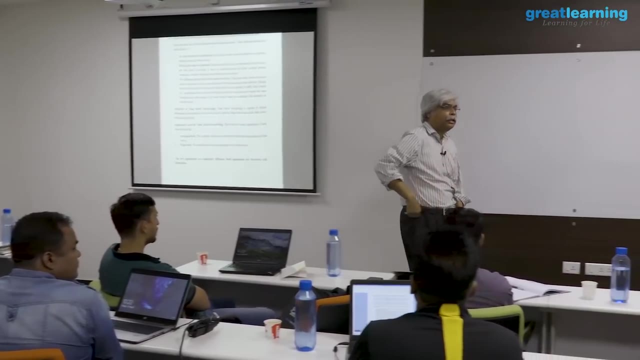 speed of the car, hopefully your speed as well. how close the car is, the speed of the car, your projected speed, the distance to the other side of the road. you will use all that information in order to be able to make a split decision as to whether this will come here or not. now you're going to make 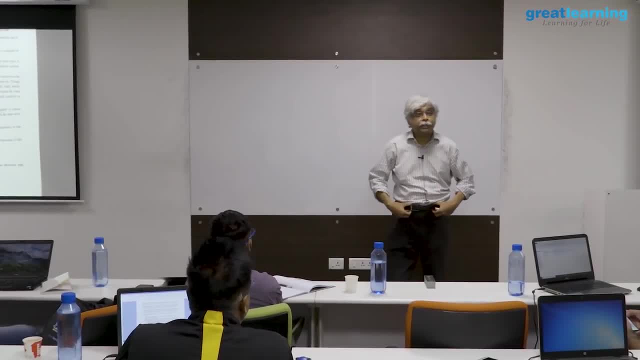 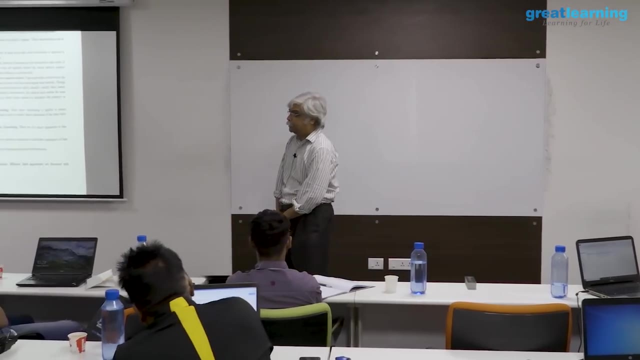 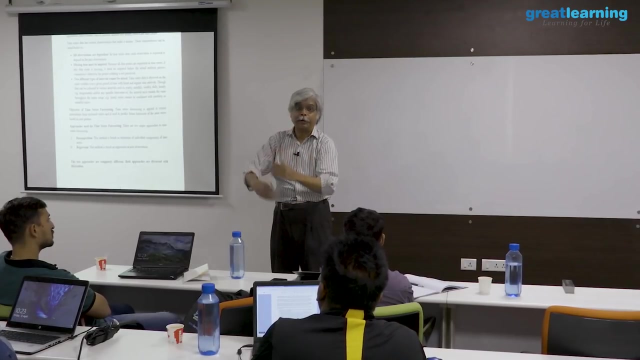 certain assumptions. for example, one entirely reasonable assumption you might be making is that this car is not speeding up. if this car is accelerating, your assumption could be wrong. now also the assumption that you will be able to cross in time and that something is not going to come into your way. you want to. 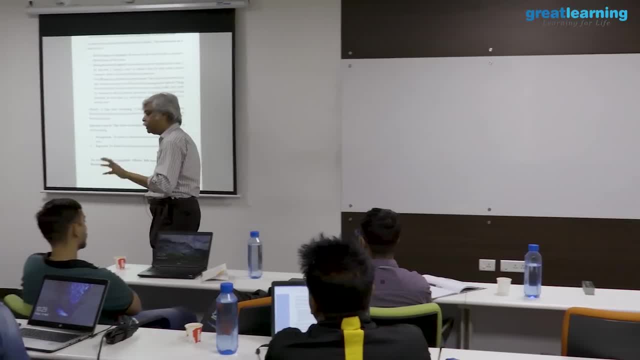 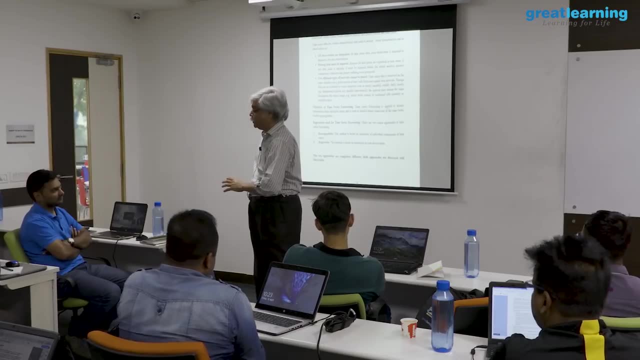 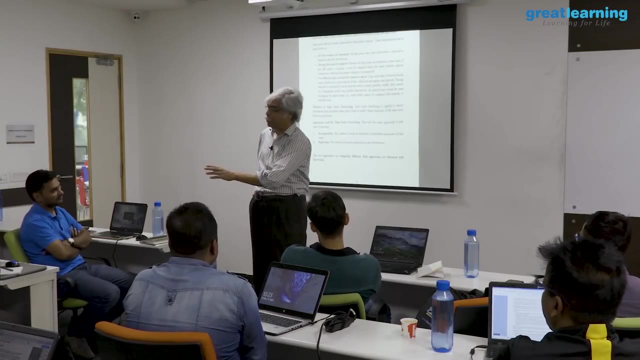 make this assumption. now, what is allowing you to make these assumptions you're going to? you're essentially saying that this is what it usually works out to be. this is what usually happens. now, if it doesn't happen, I'm going to protect myself for it. I may put, for example, certain safety margins around it, which is: 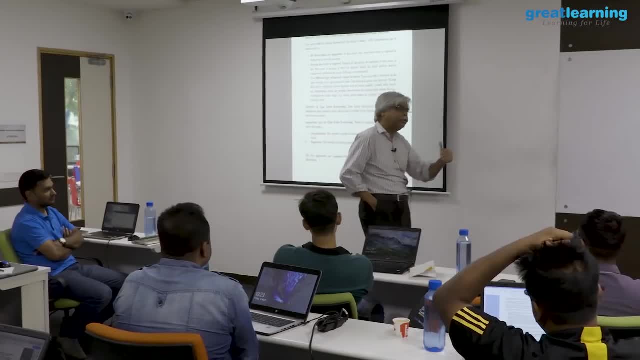 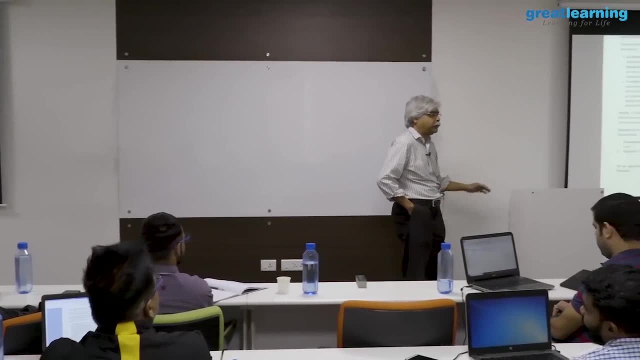 what confidence intervals are supposed to do and based on those I'm going to say I'm going to cross. if I'm relatively sure of crossing, I had a school classmate was very afraid to cross the road, probably in a statistical institute. the Barakpur trunk trunk road from outside Calcutta went through in front. 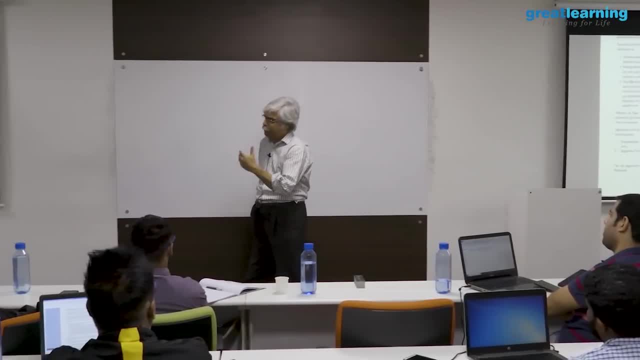 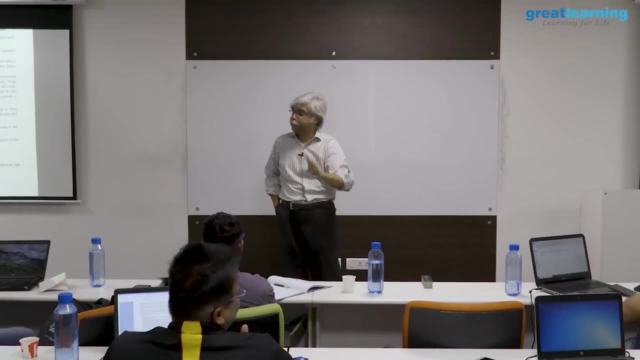 she was very afraid to cross the road so trucks would be coming. he was justifiably afraid. on this side we had college. on the other side was more interesting things like movie halls and restaurants and other inspiring places. so very interested in crossing the road. see, he began to cross the road. he reached about 80%, 90% on the 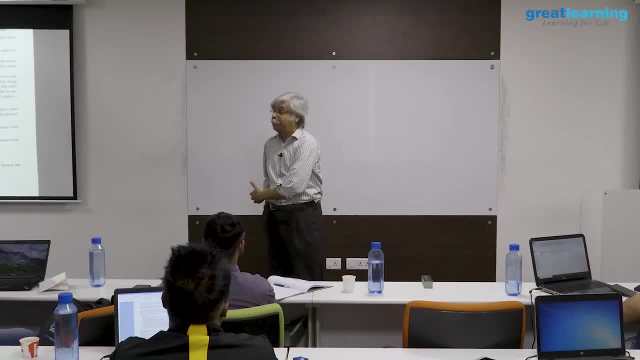 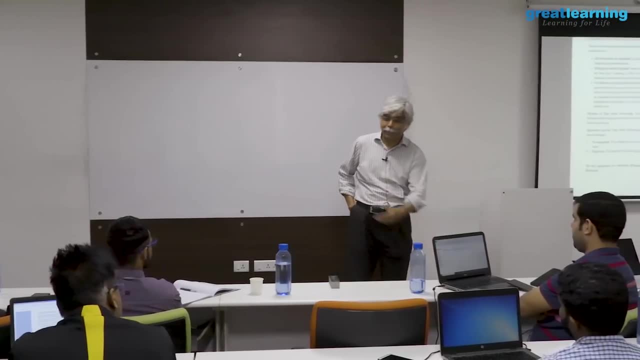 other side. and then he gets scared and run all the way back. so we tell him this is not the point. I mean you're increasing, you know risks of doing this, and to statistics students, you know we had fun doing this but anyway. so you make certain projections. so in other words, you do this decomposition all the time. 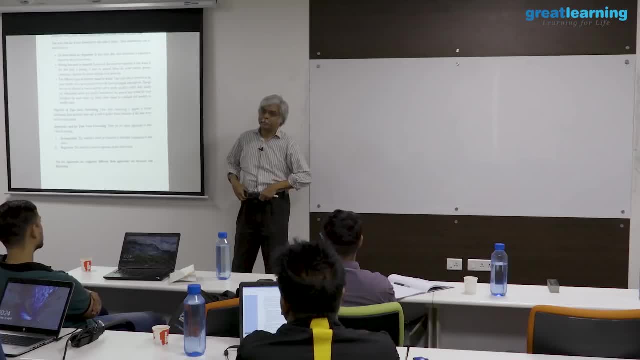 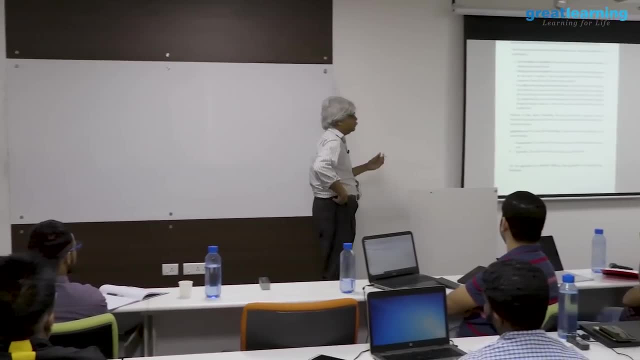 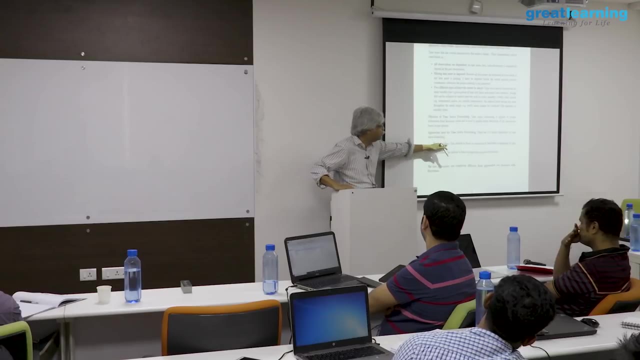 on a regular basis, on a daily basis, to figure out, to figure out what it is doing. how does how does it actually work, how? this is the way it usually works and therefore, this is the part that will be able to predict- and there'll be certain things that won't work all the time- and that is the part that I need to be able. 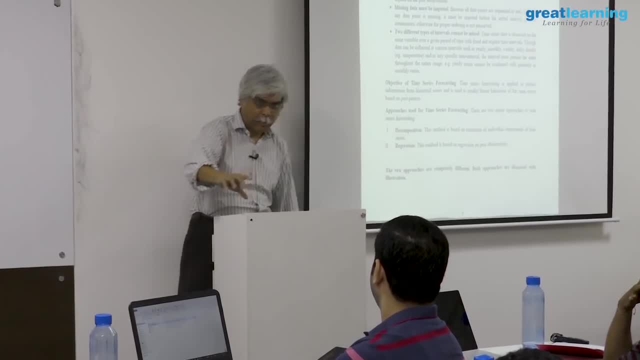 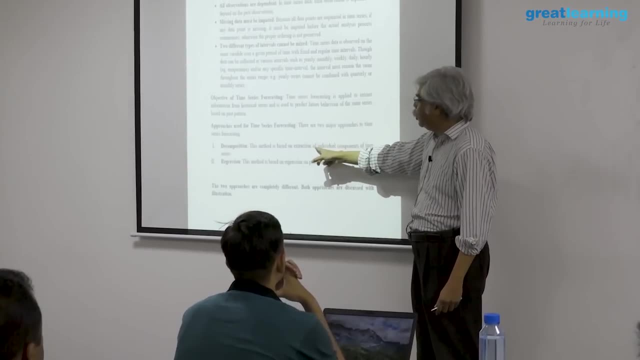 to ignore. so we will decompose it in that way and then we will decompose a little more interestingly. we will settle it on ourselves and we have to understand at what extent are we risk? let me go a little bit further and say that what about this decomposition refers to, let's say, a? 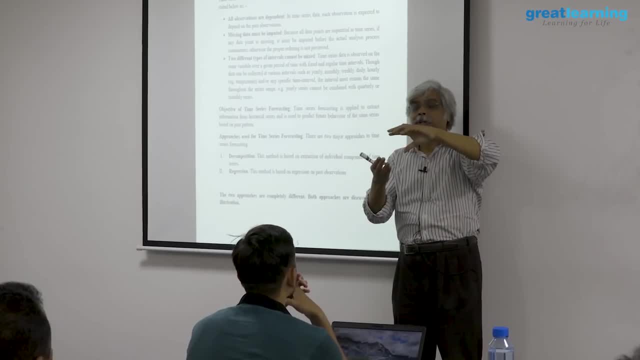 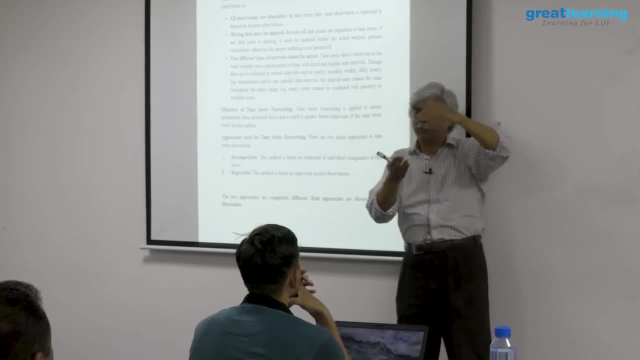 long-term trend. and what about this? decomposition refers to, let's say, a short-term seasonality. so what is happening over a longer period of time and what is happening over a shorter period of time? we'll do that as well. the second approach, which we'll do later in: 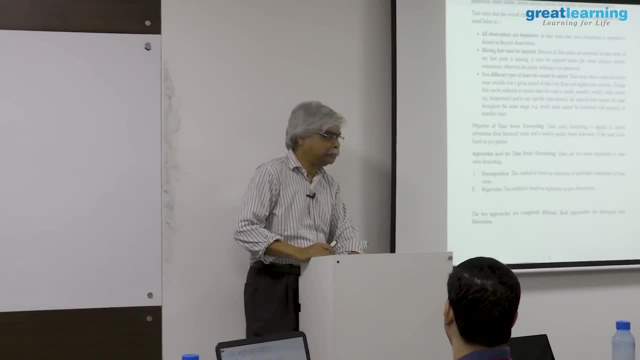 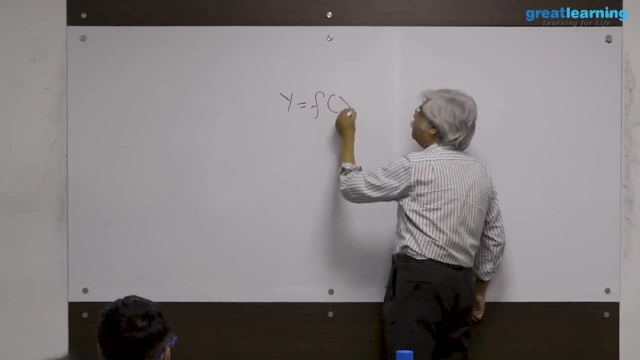 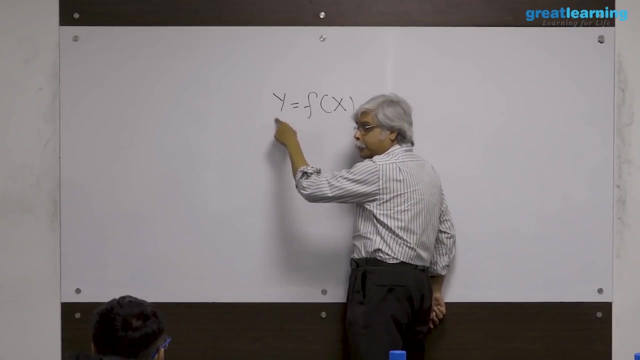 the course uses a slightly different principle. it says this in regret in in time series. in prediction, for example i looked at, y is equal to fx and the prediction problem was that if you give me an x, i will give you a y. now think of this from a time series forecasting problem. 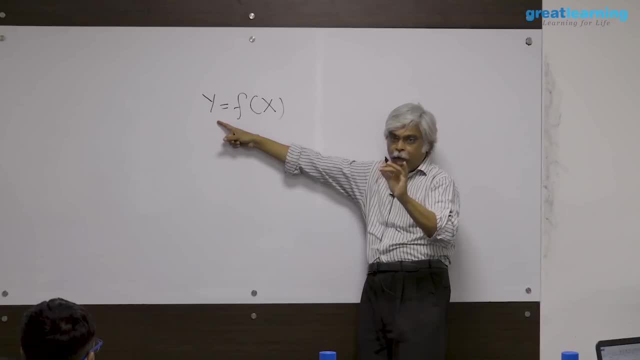 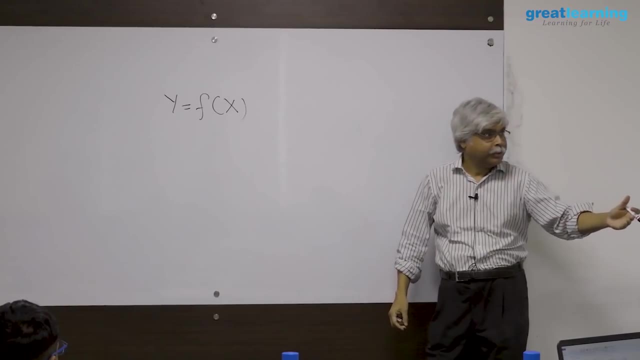 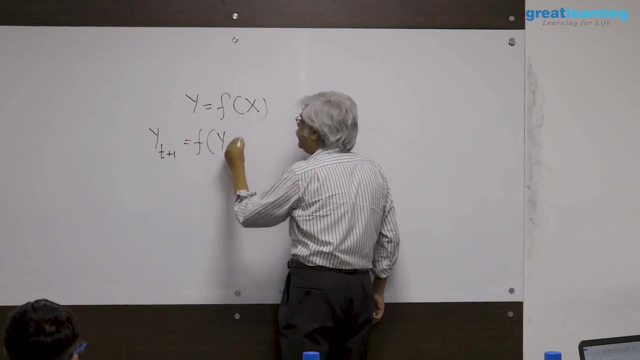 what is my y? my y is my observation in time. it's, let's say, the future observation. what are my x's? my past observations. so i can write an equation that looks vaguely like this: let's say y t plus 1 is equal to f of. let's say y t, y t minus 1, y t minus 2, etc. 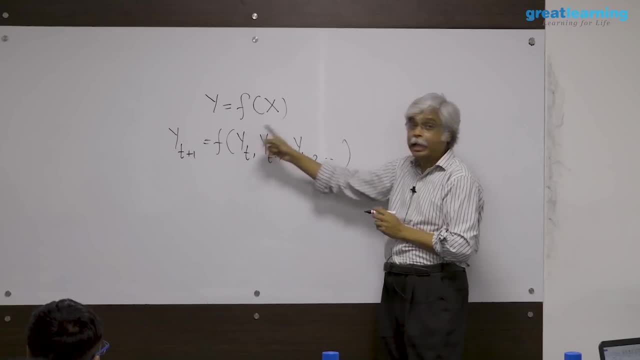 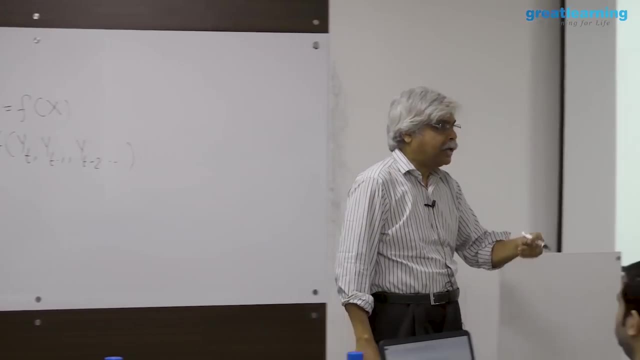 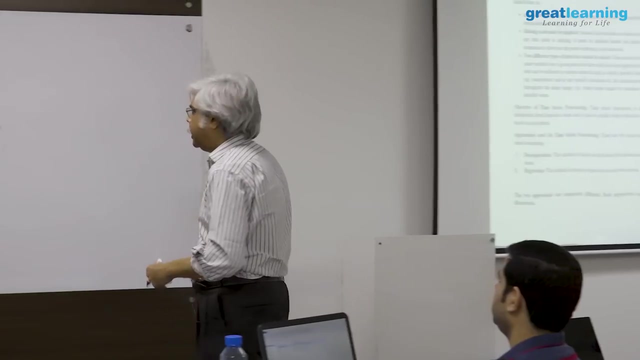 today, yesterday, day before yesterday. these are all my inputs, and my output is, tomorrow, what i want to predict. in other words, i can write the future as a function of the past. now, how would i make this work? i would say you know what, but i don't know. yt plus one. i'm trying. 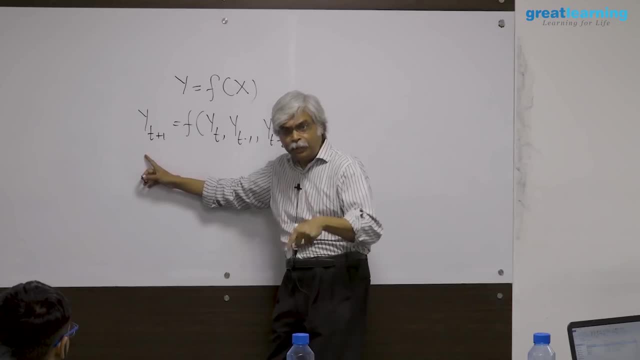 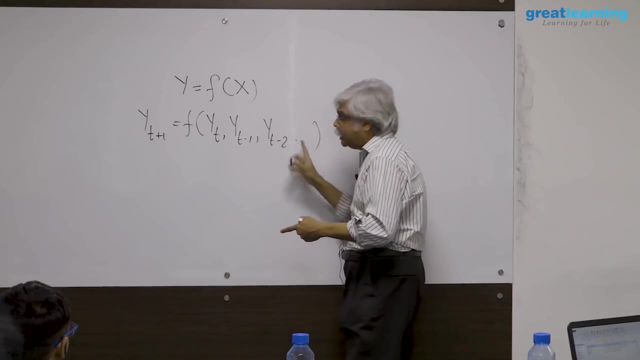 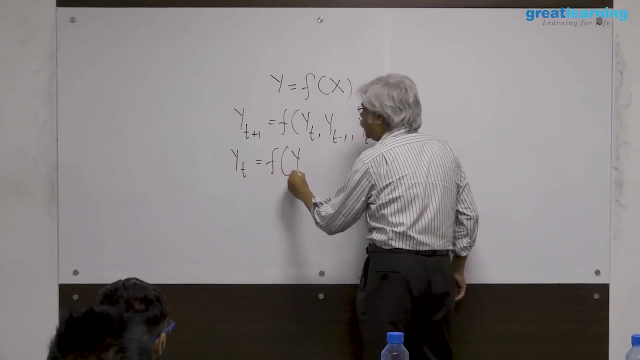 to forecast it. but if this is a model like supervised learning, in other words, there is an equation that- and this f applies to this data set- the same f can now be applied, for example, to yt. now, if i apply the same f to yt, i can now write it as yt minus 1, yt minus 2, yt minus 3. 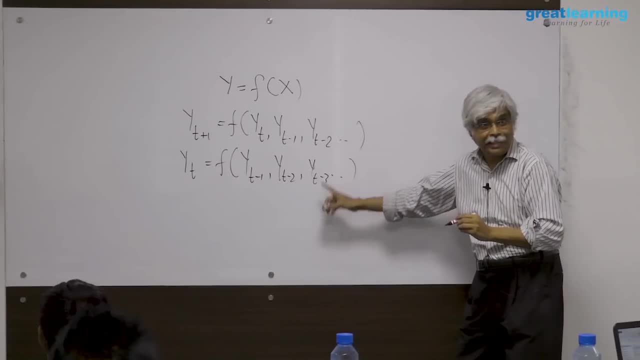 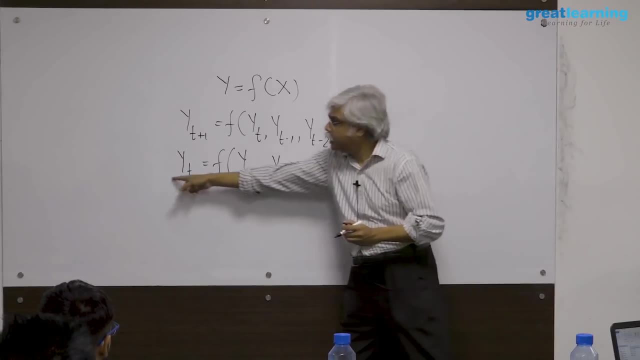 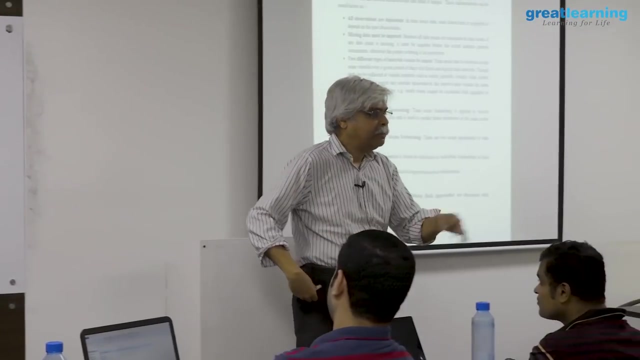 t minus 3.. do you understand? it's the same f, except that is now being applied from yesterday. now, written this way, i have the full data. essentially, i played a game. the game i've played is forecasting the future based on the present is like forecasting the present based on the past. 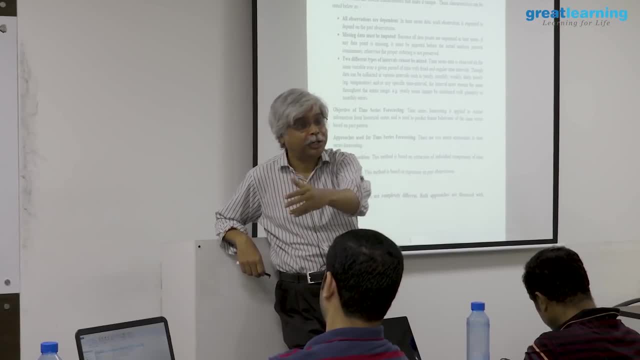 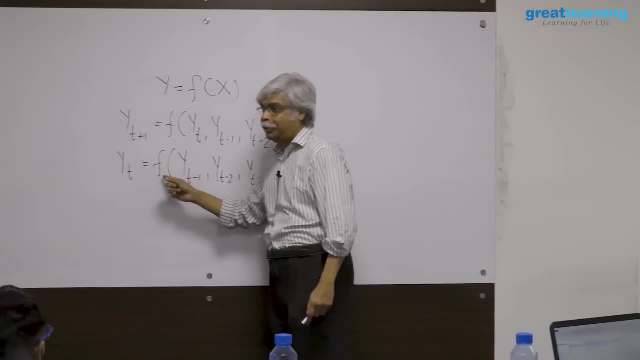 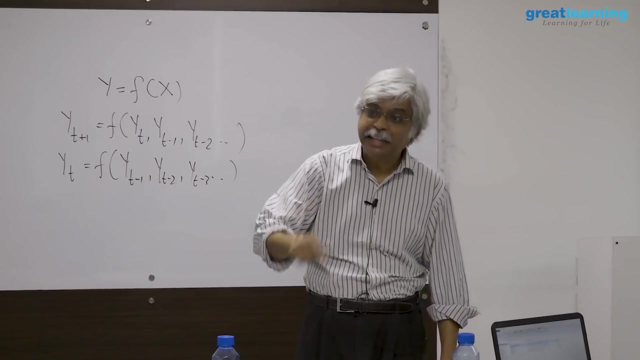 what allows me to do that is the principle that something about the future is the same as as present and in the past. in other words, I'm assuming that this f does not change. I'm assuming either that this f comes from population or I'm assuming that this f is something that has been tested through some kind of learning. 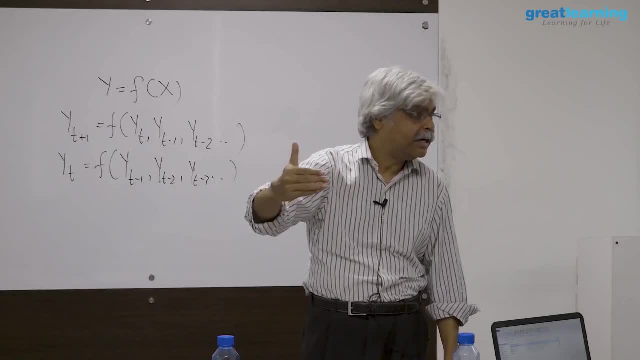 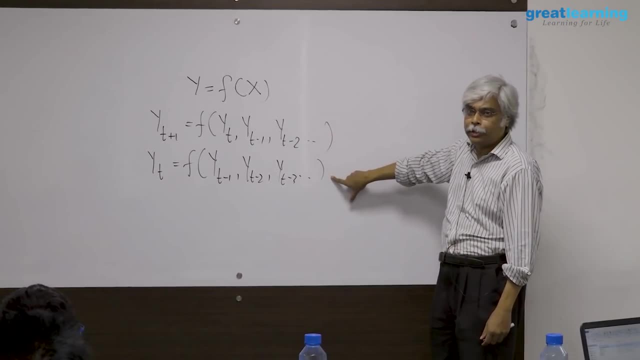 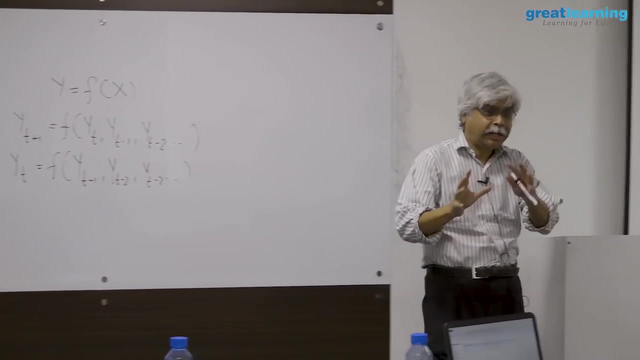 algorithm and it holds both in a test situation and in a training situation. this is that test situation and this is the training situation. now, the idea of test training is that the same f works. I validated in one and I'm using it in the other. why? because my problem is: 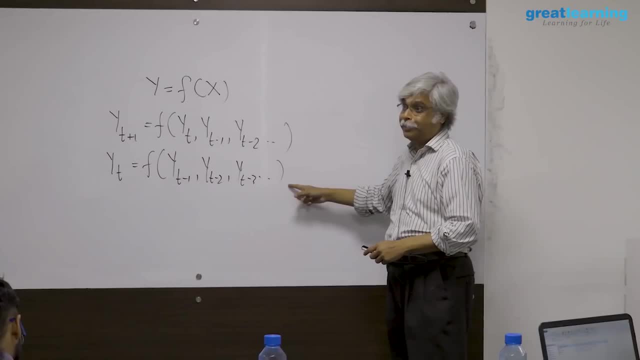 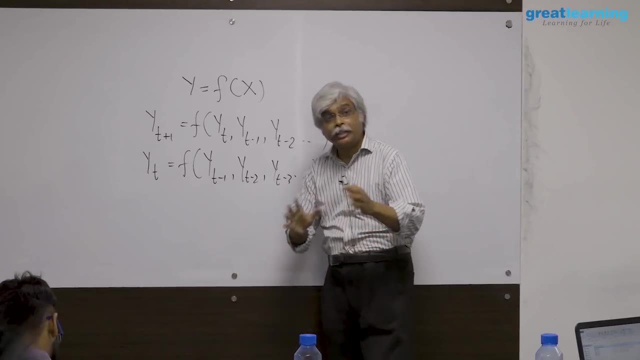 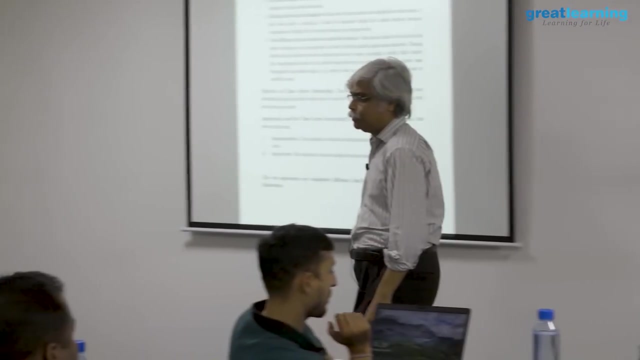 here, but my data is here. something must connect them. so therefore, if I can frame the problem this way, now, what has happened? now, what has happened is you give me a supervised learning algorithm and I will give you a time series forecasting algorithm. I will simply take my past observations. 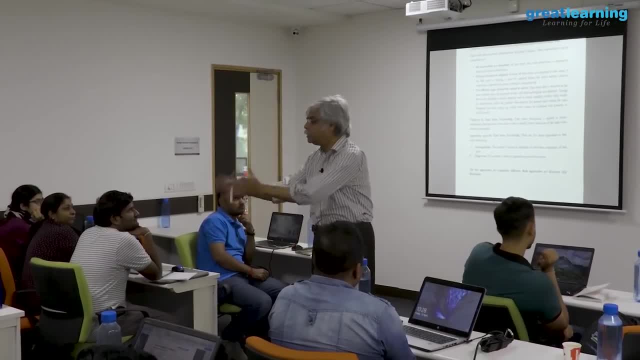 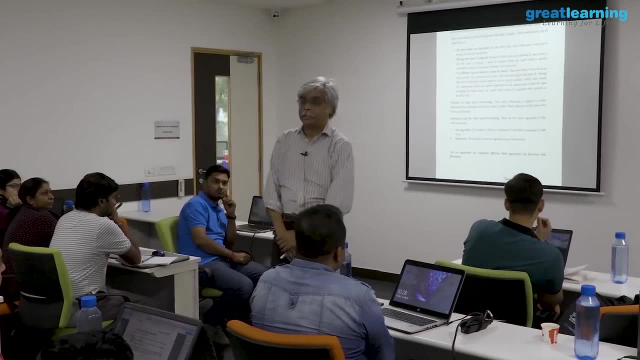 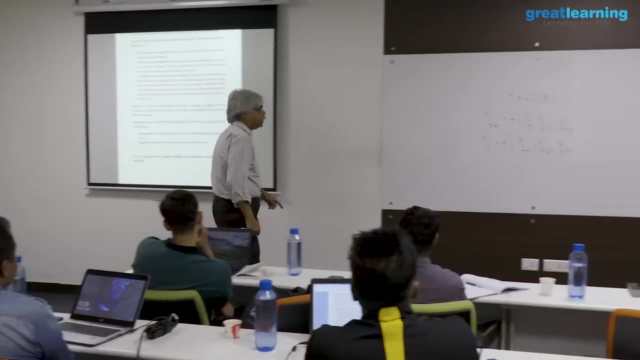 as inputs into a supervised learning algorithm. maybe that's a neural network, and people have done that: use neural networks to forecast. there are many, many such applications. what we will do is do something much simpler. what we will do is we will use this, but we will use this in the context of linear regression. 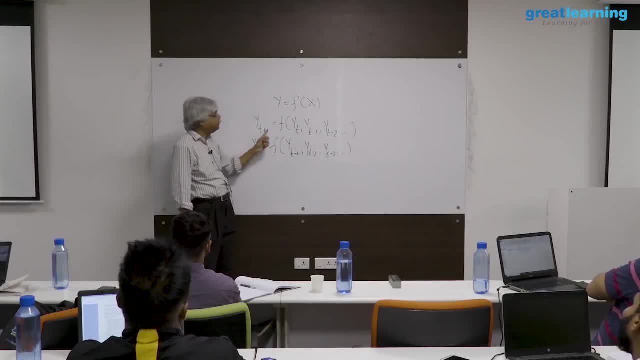 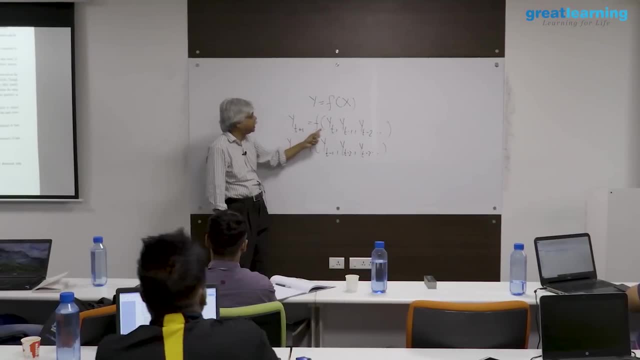 so what we will do is we will say: I will build a regression function of the future based on the present and in the past. sorry, based on the present and in the past. use it, the same regression function, to forecast the future, because this is a regression on itself. we're going to call this an auto. 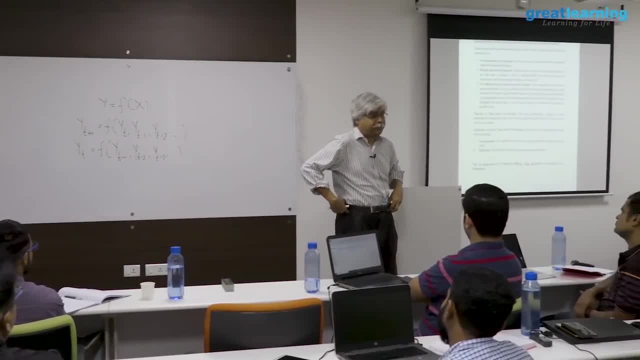 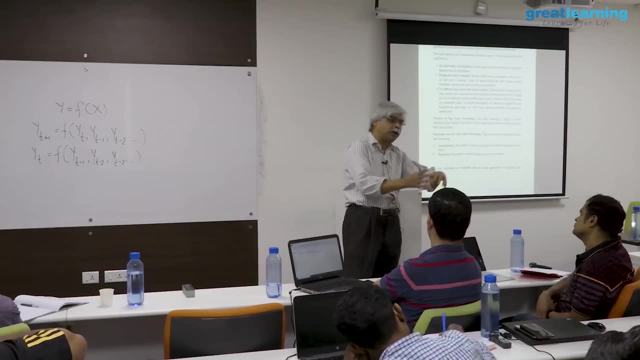 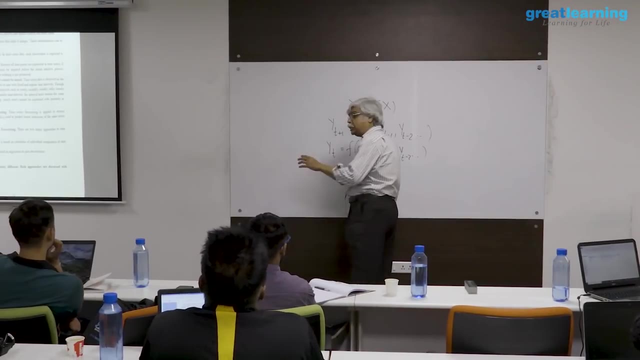 regression. auto means self, automobile is something that moves on its own, so auto regression is a regression on itself. you're regressing the same variable on itself, a different version of itself, its past, but the same thing. so essentially, you're learning from the data. so these are two different approaches. 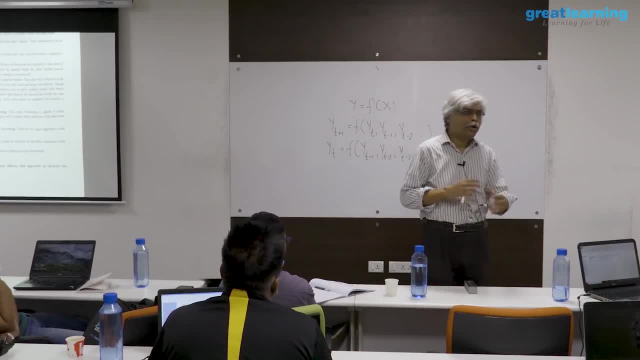 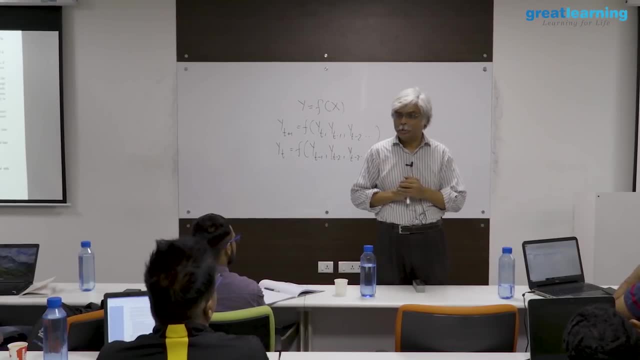 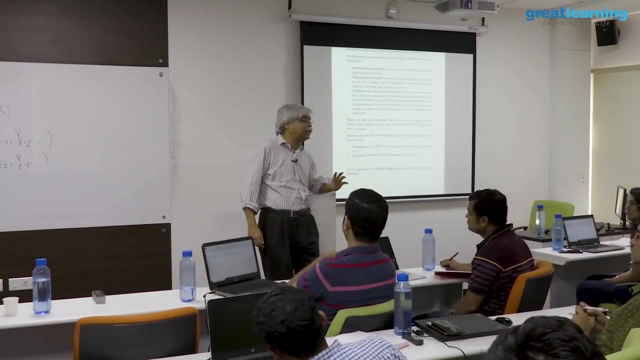 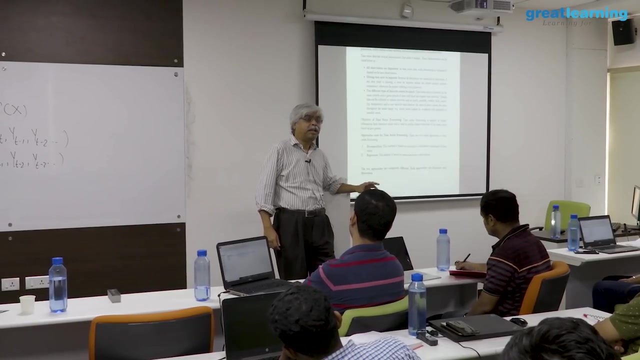 as you'll see there, they're going to be useful in different kind of contexts and they both are well used in practice in different situations. predict by decomposing into the known and the unknown the long-term trend and the short-term seasonality, or predict by building a supervised prediction rule. 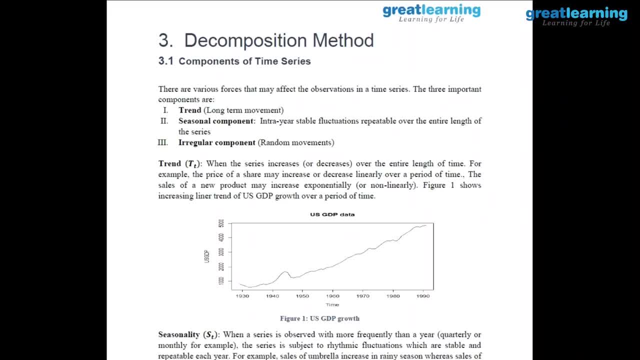 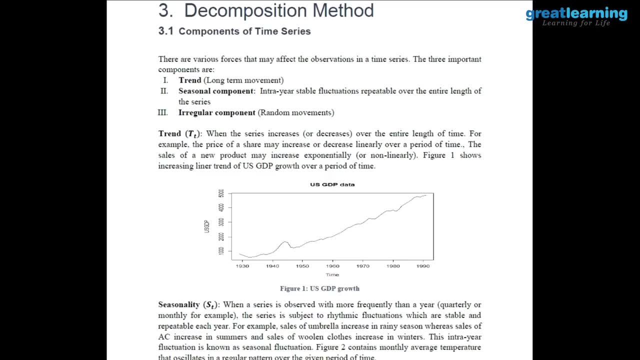 with the past as its input now decompositions. so when we decompose, we're going to decompose into a number of things. as I said, the first thing that we are going to decompose by is we're going to decompose into things that are random and things that are non-random- a regular- 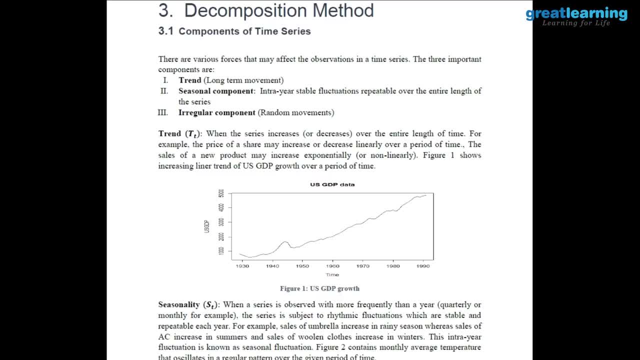 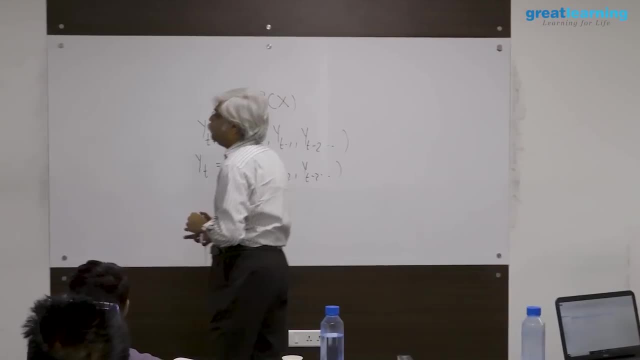 component and a irregular component. the irregular component is the component that will not play a role in the prediction. it's a random movement that happened before but will not happen in the future. the regular part of it, so to speak, can be decomposed further into many, many ways. 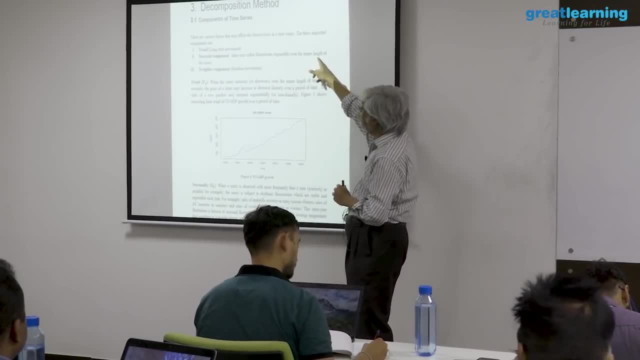 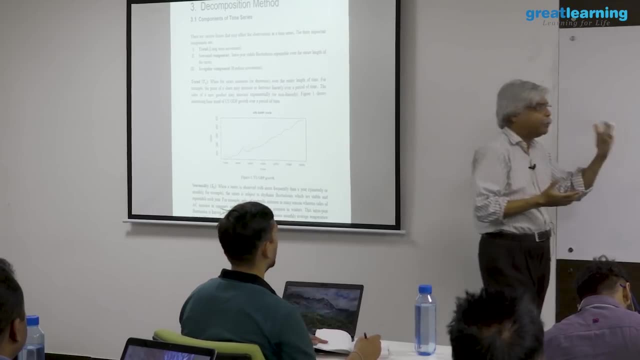 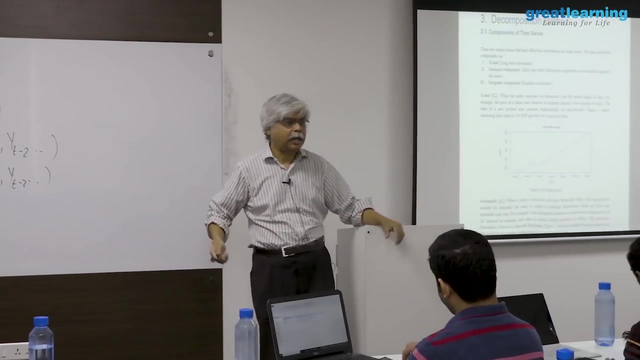 the version that we will be seeing, for example, talks about things that are long-term, like trend, and things that are more short-term, which are, which, for our purposes, we are going to call seasonality, something that goes up and down. for example, if you're looking at, let's say, air travel, there's a general 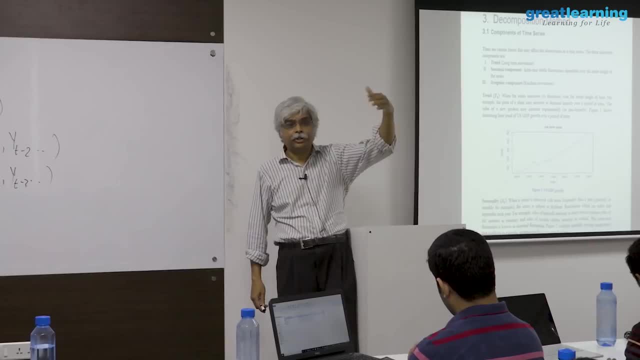 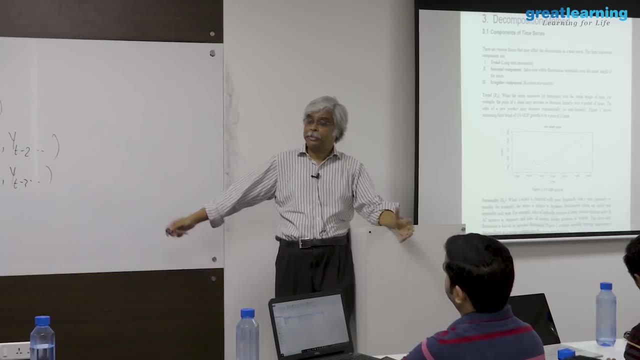 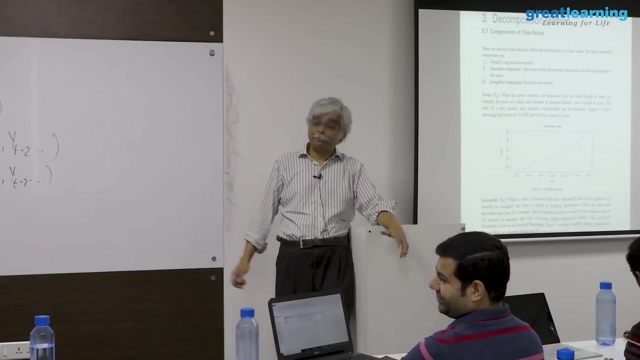 idea that air travel is going up, but there's also seasonality in the air travel. your expenses- what is the time series of your expenses- look like exponential. it should. it should, right. I mean your income should look exponential. your expenditure should look exponential and around that exponential. 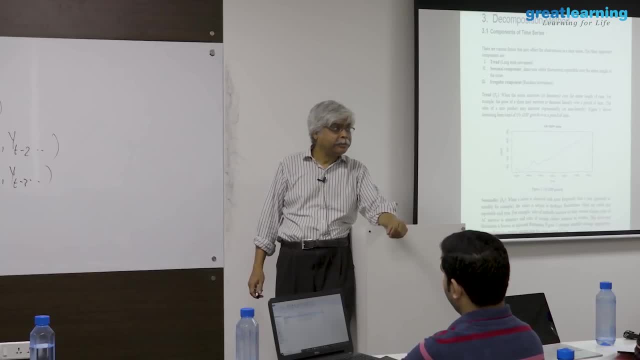 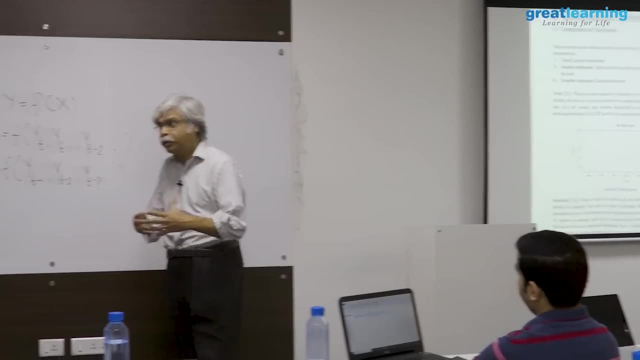 is it the same every day? is it the same every month? how does it vary? is there a seasonality to your expenditure? do you spend more at certain times of the year? for example, let's say you know summer times, if you have got kids or if you're? 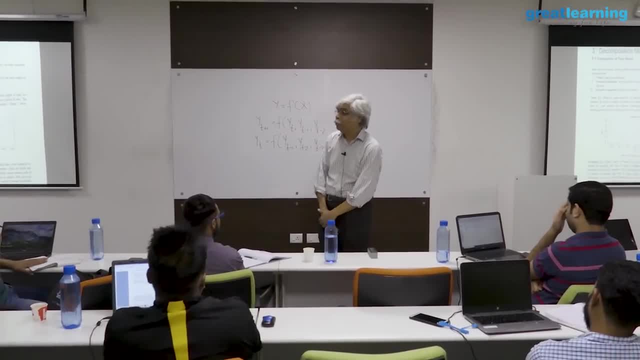 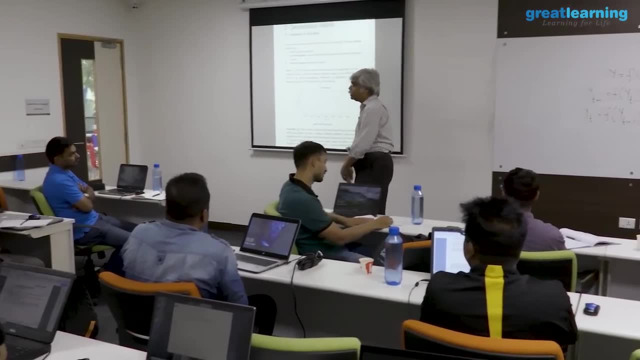 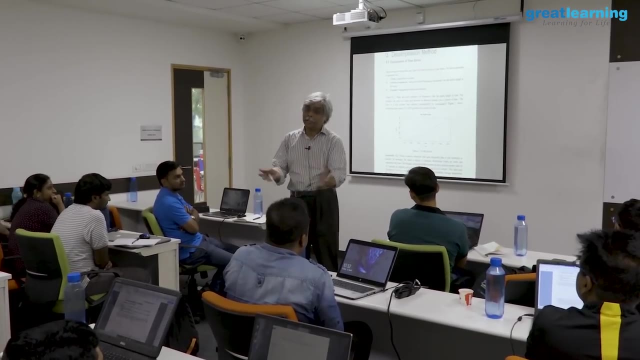 if you got extended family, there's travel you might do. there's certain festival times when you might be spending a little bit more. if you are an entrepreneur, then there will be a quarterly rhythm to this, making your quarterly numbers and things like that. so there may be certain things that are. 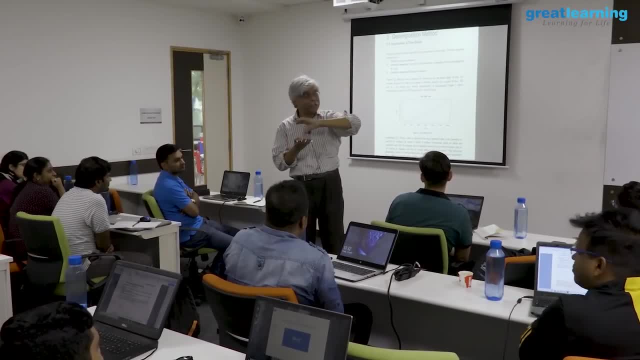 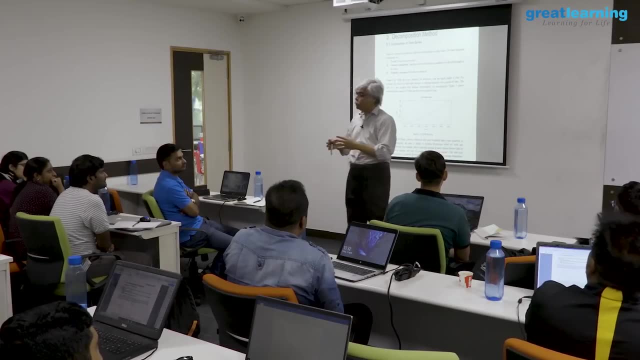 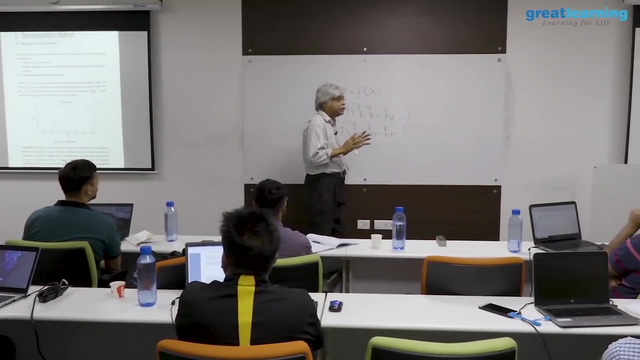 long-term. your expenditure is going up, as you said, exponentially or maybe linearly, whatever it is, and then there are certain variations around that. that variation is something that you are interested in managing now. sometimes the fact that there is a pattern itself could be a little bothersome, you would. 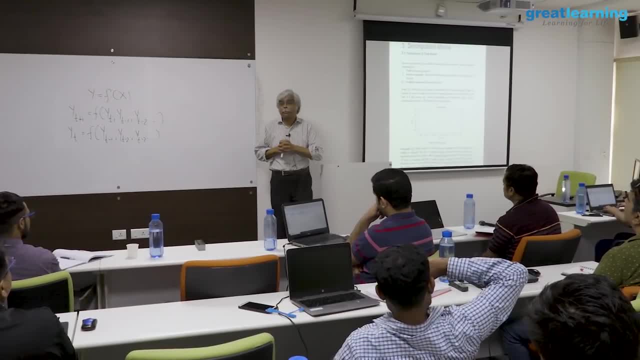 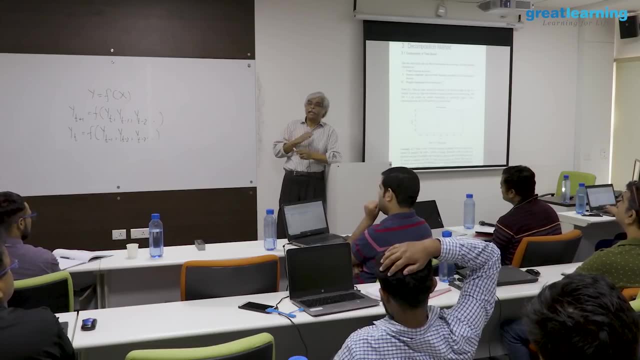 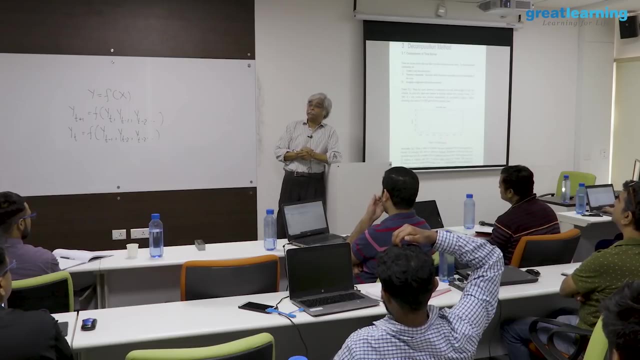 expect everything to some extent be irregular. for example, what should your blood pressure look like? what should your blood pressure look like? what should? if I take a blood pressure of your, of yourself, let's say every day, and I can, I do it for, let's say, a year- what should it look like? ideally consistent? so what? 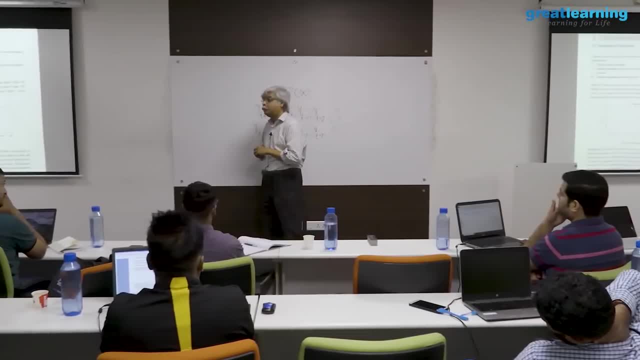 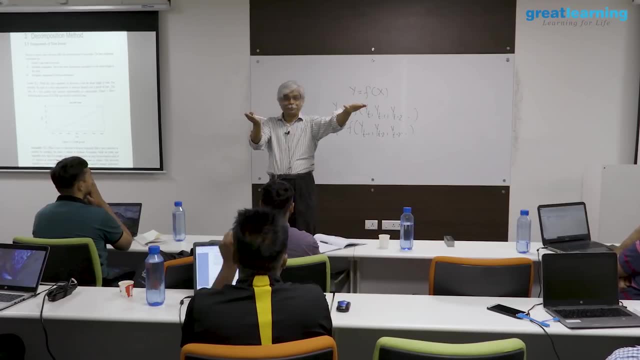 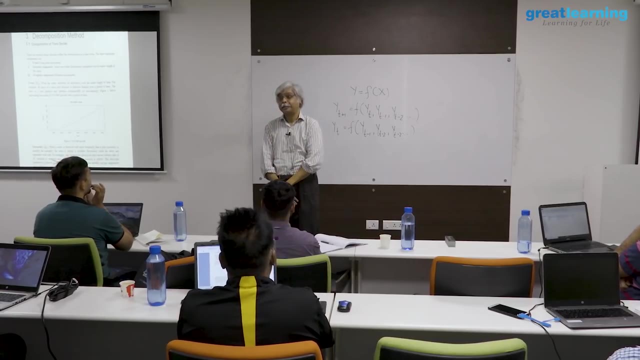 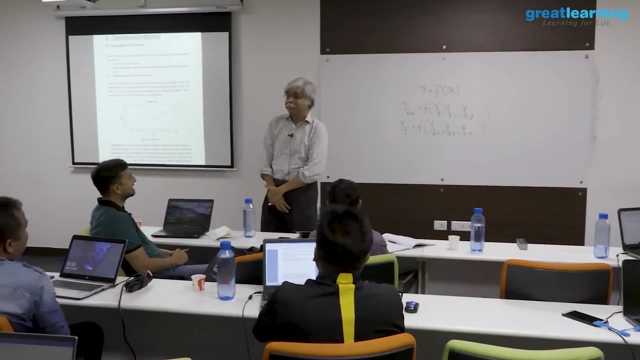 is the trend here? should it have a trend? what should the trend be? flat, so the ideal is it's flat, so mean shouldn't be did. so ideally you should say they should be flat. should it have any seasonality? but it happens. but it happens you if you are married for. 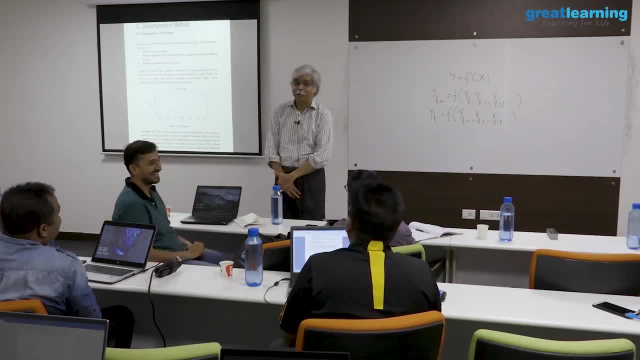 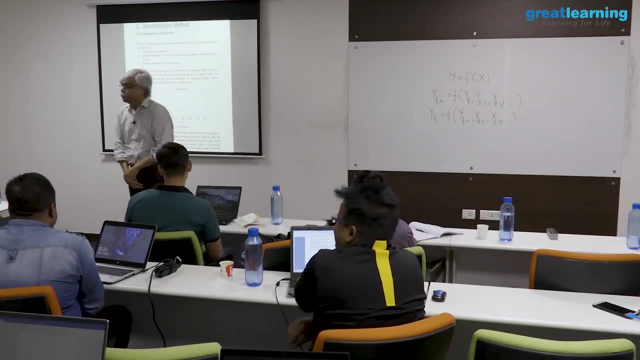 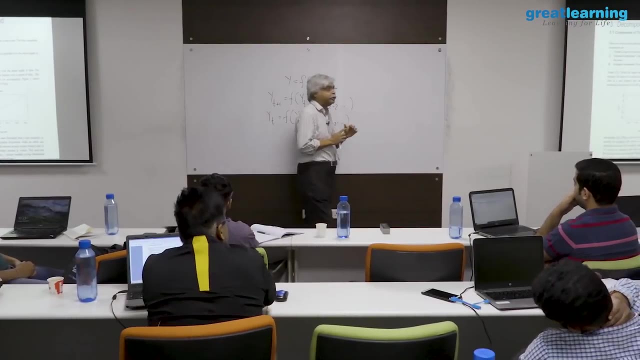 example, and you with your parents. that's one kind of blood pressure. you have with your in-laws that's an entirely different kind of blood pressure, maybe on a daily basis. but one objective of that could be, for example, one medical objective of that could be to really study, not that to understand whether. 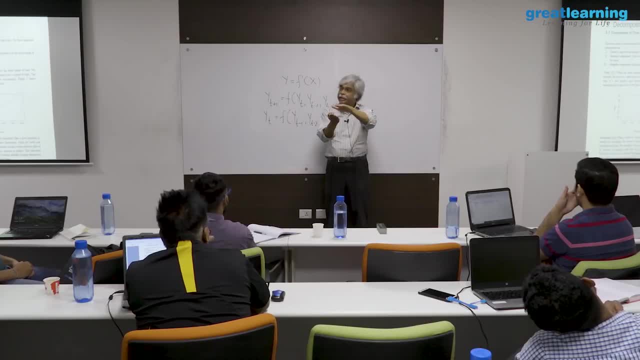 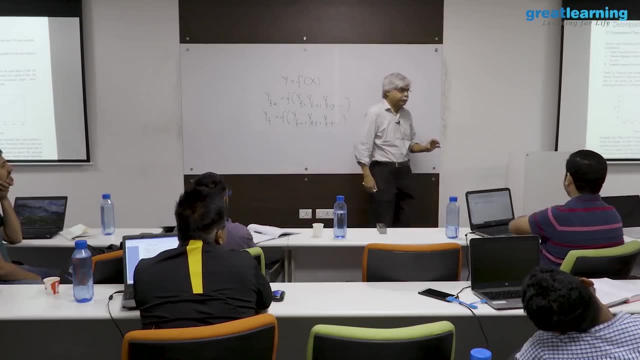 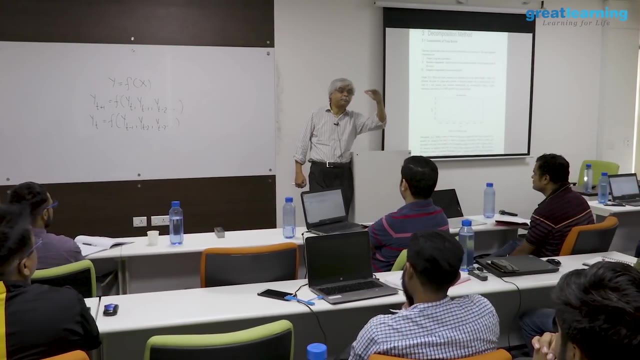 there is a trend and whether your blood pressure is going up or not, and if there is, then arrest that trend on a long-term basis. the second, also interesting part is to control. the irregular part is essentially to ask the question that: is your blood pressure also varying too much? you know, this is spiking, or is it? 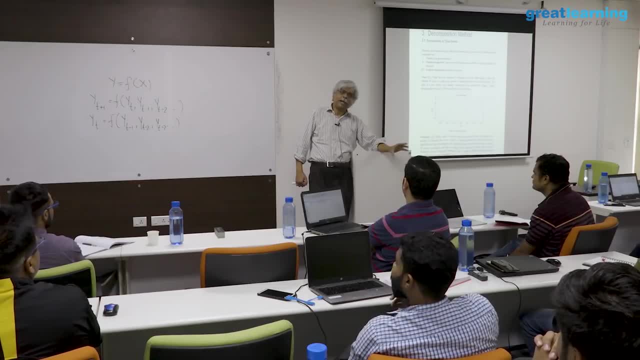 going down, which is what people often ask. this is done for many biological signals, for example, is done a lot more for blood sugar. I hope none of you are diabetics, but if you are a diabetic, then you are measuring blood sugar regularly and what the doctor is looking for is not just what the level of is, but 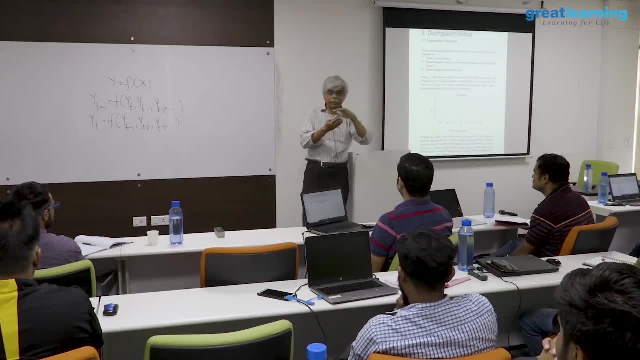 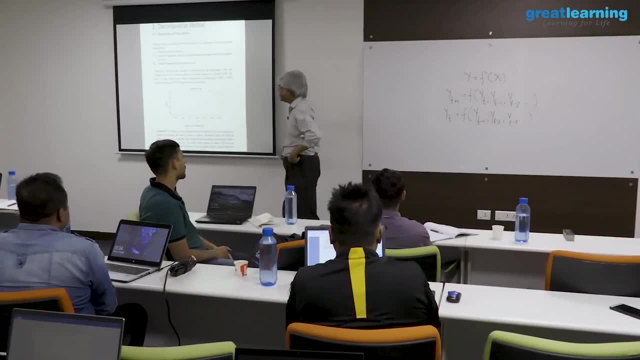 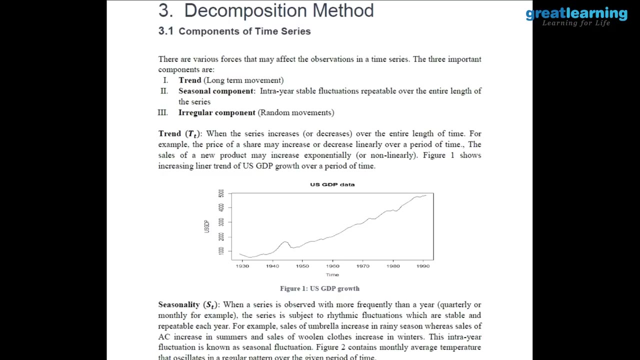 whether there are spikes and to keep it. keep it below those spikes. you know it becomes very dangerous when it sort of she shoots up, it comes down. even a blood pressure is the same thing. so there are times when you are very interested in understanding this or at least keeping this under control in business. what does 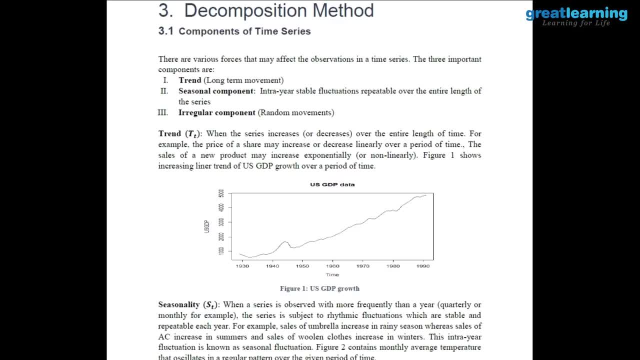 this mean in business. what this means is: let's say that you are selling something. why, I don't know. let's say that you are selling something. let's say that you are selling something. let's say that you are selling something. let's say that you sell sweets. you have a sweet. 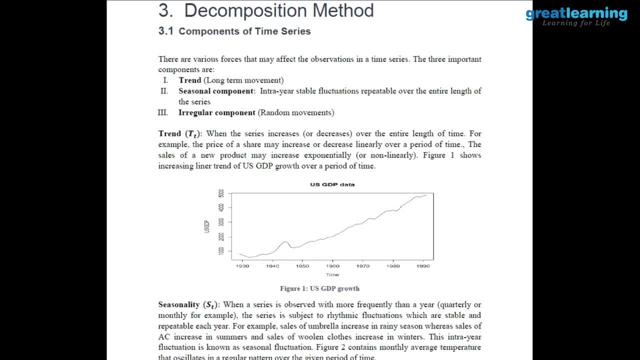 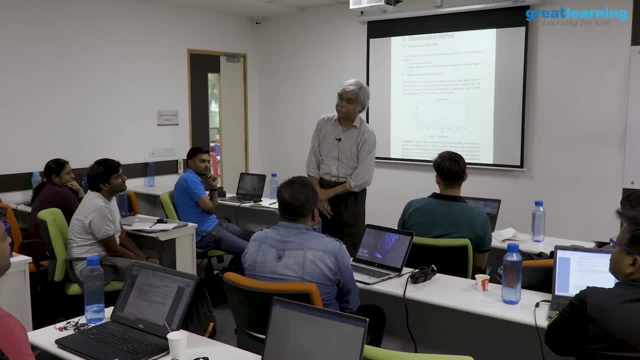 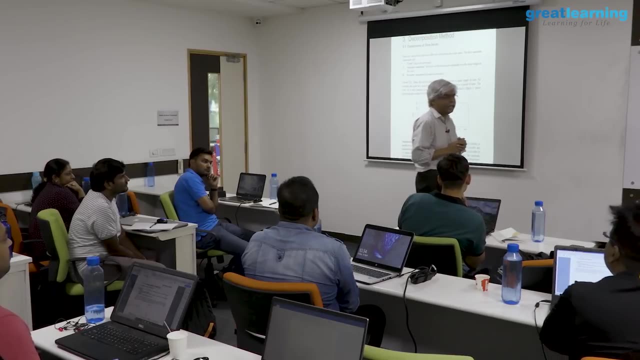 shop in Bangalore and you're selling sweets. how much sweets do you expect to sell? seasonality? this is important to know because, first of all, this will dictate how many sweets you have. let's say it's an ordering principle. in others you're trying to decide on a daily basis how many sweets should I, should I get in? 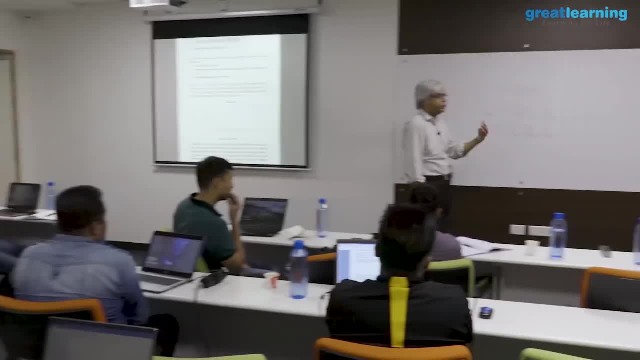 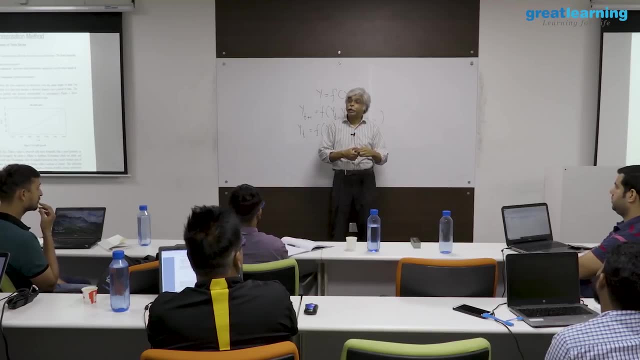 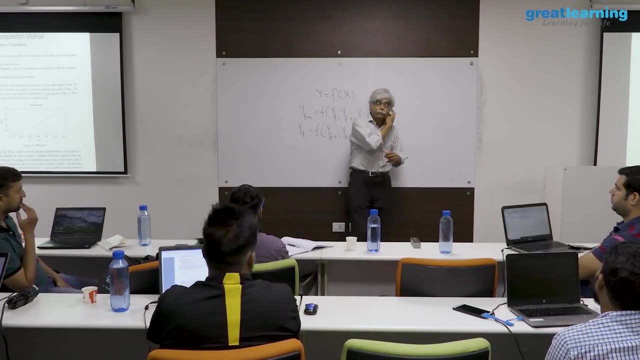 today. so now you're going to, now you're going to look at sales. now this sales is going to look like what it there will be. will there be a trend? okay, think about that. you got one shop. do you want to trend upward trend? you want more people. 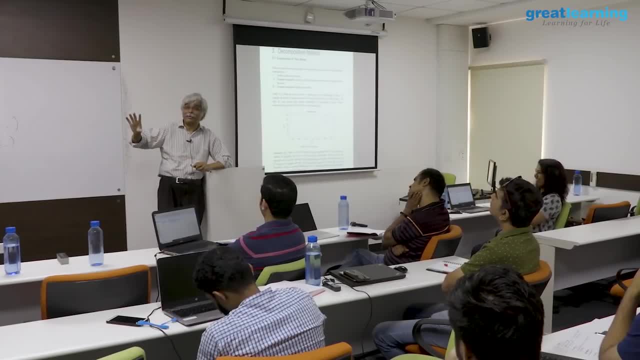 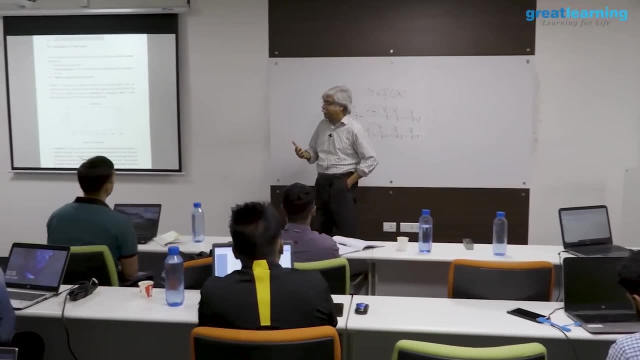 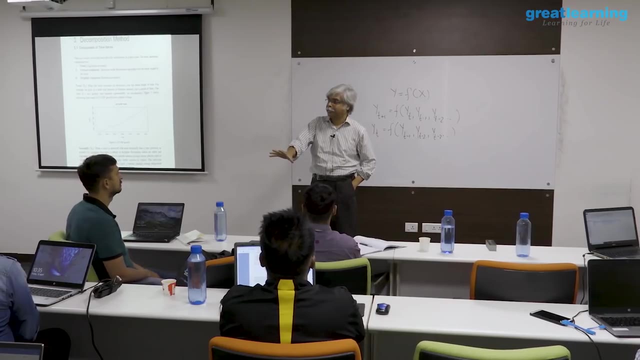 like I picked a complicated example, but you will do a supply chain exercise later, etc. if you- yes, if you have too much, if you're projecting too much growth, then there's a question of saying that how much will I be able to sell and keep in this particular store? and if you are now saying that my trend is going to be: this every day. you bring in so many sweets and by the time you are, say in the middle of the day, your sweets have all run out and now you're losing market, losing customers for the second half of the day but you can't get more sweets in. 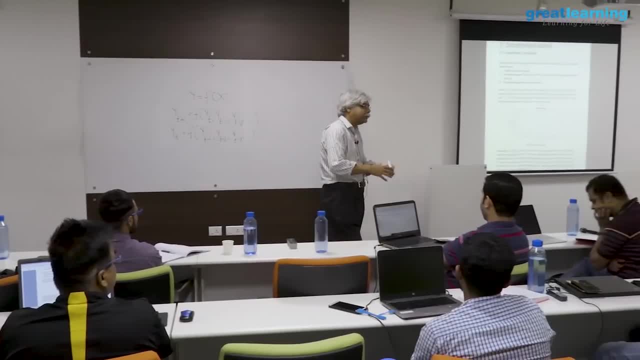 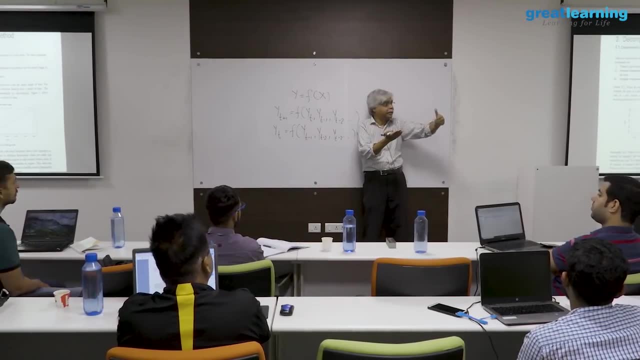 because you can't, where will you keep the remainder of the sweet? so there's there's different question there, but there's one set of quick, one set of questions that deals with whether you have increasing sales or not. then, as you were saying, a seasonality, there are certain times when you will get to see. 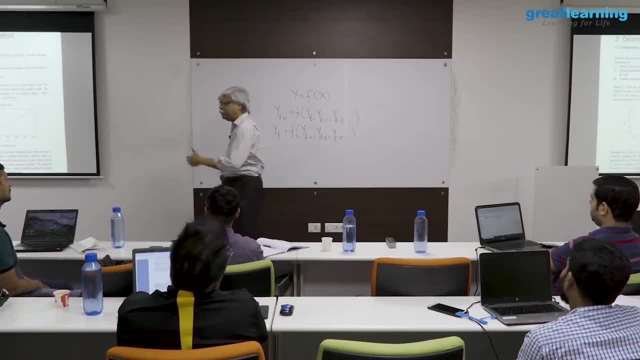 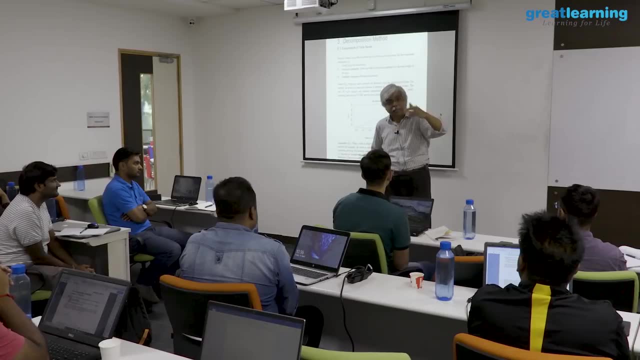 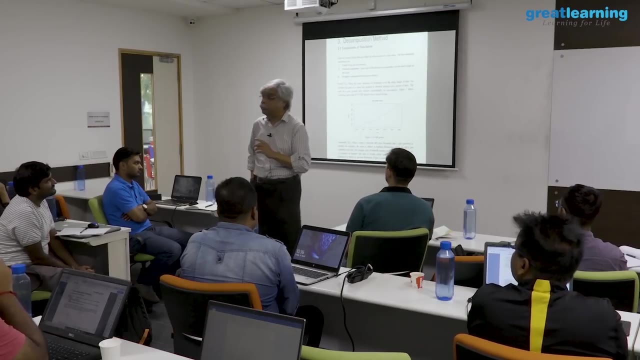 more sales. festival time is Ganesh Chaturthi, whatever festival that you believe in. so what he just went by, so the. so there'll be festival times and then what else? what you're worried about is, in some way, the random spikes, the unpredictable spikes that you see in scale, spikes in both directions spikes. 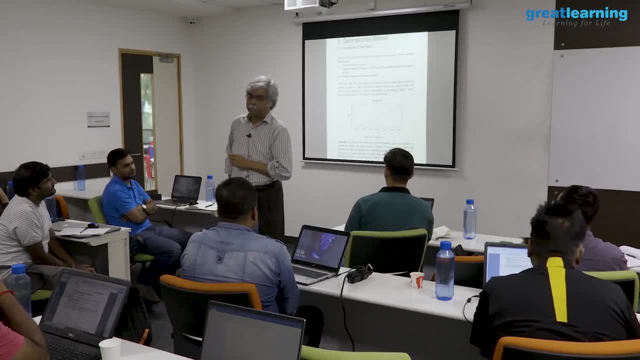 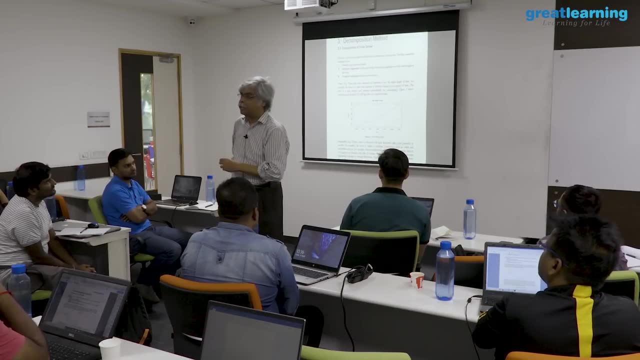 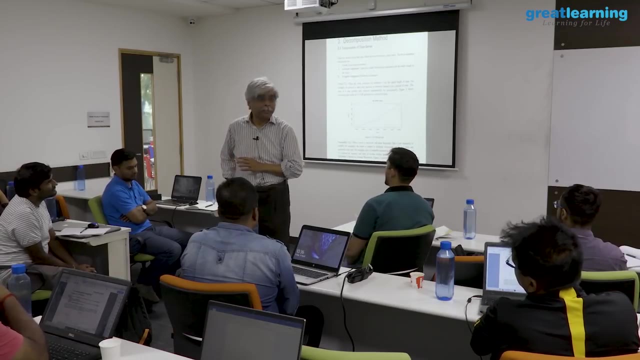 up as well as spikes down, which could be caused by a number of things. maybe something that a competitor is doing, maybe something went wrong with your suppliers, maybe a parking issue in front of your store, maybe a behavior issue with one of your sales per people, environmental issues. the sweet doesn't last that long. 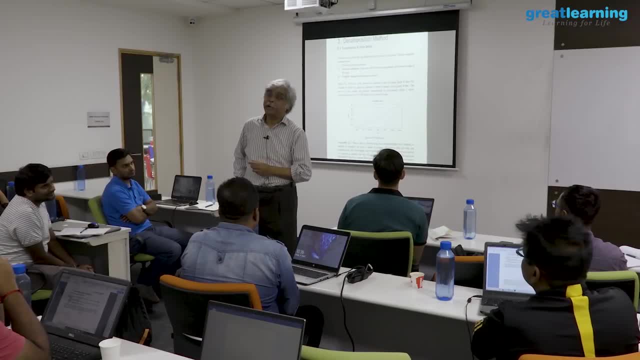 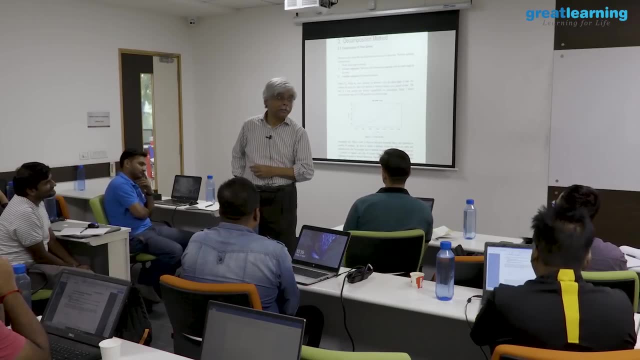 on that on that given day, or it is raining too much, no one's coming in. you can't forecast the rain that much, but if it's raining all the time, so one's going to come in, I'm sorry. India wins the World Cup. that's. that's high sales, or? 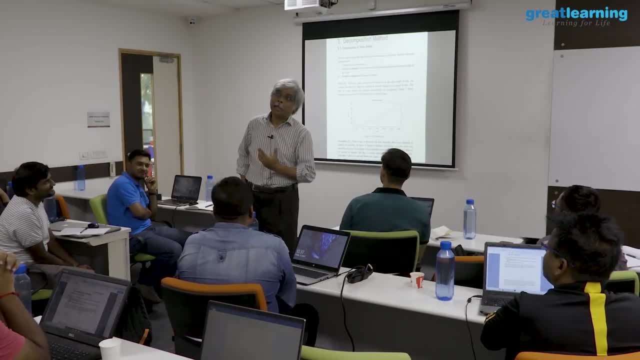 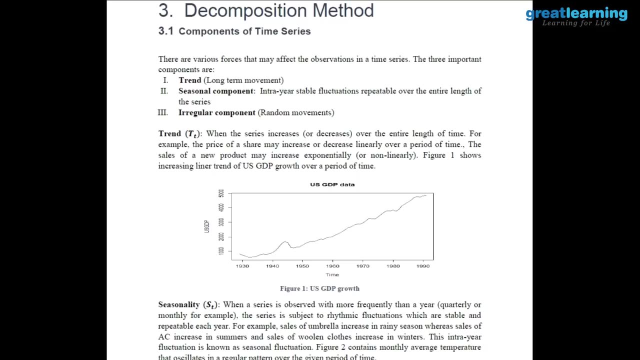 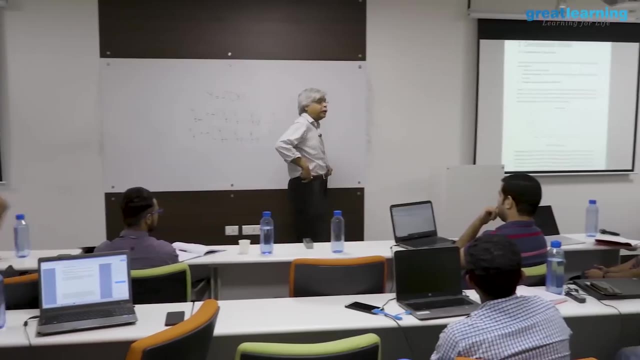 low sales. well, that's high sales after the fact that mainly to low sales a little before because everybody's watching the game. so I remember growing up we would have on Sunday mornings we would have the Ramayana and the Mahabharata on Durdarshan, and at that time 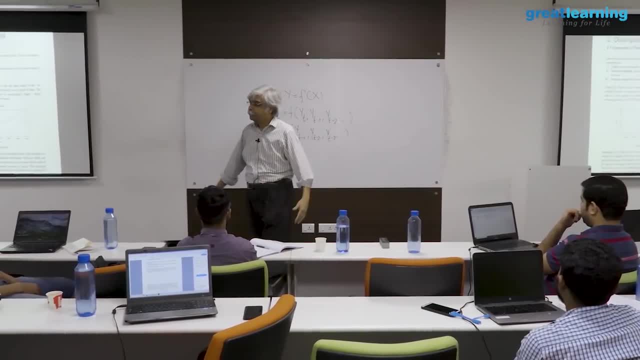 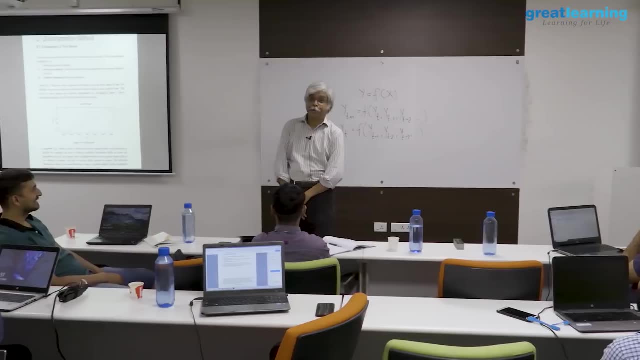 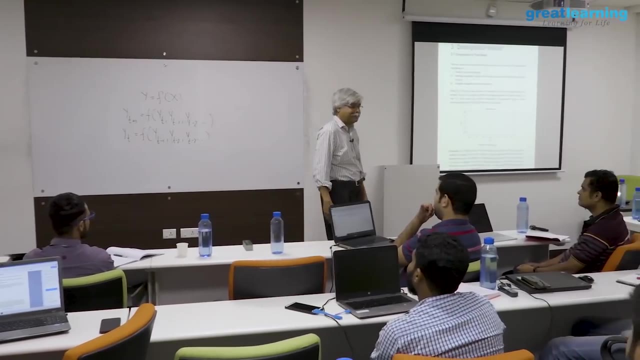 particularly, I think, when the Mahabharata came, the the neighbor will be deserted. everybody would be inside seeing, seeing television right on a Sunday morning and if you know Kolkata, any of these cities, on Sunday morning at about that time that's actually fairly peak shopping time. people are going out and they're 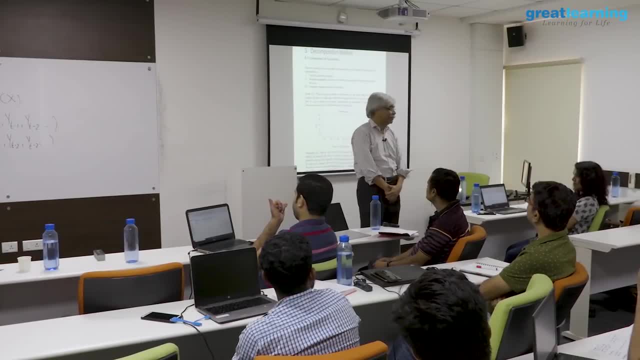 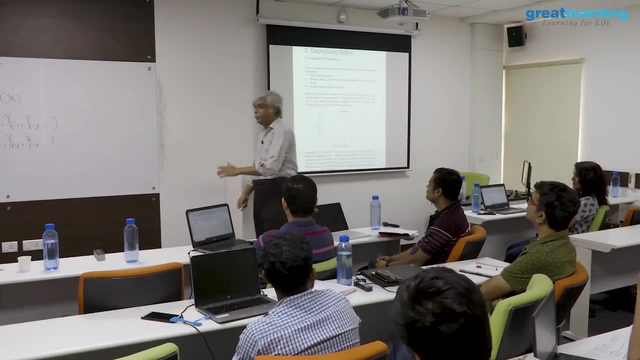 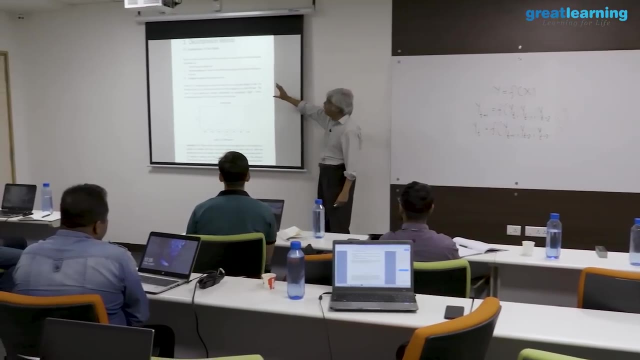 doing the visual shopping and markets would complain that this is not something. but soon, soon, they figured this out, but this is what's going to happen. people are going to come before or people are going to gone after. so the irregular component is an important component to to to have a handle on and 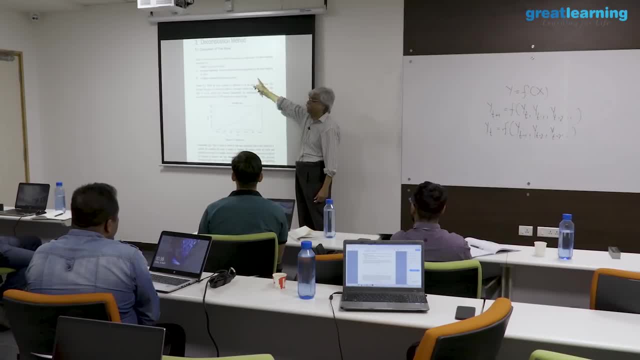 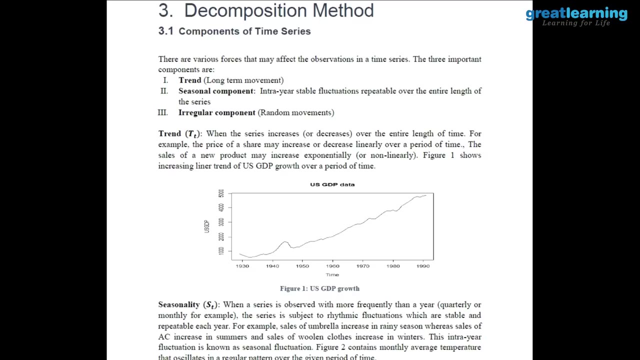 in many domains. this is the part where most of the fun is, for example, in finance. now, in finance, very little is predictable. stock prices are they predictable or they're not? not with guarantee, that's true. that's true. but what happens to stock prices? let's suppose the stock price is. 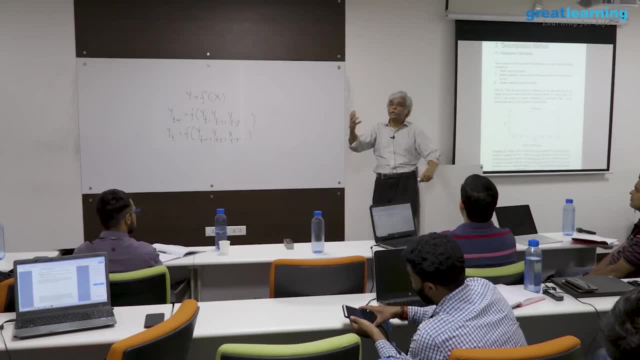 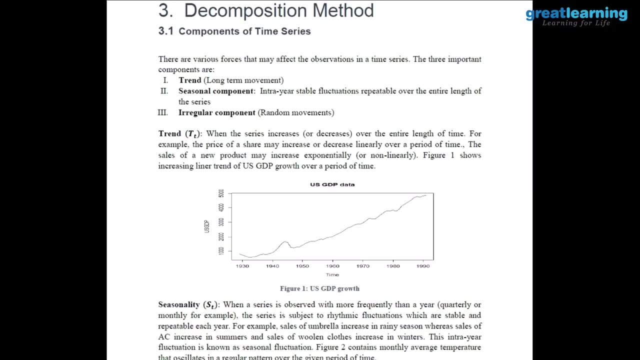 going up, what's going to happen? so think of it just as a product. so there is a product which whose price is going up. now what will happen to that product? so so people's people who says price is going up, some people who have it will now want to want to do what with it. we want to sell it right now, when they sell. 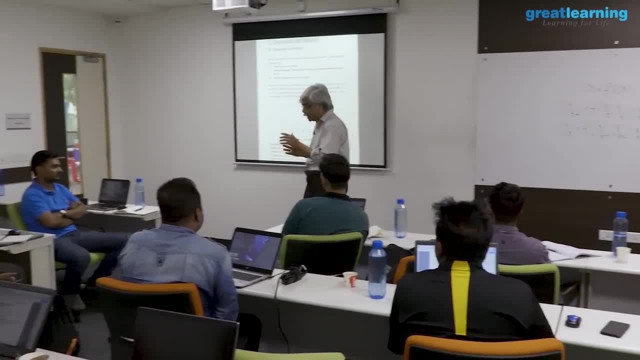 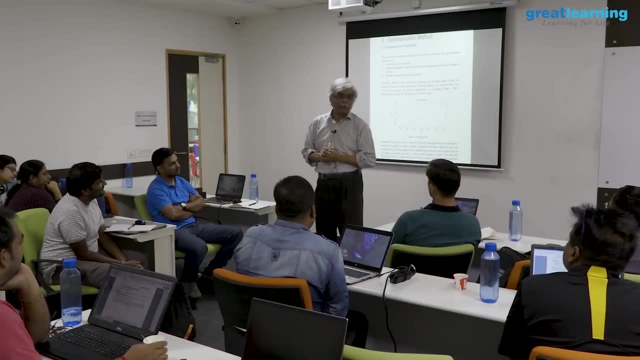 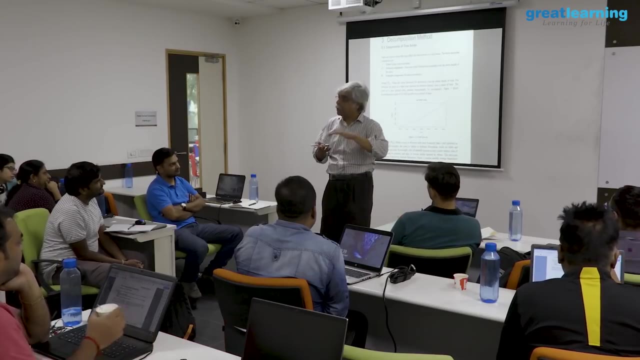 it. what will happen? and therefore the price will come down. so when the when the market goes up, it wants to come down. when the market goes down, now what happens? now it's cheap, now people won't do. we want to buy and the market will go up. so essentially, the stock market is. 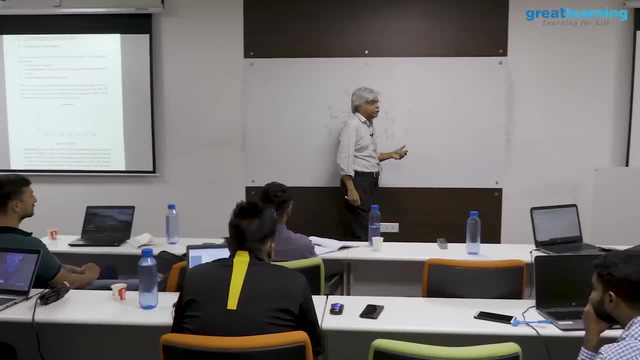 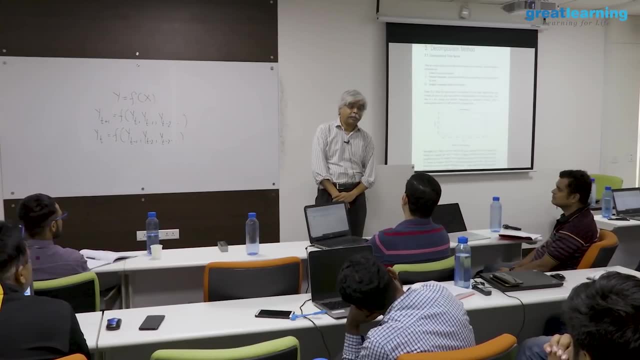 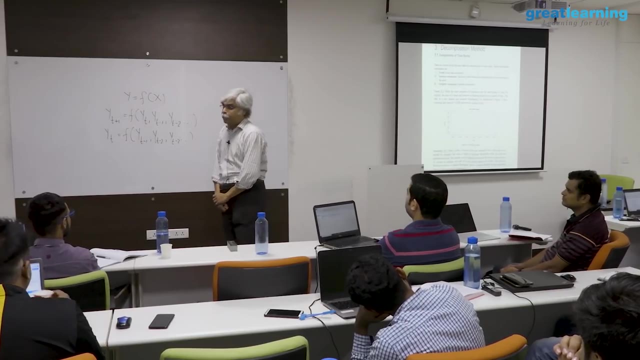 going up. it's cheap and that's why you see that there is this trend and people are going to take advantage of it. and it's a very controversial thing where, if there is a trend, then it is expected that people will take advantage of the trend and we'll make money for it. so this is a very controversial theory. 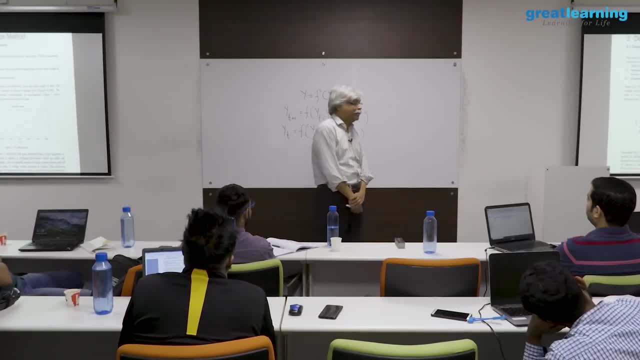 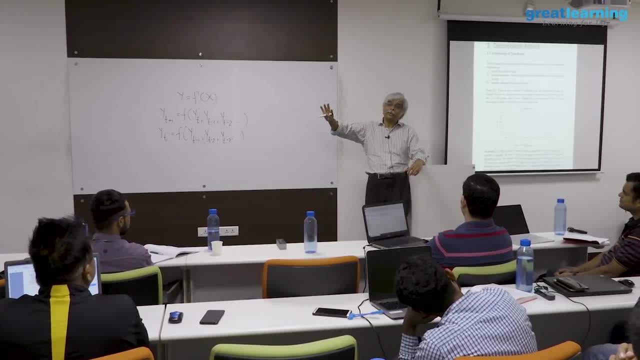 right. there are people who agree with it and get Nobel Prizes. there are people who disagree with it and also get Nobel Prizes in the same year. such things the trend, but not over long periods of time. you can't. someone will catch on, or the market will catch up, so to speak. as I say in the in the financial world. if 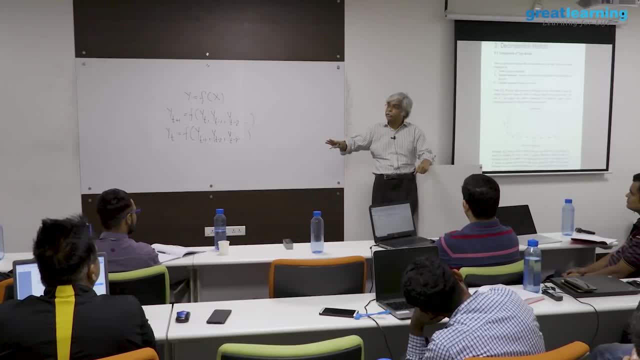 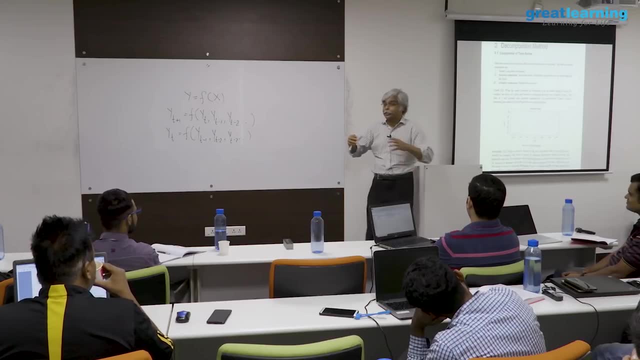 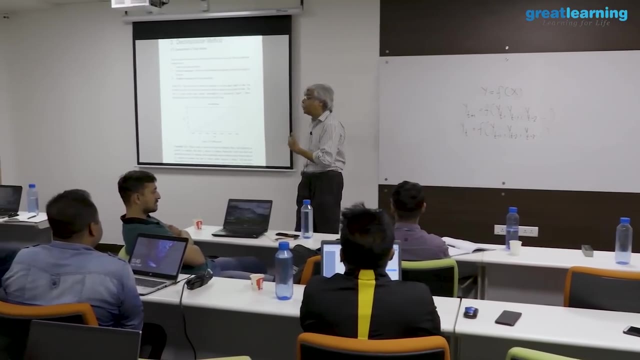 you and your friend are being chased by a bear. you need to run faster than your friend. you can ignore the bear. so, therefore, but the irregular part, the part that's left behind the volatility, is a part that nobody knows how to reliably make money on, and so what you're looking for is not the trend. 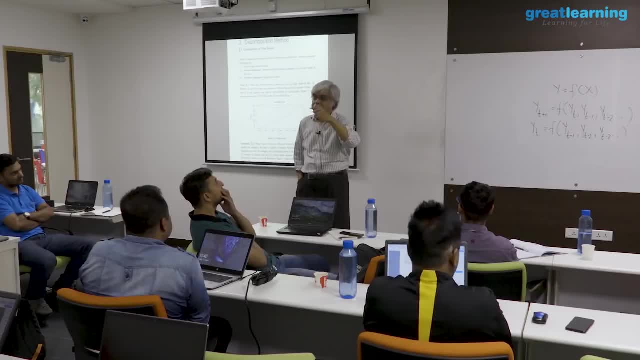 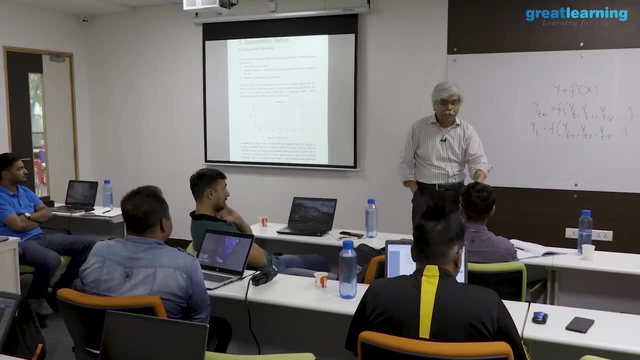 you're looking for patterns in that, then what the data is telling you is irregular, because you are understanding that this is not predictable. it not being predictable means what? it means that when he predicts and when he predicts and when I predict, we predict different things. in other words, it is 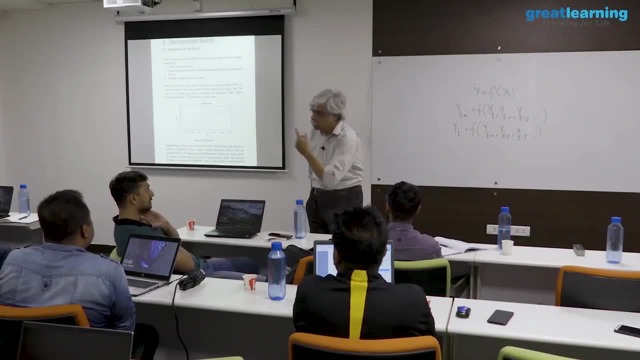 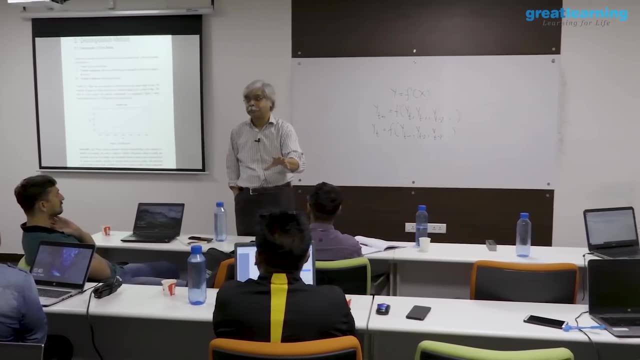 irregular. but what does that mean? it means that if I predict something, there's no guarantee you will predict the same thing, that there's no guarantee that you will predict the same thing. now I'm on to something that nobody else may know- you and now I'm not subject to these market forces. so a lot of financial. 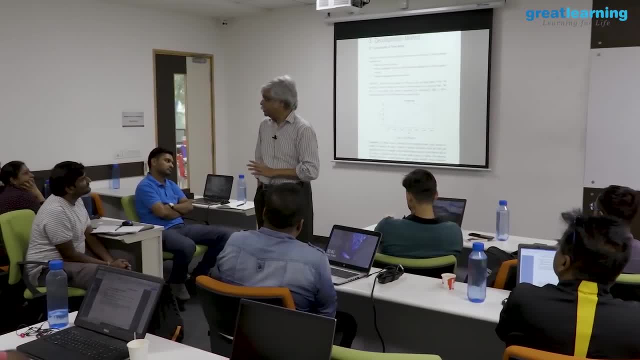 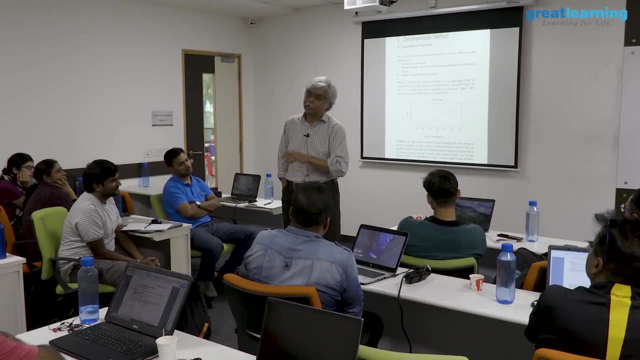 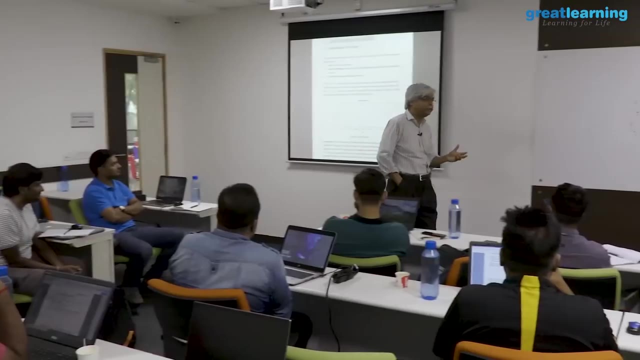 time series analysis is very focused on this irregular component, because that's where the money is to know something that nobody else does or can take advantage of: a trend of the seasonality anybody can take advantage of. and because anybody can take advantage of it, nobody can. you said this movie. 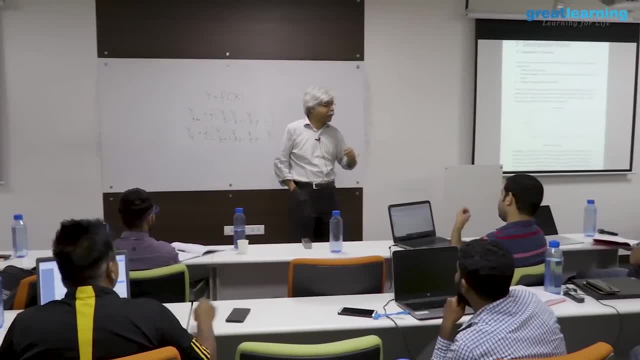 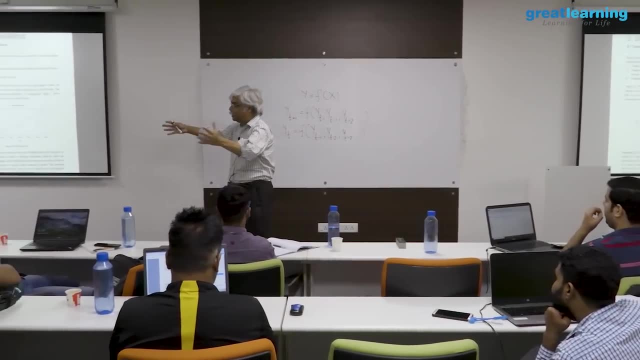 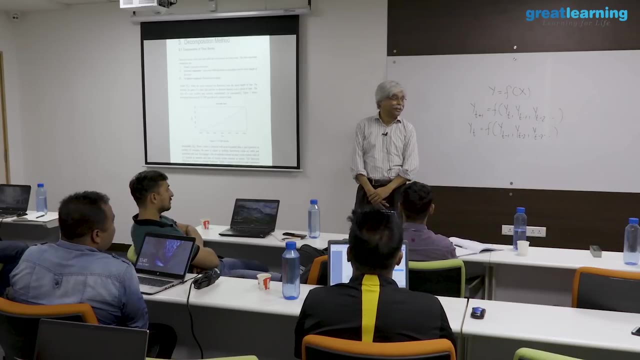 Incredibles, right? so there's this guy who's not a, who doesn't have supernatural powers. see, he gives an interesting and he said that and when. and his objective is to give everyone superpowers and so he goes. and when everyone is a super, then no one is. he has a wonderful, almost philosophical 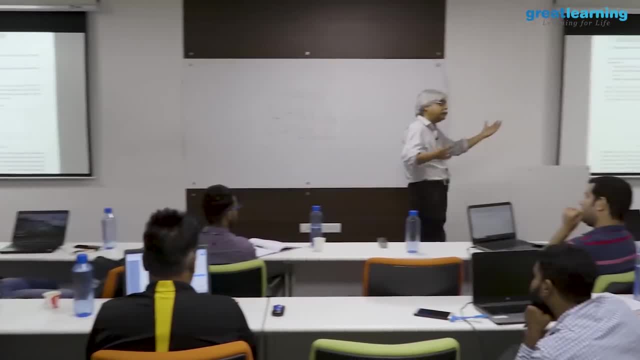 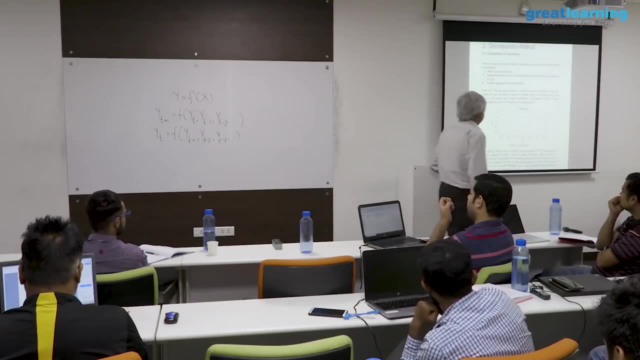 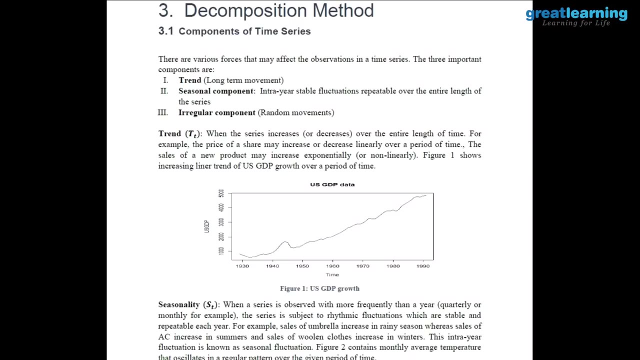 line and everyone is a super. no one is so. when everyone sees the trend, no one sees it, so to speak. no one takes advantage of it. so therefore, here, for example, is a is a series, and this series talks about US data, US GDP data. the India GDP data also looks like this: 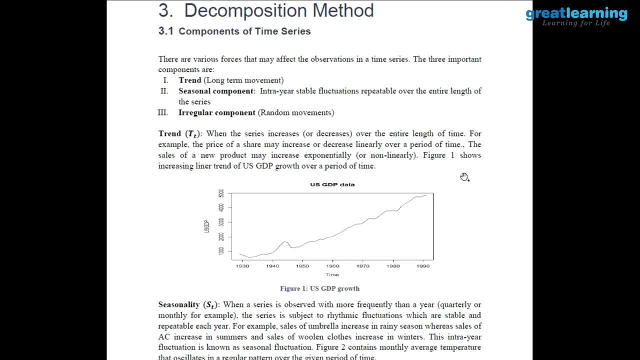 it's actually. this goes up 1985. the Indian kind of GDP data is growing up even more. a lot of economic growth is about understanding what these trends and what these shapes are like. for example, a US president once gave a promising view of the US economy. this is decades ago. he said: the rate of increase of inflation is not свăршки. in reoccurrence from 2015 to 2020. esto es décades de giờ. he said. the rate of increase of inflation is not an issue. the receives upon this since the beginning of this week, because of the fact that the 2016 is not Obama was elected, but after 2016 may be world's regure about including a few of the re-el条 born of Brexit experience. because of Google, about Pfizer in the United States, as you say, very early in 2020, during the nextulegals, he received articles on those items related to generalную перี. ogniChrystian baixar's. 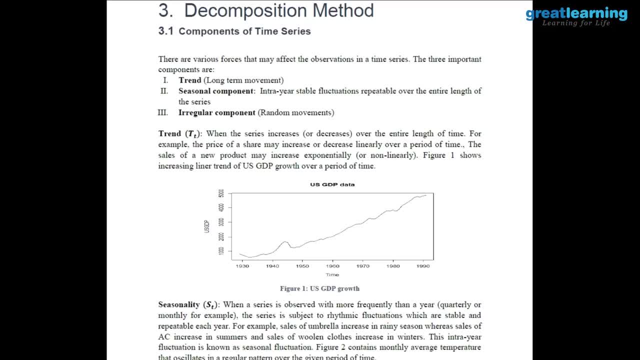 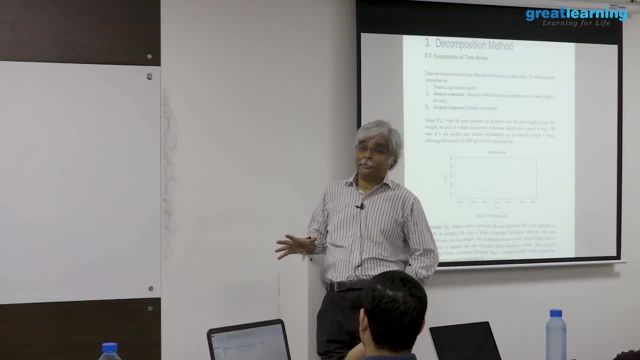 said, the rate of increase of inflation is going down. positive story: the rate of increase of inflation is going down. not only a price is going up, but the rate at which prices are going up is also going up. inflation is also going up. things are not good at all, but what? 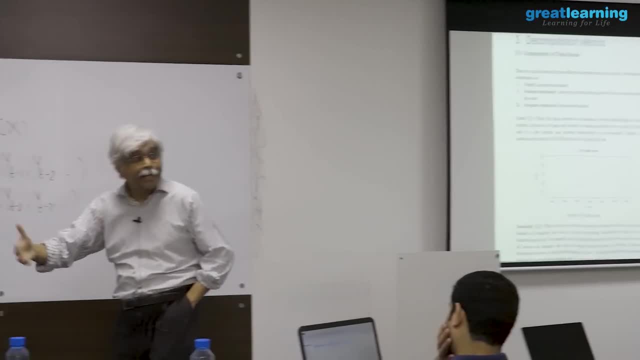 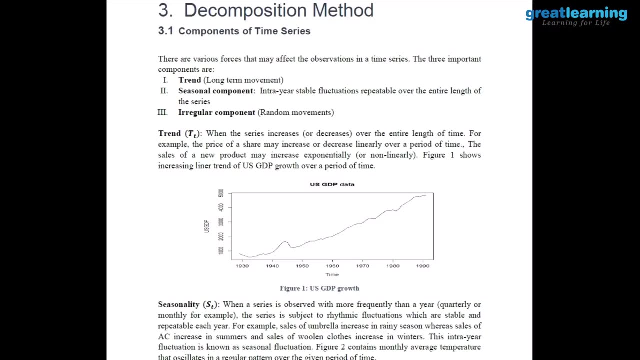 is the positive spin on it that the rate could be worth, that the rate at which the prices are going up is going going down. it's like a third derivative effect. so so different economies grow at different kinds of rates, at different kinds of time, and some of this 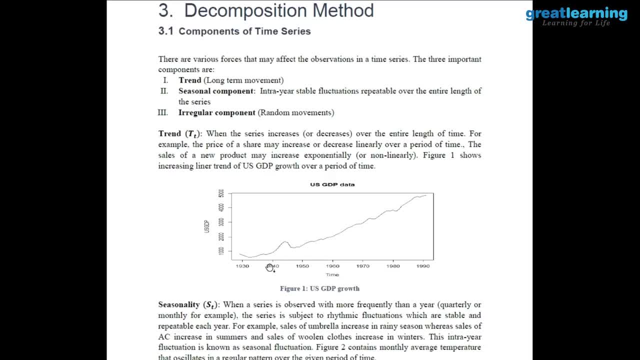 is about trend, and some of this could be say something like this now. something like this, for example: what is this? this is the US GDP. what is this? this is World War two. this is World War two. now is the World War two trend seasonal or irregular? the World War two is irregular, okay. 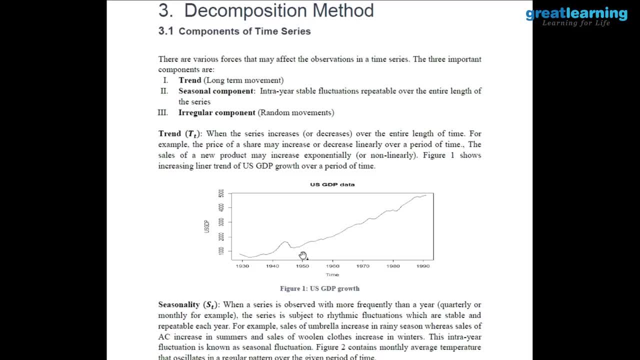 so that irregular lasted for quite a few years over the entire horizon. it lasted, however, only very short period of time. I remember in economics class many years ago that I did in the PhD program In which one of my classmates got into an argument with his professors in the business. 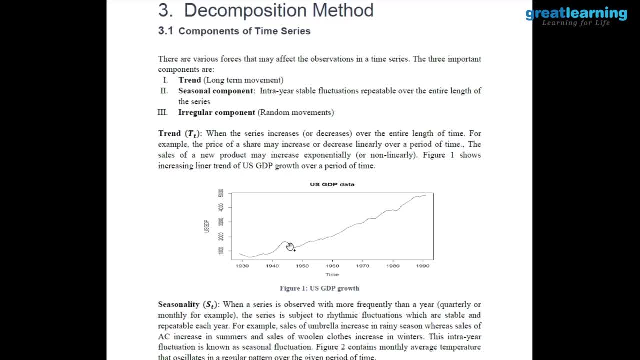 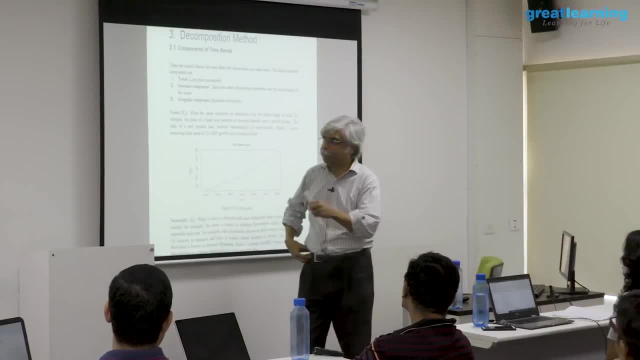 business and the professor was arguing something about business cycles, saying that you know, businesses go up and businesses go down. the economy goes up and the economy goes down and she was drawing a picture, the economy going up. and my, my classmate looked up and said that, oh, but the economy is. so he's drawing a picture like this: it's going up and going. 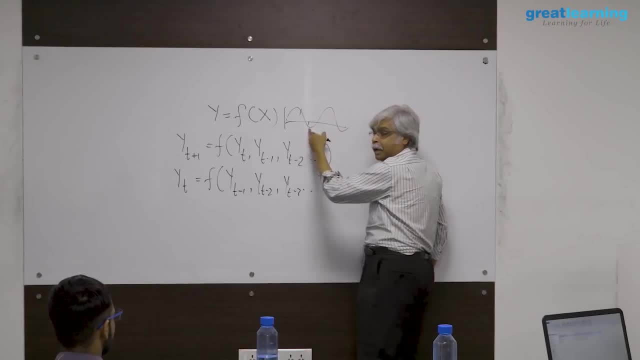 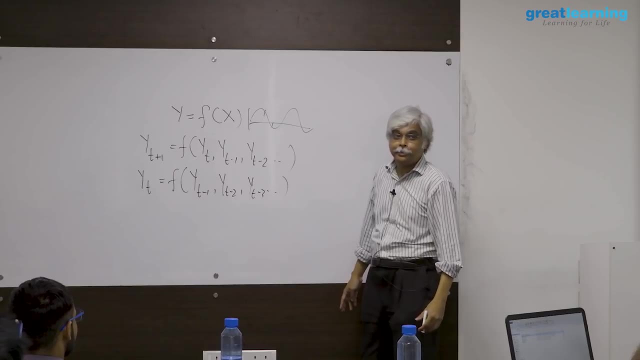 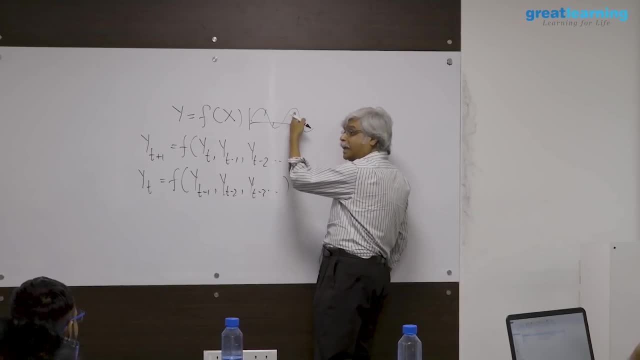 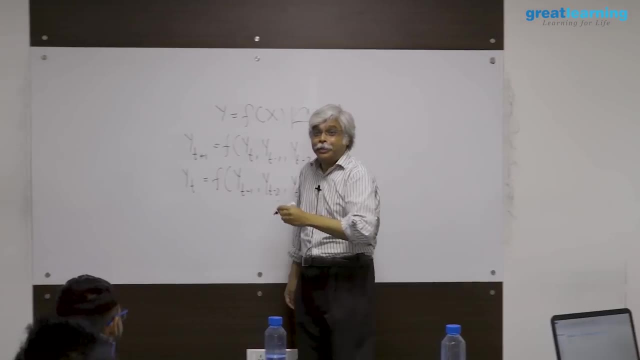 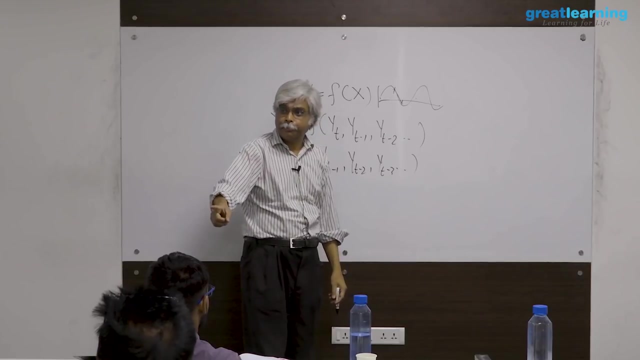 The economy sucks. now you're giving me hope, saying that no, no, no, no, this is, this is temporary- is going to go up again. who cares? I'm dead. so, from his perspective, this is a trend, and a trend that's hurting him. from my economics professors perspective, this is the trend. 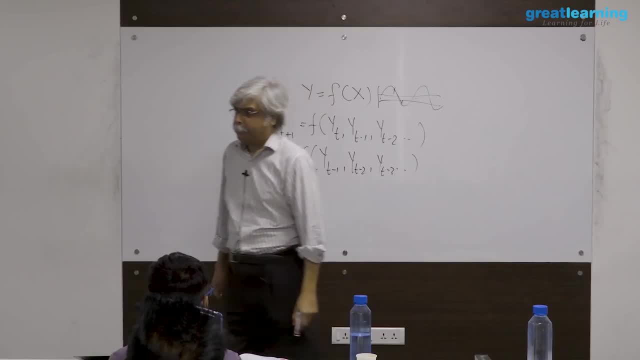 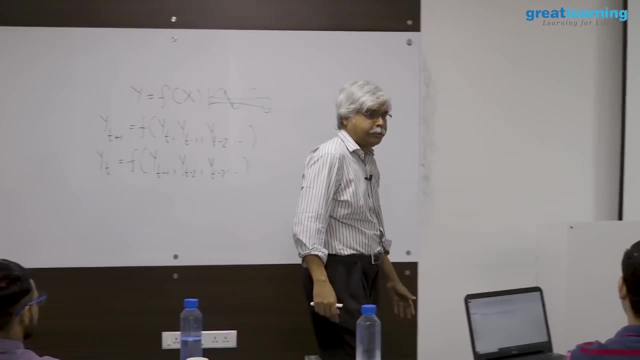 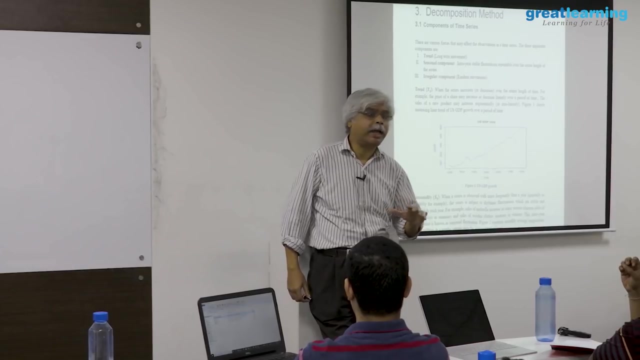 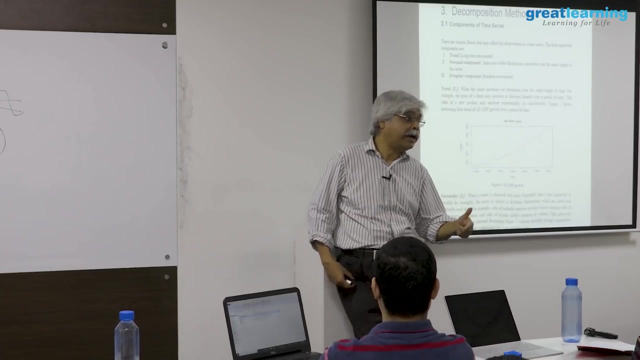 and this entire thing is a seasonality. so there's a question of over what horizon do you intend to do this? the same thing is true in businesses. if your business is doing badly, do you think of it as a trend or as something seasonal or something irregular? if you think of it as trend, that means what that means in. 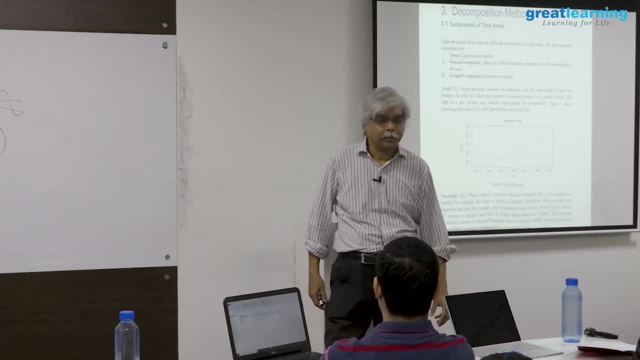 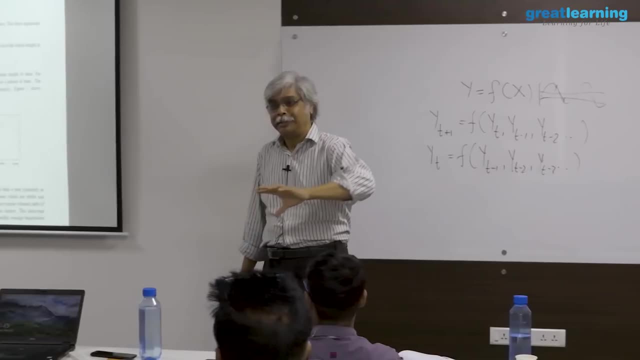 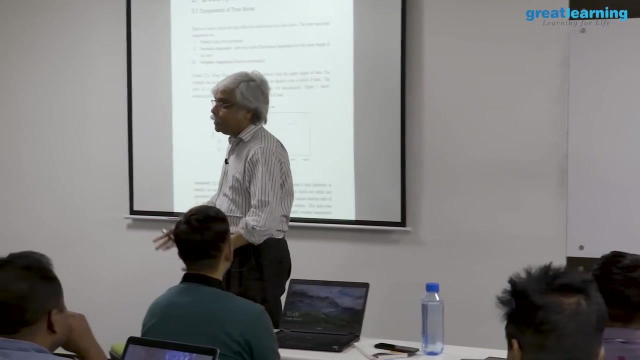 the future is going to continue to do badly, fix it. if you think it was seasonal. what it means is: wait, hold on, it's going to get better and then maybe worse again. if you think if it is irregular, then you sit and say there's nothing much I can do about it, but I've got 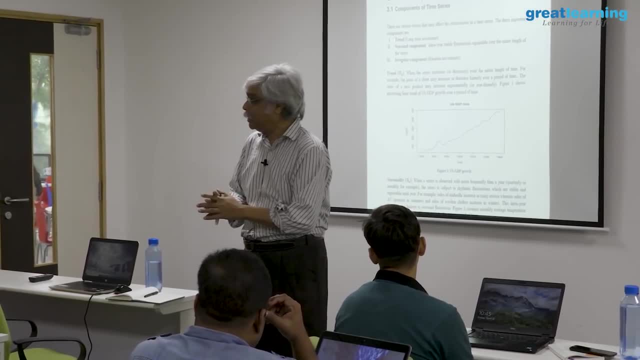 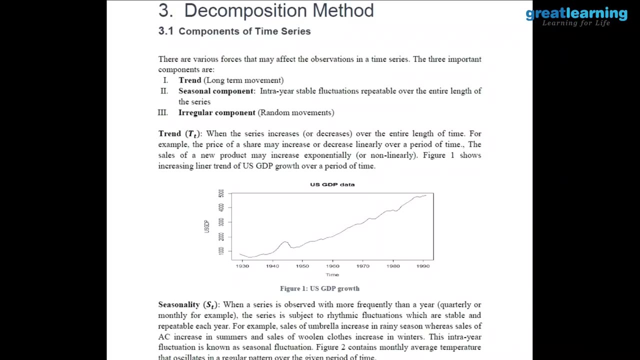 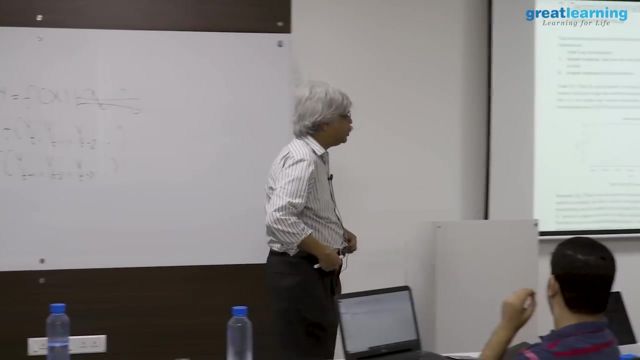 to prepare for these things. something bad happened and I go to make sure that when something like this back, something bad like this happens again, I am ready, but I don't know when it will happen or how bad it will be. but so a lot of this to some extent is subjective and depends on your interpretation or your your point. 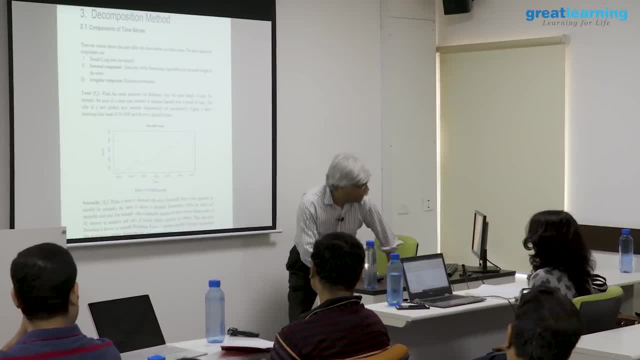 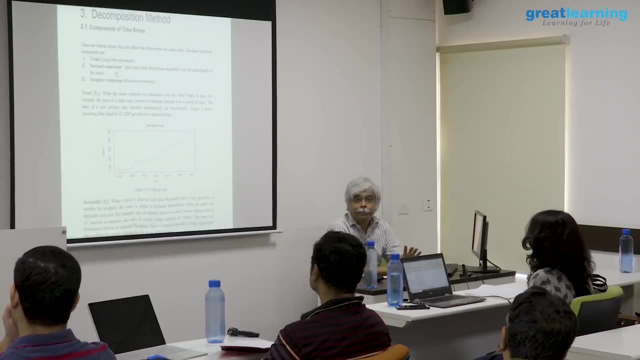 of view, which is why people like this kind of analysis, because they say that, at the end of the day, all I am doing is describing data. how you interpret it is your problem, which is where we will leave it as to whether you'll think of it as something long term. 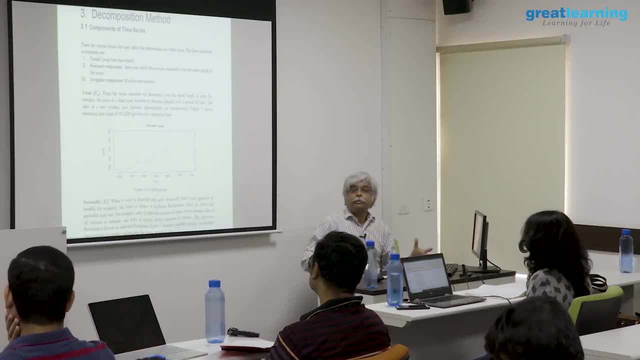 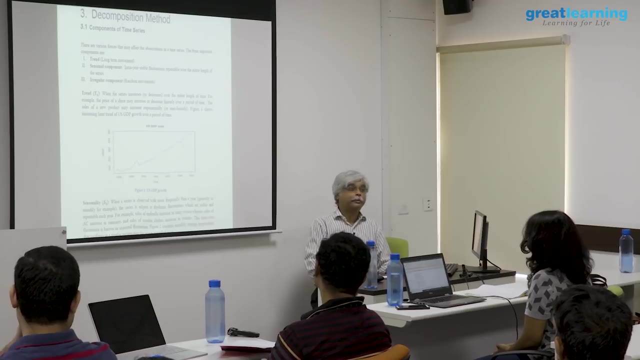 whether you'll think of it as something short term, etc. etc. why do I care? for example, a big confusion going on in the world- say global warming correct. many Americans, for example, say global warming good, it's too cold, particularly if living in, let's say, the northern US or 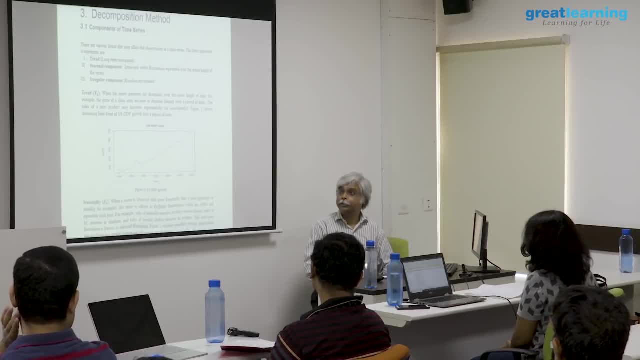 in northern cold country and it's snowing all the time. global warming sounds good, but it's not about global warming. global warming is about unpredictable behavior. it's as much about the variance as it is about the mean. so and so there's some confusion around this. 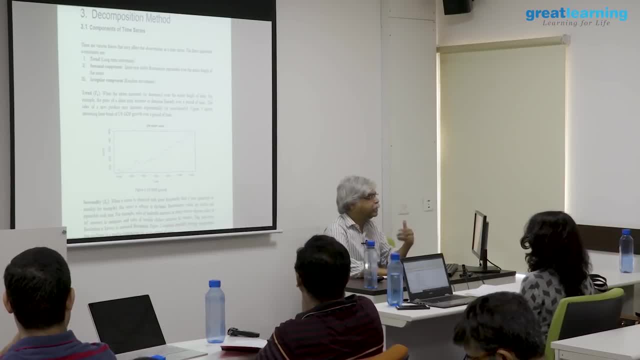 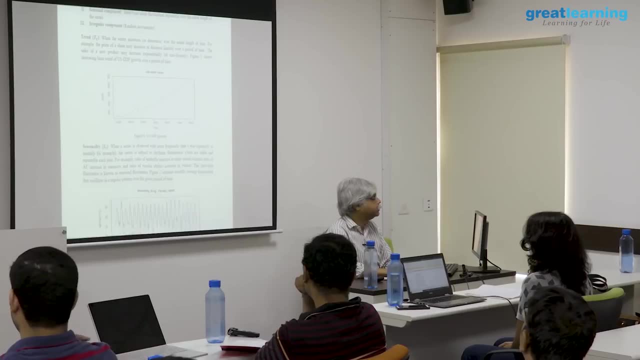 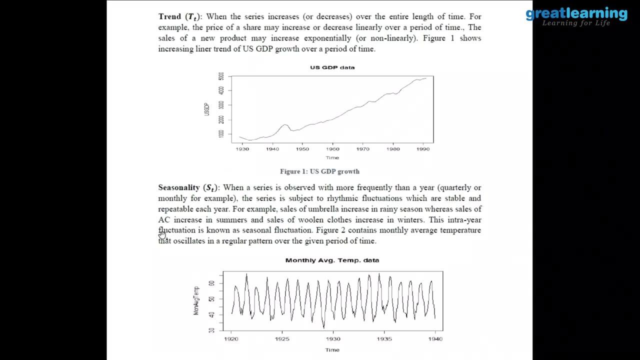 so what people do is people don't necessarily try to interpret the understanding of it, but simply say this is what it looks like. so descriptive understanding of this is given seasonality. seasonality is something that changes over time. sales of umbrella increases in rainy seasons, whereas sales of ACs increase in summers and the sales of woolen clothes increases in. 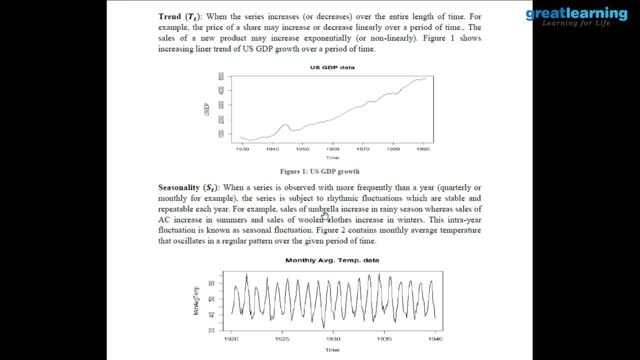 winter somewhat obvious now. the sales of umbrellas increases in the rainy season. this is correct. but let's suppose, for example, you are trying to predict the sales of umbrellas. let's say that you have an umbrella store in HSL layout or wherever you are. now, how many umbrellas do? 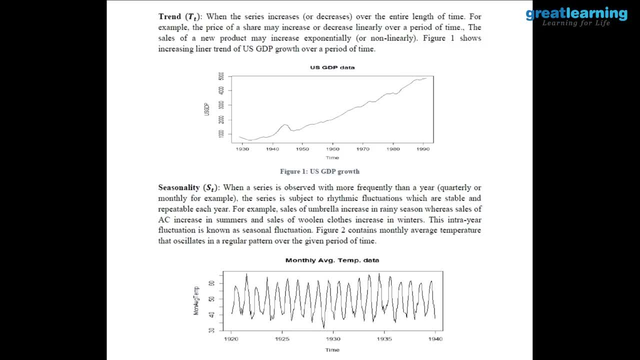 you expect to sell? how would you forecast that pass data? which period? so let's say that I'm trying, let's say that, let's say that I've given you data for let's say that you've gotten running establishment. in other words, establishment has been, has been. 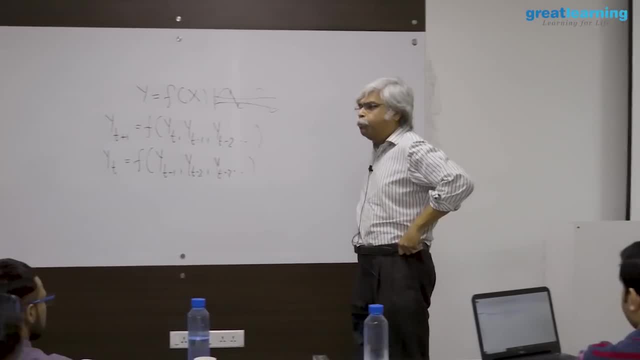 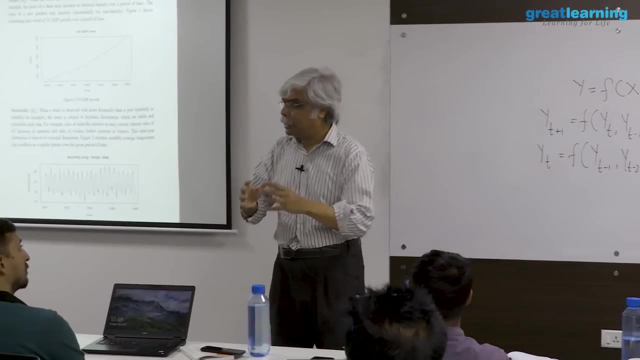 going for a while. you've been selling umbrellas for five years and I'm giving you monthly sales data. let's say for so, monthly sales data for five years, how much is that sixty? so I've given you sixty numbers and I'm, and you're, using those sixty numbers. your job is to predict what is. 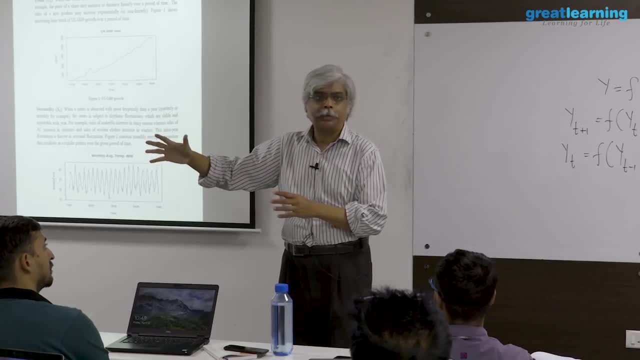 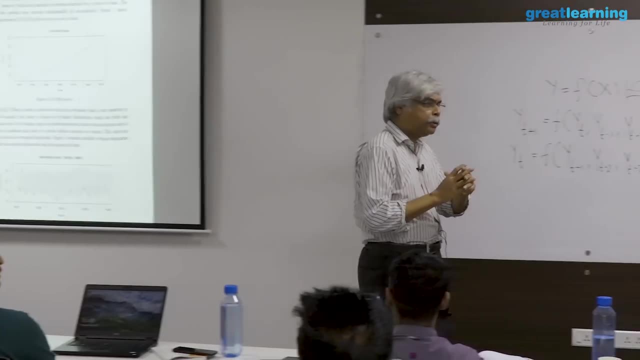 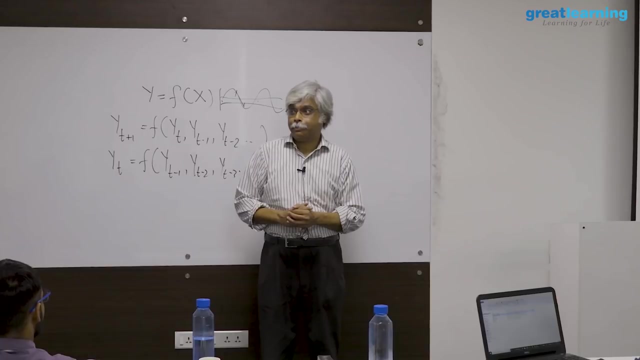 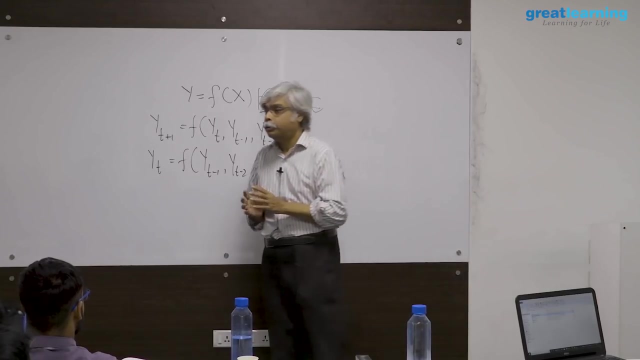 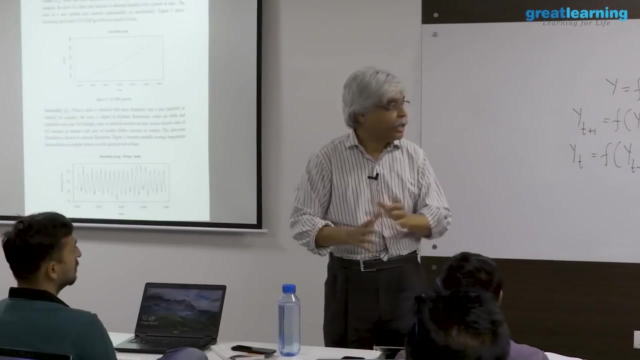 going to happen to the sale of umbrellas. let's say, in weirdom, this is what this April, let's say me this May umbrella, now what? what are the past sixty numbers is going to help me predict sale of umbrellas this May, last May, okay, last four, last four Mays. why seasonality? so what you're taking? 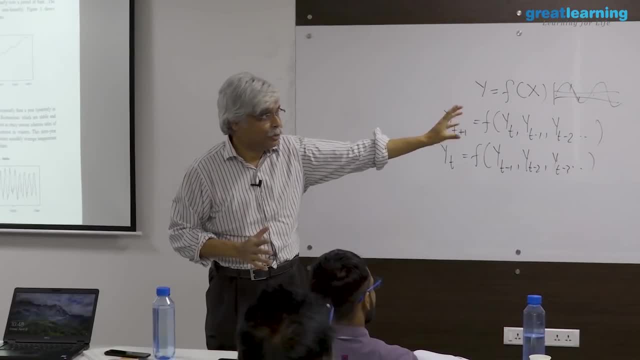 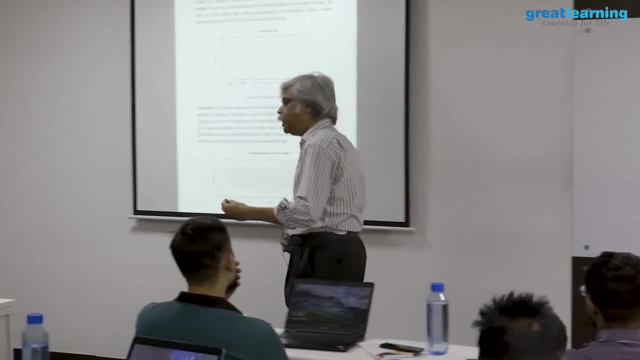 advantage is of. you're taking advantage of. you're trying to find this ST. you're saying that the sale of umbrellas is going to be driven by seasonality. okay, now what else does the sale of umbrellas depend on? they'll give you a hint: who buys umbrellas? people who don't buy umbrellas in. 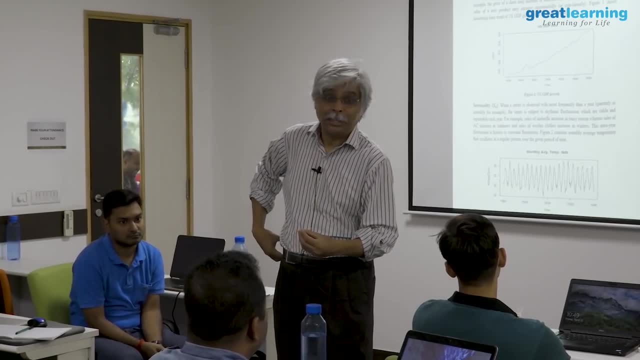 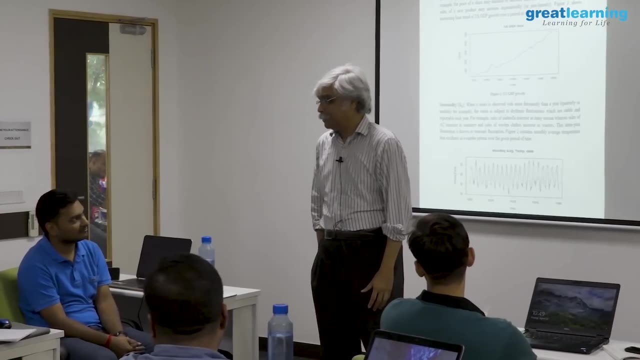 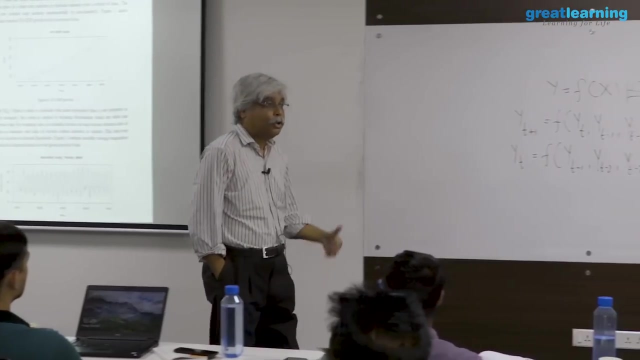 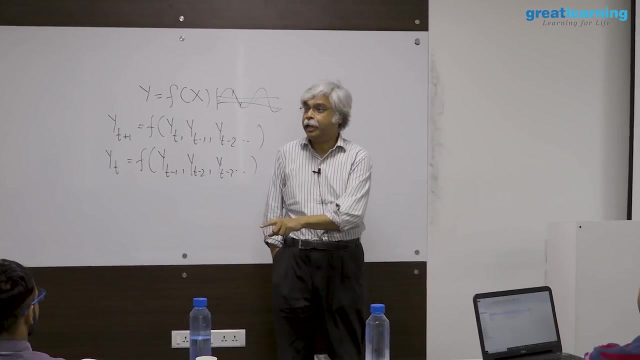 short people. guns don't kill people. people do things like that, so people buy umbrellas right now. what determines how many people there are population? what is the population doing? it is increasing. so now, if I want to predict how many people will buy umbrellas in May, what? 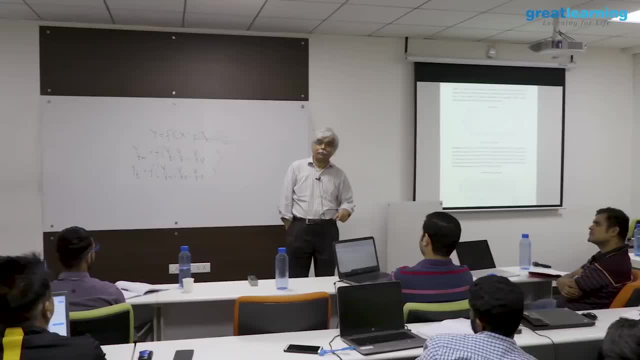 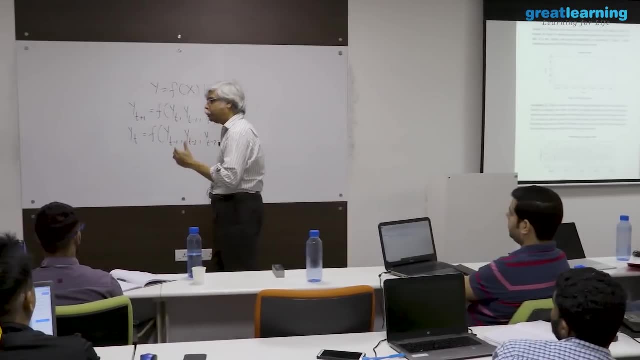 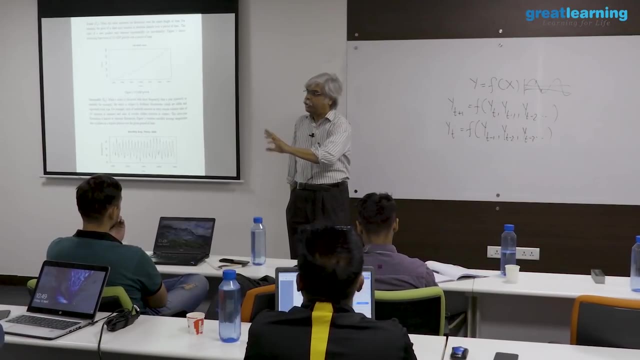 is going to pick up, how many people there are, for example, would I look at. so let me rephrase the question: I'm going to look at, I'm going, I'm going to take two months of data. which two months should I take? should I take last May and the May before that, and what I should do? one of the things: that have happened? who picked up? how many people are there? who pick up how many people are there to be included in the specifics? because what if you have enough people who they all choose to buy umbrellas? they are Extreme in kasほう m Maar ja s 너 men? ih automated as a whole not to become. 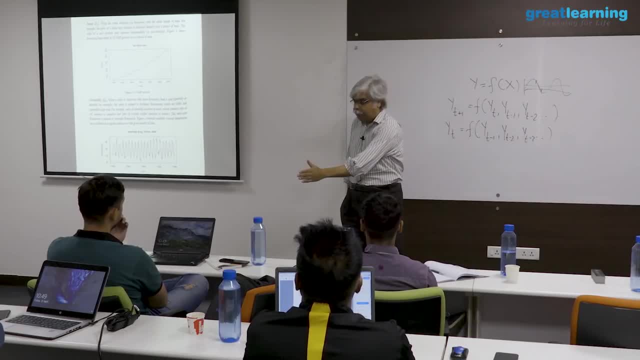 you know why I am E villanova student. you could tough to compare to tradition, but the point is something from the past two months. now I'm not even, I don't have that number, I don't watch, I. am I going to the that, or should I take this April and this March? this April and this March is 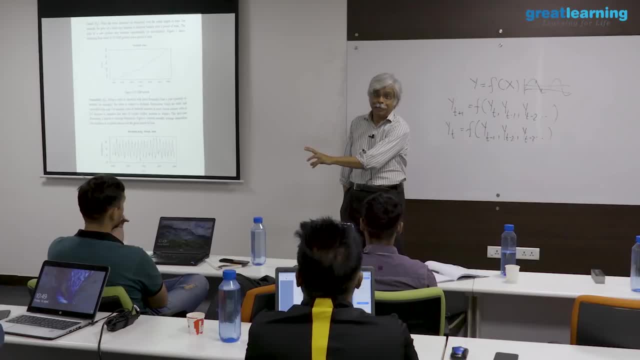 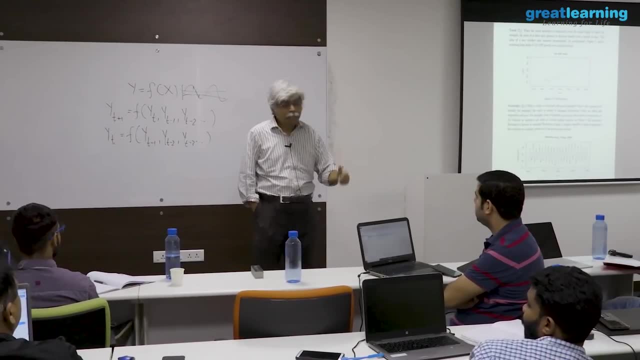 going to get. give him, give me a better idea of the size of the market. you know the number of people. on the other hand, the last me to maze will give me a better idea of the seasonality. one of them is picking up trend, the other is 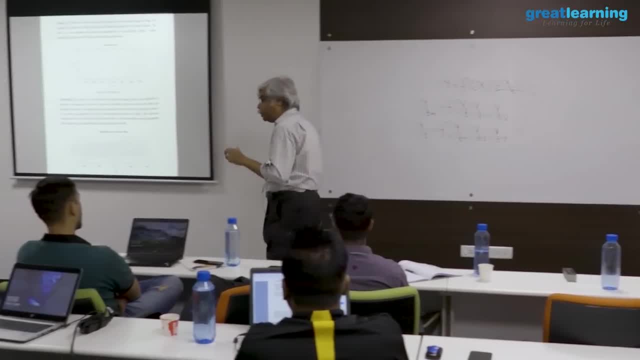 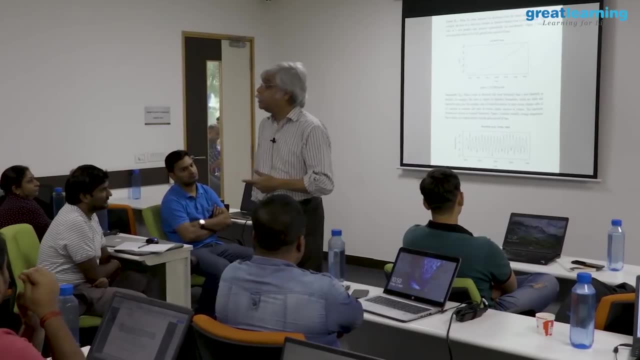 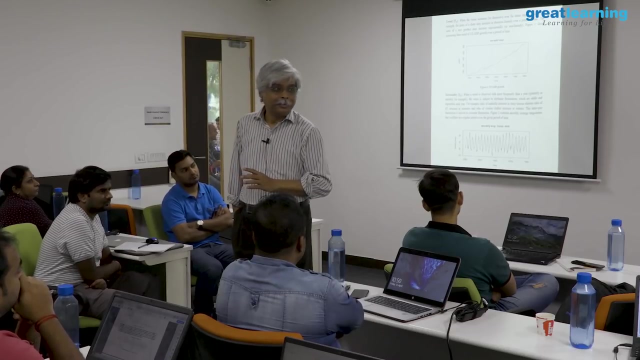 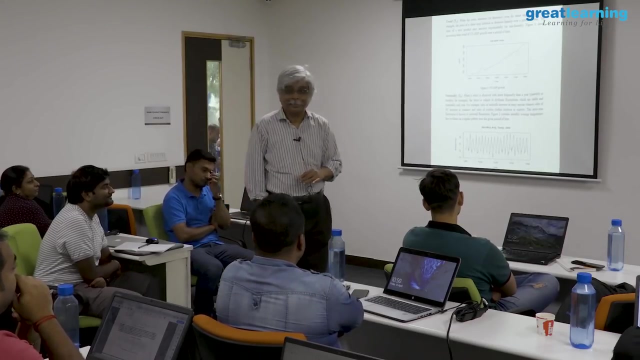 picking up seasonality to two separate things are driving my sale of umbrellas: how many people there are, and is it raining or not. how many people there are is sort of independent of the season. whether it is raining or not is also sort of independent of the people. but what you have done is you put these two 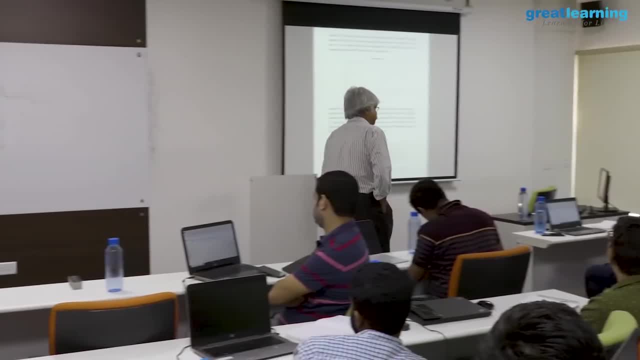 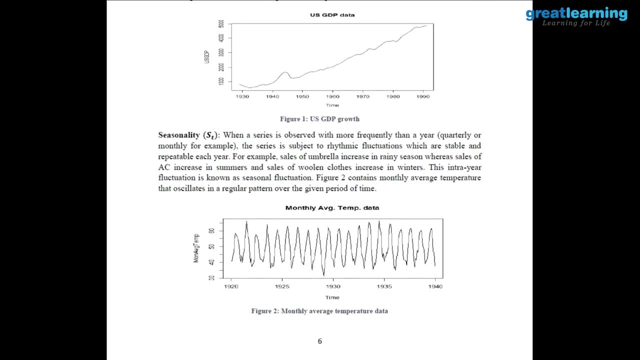 things together, so both of these things could be at play. it becomes interesting. same thing for any of these temperature, on the other hand, is going to be at play. it becomes interesting, same thing for any of these temperature, on the other hand. as I said, if you believe in global warming, there may be a trend or 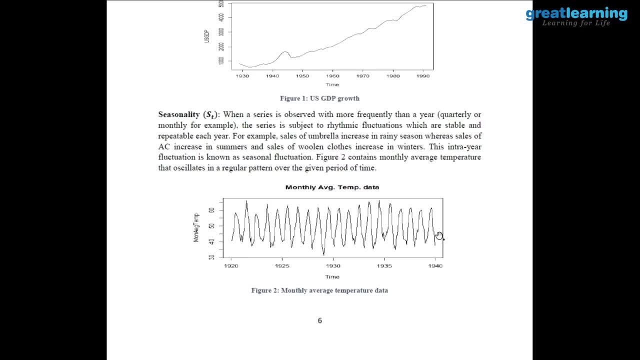 otherwise, over a short period of time you could say: this is flat, my wife and I sometimes, you know, since we've been in Bangalore for quite some time now. this is so. we came in 2002 and we moved here from Delhi and so Delhi to Bangalore. the weather shift at that time was somewhat remarkable, it was much. cooler here and, much more importantly, it was more predictable, so to speak. 16, 17 years ago, on a regular basis, it around 4 o'clock or 5 o'clock or thereabouts, it would rain a little bit. as the years have gone by, the city's weather has become a lot less. 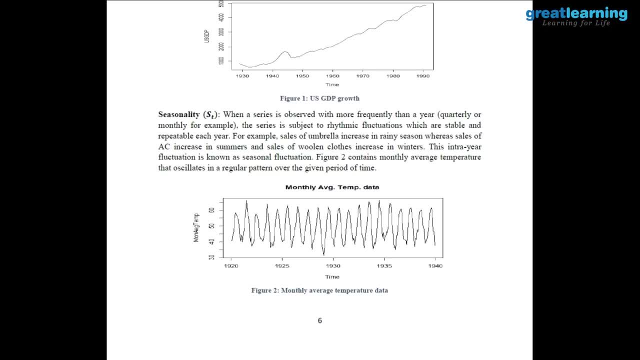 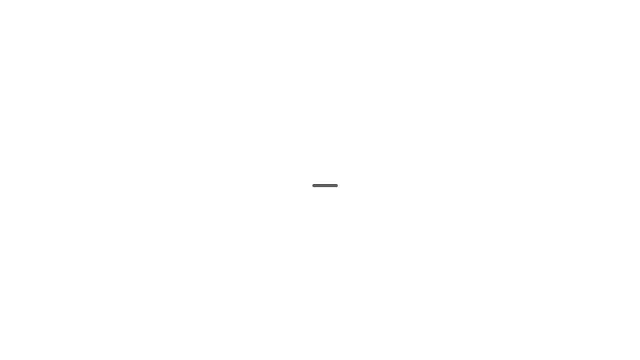 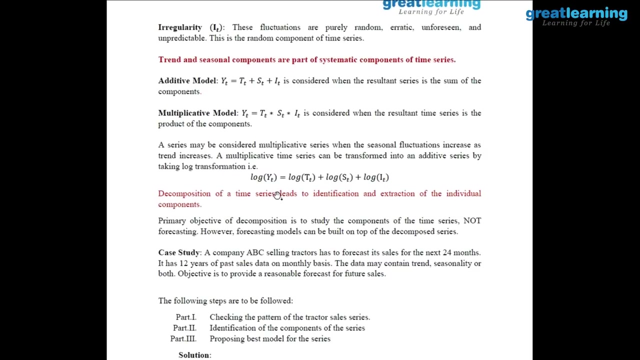 predictable. the seasonality is there, but the seasonality doesn't appear to be as clean, so to speak, maybe for a variety of reasons. so there may be a trend, in addition to the seasonality component that you have, you OK the irregularity part to this. so the irregularity here puley random, erratic. 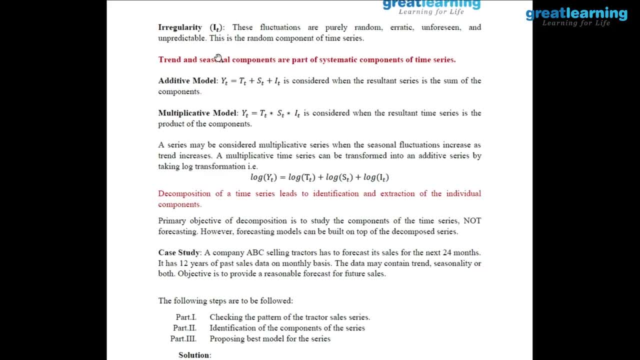 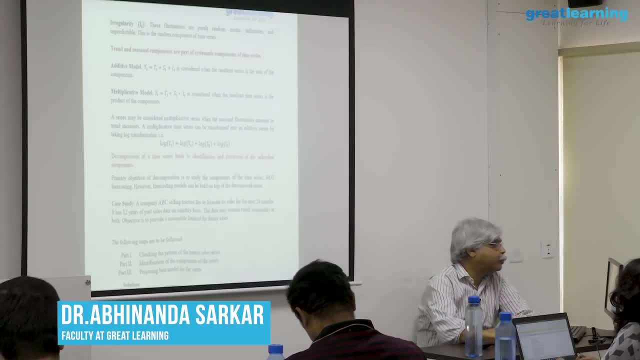 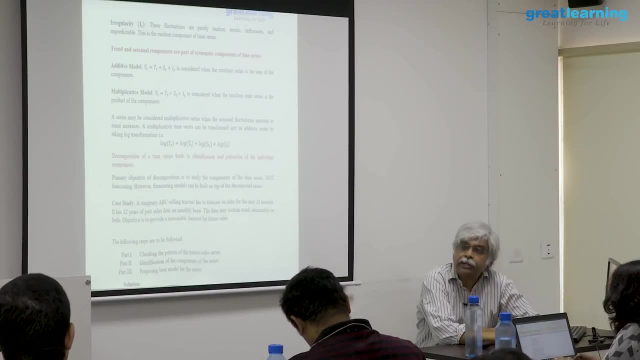 unforeseen and unpredictable. from an analytical perspective, this does not extend into the future, mmm. For a forecast perspective, I therefore will tend to ignore it, But from a data analytics perspective, I need to still find it, Because I need to subtract it away. 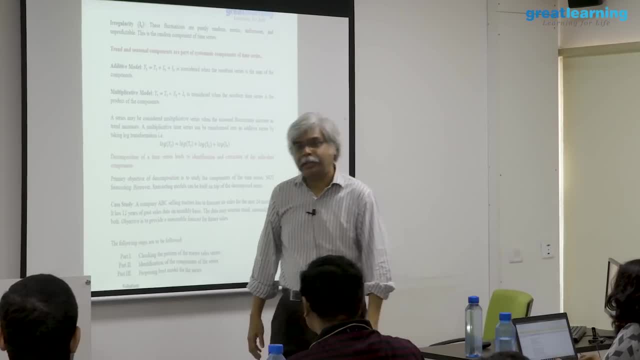 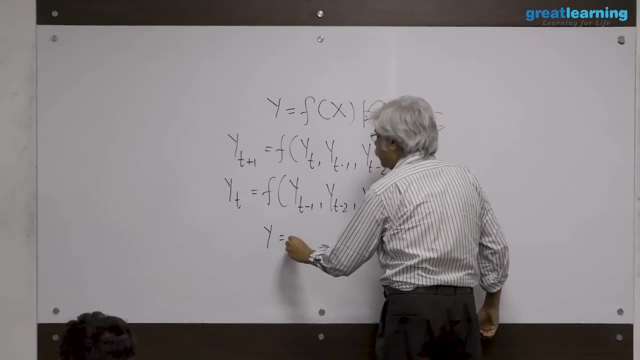 You did this in regression. You did this in neural networks. You have done this in classification. You have done this in pretty much any model that you have done. What have you done? For example, in regression, you built a model like, say: 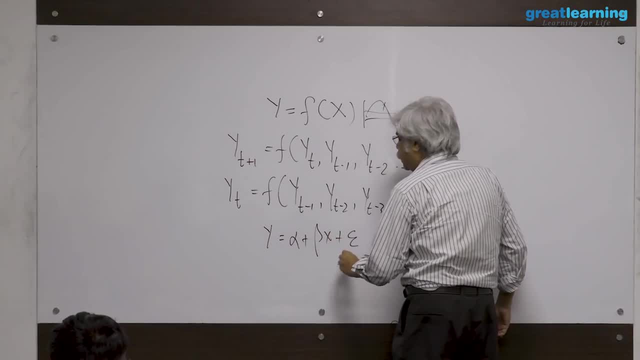 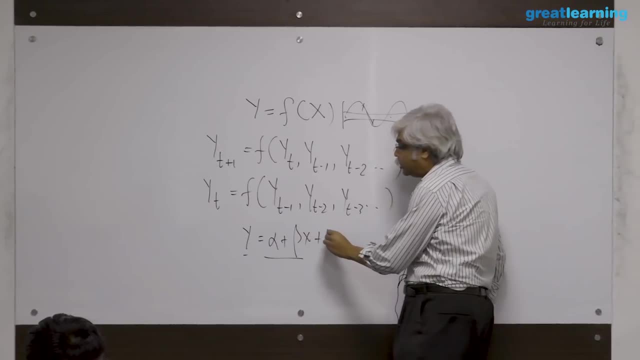 a is equal to alpha plus beta x plus epsilon. How did you fit this? You went y minus alpha plus beta x and you got an epsilon. And then you minimized the sum of squared errors. You made this small. You wanted to make this go away. 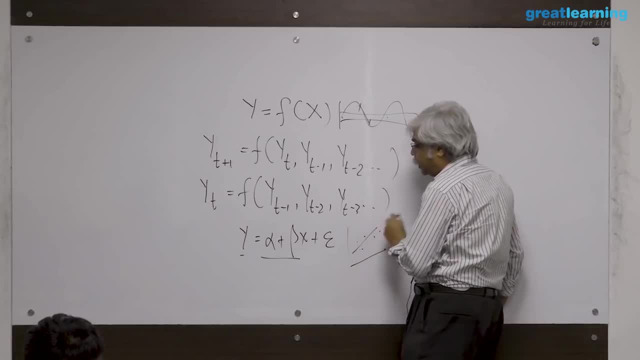 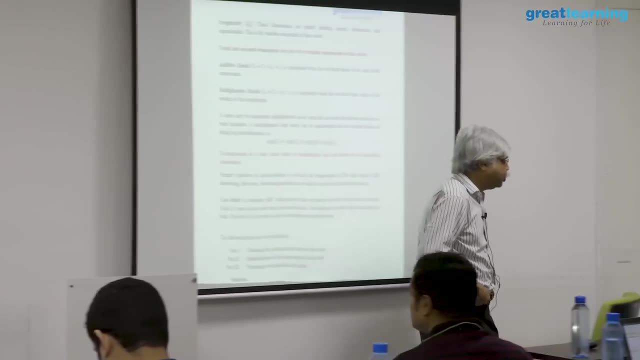 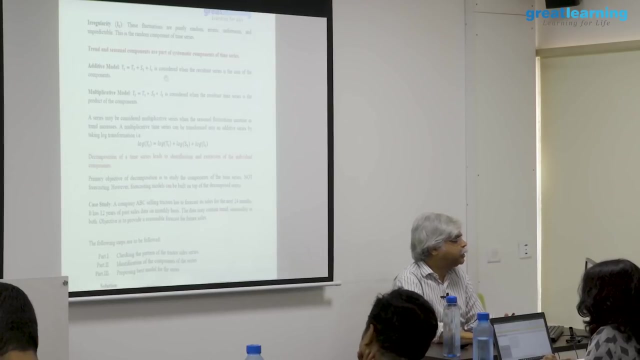 But you could not make this go away. This will still remain as a residual in your plot. The analytics exercise will not make this disappear, So your job is to be able to split this up. Now, how do I split this up? There are a number of ways in which I can split this up. 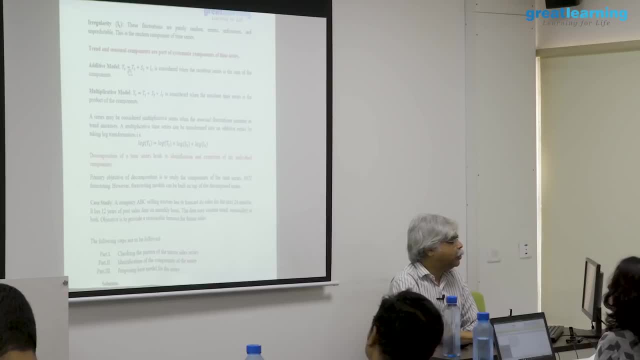 And this will take a little bit of thinking, but we'll see data and figure it out. One is things add. The second is things multiply. This means that your observation is the sum of things And this means that your observation is the most. 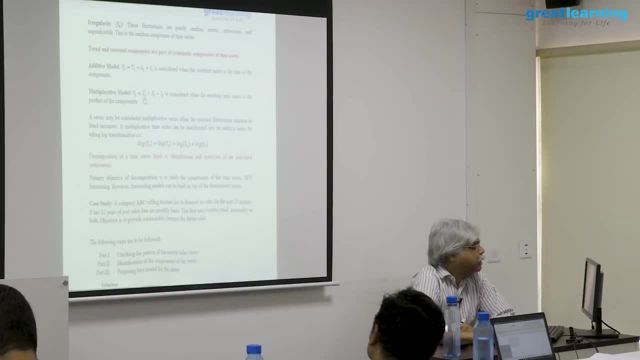 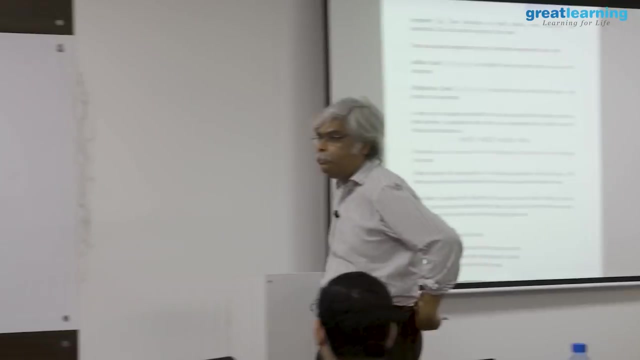 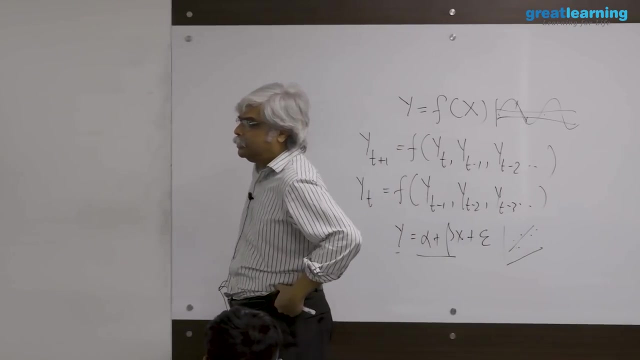 More things tend to be this way. So let's say, for example, you order for a meal in a restaurant And the meal costs say 500 rupees, What would you expect your bill to be like? Exactly 500 plus GST. 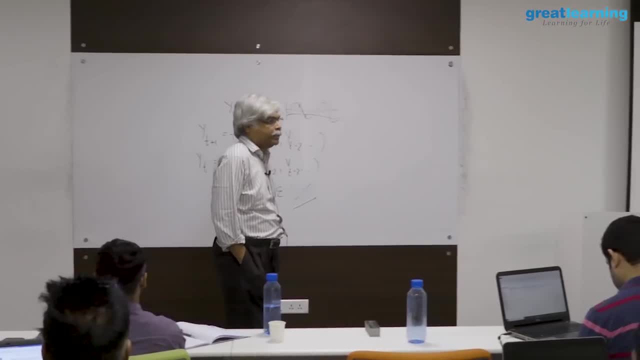 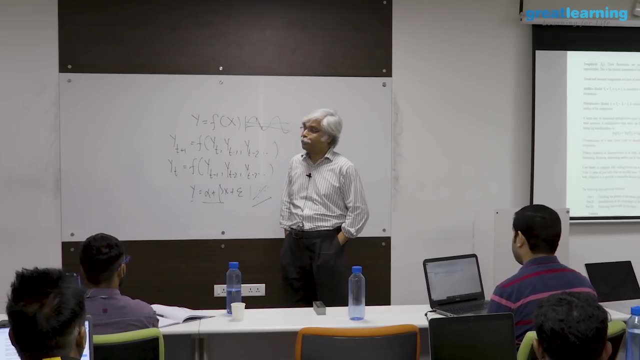 Okay, You'll do the calculation of GST in your head, Right: 18 percent, 5 percent Depends on whether the restaurant is luxury or not, etc. I suppose What kind of an error would you tolerate? Would you be okay with, say, a 600 rupee bill? 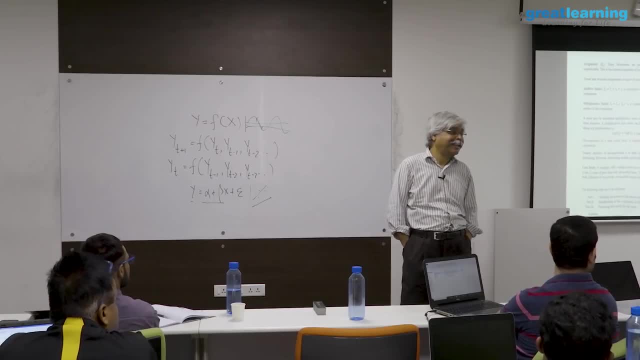 550?? 20 percent Maybe, service charge, and you don't know whether the restaurant gives a includes a service charge in the. you didn't read the fine print in the and you don't know whether they've included a service charge in their bill or not. 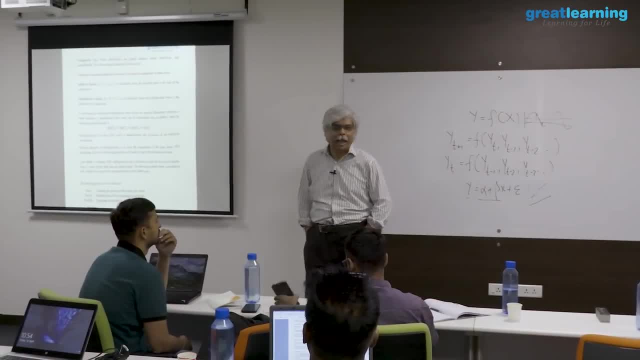 550, 600, something of that sort, maybe 50 rupees, 100 rupees max. you'll be allowing for, and shall we say, an error, An unpredictable error, An unpredictable error, An unpredictable part of the bill. 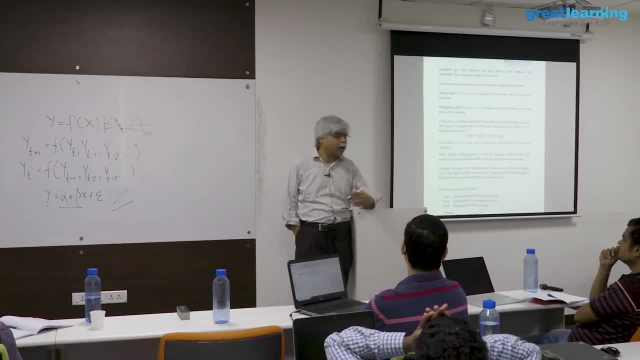 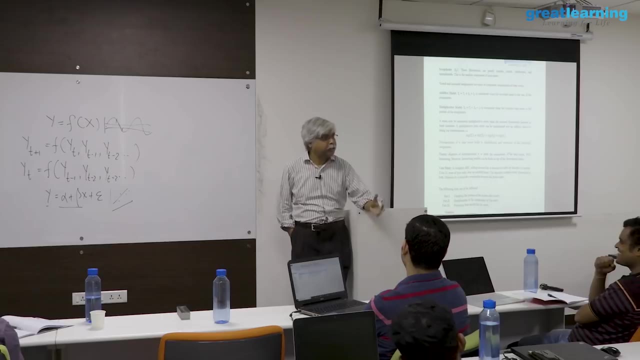 Now, let's say that you are buying an apartment in Bangalore. How much does an apartment cost? I have no idea. One crore, One crore, Okay, one crore. He's optimistic about life. So now, if you have one crore, let's say you're ready to spend one crore. 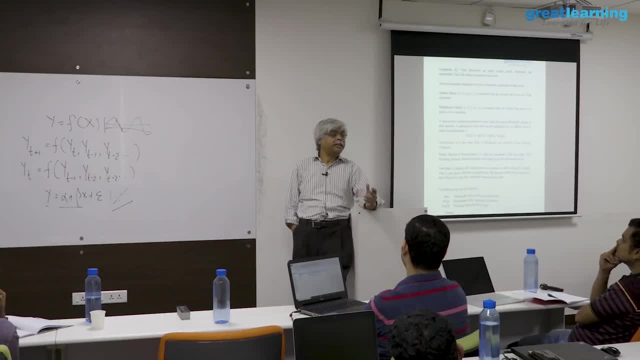 Now, how much more or less are you willing to pay? Or let's say, more People won't pay less, but how much more are you willing to pay? 10 to 15 lakhs. 10 to 15 lakhs. 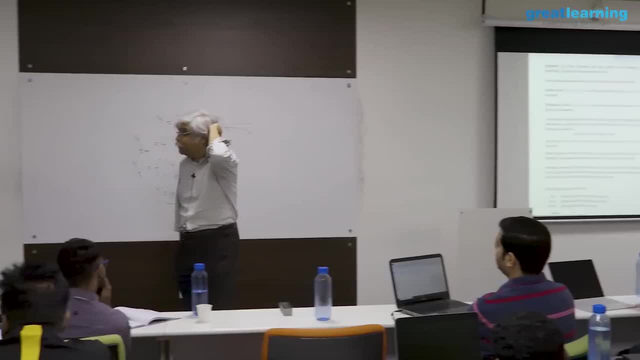 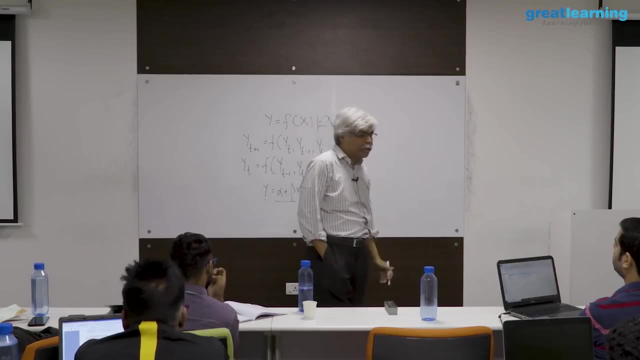 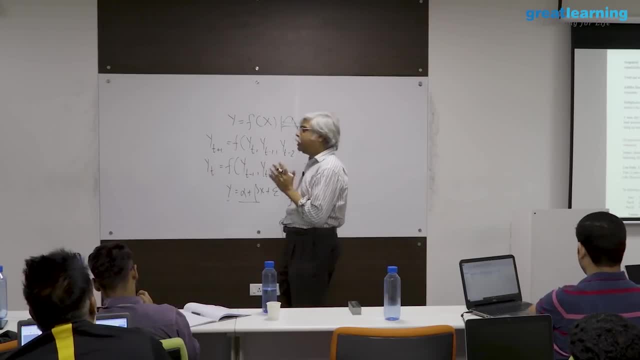 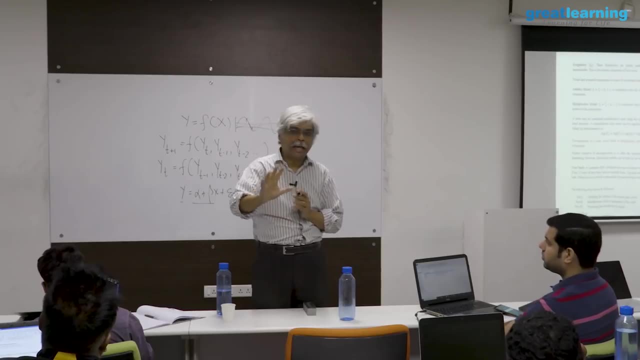 10 to 10 lakhs for the apartment, But the amount of uncertainty you are willing to tolerate for these two numbers was different. My question is not on the number itself. My question was on the size of the error. The scale is different. 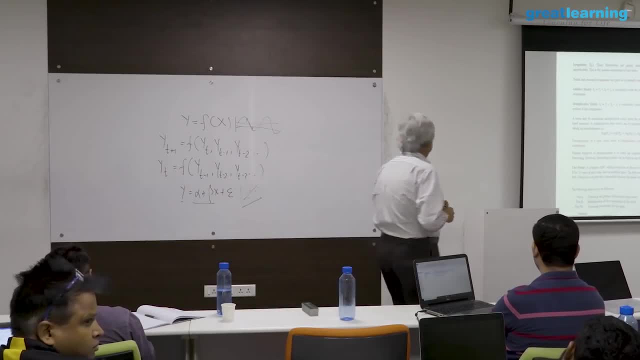 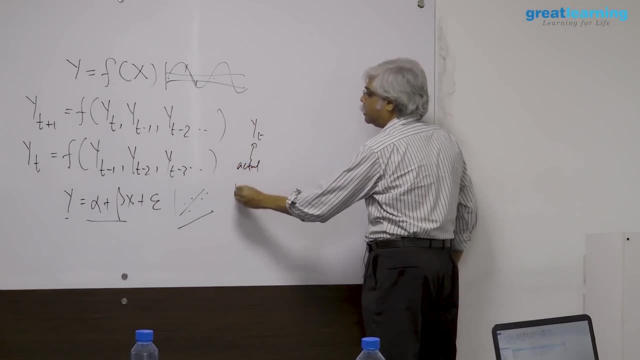 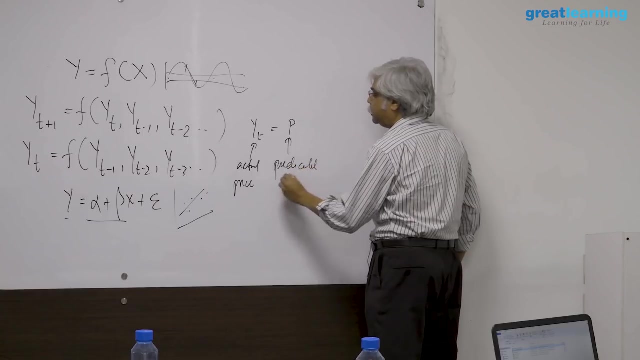 The scale is different, right? So now let's suppose that the predictable part so you got, let's say, the y of t. this is your actual say price. This is equal to, let's say, your predicted price or predictable price. 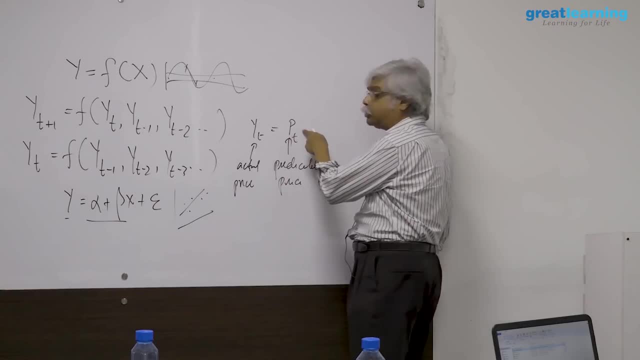 For the restaurant, this was 500, and this was your actual. For the apartment, this was your 1 crore and this was your actual. Now, this actual is now going to be a modification of this price. How do I get to that modification? 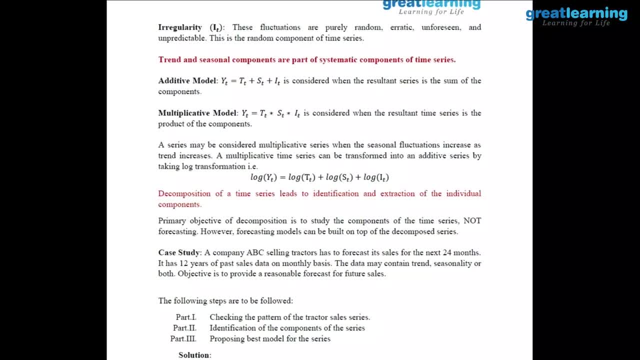 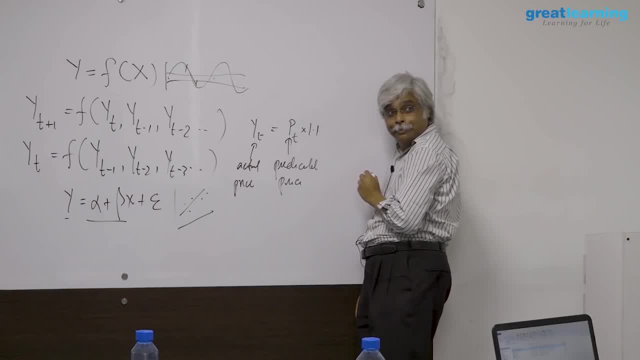 If it is a percentage, what should I do? So let's say I do this. Let's say I do this multiplied by 1.1.. Now, what will happen to my 500? 550.. What'll happen to my 1 crore? 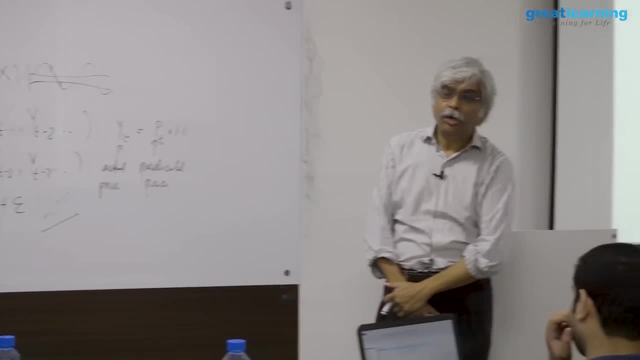 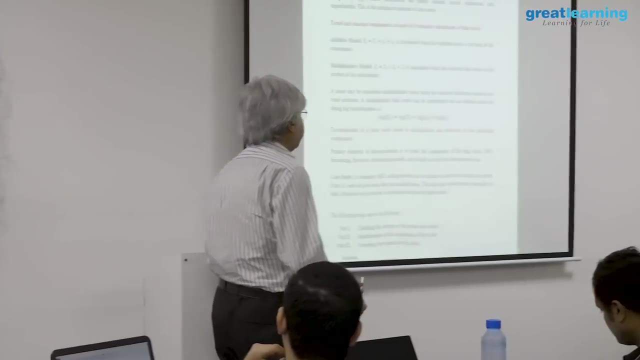 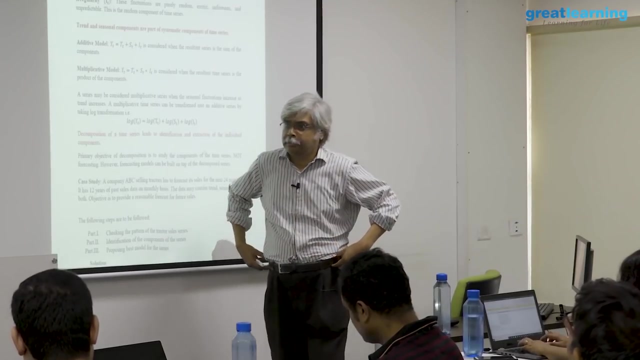 10 lakhs. what you just told me is that your error is multiplicative. the irregular part multiplies and in many financials and in many growth oriented things, this is what it actually looks like. it doesn't add, it multiplies. on rare occasions things do. 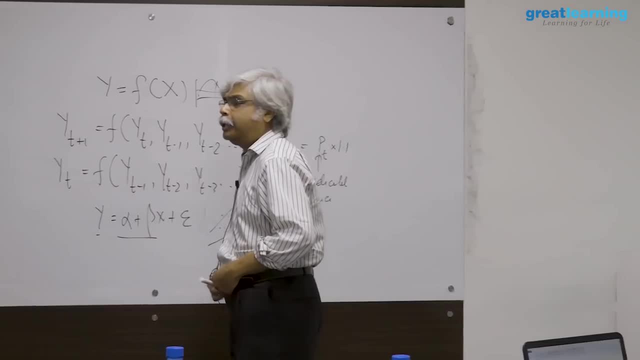 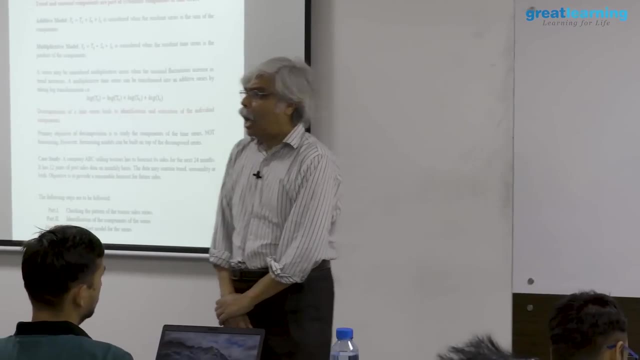 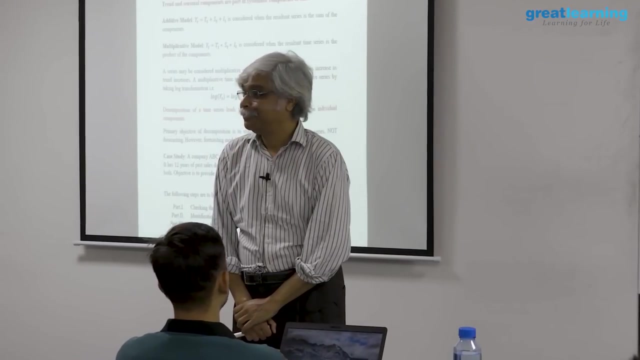 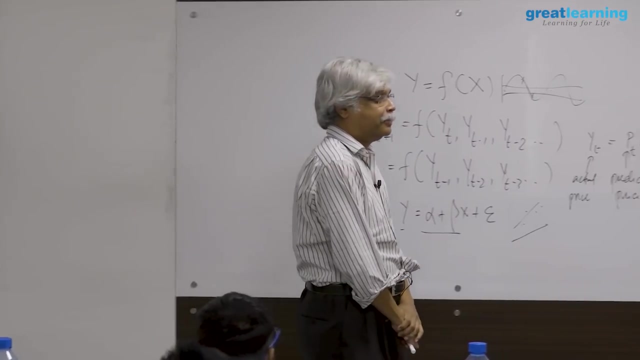 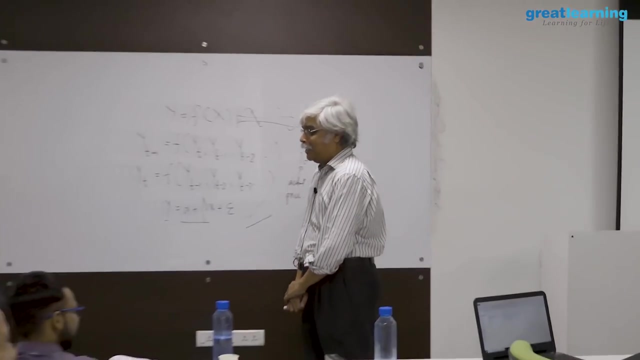 add. give me an example of something that, an example of something that, for example, adds: how much do you expect to eat for lunch? two chapattis. two chapattis. with what error? if it's free, then more. I agree. I have uncles who do that and now I do that. 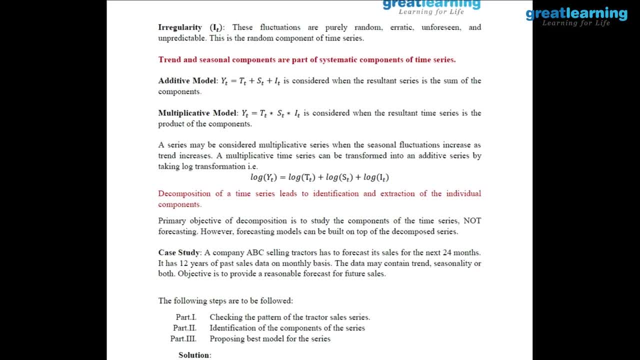 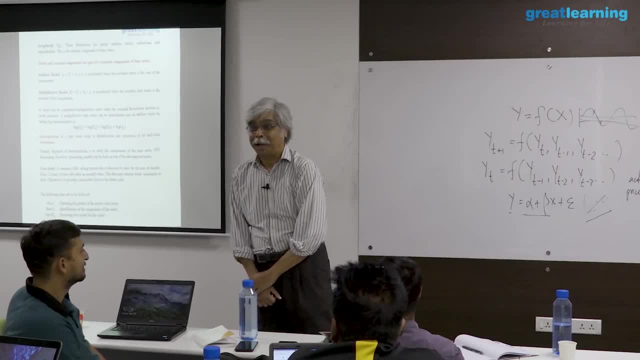 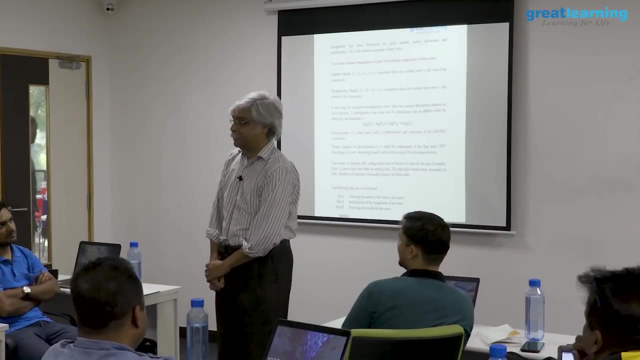 but if you're hungry- let's say you're more hungry than usual- how many more chapattis will you eat? hmm, plus, does this depend on how many chapattis you've already had? no, my question is: if you're hungry. so why is the number of chapattis? 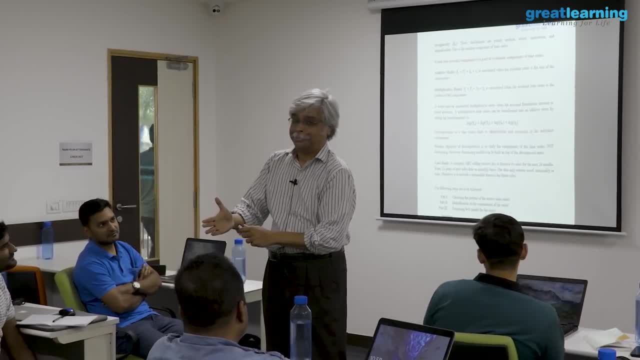 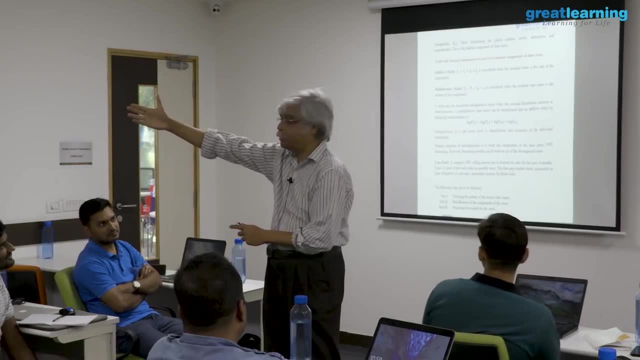 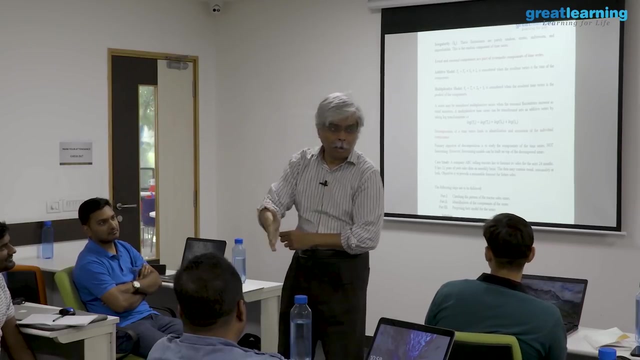 you're having uncertain, which is probably the first question to ask. this is not a trivial question. this determines how many chapattis the guy is going to get. he's going to make an estimate of how many chapattis you will eat now from your perspective. so it could be that someone thinks the 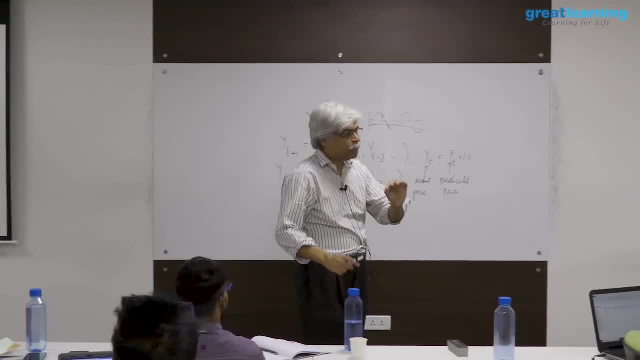 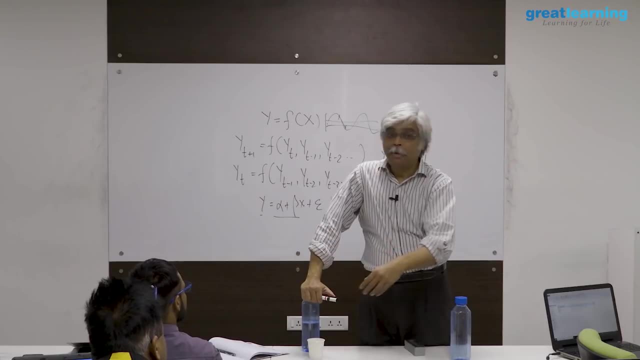 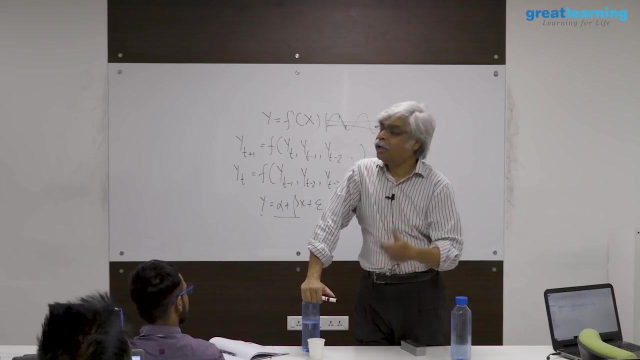 following way: that, or he thinks the following way- that if someone is particularly hungry- in other words, this class is hungry- their, their, their training went on too long, or maybe the they like the sub G. they will have more chapattis. now how will they calculate the number of more chapattis that will be there? how? 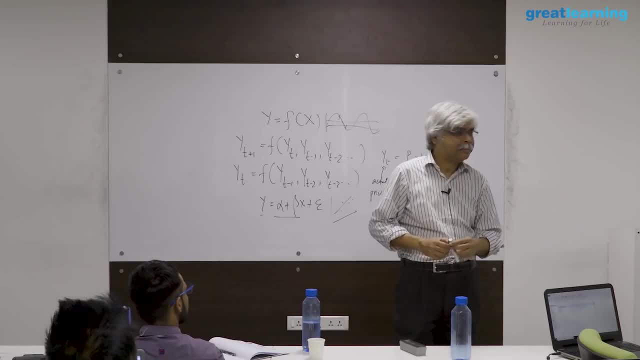 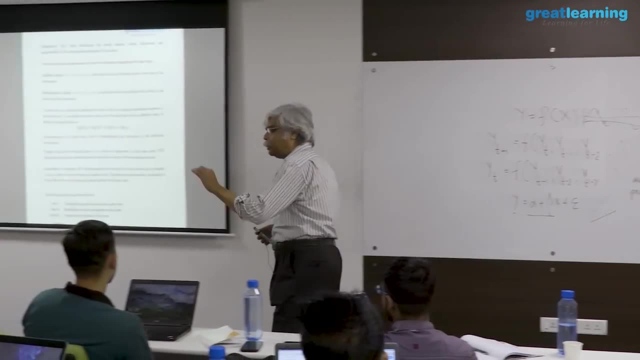 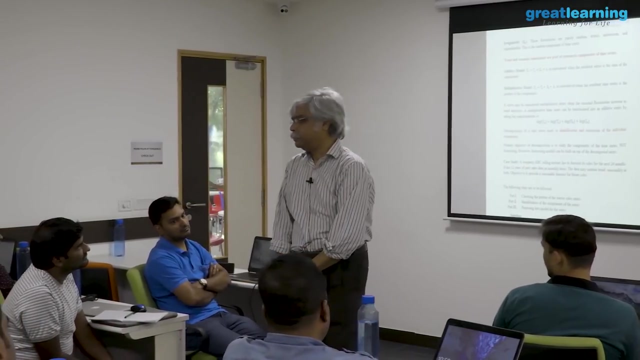 many more chapattis will they add? so one way they can do that is they can add a plus based on how many people there are. they may do a plus one or a plus two, so they'll say that everyone will have, say, one extra chapati. that's an additive error. 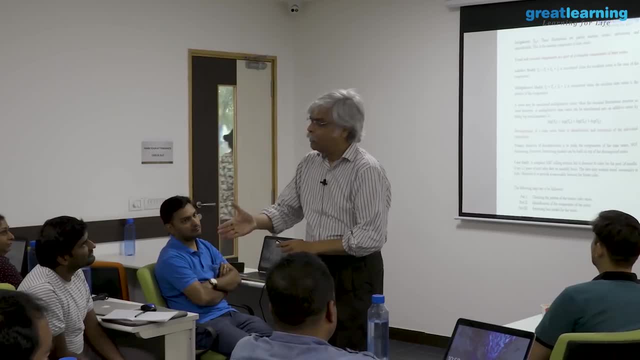 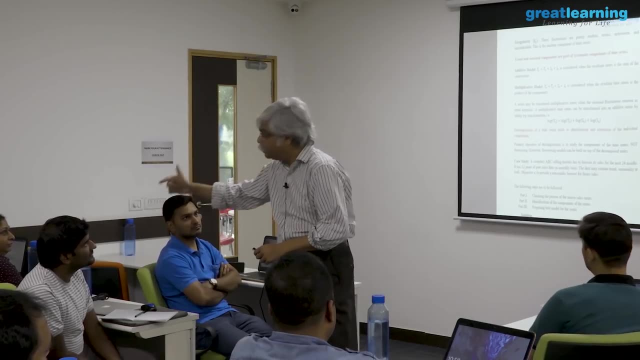 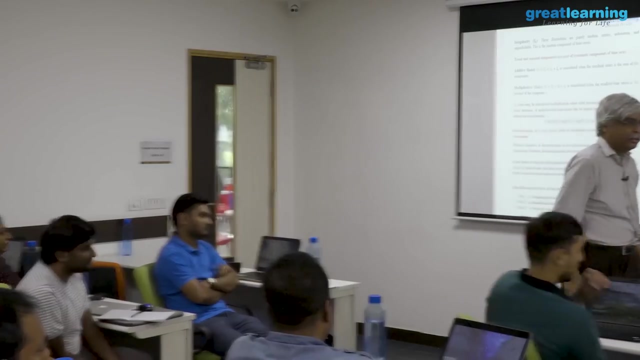 you, someone who would have had one chapati will have two. someone who would have had two would will have three. someone who would have had three would have had four. someone who had four would have five. it's additive- the first one- was not the first one. additive would have meant what the error is: 50 rupees if it's one rupee. 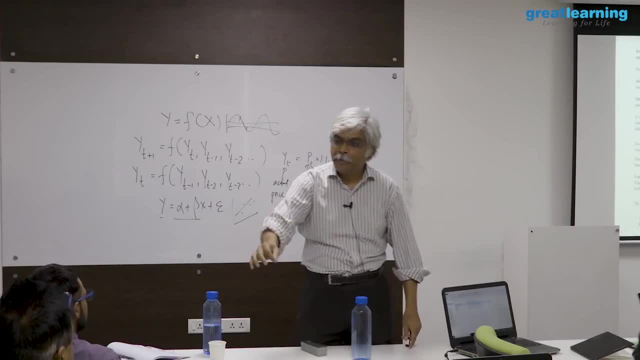 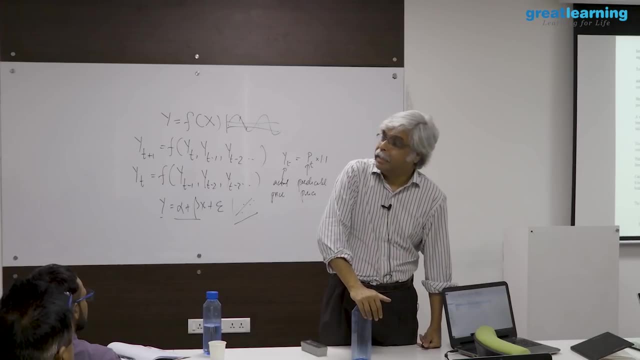 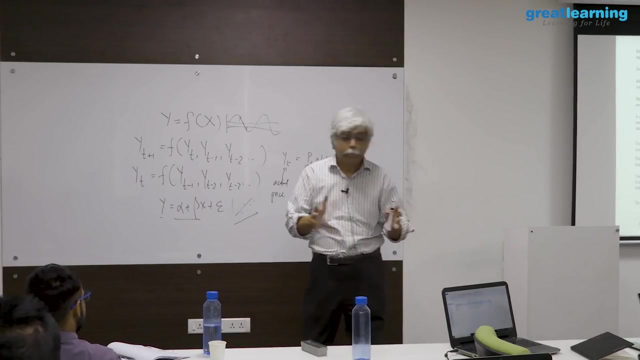 it's 50. if it's two rupees is 50. if it's five hundred rupees is 50. if it's ten lakhs is 50. if it's one crore, it's 50. it's always 50. that's additive. you understand the difference between the, between the two. so one of the things: 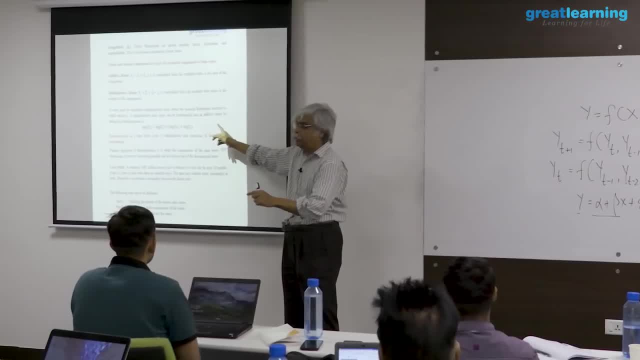 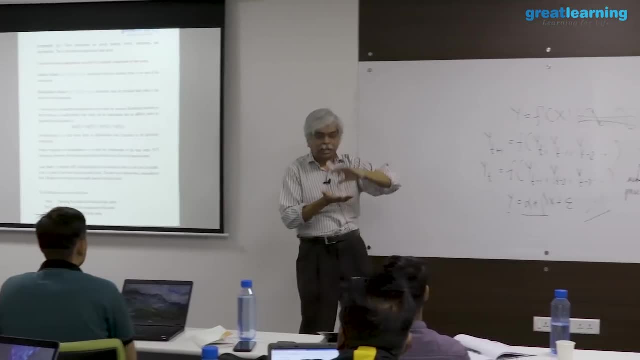 that we need to decide and the software will need to decide. when we run the code, you'll see that you'll have to specify whether it's additive or multiplicative. you need to see whether your series is growing in this multiplicative way or it is growing in this additive way. are you adding? 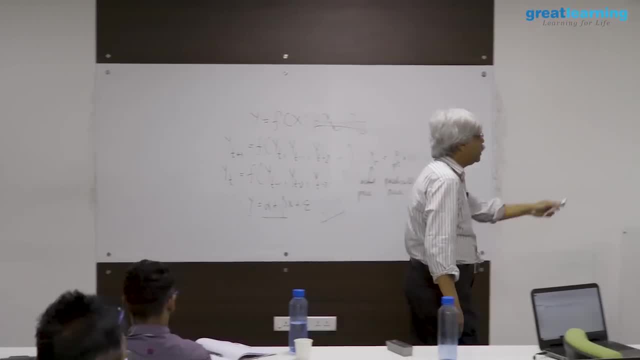 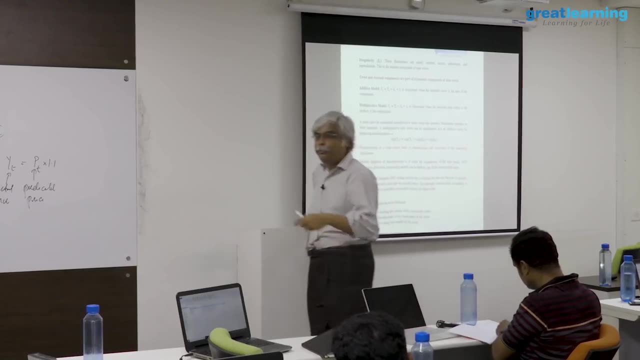 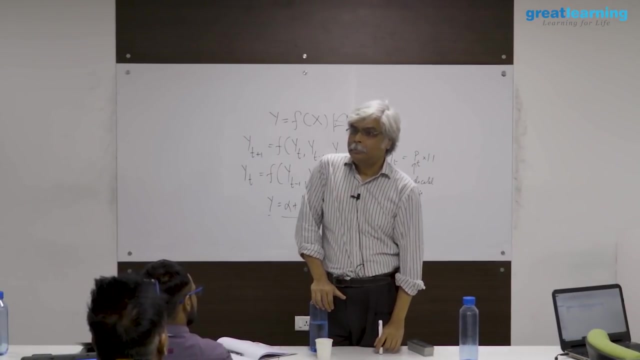 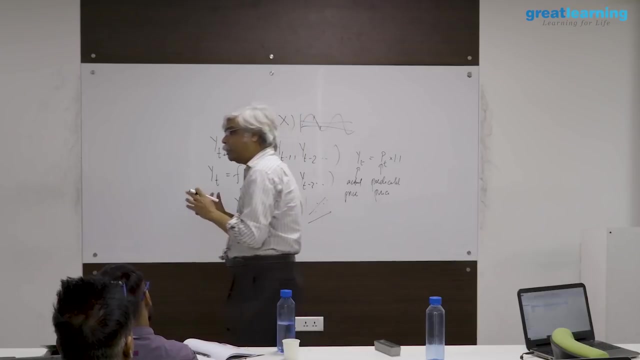 something on, or are you multiplying it with something, particularly when it comes to the error? now, the same thing, as you will see, is also going to be true for seasonality. if you are running a sweet shop in festivals, how many more sweets will you sell? will it be a multiple or will it be a plus? it could be multiple. multiple means what? multiple? 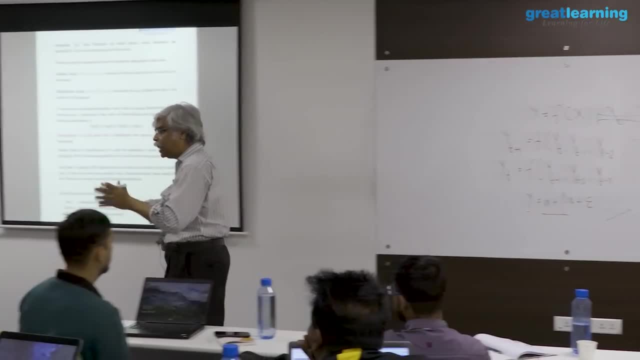 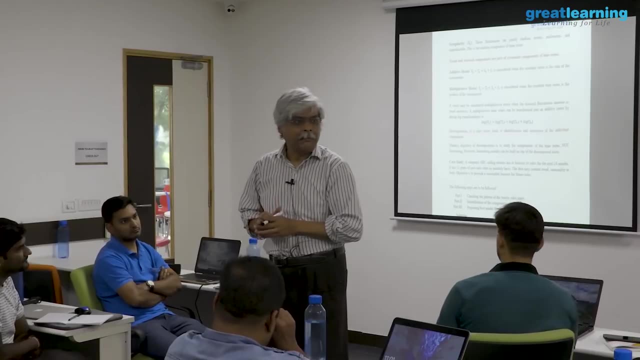 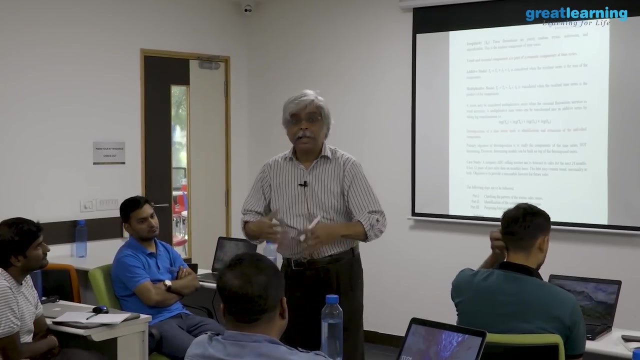 means. let's say you say 10 percent more, which means that if you are selling 50 sweets, you expect to sell 55. if you are selling 100 sweets, you expect to sell 110. if you were selling 400 sweets, you expect to sell 440. if it's multiple, if it's additive, that means 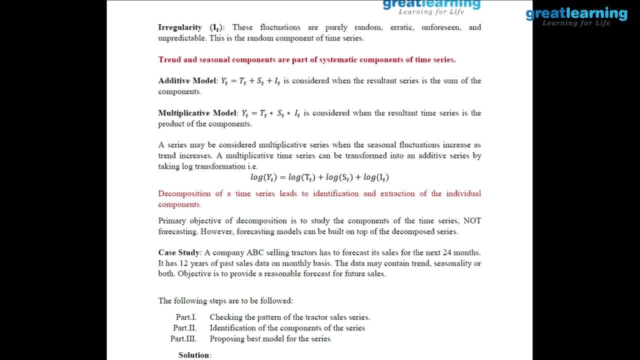 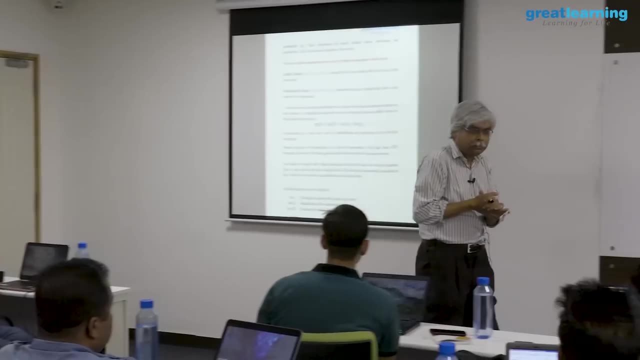 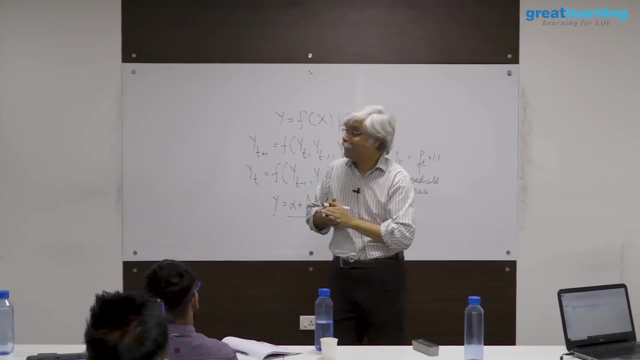 you expect to sell, let's say, 20 boxes more, whether it was some, 30 will go to 50, 100 will go to 120, 500 will go to 500. so these are two different assumptions. both could be right. do you expect to raise next year? don't answer personal question, but if you. 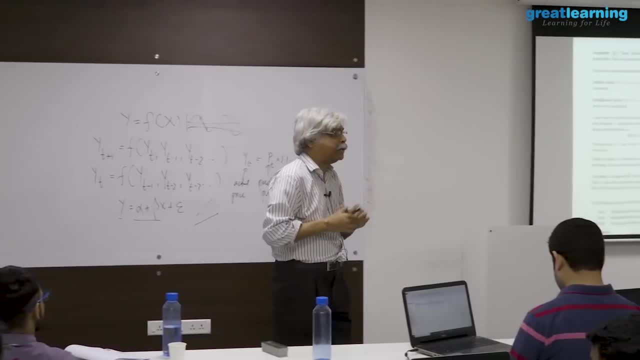 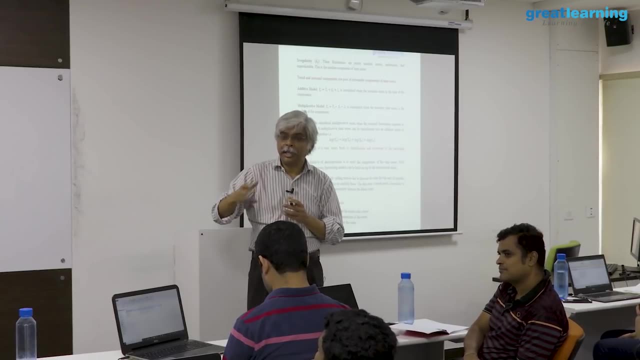 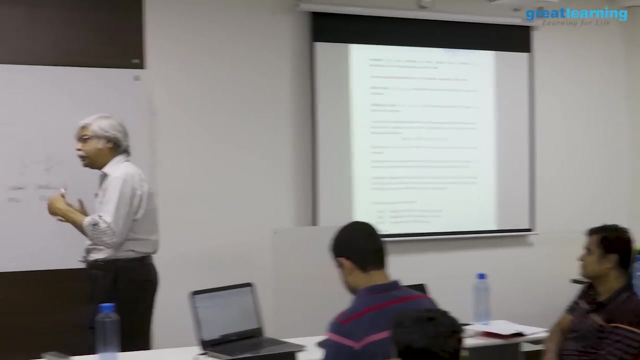 expect to raise next year. how is that working in your head? how much raise do you expect? usually it's multiplicative, which means you're saying: i want a 5 raise or a 10 raise. sometimes, on rare occasions- you also translate this into additive numbers. what does that additive numbers means you? 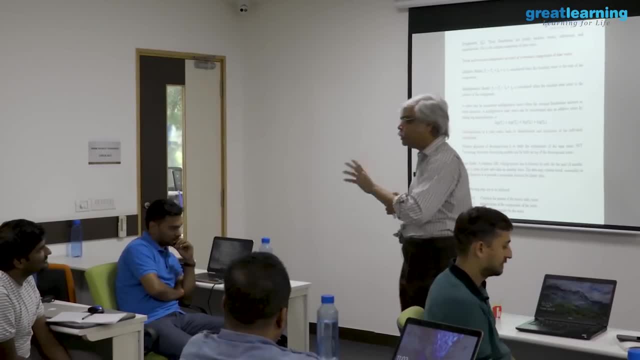 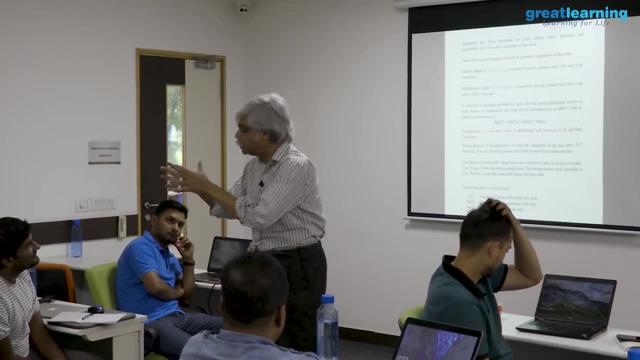 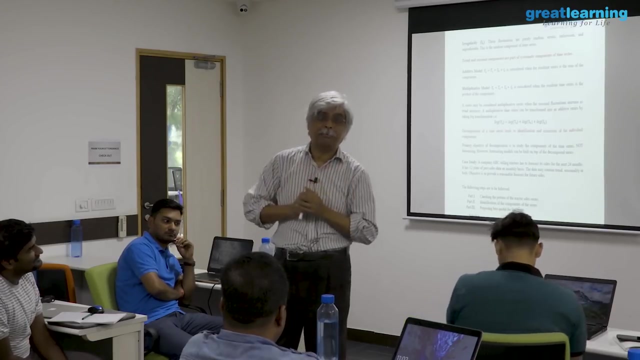 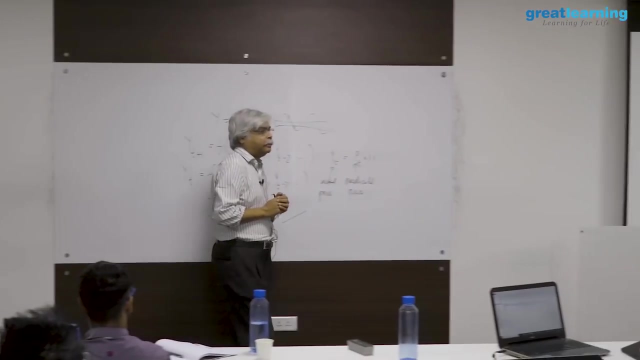 think, not in terms of multiplication, but you think in terms of saying: okay, I want three lakhs more. what matters is not the, not the five percent increase, but what matters is the three lakh increase, that that actual money matters. so you're interested in an additive jump. but usually salaries grow, multiply. 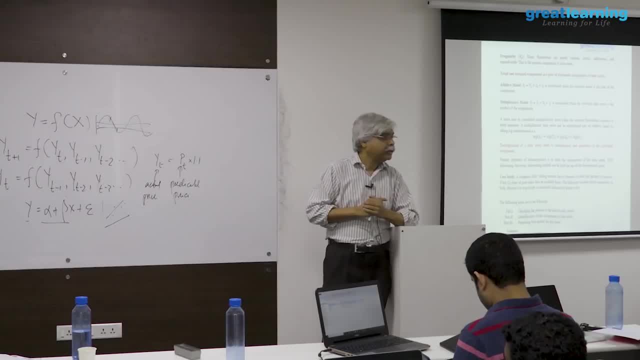 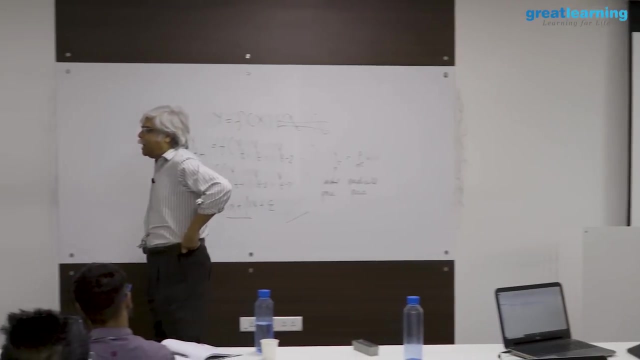 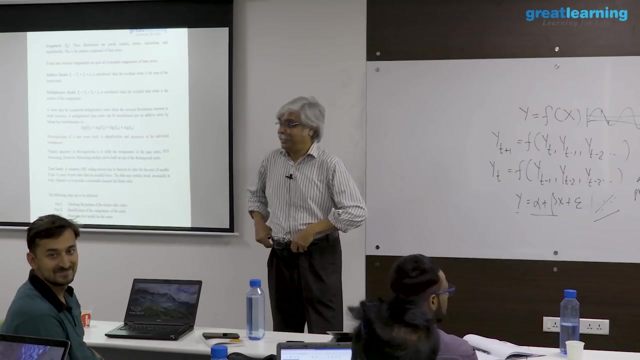 multiplicatively. why? but why is it? because? yes, because to some extent, everything is multiplying. prices are multiplying, therefore, wages are multiplying, therefore, all of this is multiplying. are any of you kind of managers or are responsible for paying salaries? not there yet. this leads to a very interesting problem, because what happens is that the your 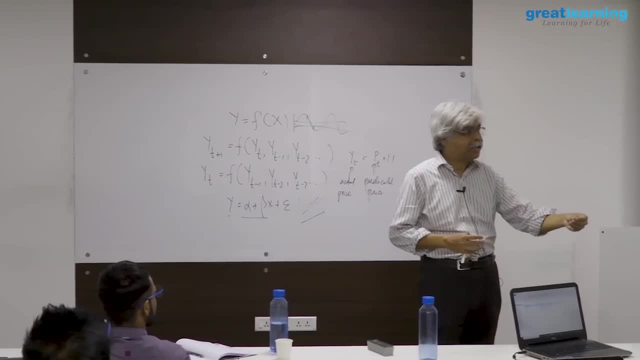 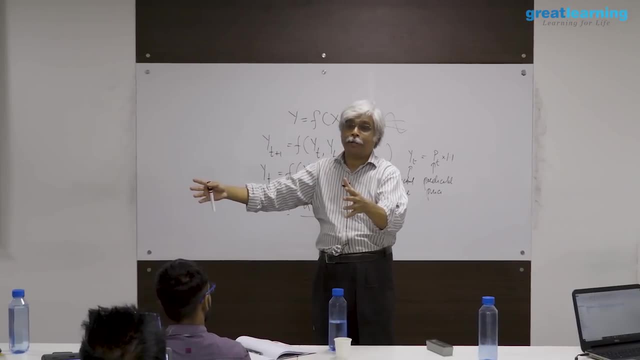 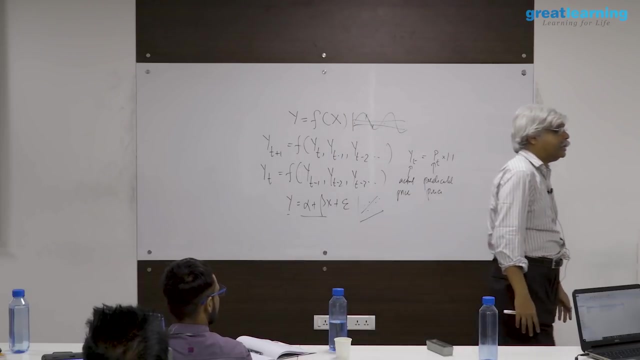 employee is, if your manager employees what expect a certain percentage increase, correct, but that increase often has to come out of a lump sum of money that has been given to the manager. so the manager of the business says that this is the extra amount of money that I have to distribute as salary increases and that 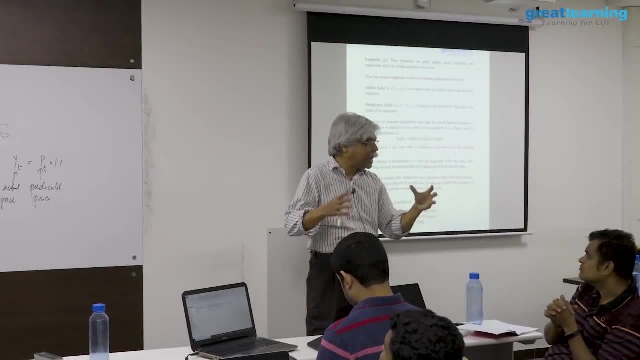 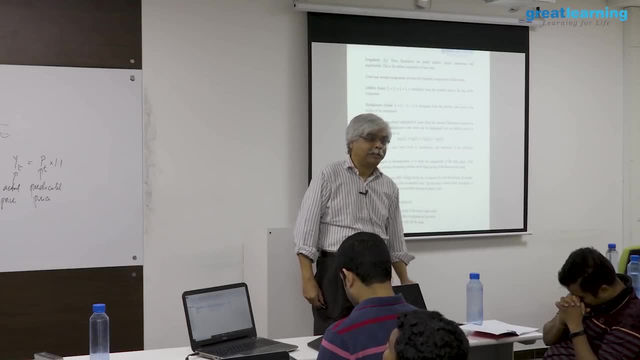 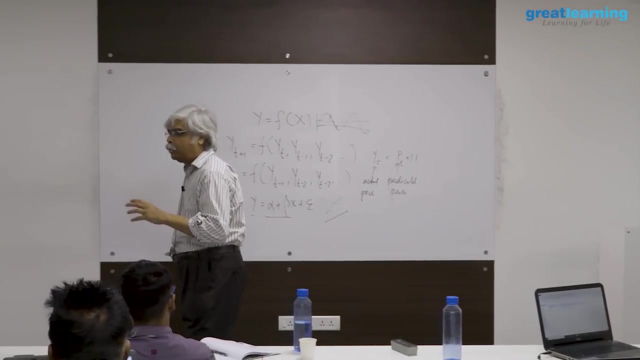 has to be now distributed among everyone. it's an additive concept that has to be implemented multiplicatively. this is to some interesting situations in your own mind. you can think of it as you can think of it, as you can think of it as it is there. what story to pick out from this right, from this injector? you can also pick. 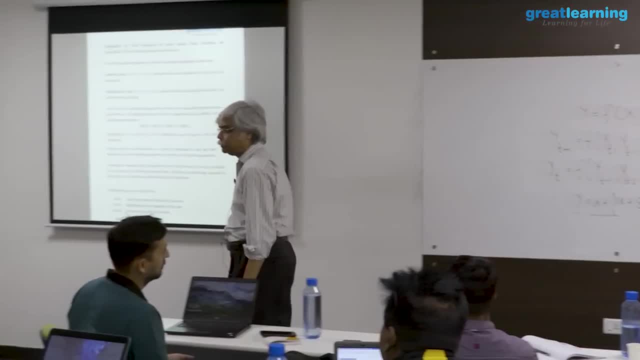 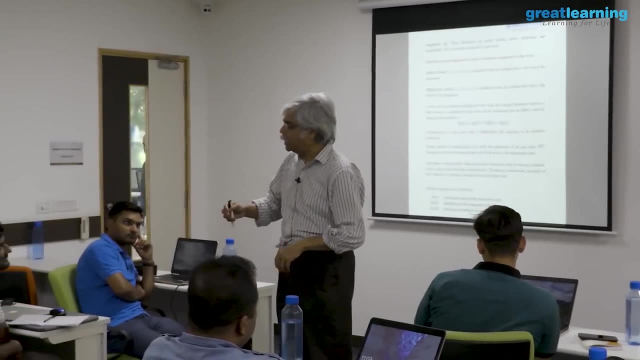 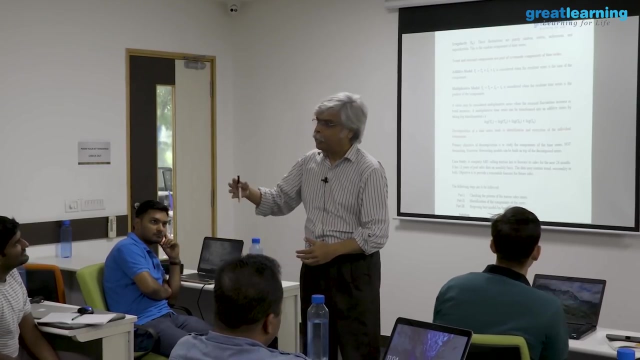 out why I paid you 1 lakh in this year after look at it. so this is to limit the services. there are more staff. well, what you can do to get every employee to have these services, there are many ways to increase it better. if youall you know, it only save very much. 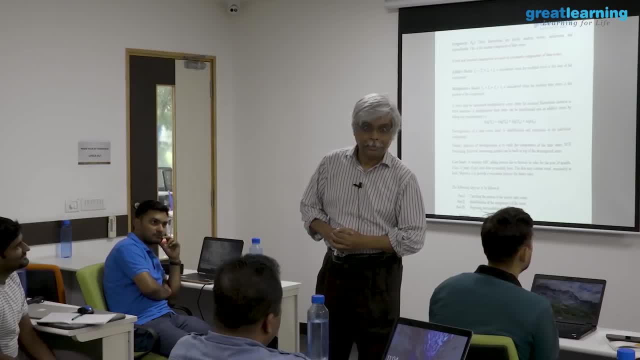 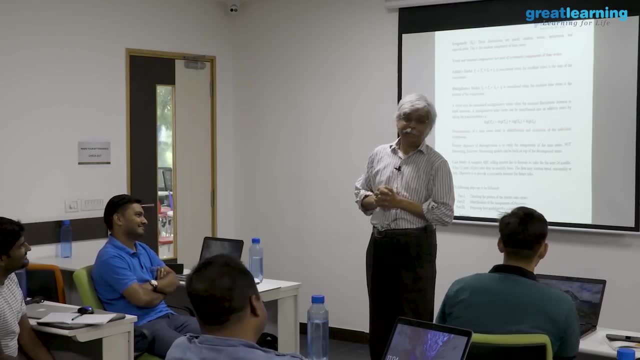 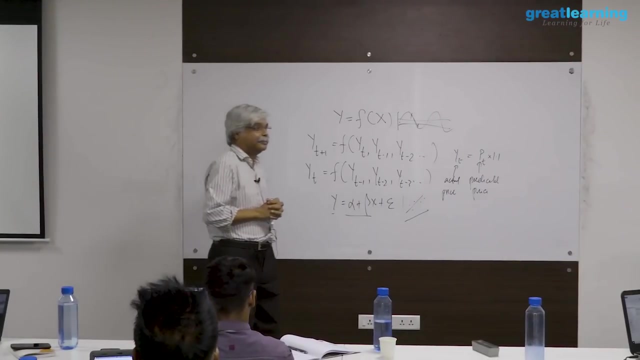 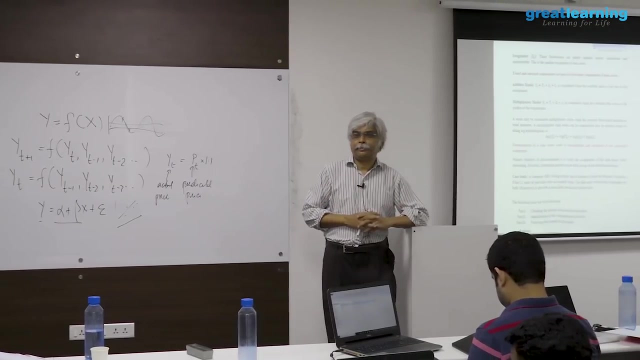 dollars. when youiry out yourime, which is at least about put in your element, is: think about what's going to happen, depending on who it is. you understand the nature of the problem in practice. what therefore happens? higher paying people in this distributed situation tend to get less, which leads to a 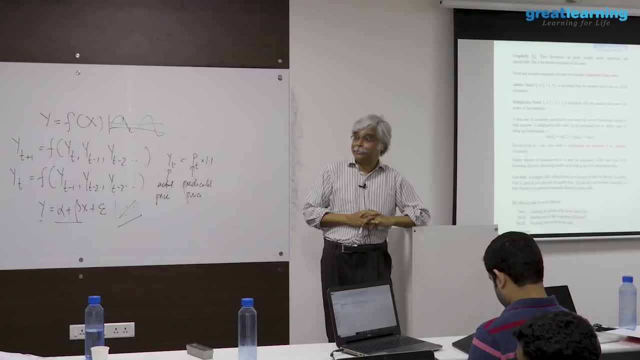 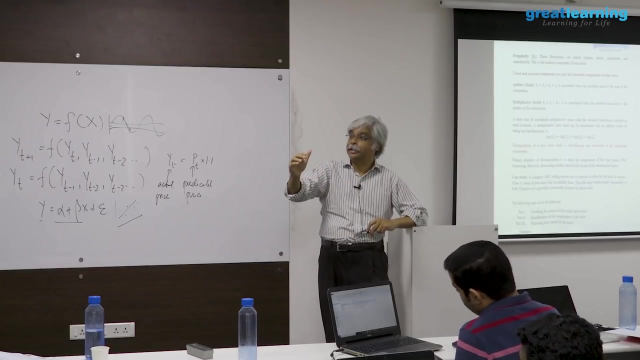 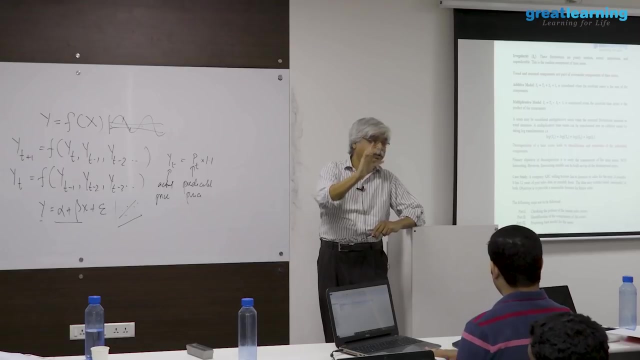 certain amount of mid-career frustration. I say Q with I. I'm doing very well, why am I not getting my raises? and one reason you're not getting your raises is because your baseline is very high. so giving you a reasonable multiplicative raise actually costs a lot of additive money. the actual rupee amount for even a 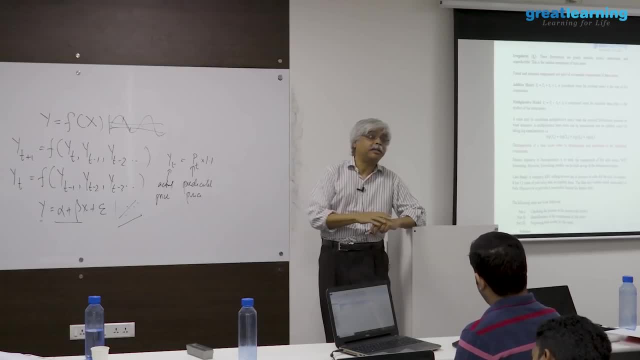 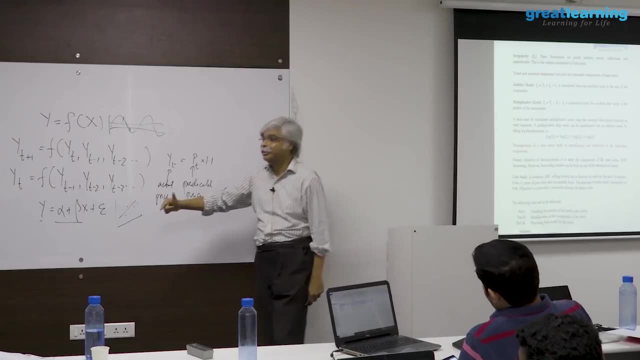 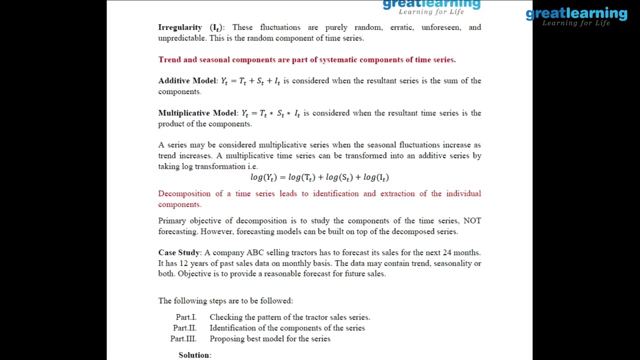 small multiplicative raise is a lot of money and that takes away a lot of money for other things. so the more you make, the more the pressure on the organization to give you less. this is not nice, but these two things often pull together. so before we break, I want to just 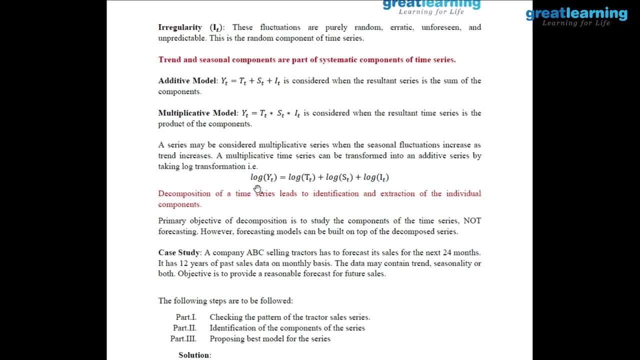 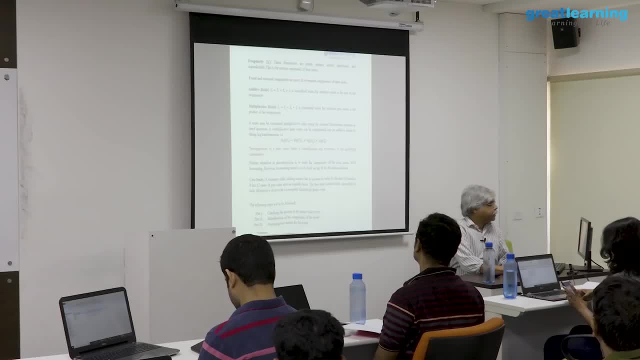 introduce things a little bit first, a little bit of a math issue. the math issue is this: that if things multiply- and I take logarithms- then things become plus. you can think of this as just algebra or you can think of it as saying: what is a log do? log essentially counts the number of zeros. for example, log base 10. what is? 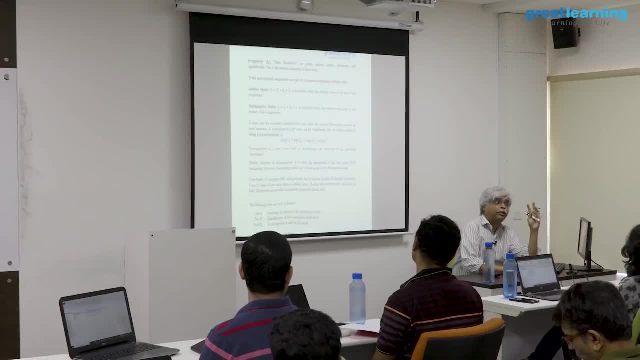 log 10, 1. what is log 100, 2, what is log thousand, three log calculus, a number of zeros. so this basically says the, the number of zeros that gets added remains, to some extent remains the same. you know, 10 becomes 11, now hundred and hundred becomes hundred, and ten thousand becomes thousand one. 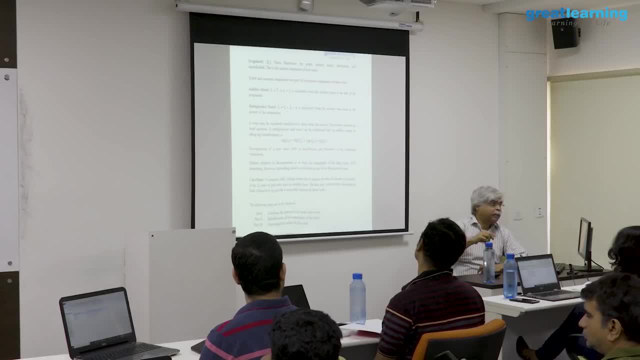 hundred. so something in which is which is multiplies means that on the scale of the number of zeros it becomes additive. so every time I'm still, I'm adding the same number in the logarithm scale. so multiplying by hundred means adding one in the log scale. multiplying by 10 means adding one on the log scale. so anything that's multiplicative on the original scale becomes additive on the logarithmic scale, from from a. from a software perspective, what this means is that you don't really need a multiplicative model. the question becomes: should I act on the original scale or should I act on the logarithmic? 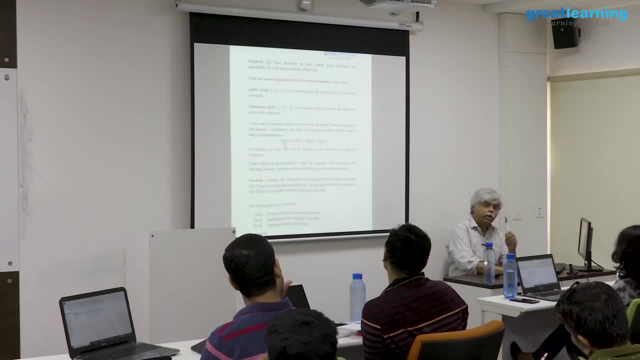 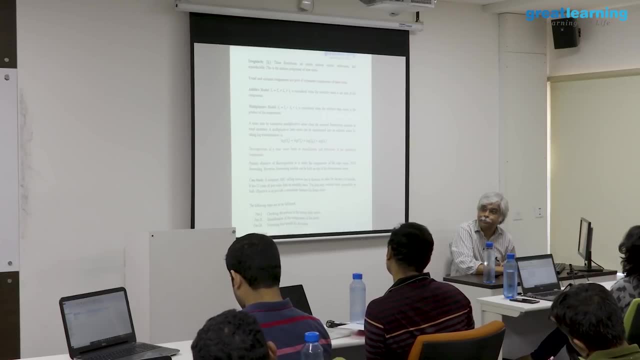 scale. if it is multiplicative, then I should act on the logarithmic scale. I should not try to predict your salary, I should try to predict the number of zeros in your salary, zeroes on the back end, not the front end. so all right. so now to introduce the case. 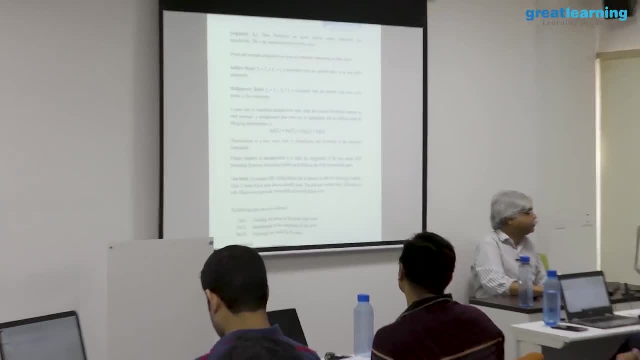 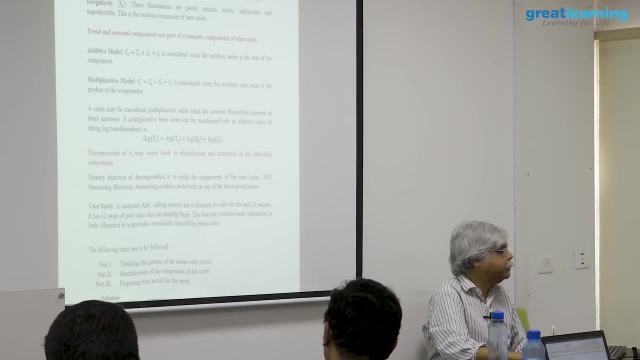 study a little bit. a company selling ABC tractors has to forecast its sales for the next 24 months. this is the problem. it has 12 years of past sales data on a monthly basis. the data may contain trend seasonality of both an irregular part. objective is to provide a reasonable forecast for future sales. so you got. 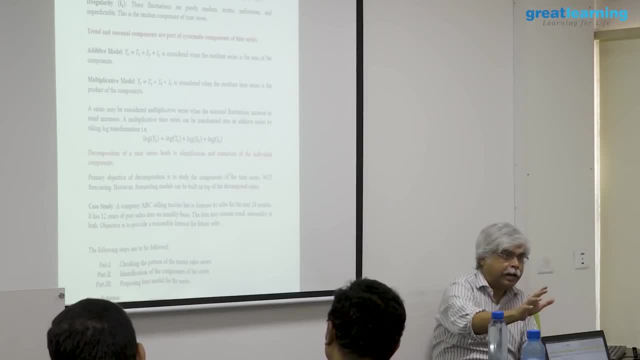 sales of tractors. now, to predict sales of tractors you may need many things, but, as we just argued, for teaching purposes we don't look at this. and even from business perspective, it could be that all that other information is already been baked into the sales. competitive pressures, costs. all of that has already been. 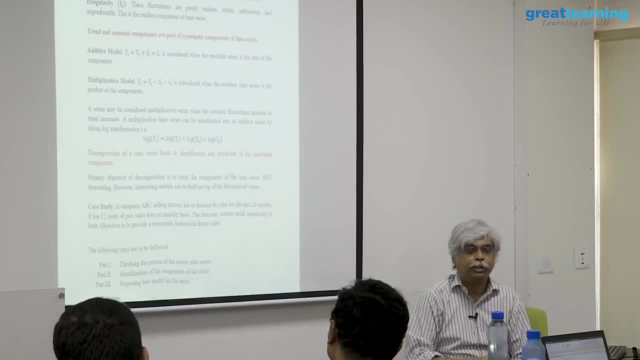 factored into the number of tractors that you are selling. so simply being able to predict the sale of tractors based on the sale of tractors that has happened before may be good enough, right? okay, now let's do this a little bit and then we'll take a break. let's at least see the data and then we'll see. 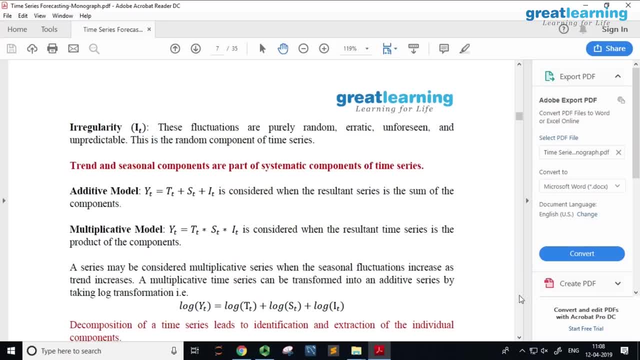 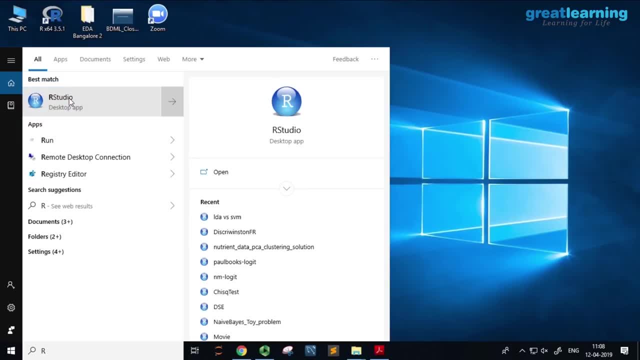 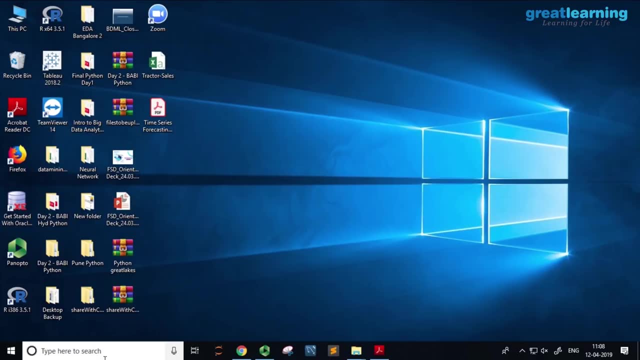 this. so if you could go to R, there is only one, so R, there is only one data set. so this data set will be called tractor sales. it should be an excel spreadsheet, it should be a CSV file. okay, now, before we, before we see it or get to. 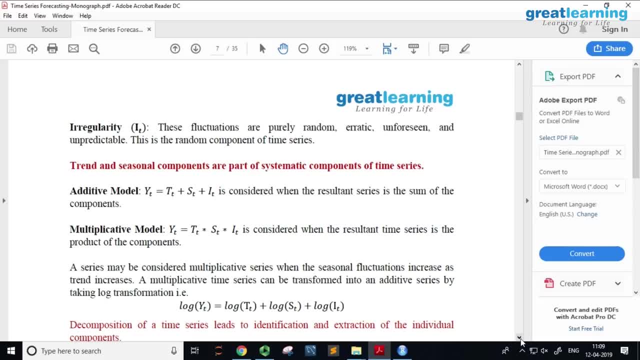 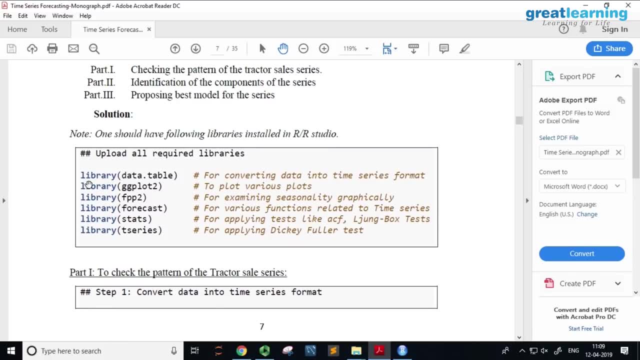 it. we're going to need to do a little bit of prep work for the descriptive part. there are certain packages that need to get in these things here. this is going to take a while, and if it takes a while that's fine. so, for example, there's: 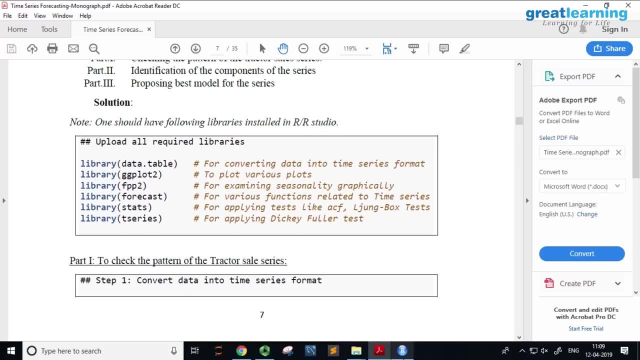 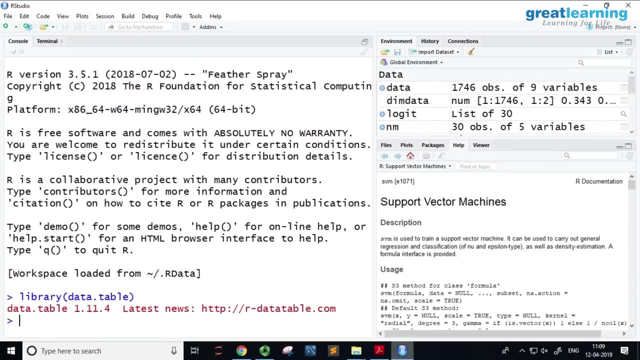 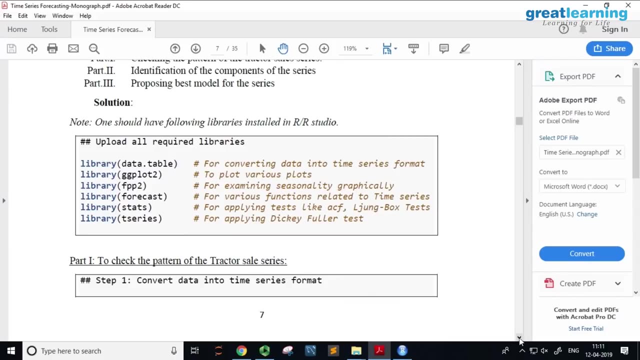 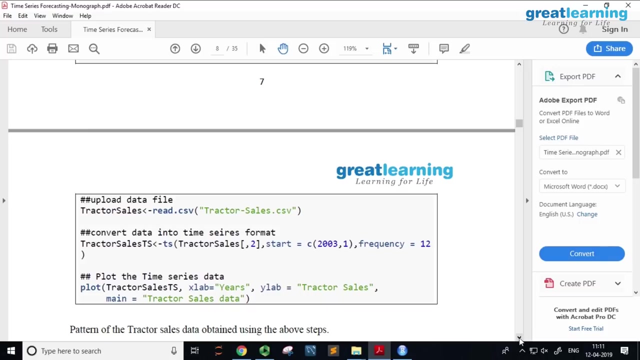 so these libraries will need to be added on. so library data dot table in this computer. a lot of this should be there. ggplot2, this is also something that you should have used. the R file is here. I mean all the R code is here. so all the R code is embedded. 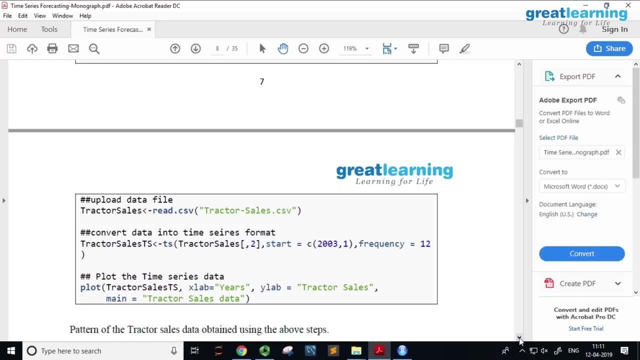 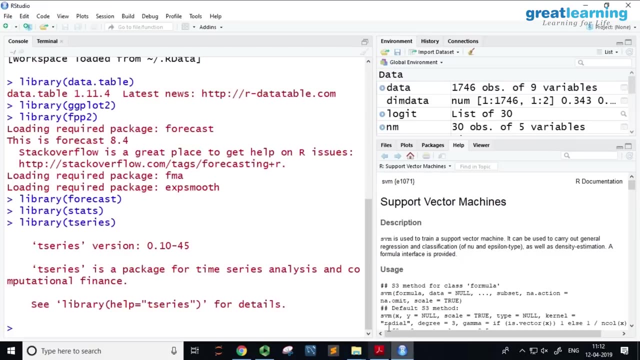 all the R code that we'll use. by Sunday we may have enough experience to do our own analysis on this so we can repeat this for other data sets. but with that spreadsheet and this material, it should all be self contained within this. so tractor sales: now for me. 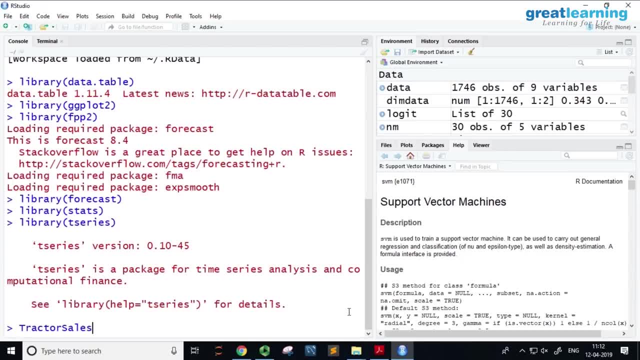 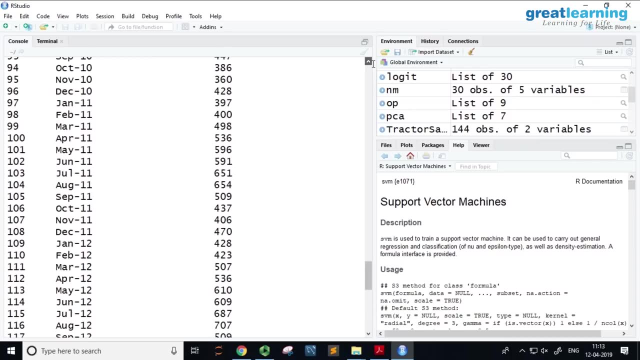 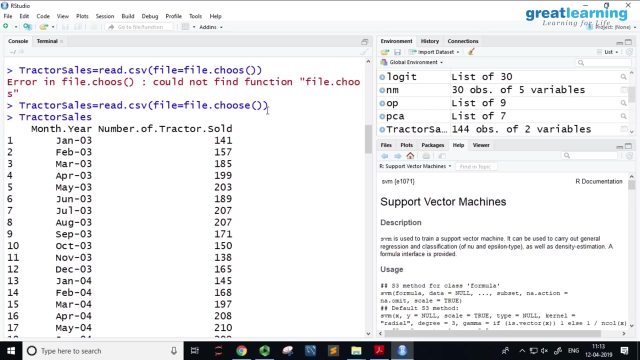 ggplot2. it's probably necessary to get the naming of this little bit, so from the way I will do it. so this is what tractor sales looks like. this is what it looks like in the spreadsheet. do it this way or do it through you know path, or whatever you want to do it. 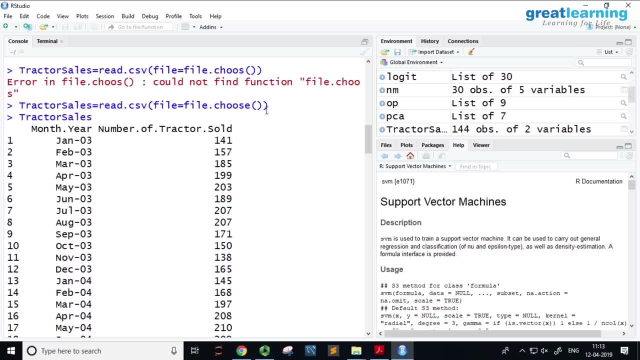 so your computer should be set up to read this spreadsheet. so this is what it looks like in the spreadsheet, so you can read things a certain way. this I'm doing simply because every time the course is done it's on a different computer, so it's always on a desktop. 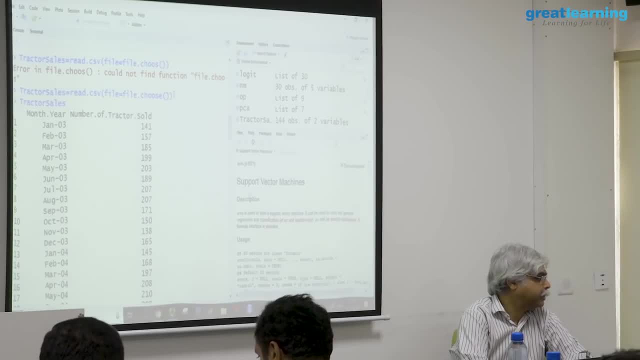 the path is different. so this is a little bit of a hack, that's all. I suggest you not do this, but if you are uploading the libraries for the first time, it may be a little slow. this computer has the libraries already uploaded now. one possibility is I can simply do something like this. let's say 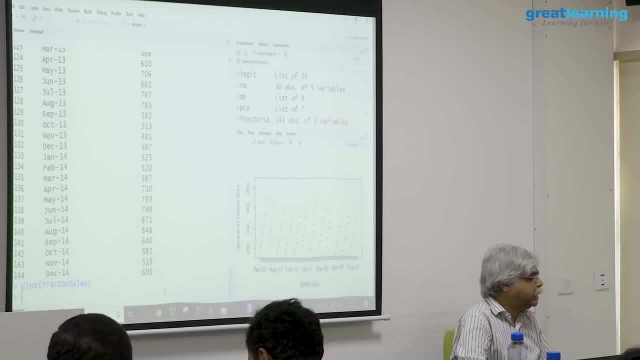 now, if I simply plot this series, as is, this is what I get. this is what I get now. why does it look like this? the reason it looks like this is when I give it a plot, it's taking this as the x-axis and taking this as the 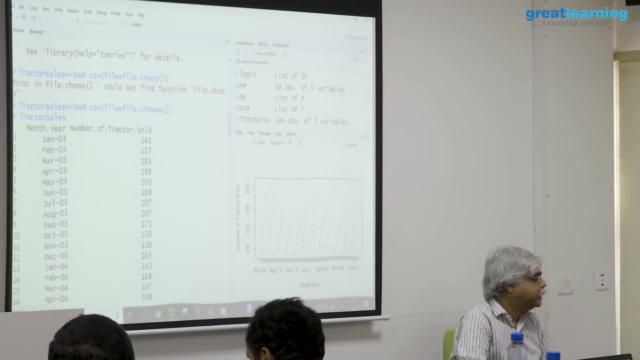 this month dot x-axis and my number of tractors cells becomes my y-axis. but as soon as this becomes an x-axis, where does this variable begin alphabetically? so it's going to begin with April or August, or something of that sort. in short, it doesn't know that this is a time series. 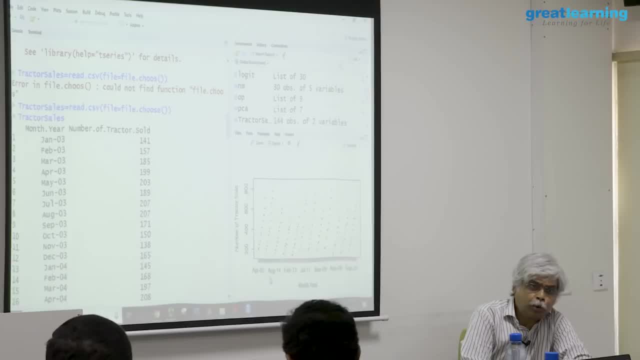 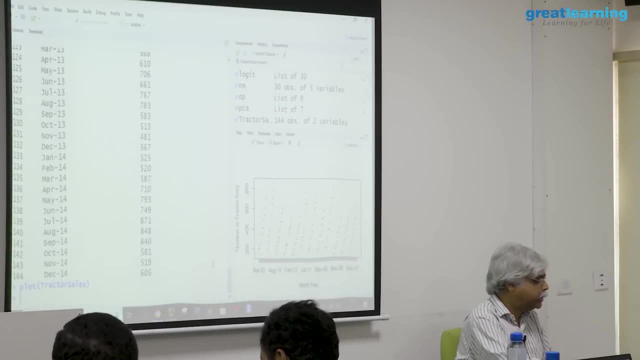 it doesn't know that this thing is a time series. now I can do only the second one as well, but if I do only the second one, in other words, other words, if I do it this way and I do say comma 2, which is not the first one, 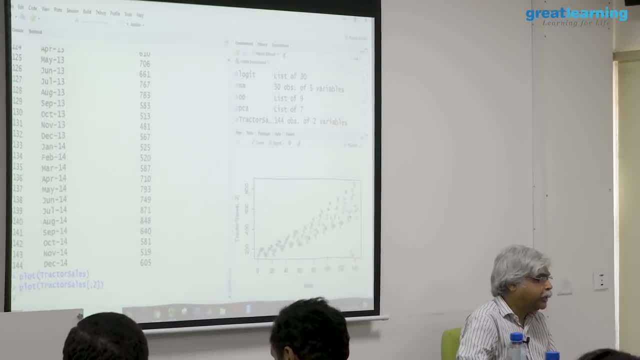 but the second one. then I will be able to recover it. but now, what has happened now is number. I've lost the, the months. I can in fact even remove this and let's say I go something like type equal to I don't know L and see it. 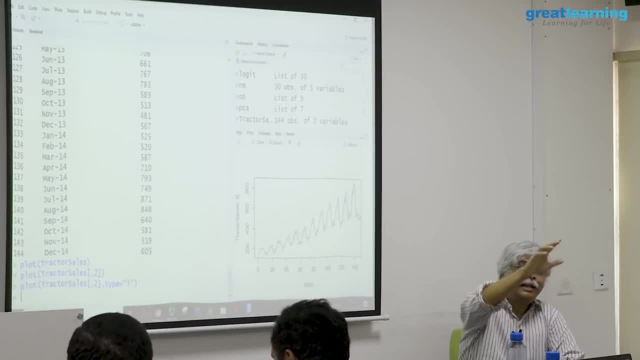 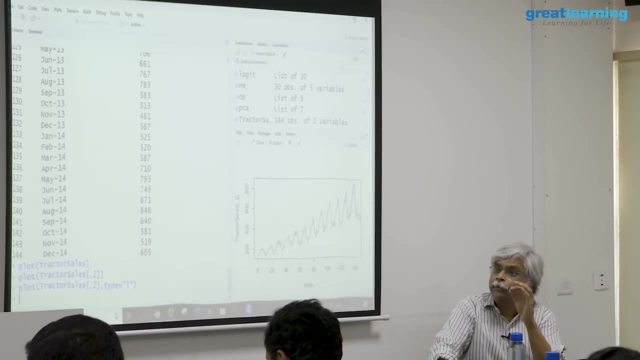 but either I lose the, the variable, or I lose the label. so what I need to do is I need to convert this into a time series object before I do any analysis. this, this, this, this data frame inside R doesn't look like a time series object. I. 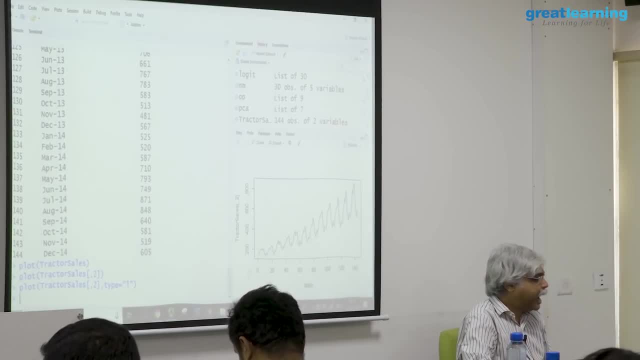 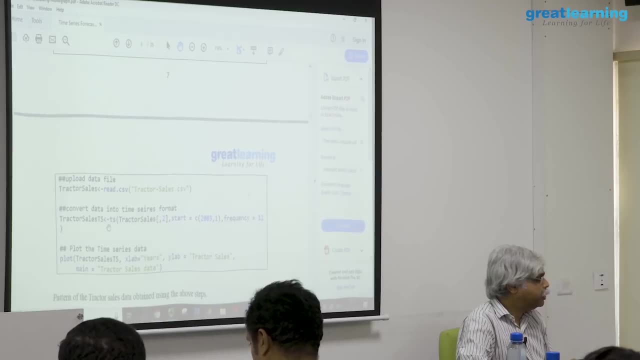 need to convert this into a time series object. so the way that happens is: here this thing, here this TS. now what? what does this trick? what is this requiring me to do? first of all is requiring me to identify the time series. is requiring me to tell me, tell me where. 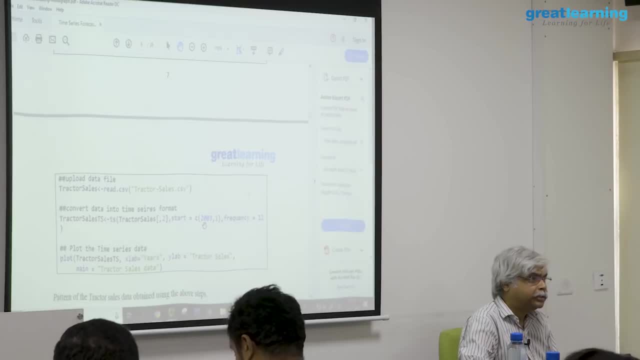 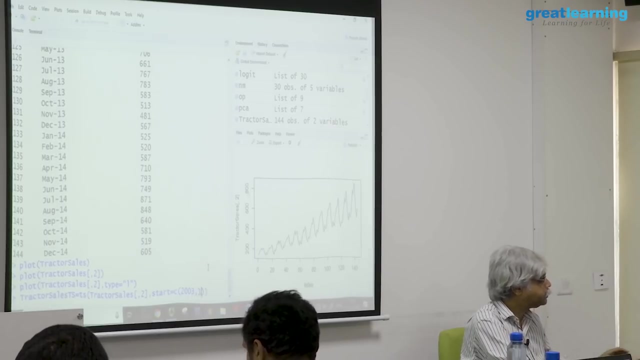 do you want it to start? right, where do you want it to start? and is also giving this frequency equal to 12, which is any, which is an interesting thing to see. where does this 2003 come from? so 2003 is the first year where it starts. so I'm saying: begin on 2003 comma. 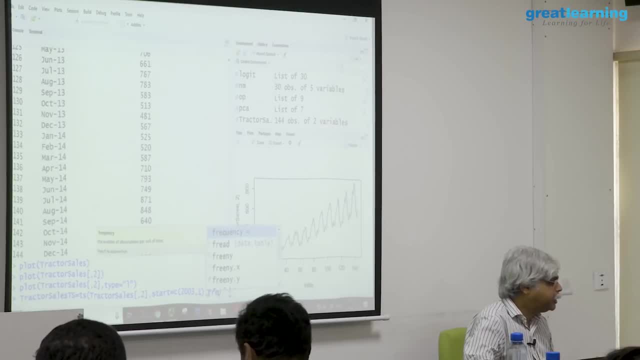 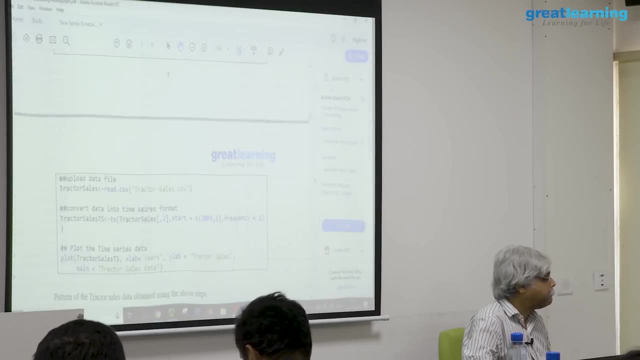 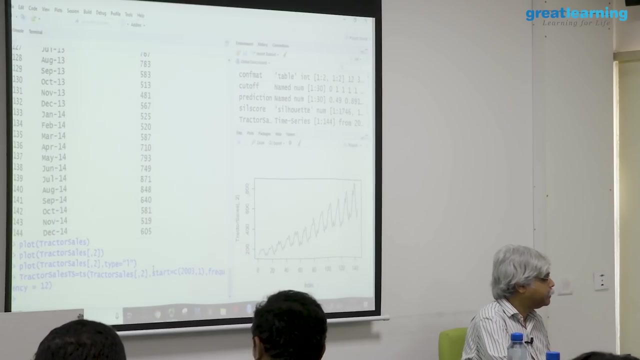 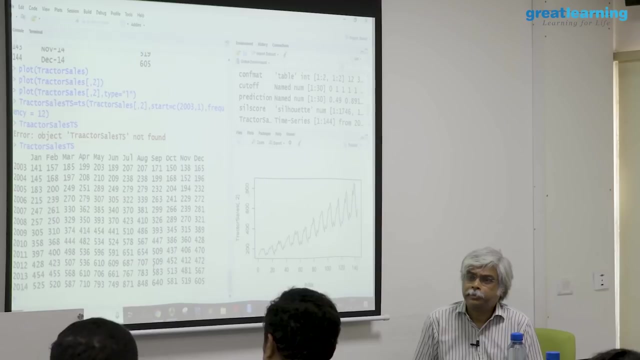 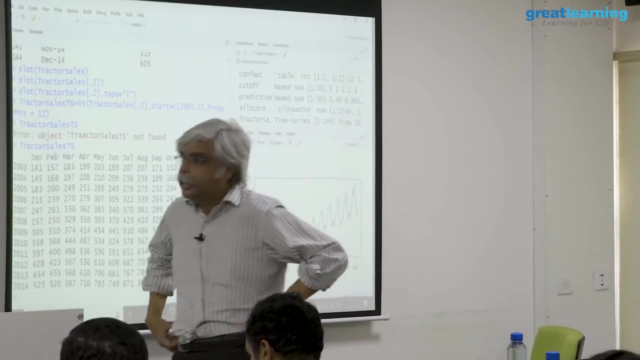 1 will see where that goes. and then frequency equal to 12. right frequency equal to 12 tractor sales TS. you, you, this. let's see what this is. as you will see soon, my art skills are other limited. this is what it looks like now. some strange things happened. one somewhat odd thing happened, is it somehow? 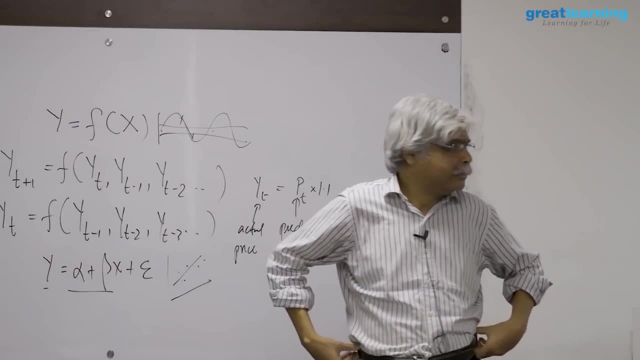 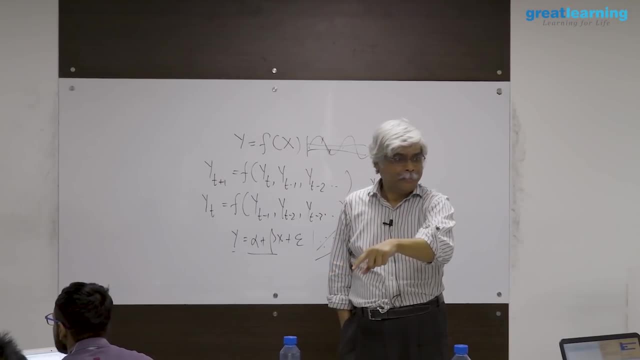 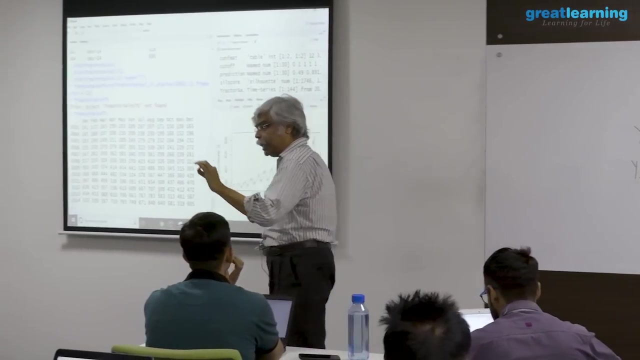 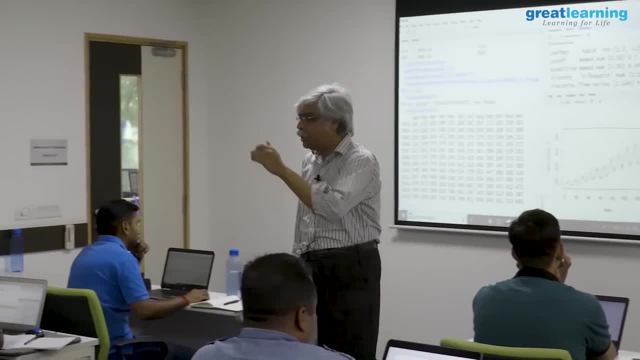 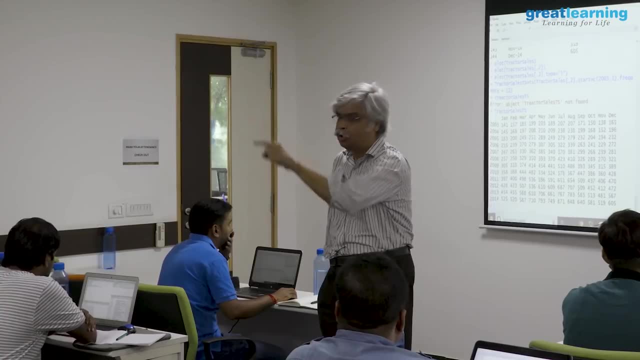 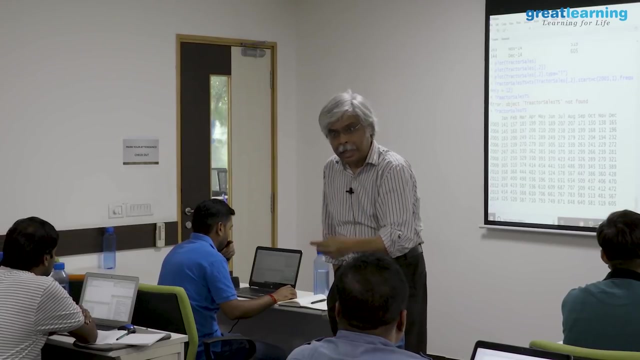 understand what that one was. so now says: how many of these do you want in? two thousand and three before I get to 2004? frequency called it. well, says: go twelve times 2003, comma 12, and now it will become 2004 comma 1, because frequency has been given as: 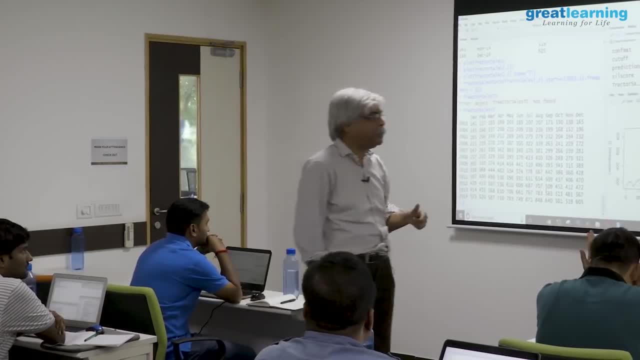 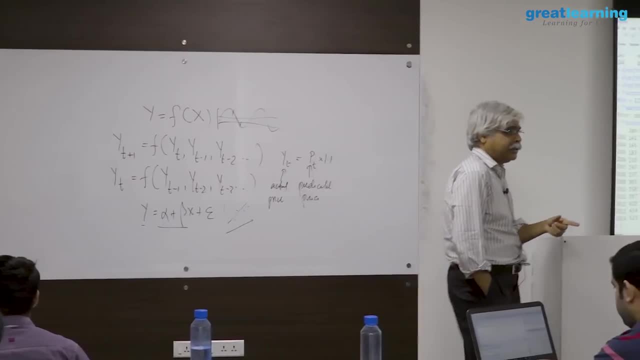 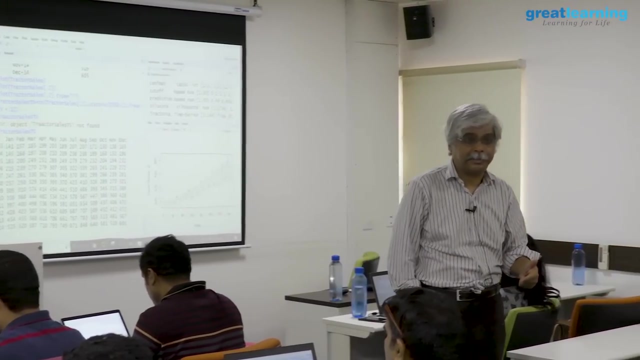 12. now what happens is because of TS. it is assuming, perhaps unfairly. it is assuming- that what it has given me is months and the 2003 corresponds to years. this is hard-coded into it. this is not common sense. this simply the idea that if you, if someone is saying frequency, 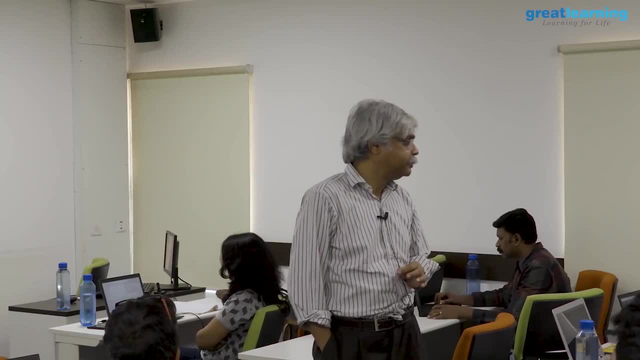 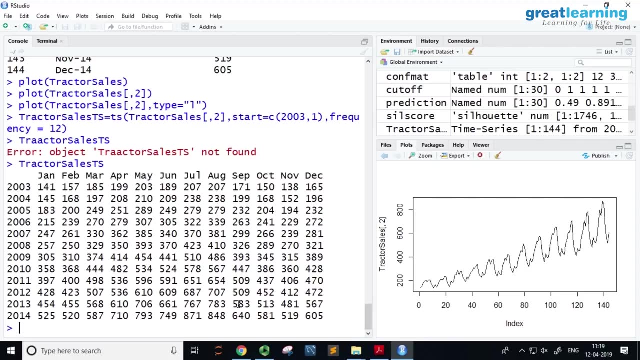 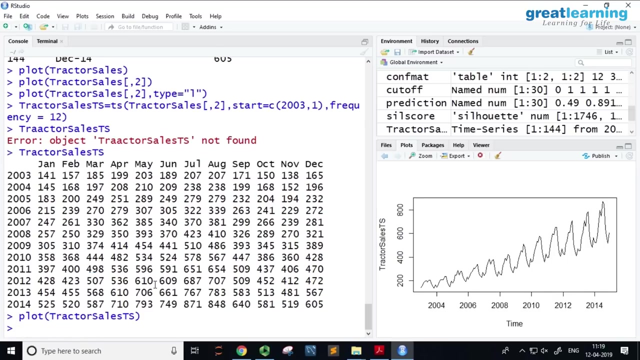 is equal to 12. somebody is wanting to give me months. this is now a time series object, so, going forward, if you want to treat this as a time series, this is the object on which you will. you can do your calculations, true, which is why I am saying it is a little too. 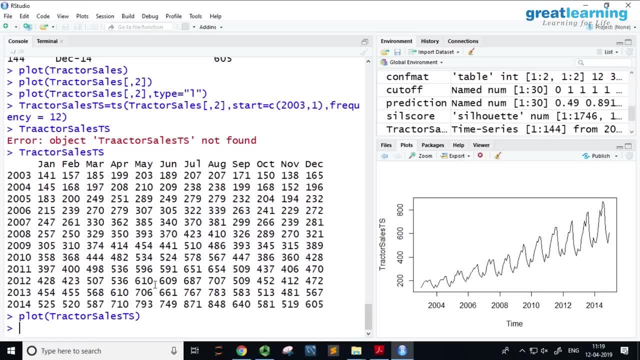 it is, it is been hard-coded into it. it will not. it will not. so, in other words, if you want to give it 30, you can try if you want to. so, for example, if you want to give it 30, you can try if you want to. so, for example, 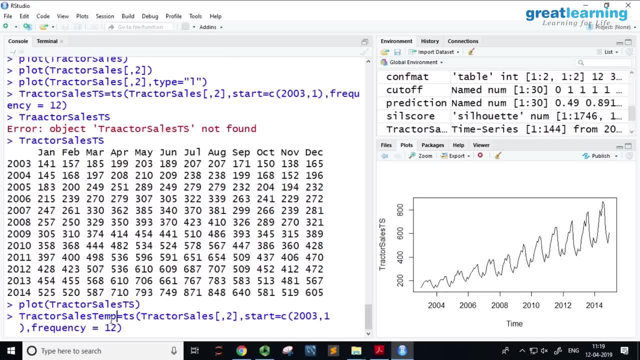 you can try and see what happens. so what I am going to do is I am going to- and let me change this- let us say to 4. if I change this to 4, it is going to pretend is co-quarterly, but it is going to do so, it is going to do something interesting. so let us say I do this. 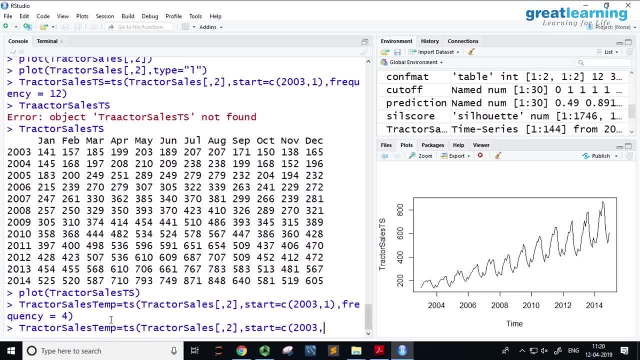 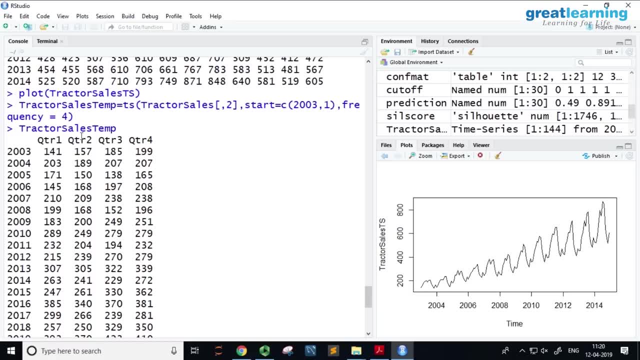 and now let us say: I do so. in other words, I see what this is. here is what this is. it now is going to say: quarter 1 quarter, 2 quarter, 3 quarter, 4 quarter, 5 quarter, 6 quarter, 7 quarter, 8 quarter, 9 quarter, 10 quarter, 11 quarter, 12 quarter, 13 quarter, 14 quarter, 15 quarter. 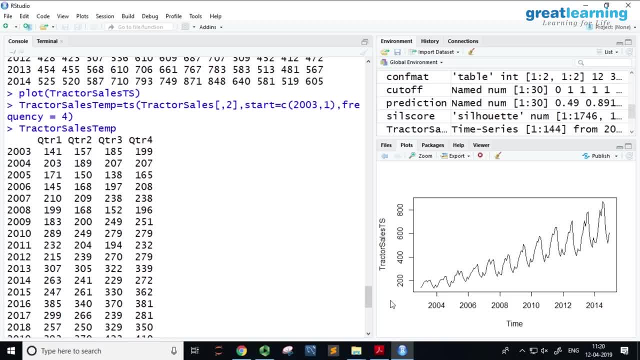 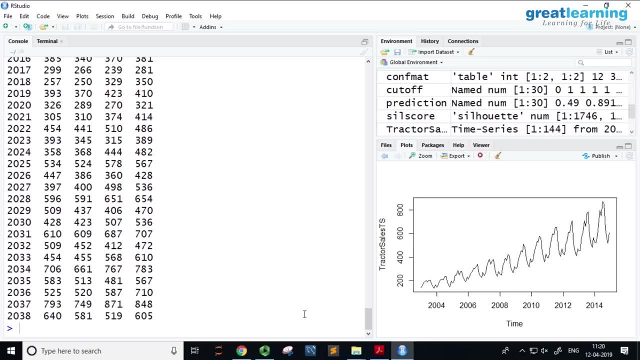 16 quarter, 17 quarter, 18 quarter, 19 quarter, 20 quarter, 21 quarter, 22 quarter, 23 quarter, 24. it assumed that it is quarterly, but it goes up to 2038. why? because it saw 144 observations and therefore 144 divided by 4, it saw 36 years. remember? it has not seen the first column. 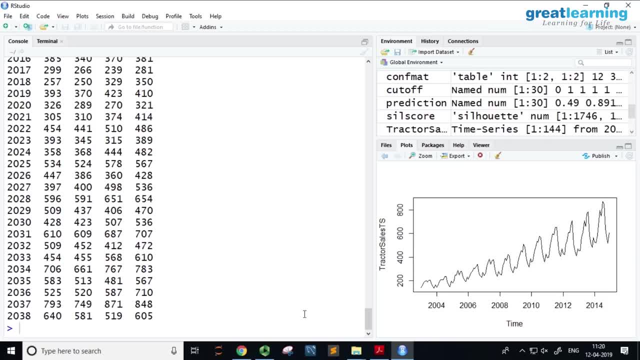 at all. it is only input, is a second column and now it is saying: okay, you want it to be okay, you want me to begin at 2003 and then go quarterly, cool, but now it is going to pretend that is gone up to 2038. it might be interesting to see if what you are saying. 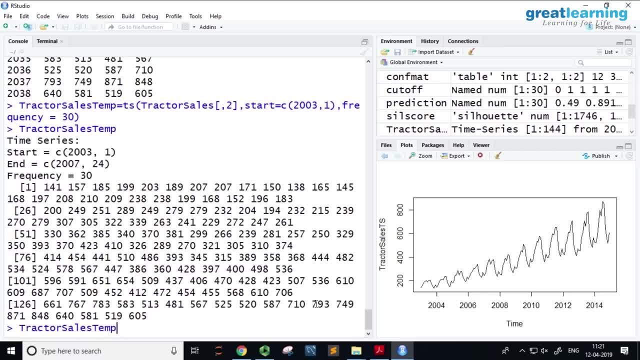 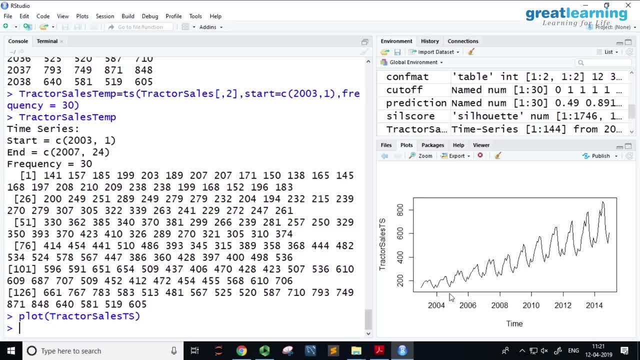 is correct that if I give it 30, what happens? so this function. so now, if I go back to tractor dot, sales plot here and you can plot it. this is now a time series. on this axis this is, you can see the years and on this axis you can see the sales. in between there are of 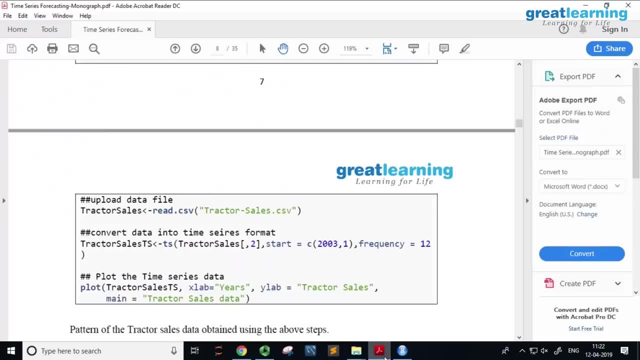 course, 12 readings for every year. you can see a more sophisticated plot if you want to, if you want to put labels on it and things of that sort. if you put x tab equal to years, y lab equal to tractor, sales, main equal to, it will just put labels on it. that is just 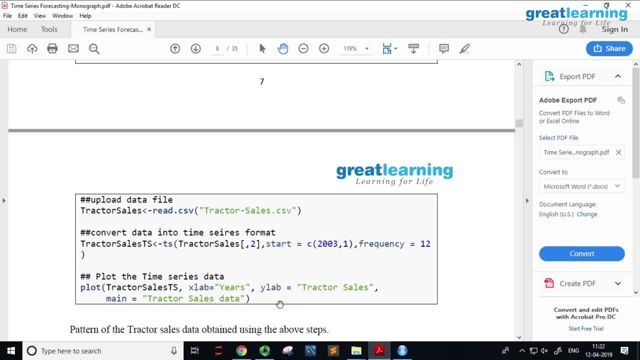 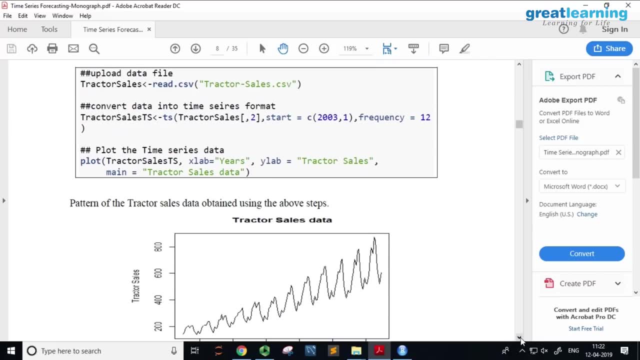 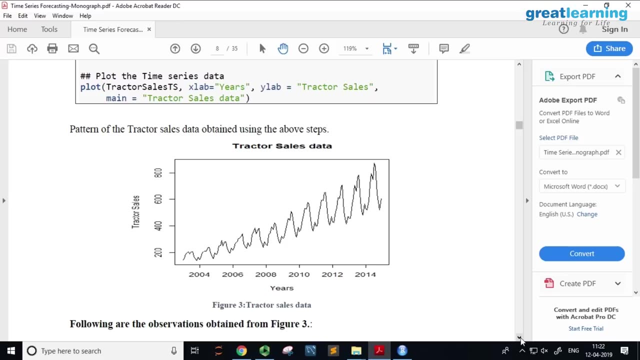 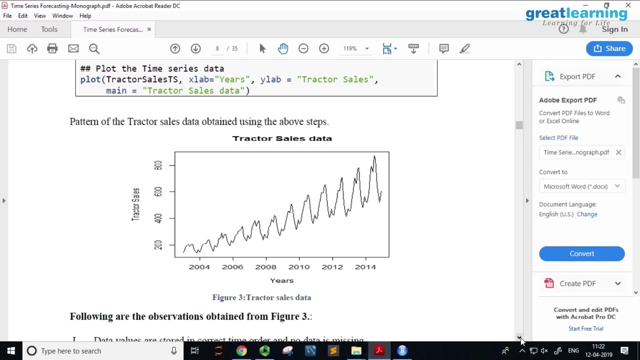 if you want to, you can do this as well. but the most important thing is this is the plot of tractor dot sales now shows the patterns of this. now, from this, what do you see? so, point number one: there appears to be a trend. trend means what? trend means that over the years on, the average, tractor sales is going up. that is. 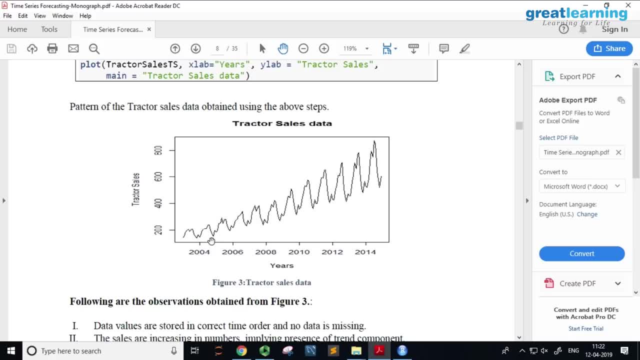 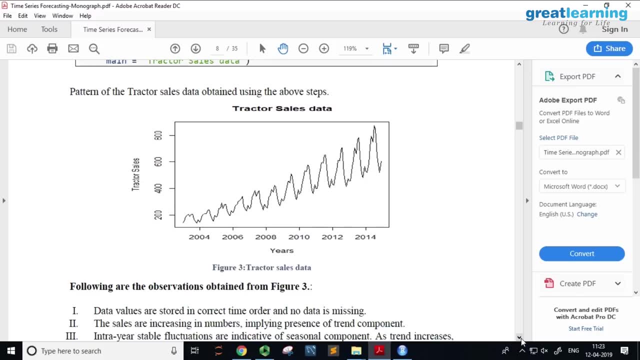 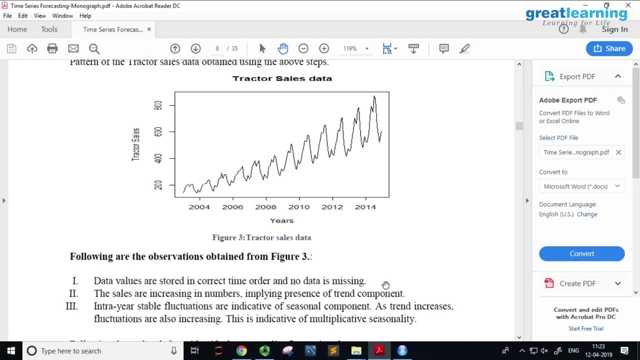 point number one. point number two: there appears to be a seasonality right. these two seem obvious. let us see if there are some other points. data values are stored in the correct time order and no data is missing. this is important for one sightly technical reason: in a time series, missing data is very toxic, because you cannot throw 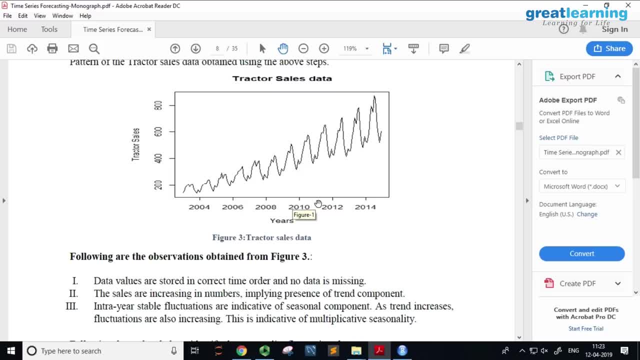 it away. if you throw it away, what happens? others will fill it in. there is a whole good that is going to be created in. the whole time series will jerk backwards, so everything will go wrong after that. so you can't have missing data. you have to do something with it either the code has to. 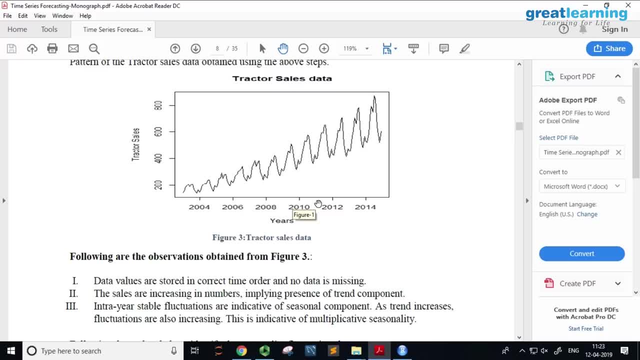 recognize it as missing data, or some number has to be put into it before you start the analysis. you cannot throw it away, so in this particular case that is not an issue. the sales are increasing in numbers implying the presence of a trend intra year stable fluctuation are indicative of a seasonal 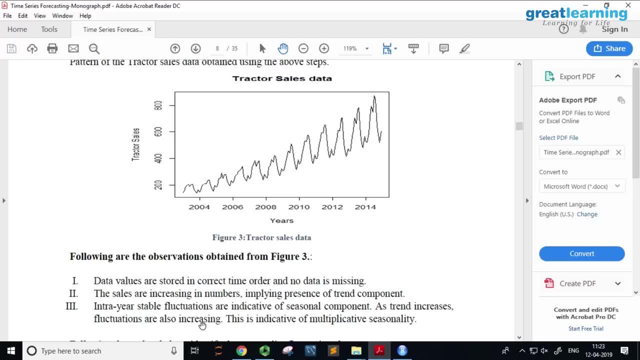 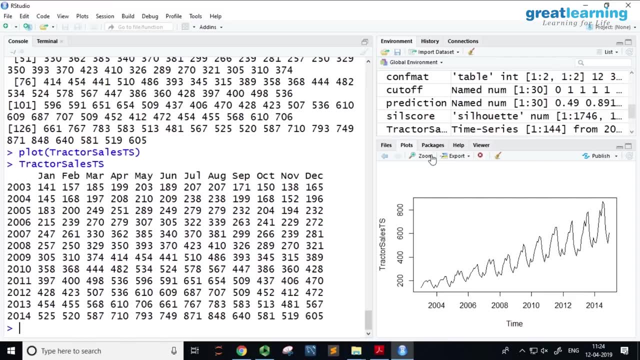 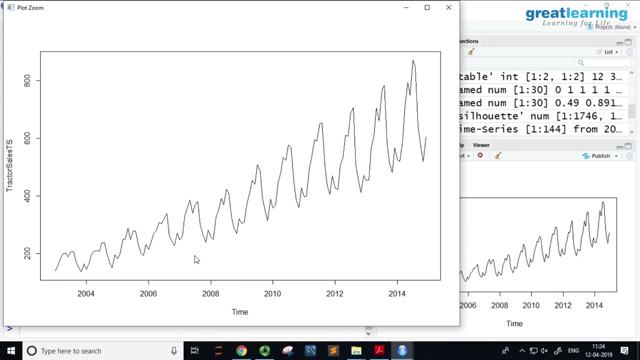 component. and then comes interesting point: as trend increases, fluctuations are also increasing. this is indicating a multiple of multiplicative seasonality. so if I do this, for example, let's say here, now look at the error here. so let's say that I look at sales around, oh, I don't know around, maybe, say 2006, now around in this. 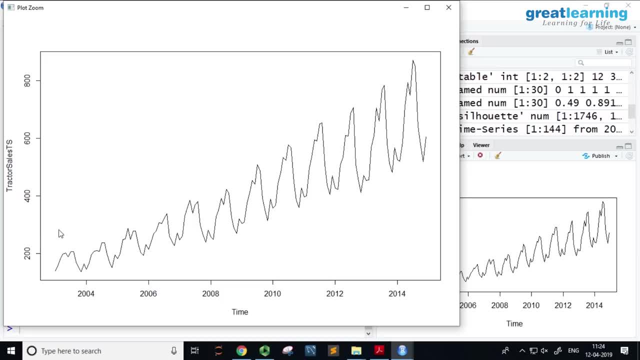 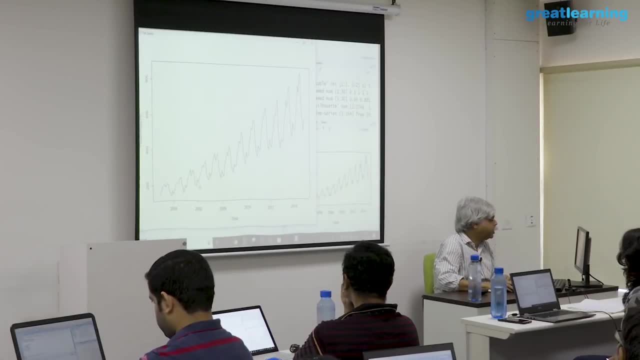 area. let's say 2006. what are sales like? sales are around 300 roughly plus minus what. in 2000 it's plus minus 300 plus minus what, about 300 plus minus 100, maybe some between 200 to 400. so in 2006 sales was about 300. monthly sales was about 300. 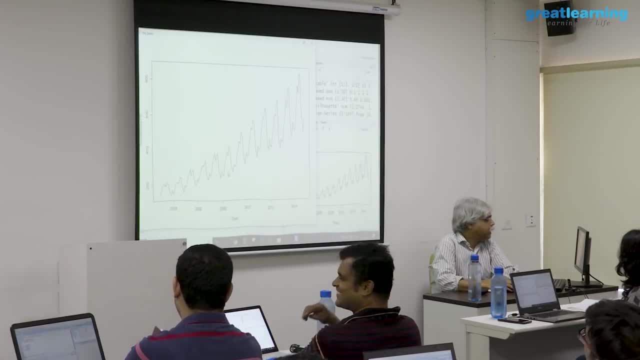 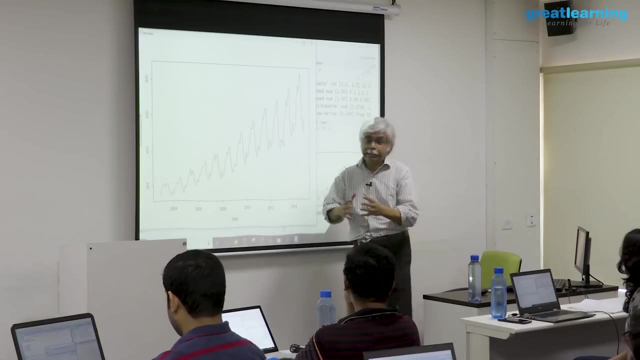 plus minus 100, roughly. now let's look at sales around, say, 2012. what was it around 2012? it was around 500 plus minus what? 150, 200, 150, 200, 150, 200. so the error is increasing as the sales of tractors increases. so now, if I want, 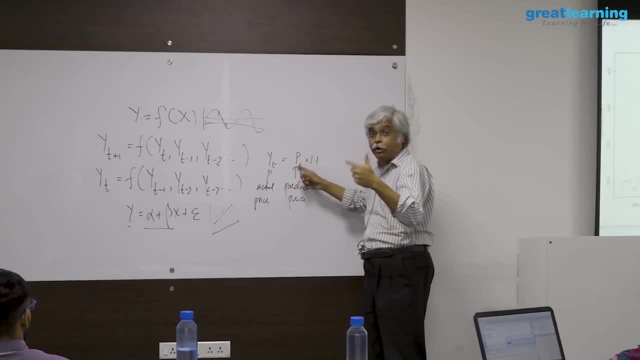 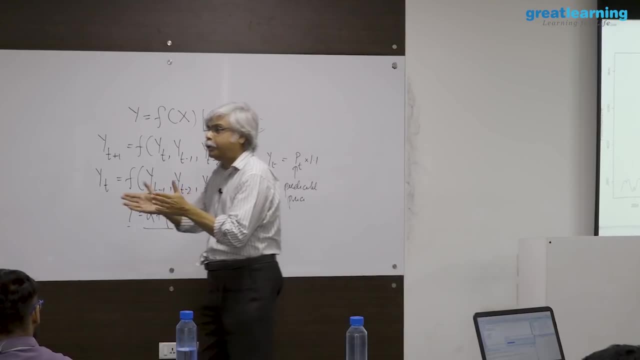 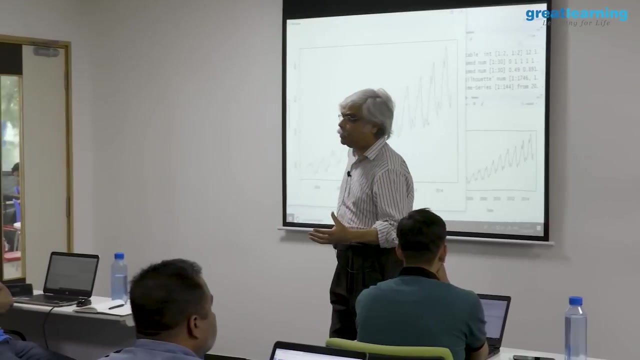 to write my actual sales as this predicted, or average sales. what should I do? I should multiply by a number, because this error is going to be plus minus. say, around 200 is going to be plus minus 100. around 600 is going to be of 300 is plus. 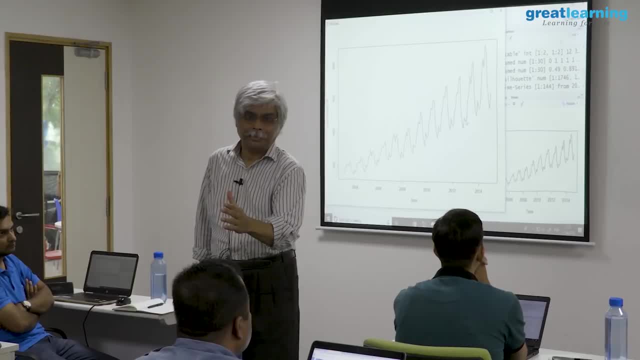 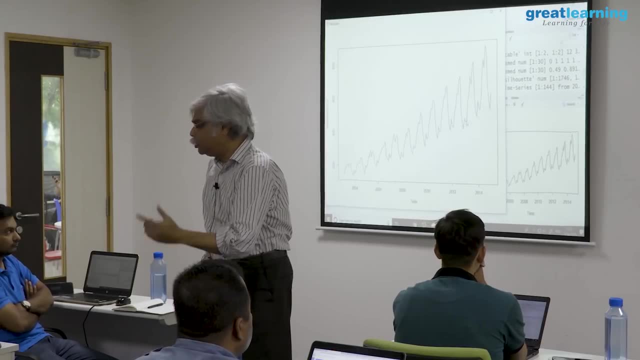 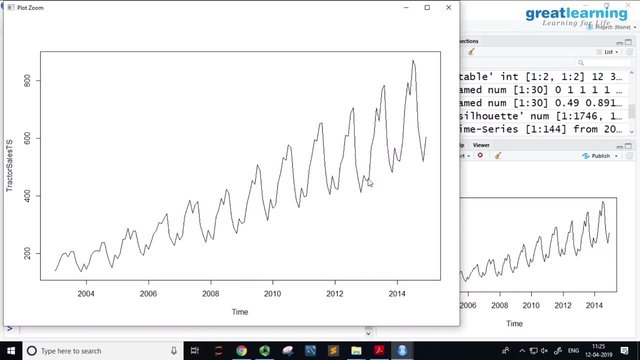 minus 100. around 600 is plus minus 200. so as the sales doubles, the seasonal movement also doubles. so the seasonal movement multiplies the trend. so which means that what you are looking at from this is the idea that the correction- the seasonal correction that we should employ should be a multiplicative factor. 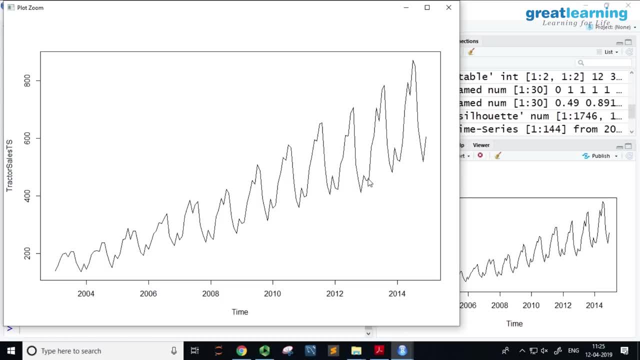 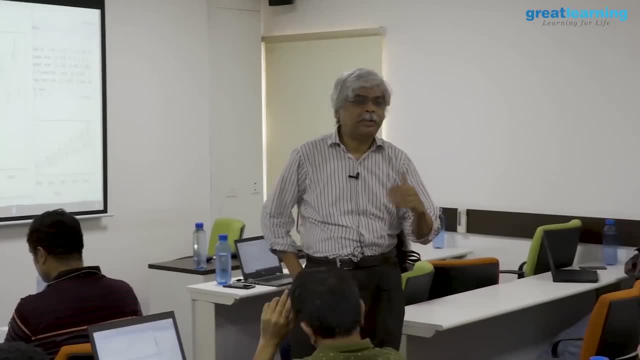 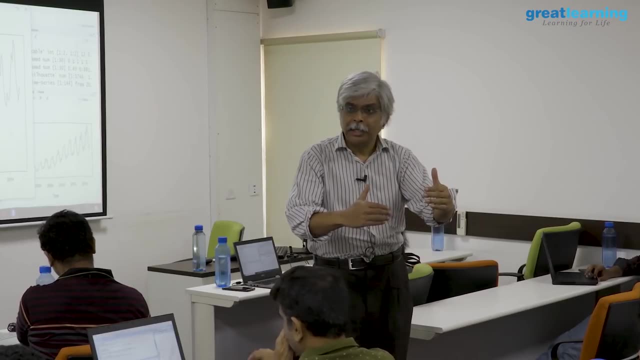 something like one point one, one point two, point eight, point nine, something like that, not an absolute number of the tractors. the number of the number of tractors I will sell more tractors I will sell in an offseason- sorry, in a in on season, is not something like a hundred tractors more, it is something. 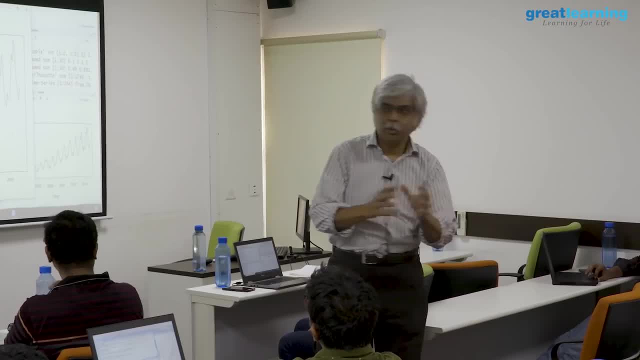 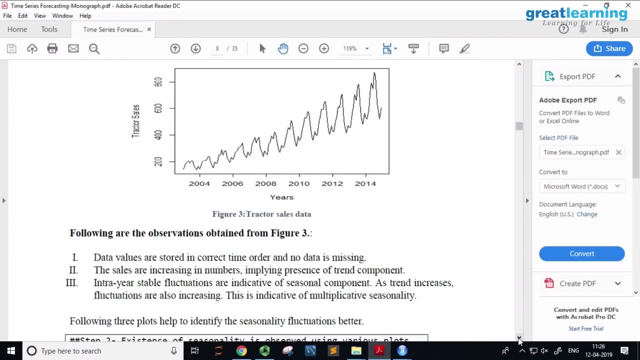 like 20% more, and as soon as you are in that situation, you're in the situation of saying that I am looking at multiplicative patterns. so, very roughly speaking, these are the patterns that we see. what we'll do after this is we're going to investigate this. 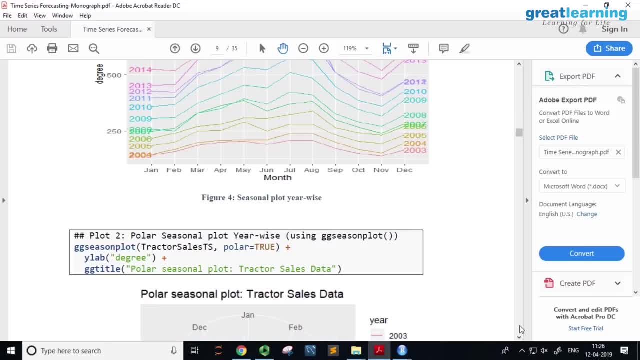 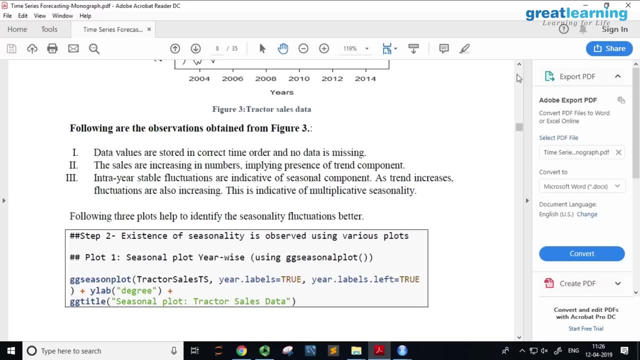 a little bit more and go into some descriptive graphics of this, eventually ending with a graphic that does this decomposition- a decomposition into trend, seasonality and an irregular component. as you'll see, the decomposition itself will be very easy to execute. it's more important to understand what it does than 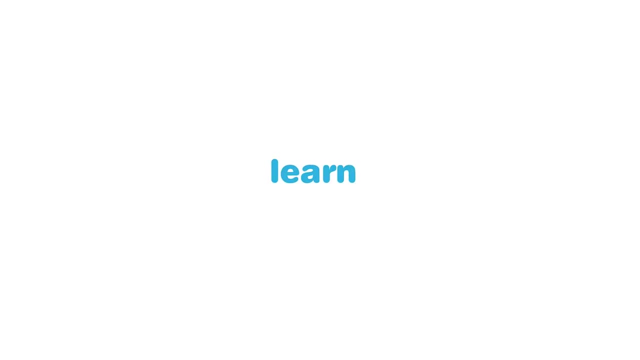 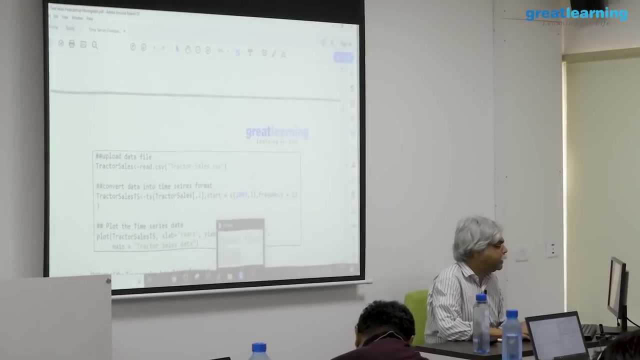 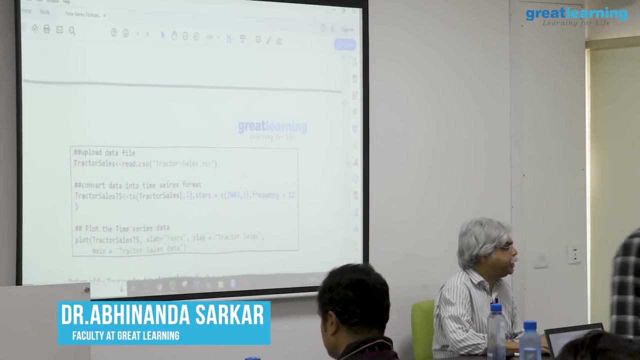 the actual algorithm behind it. so what we have done is we've kind of read. we figured out how to read a time series file. so once again, the series itself was a spreadsheet. so I said this was, it was here. this was the way the spreadsheet looked, why it was being read. 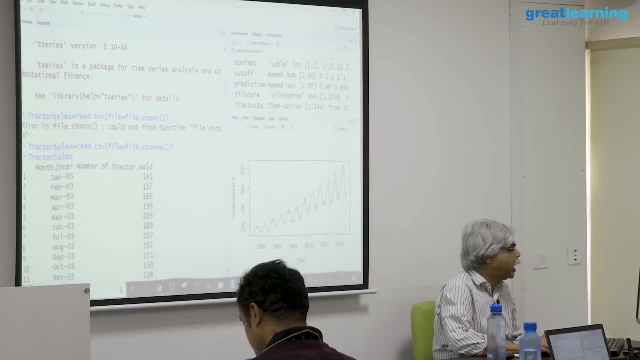 as you know, with going from Excel to R, introduces these dots. R doesn't like gaps, so it introduces dots where it is, but this in itself got me nowhere because I was unable to deal with this field. for those of you work in Python and other search data management software, you'll know that there are DDTM. 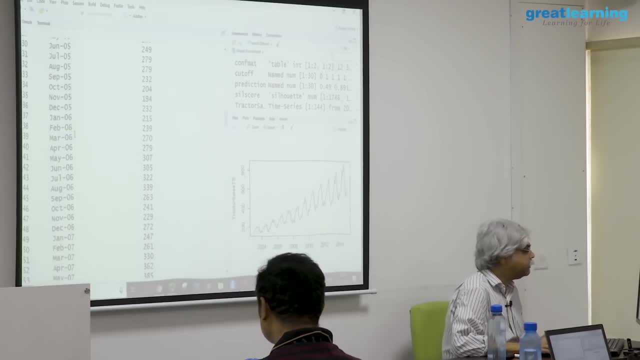 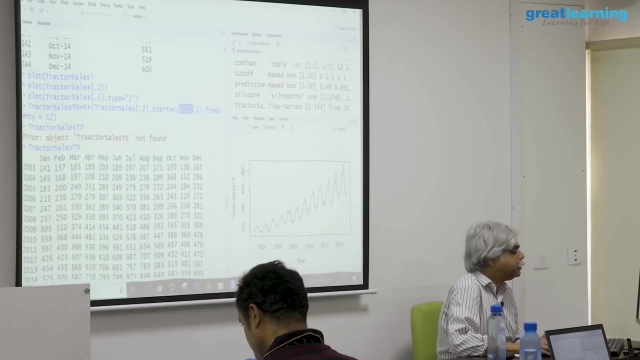 fields and things like that that can be taken of data fields of this type. R can also, and the way to do that would be to create a time series object. and the time series object simply reads in the set of numbers. it indicates a start, which is 2003, and a seasonality stamp, which is 1. it recognizes the frequency of 12 as monthly and 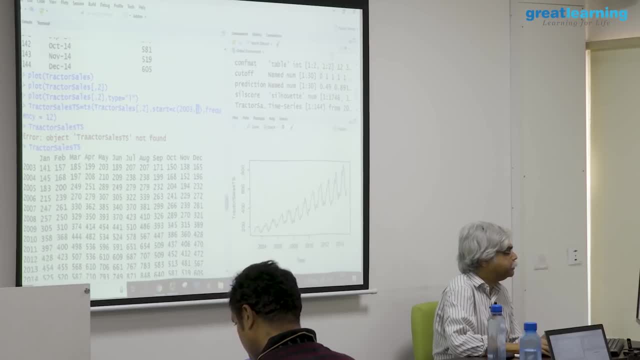 generates a time series object that looks like this: this frequency equal to 12, say again for the significance of one interesting. you can start this with two, if you want to, and see what happens. yes, begin with February. so if you, for example, begin with 2002, comma 2, then the first thing. 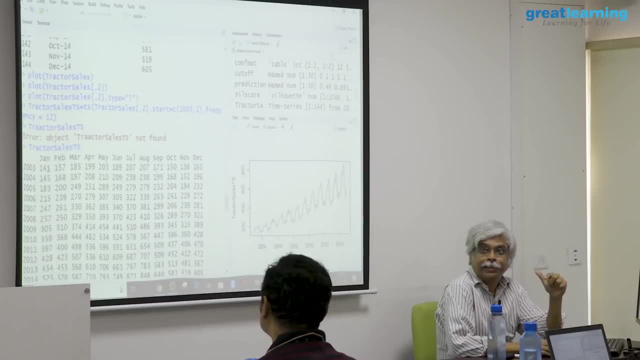 will be 2003 February. I did begin, it'll end in January. logically, what it should do is have the frequency equal to 12 should come before this. but R doesn't care at the R's sort of read hierarchy, will read frequency before it reads start. 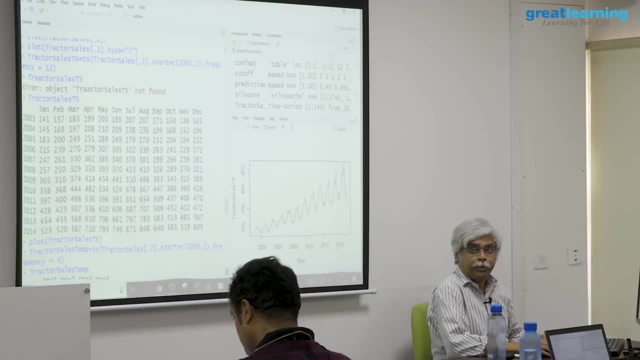 you can, we'll get to it. so if you want to forecast it, you're going to have to split it up into into bits, which is one of the things that we'll do when we, when we get to the test, training part of doing this, okay. so the basic visualisation associated with it, of course, is this visualization, which is simply the: 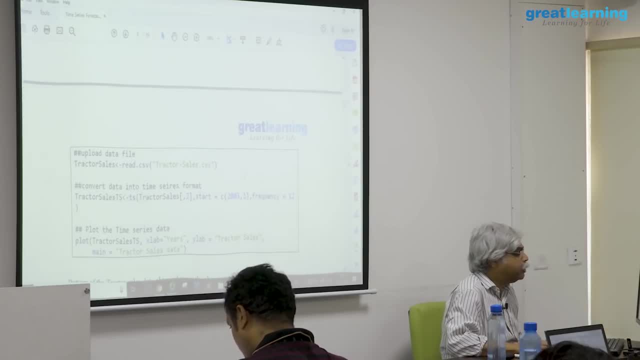 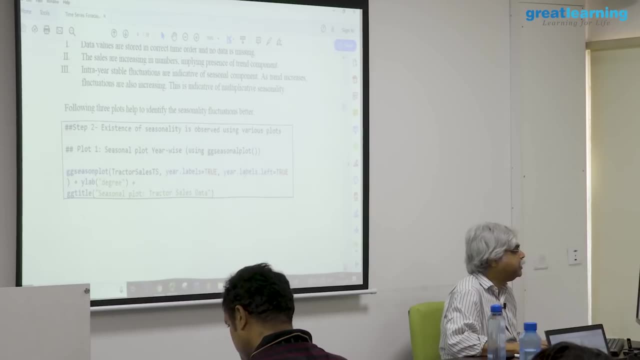 visualization of asset as a time series itself. you can do some other visualisations of it if you want so, for example, various kinds of plots, see can do seasonal plots. now, what I'm going to do here is do something that I would suggest you not do, but I am very fond of the very sophisticated technology. 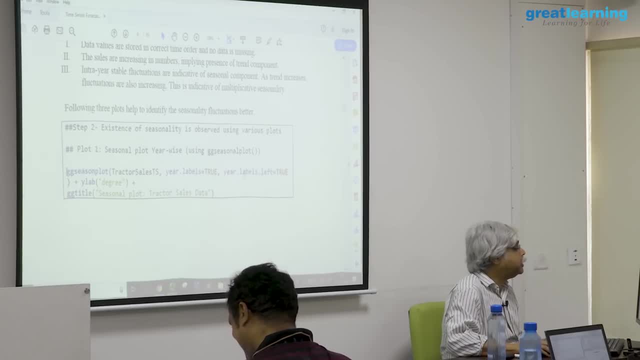 called control C, control V, control. control V, control V. I have discovered that when you tell if you have an ON command, you turn the control C control over to control v. when itㅋㅋ çıkarchs and control it opens, or it It's templates. terminal environment- Activation of an contraientrasu. 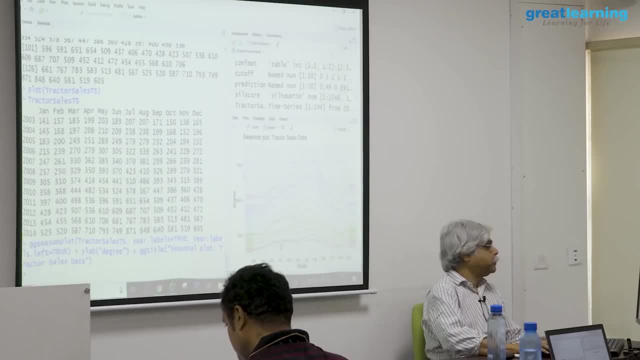 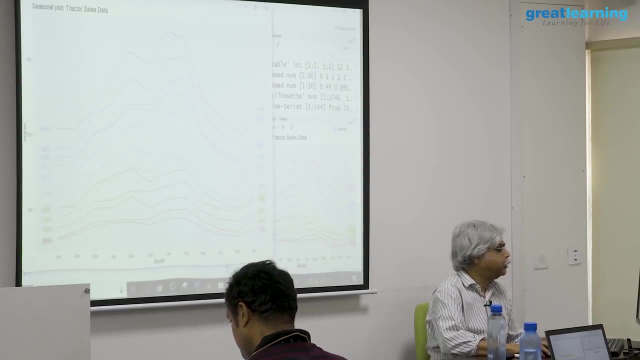 control C, control V, control or anomalies control, control v. and let's start with that function that we can is very important in life. so this is a season plot, what this is doing, and the code is there, of course, available and you can, you can use it at you as you at. 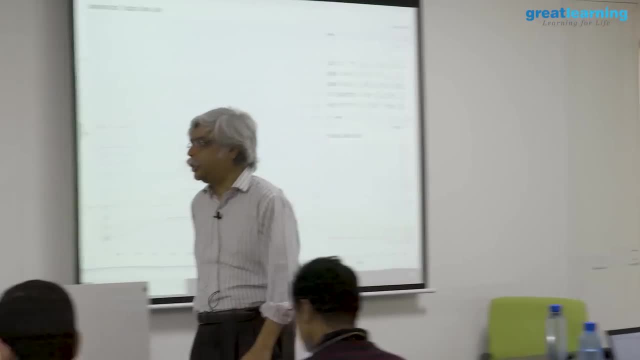 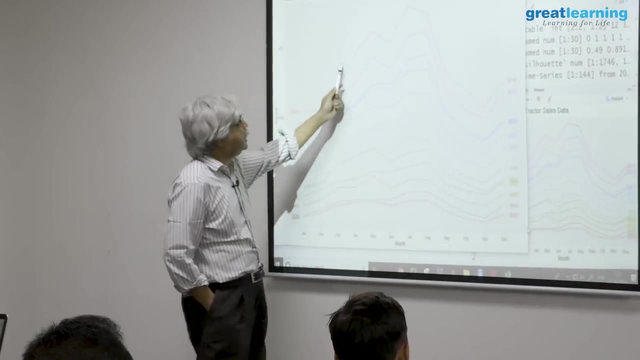 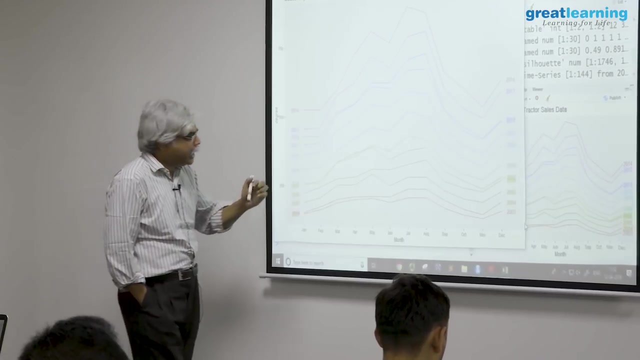 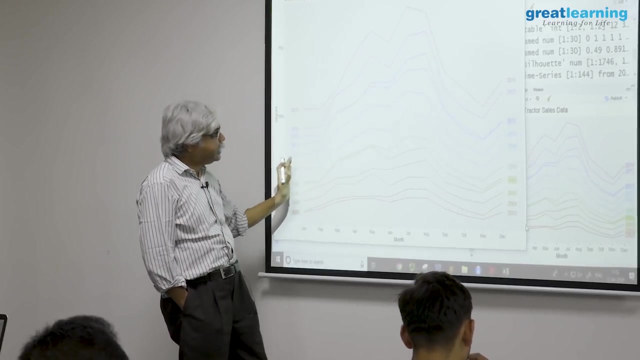 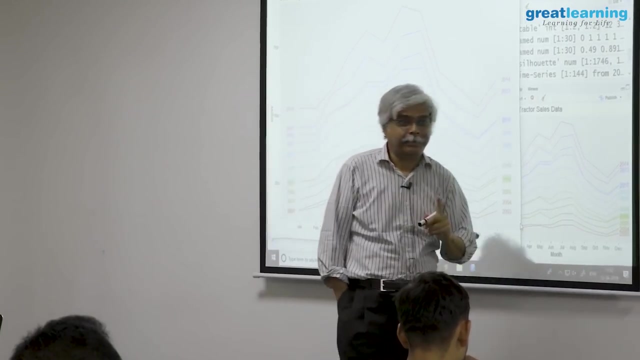 your leisure is. it's trying to go after a visualization that essentially splits apart the years, so each of the years gets its own curve. so two things are obvious from this number one: as the years go by, sales increases to. there is a common seasonality pattern, going from left to right, but it is not identical. it. 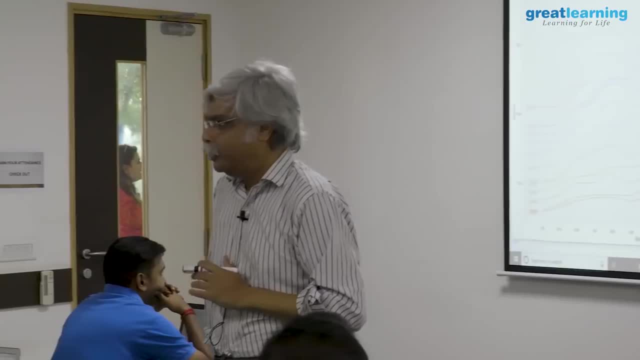 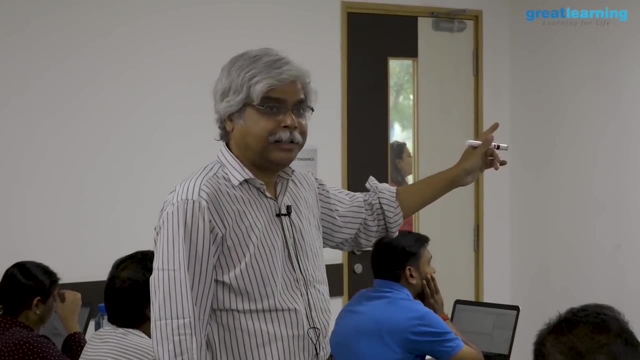 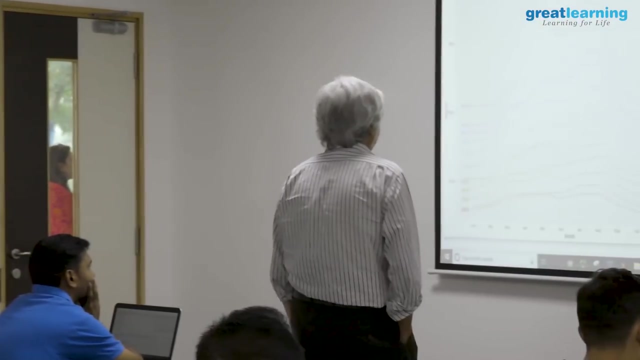 is similar but not identical, which means that there is a trend, there is a seasonality, but there's also something else that is peculiar to a given year and a given season. so, for example, something that shows up in a in a particular year but may or may not show up in any other year. so, for example, 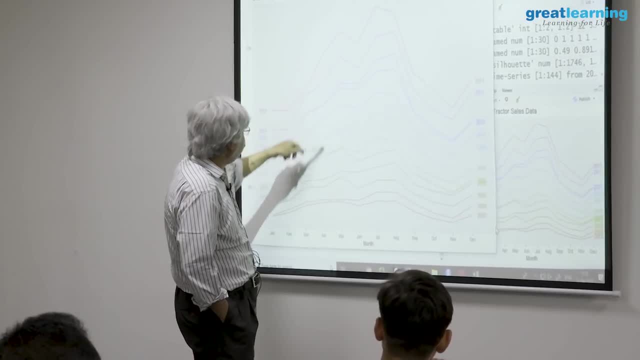 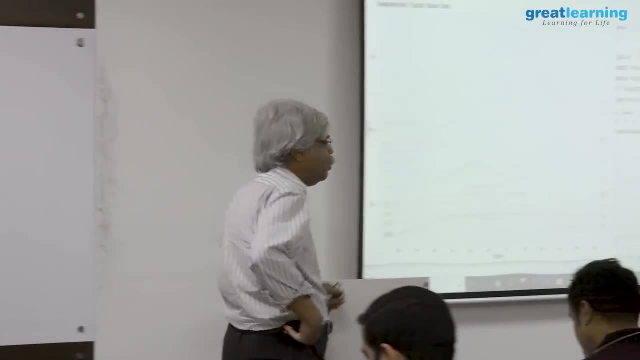 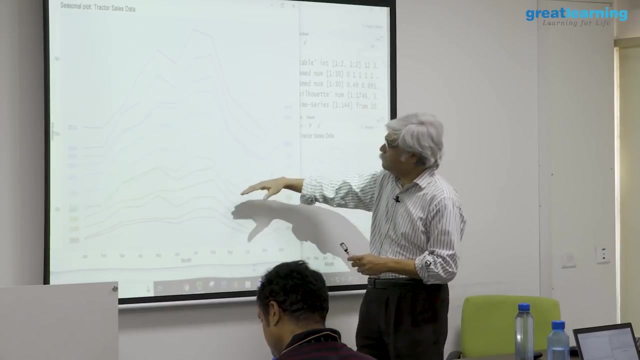 let's say, a little bump here, say in April of 2003, that may not be showing up in any other year. so this visualization gives you a sense of how, how strong in some way, the seasonal pattern is. also, as you can see, the bump gets more. 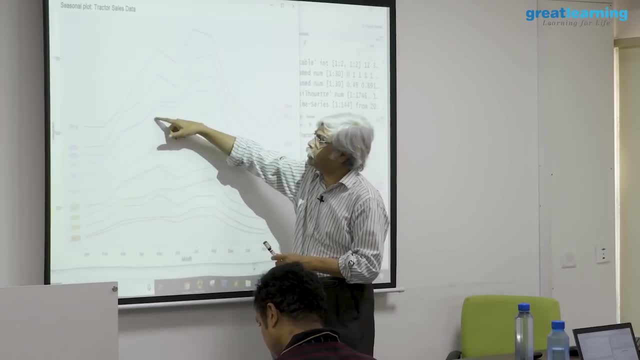 pronounced as the year goes by. so this visualization gives you a sense of how strong, in some way, the seasonal pattern is. also, as you can see, the bump gets more pronounced as the year goes by. so this visualization gives you a sense of how, how strong, in some way, the seasonal pattern is. also, as you can see, the bump gets more pronounced as the years go by. the reason is because in some way, we 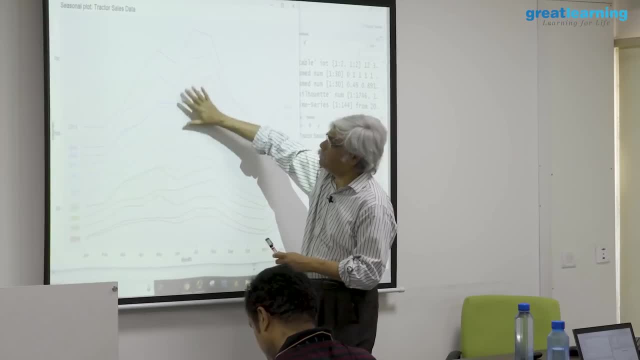 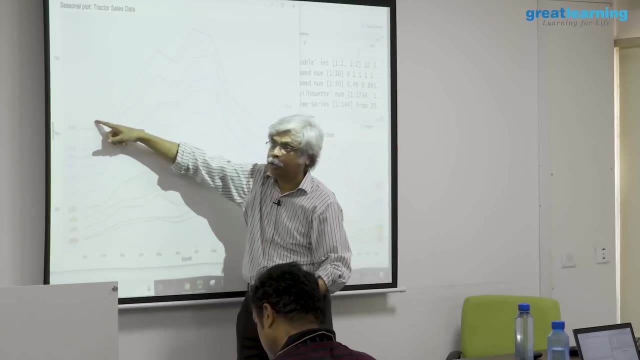 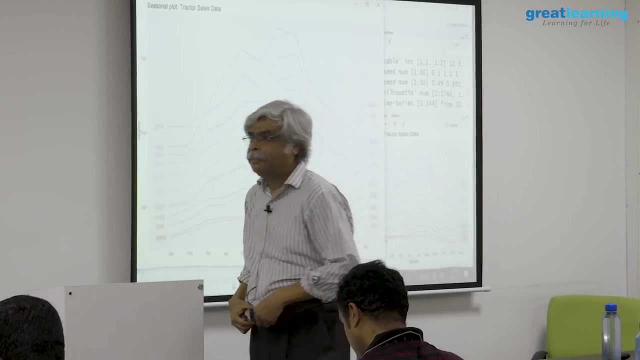 are assuming or not assumed yet, but the error, so to speak, is multiplicative, which means that the seasonal lifter trans of actual tractor sales is much more when the sales themselves are higher, so the bump increases. it's a little bit like saying that if you are making, say, fifty thousand a year, then a 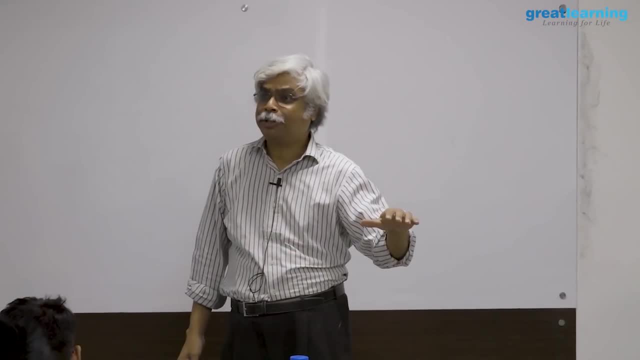 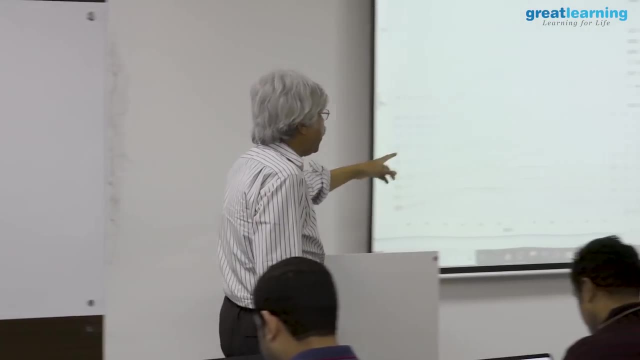 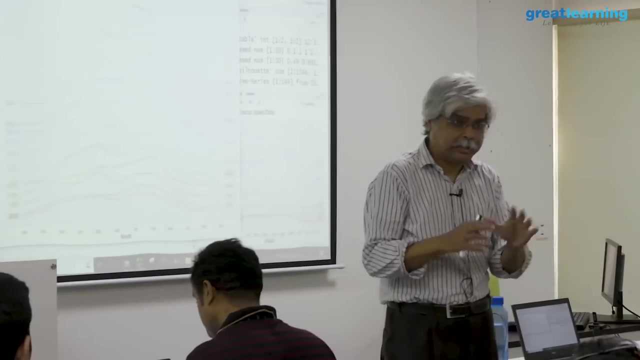 variation of ten percent is not as much, but if you're making fifty lakhs a year, then a variation of ten percent is a lot more, which is why the seasonal shape, so to speak, looks a lot more pronounced in later years. we will remove this by simply taking the seasonality as a 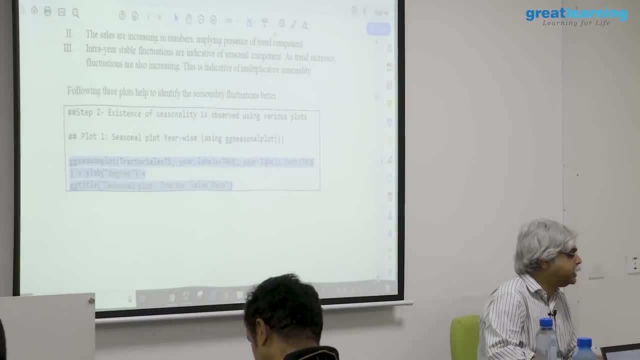 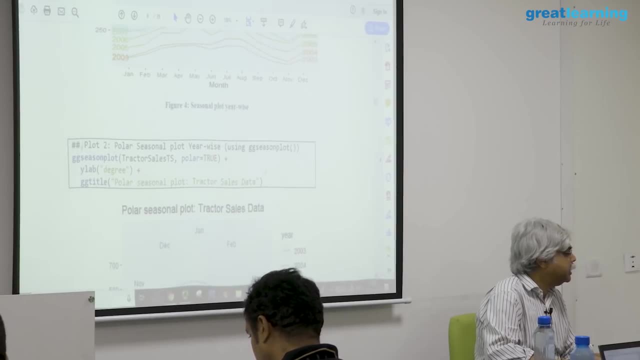 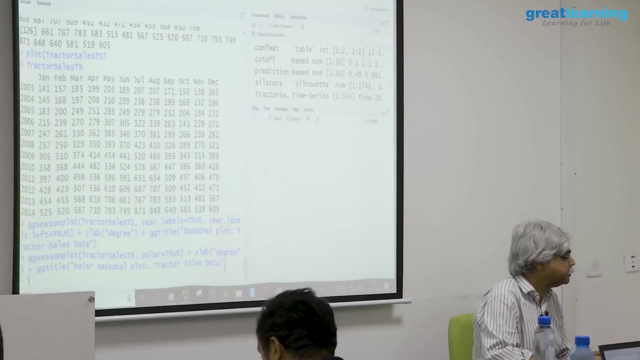 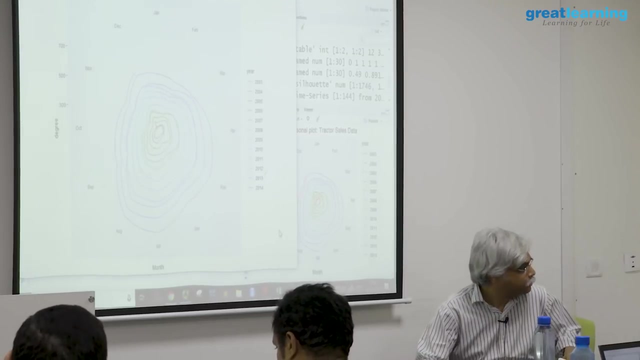 multiplicative. you can visualize the same thing in alternative ways as well. this is a year wise plot of it, using another representation called a polar representation. so what the polar representation will do is it will show this thing as circles. this is called a polar plot. the reason is because it looks like the lines of 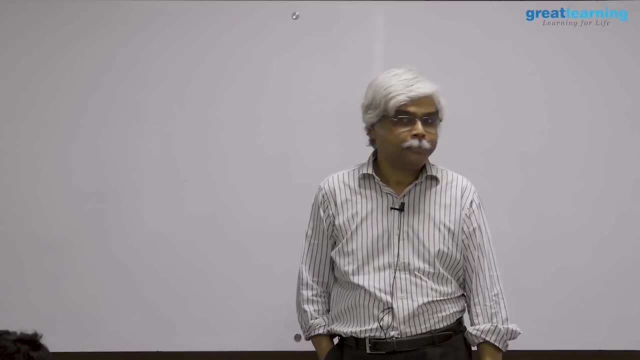 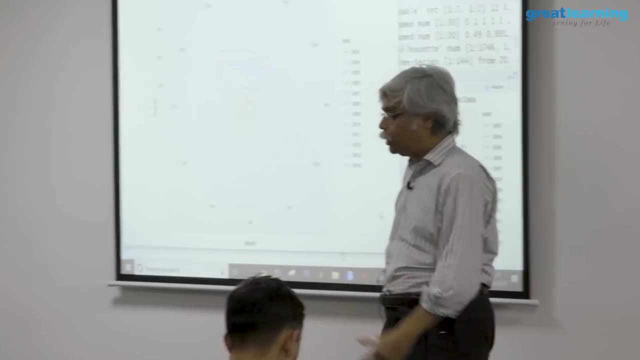 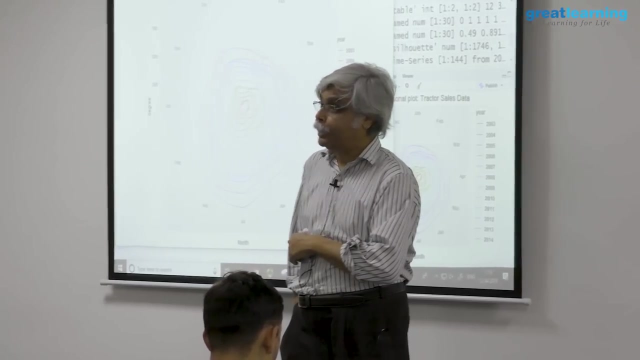 latitude seen from, say, the North Pole. so there's a, there's a, there's a joke, right? so there's a bear who walks a mile to the south, then a mile east, then one mile north, and it ends up in exactly the same place where it began. so it moves south, then east, then north and ends up where it. 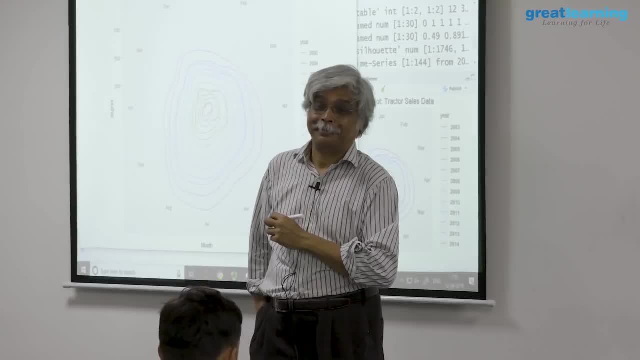 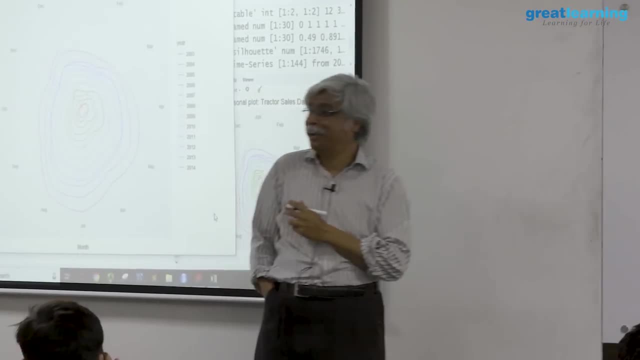 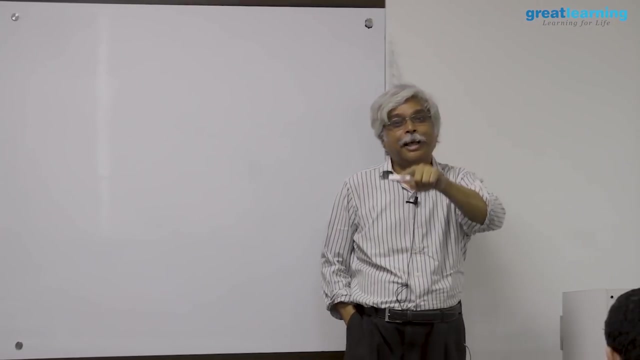 is: what is the color of the bear? same color as what? so good answer. so good answer, so good answer. but so the point is that if you are, if you are going south and east and north, you're covering three sides of a square, so a typical bear will not be able to get. 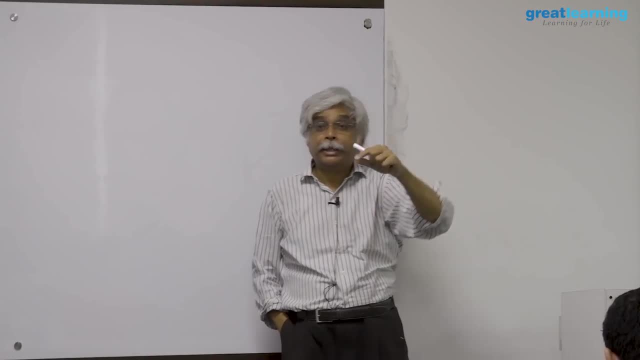 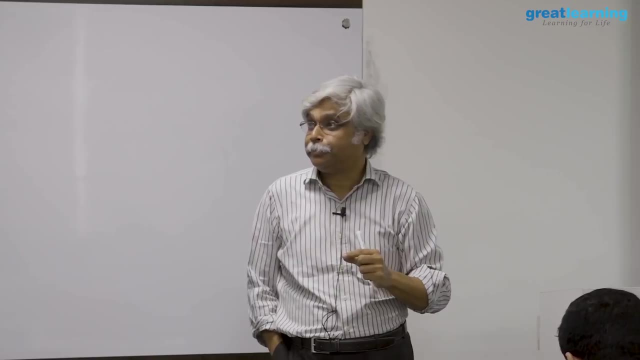 back to the same place. you should try to cover four sides of a square, but there's only one situation where this is true, at the North Pole. so the answer: this is a polar bear, the color is white. you can get another bear there, I suppose. so the 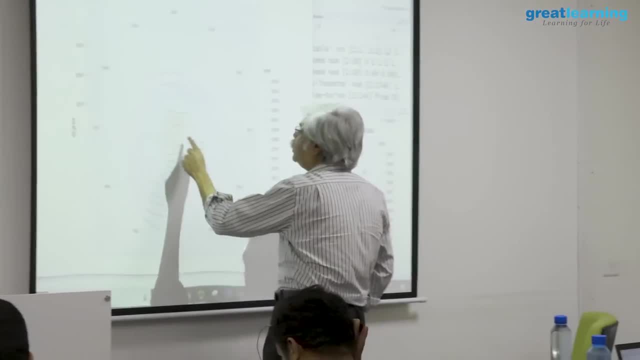 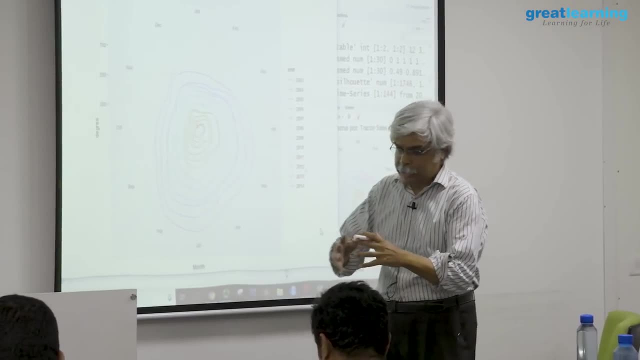 idea of a polar plot is to be able to show small deviations as things like this: small deviations as things that are near the North Pole and these larger deviations go out. so this uses the idea of a radius in order to show what the seasonality is. so use plots such as these carefully, but there are some. 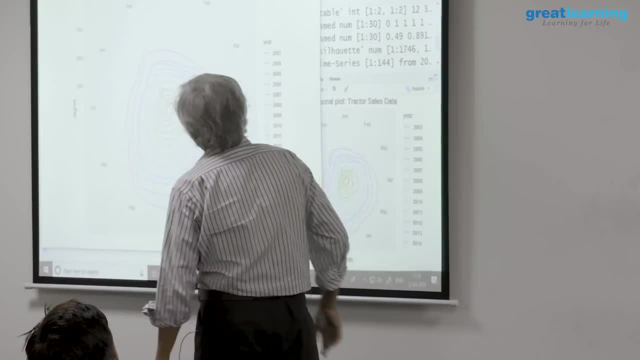 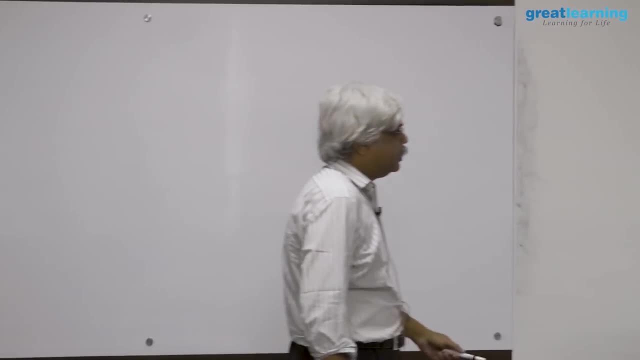 situations where this gives interesting patterns- and this is one such- is exactly the same thing that you saw before. what are the radials? the radials are the months, so if you're going along a certain direction, let's say you're going right. you're seeing the progression in a 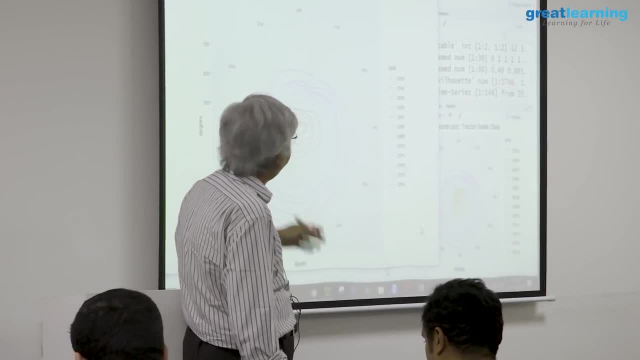 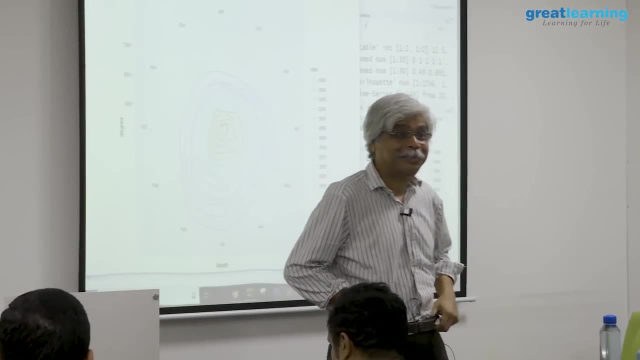 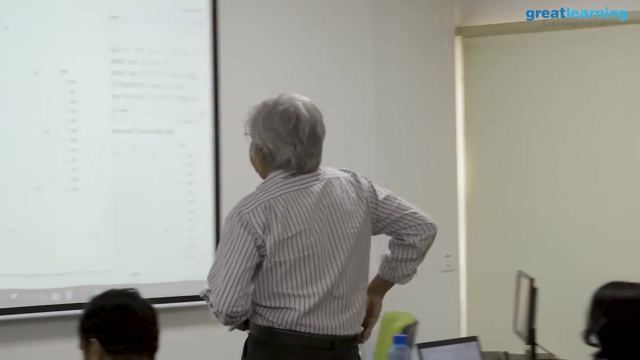 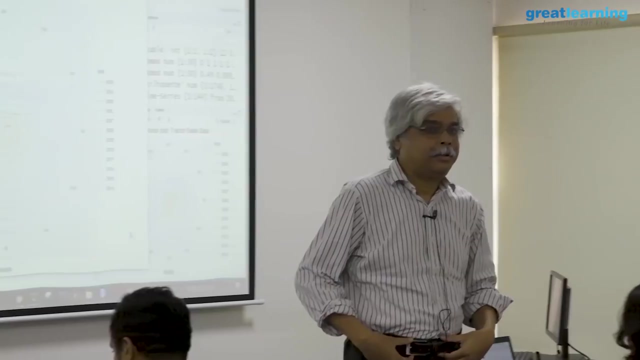 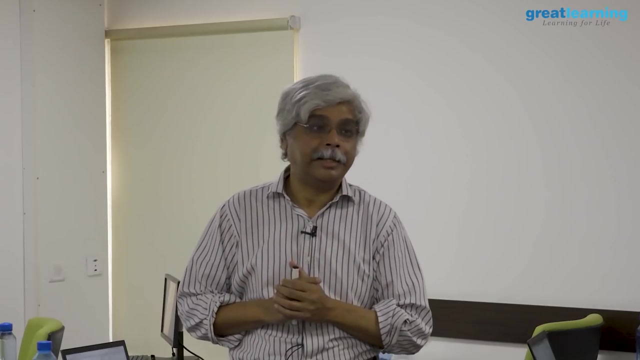 period. if you're going north or if you're going upwards, you are seeing the progression in January that the previous plot tells us. so what would happen if these things look circular? no, yes, if it is circular. what does that mean? if it is circular, that it means there is no seasonality. so the idea of seasonality translates into circularity. 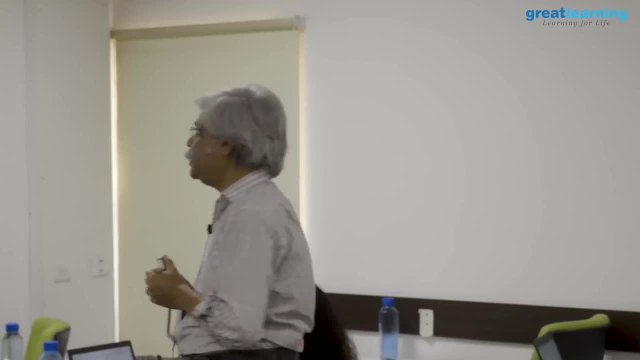 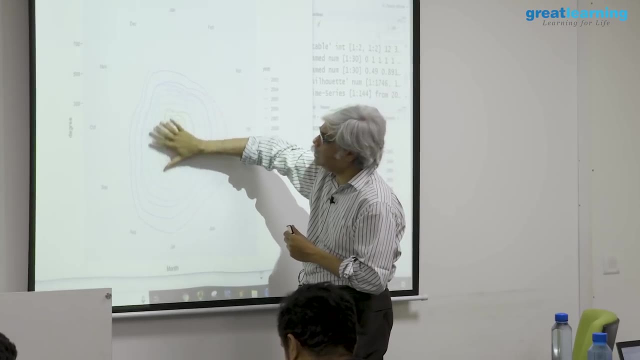 so to speak, roughly speaking. so if you are thing, if you are seeing things are not circular, is just a question of seeing how the eye moves. the other is if you are seeing things that are circular but are shifted, in other words, the center is, so to speak, in the wrong place. 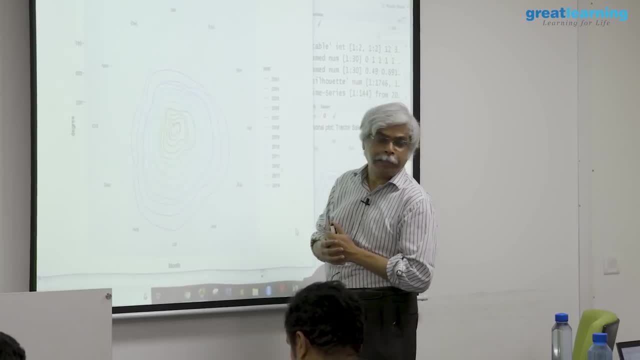 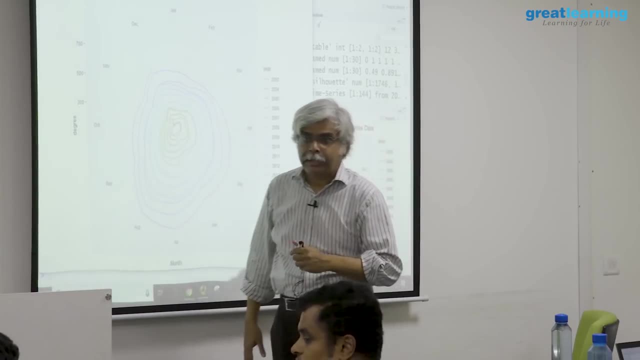 the hill is not in the middle. climbing Everest does not look the same from India as it does from Nepal, things like that. so the hill is not symmetric. what does that mean? that means that there is a seasonality pattern, but that seasonality pattern is sort of the same across. 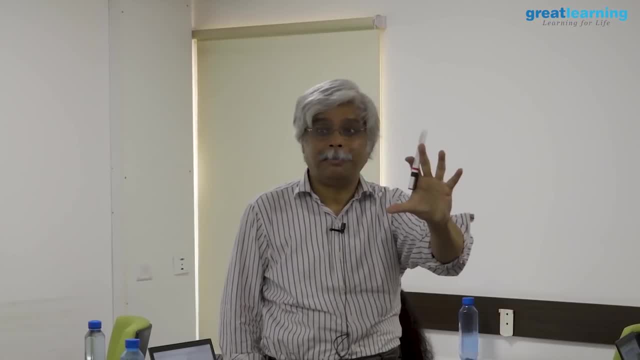 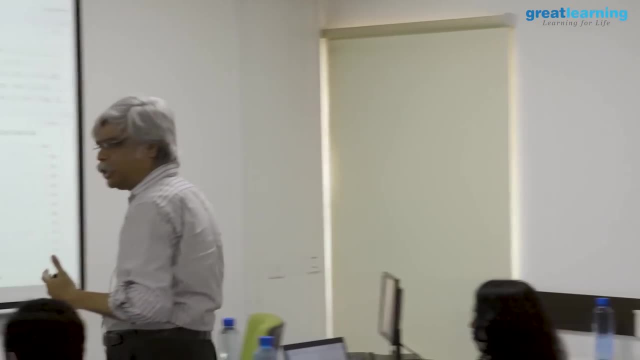 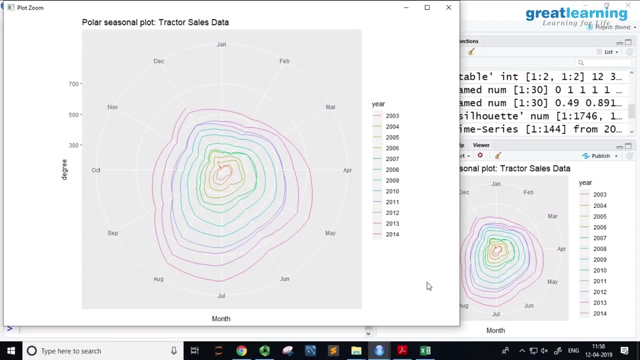 the years the circles shift in the same way for all the years. visualize it. have you done a visualization session tableau and things like that? is it in the schedule? I don't even I don't not yet done so ask your visualization professor. so visualization is an odd thing. it's a question of you. know what the human 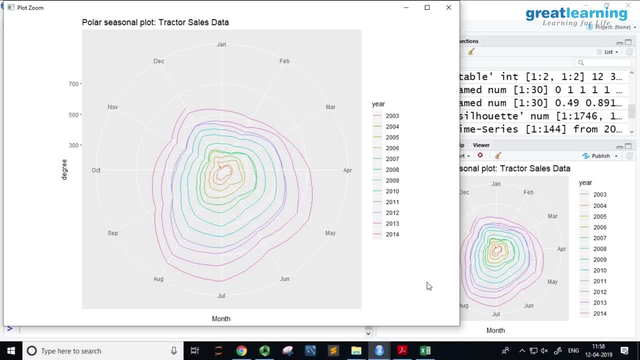 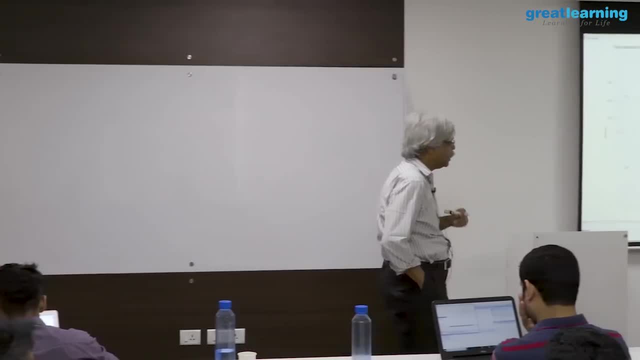 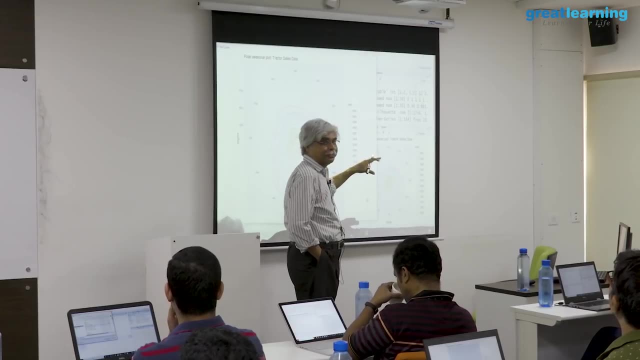 eye is supposed to is good at at seeing differences, for so these are. these are ways in which seasonality is often are often represented. they are purely as a part of descriptive analytics. you will not do this to forecast. a simple bar chart would also work. we'll see a simple part chart. 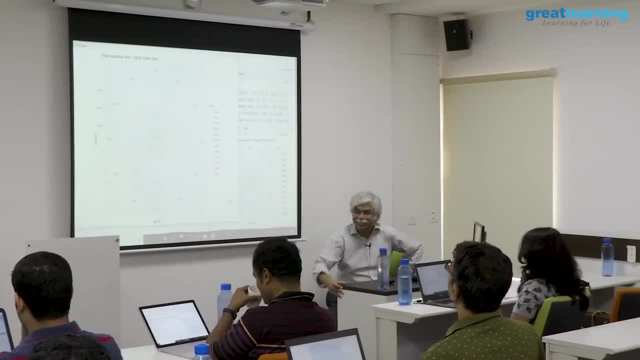 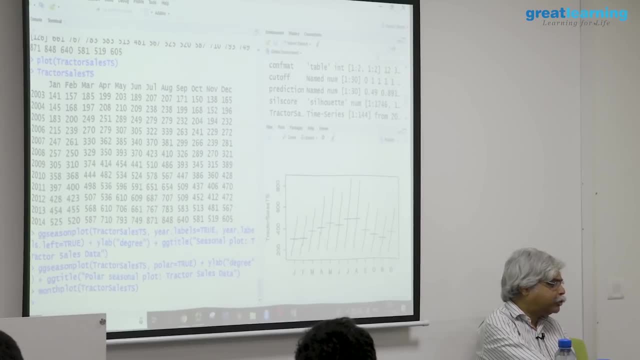 or the equivalent of a simple part chart. so two subpar things. so that is that is the idea. okay for your liking, I agree with you. I agree with you. this is the function that acts on a time series. in order for this to work, it must recognize the notion of a 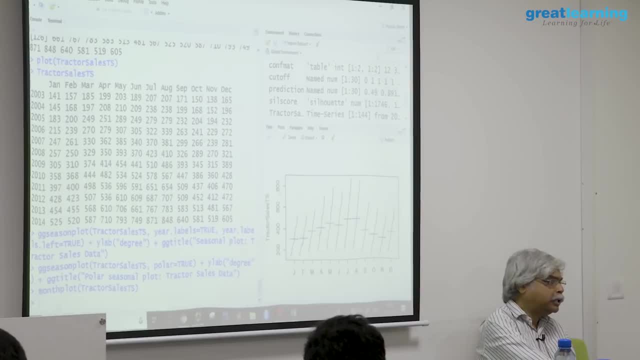 month. it doesn't need to have a month. it will do the same thing for quarters. it's called a month plot, but if you give it quarters it will plot it as quarter one, quarter, two, quarter, three, quarter, four, like we had done. so it doesn't necessarily need months, but it makes the most sense if it has months, of course. 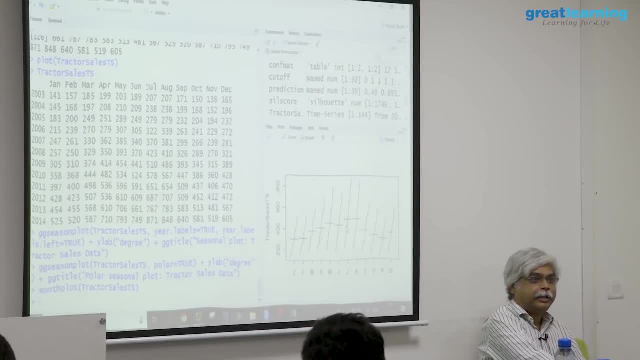 here, the years are not there. it will average over the years. it will average over the years. so, therefore, what is it doing here? so, over this gap, over this gap, it is doing the entire January season of all the years, again, over this gap, is doing the entire thing. what, where is this? where is this? what horizontal? 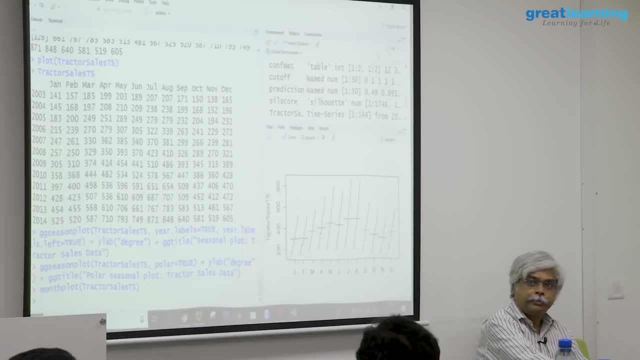 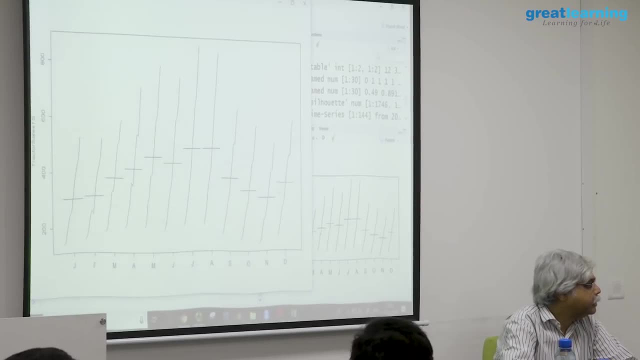 line. this horizontal line is at the average, yes, yet this line is at a certain level. this line is at a certain level. so if I want to find out the average of July, the average of July is extrapolating back along this line. the size of this line tells me how way this July data is this. 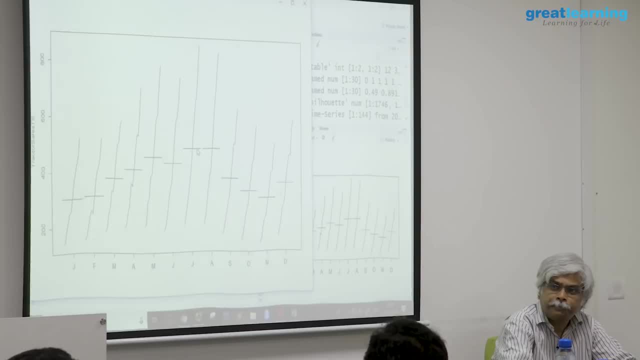 is at its earliest point. this, at its latest point, is more or less the same. yes, is more or less the same, and it is the highest in August and July, and it is the highest in July, but I've lost all sense of annual trend. it's as if I'm only interested in forecasting umbrellas based. 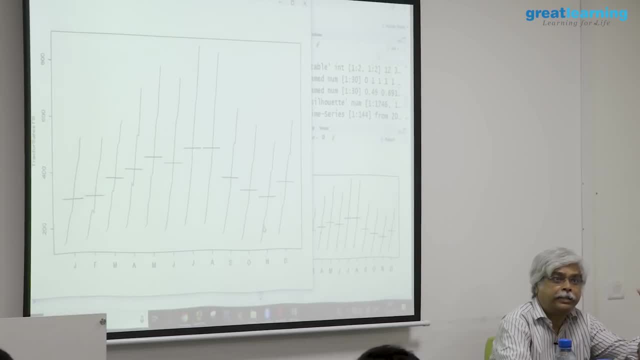 on what happens in May, don't care about last year's April and the April before don't care about April. so therefore, this is, this is another plot which is in some ways equivalent of a bar plot, so to speak, to say that what is the, what are the numbers stacked like? another interesting thing is, as I 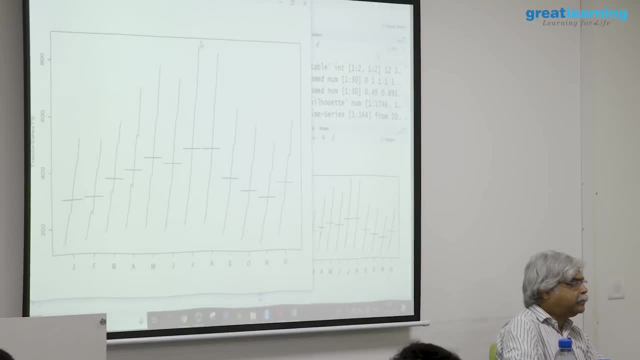 said, the, the annual variation is here, but this variation is a dangerous variation to see because this variation is effectively capturing a trend. as we have seen, that trend is not necessarily the same every year. so for example, in here you are seeing a little bit of a blip here about one-third into the year. 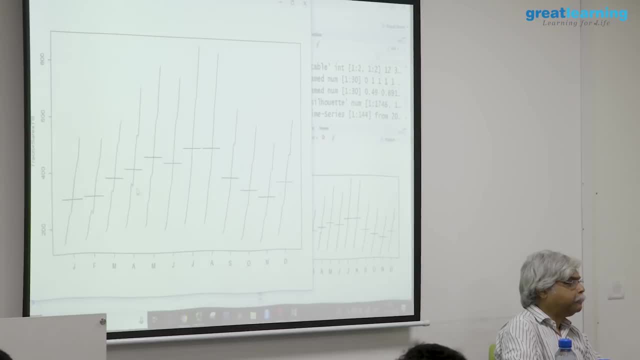 but that blip is not visible in other years, which means in April of maybe 2006 or something. something odd happened thisカット, so we need to investigate that a little bit more. not investigate? or at least you visualise that. YES, I see. so you are saying that let's pretend that I do this plot only for a 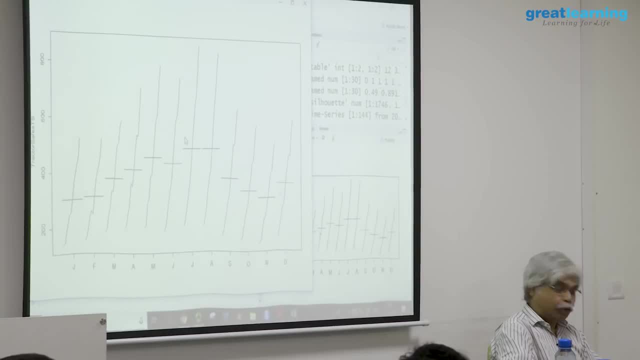 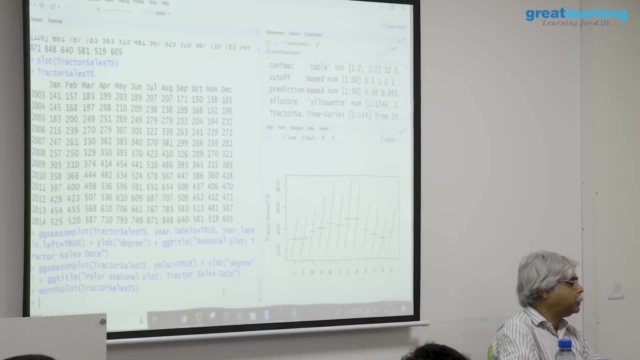 small period of time, true, true, true, true in others. so that's an interesting thing to try. how do we? how huh, block of block of へえ, certain parts of it. so we, I can do a start, stop on this. or I can probably do few rows I can take. let's say: 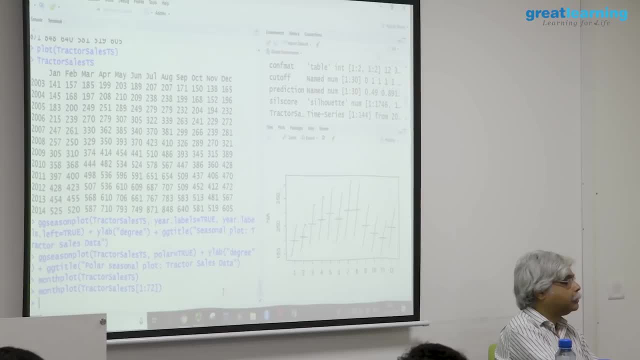 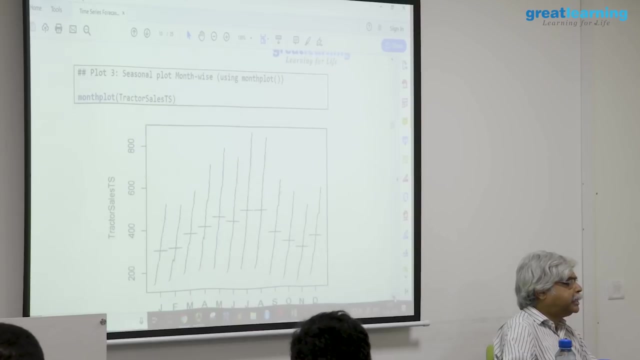 this is for the first half of the data, this for the first six years, and so, of course, if you want to follow through with him now, this is not there in your notes. but what would I do? I do something like this, okay. so this is. these are, in some way, visualizations. they show that the sales of tractors increasing year on year. 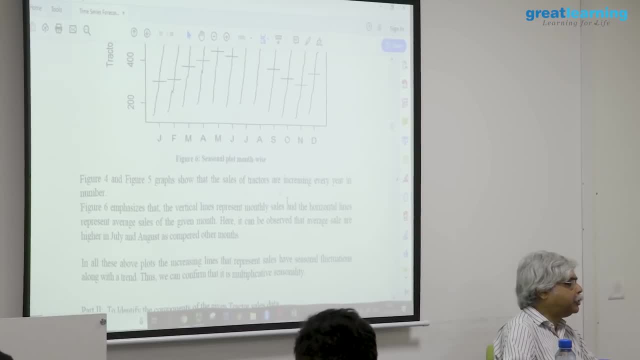 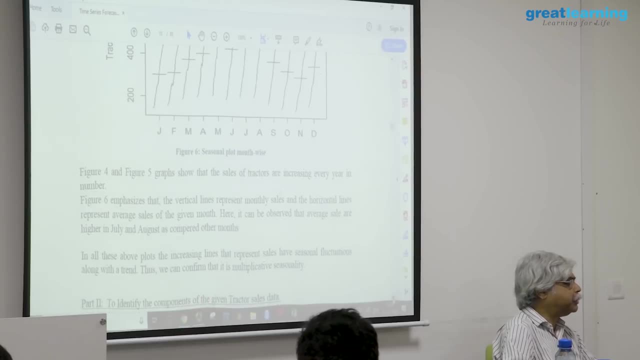 the vertical lines on this plot represent the monthly sales. horizontal lines represent average sales in a given month. the average sales is higher in August and July as compared to the other months, etc. when you do little spell checks on this, yes, it may not extremely be increasing. so, for example, here, as you see, there's one particular situation where in August, in April, 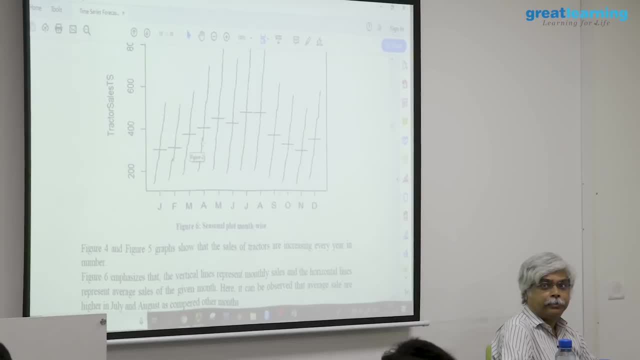 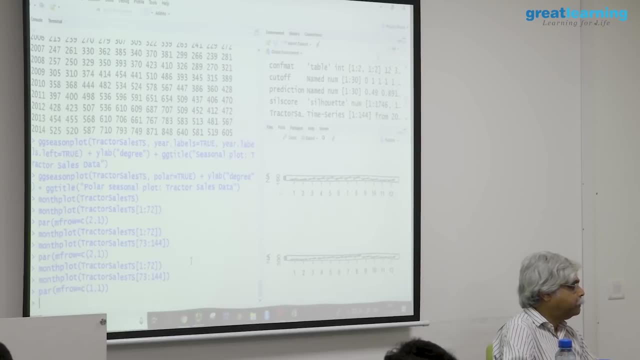 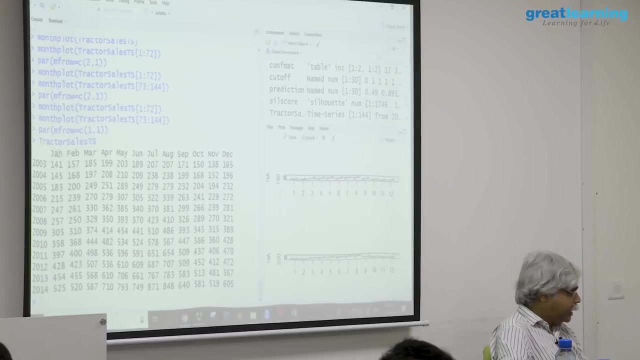 it did not increase. so it looks at all of all April's and then all means after it. essentially what it does is: it looks at this guy, it looks at this thing here and it looks at it column wise, ha ha, plotting in this way. so the plot, so the so the plot is on the column, so to speak, and 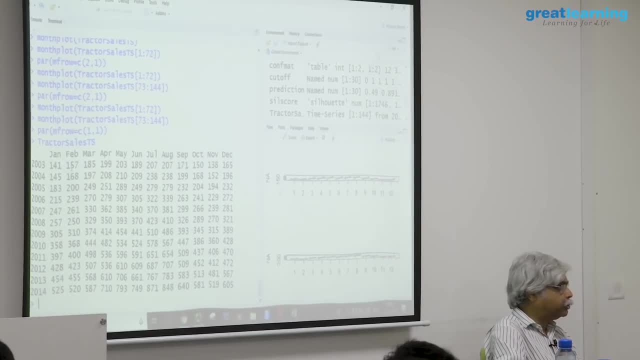 then within each column it now plots this as a little time series all on its own, a January time series, every time series, an April time series, etc. that dip is here 362 to 350 and then, though it is increasing, it came down. so here on year, this sales, 2008 April, was actually lower than 2007 April. seasonality trend is not suggesting that, because the same trend should. 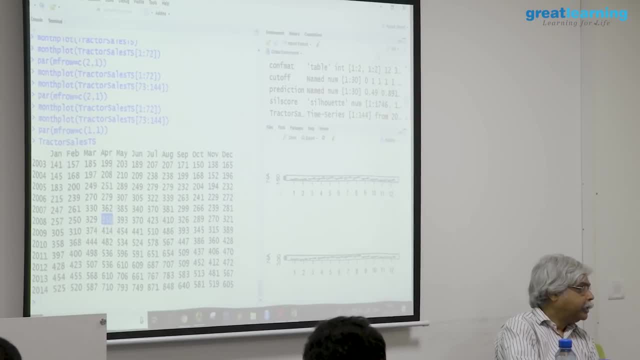 apply for every year and, oh, across it is increasing. everywhere else it is increasing. this is 79, 62,, 14,, 14,, 18 and across all other years it's increasing: 7-3,, 85,, 39, etc. every other year is increased and 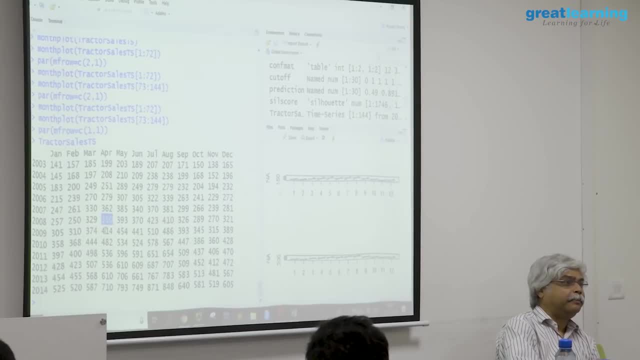 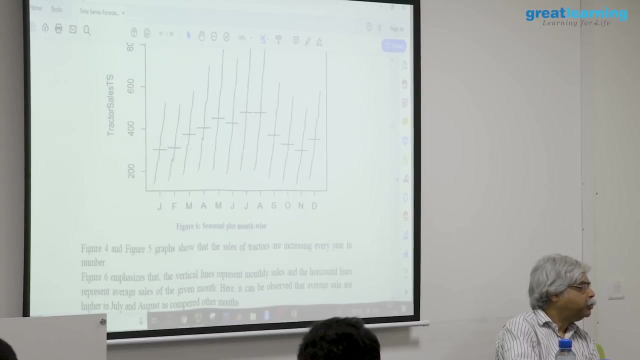 every other month is increased except April. so one would suspect that there is a, there is a low irregular component here. for the others, maybe the plot didn't see it. it was, it was to, the plot was maybe to February has that as well. so something went wrong in this period of time for that year, for that year. 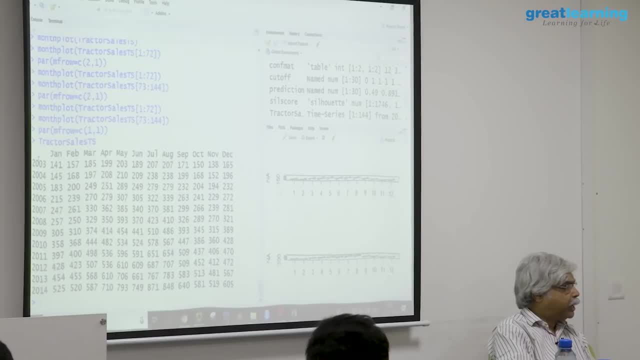 remember what we are trying to do with. the trend is trying to find what is essentially a effect across the columns, I'm sorry, across the rows. seasonality is trying to find an effect that's across the columns and there is stuff that is not explained by the row and is not explained by the column. that will be the 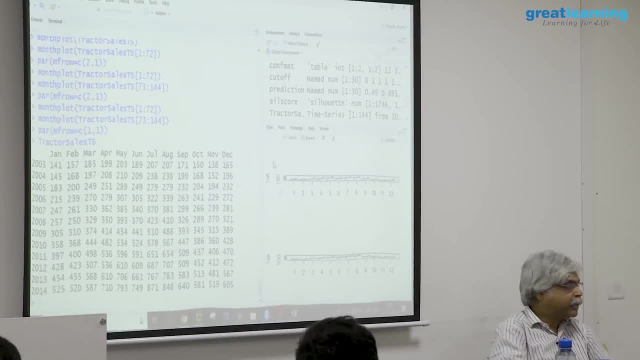 path that is unpredictable, because if something strange happened in 2008, for only a few years, the question is: should we be using that in order to predict, say, 2014, 15 or 16 or onwards? or if I want to predict, say beyond this, should I simply be looking at the average of all these? 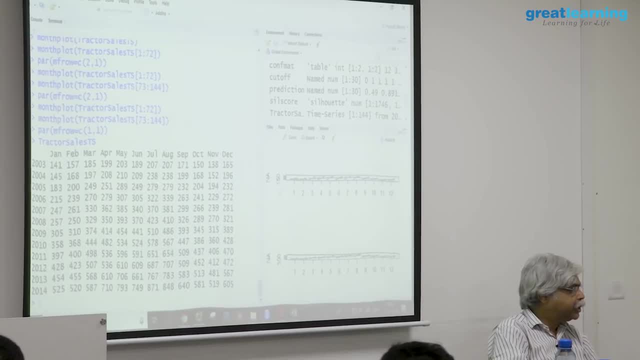 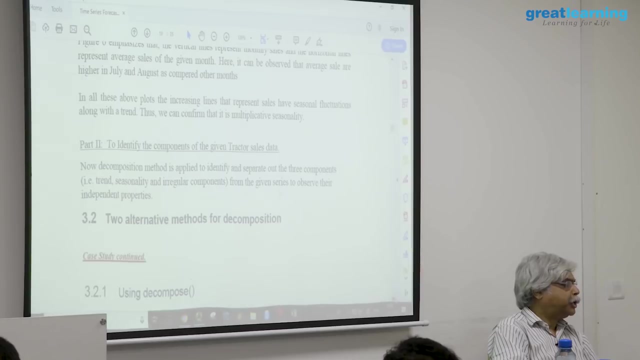 years and predict trend words and then apply a seasonal correction that applies to every month, irrespective of the year, which is what we will do. just hold on, we'll do that. now the decomposition aspect of this. let me do the decomposition after I've done the decomposition, you 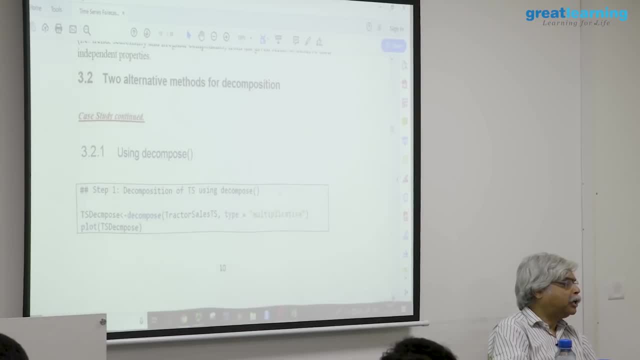 see what it does now. the syntax for decompose is startlingly simple, so simple that you have no idea what is going on. you don't, I don't, none of us do? all it says is that you decompose, decompose what? where? how you know we. 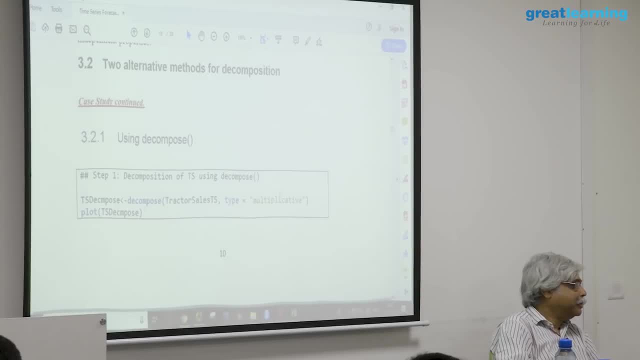 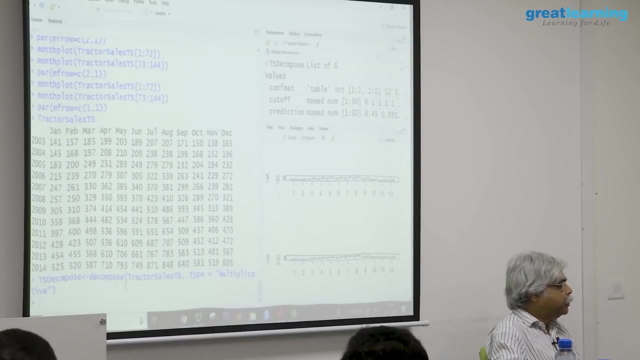 don't know, we'll see what it does sometimes, as it will do smart for its own good. so fosters decompose this. another version, so the spelling is a real off, but the function is decomposed. the spelling of that is okay. now what did we do? all we did is we took the time series object, we decomposed it. 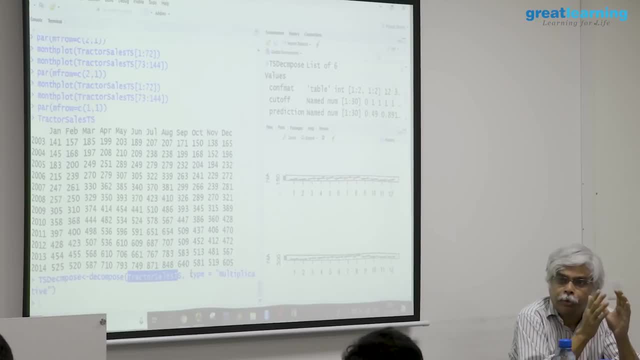 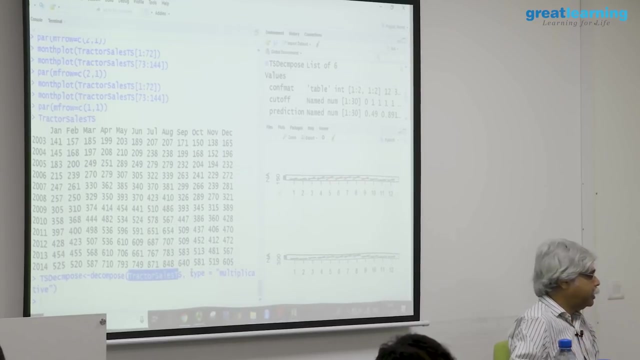 and we say type equal to multiplicative. why did we say type equal to multiplicative? because what we're trying to do is we're going to say that the multiplicative, the seasonal correction, is going to be a multiplicative factor, is not going to be an actual sales is going to be a multiplicative term. now, 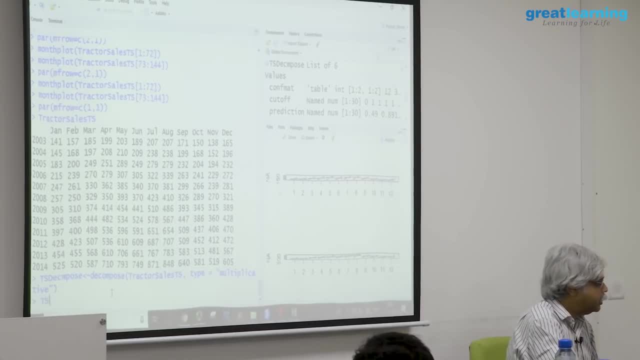 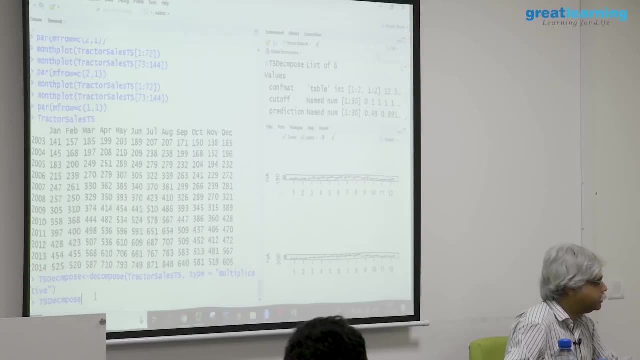 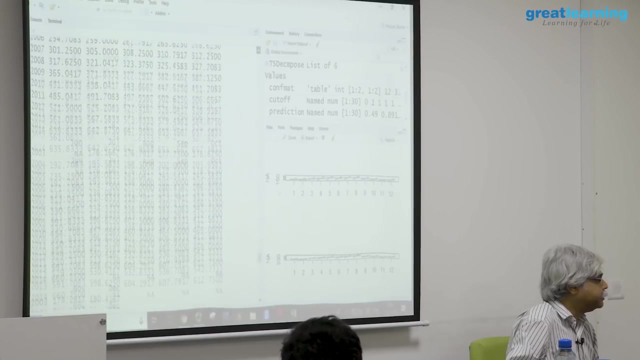 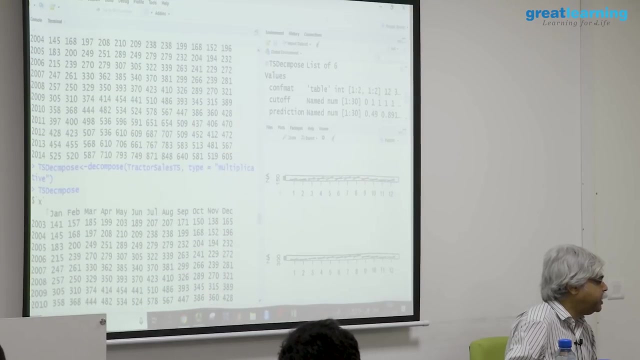 before we plot this, we can see what it is. so in other words, if I now look at what T has decomposed is, this is what T has decomposed is as an object. as an object it does certain things, plotting it is going to be easier. so the first thing that T has decomposed gives 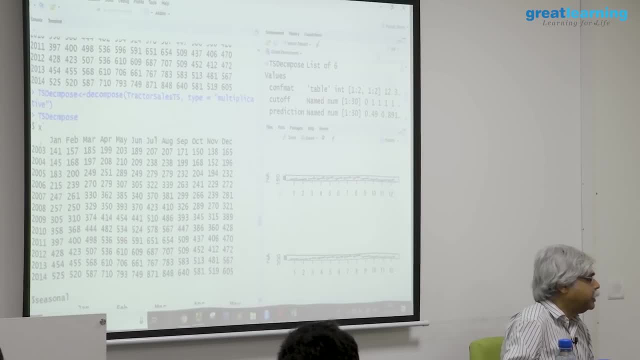 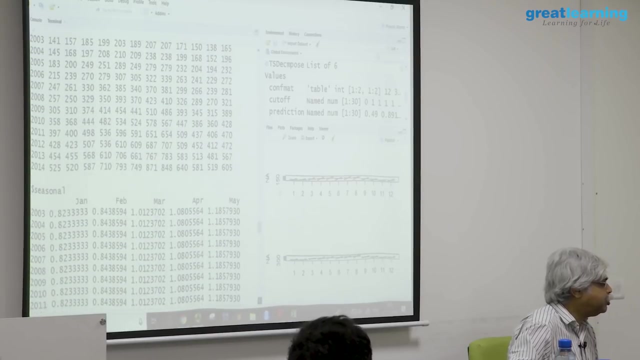 you is. it gives you the original series, which is X. this is the original series. no modification of it whatsoever, no changes. it just gives you the raw data. it includes the raw data in the output. cool, now it starts adding certain things. the first thing that is showing you is is showing you seasonal. 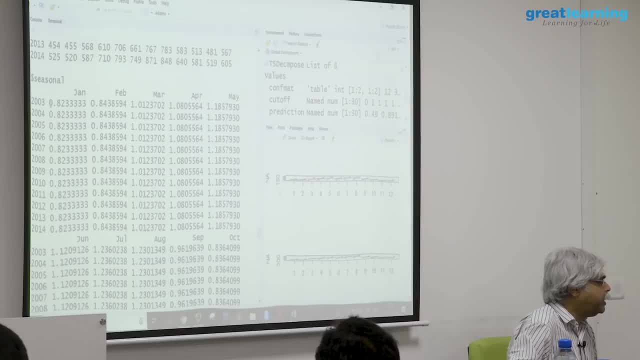 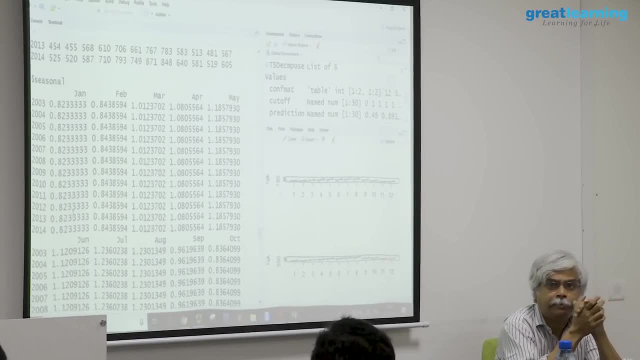 hmm, now what is seasonal? let's look at this. this is January, February, March. but here's the interesting part: the seasonal factor is the same for every year. so all I need to do is look at the seasonality for one year. what does this mean? it means that in January, you are going to sell about 82 percent. 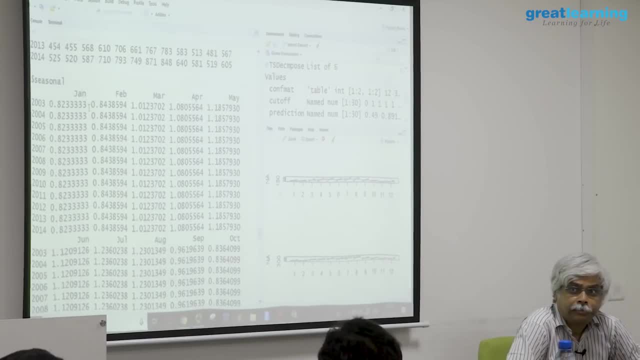 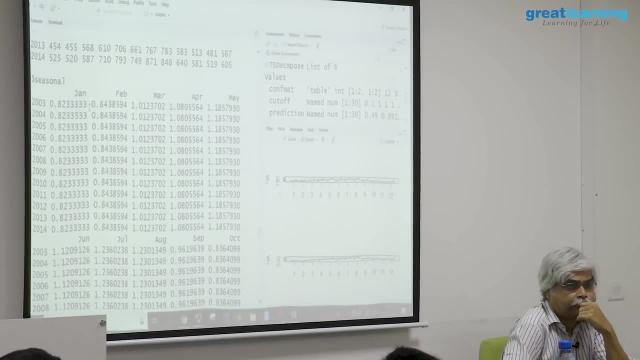 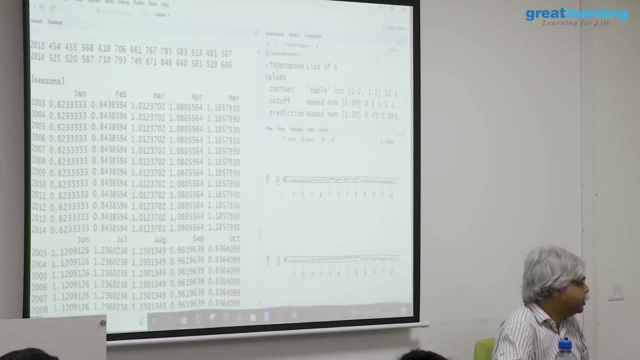 of your annual trend, whichever be the year. in January, if you SKU is sitting in this, you encounter some kinds of Cube that is called They goal standards. you sell about 18% less in February. you sell about 16% less. in July, you will sell about 23% more. in August, you'll sell about 23% more. 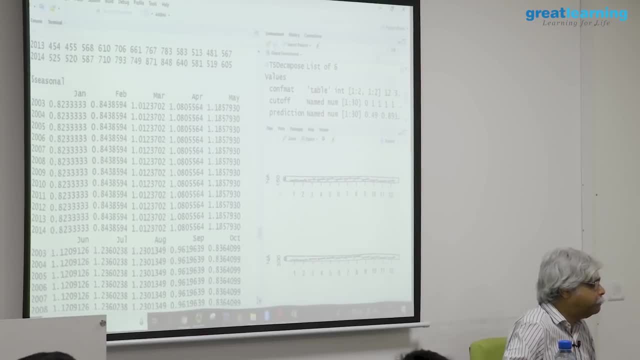 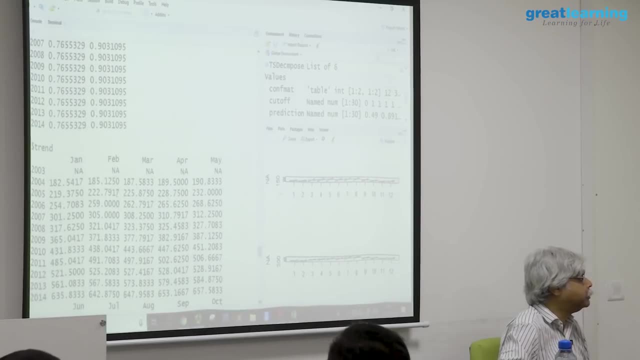 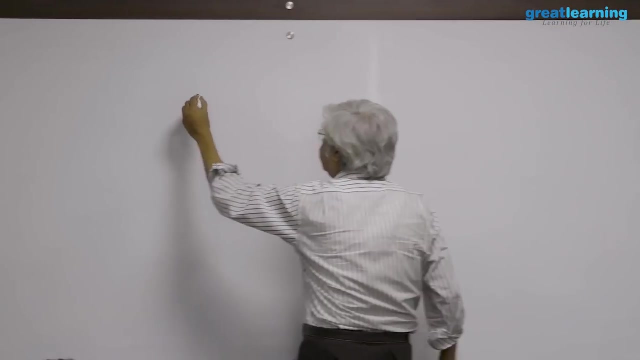 good question. so to do that, we need a, we need a baseline trend on which this applies. so let's see what that is. so this is the seasonal part. then comes a trend part, then comes a trend part. now remember what my equation is. so let me write down my equation. my equation is that, whatever be my series, let's say my. 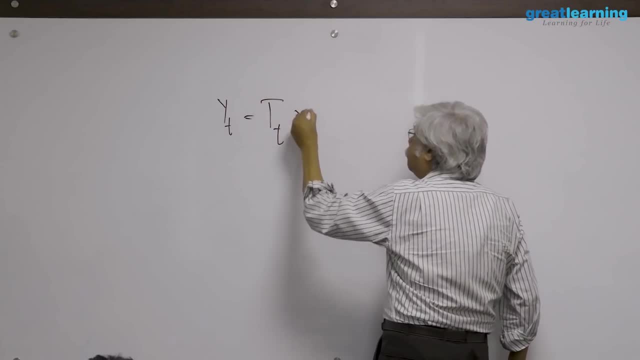 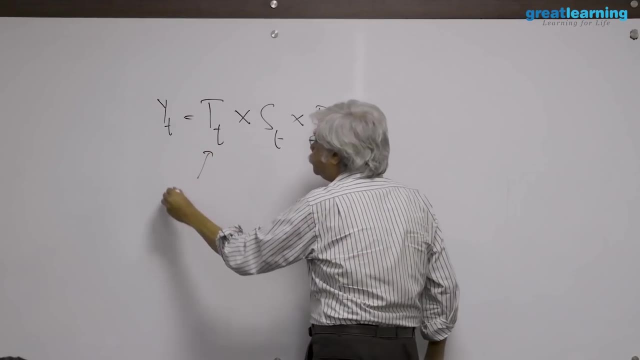 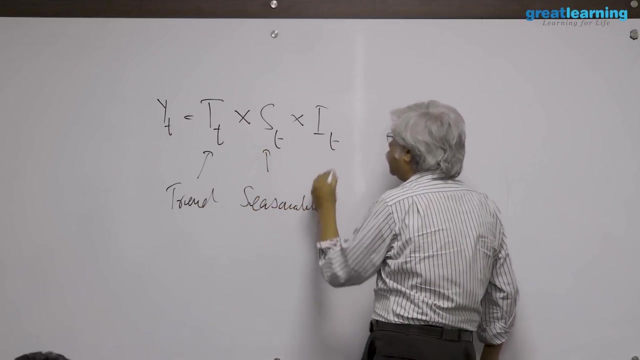 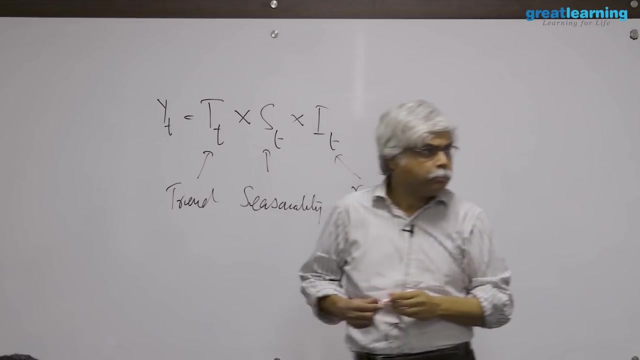 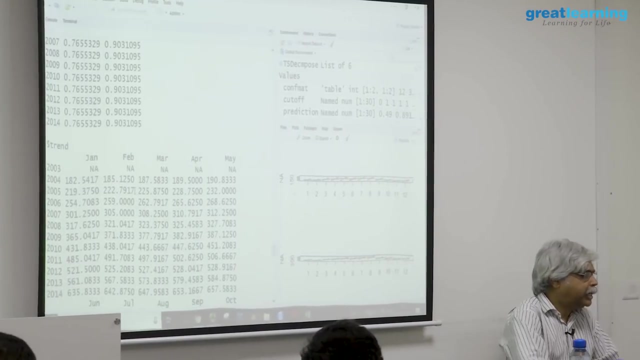 Y of T in this particular case, is trend multiplied by seasonality, multiplied, let's say, by my irregularity component. this is my trend, this is my seasonality and this is my irregular or random component. then what it does is in trend. it doesn't fit a straight line. you'll see what this trend 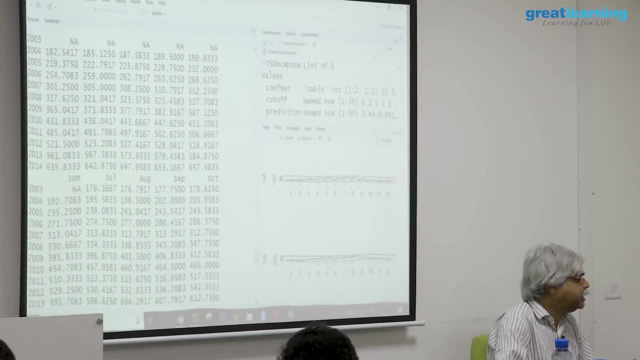 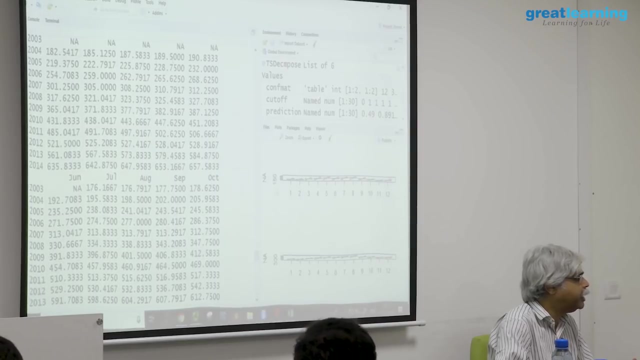 looks like. so it calculates a trend and, as you see in this trend, this trend is a steadily increasing number. this trend is a steadily increasing number. if you, if you track it year to year, we'll see the plot of it soon. but this trend is a steadily into 182, 185, 187, 189, 190, then after 190 is going to be seasonally. 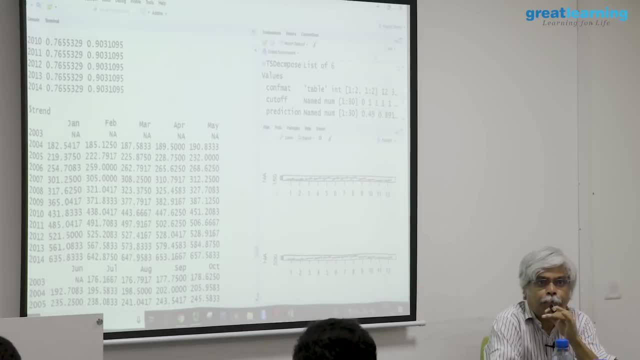 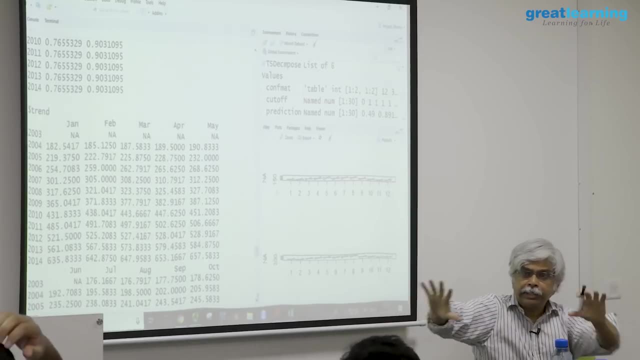 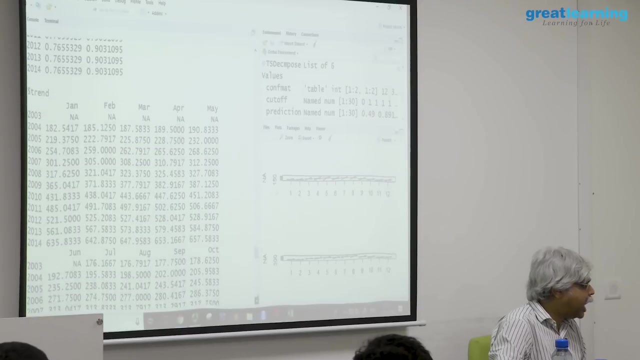 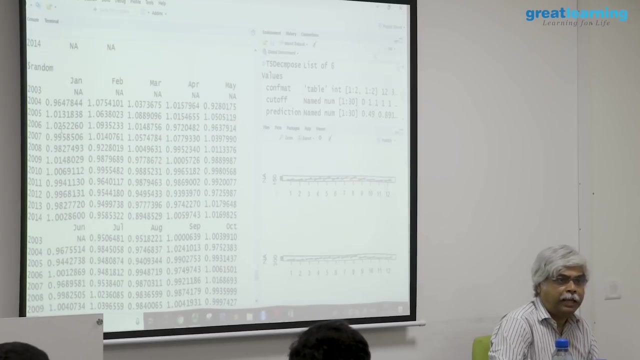 value will always remain the same. that's the whole point. that's the whole point. the seasonality factor is independent of the trend factor. trend is taken out, seasonality is taken out. these are separately taken out. and then, after the trend is, after the trend has been calculated, then it calculates a random. what is this random? this random? 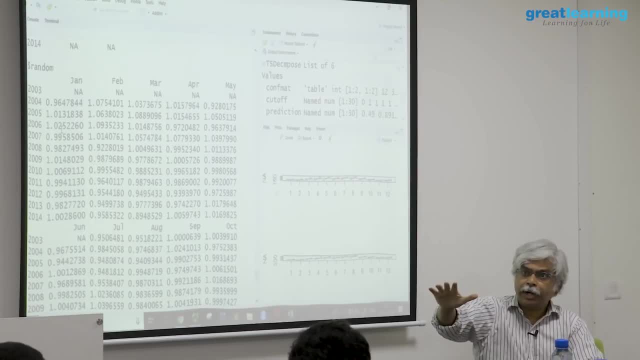 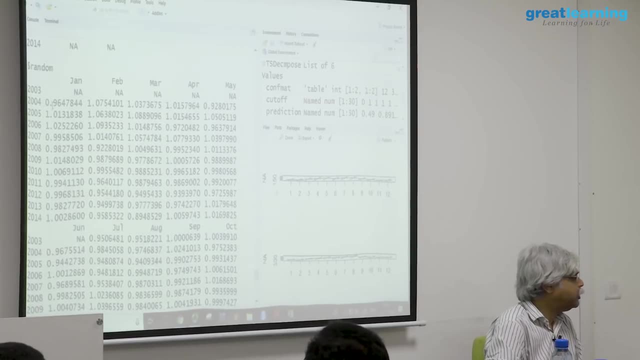 is: you take the series, you divide out by the trend, you divided by the seasonality. this is the error that is there in that specific month, which means that, let's say, 2004 January, 2004 January was about four percent less than it should have. 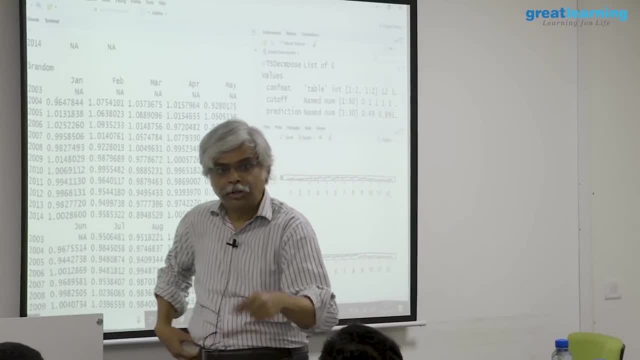 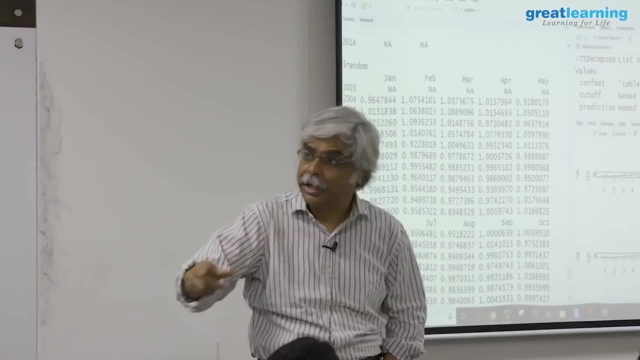 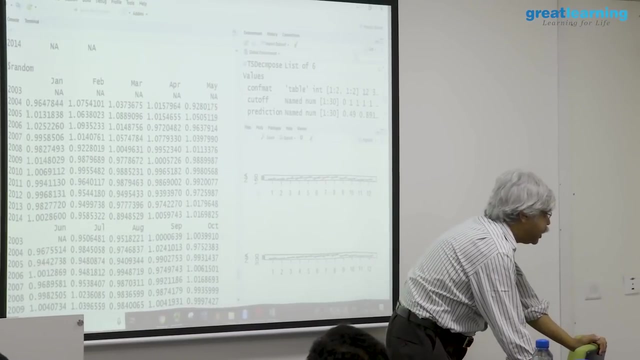 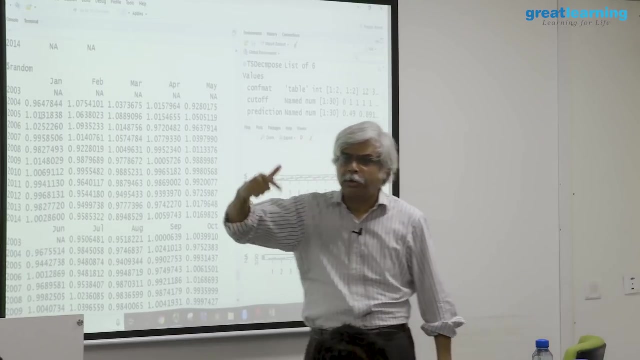 been after accounting for trend and seasonality. this two percent has nothing to do with that year or with that January. if I look, for example, at the at the next January, the next January is 2005, where I was at about maybe about little, about one percent more than what my trend and my seasonality forecast this. 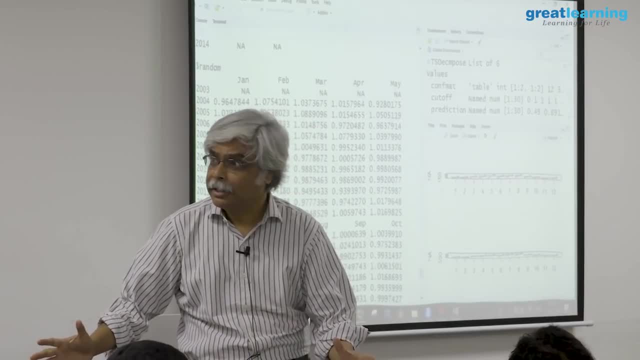 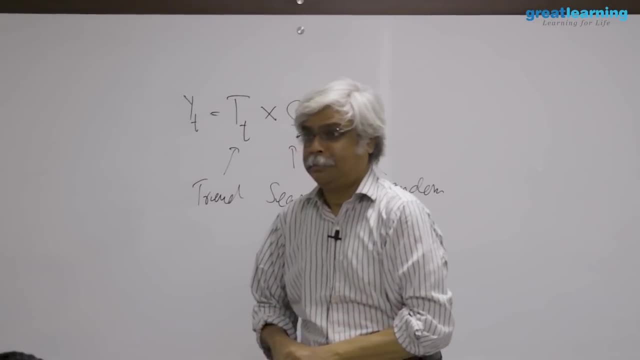 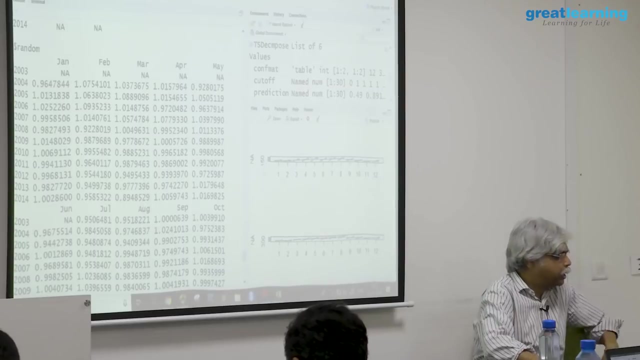 is unpredictable. it has nothing to do with the trend and it has nothing to do with the seasonality. it's the peculiarity of that month for that year. this is what it says. if you are looking at hacking numbers, it may be simpler to simply plot this in other. 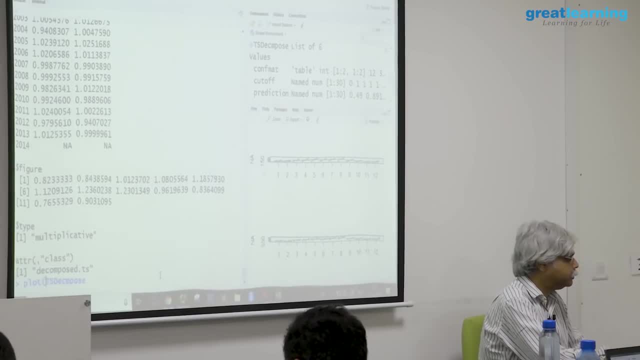 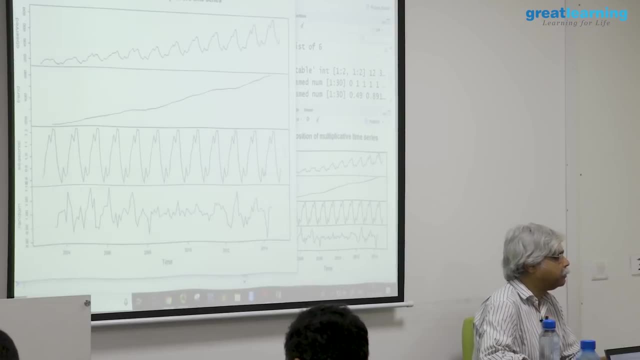 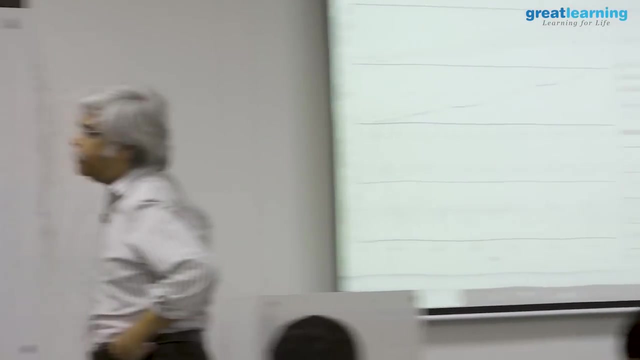 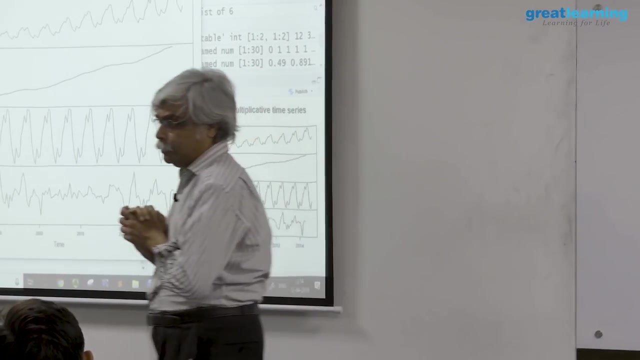 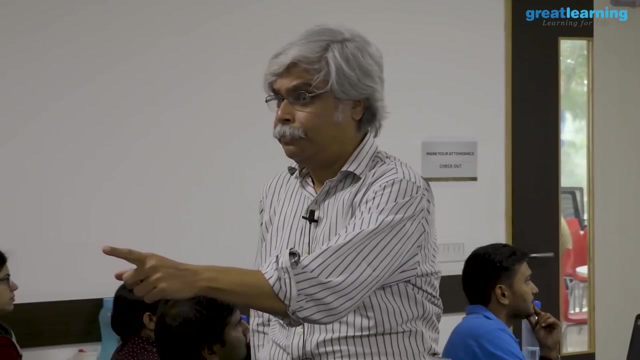 words. what I can do is I can just plot this. if I plot this, this is what I get, and this is sometimes an easier number or an easier graph to see. what is the first graph- the original series. the first graph is the original series. what is the second graph? the second graph is the trend. it has removed. 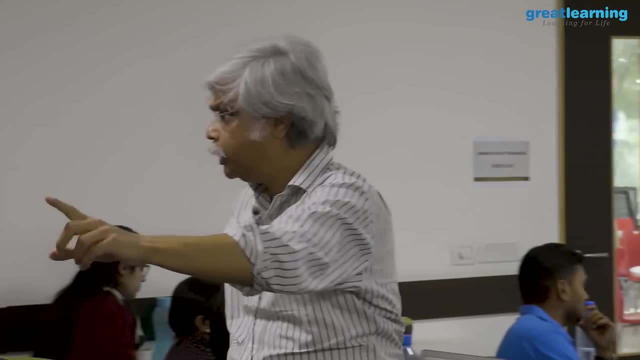 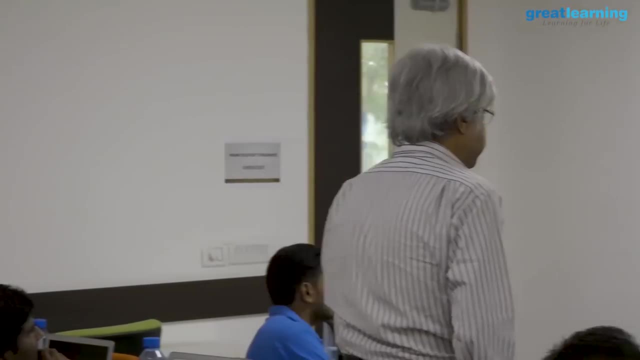 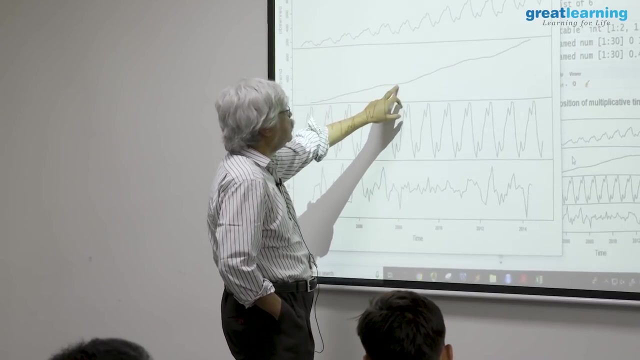 the seasonality. the seasonality has been taken out. what is left is the year on year trend. what it tells you is that it increases. there's a little bit of a flattening that is happening here, maybe around two thousand and maybe five or six or thereabouts. a little bit of flattening that's happening here may be. 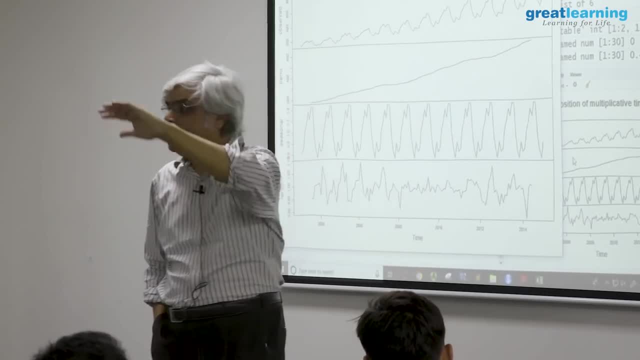 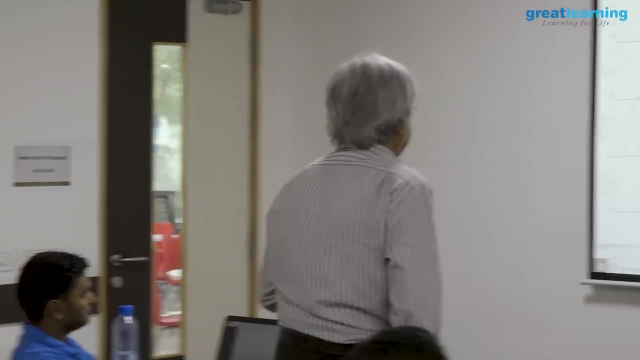 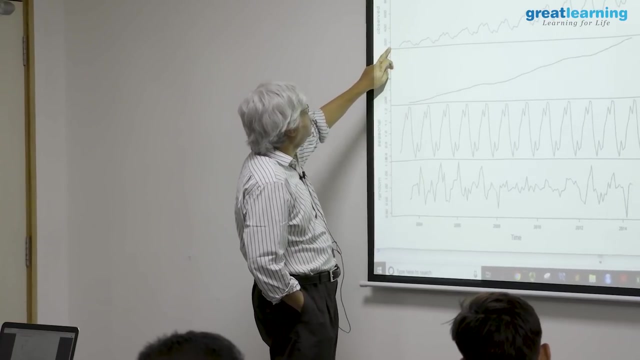 around 2011, but, by and large, is an increasing trend- is average of the seasonality. then comes the seasonality correction. Now, at this point, what I would like you to see is I would like you to see the units of the original series. you observe series. the units are here from 200 to 600 or 800. or thereabouts, which is in the actual sales. the units of trend are also like that, but the units of seasonality are not. the units of seasonality go from around 0.79 or 0.8 to about 1.25, it is a dimensionless quantity. it just multiplies. 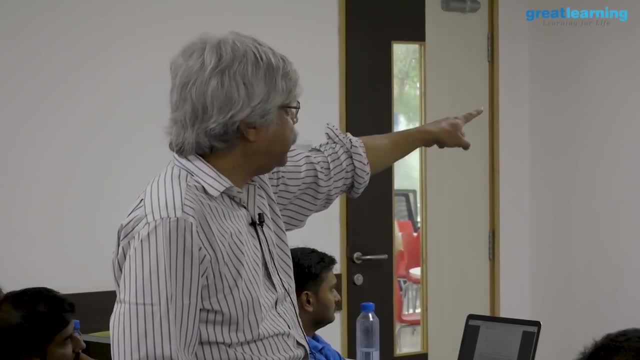 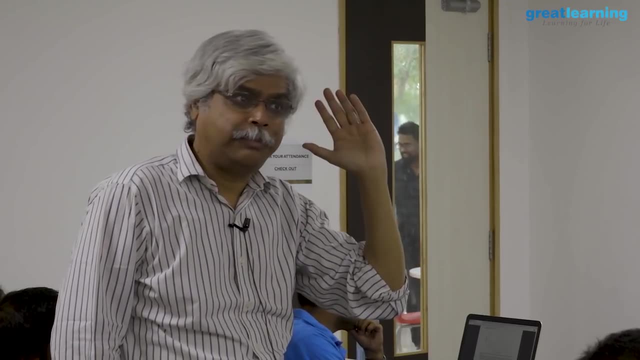 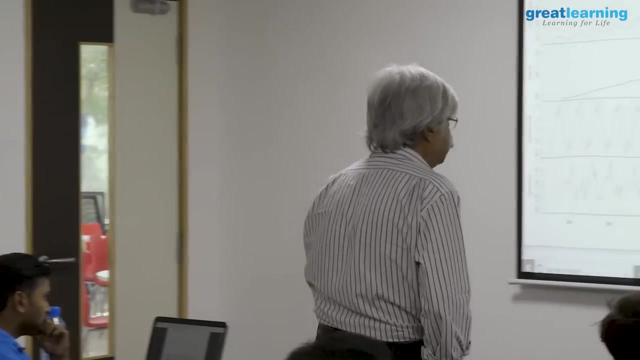 How much does it multiply by whatever that seasonality is? also, that seasonality shape is identical from year to year. trend has been taken out. the irregular part has been taken out. So there is nothing irregular about the seasonality. the seasonal part is repeating. 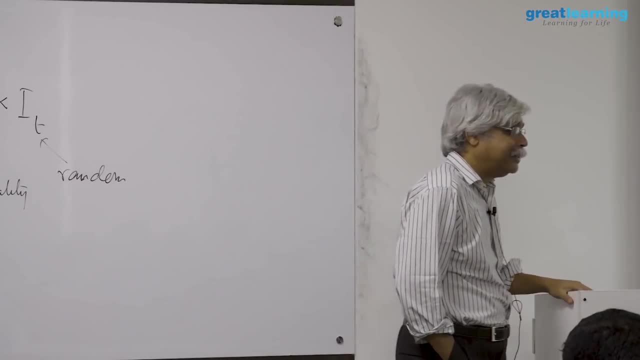 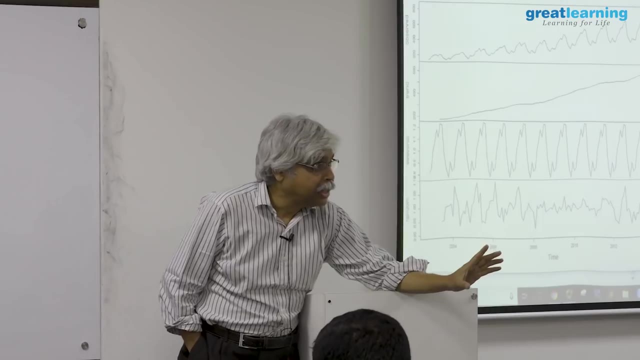 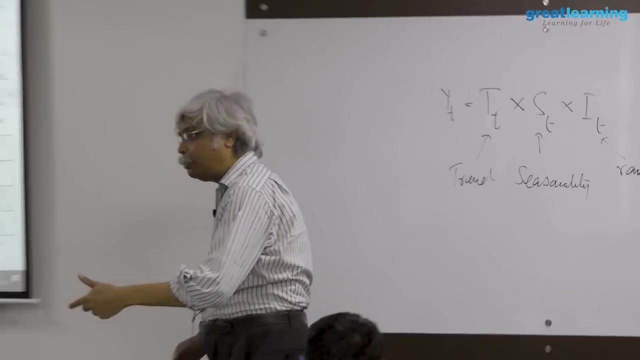 It will do this for whatever data you give it, If you have. if your original time series was created with frequency equal to 12, remember, when I created the time series object, I created it with frequency equal to 12, now I then ran decompose on it. when it ran decompose. 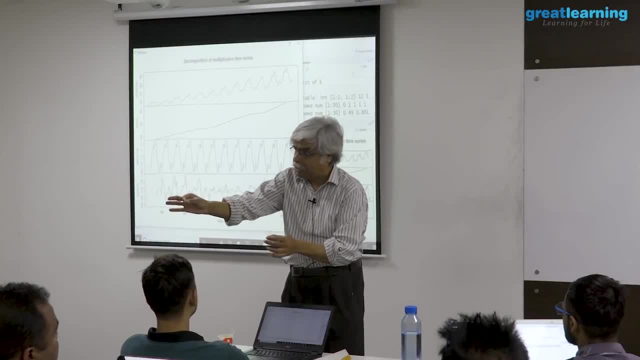 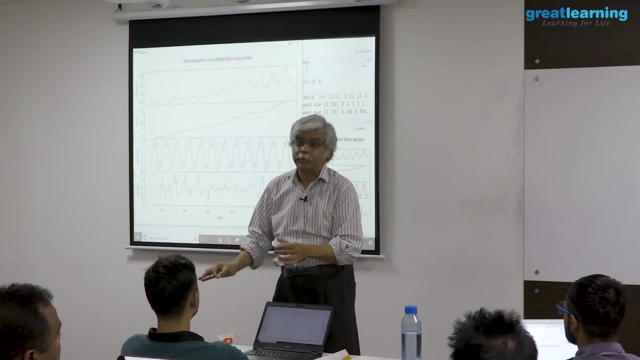 on it. the decompose function ran on the time series object. the time series object inherited the frequency value. as soon as it inherited the frequency value, decompose knew that I now needed to have 12 seasonal parameters. I needed 12 seasonal terms. 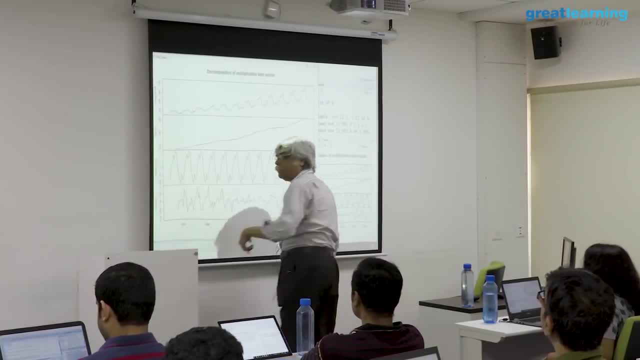 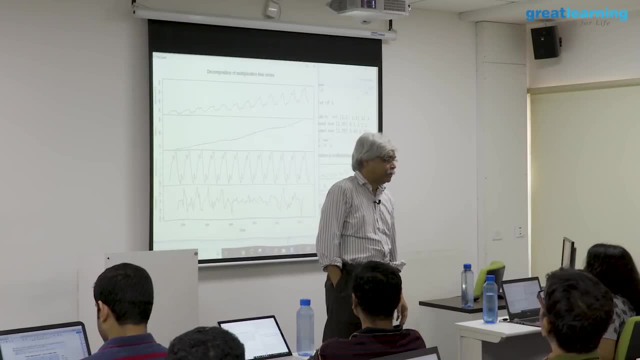 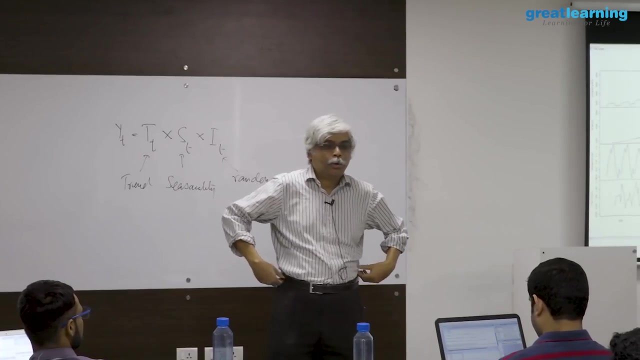 So it is split it up into this. if you give it a series in which it is also monthly but there is no seasonal effect, let us say there is nothing seasonal about this particular thing that happens monthly. No, that is the whole point of seasonality. remember, it is a decomposition and the decomposition 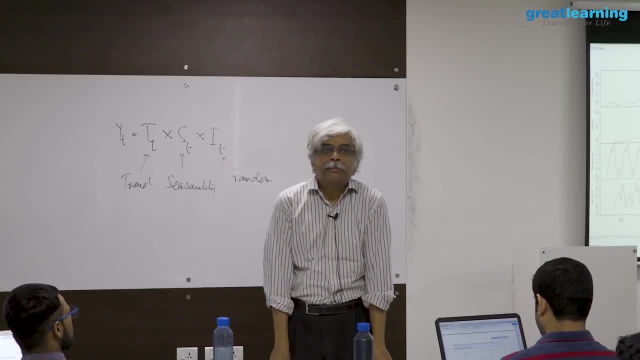 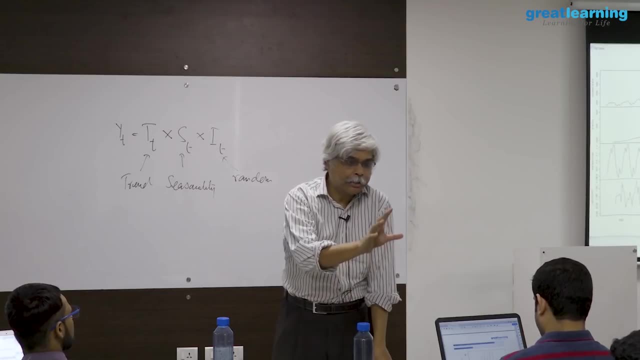 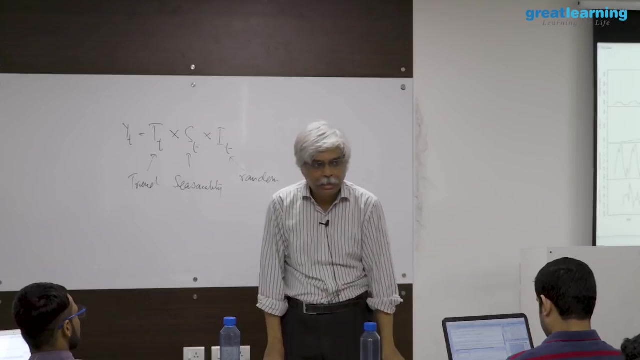 says, is that how do I understand the sale of tractors in, say, August 2007.. I want a description of this, of August, of the sale of tractors in August 2007, and I say I am going to decompose it into three pieces. one is because it is 2007,. the second 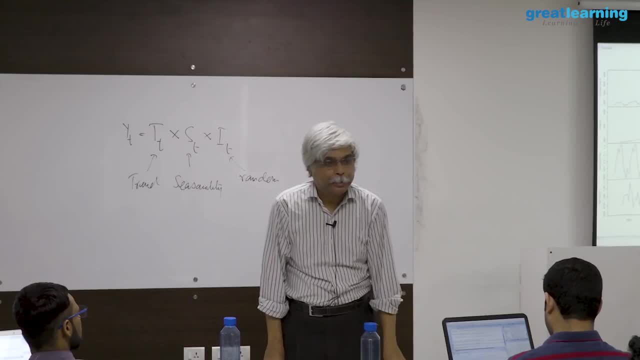 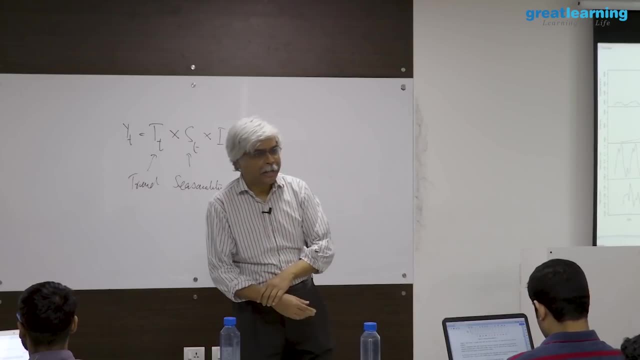 is because it is August, and the third is because I have no idea what it is, because whatever is unexplained, whatever is random. So I am decomposing it that way. if I do it that way, then the correction for August should be the same for every year. 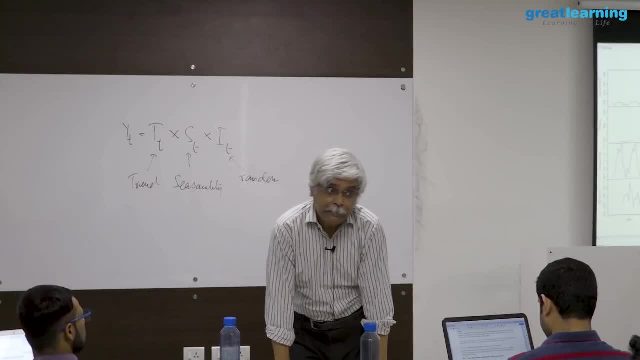 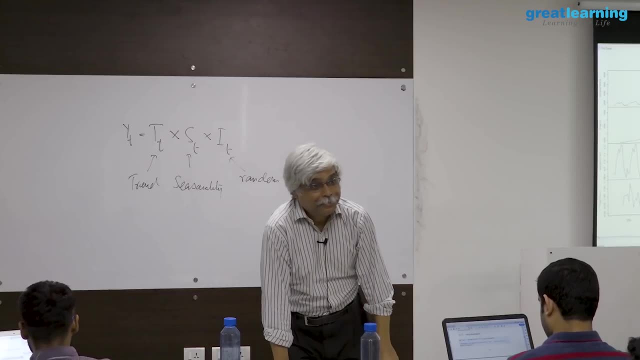 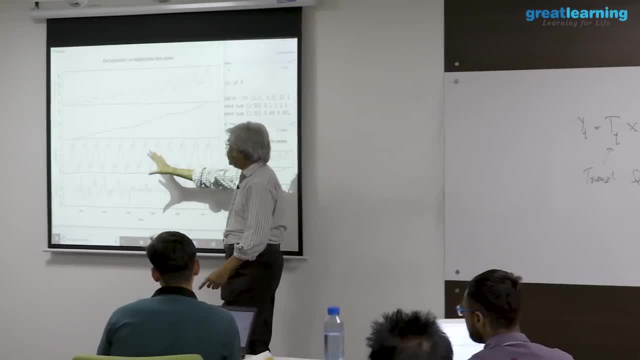 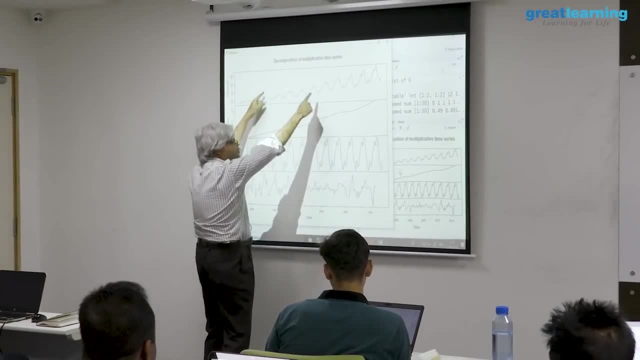 Now the reason is written this way is: strictly speaking, this plot should not exist. what should simply exist is one of these shapes. the other shapes are just copies, but it is done this way for the visualization, so that you can sort of go up and down this picture. 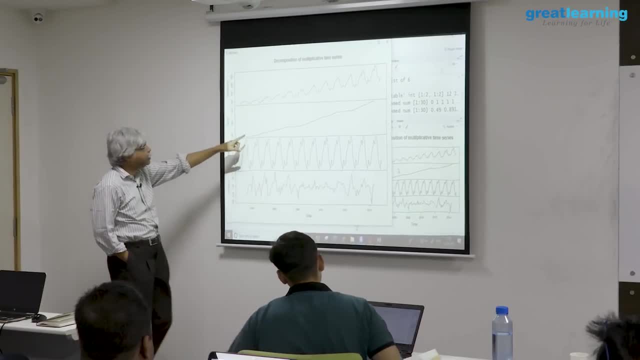 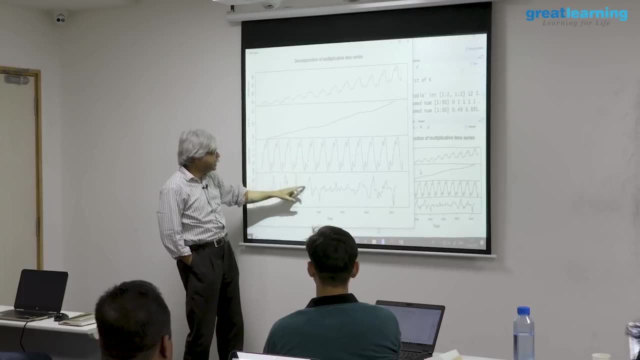 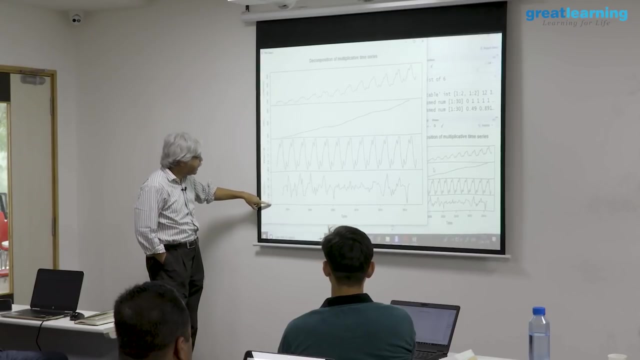 because now, what is this third component? This third component is simply this. it is: take the observation, divide by the trend, then divide by the seasonality and see what is left. this is the error. This error goes from about 10 percent is about sort of minus, sort of 90 percent to about 1.1 percent, which means that this unpredictable, unsystematic error is about 10 percent A plus 10 percent on. within course of good year you have a surprise sale of more than 10 percent of 10 percent positive, or you have a surprise loss of 10 percent on the negative. 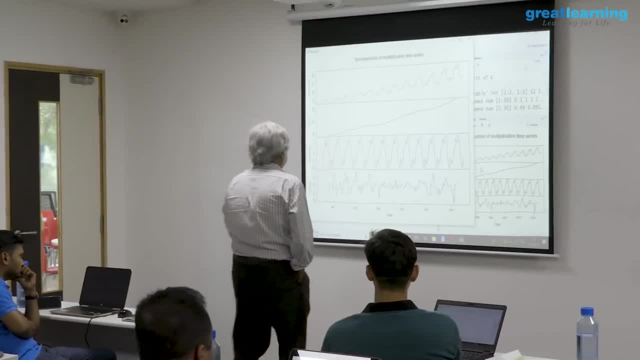 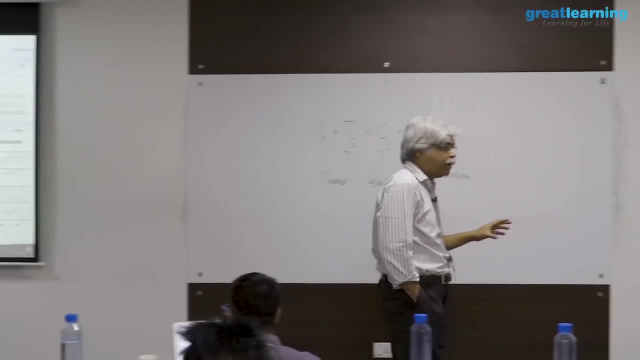 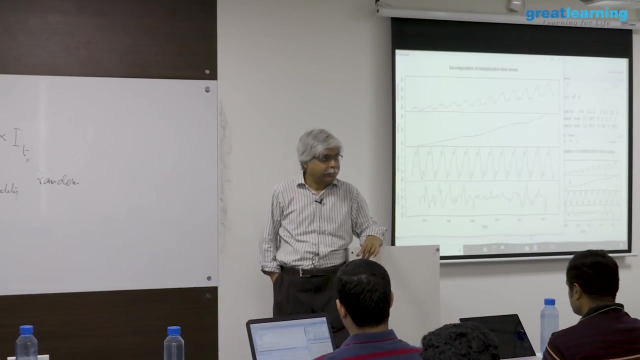 side. but here is the. here is the interesting thing. this particular here has no shape to it. it should not. it should have no, it should have no trend. it should have no seasonality. it should look random, which in this particular case is ok. if this has seasonality, that should. 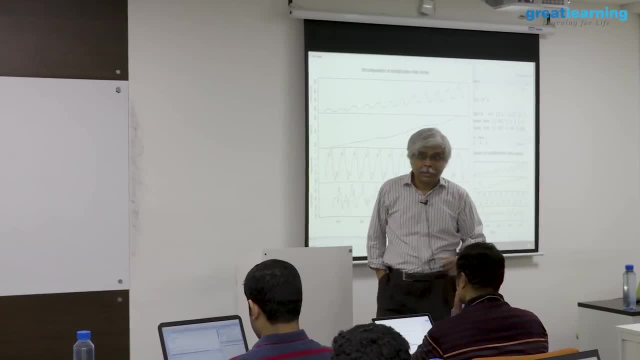 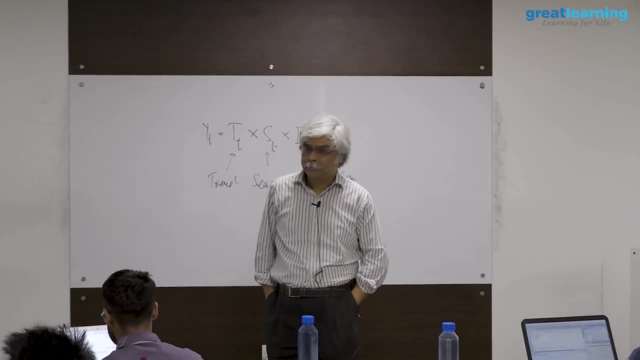 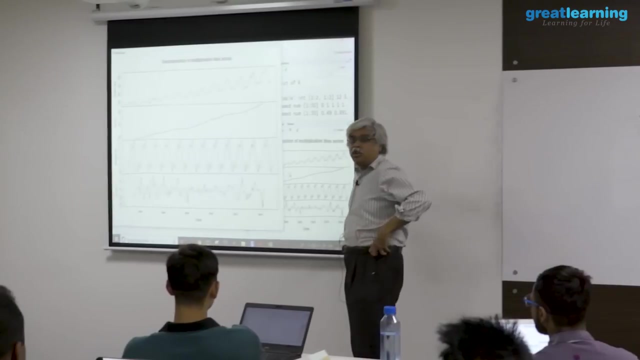 have been captured in the third plot. Ok, If this has trend, that should have been captured in the second plot. So now, if we use something like this to forecast which we may get to today- I am not a 100 percent- 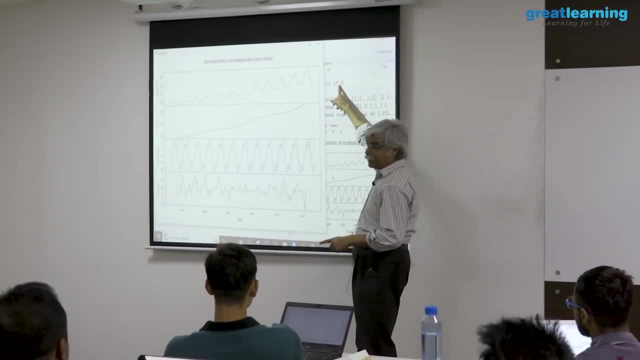 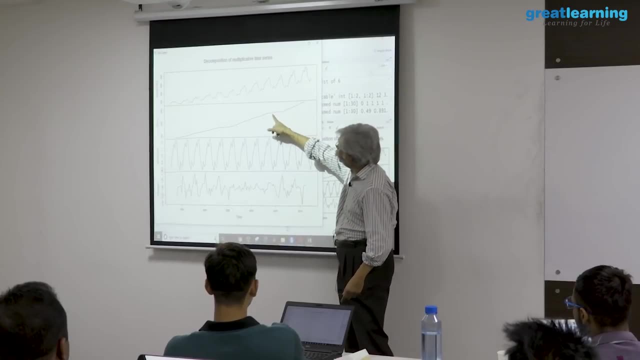 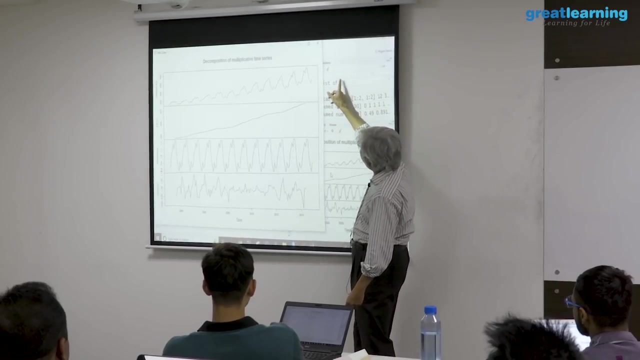 sure this will forecast. when this forecasts, how will my forecast operate? My forecast will operate this way. I need a way to predict extend this line. Once I have extended this line, then I will see what month am I in, whatever month I am. 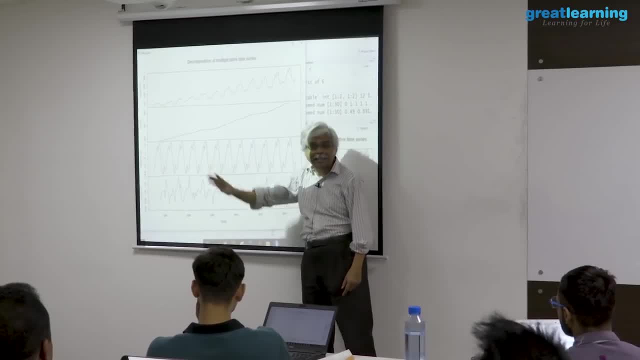 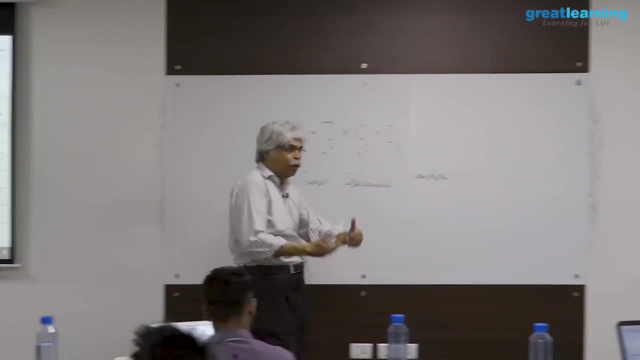 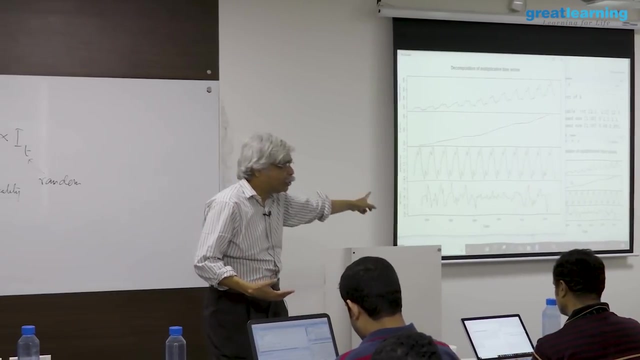 in. I am going to multiply by that number seasonal correction, and that is it. I am going to ignore the third one. So my forecast problem becomes a problem of simply forecasting the trend. I am not forecasting seasonality. I am not forecasting seasonality at all. all I am doing. 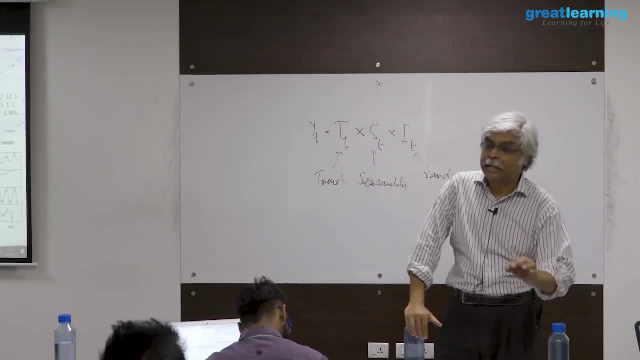 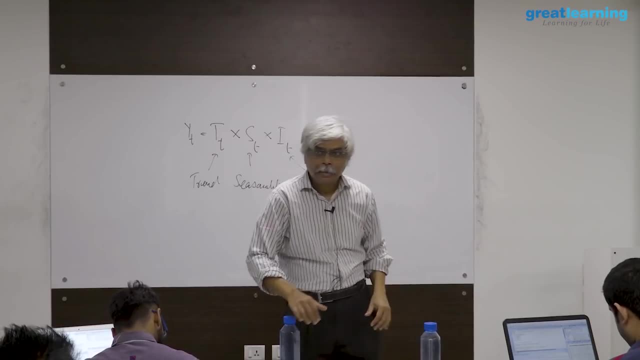 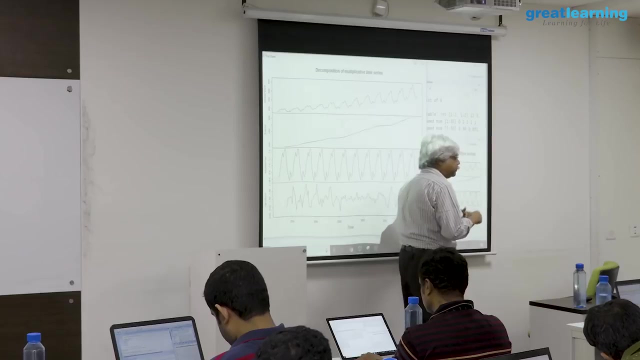 is, I am estimating seasonality based on the past data and applying that same factor in the future. That is all that the forecast will do, which is what typical decomposition based forecast do. Now, the purpose of this decomposition is not to forecast. yes, randomness is for ignored. 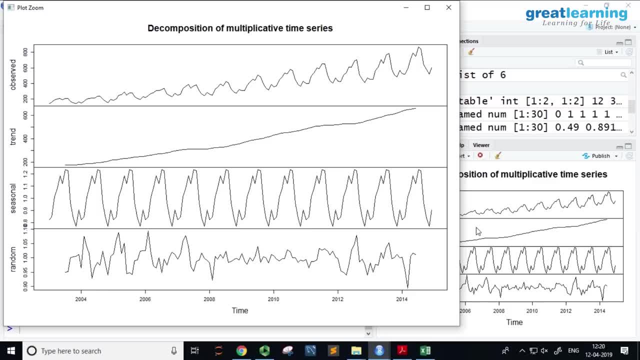 not for forecasting. The randomness part you are seeing is the part that is unpredictable, because in the future you do not know. You do not know what this number will be. If you do not know what this number will be, What is this? 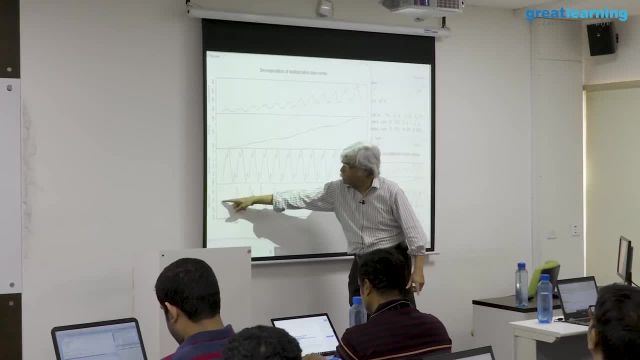 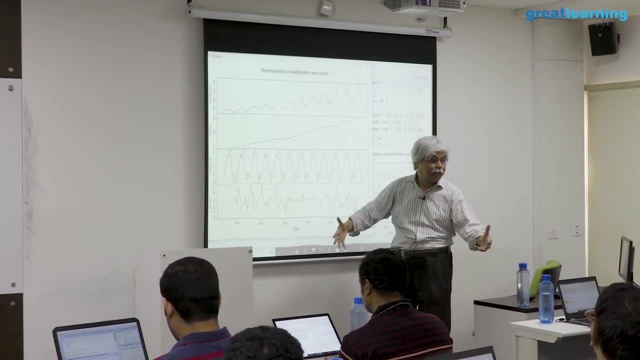 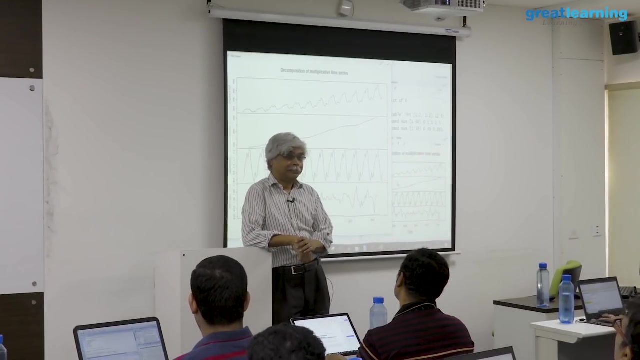 What is your best guess? Your best guess is in the middle, and your best guess is one: No one means do nothing. multiplying by 1 is equivalent of doing Nothing. Is that linear regression where for epsilon you add 0?? Hmm. 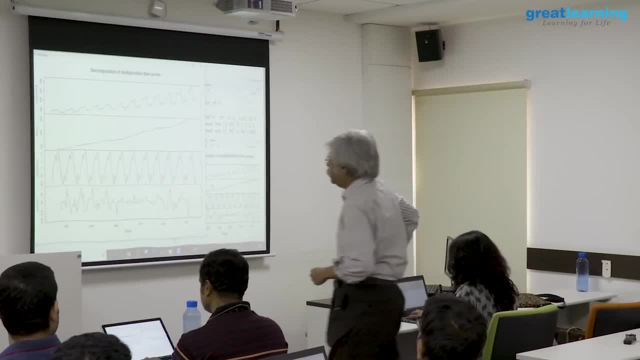 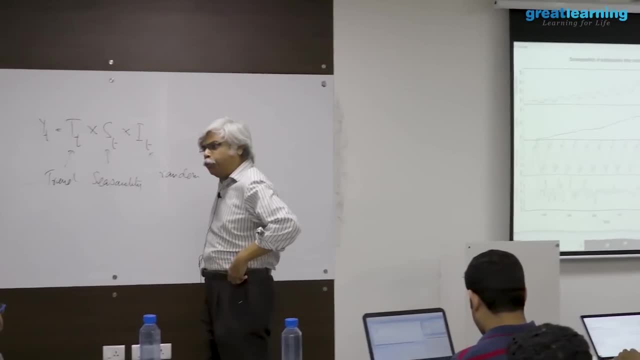 Haa…. So he is asking very interesting question. He is saying: arm, let's say that I'm running a business and I want to estimate the sale of tractors and I want to focus the sale of tractors. now, why do I want to focus the sale of tractors? why would a business want to? 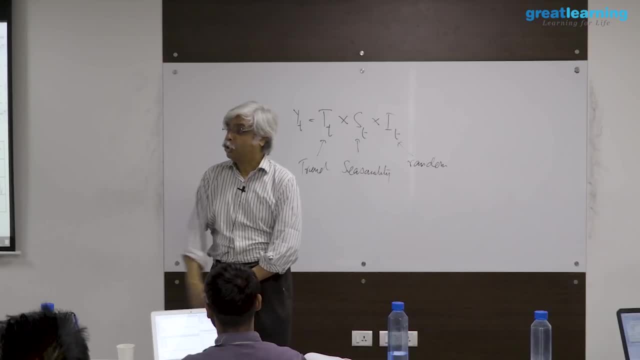 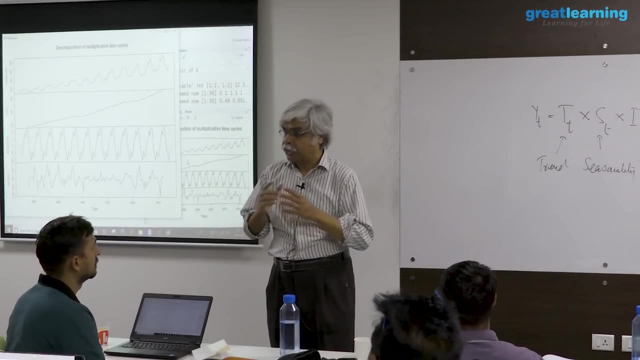 forecast it since, to get up, to get the production right to the plan for production policy, that I am the factory, I'm the factory manager for the tractor company and I want to and I want to focus with since, from since now, when she has given me that forecast. 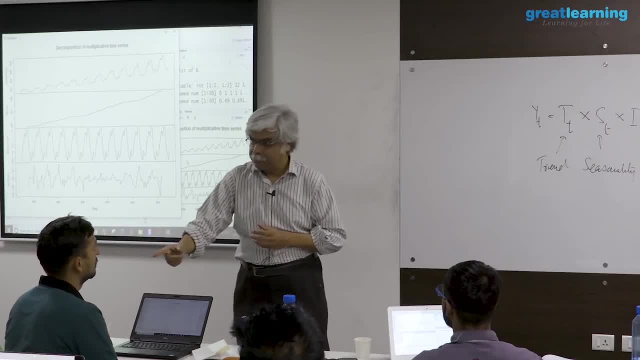 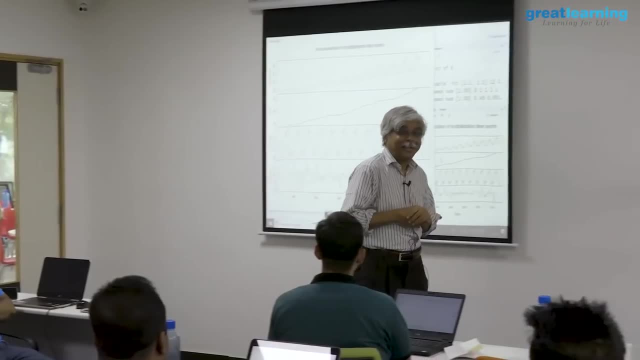 How many tractors will I make? Will I make that many? Will I make more? Will I make less? I'm not asking a statistical question, I'm asking a common sense kind of question. It will be more You would, So it depends. 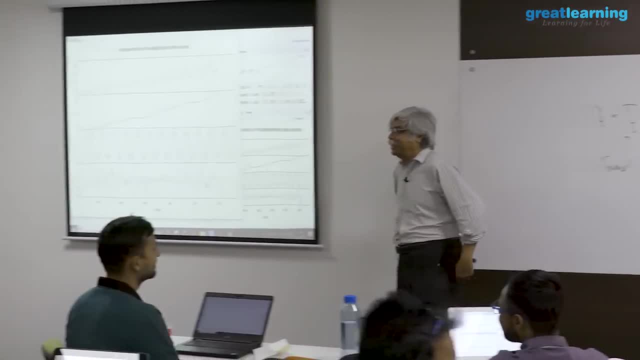 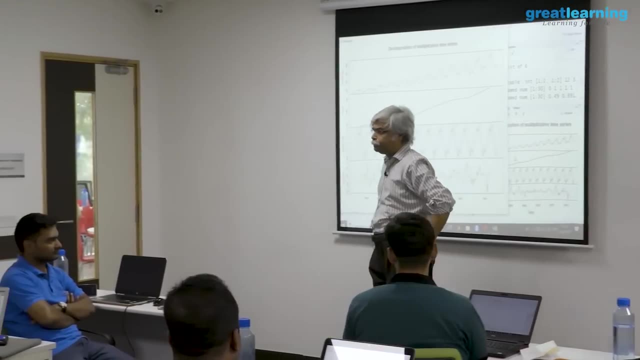 Nice statistical answer. It depends. So, all right, Let me say this, Let me put it this way: How many lunches should be out there for you guys? Number of campers. So one possibility is you're supposed to be 43 or something of that sort. 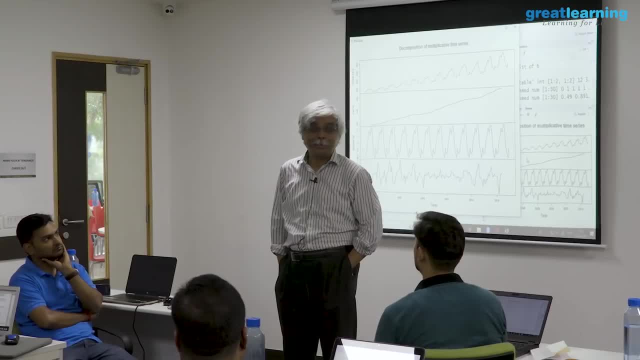 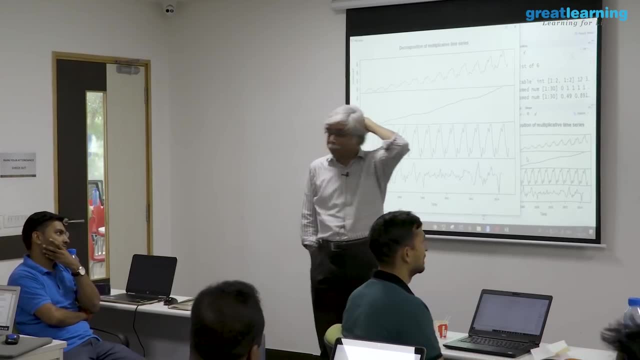 They'll just be 43. That many, At least one more for the hungry person, Or- yes, good point, Lost in carriage, or something of that sort. So that gets to the point that whenever you're in business, certainly. 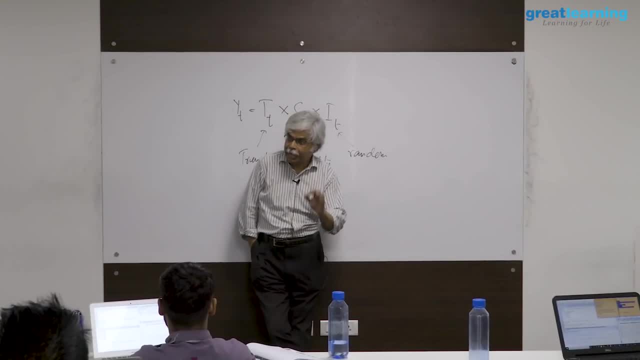 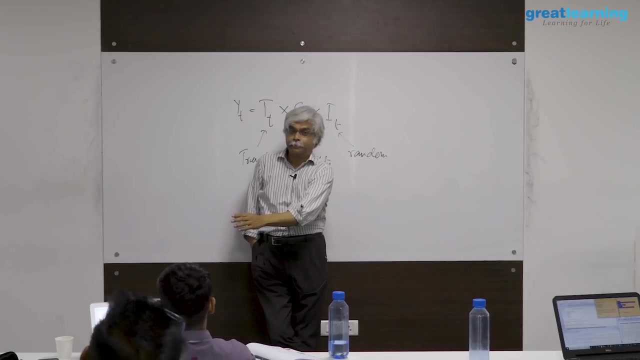 that whenever you get an estimate, whenever you see a forecast, whenever you get any analytical number, you typically use that number in a certain way. that corresponds to either the value exactly, or some upper value of it, or some lower value of it. Now here, for example, for tractor sales, what should it be? 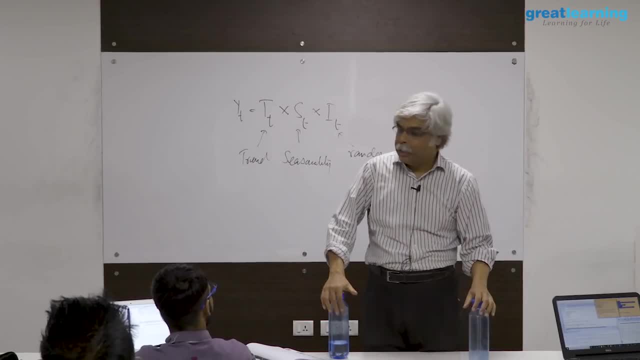 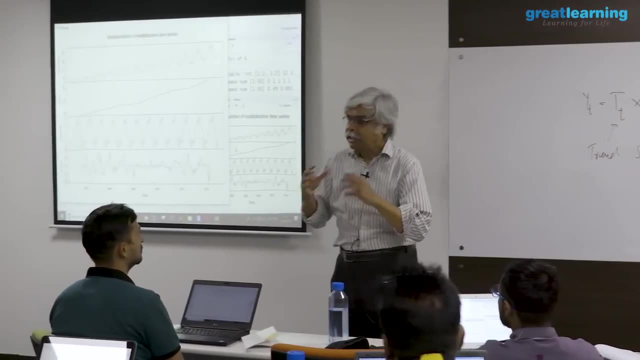 So I can argue the number of ways. For example, I could argue that if sales tells me that I should, i suspect, to sell 500 tractors, I could argue to follow me. I need to make sure that sales is able to Temporarily be. 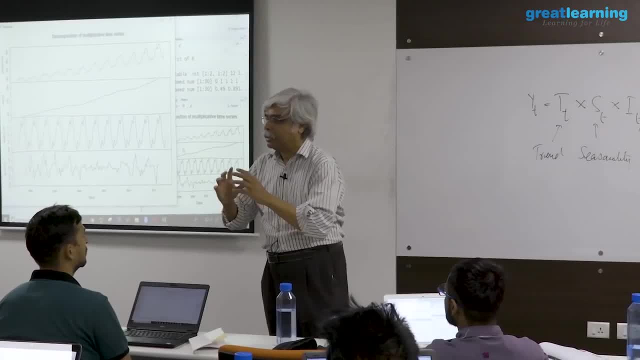 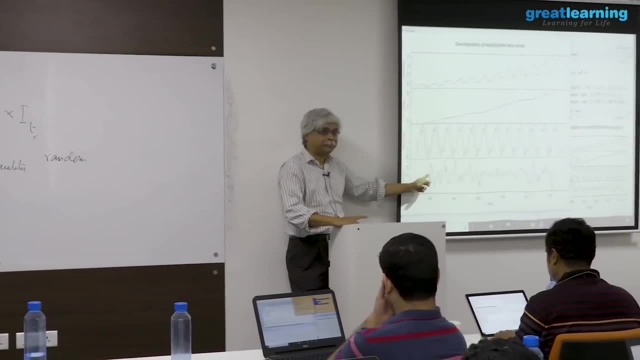 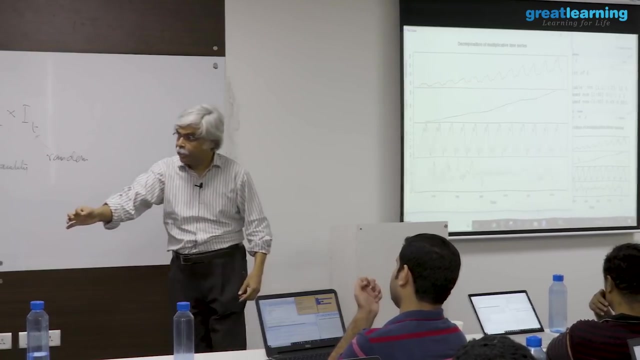 Perfect, that sales will be able to sell 500 tractors. now I know why is this a random question. it's a random question because I know that in the past years sales hasn't always been predictable. so when sales says that it is 500, I know from. 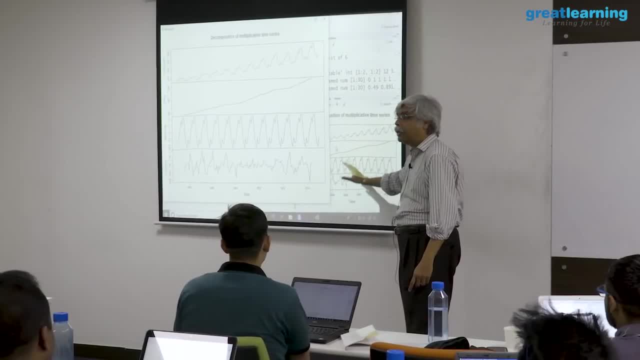 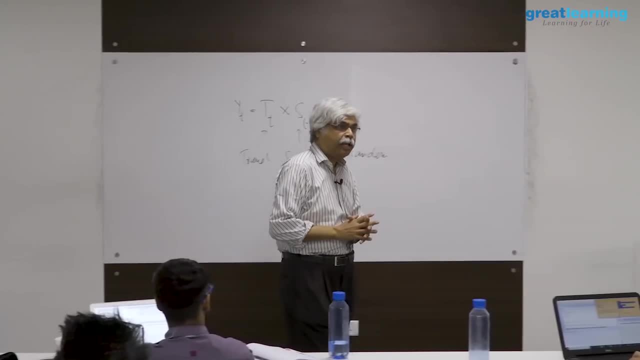 past experience. I do not know whether it will be more than 500, less than 500, but I know is going to be plus minus 10 percent, which means I know that it may end up being 550 or it may end up being 450, but I do not know which way. my trend. 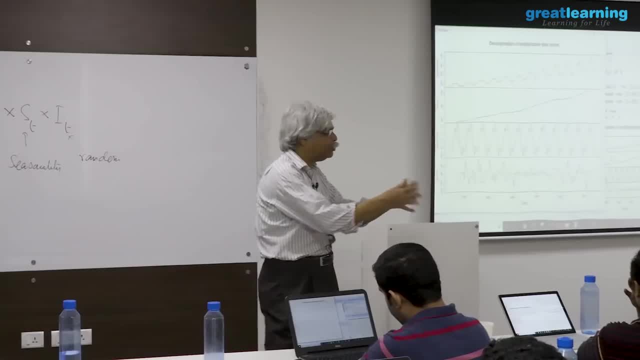 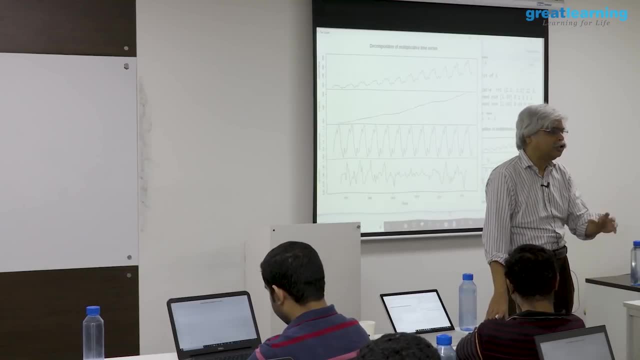 and my seasonality are not doing that. my trend and my seasonality have both combined and I've told me that this is 500, for example. my trend would have said that this is 450 or something, but this is June, month of July, multiplied by the 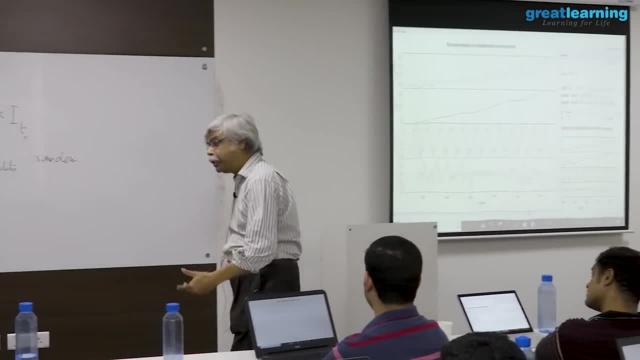 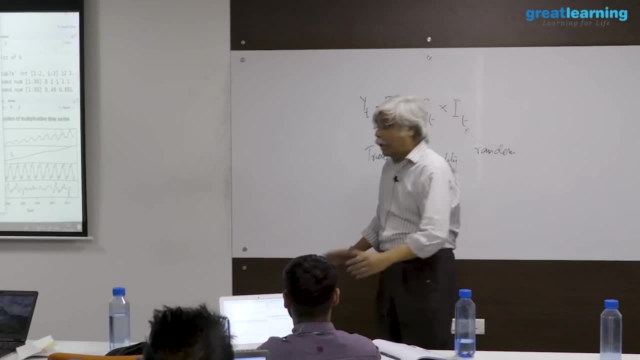 seasonal factor and I've ended up with 500. but even after taking everything into account, I still know that there is an unpredictability to this- and could be between 450 and 500- 550 now I could. now I need to make a decision as to how many tractors to make I could. 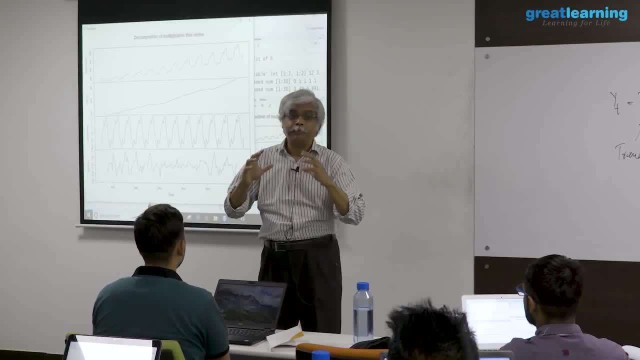 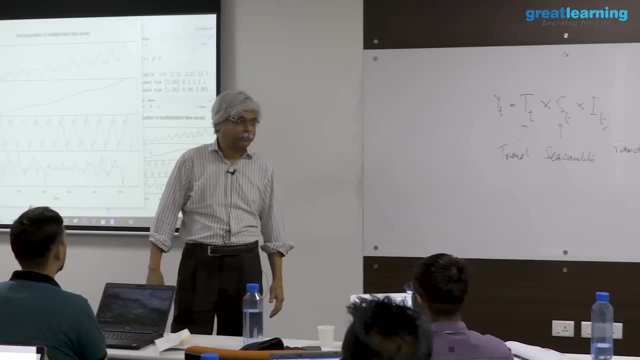 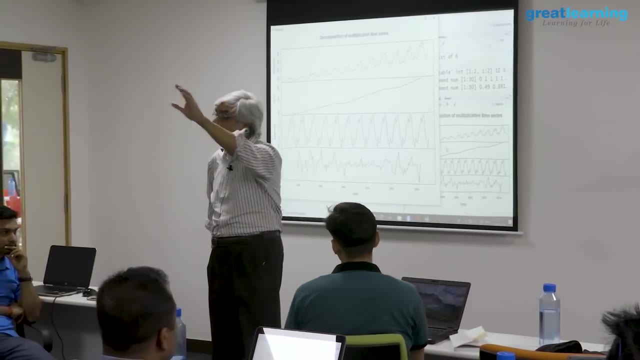 argue in various ways. for example, I could argue: I need to make sure that every customer is satisfied, every customer is met. I do not turn sales away. I don't create a backlog, which means I now need to make 550, which means that even if there is an overshoot on the sales estimate, I'm going to end up with 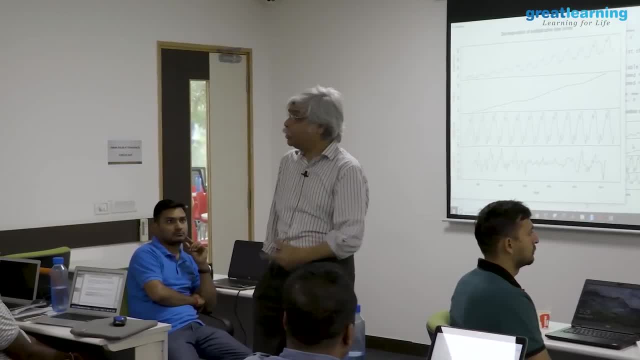 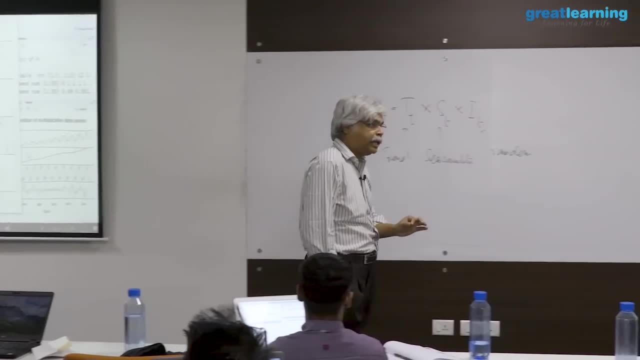 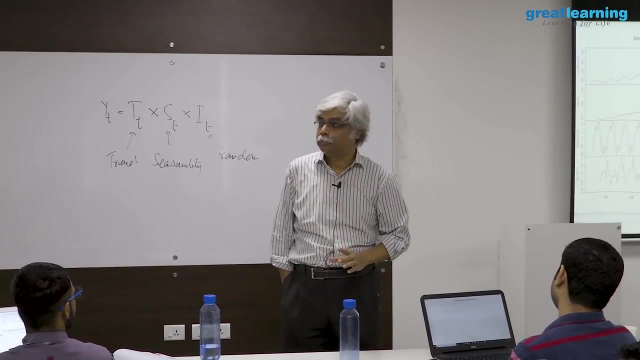 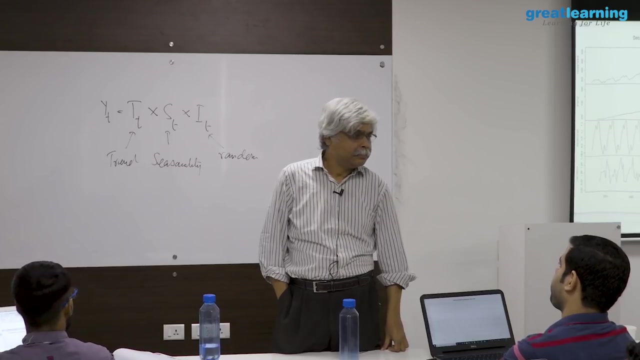 550, or I could say: you know what business is? business is bad. costs of tractor production is high and I already have an inventory. I don't want to produce one more tractor than I need to, in which case I'll probably make 450 tractors. that depends on what I want, for example. 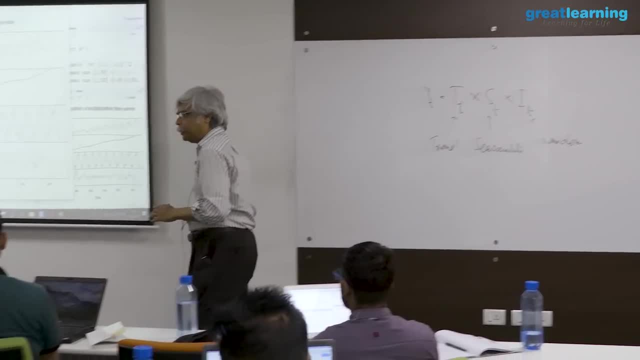 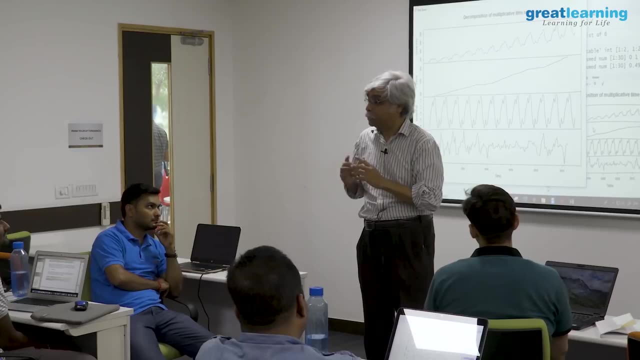 let's suppose that you are trying to understand for these meals or for a sweet shop. now, how would he think this through? he would think this through, possibly. he think he probably thinks of this in a much smarter way than I do. he actually does this. I teach: if you can, you do, if you can't, you anyway. so so he. 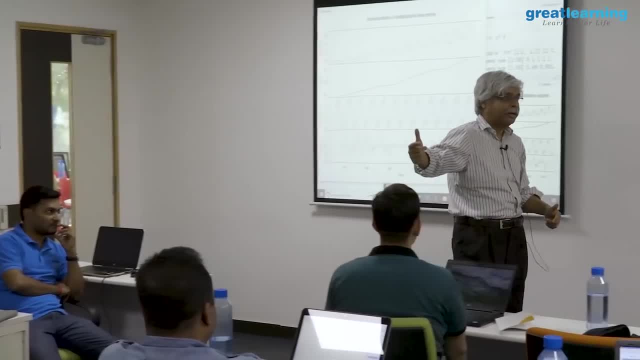 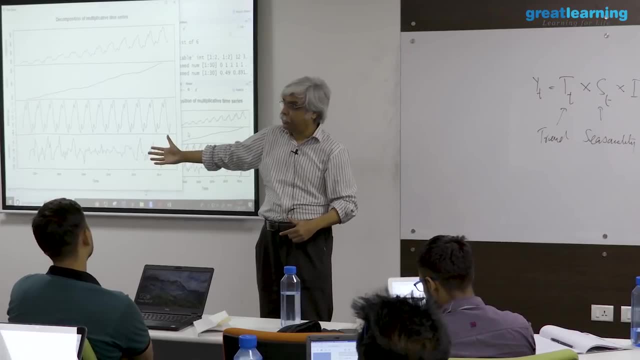 would think of it this way that if I overestimate what will happen, he's going to have to take food away. maybe he has other means of throwing it, or maybe he says that I have to throw it away if he underestimates now, there'll be people. 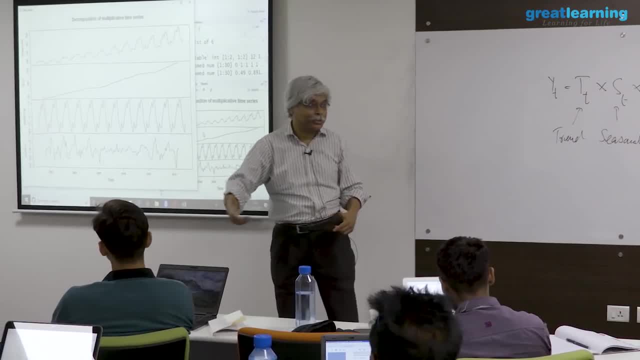 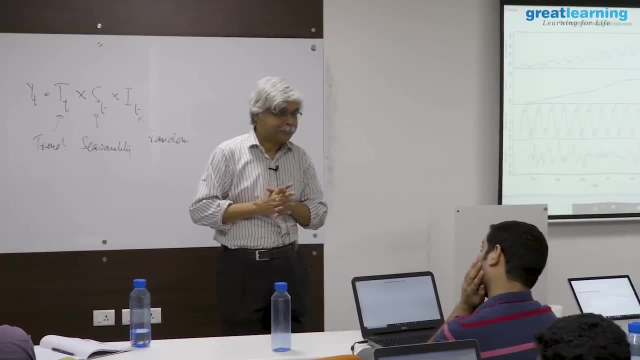 who are going to complain. so now he's going to have to figure this out. so let's say that you are a sweet shop person and you know that you are making something that you cannot store. now if you, if you make too many sweets on that particular 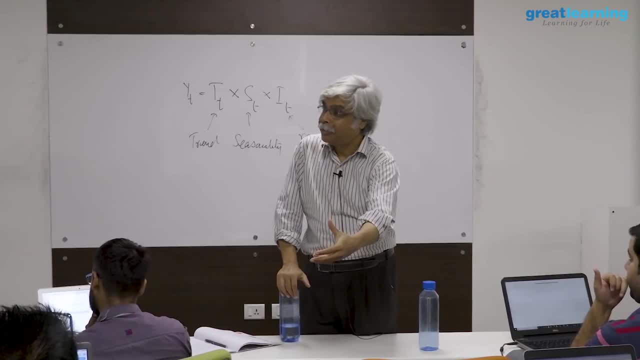 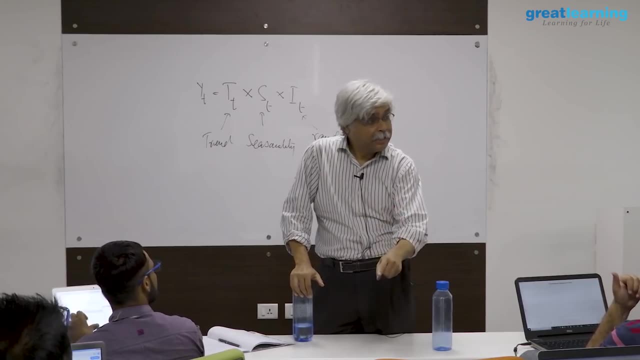 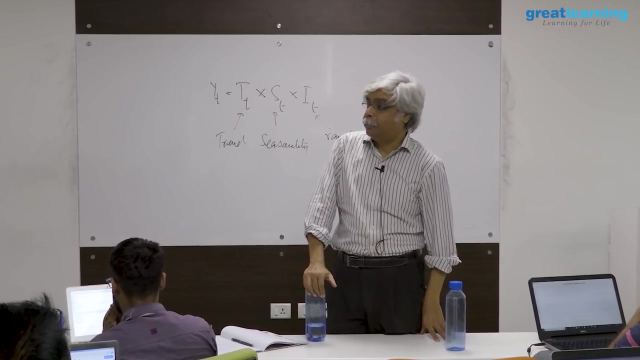 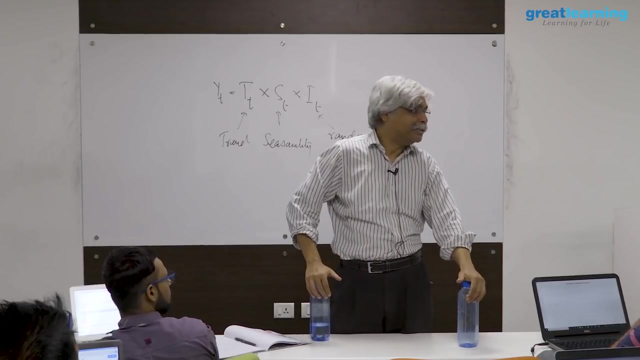 day, you are going to bear the cost of those extra sweets but not make revenue for it. if you make too few sweets that day, then there'll be sales that you could have made, but you do not make correct, which, for you, is the bigger problem. well, you said it depends. it depends on a number of things. so, for example, for 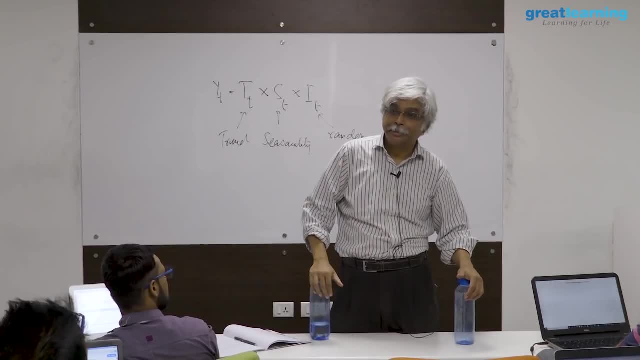 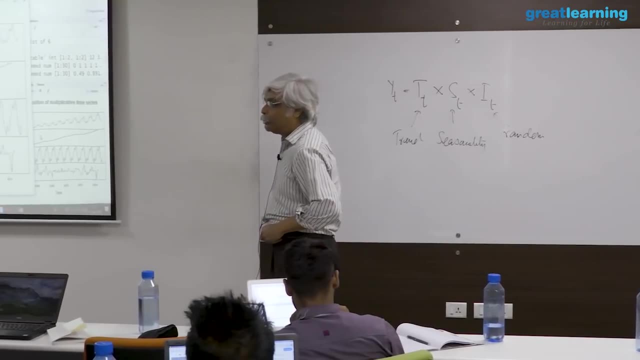 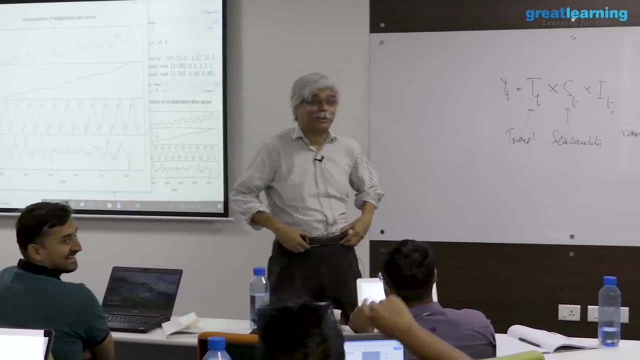 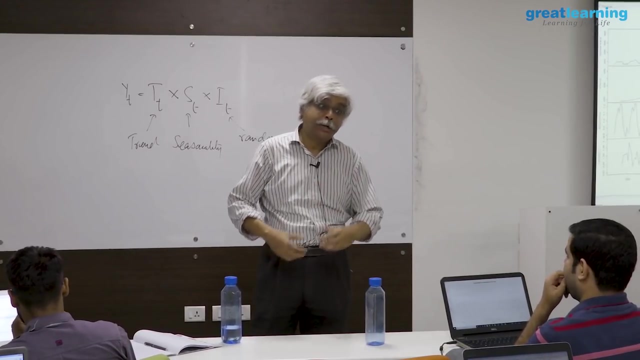 sweets. overproducing may be a far bigger problem than tractors. you decide, yes, you decide what it is. so what is the analytical solution to this problem? the analytical solution to this problem is: I am giving you the range, so of course, that's why I ask the question. when you did optimization, where 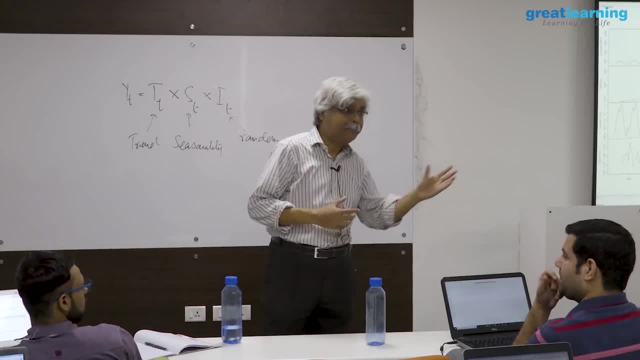 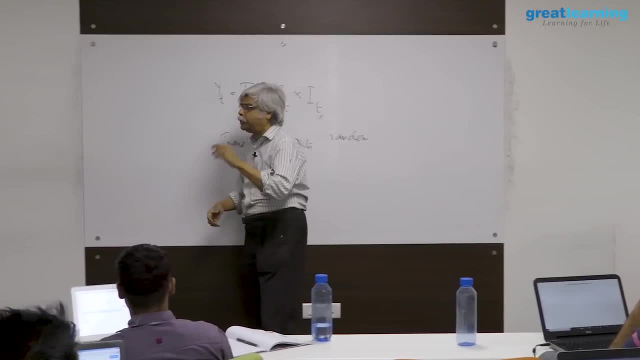 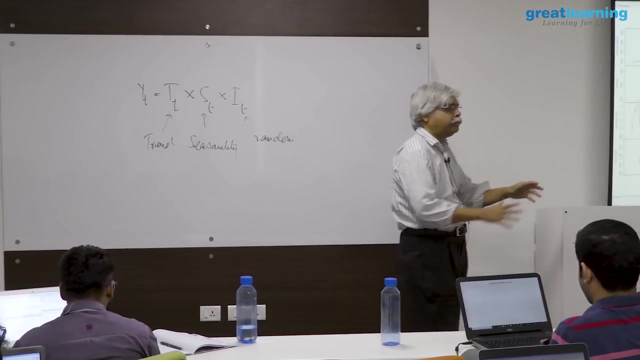 did those numbers come from? it comes from stuff like this. so correct, absolutely right. so now you put it in. you look at costs. you look at, for example, inventory costs, you look at opportunity cost, you define it, your cost, based on your business concepts, and then you figure out what is the minimum cost. 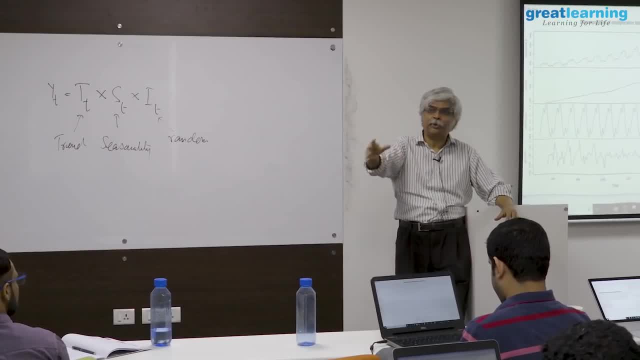 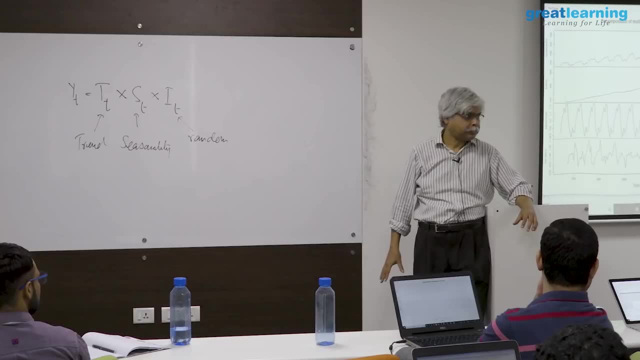 involved in this. the opportunity cost is the cost of sales foregone in other sales that I could have made but I did not make. inventory cost is the cost of keeping something that I have made but have not been able to sell. you make estimates of both of these and then take something of this sort and put 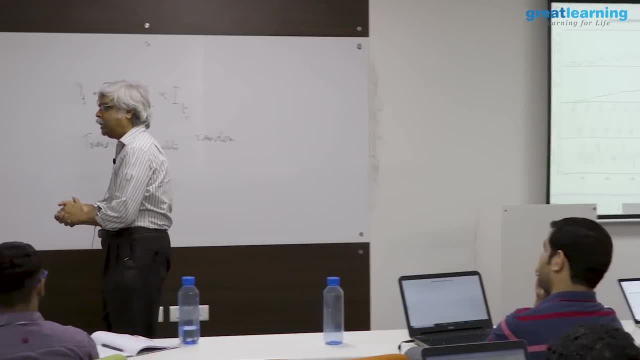 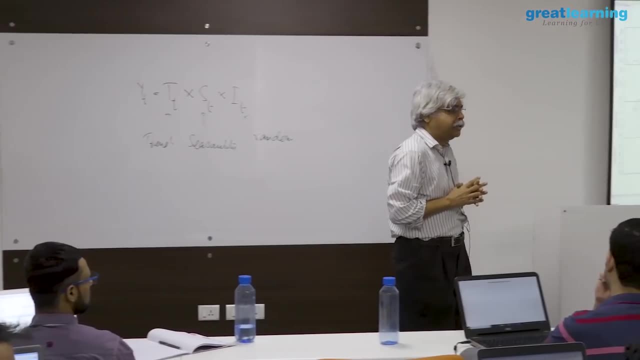 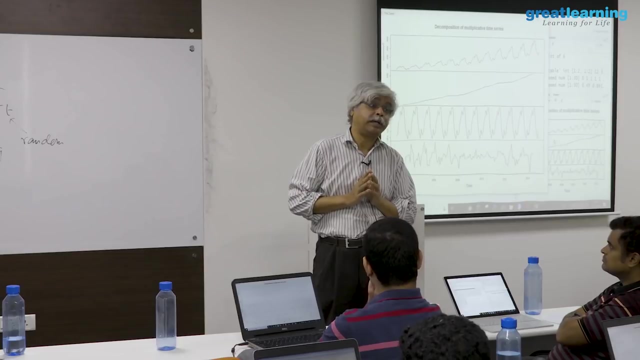 it in and see what happens, which is what inventory management essentially is. so therefore, you're absolutely right, you're bang-on, in other words. so, therefore, the obligation is not to give a point forecast, but to give some kind of plus minus on the forecast, and we will do that by the time we are done on Sundays. 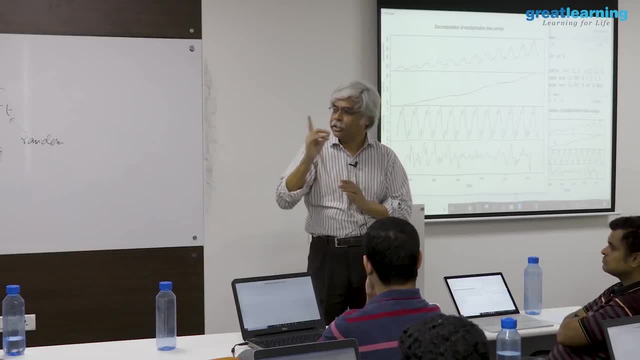 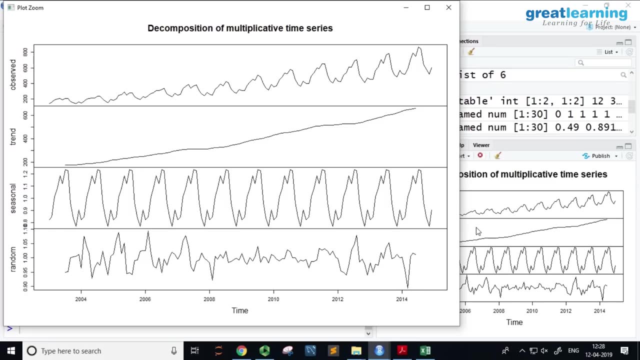 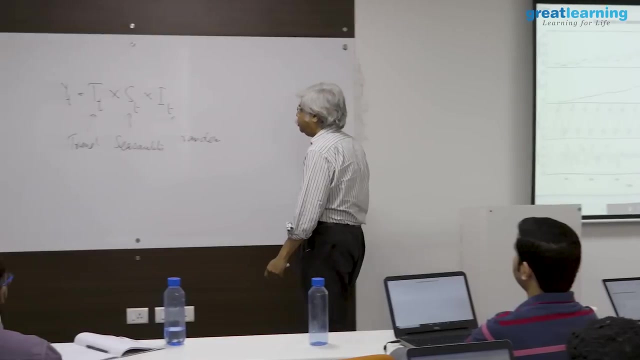 you will see interval forecasts, not just point forecast. you will see upper limits and you'll see lower limits of forecast. yes, ah, okay, okay, okay, so that, so that that complicates things a little more. so some of that is some of that is taking into account when you do inventory management. 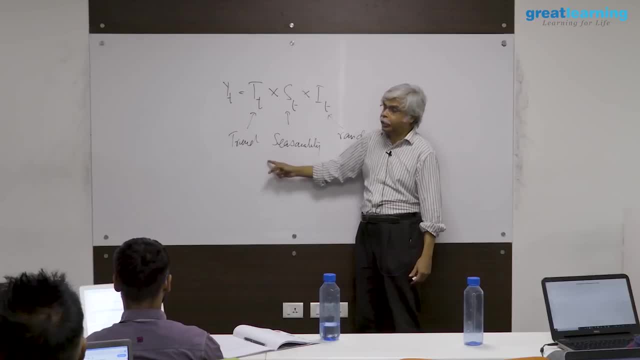 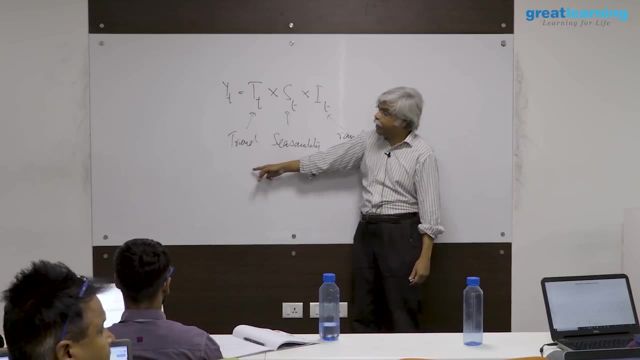 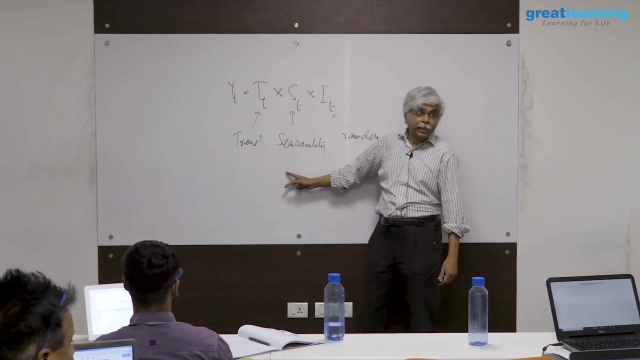 in other words: so when you do inventory management, you depreciate it. in other words, you are making the tractor now, but you're going to sell that tractor in the future. so the rupee value of when you made the tractor and the rupee value when you sell the tractor are going to be different, and so the discounting is. could be done as a depreciated value of this. so so you- those of you who have insurance- probably see this in your insurance. no, not no claim bonuses. your premiums, your basic premiums, your premiums go up or down as the years go by. what should they do? health: you have to go up car premiums like, but no, I'm. talking about an auto insurance, a two-wheeler or a four wheeler insurance. it comes down why: because the value of a decreases, right the value. the value depreciates, so similarly you can depreciate an asset that is not being used to figure this out, but the core question you are asking is a little more. 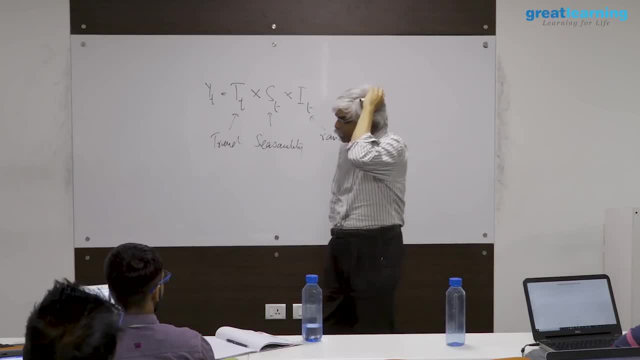 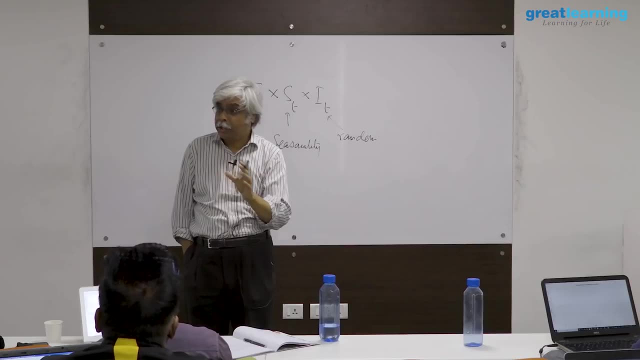 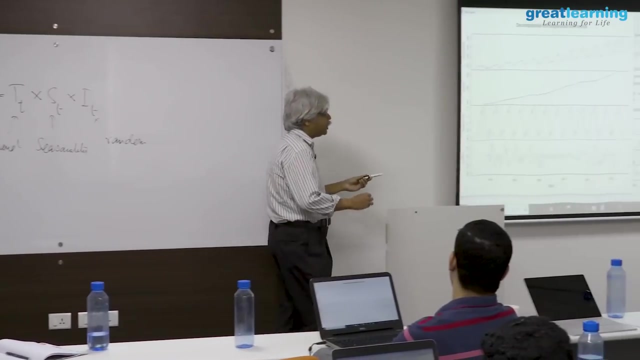 fundamental than that. in other words, if you are unsure as a the value of the of the product itself, ask your finance professor that how it works now. if in our case that probably is, is a small number corresponding to the tractor sales itself, but if that becomes a big number, in other words, if 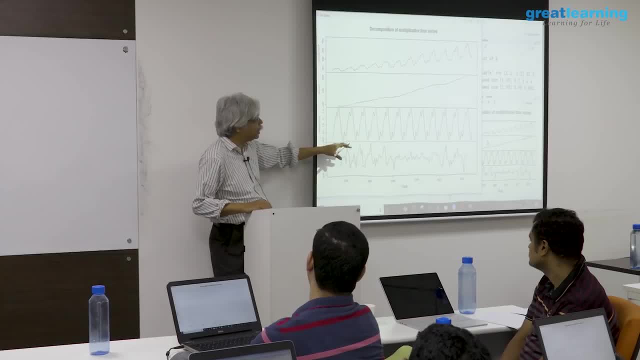 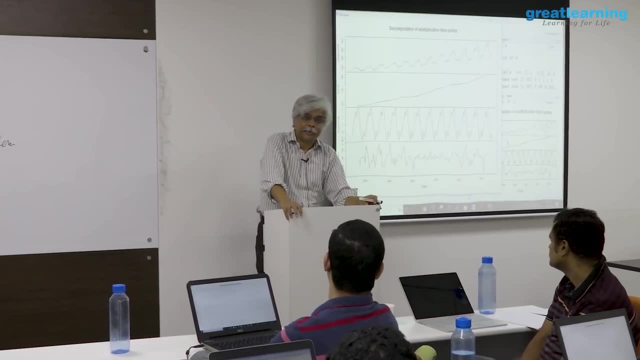 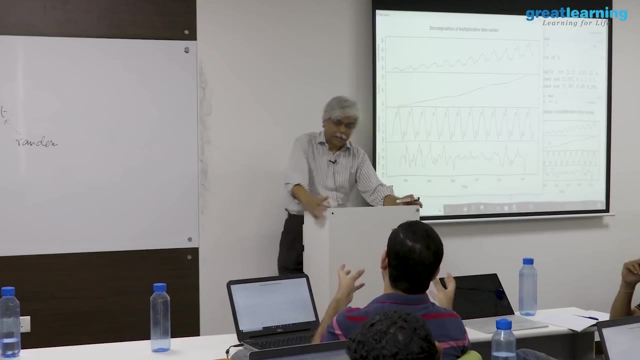 the variation in the product or the variation in the revenues of the product are not due to the sales but but due to the, due to the financial fluctuations of money itself, then, yes, then most serious financial tricks need to be played. try, so, yes, so now. so now the question becomes that, as tractor sales increase, 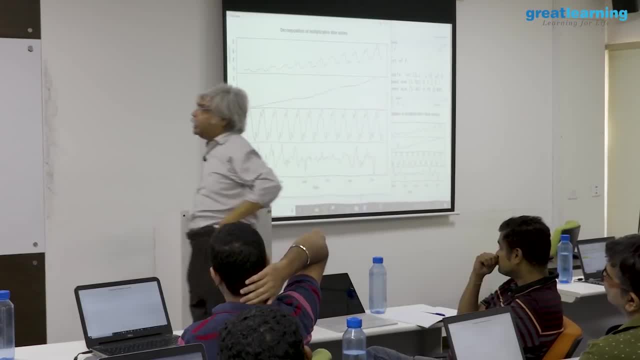 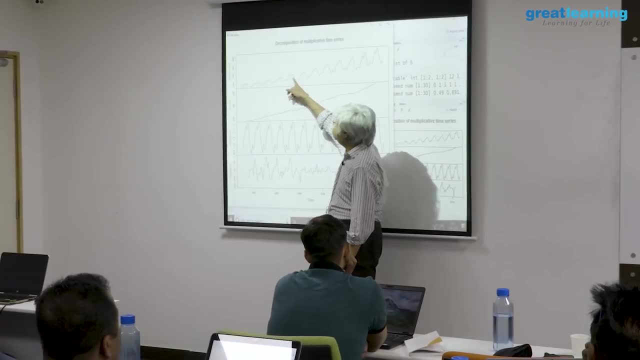 this way. what does to some? what does that do to your business? now, remember that this is sales. now you could argue that this sales has two pieces to it. number one: how many tractors, and then what is the money per tractor, etc. so there are. there are both of these two things. 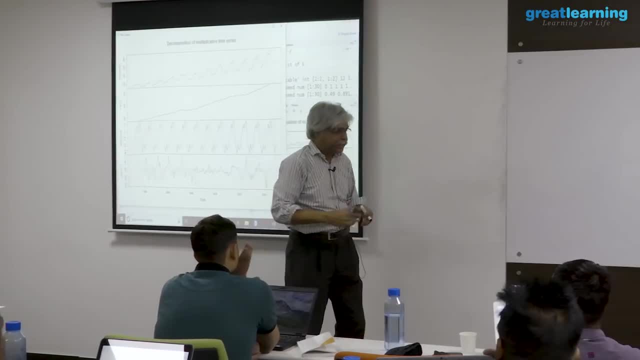 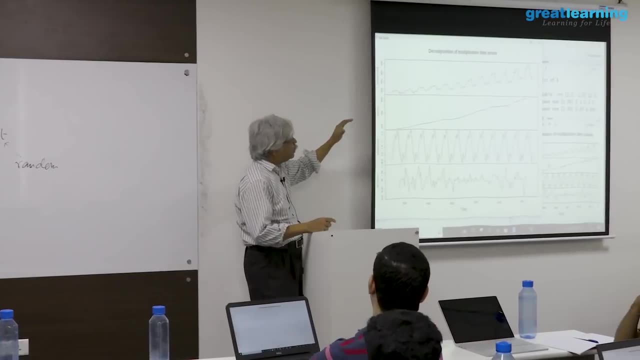 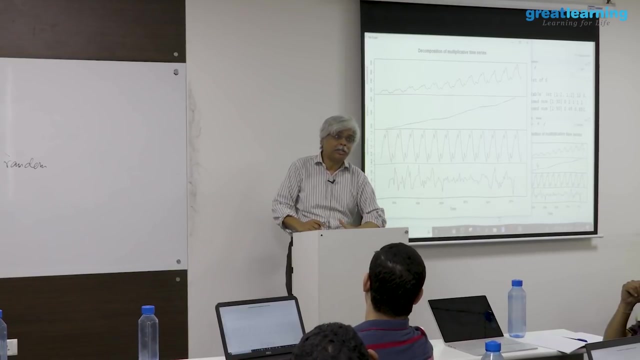 so when businesses grow, they tend to grow in order to be able to adjust for what they expect, the cost and also what they expect money to be in. so in economics of economics have two notions of what growth is. one is called nominal growth and the other is called real growth. nominal growth, essentially, is the 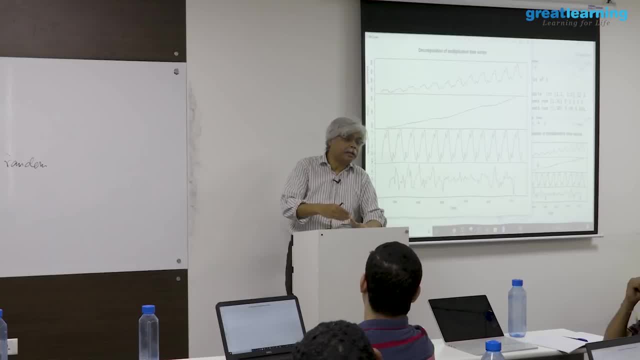 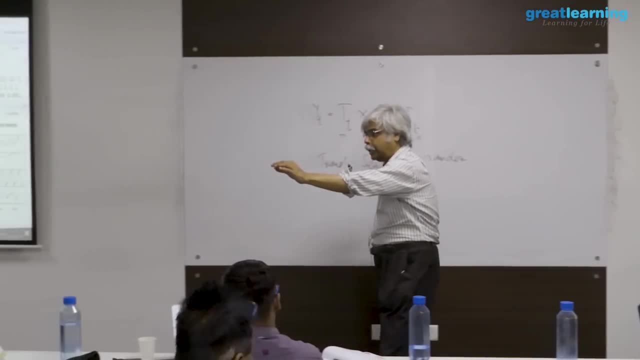 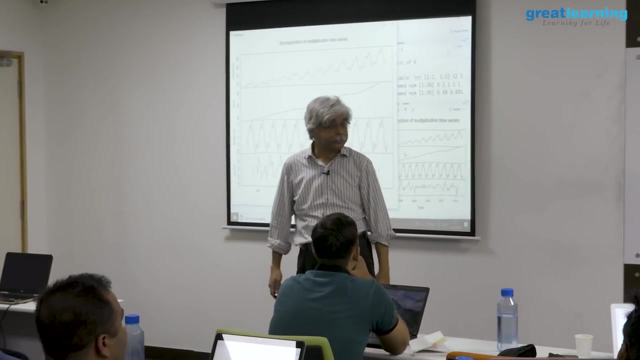 actual growth in money. real growth means is discounts for the cost of money itself. it's little like this. so let's suppose that you, you, you have a raise of, say, 10% and inflation is, let's say, 8%. if your effective raises 2%, the rest is 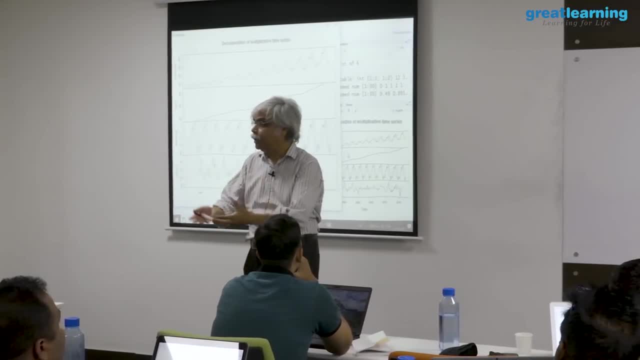 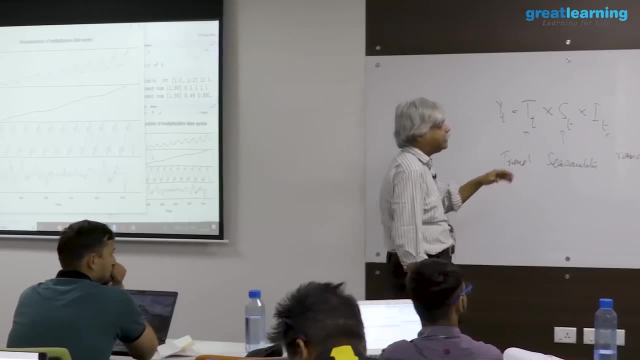 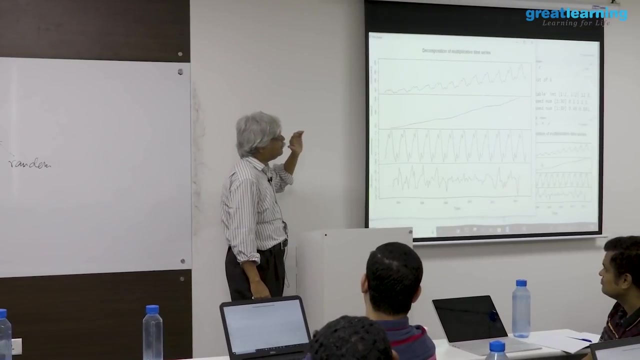 being swallowed up by the, by the inflation, by increase in rent, increase in food prices, etc. etc. so therefore, it so what a business would look at and say that, if I'm looking at sales in some way, what is the nominal growth and what is the real growth? so you could say that if the growth in the agricultural market 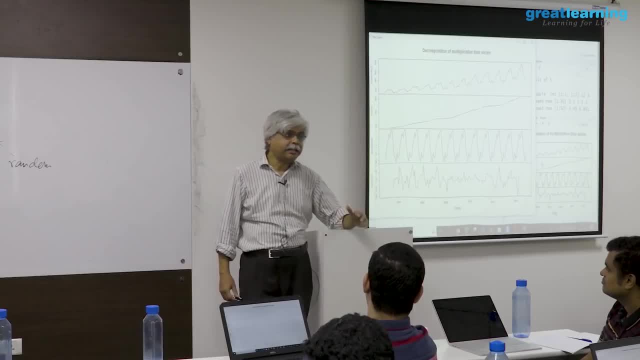 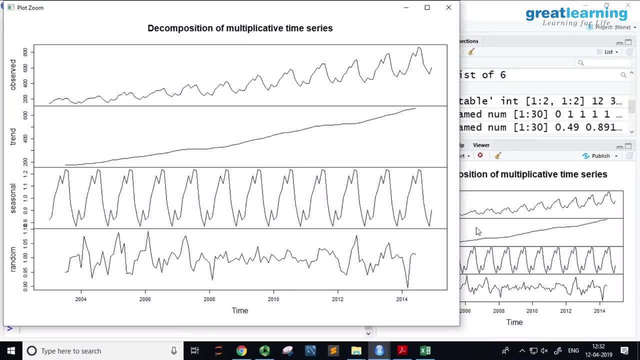 is at 7%, then my tractor sales should at least keep up to that 7%, otherwise I'll be losing market share. yes, that's a different question that I was getting to. that question is not being addressed here. that's a. that's a more. 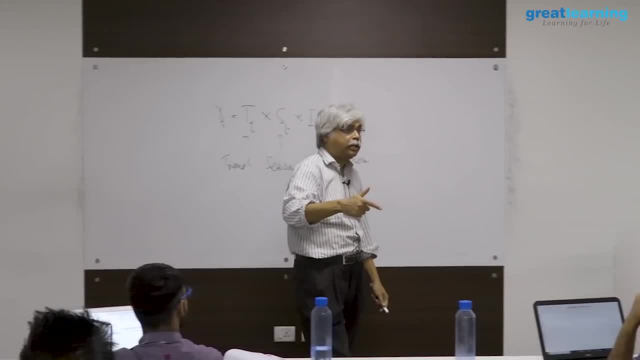 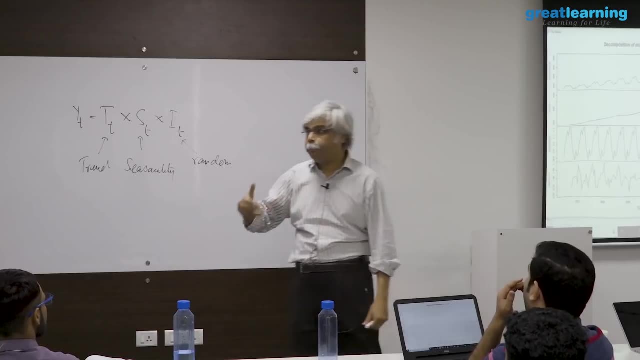 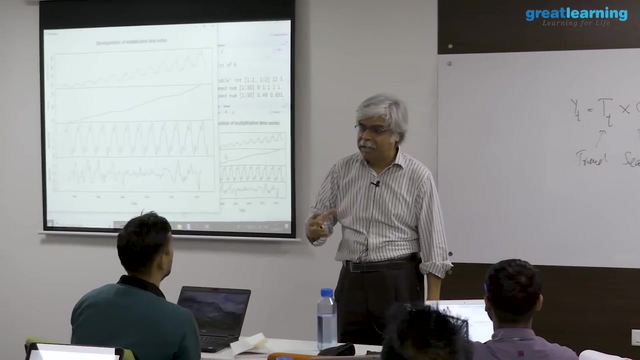 sophisticated question to do. you will do that in the other part of this residency, so ask your marketing person that as well. that when I, when I, when I price something, do i price for to make more money per unit sold or do i price it to sell more units? 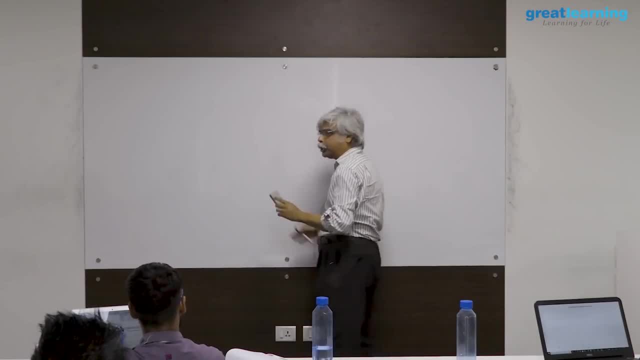 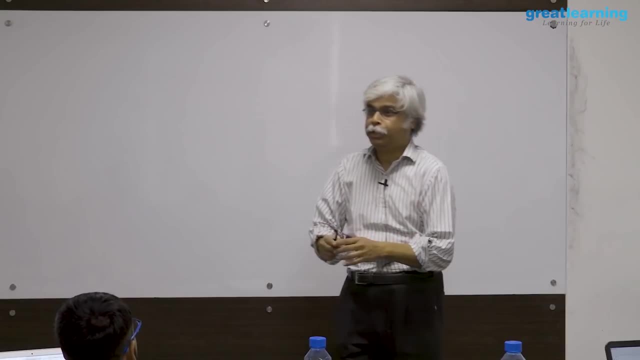 yeah, that's, that's not a time series question, but but this is an interesting question to ask. in other words, to say that that you can think of it mathematically if you want to. some of you, i know, are mathematicians, others hate the subject, but but if you want to maximize, let's say your. 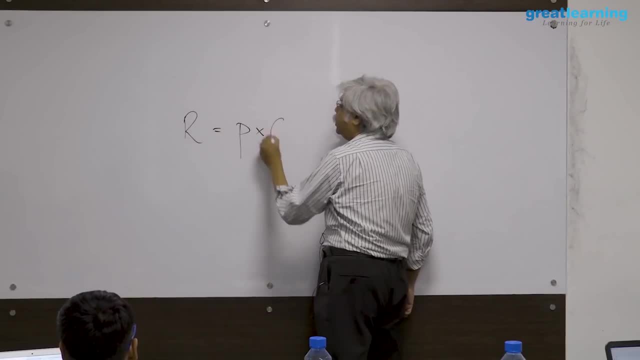 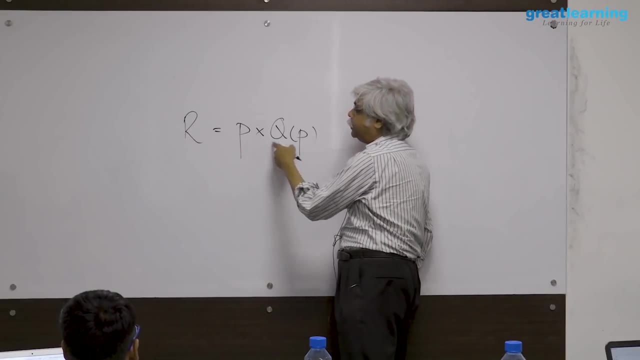 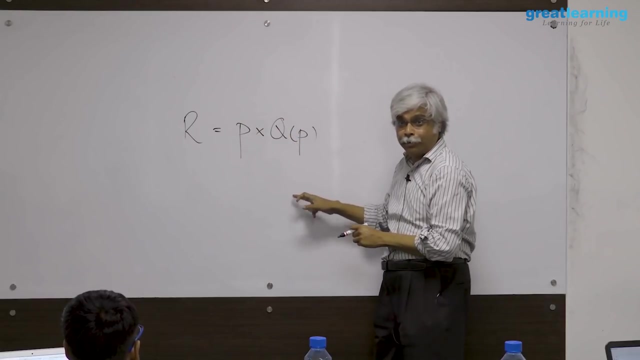 revenue is equal to, let's say, price into, let's say, the quantity. but this quantity is also going to be a function of price. you want to maximize this revenue is equal to price into the quantity. now, as price goes up, this part is going to go up. but this part is going to go down because 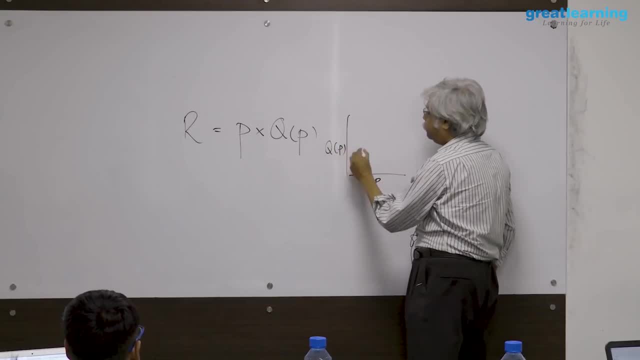 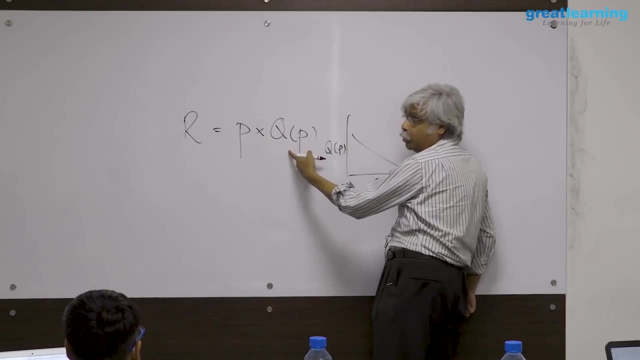 this relationship. this is p and this is q of p, and as price goes up, the amount, the number that you will sell, is going to go down. so as p goes up, this guy goes up and this guy goes down. where is this optimum going to be hit? 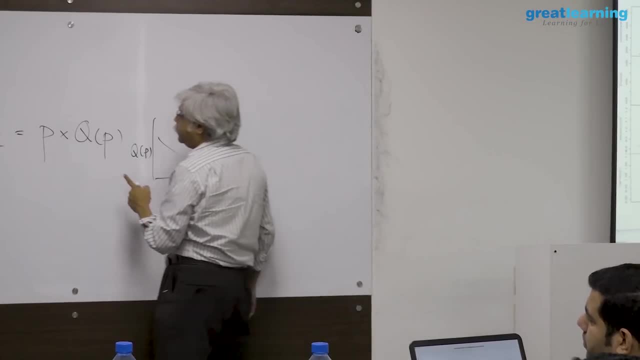 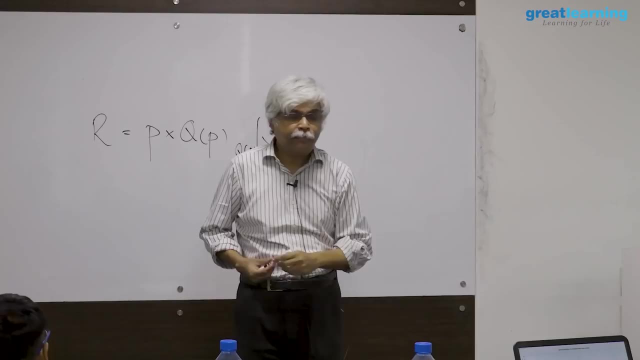 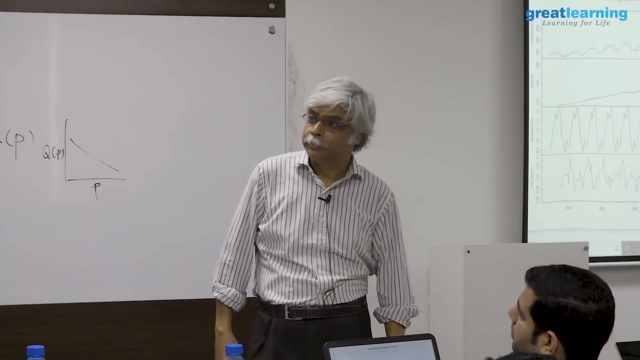 somewhere, right somewhere, where you say that if i make it cheaper, then i'm making too little money per unit sold, but if i make it more expensive, then i'm losing too many customers. there's going to be a sweet spot. true, it's almost never in your control, because this curve is not in your control. 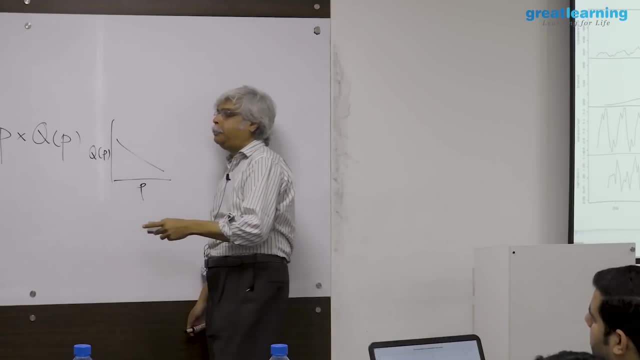 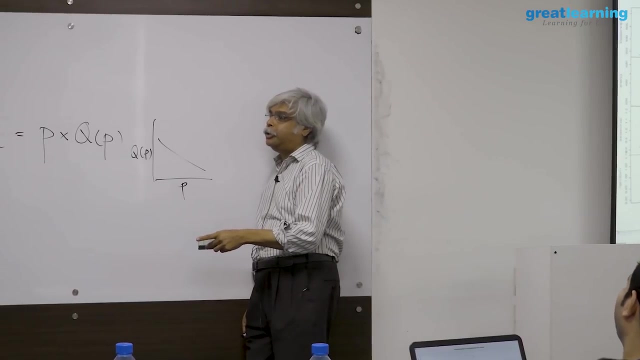 yes, true, you won't um, by the way, i'll make an. i'll make a, make a unnecessary, irrelevant comment at this point in time, but please be patient with me. so, um, have you seen? uh, uh you, if you remember your biology book, in your high school biology book, there is a picture of an animal cell. you don't. 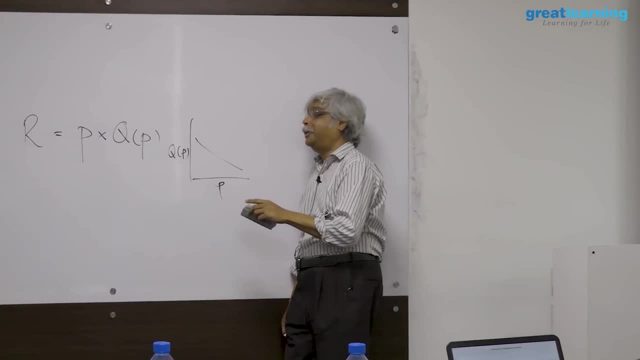 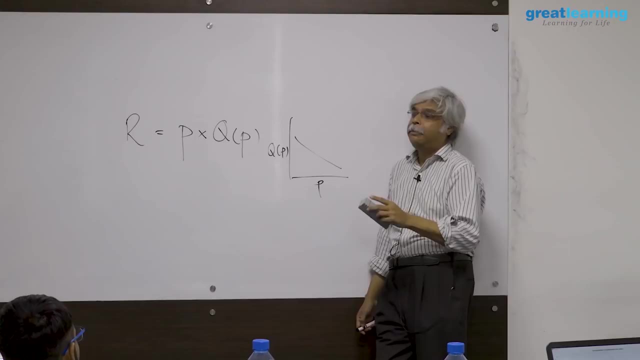 remember what it is, but you remember that such a thing existed, right. so? so now, now here's the catch: no animal, no human, no animal ever in existence ever had a cell that looked like that. that cell is fake. that cell doesn't exist. why not? because in every real animal, including people like you and me, every cell has a very 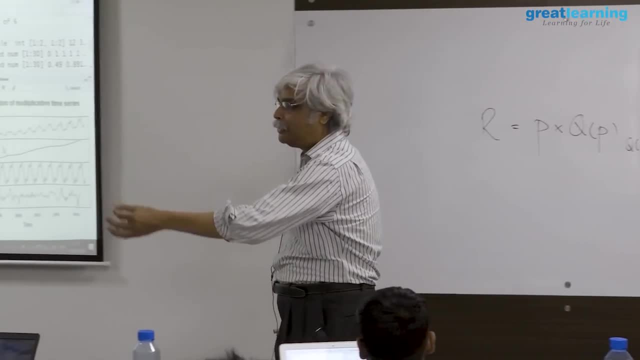 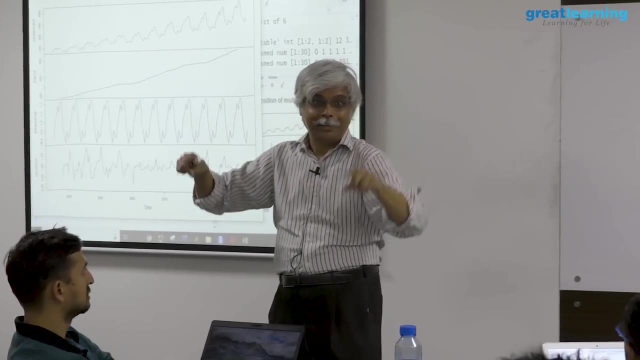 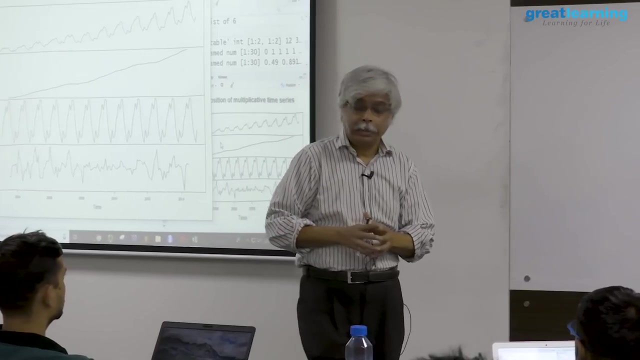 specific function. your red blood cells, for example, carry oxygen. your brain cells carry electricity, so they're shaped like that. your red blood cells have no dna in them. their job is just to pack full with hemoglobin, carry oxygen around. every cell has a job to do, but if you now want to understand, 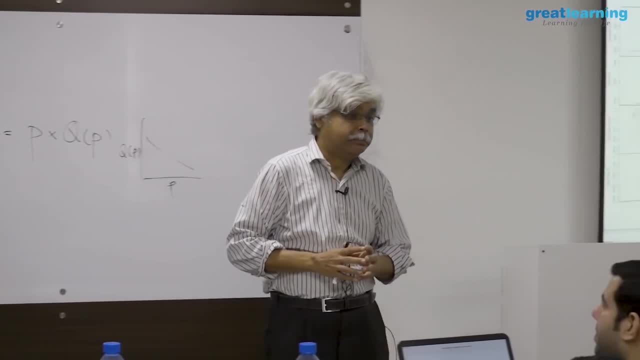 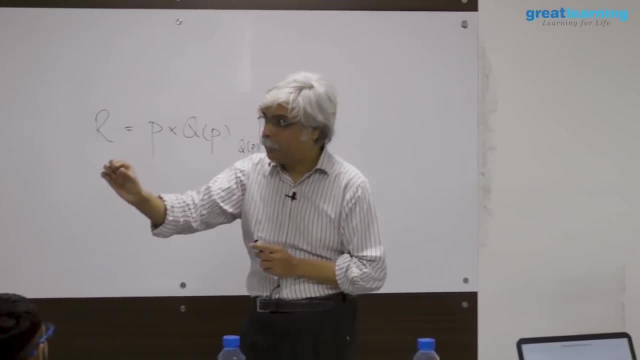 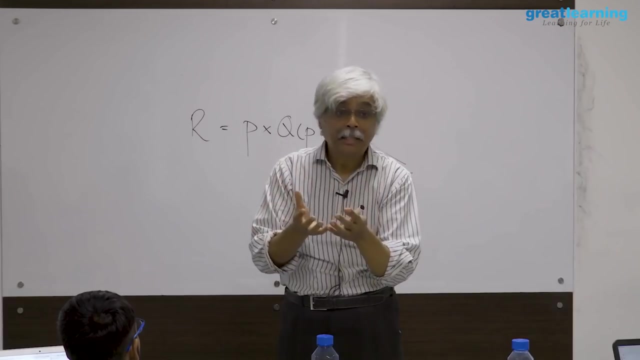 every cell in the human body. all you'll be doing is cell biology, no history, no mughal empire, no other subject. so, to simplify things, what people do is people take more the most common elements of all the cells, put it together and make a fake cell and say that if you understand this cell, 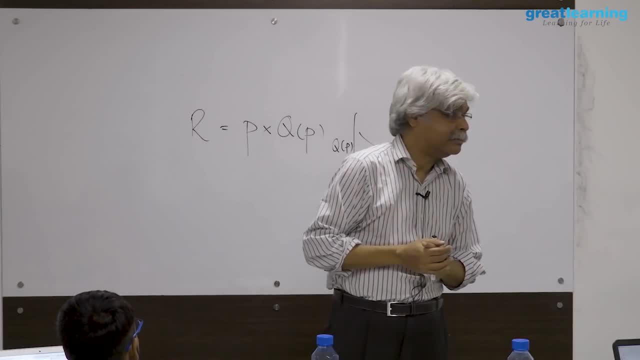 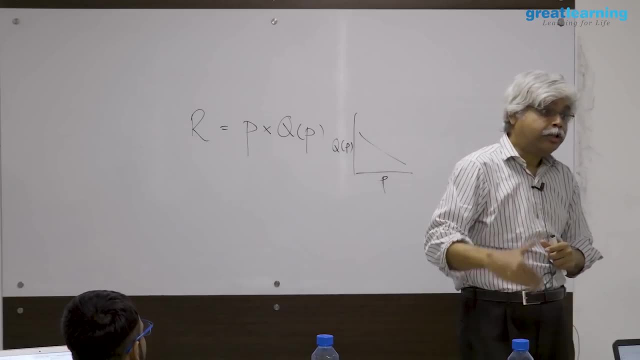 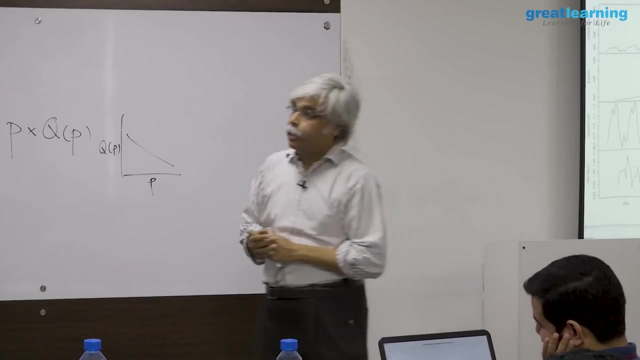 you will be understanding ninety percent of the function of ninety percent of the cells, but no cell looks like this correct. the training that you receive looks like the animal cell right. ninety percent of projects will have ninety percent of the material covered in this, but no actual project like what you are. 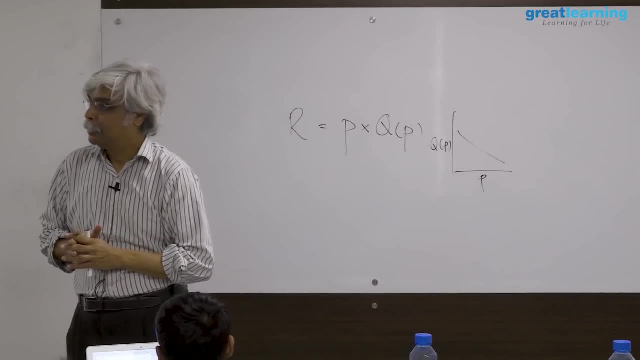 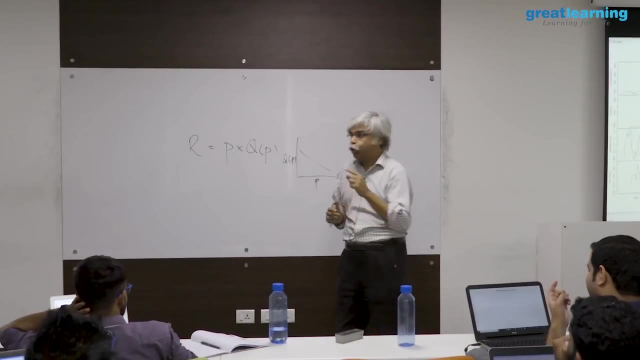 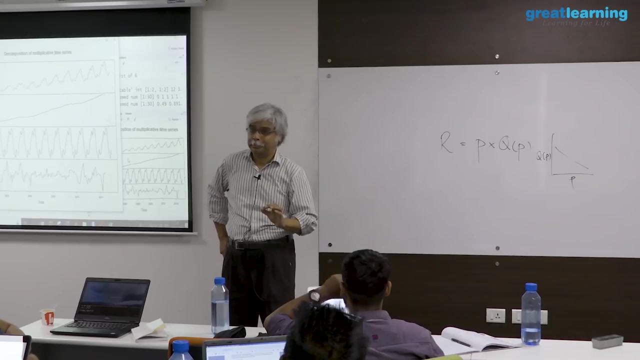 describing will be covered. now, what is the solution to this? the solution to this is to take the project and then to say that, for this project, what are the elements of the theoretical cell that I need? and take a little bit of optimization, take a little bit of forecasting, take a little bit of 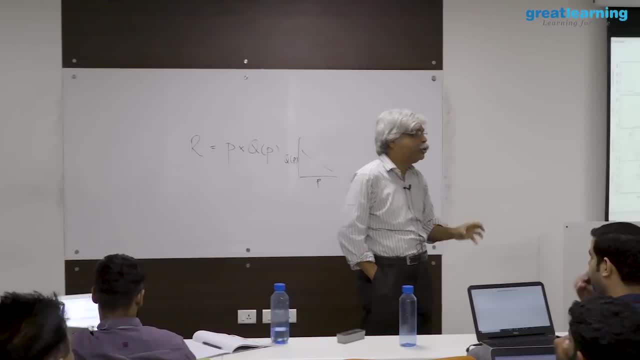 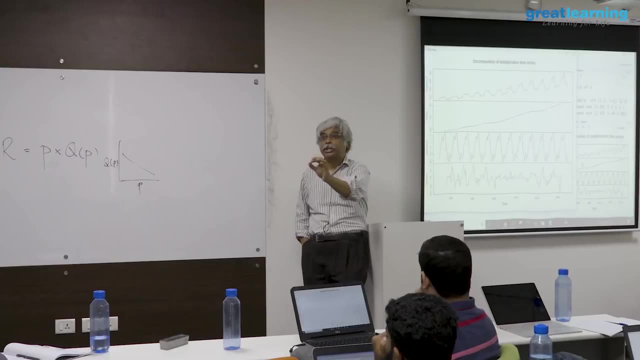 regression. take a little bit of principal components, take a little bit of all of that and string it together. now, most of us find that very, very hard. so what we typically do is we begin the project using one core technology and we say: this is essentially a supervised learning problem or this is essentially 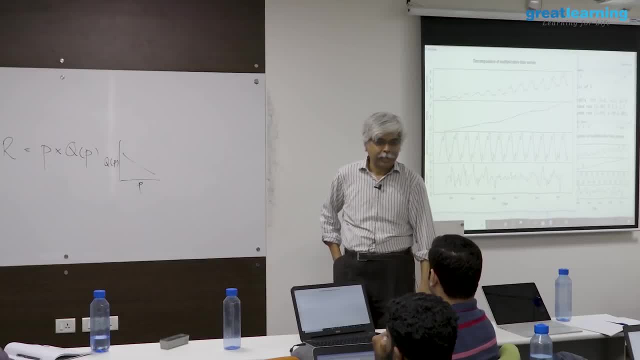 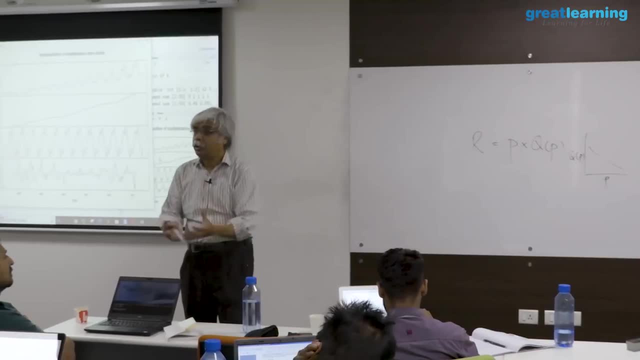 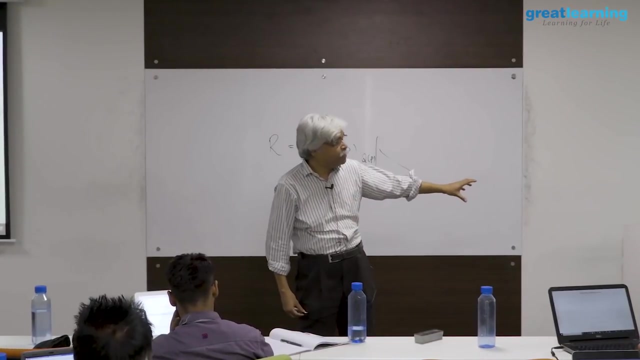 an optimization problem. this is essentially a forecasting problem. and then we say: but there are pieces in it that I don't know what to do with. so, for example, I'm trying to understand pricing and I'm trying to forecast pricing. now, part of that is certainly understanding what prices have been like, but a part of that is also for 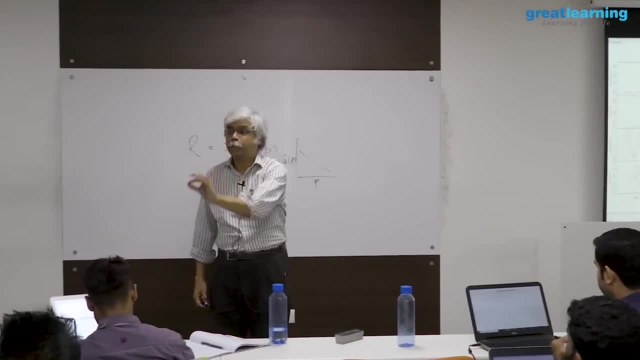 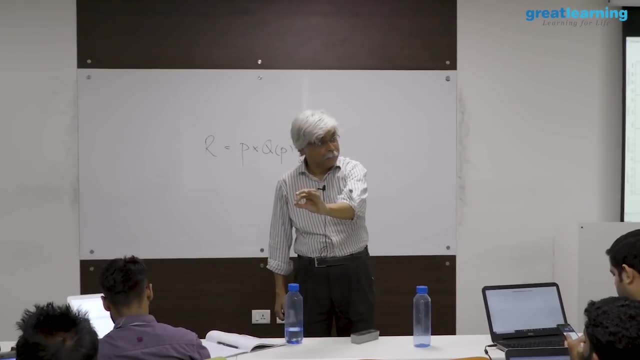 example, understanding what that has to do with the set comparators price, what that has to do with your costs, what that has to do with the value of money that you have, that you, that you would accrue or not accrue based on this spending. so all 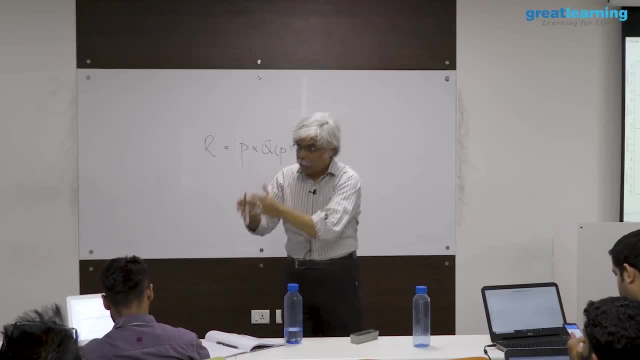 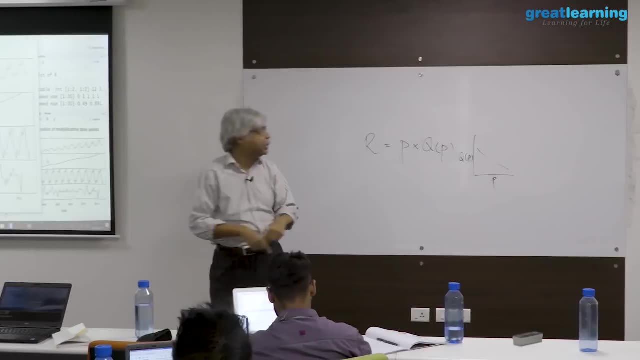 these different pieces need to fit in, and how you will do that depends on different techniques. so, for example, you could say that I am going to do a linear regression analysis to try and understand this curve. so I'm going to see if this is the price and how many people are expected to buy do that curve. 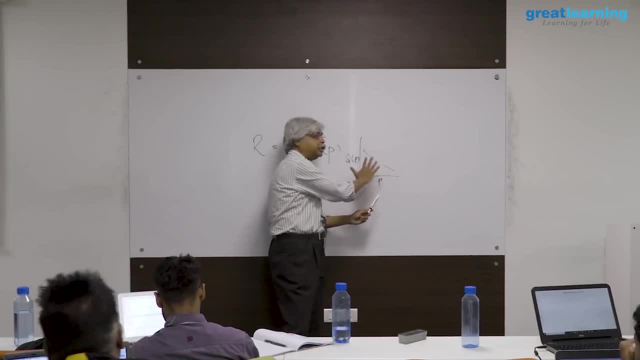 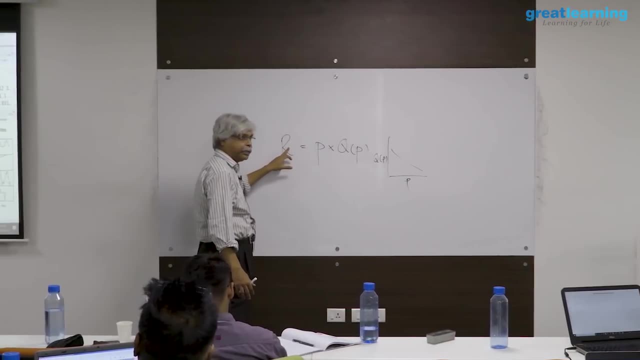 fit a straight line, and you might do that in marketing and do a regression analysis to understand relationship of this kind. you can do an optimization exercise and put that in somewhere here and therefore understand what happens to this highest speed, and then you might go ahead and test it in a particular time when you want it toHH. but then also, what a very good table is is you could say there's better performance. 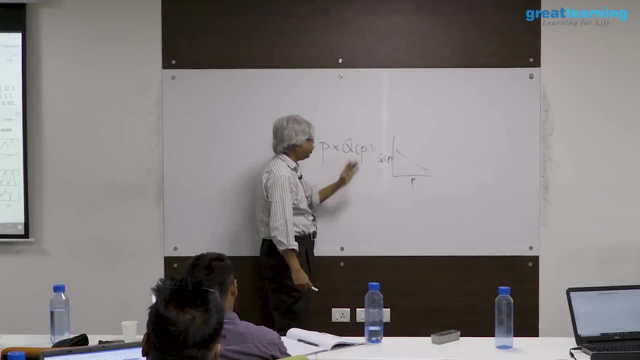 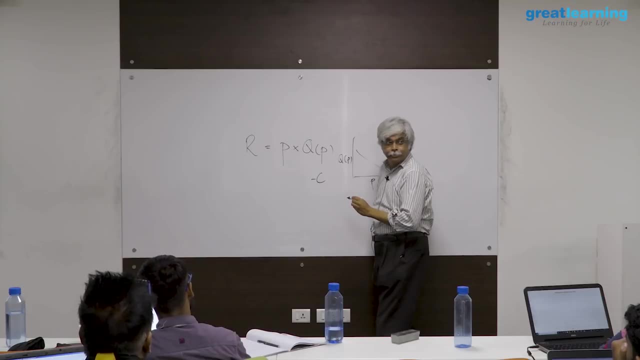 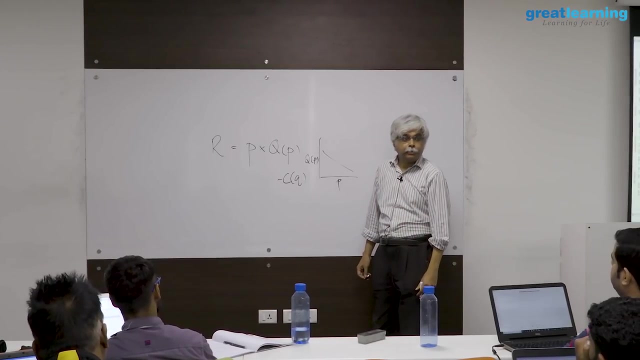 might say: but you know what? I'm not interested in this at all. I'm interested in this guy, which is my revenue minus some kind of cost, and the cost strangely depends upon Q, which is how many I make, which is this object here. so again, now this comes into the picture and you say: 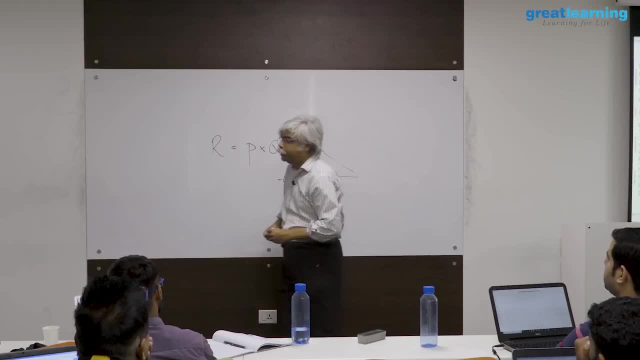 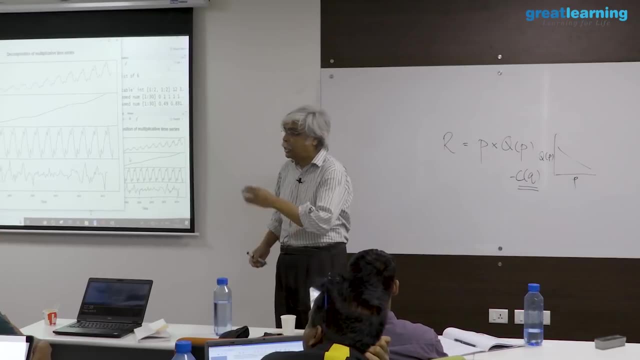 now, how do I understand what this cost is? so now you'll say: how do I do that? so I'll say: what are the factors that go into the cost and what happens and how is that evolving? and you say: the factors that are going into my cost are now: 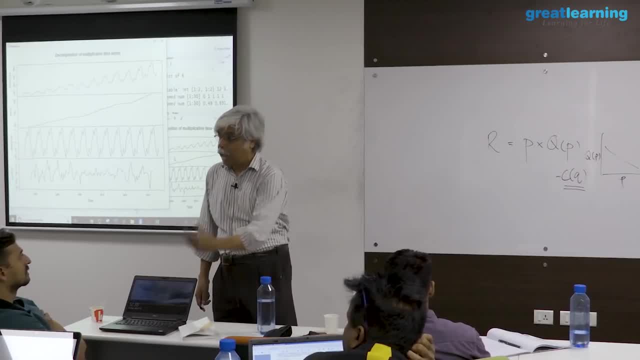 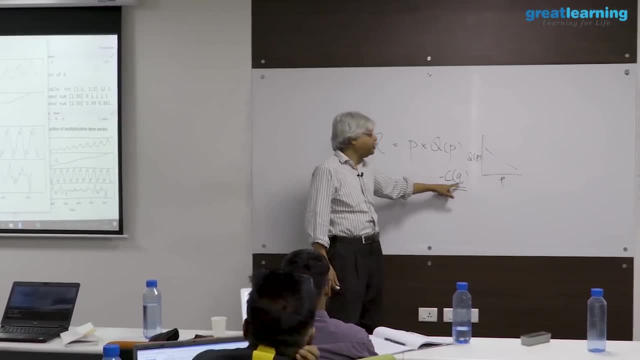 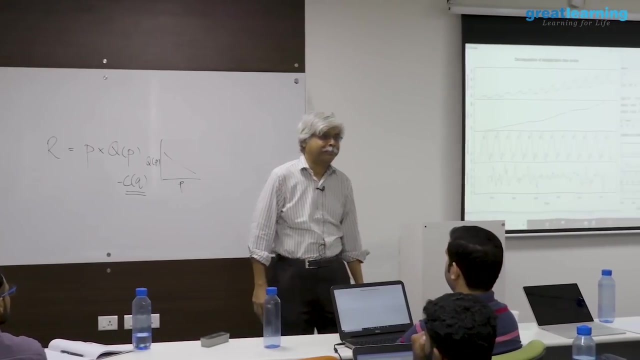 changing in time, things are becoming more expensive. so now my problem becomes: I need to forecast cost. that becomes a time series problem. so you got regression sitting here, you got optimization sitting here, you got time series sitting here and you create your own cell, realistic cell, something that 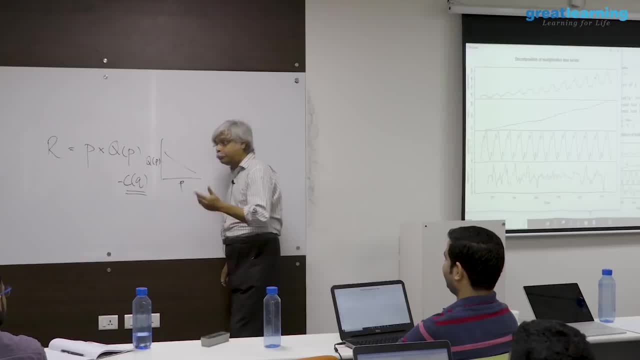 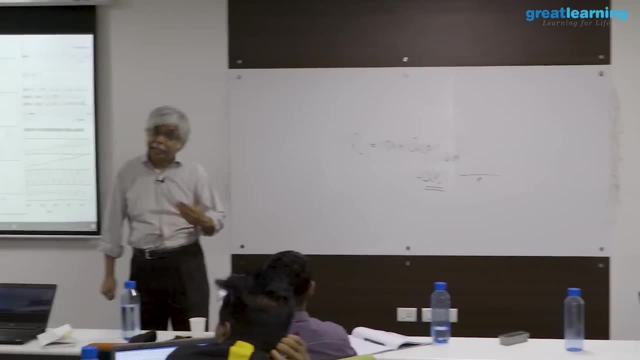 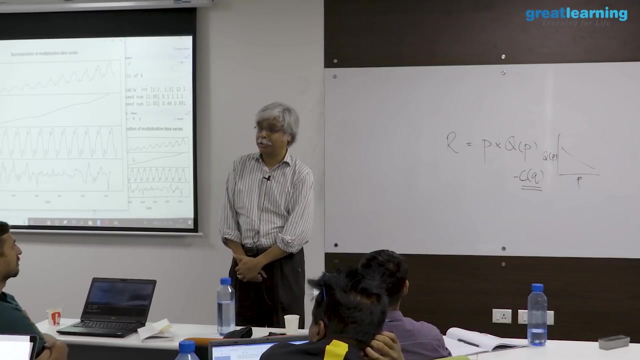 makes sense for you. you, that is what your capstone project is supposed to give you training on how to do that. but it gets hard, but it also gets interesting. it also gets interesting- medicine in some ways more interesting than biology. so it gets a little more interesting when you get that and you. 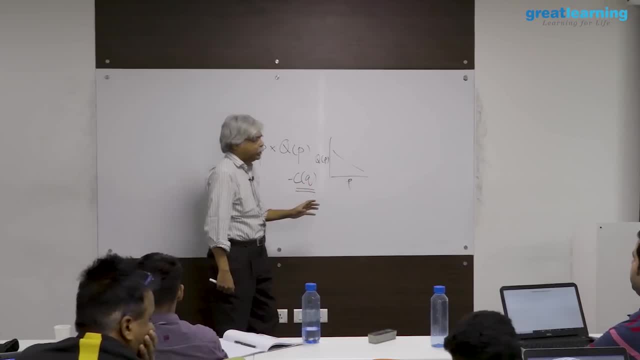 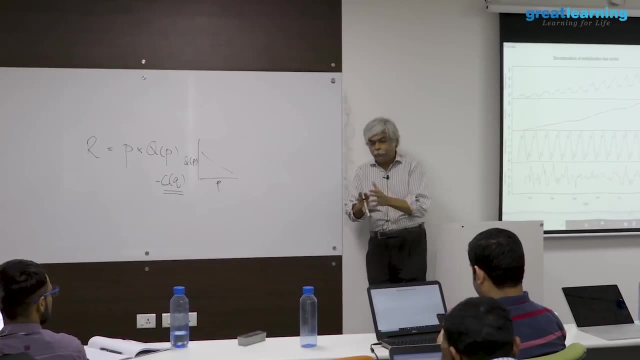 figure that out, and that is, to some extent, where your value proposition comes in. so once you've nailed it down, you now say that therefore, it is important, separate from everything else, for me to be able to predict costs. if I can predict costs, then I can put that into other things. 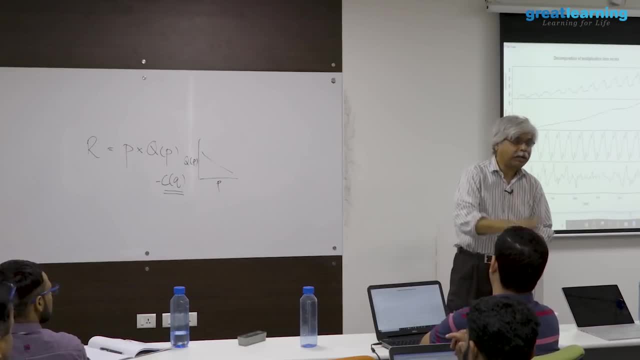 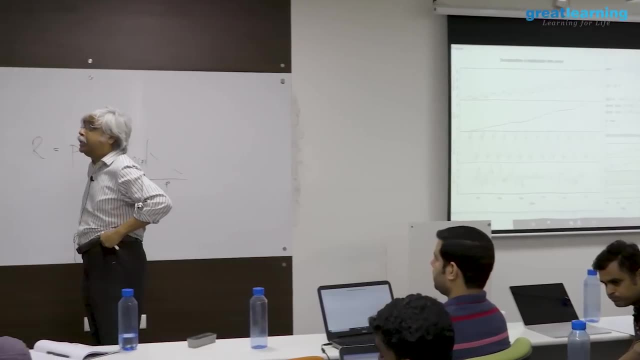 and now you say: now, how should I predict costs? what aspects of cost is relevant? so now you can go back and say, but you know what? the most important aspect of my cost is this thing that I am importing. and you say now, why is that a problem? 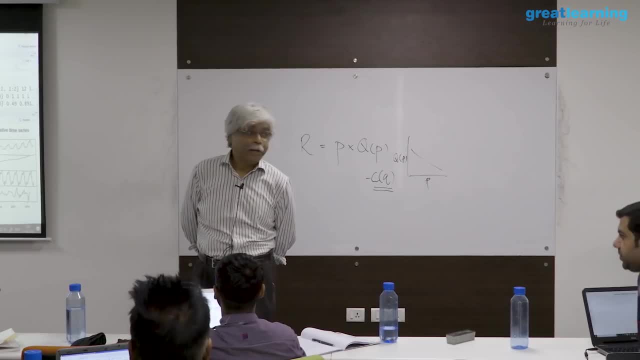 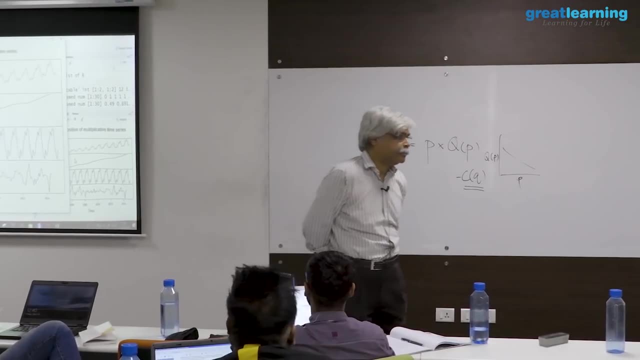 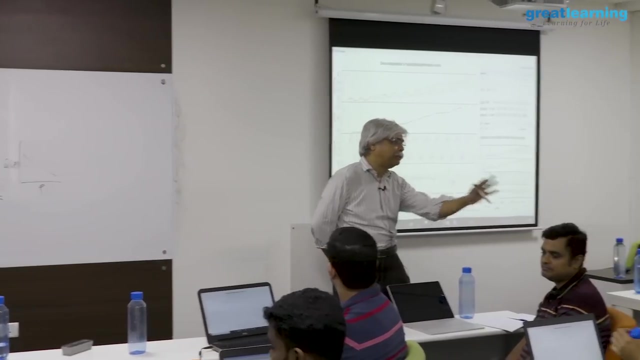 because my foreign exchange is out of control and I don't know what my foreign exchange is. so now you simplified your problem. you said I'm not predicting costs, I'm predicting Forex, because if I know Forex I'll be able to calculate most of my costs. the rest of the cost is in my 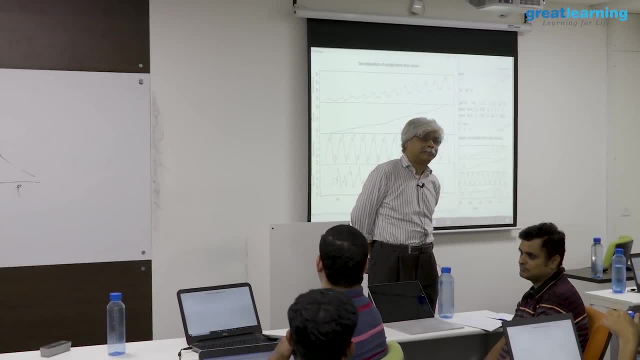 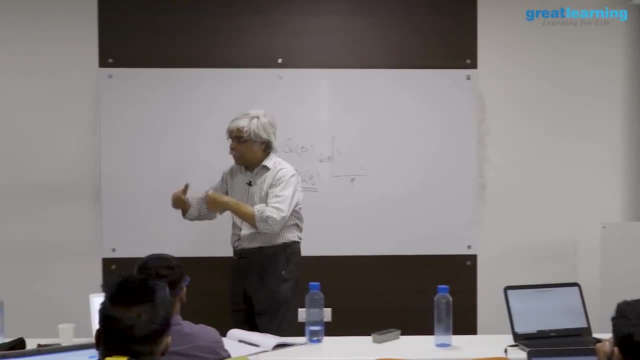 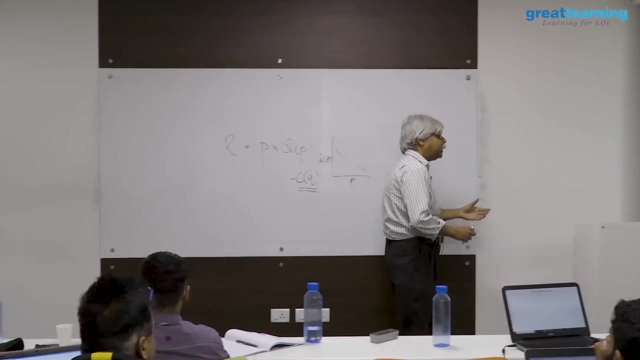 control local when vendors or Jagger, but the import market and the forex market I have very little control over, so you chip away at it and then you, true, but they need to, but they need, but they need to know to some extent what the cost is and 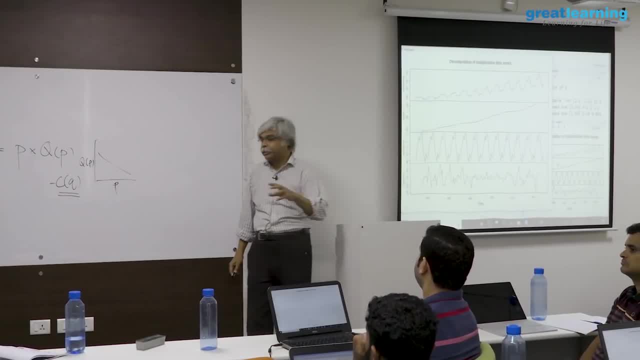 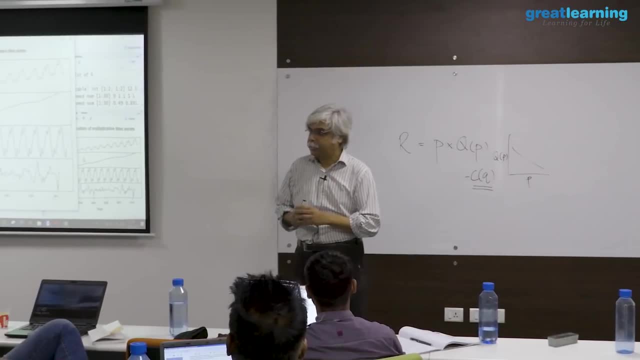 what to do, and that's your job. so, for example, there's a story of an engineer, who was, who was once called in to look at a turbine and the turbine was not working, so the engineer was brought in. he was brought in as a consultant and he 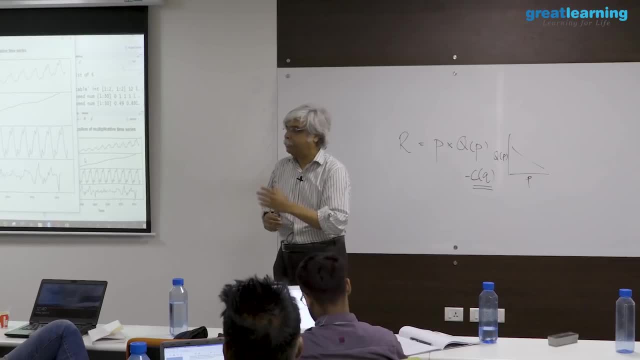 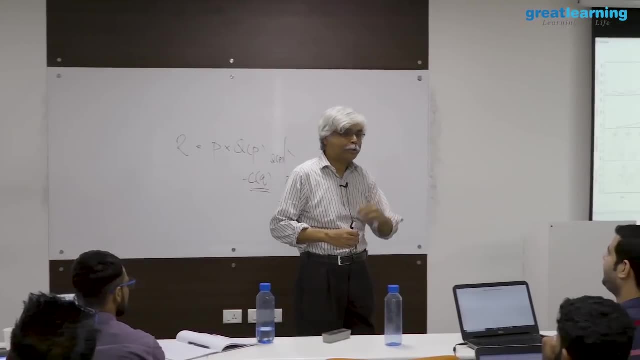 looked and he knocked at the turbine, etc, etc. and then he went away and he gave a bill for a thousand dollars and the manager of the flam said: what thousand dollars? he didn't come and do anything, he knocked it. so he said, he said, he said: so I'm give me a breakdown. 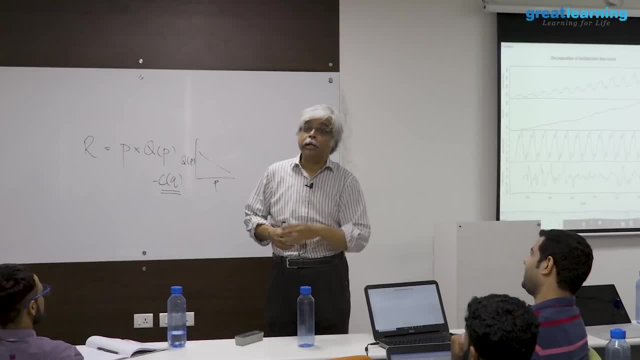 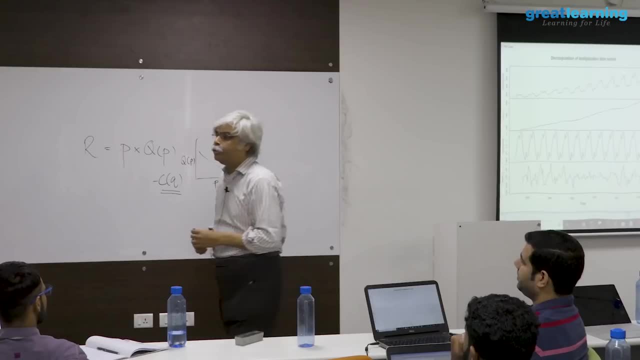 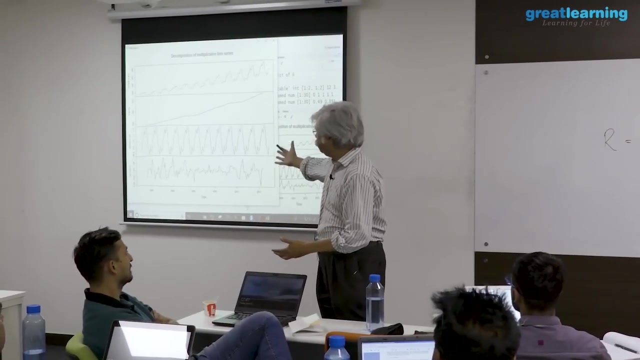 so I'll give you a breakdown: one dollar for knocking on the turbine, $999 for knowing way to knock on the turbine. your job is to know what analysis to do. the analysis itself is, as you can see, one line of code. even a more unlike me can do it. there's not hard. the hard part. 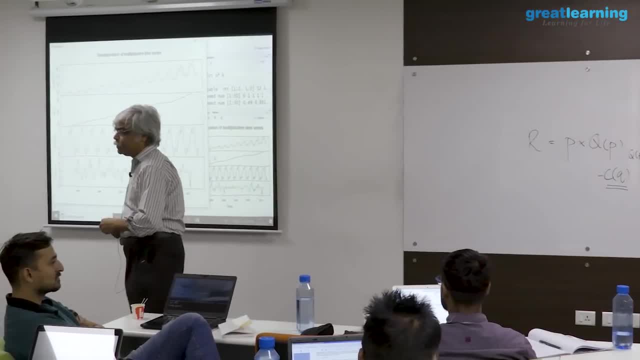 is knowing. this is the analysis that needs to happen. things like our and things like Excel, then make it a very easy exercise so that you don't get stuck in the programming and you can look it up from a book or look it up from, etc. and so on. 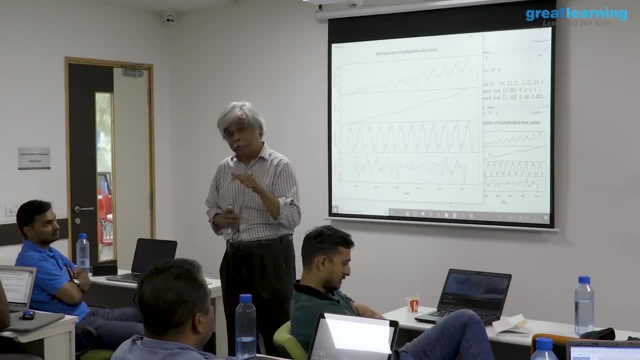 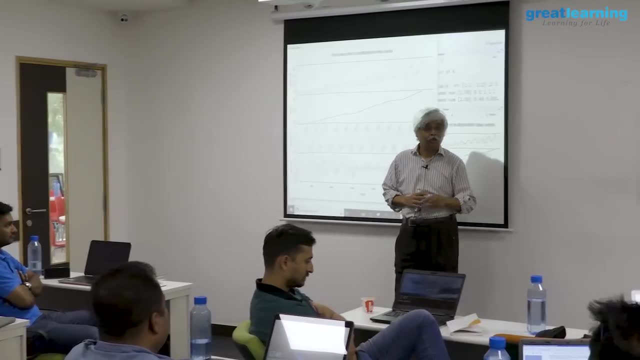 That's not the skill that we are looking for. That's not the skill you are looking for. You are looking for to know: Your skill is not to do a decomposition. Your skill is to know that a decomposition is what you should do. 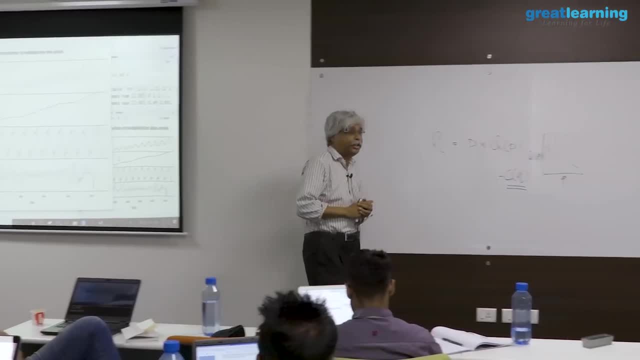 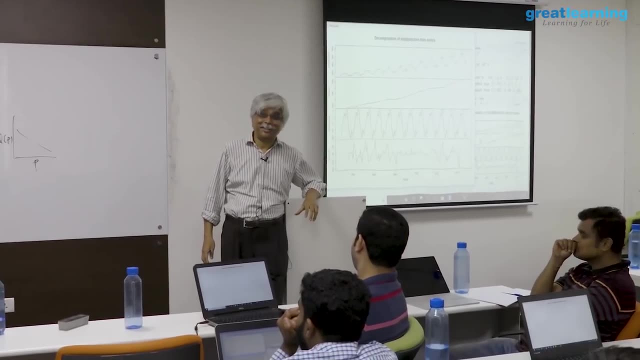 Which is a different skill to have and an interesting skill to have. So very good question, But it's a part of a much bigger story That I hope I don't have to answer for you. Yeah, What do I infer from the random part? 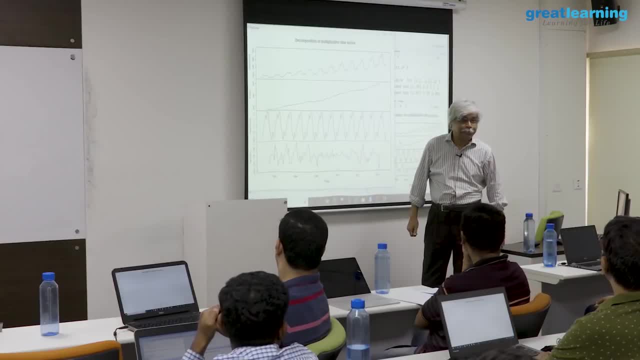 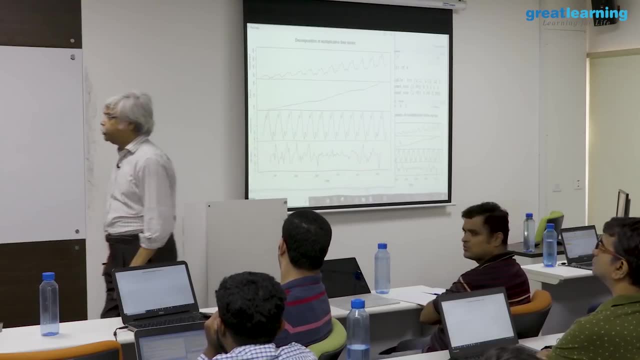 What I should infer from the random part is that there is nothing there, In other words, there is no pattern there. I think one of you was asking a question in the break, I think you were, So one way of doing this is to say: is there something there? 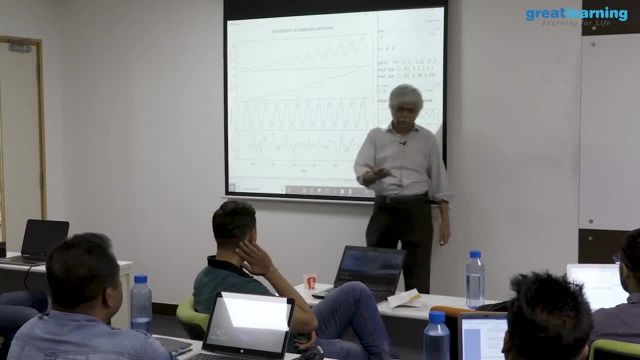 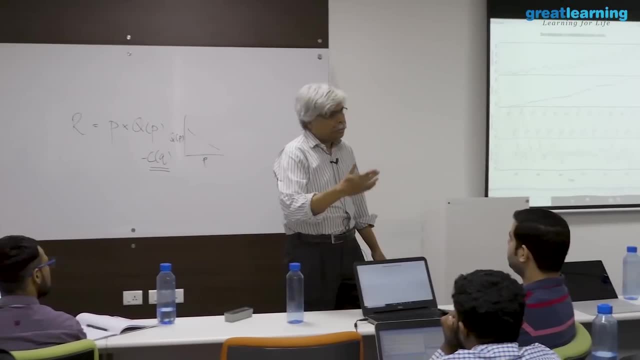 And so is there a pattern there, Is there seasonality there, And so early on today, when I give presentations, I give presentations using computers and maybe PowerPoint or something like that 20 years ago, 25 years ago, 30 years ago. 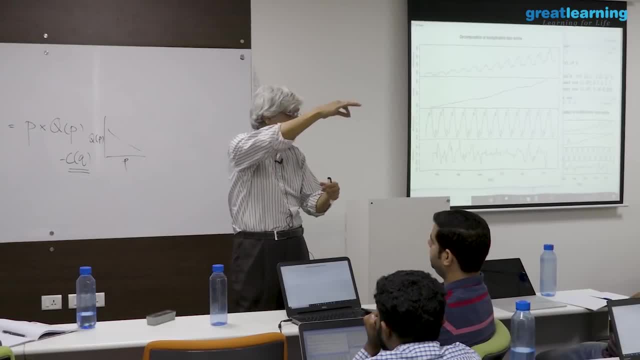 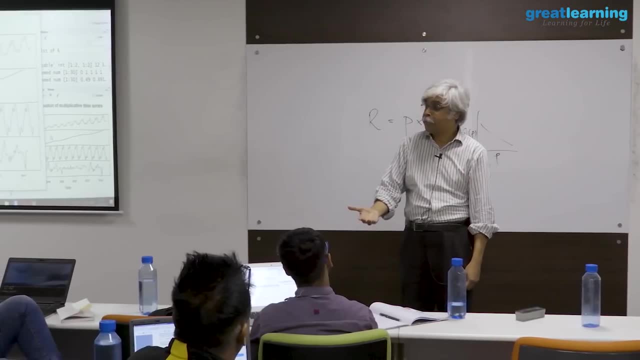 when you were giving presentations, you would give it on transparencies. You know what transparencies is. It's a little film And you'd put it on a projector, Light would shine, et cetera, And so then we would often have what's called a transparency test for time series. 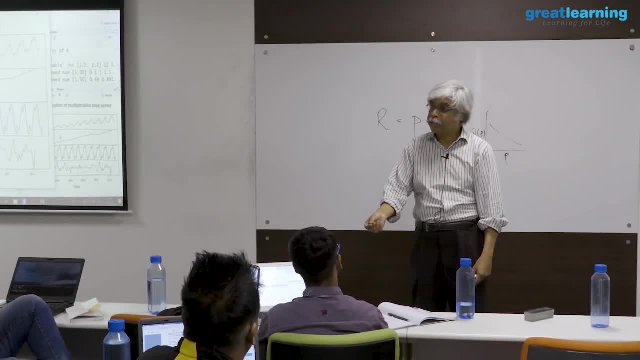 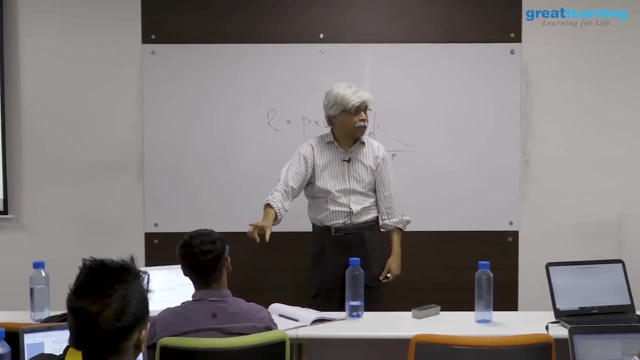 In other words, you plotted a time series on a transparency And let's suppose you've taken the transparency and you flipped it over, And now you're seeing the time not from front to back but from back to front, And the question often asked is: can you tell which is which? 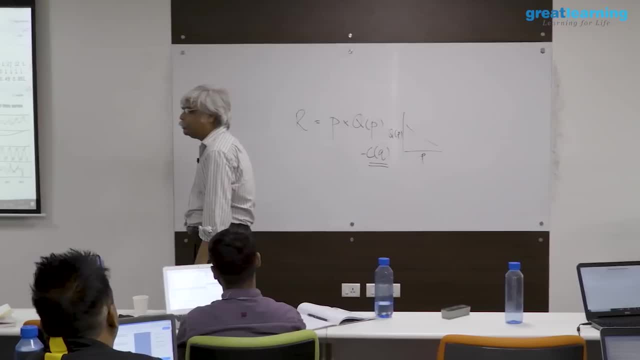 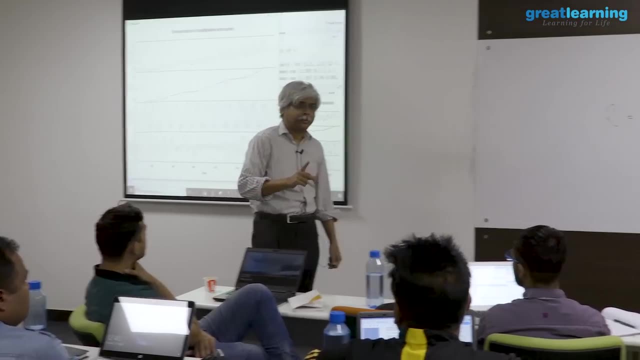 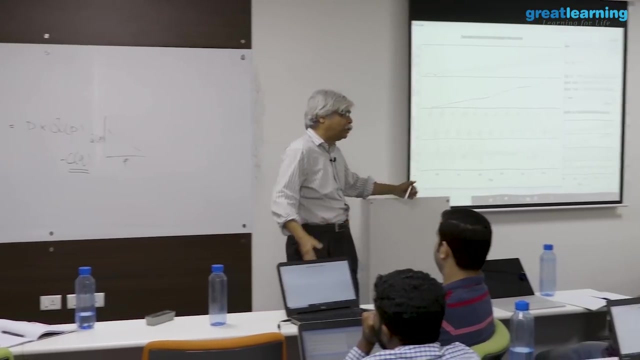 Can you tell which was the forward series and which was the backward series? If the answer is you cannot, then what you have is an irregular pattern. In other words, there's something in which all structure has been lost. And if all structure has been lost, it looks the same whether you read it from left to right or right to left. 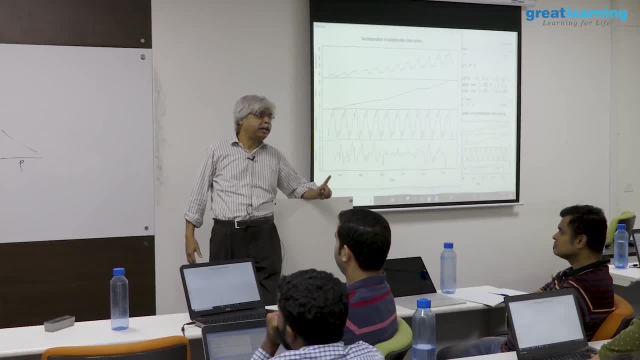 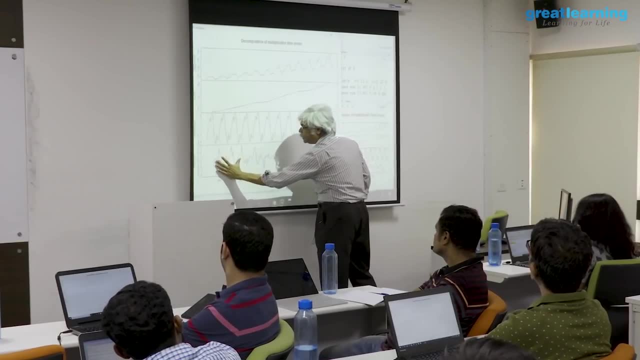 We'll deal with that concept again on Sunday. It'll be called stationarity. It means that every part of the series looks the same, whether it's on the left, whether it's on the right. So this part of the series looks the same as this part of the series. 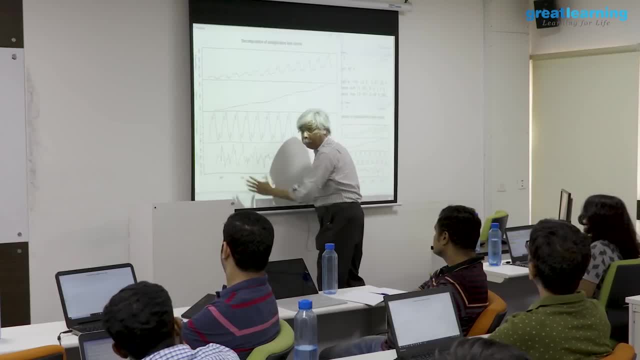 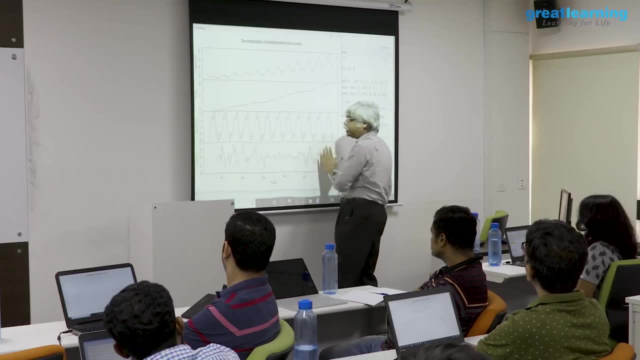 Now you'll say, no, it doesn't. This part looks flat and this part looks bumpy, But that has nothing to do with the fact that this is the beginning and this is the end. Is that what it is at random? and that's what it is at random? 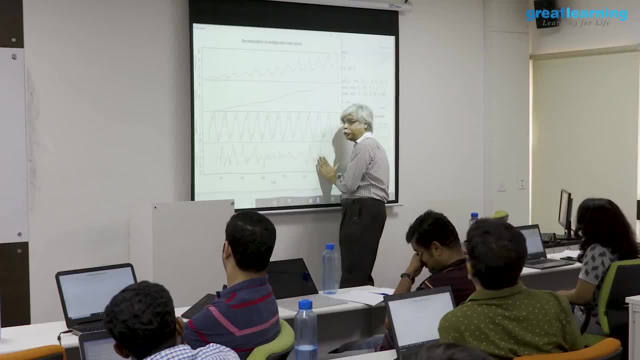 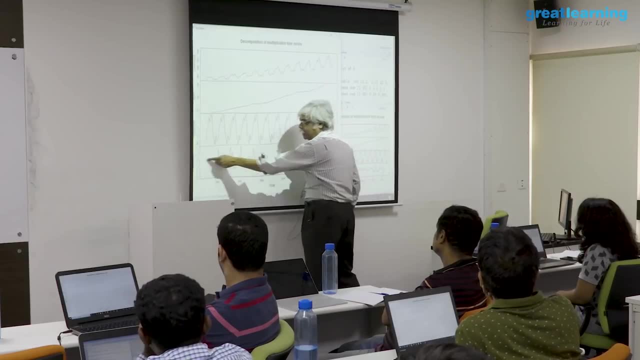 And you do not know whether this one will be high and this one will be bumpy or not. So the whole point of this is that the only thing you can extract from it is its width and its middle value. You cannot extract a pattern from this. 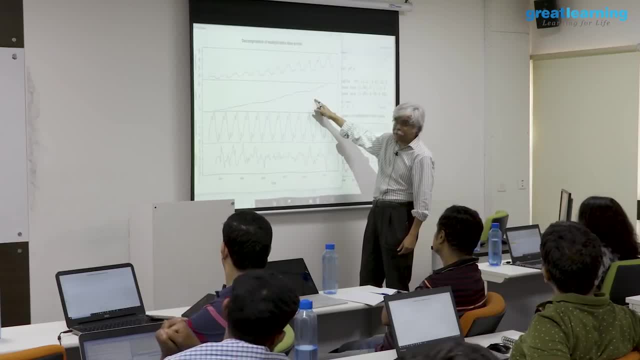 If you could extract a pattern from this, you can put it here. or you can put it here Or you can build. This is the most sophisticated model, Saying I'll have another parameter, I'll have a cyclic parameter or I'll have something else. 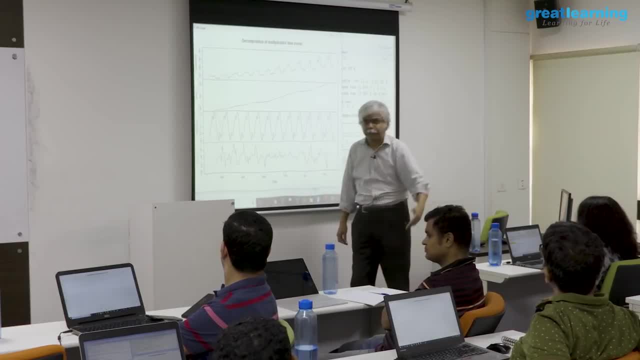 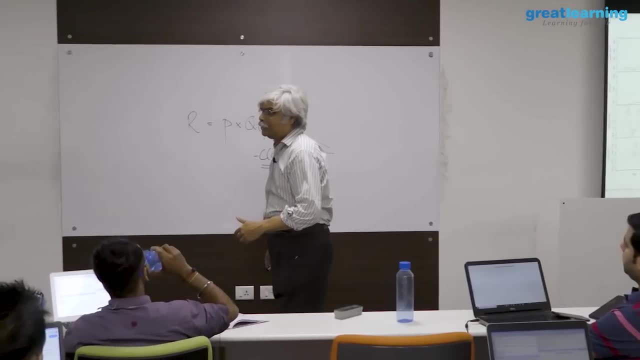 You can keep adding structure to it, Keep adding details to it And saying no tractor sales. you know there are these other factors And I'll say, okay, give me the data for it: Agricultural demand or something of that sort. 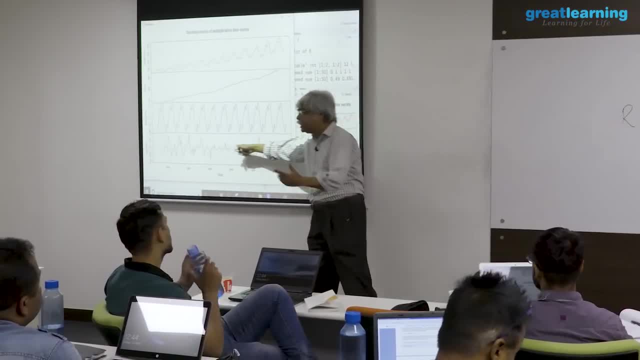 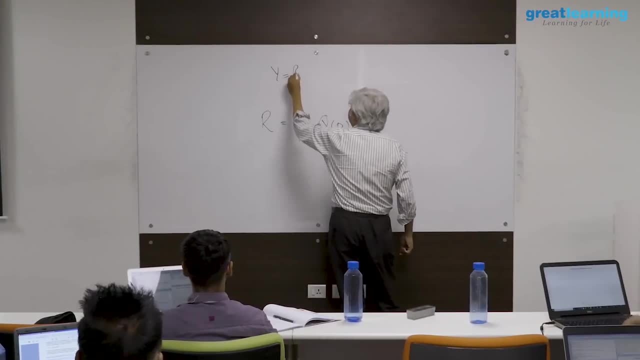 And so that will explain this. So if you can explain it, explain it Like in regression. You've done this in regression as well. In regression, for example, you can say y is equal to say beta, naught plus beta. 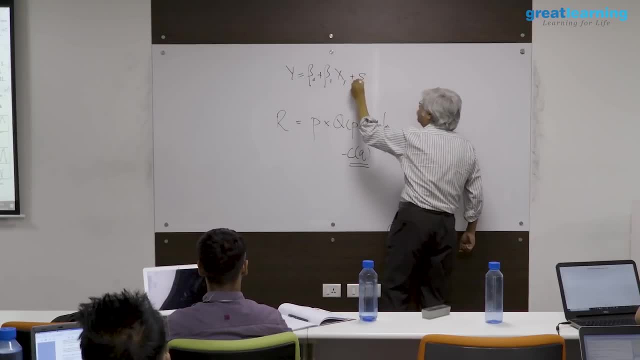 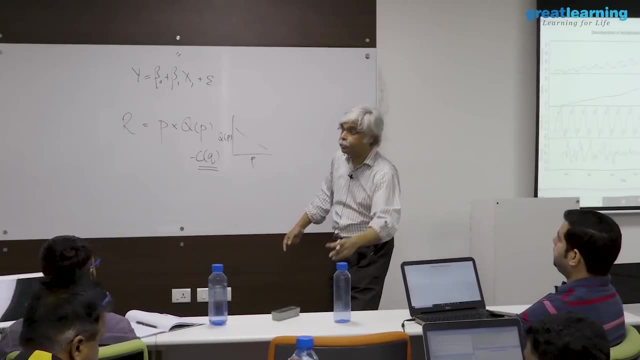 1, x1.. I'm sorry for using different rotations every time, Plus epsilon. And then you say that, but this epsilon has a structure And I'm going to explain this epsilon using another x. And now what you do is you write this: 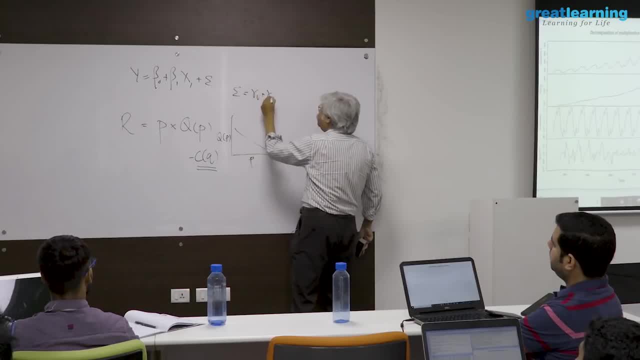 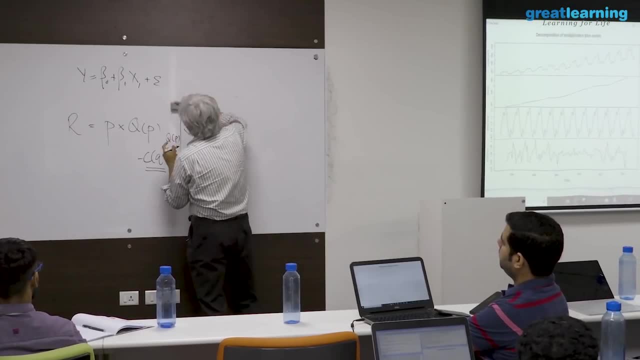 Epsilon itself becomes something like say gamma naught plus gamma 1, x2 plus say delta, Something like that. Now, when I put these two things together, that results in this being replaced by beta 2 plus x2 plus say epsilon. 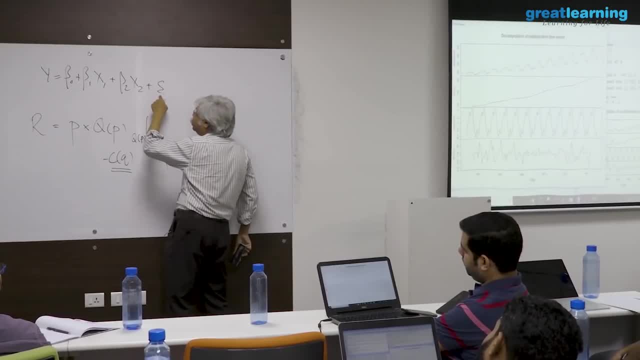 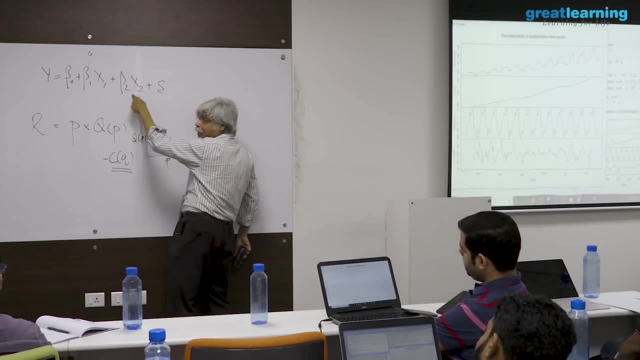 In other words, the old epsilon got decomposed into a component due to x2 and an error. So every time around you explain something, and then you say: is there something else that can explain this? And so you can keep doing this. 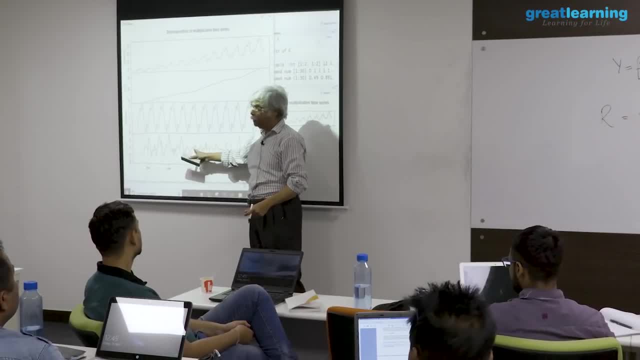 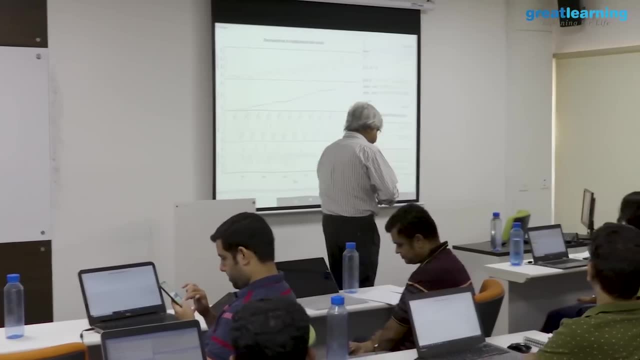 We won't do it, but what you can do, of course, is you can take this series- and you can do a decompose on it as well, And see what happens. I've never done that, but we can try it. 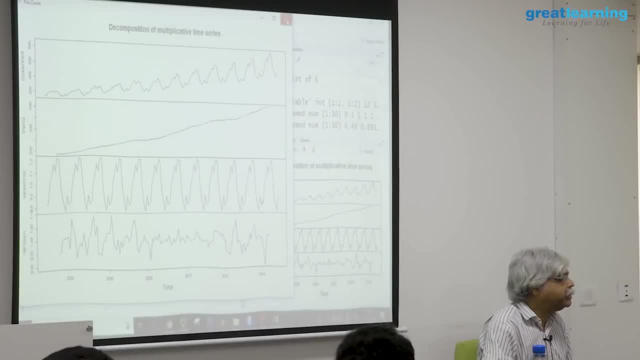 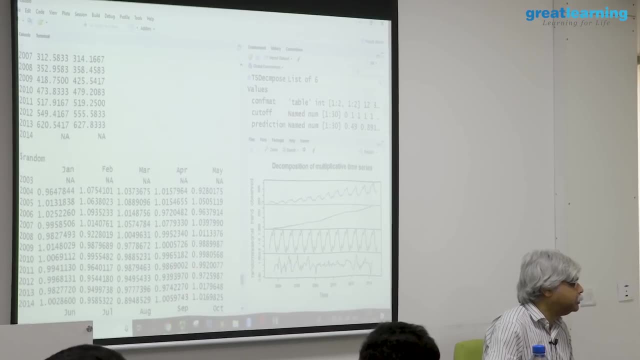 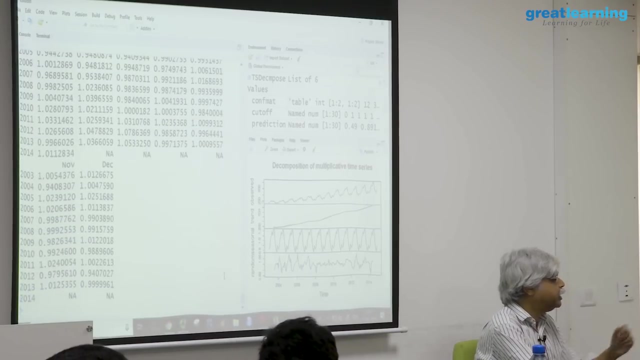 Let's see. So where is this series? Where is it? What's it called? No, It's called random, Right? So it's this, So it's this thing here. This is the random part. This is the random part. 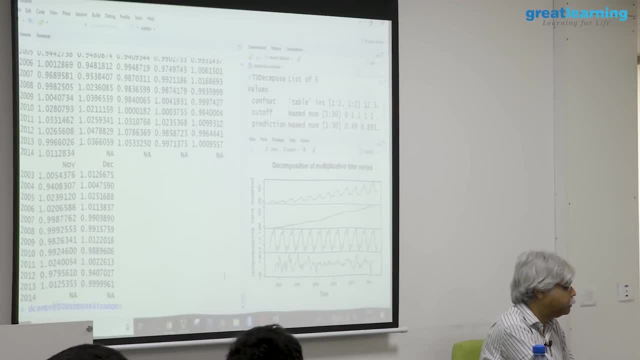 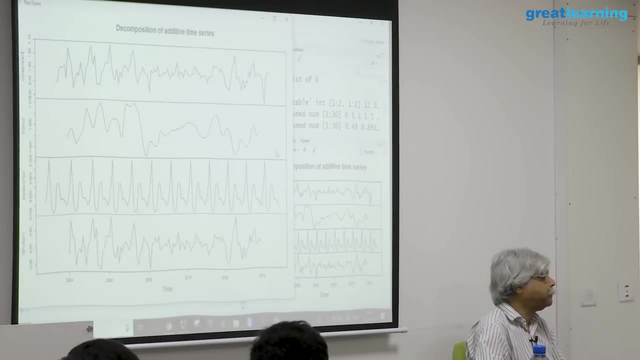 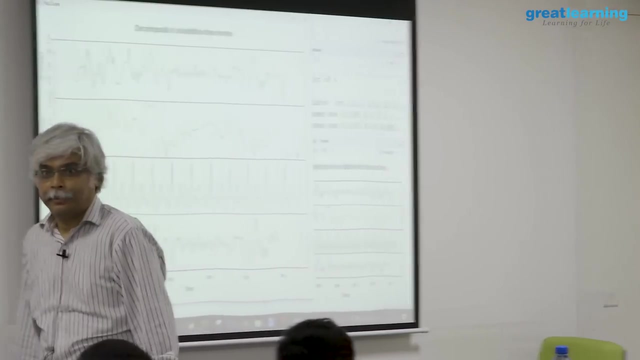 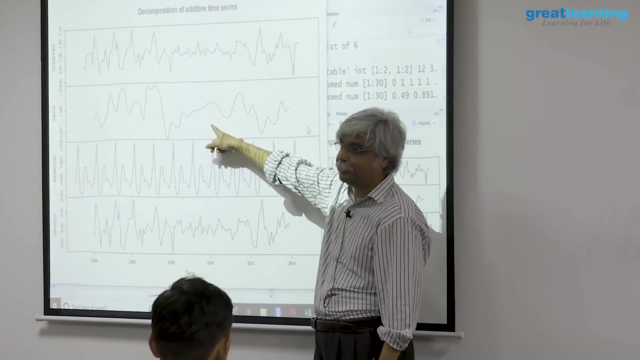 Now I can do, decompose here, Here, What is this strange creature that I've just created For the first time? It's the plot of the unpredictable part of sales. So the original is this: This is its trend. This is its trend. 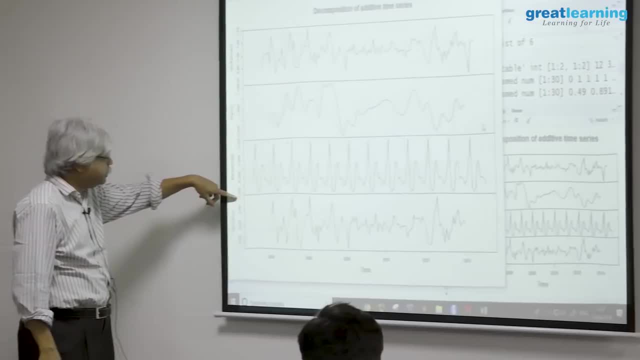 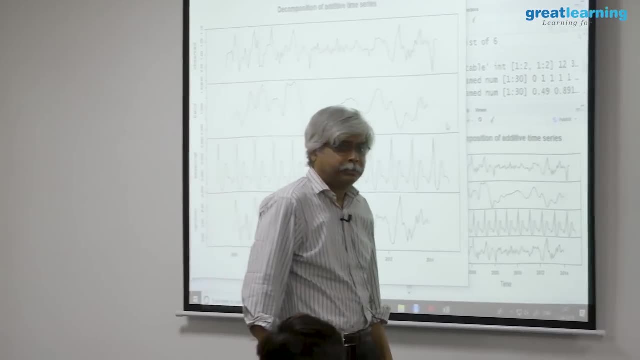 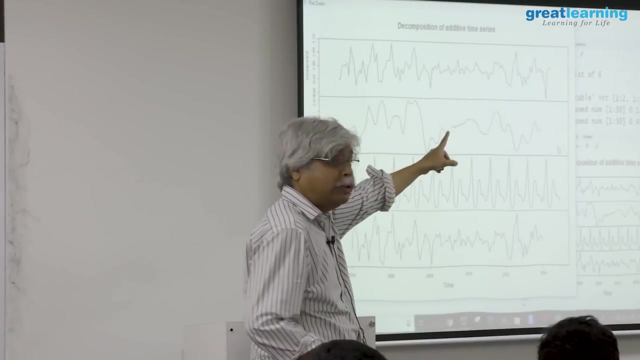 This is its seasonality, From minus 0.004 to about 0.004.. And this is its irregular component. There isn't a trend there. That trend itself is all over the place. There's nothing predictable about this. If there was, the trend would have captured this. 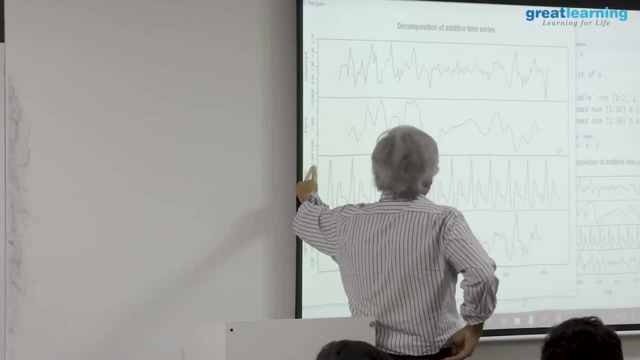 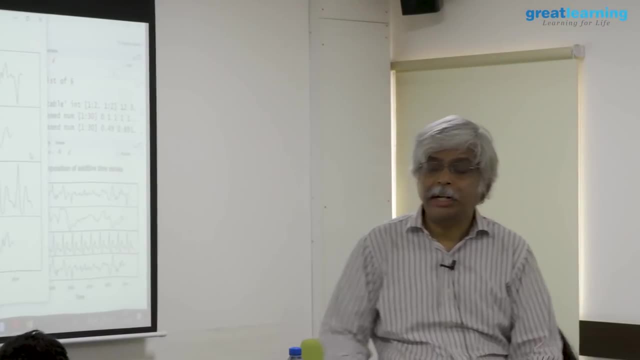 Is there a seasonality? Yes, But that seasonality is very, very small, Tiny numbers. There's no seasonal effect there. Essentially, what this says is that there's no trend and seasonality. in the irregular part It's all being taken care of. 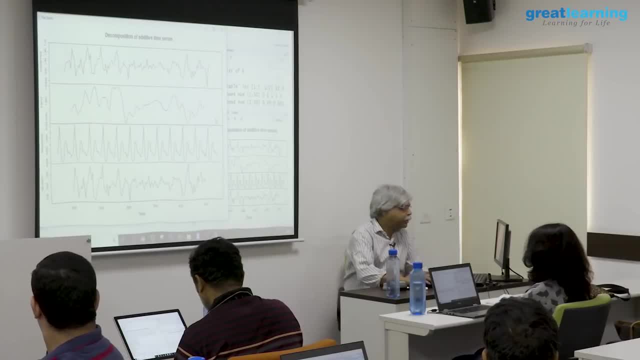 Correct. That won't be captured by this. It would come in the random part, provided that that has gone away. If that investment had continued, what would have happened is it would have lifted up the trend, And we'll see that a little bit when we do the forecasting. 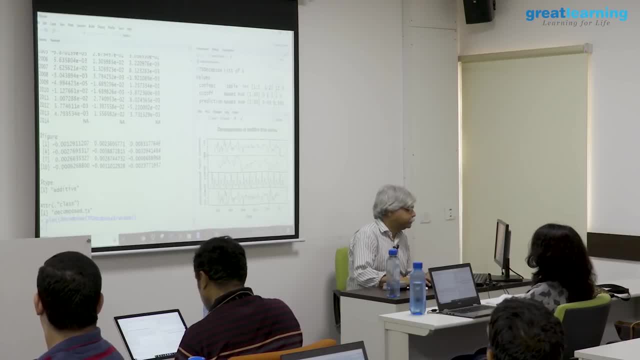 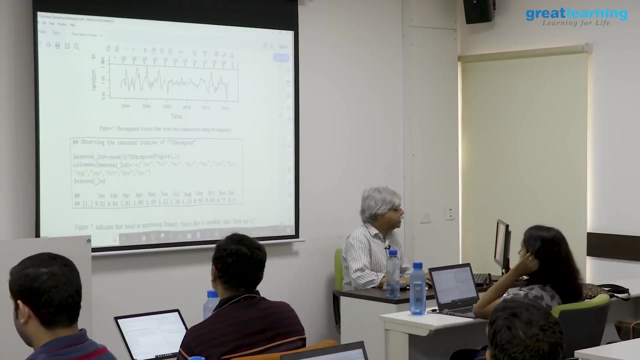 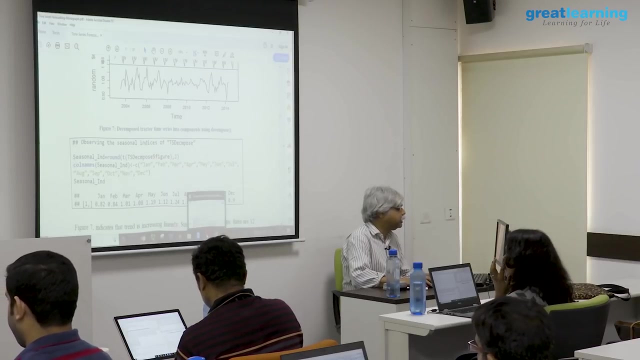 Something like that happens slightly. So this is the decomposition. Now there's another decomposition that we'll get to. You can see the seasonal, Seasonal part to it as well. We've already seen this. So what were the seasonal numbers? 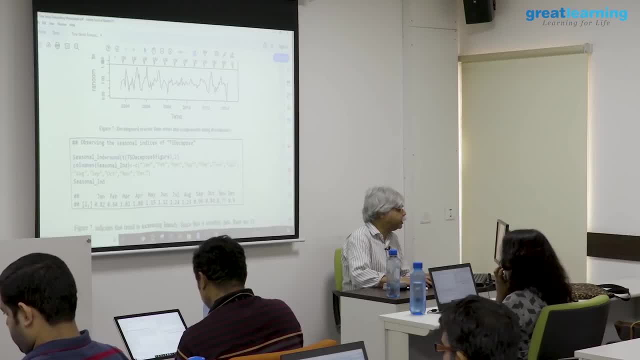 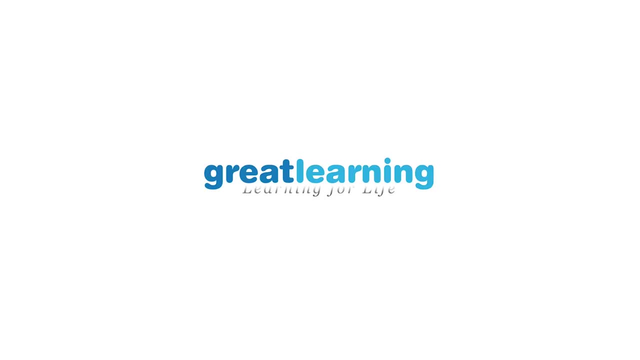 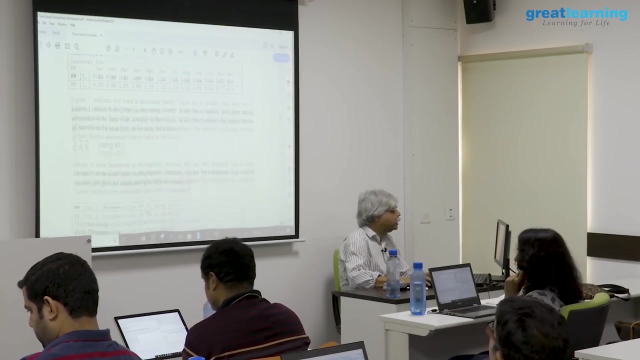 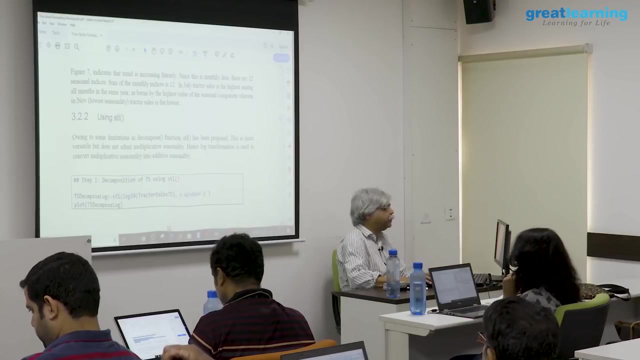 The seasonal numbers you can see here: The 0.81,, the 0.82,, the January numbers here. Thank you. Now the other version of this is the same thing. There are some technical limitations and you don't need to use both of these. 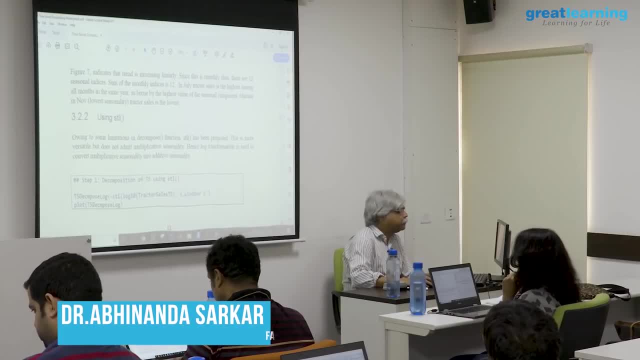 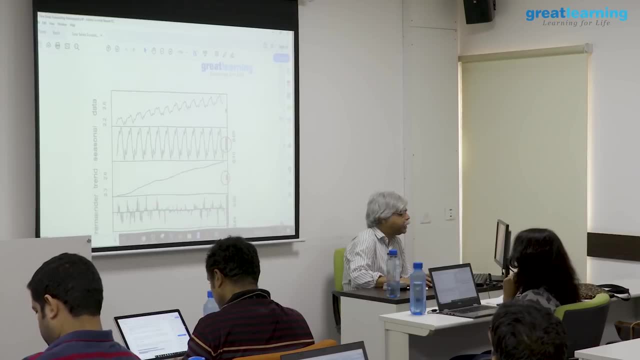 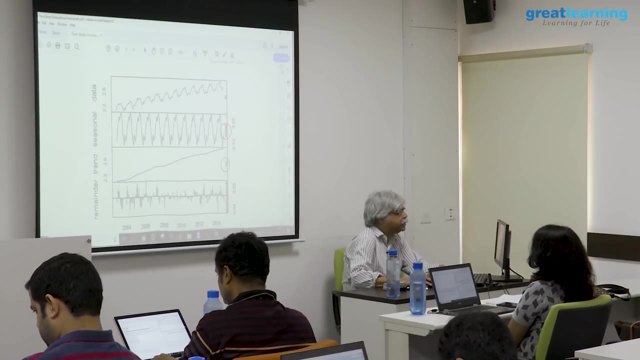 I think decomposition itself is fine enough, But there are some technical limitations to it And sometimes you need to see a little bit of understanding as to the error. And here is the outcome of the second decomposition function. This is called a function called STL. 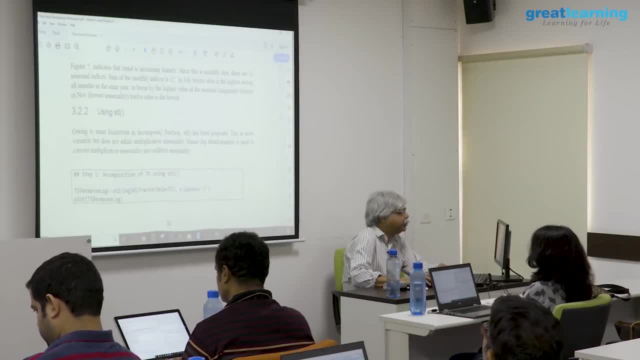 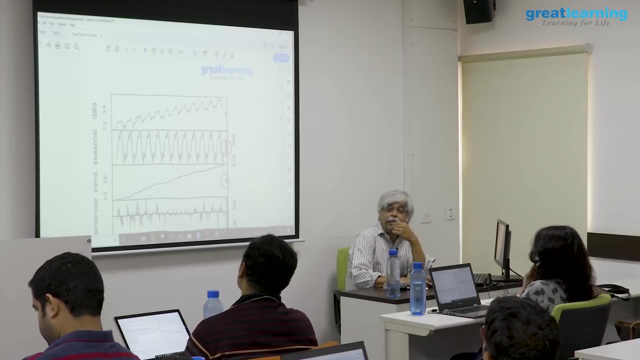 STL stands for A seasonality and trend using low S. Low S is a particular way in which this trend is found. The only reason to do it, from your perspective, is that it gives you these error bars. What do these error bars tell you? 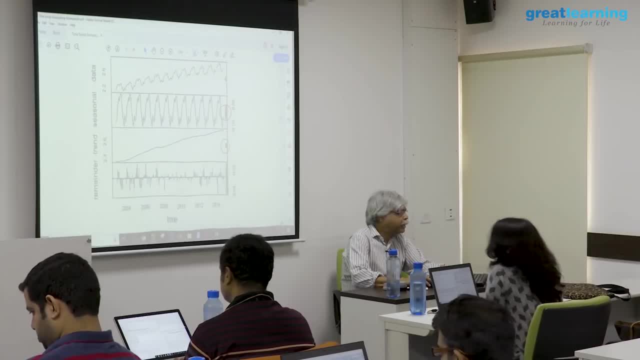 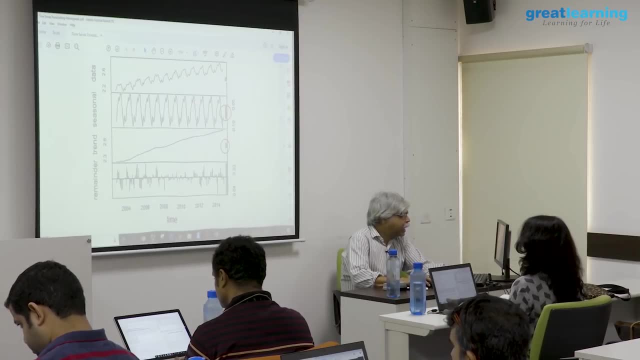 These error bars essentially tell you as to whether this trend and this seasonality, all these things are significant or not. This error bar being very large, essentially tells you. This error bar being very large, essentially tells you that the irregular part or the remainder part, the residual part, is effectively zero. 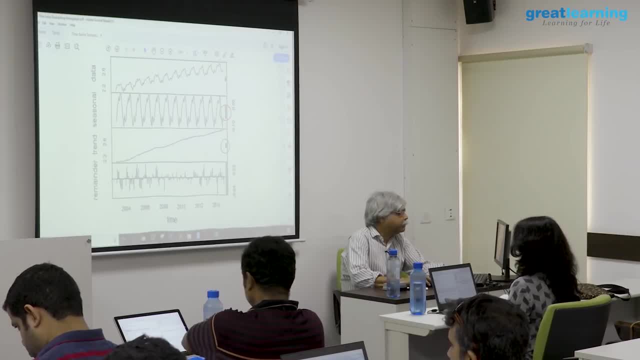 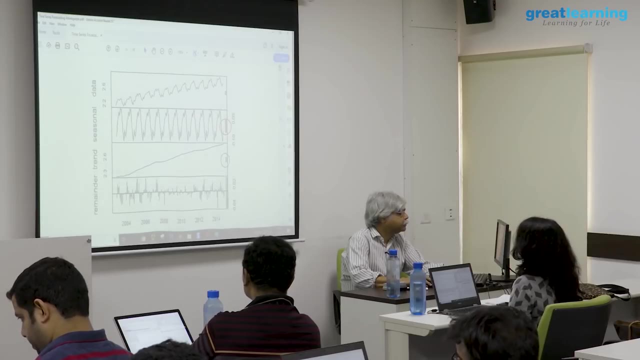 Or if it's multiplicative, then effectively one: This is the residual, This is There, isn't. This is exactly the same plot as before. This is exactly the same plot as before. Hmm, So those are the right side. 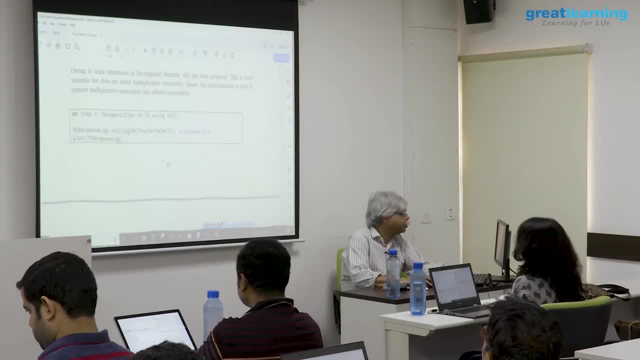 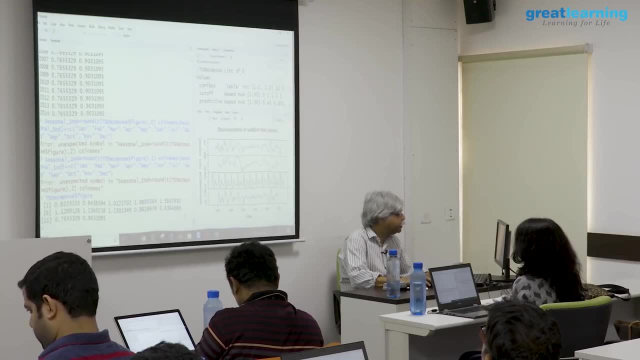 Then: So those are the right side. So those are the right side. Yes, So if I do this, I'll get a plot that is very, very similar to the plot that I saw last time. Okay, Why am I doing this? 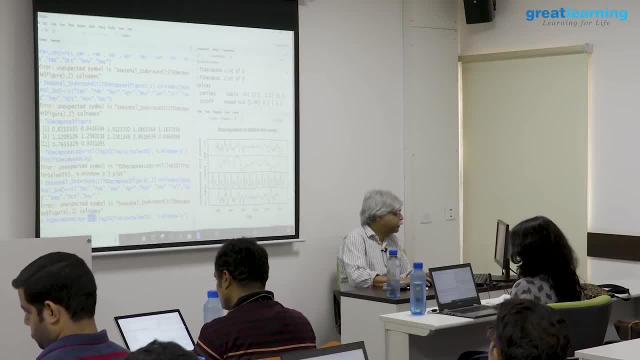 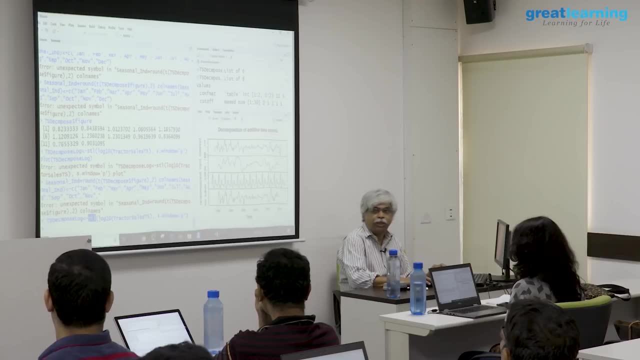 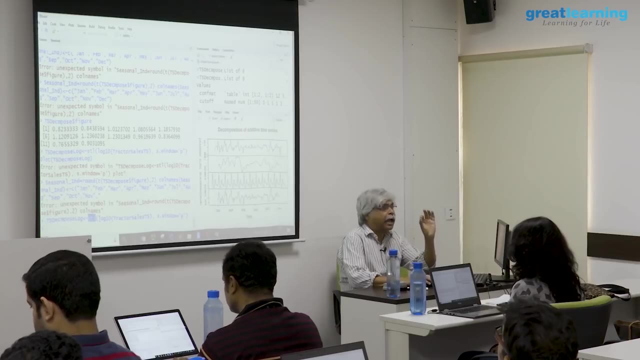 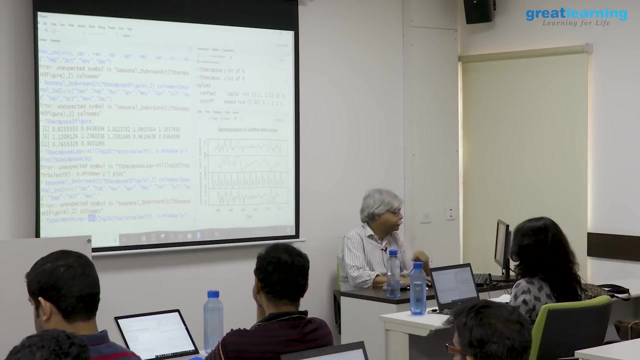 This particular function. This particular function allows for only additive models. There is no multiplicative option for this. I'll explain why. Because there is no multiplicative option, I need to work on the logarithmic scale, So I need to add logarithms, which is what I have done here. 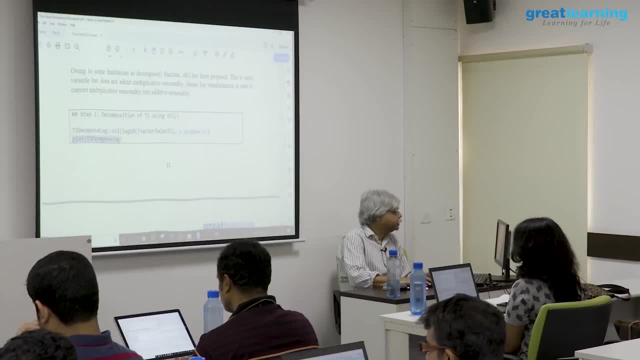 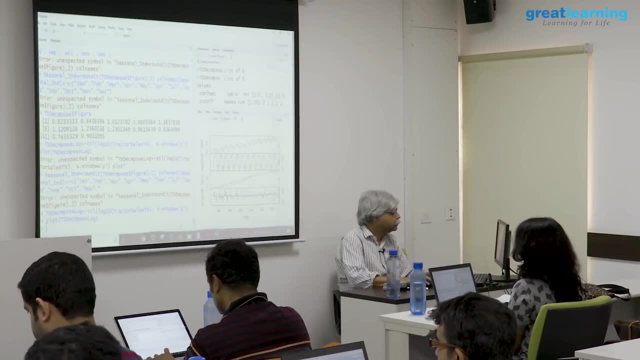 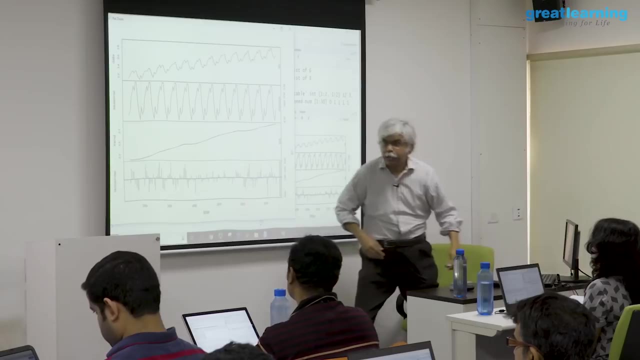 And now I'm going to plot it. When I plot it, which is, I plot the object that is on the log scale, I get this plot here. This is almost identical to the plot that I've seen before, with one major difference in the axis. 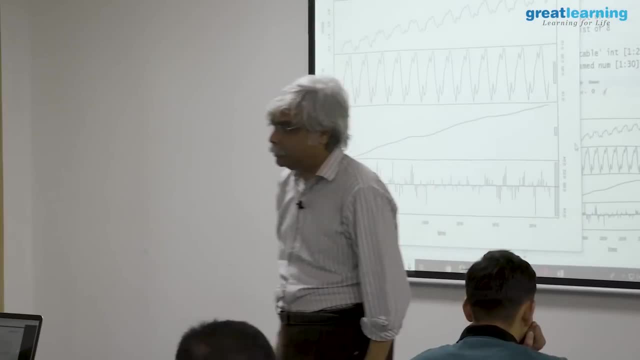 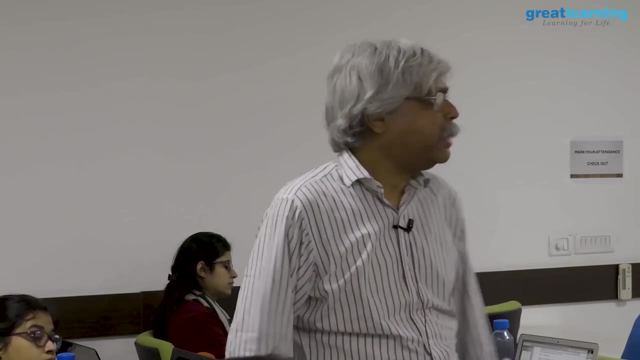 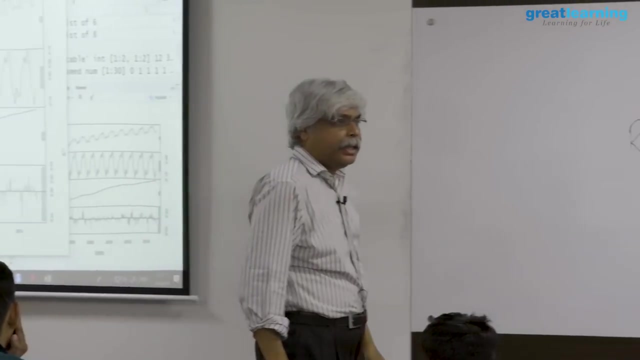 This is logarithm of sales. This is logarithm of sales, Essentially, the number of zeros in my sales. When I look at logarithms of sales, what do you see happening to that data plot? It also has an increase in trend. 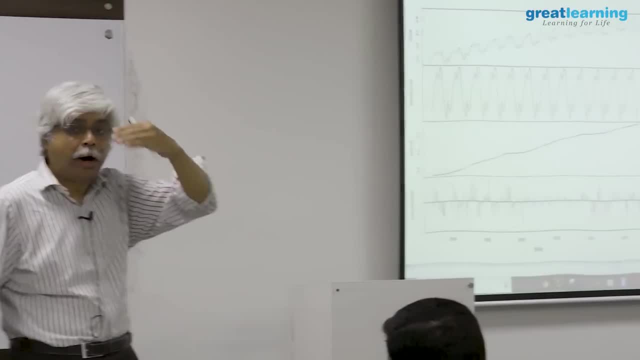 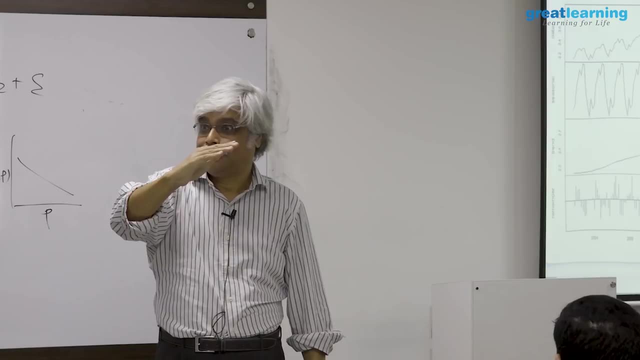 Okay, It also has an increase in trend. However, the seasonality parts have now become flat, So the seasonal correction is now a constant number. It is not additive. It is Sorry. It is not multiplicative. It is additive. 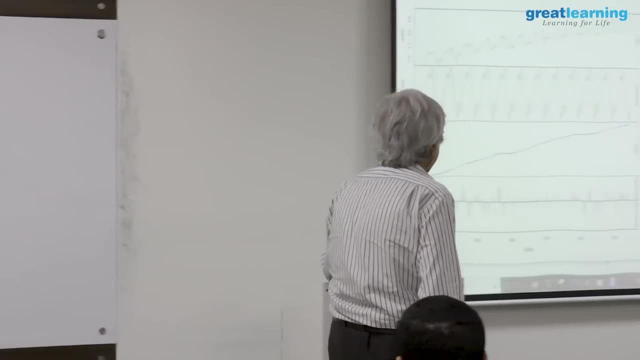 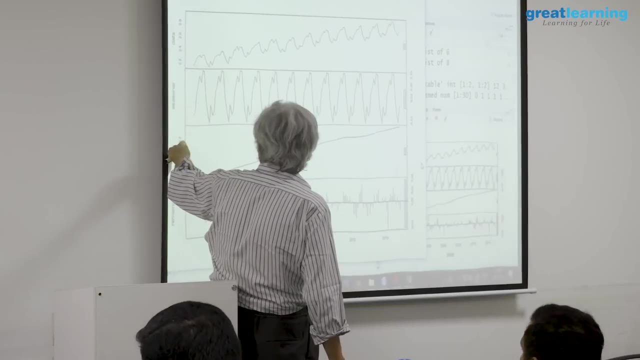 So now what I need to do is I need to add, Add what Here is. my trend On the logarithm side is 2.2 to about 2.9.. The trend again goes from 2.2 to 2.9.. 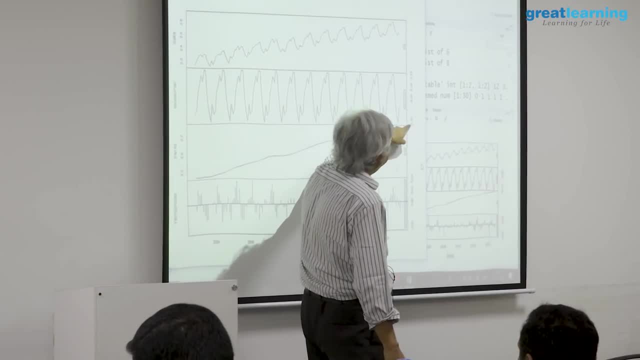 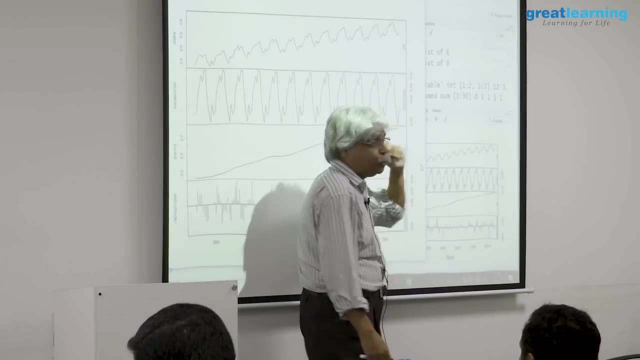 And I need to add those components. Add does not necessarily just mean add. Add could also mean subtract. So on the logarithm scale I go from minus 0.1 to about 0.1 addition on the logarithm scale. 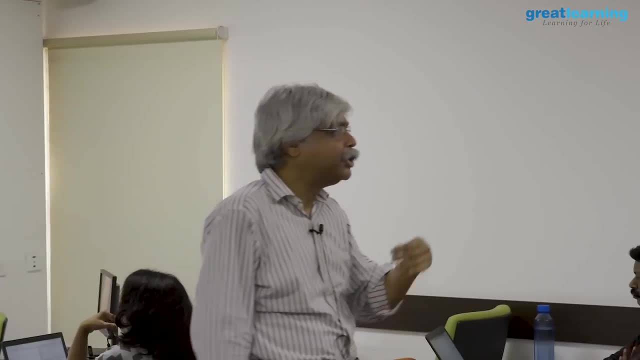 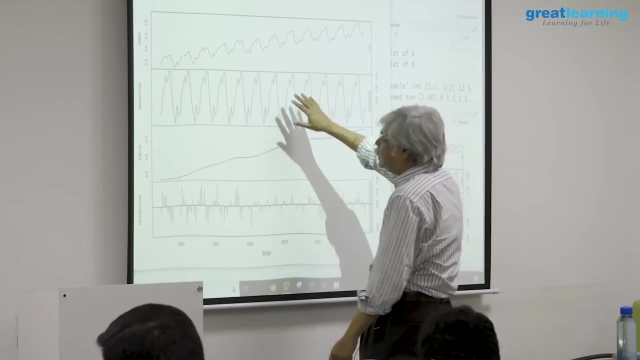 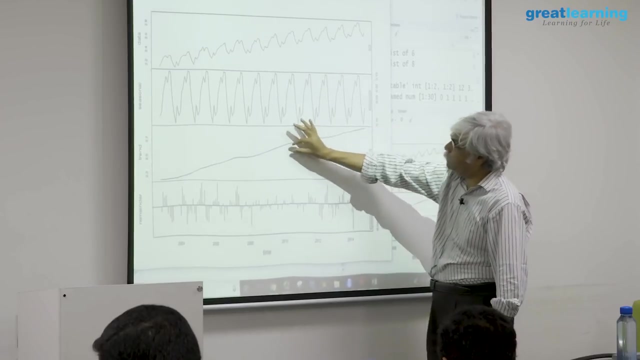 Addition on the logarithm scale, which is equivalent of multiplication on the original scale. So this is exactly the same plot that I've seen before, except the seasonal has been plotted above trend, But this is the error bar that is associated with this number. 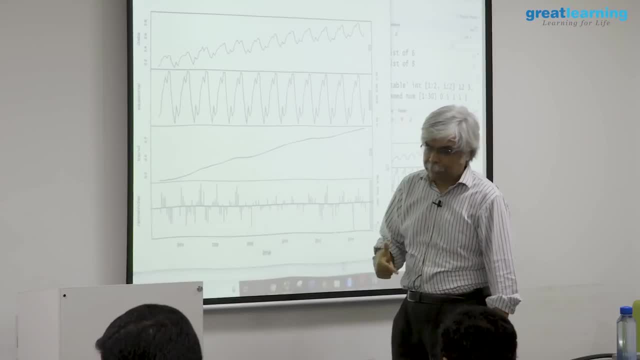 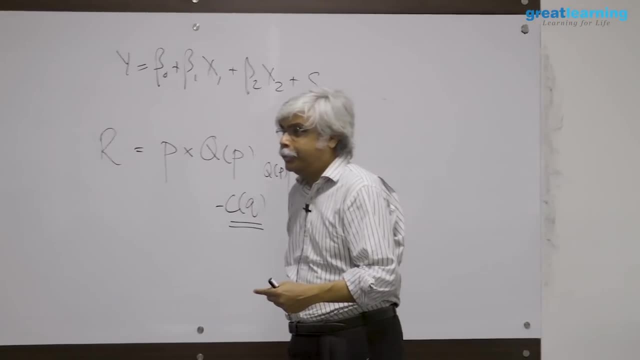 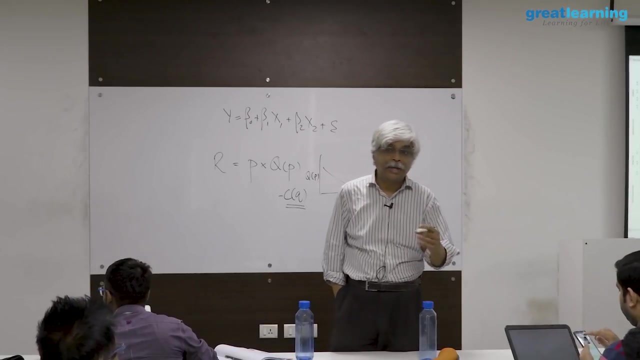 Statisticians find it comfortable to work with additions of things because variances add up. One of the more painful things that we often have to do when we teach basic statistics is we have to teach two notions: one of variance and one of standard deviation. 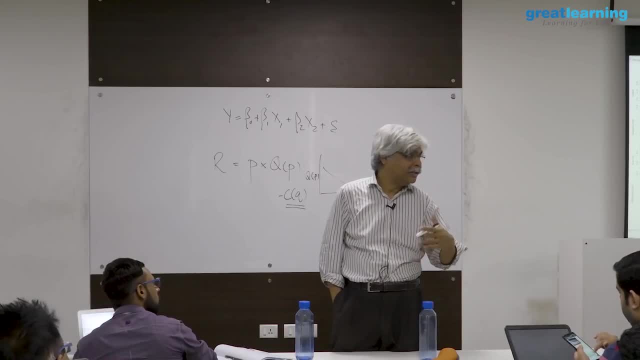 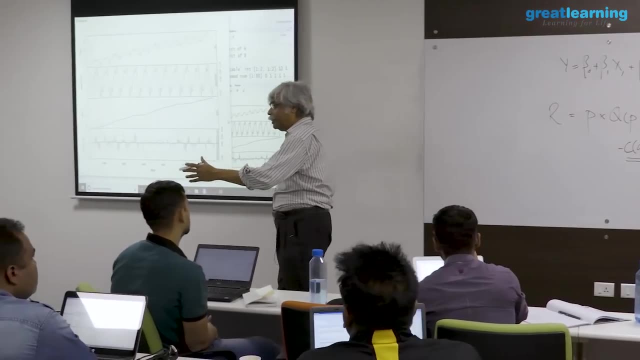 People often ask that why are both variance and standard deviation taught? The reason is because standard deviation is what you use. It is on the same scale as the mean. It has that 68 percent, 95 percent, 97.3 percent interpretation. all that works well. 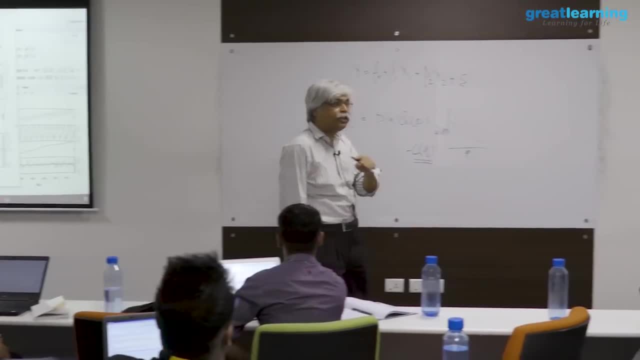 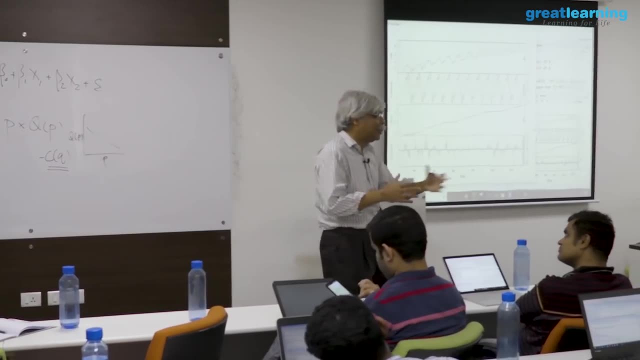 Standard deviation is what you want. The problem is, however, the standard deviations do not add Variances add. So when you want to add up things, you add up variances. You cannot add standard deviations up, which is why people calculate variances, because 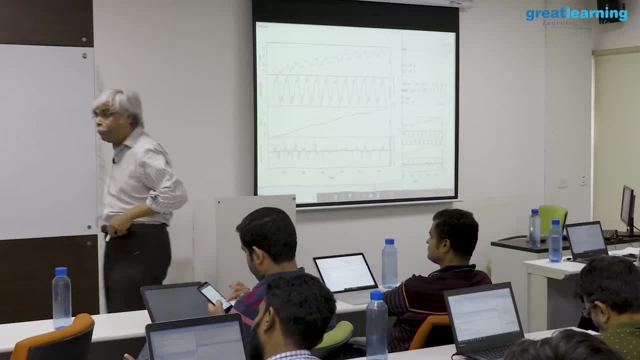 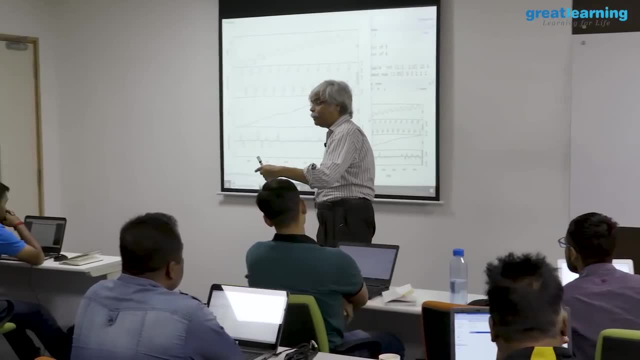 you can add up error on the variance scale And because you can add up something like this has to be done. So if the model is multiplicative, the errors multiply, But multiplying errors is a lot harder for the statistician to deal with. 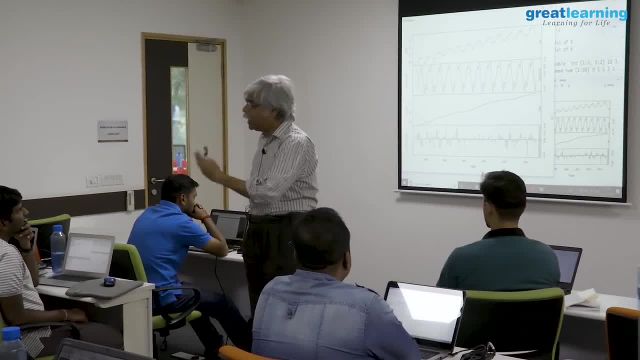 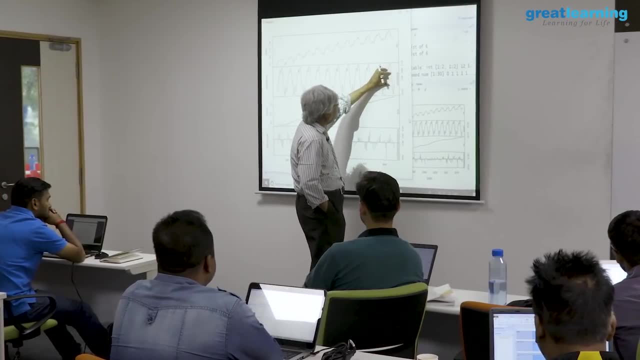 So they say: let me take logarithms and let me add up errors, And when you add up all those errors, you get these error bars. So what does this error bar mean? This error bar means essentially, anything that is between these error bars is indistinguishable. 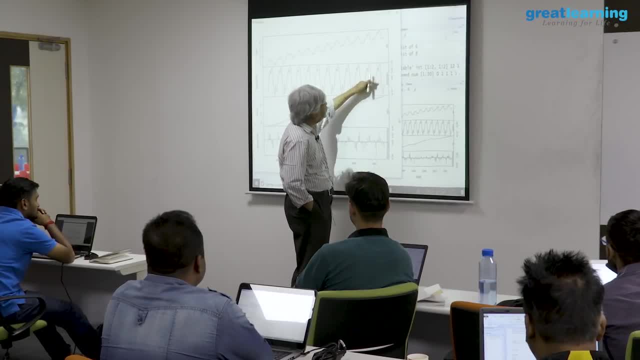 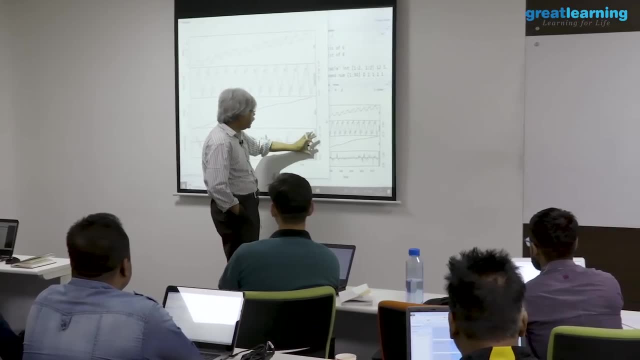 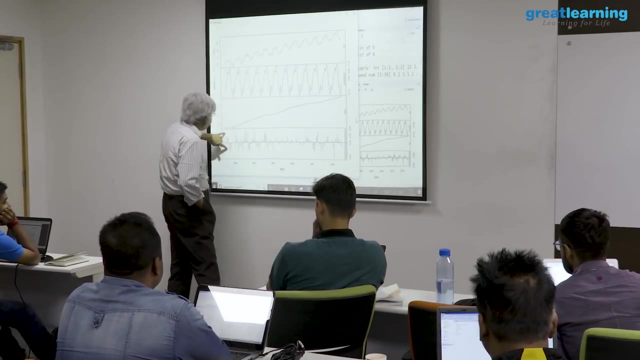 So the fact that this error bar exists and the seasonality extends out of it is telling you that the seasonality is statistically significant. But here all my errors are within my error. So now you are saying that the error, this error, the remainder, so to speak, is statistically. 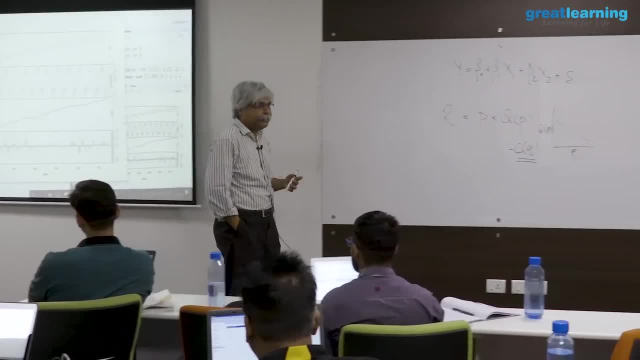 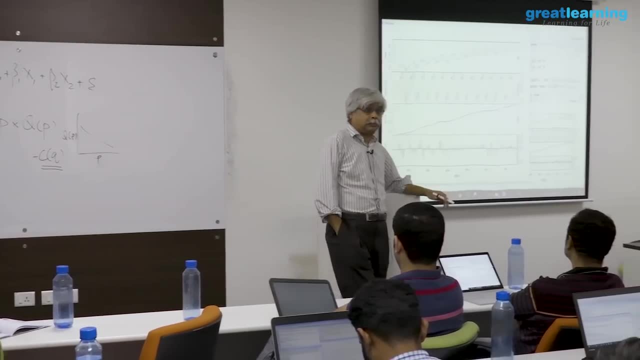 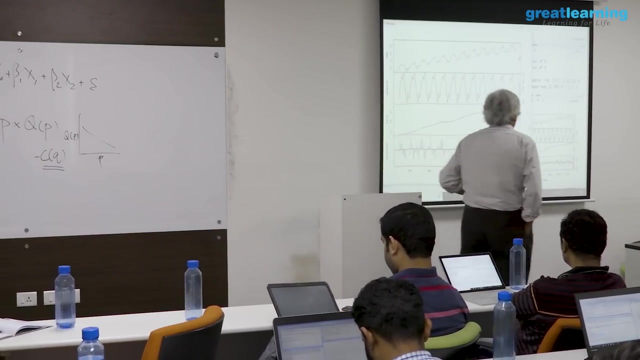 insignificant. They all fall within, shall we say, a confidence interval around zero. Not yet, We haven't figured out autocorrelation yet, but we might get to it. So there is. So, which gives us the confidence to say: 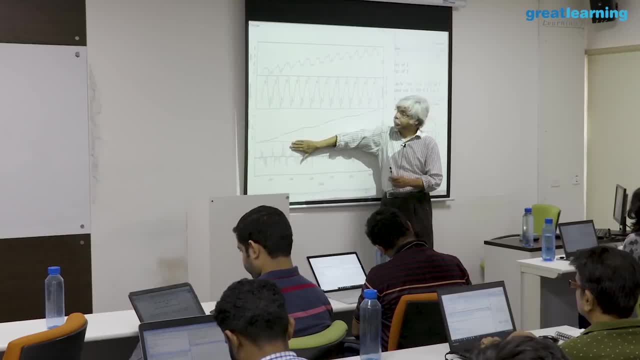 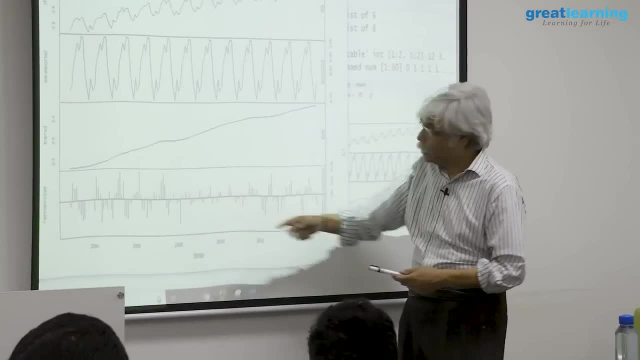 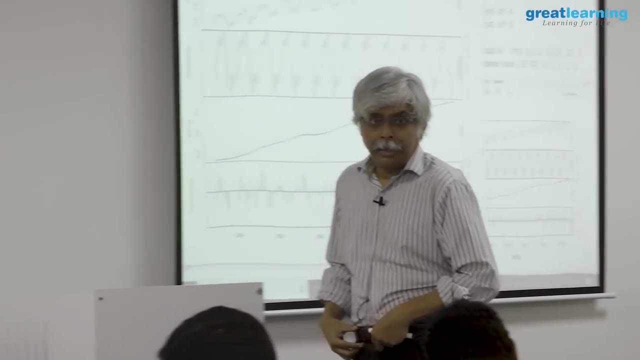 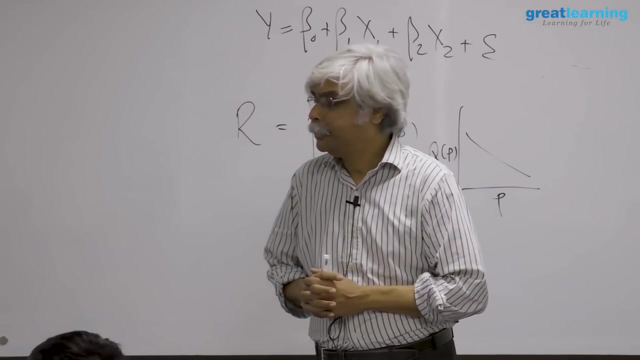 I can ignore this guy. This guy is statistically insignificant from zero. All these numbers are insignificant from zero. Why they all insignificant from zero? Because they all are within the permissible error bar around zero. But if this becomes a little too unnecessary, you are welcome to simply work with decompose. 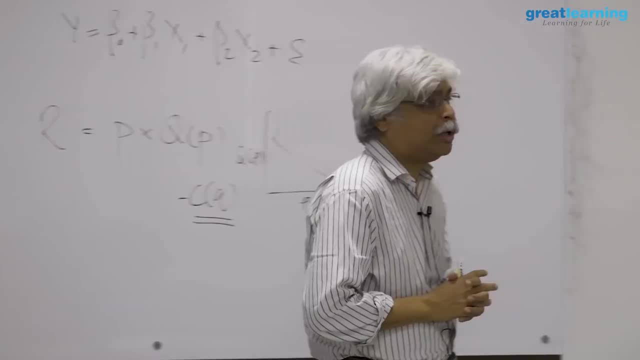 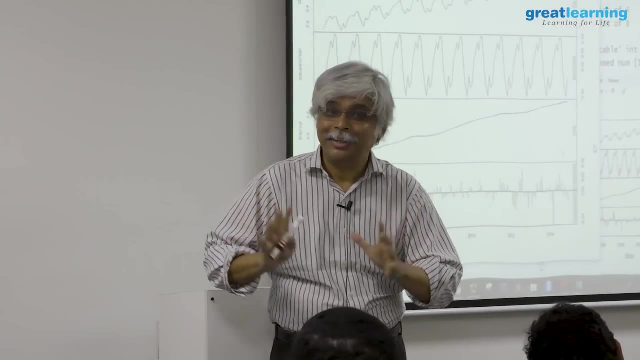 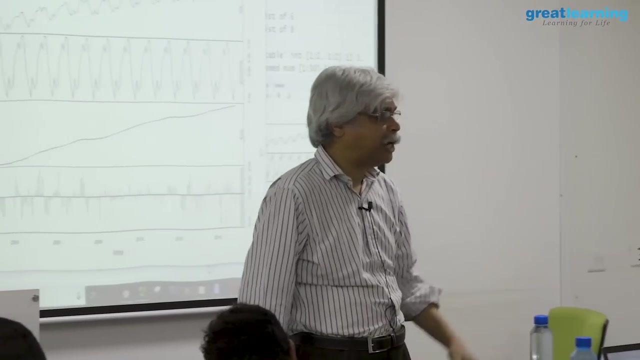 The model that it fits is not dissimilar. The model that it fits is more or less the same. Remember, till now, we have not actually forecast anything. We are simply describing, We are visualizing, We are conceptualizing. I am getting numbers that tell you what is happening in January. 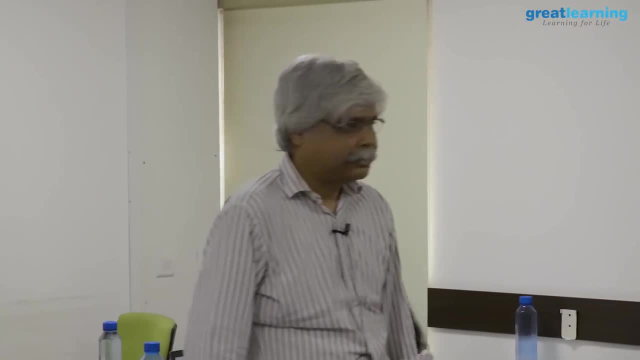 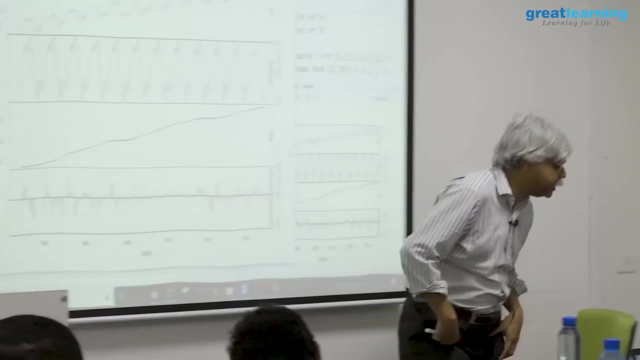 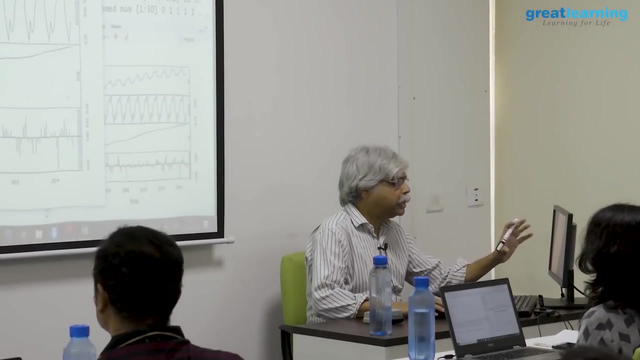 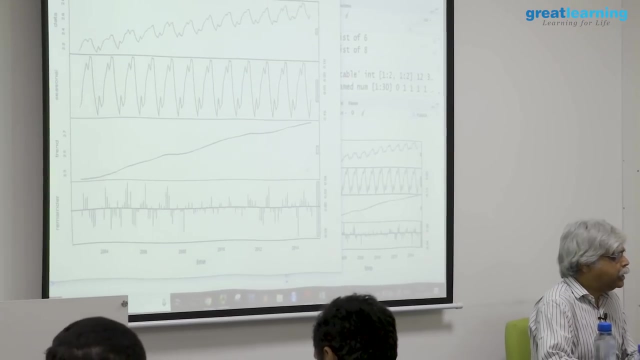 What happened in 2008.. This gives a little bit more faith that the numbers that come out of these models are to some extent statistically robust. So I am going slightly beyond description here And going towards, shall we say, inference. this is included in in forecasting. one reason is because 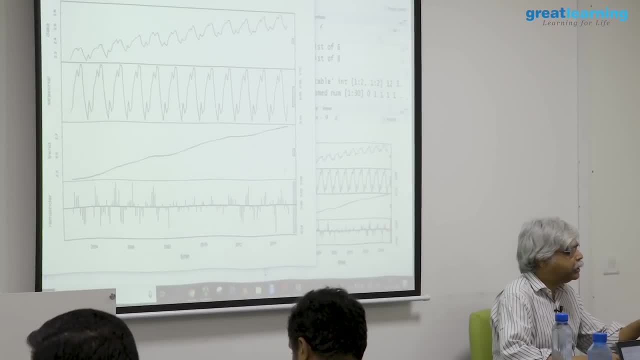 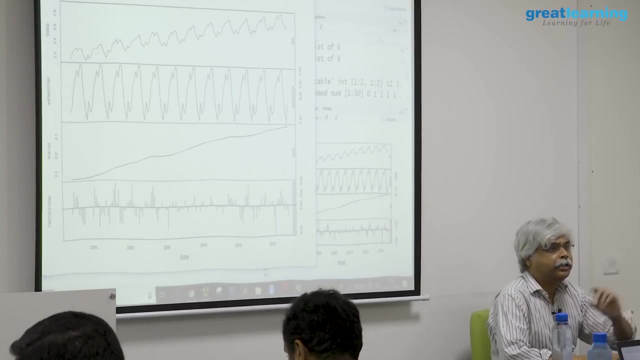 future. in future, when we do forecast, you're going to have to include these error bars in those forecasts. not today, but we'll get there, okay. I know this part was a little quick, but it's it's. it's a little add-on to the descriptive technology for your projects or for any purposes. decomposes good enough. this. 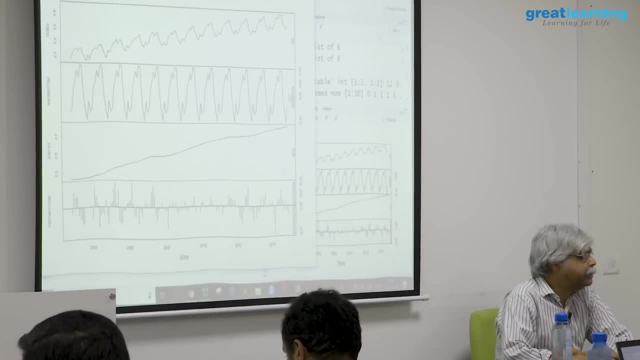 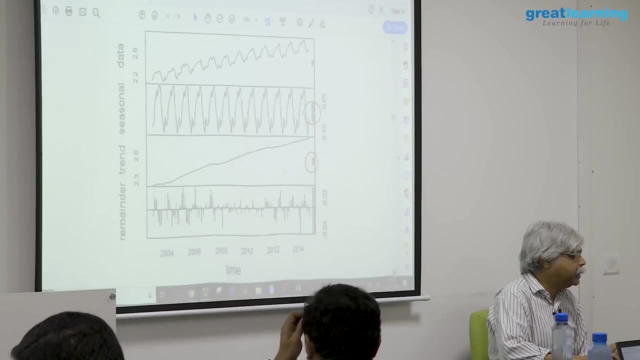 gives the additional feature of these little uncertainty bars around it. no, it's not a question of smaller the bar, it's a question of. let me show it here. it's a question of: does the data lie within the bar or not? if they didn't, if the data 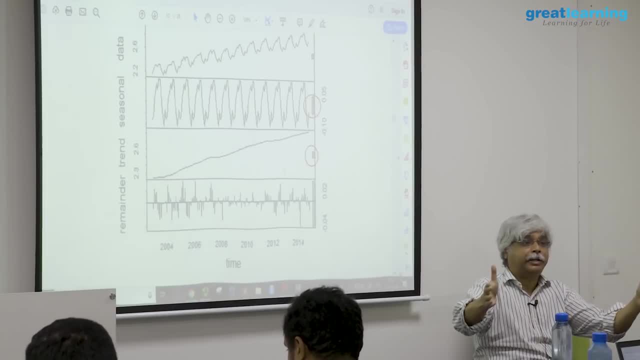 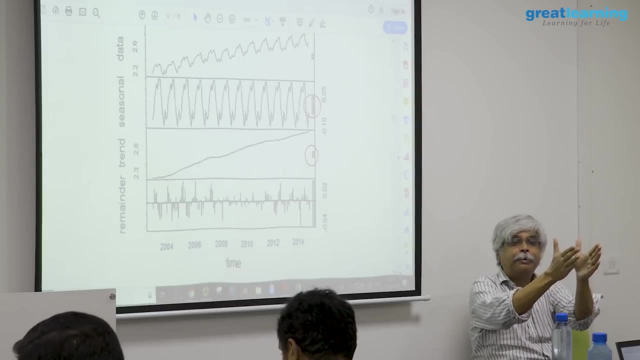 goes outside the bar, then it is statistically significant. if it stays inside the bar, it is the same as noise. that bar essentially dictates how much of this is explainable by noise. you may have seen this when you did confidence intervals in SMD em. if you, if 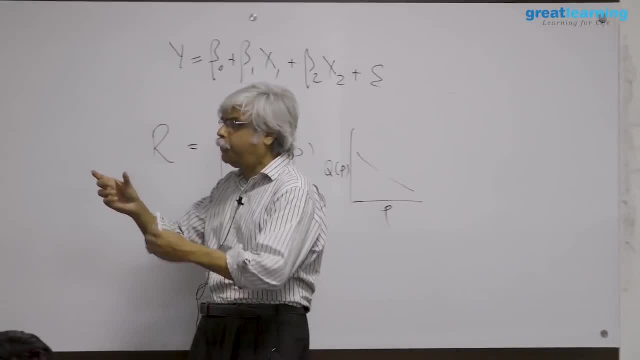 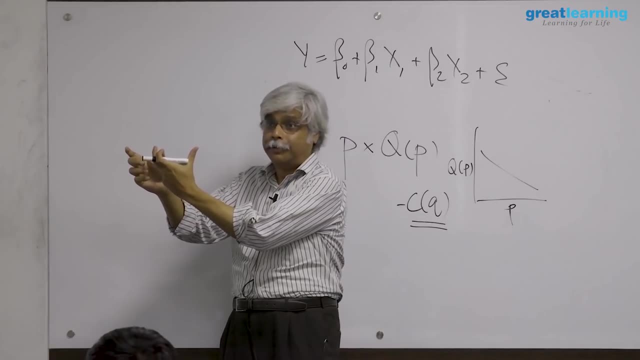 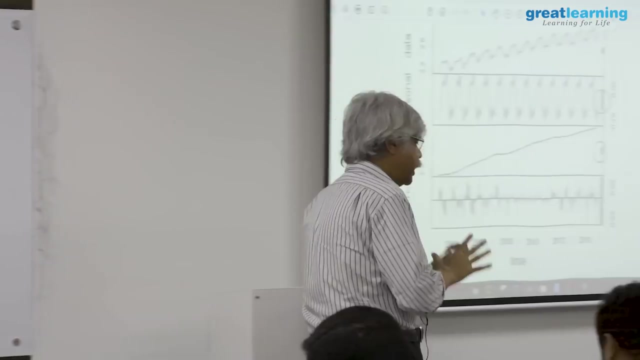 you did confidence intervals, that there's the idea that does the confidence interval contain the parameter or not, or does this confidence interval intersect with another confidence interval? so that idea, so this, basically giving you a confidence interval around that again, if that's unnecessary in the sense that that's a little bit of an overkill, then that's. 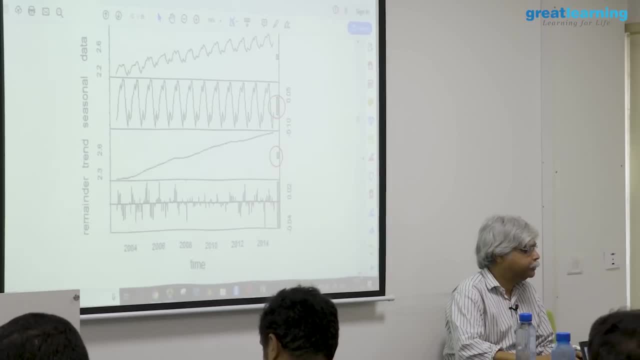 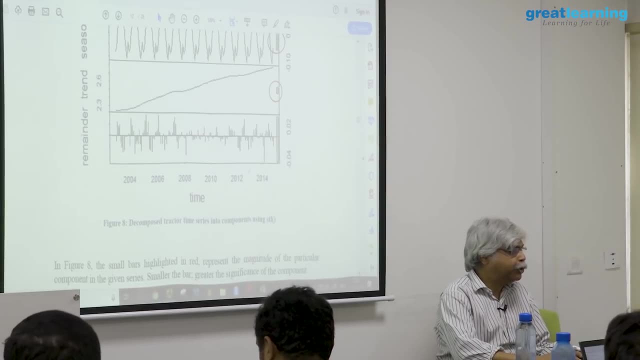 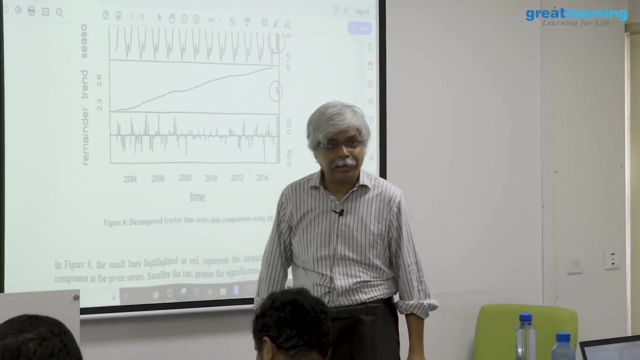 that's fine, not yet, not yet. not yet because, at this point in time, what you are doing is you're calculating standard errors. so, for example, the standard error of the sample mean is Sigma over the square root of n. this formula doesn't require any assumption of normality. this is true whatever it is. 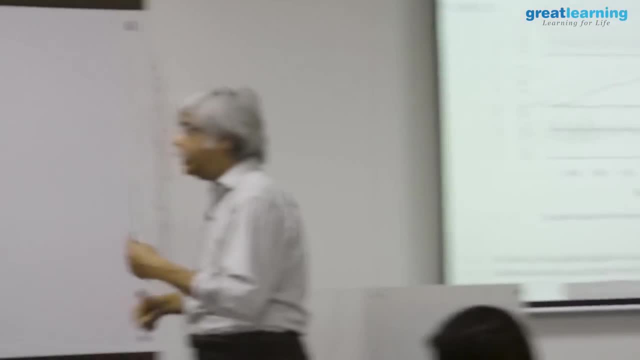 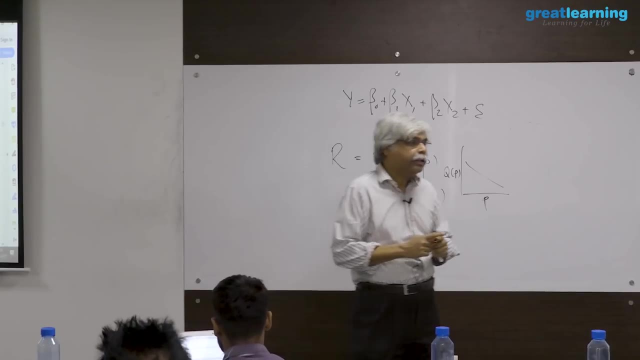 now the, the, the, the 95% part of it or the 90, 99 percent part of it could involve normality. knows where do I get that? so yes, if you are converting this into some kind of confidence interval, some assumption of normality may be. 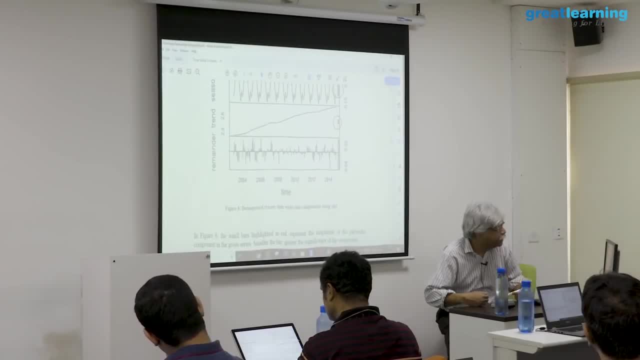 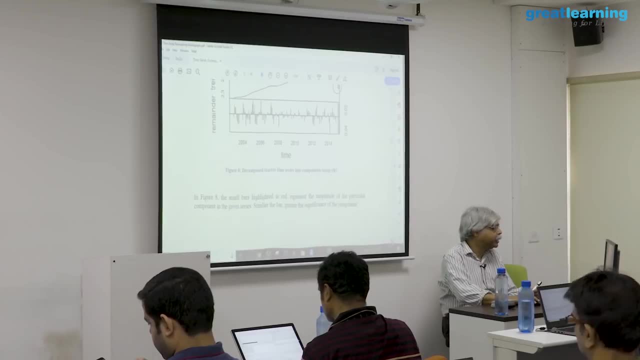 needed, but for the error estimation itself. normality typically is not. you can always do test for normality and things like that around. I suggest you don't, because normality testing is here: smaller the bar- greater the significance of the component. smaller the bar- greater the significance of the component smaller. 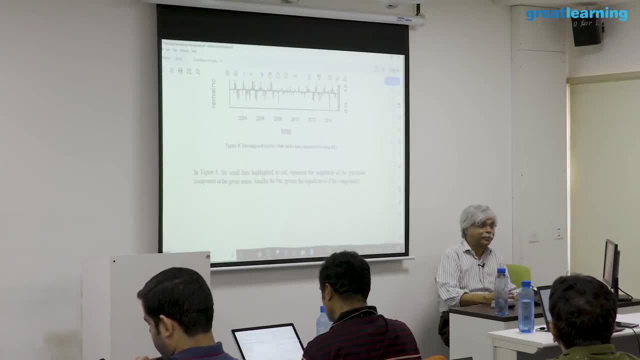 than what? small compared to the signal itself. so the signal is large and the bar is small, then the signal is significant. if the signal is small, the bar is large, then that signal is essentially zero. though that's just the way it is plotted. no, everything is discrete in some way, everything is. 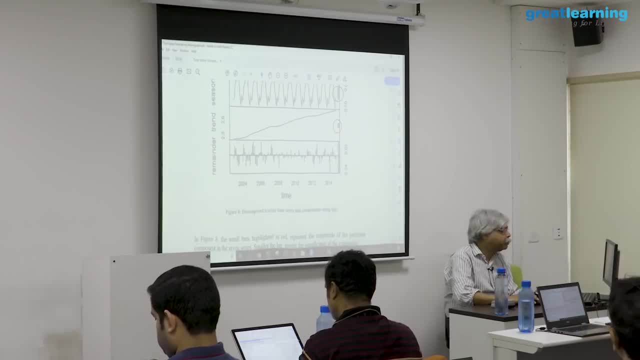 counted only at 144 times. it's just that this is like plotted as type equal to L and this is plotted as type equal to B. it's just the way. it is just the way it is plotted. yes, that you can say that the trend part is more. 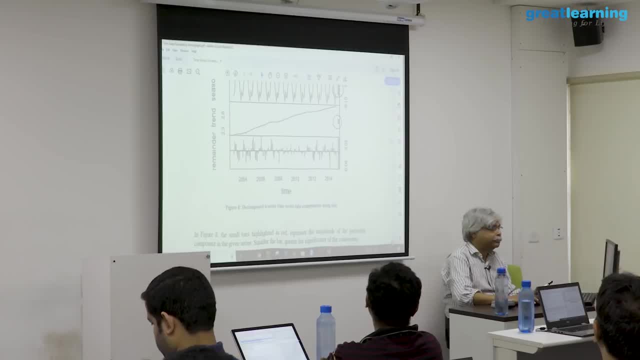 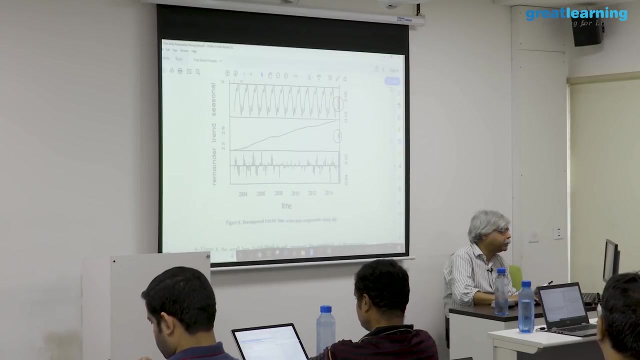 significant than the seasonality part, if you want to. because essentially what? what does this mean? it means that if I am here, what is the trend? the trend is this number plus minus, this little thing here. similarly, if I am here, what is the seasonality number? the seasonality. 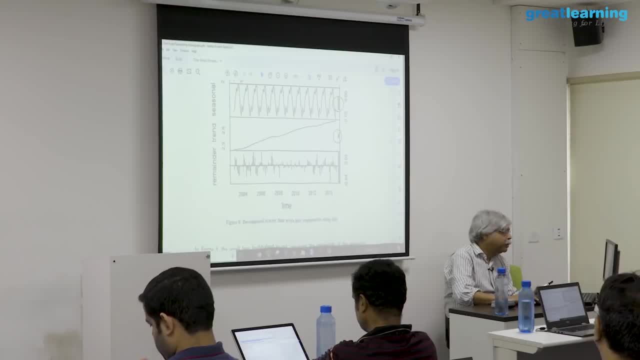 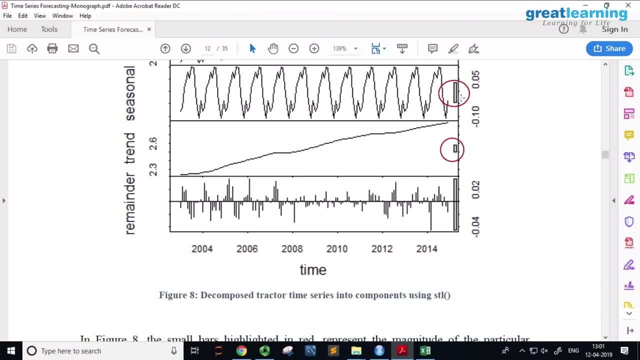 number is this number plus minus this little thing here. but because the bar it's itself is much smaller than the value of these numbers, this number plus minus this bar and this number plus minus this bar do not intersect with each other. that means they're statistically different, that means there's a seasonal. 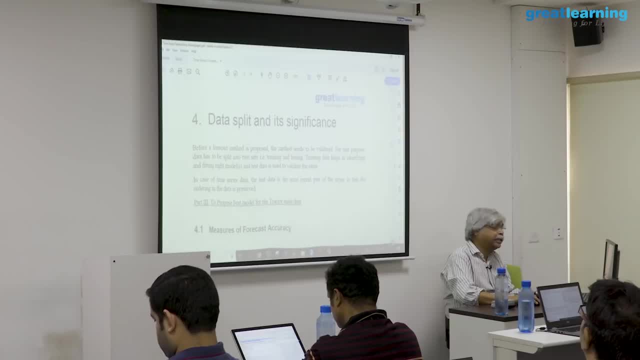 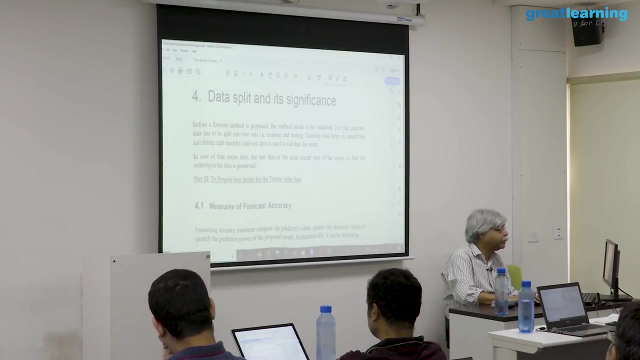 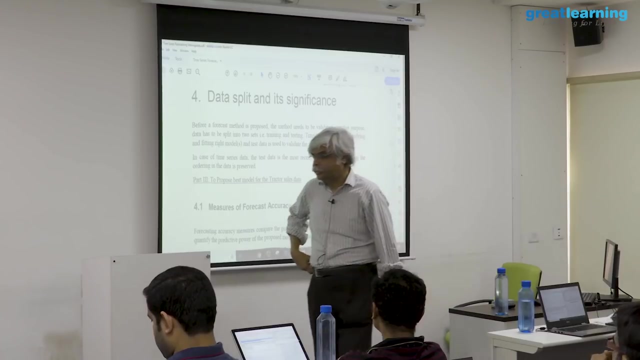 effect? okay. are things going too quickly? no, all right. are they getting boring? possibly, yes, okay. I want to do this a little bit before I think I think we've covered quite a lot. actually, we'll see. so this: the statistical purpose of this is to get some kind of error assessment around it, but the machine learning view of it is: 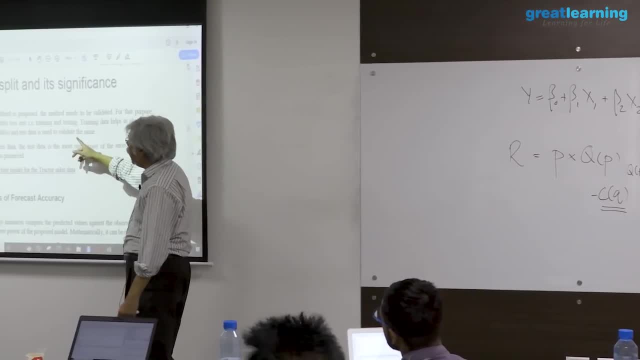 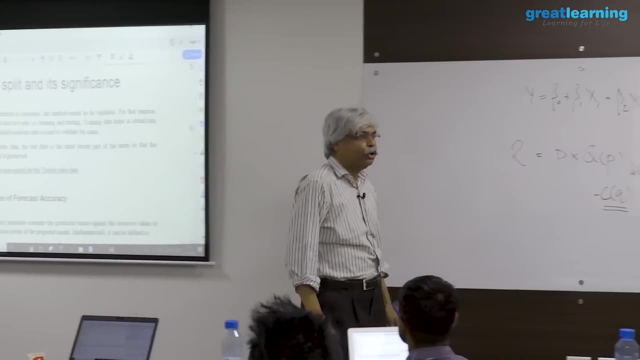 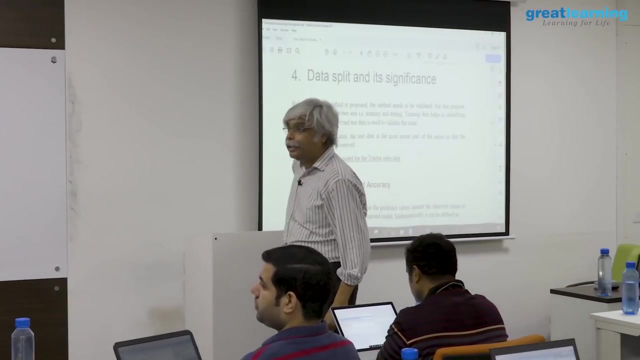 also valid. which means what? which means I now need to be able to see whether this model forecasts or not. but how do I know whether a forecast is good or bad? so here's one particular. I'm sorry say again: train and test in machine learning. how did you do? how did you pick a training? 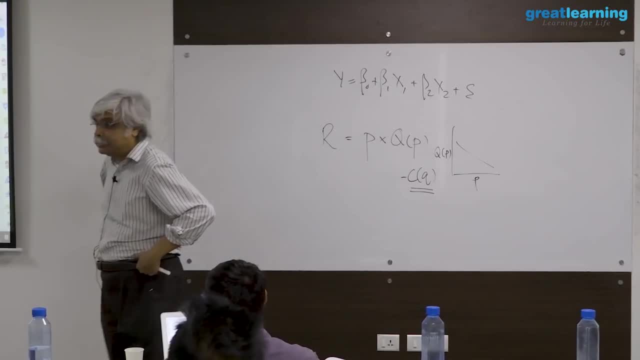 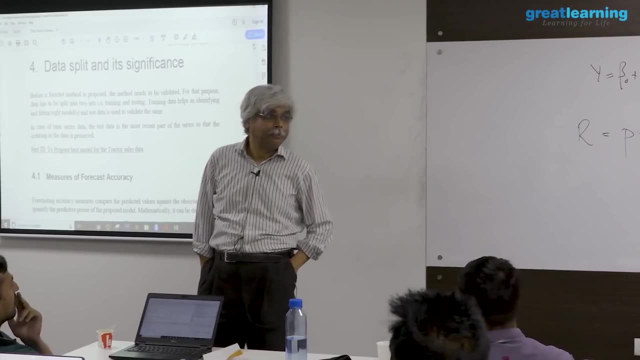 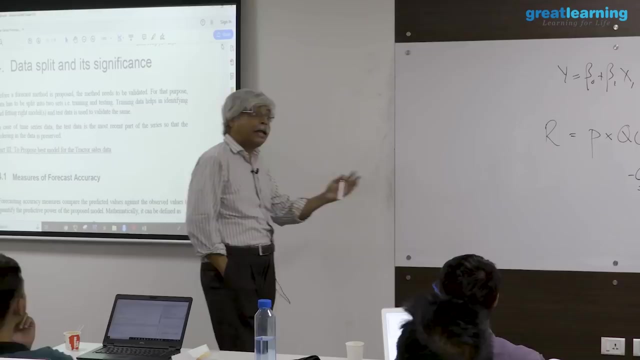 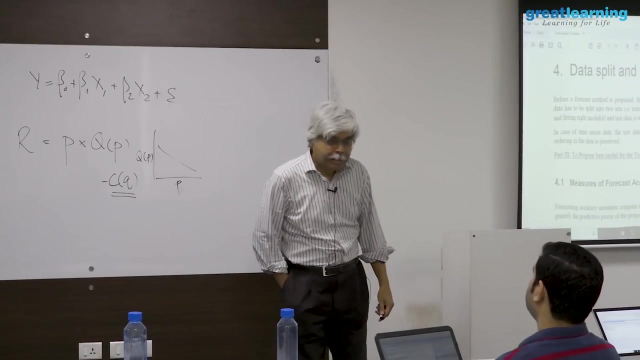 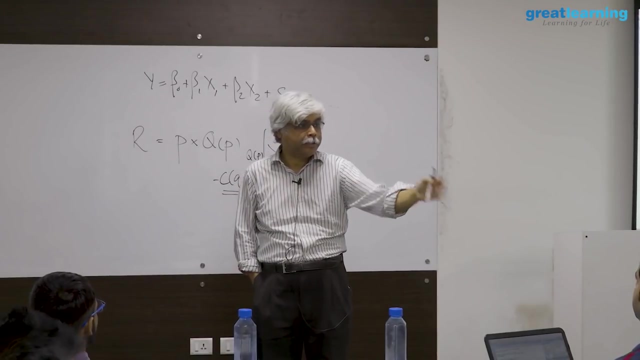 set how. which 70% did you take? random? okay, can I do that here? why not? because the time series, so I lose my old my whole time. my time concept, yes, so so. so the easiest thing to do would be to say something like the first 70% is my training and my last 30% is my test. so it would look a little bit like: 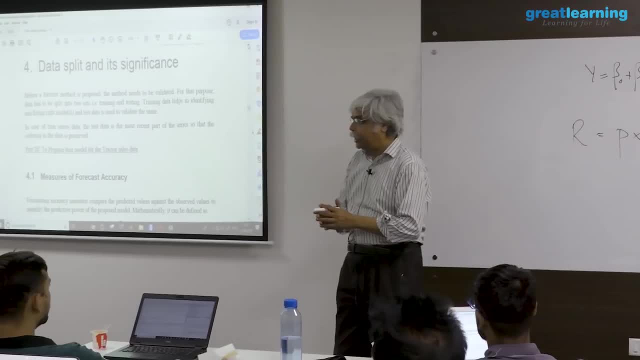 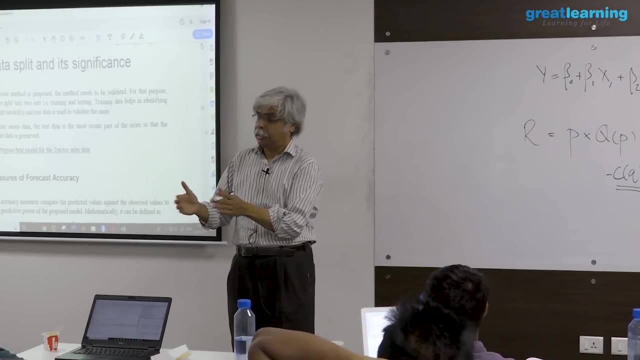 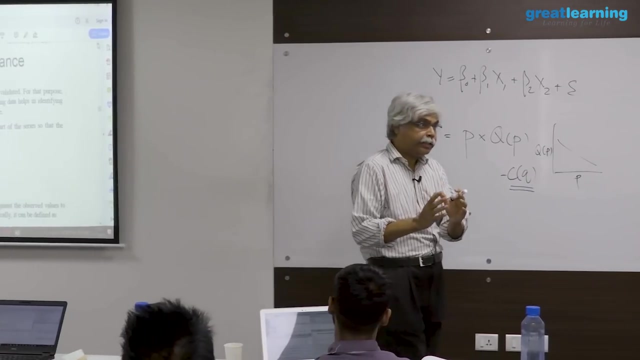 this. I am sitting at the end of, say, 2014, wherever it is, and I want to forecast from 2014 to 2016 and I want to develop an algorithm to do that. now, how do I do that? I need to forecast two years. so now I say: can I forecast two years, two years? 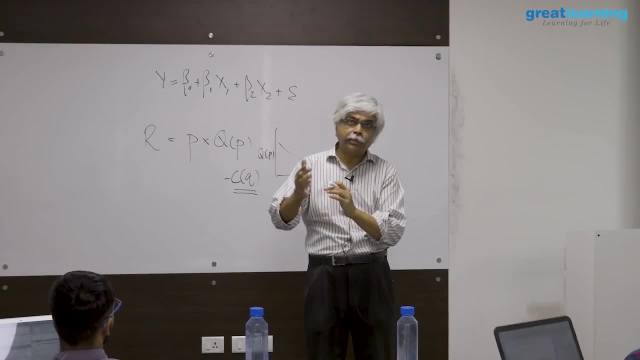 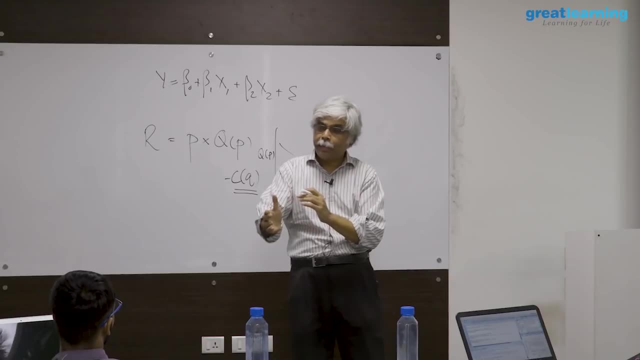 So therefore, I will say that if I need to forecast 15 and 16, can I forecast 13 and 14?? So I will take my time series not up to 14, but I will take my time series up to 12 and 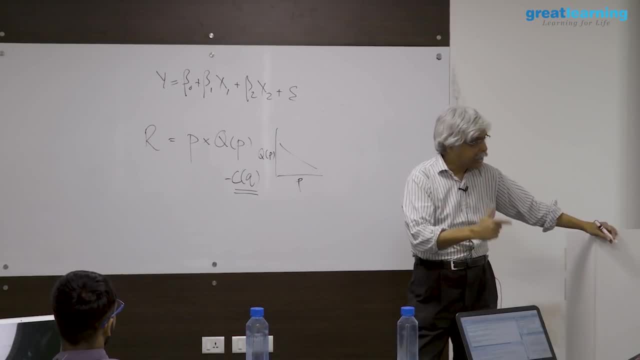 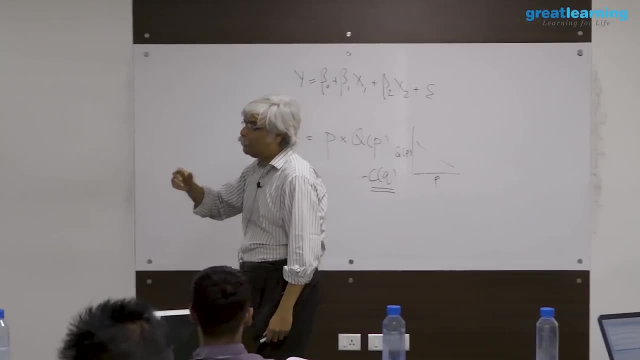 I will build my model or whatever, and then I will say: using that model, can I now predict 13 and 14?? If I do that, I can then trust myself to say that I can forecast beyond 14, if I am sitting at the end of 14.. 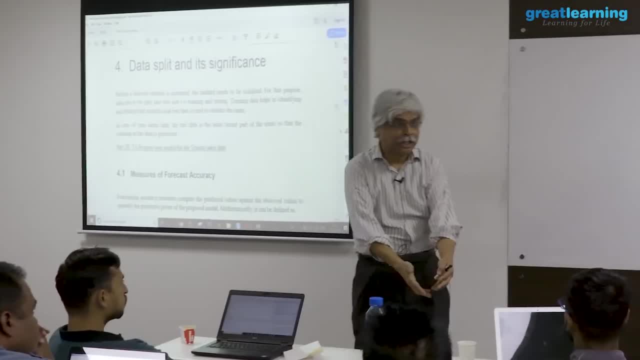 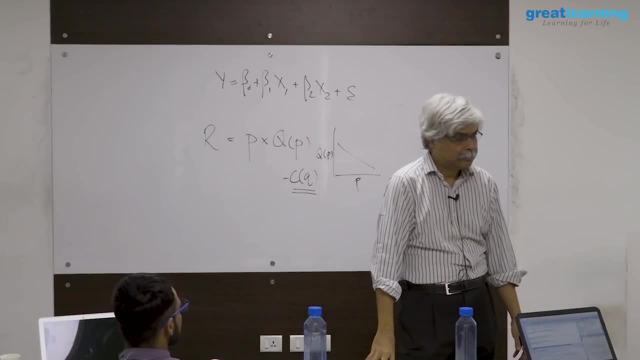 Now 14 is already historical, but you can ask that question now. So if I am sitting now in my company and I am trying to forecast, say, sales for the next two quarters, So I am trying to forecast sales for the next two quarters and I have all past sales. 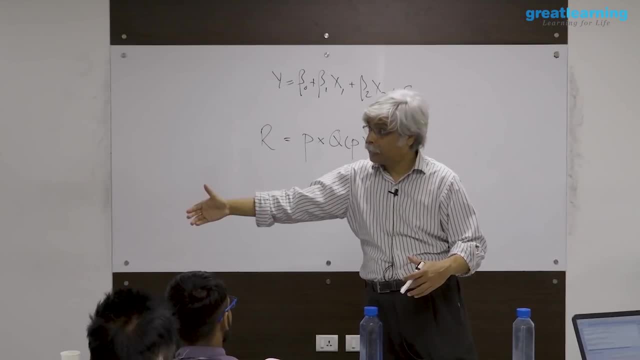 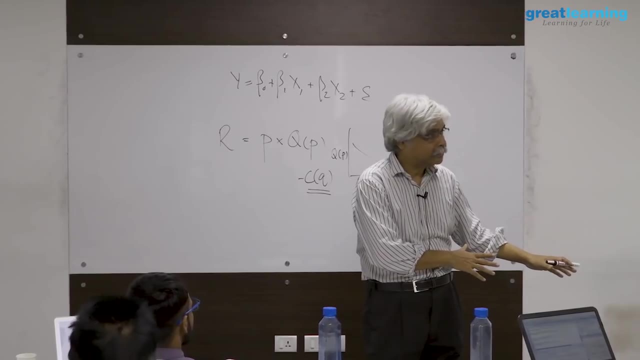 data. How do I know that I will get a good forecast? What I can do is I can take the most two recent sales quarters that I have and take it out of the data set And now look at the remaining data that I have. 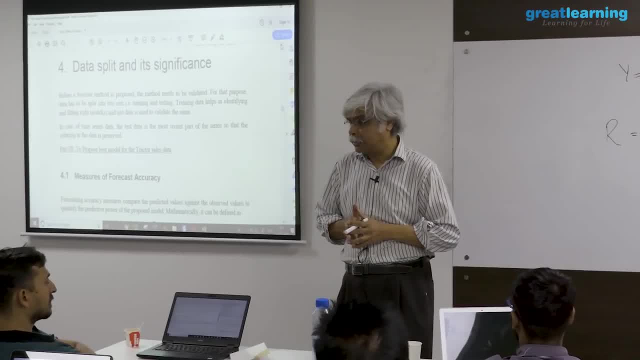 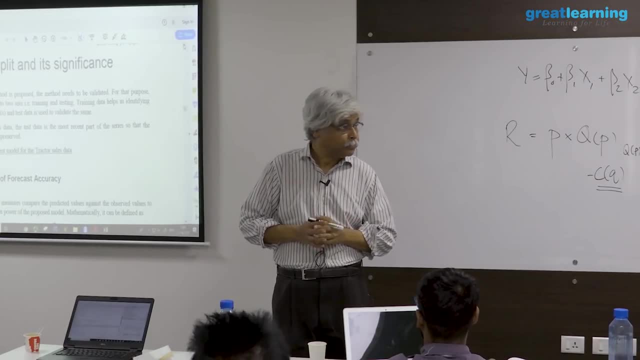 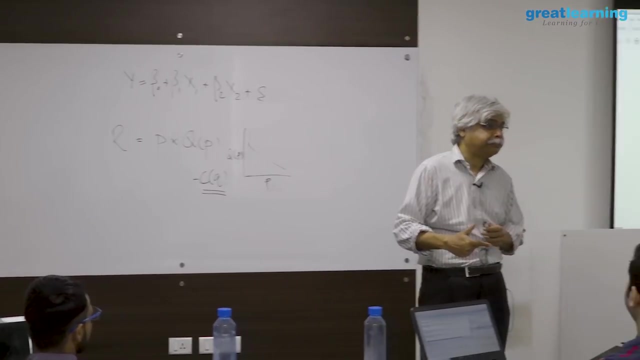 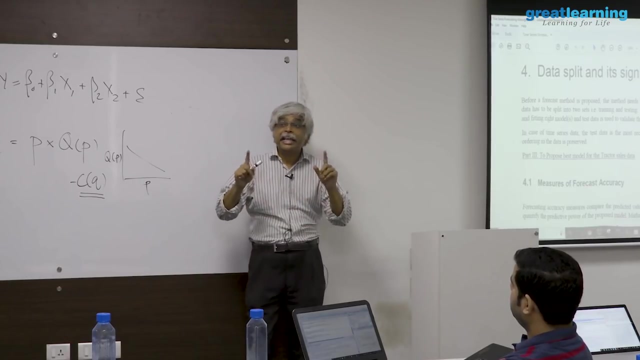 And use it to forecast my two most recent quarters, and if that works, then I can use that to forecast my next two quarters. Now, in order for this logic to work, what assumptions do I need to make? Yes, in other words, I need to make some kind of within quotes sameness argument that these 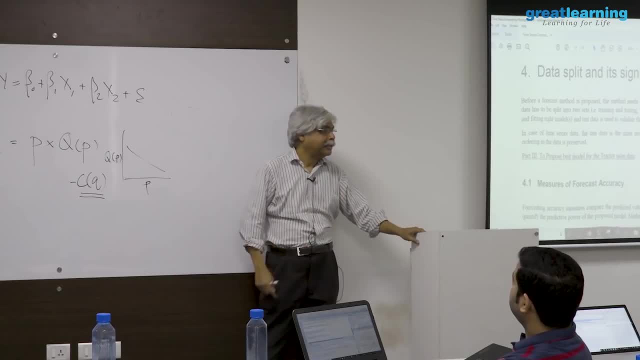 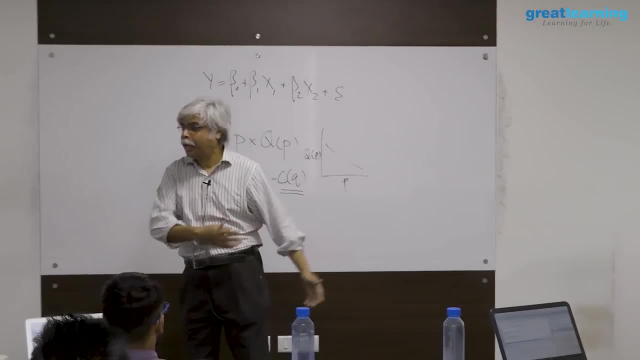 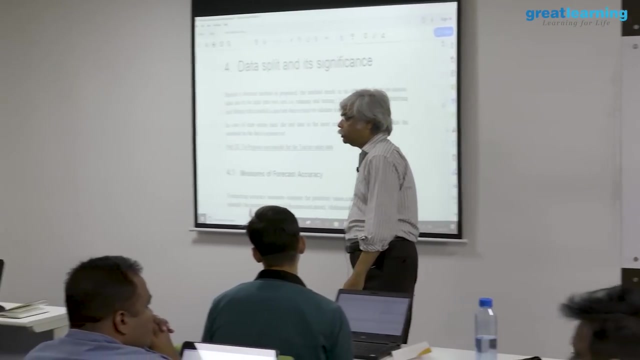 last two quarters are the same in some way, Whereas the next two quarters. something is common between them? Because if there is nothing, then why will the logic carry over? Why will it be that if I can predict the last two, I can predict next two? 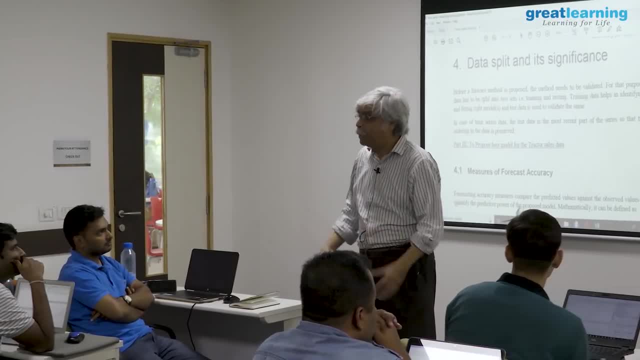 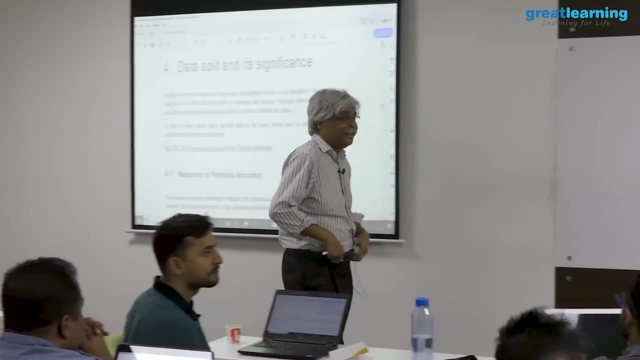 In other words, is there anything common about it? Now you may say, maybe there is, maybe there is not, I do not know Right. Yes, So, sir, you don't necessarily need to assume that the business environment remains the same. 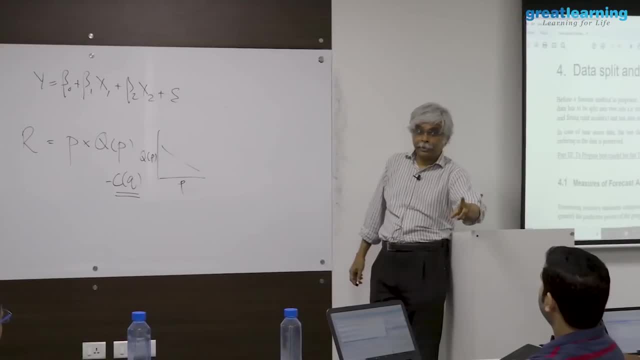 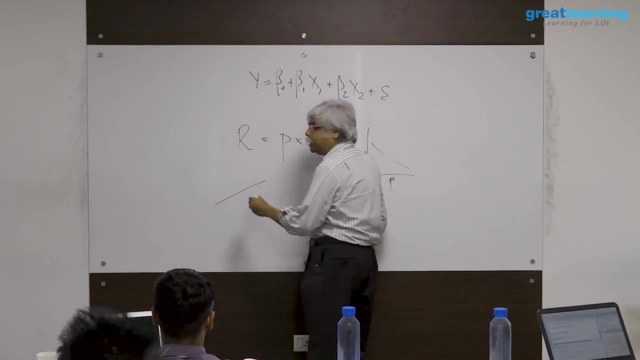 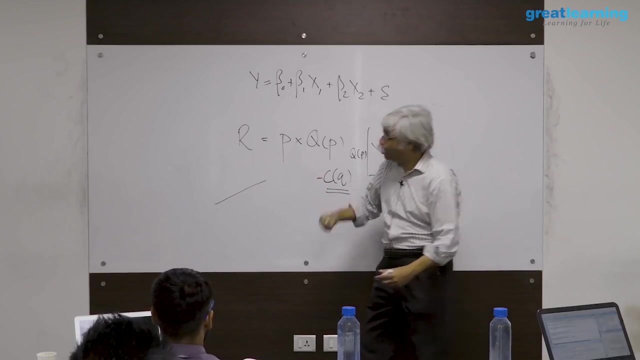 what you need to assume is: something remains the same. now you need to assume what that something is. so, for example, you could say that the business environment is actually continually getting better. it's not the same, but it's continually getting better. so, what is the same now, what is the same. 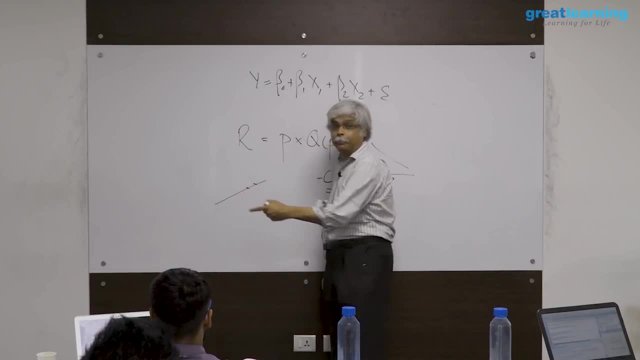 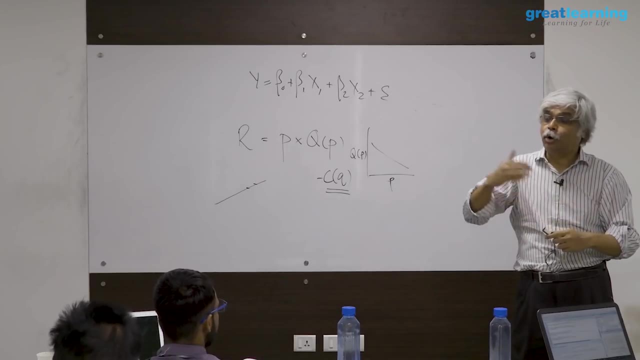 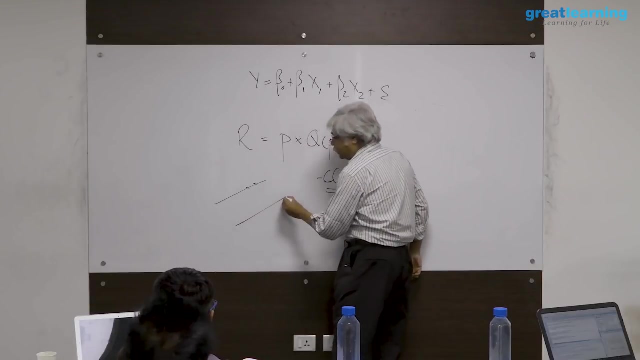 could be that the increase in my business environment is the same. so, in other words, it's getting better, but it's getting better at a constant rate, same as the past. so in other words, my series looks like this now. if my series looks like this now, when I want to forecast beyond it, I need to get a line that 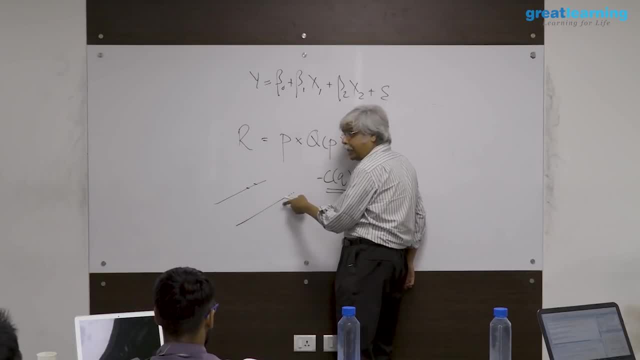 looks like this now. this is not the same. this is not. this is an increasing line. my future is getting better and better, so my forecast should also get better and better. but it should also be the case that if I cut my series here and if I can predict this increase based on this data now, I should be in a position 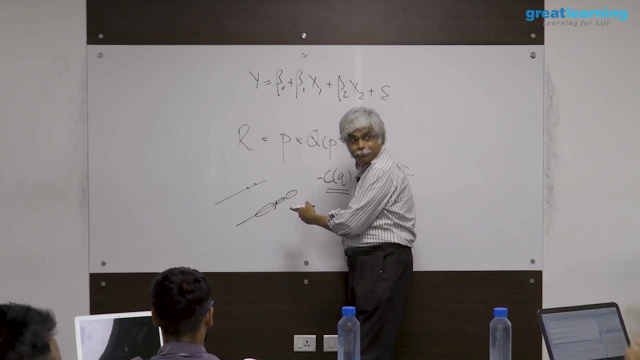 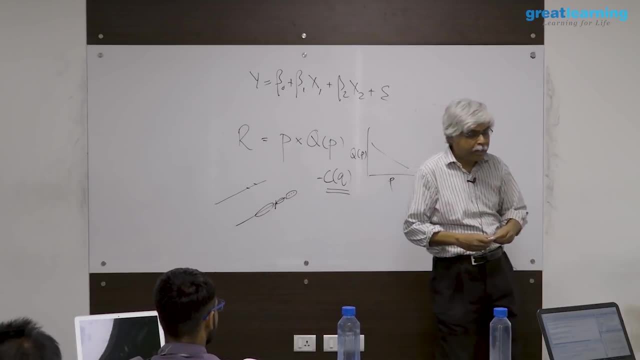 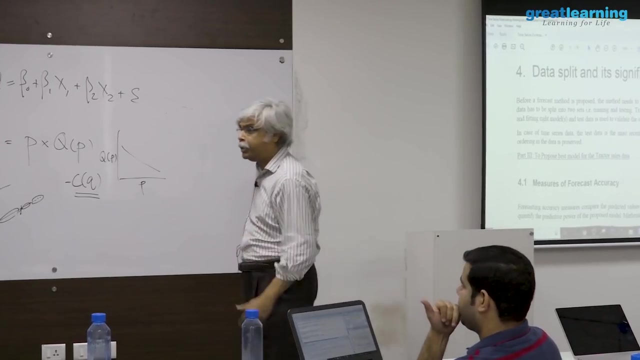 to be able to predict increases. sure, you can do running, you can do running things and we would do that. so, for example, in my, in my former life, in, in, in, in the retail finance business, we would continually run campaigns on things like credit cards and personal loans and things like that, and we would run it in. 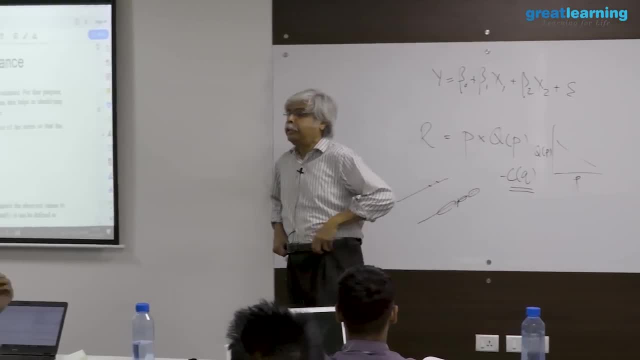 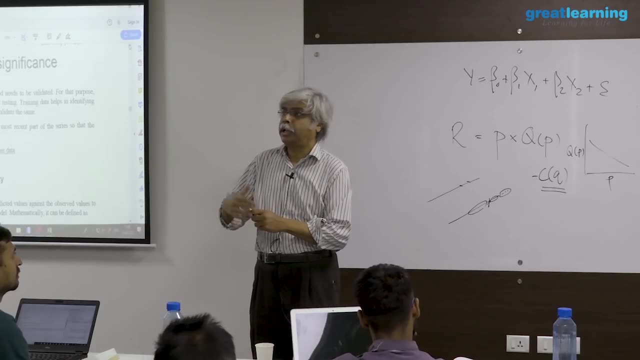 the following way. we would say that I need to. I need to see whether so. one possibility could be that that what do people want in their products? do they, you know? do they want your lower interest rates? do you want lower fees? what is that people want in their in? 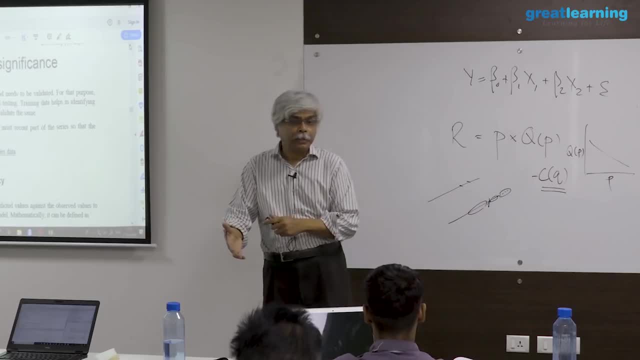 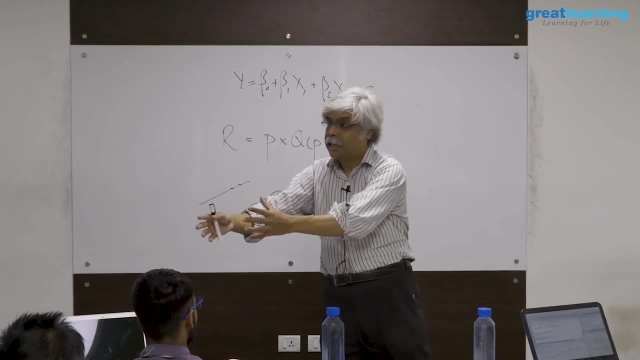 their in their products. now, how was that done? that was essentially done by running what are called campaigns. in other words, some people were given this kind of a product and some people were given this kind of a product, and then they were tracked, and then you would say: who? 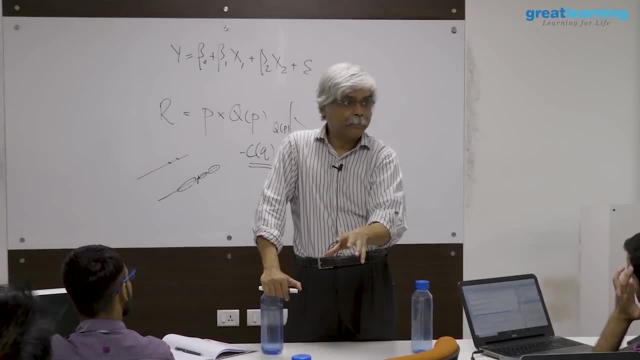 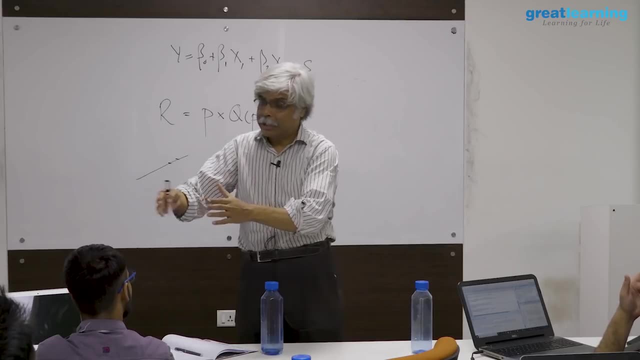 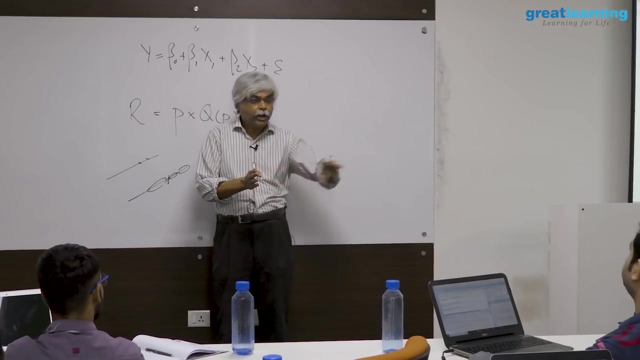 who do better, or where did we get more sales from? and then we would extrapolate that information to say, therefore, this product is doing better and we try that around. but how do I use the data cinemas? how do I know that this product would work? so you look at historical. 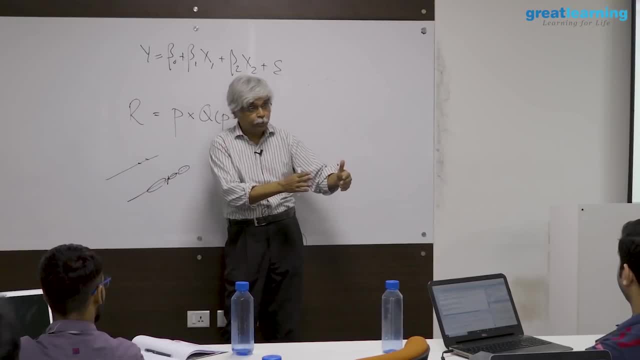 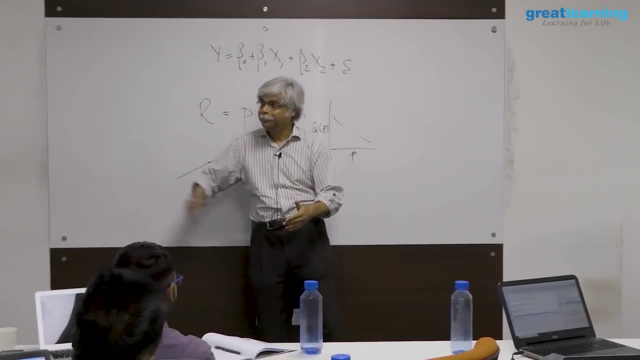 data. you again hold out something like three months. you go three months before you look at the data. now you design your campaign, then you run that campaign for about three months. you see what happens and you keep doing this. you keep doing this over and over again. so in other words, if you do it quarterly, then every 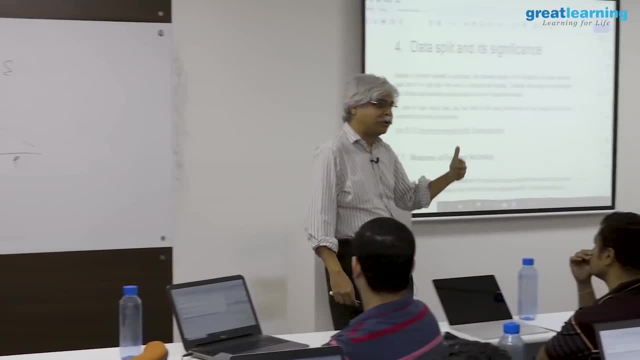 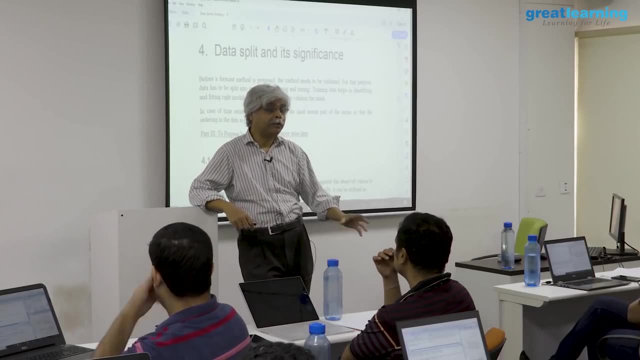 quarter, you're predicting the next quarter, and every time you're doing this over and over again. if you're a professional analyst in the company, you will get used to this idea that any moment in time you're, for example, doing multiple projects. some project you're just understanding the specs, some 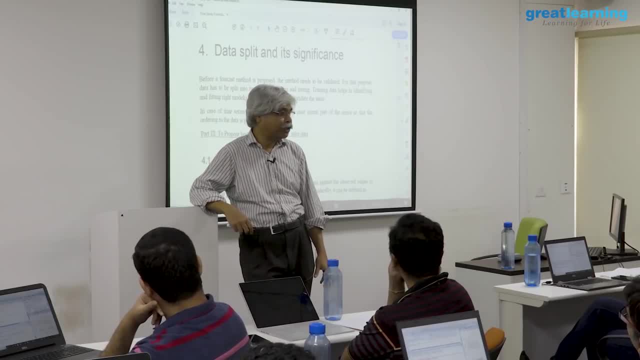 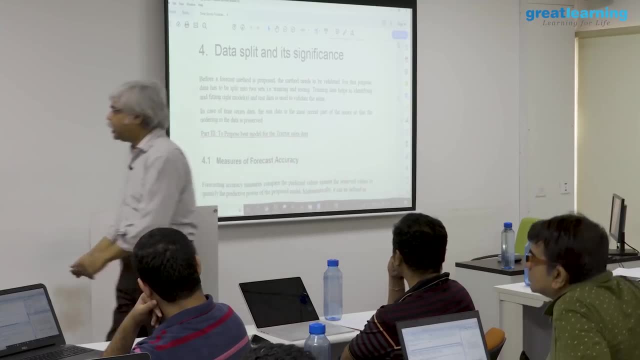 projects, you are doing the analysis, some projects, you writing the report and you finish. you know when you do all doing it at the same time, there's this, there's this paralyzation that happen. so forecasting is not done one-off, so is done in a continuous process. but if the process is such that it manages to pick, 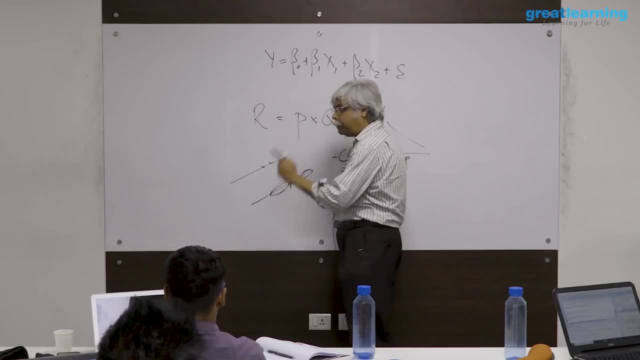 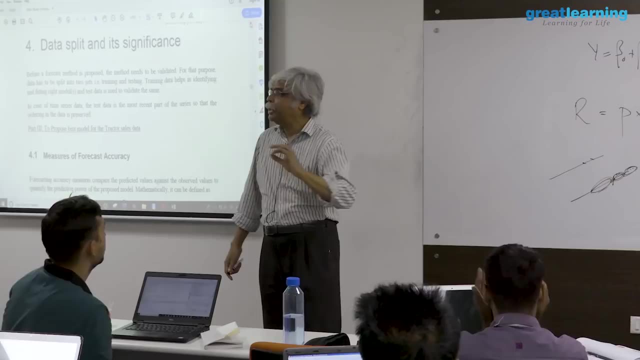 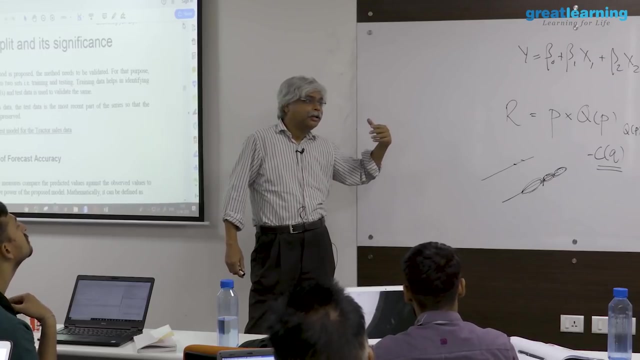 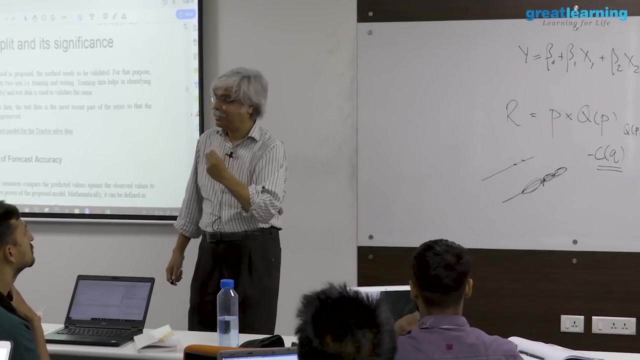 up trends, remember. i do not want repeat. i am not assuming that there is no change in the process. I'm assuming that something remains constant and that constant could be a change. my hunt is not for constancy everything. my hunt **** constancy in something and that I will bite and forecast using what is the same. 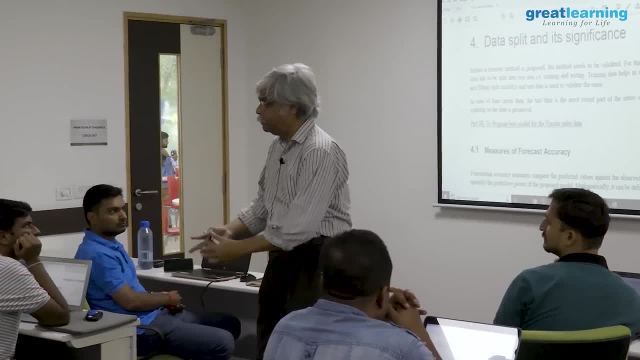 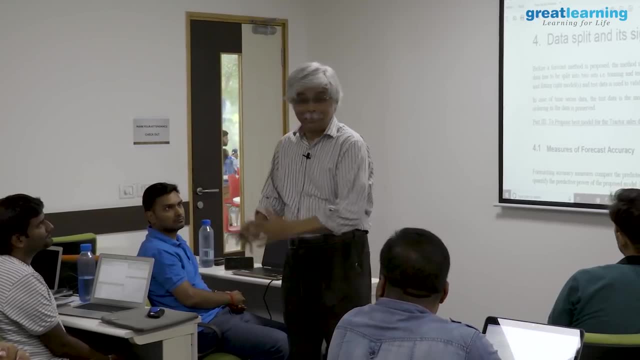 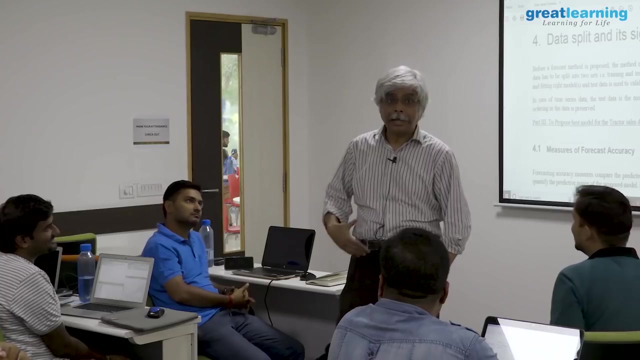 is my. is your salary the same? no, is your annual increment the same? maybe yours is the same. maybe he's real. he's very honest about these things. so what is what is the same? now? what can I predict? can I now? can I now? so if he's his? 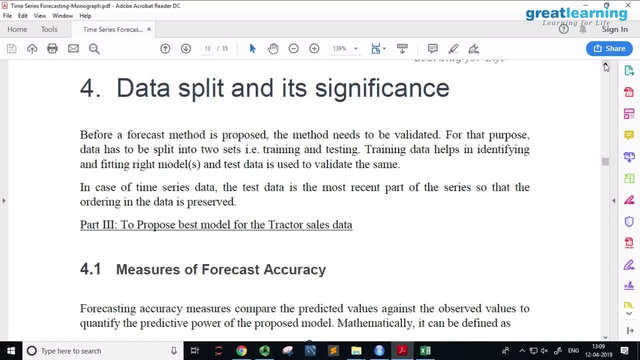 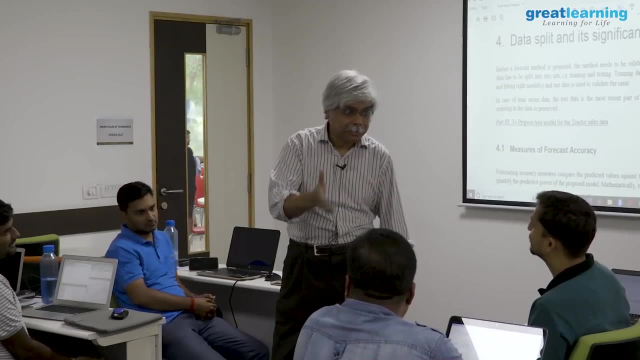 interesting question to us. if he is kindly giving you the information that his salary is not the same but his increment is the same, he's giving you this information. with this information, can you predict his salary next, next year? how? multiply what with what? yes, but why did you multiply with the? why what? 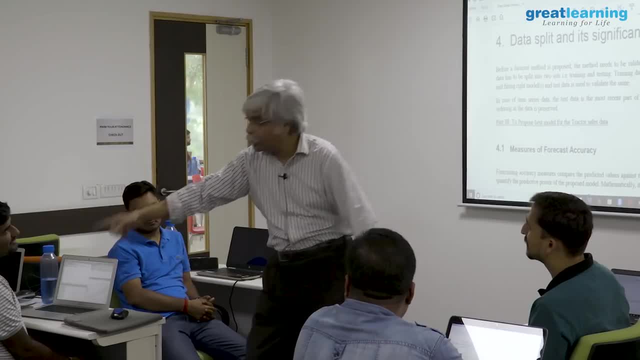 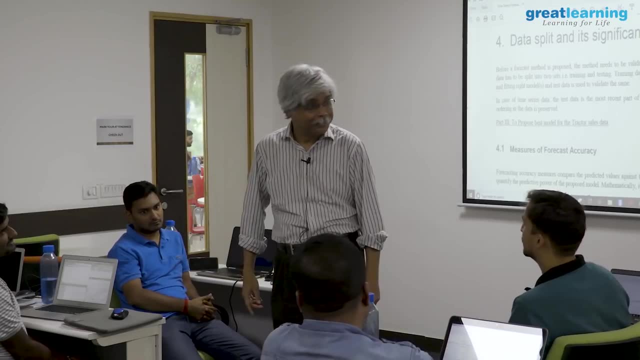 allowed you to multiply with the increment, because that's the constant. he told you that that is what is not changing. he didn't tell you that that is what is not changing. he didn't tell you that he salary was the same. he didn't tell you the salary was the same, but he did tell. 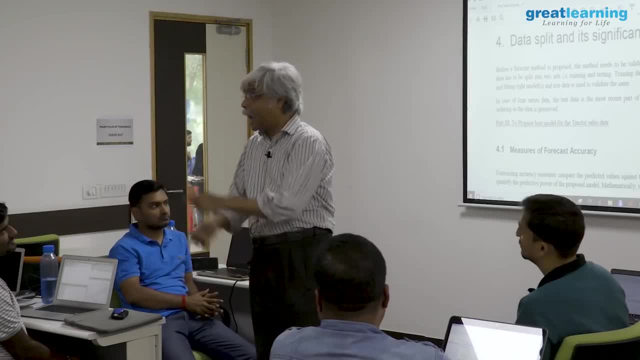 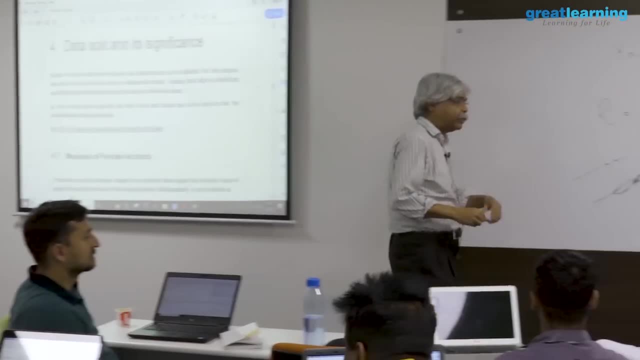 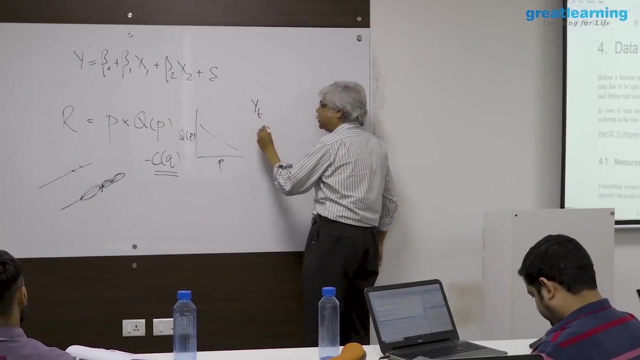 you that the increment was the same and that information you took and applied to the next time point, so it doesn't have to be constant. in fact, what we will do soon, probably tomorrow, is we'll ask the question: should I look at YT, which is my time series, or should I look at YT minus YT minus 1, which is the first difference? 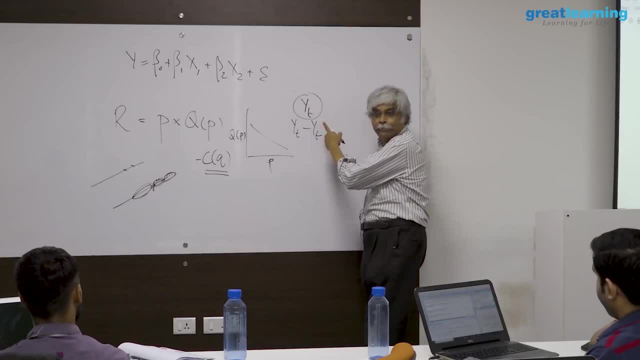 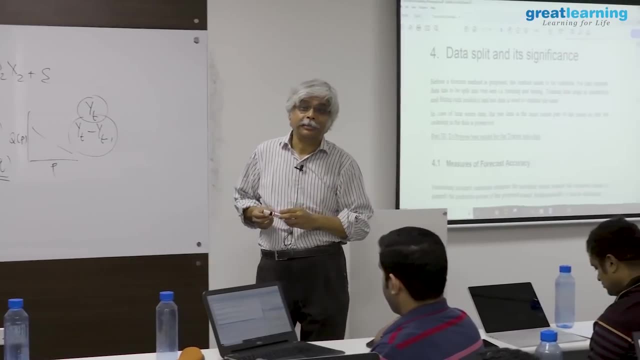 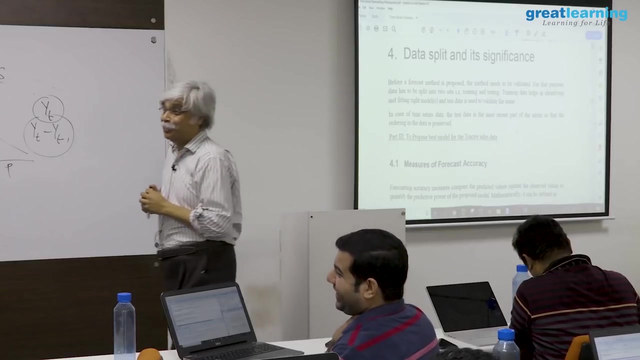 in my time series. is this the thing to study? is this the thing to study or is this the thing to study? is the series constant or is the change constant? it's like management philosophy, right, the only thing that's constant is change. this is the analytical version of that, the only. 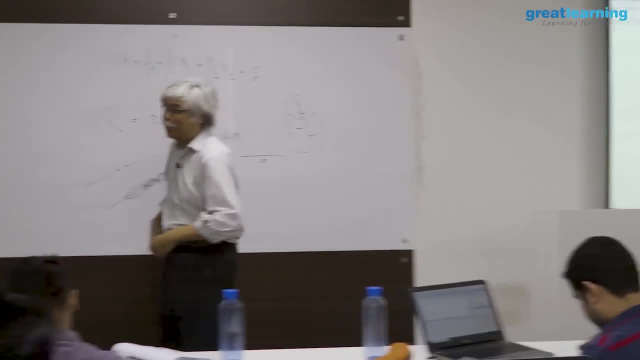 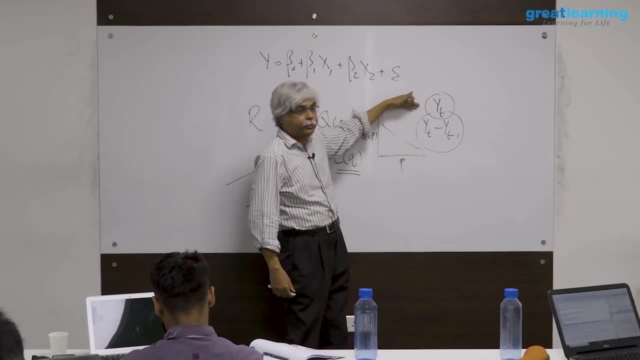 thing that's constant is change. change is the only constant anyway. so we will do that. we'll build a model in which we will study this instead of this, because we believe that this is what is the same, the change is what is the same. therefore, the change 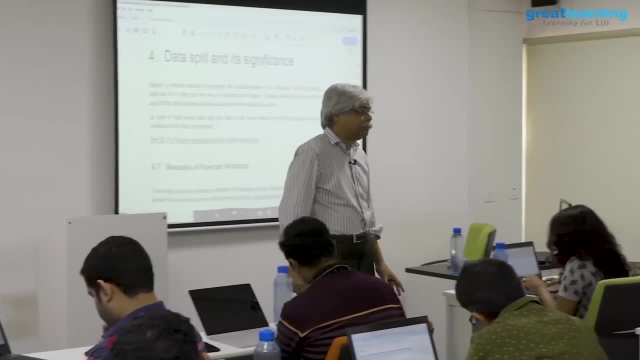 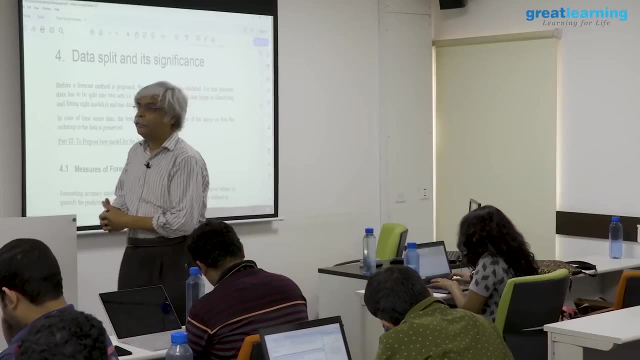 model can be used again. therefore, the change model can be used again and you can do forecasts based and you can do forecasts based on that. as I was explaining, I have a six and a half year old daughter, so when we buy her clothes, how do you think we buy her clothes? how do we size her? 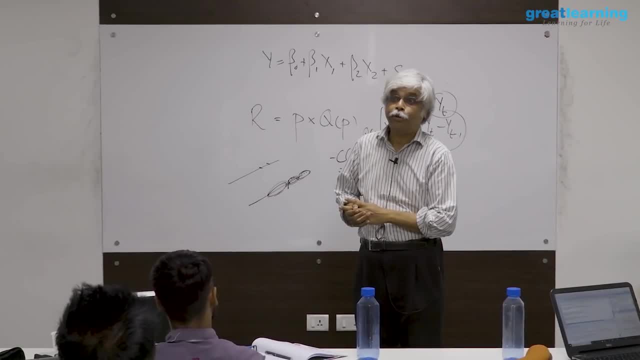 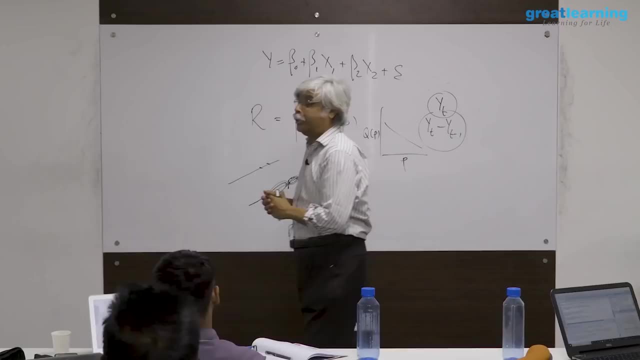 clothes. those of you have kids, you know this. how do you buy clothes for growing kids? what size do you buy? ha, so, so, okay, we have a question here. what do you think about that question? okay, so you, so what is your prediction here? she'll grow, so and your size, your, your, your. 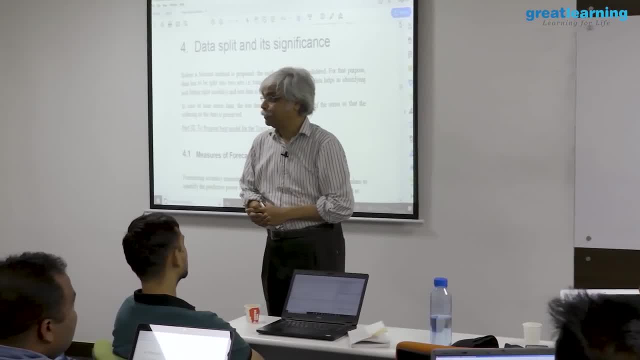 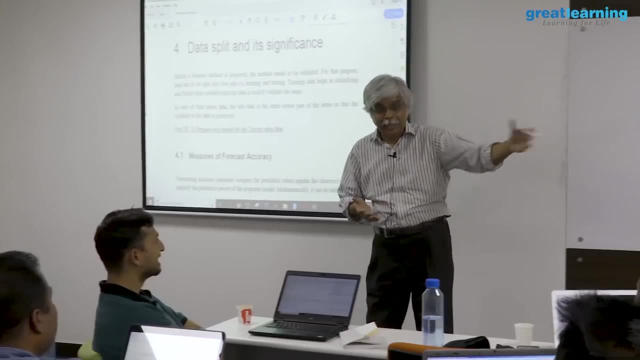 your clothes are fit to what forecast. it depends on how long you expect that to last, right? so if we expect it to last for one year, then yes, t plus one. if you expect it to last a month, depending on what you know, the child, I suppose, if 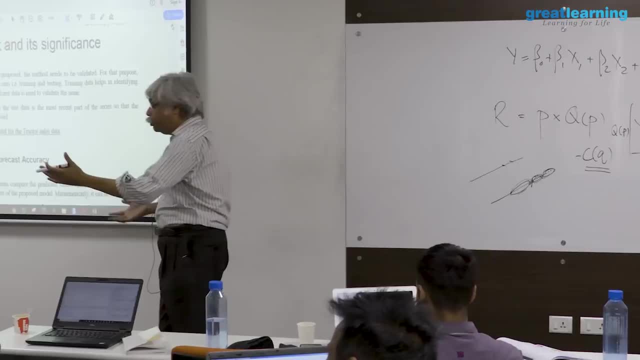 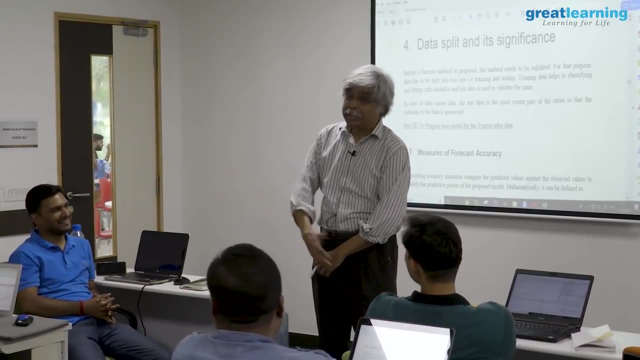 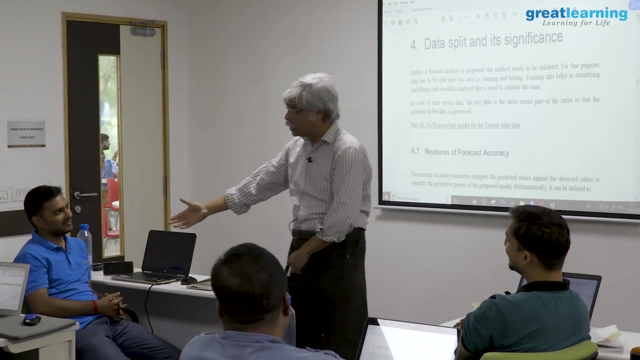 it's a very destructive child, or is it happening? so you do that now for you. would you do that if you buy your clothes? you would you do exactly the same thing. you do exactly the same thing when you buy your clothes. if he buys his t-shirt. he would buy his t-shirt with the expectation that he'll wear it for a 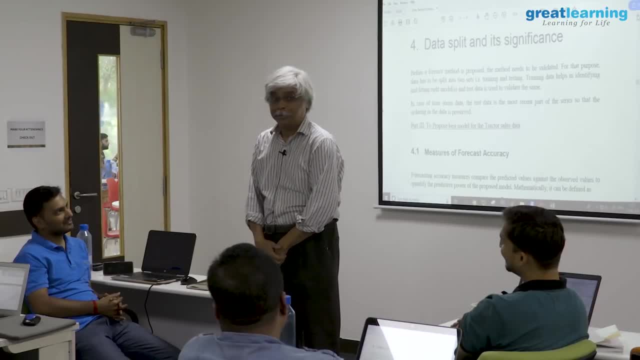 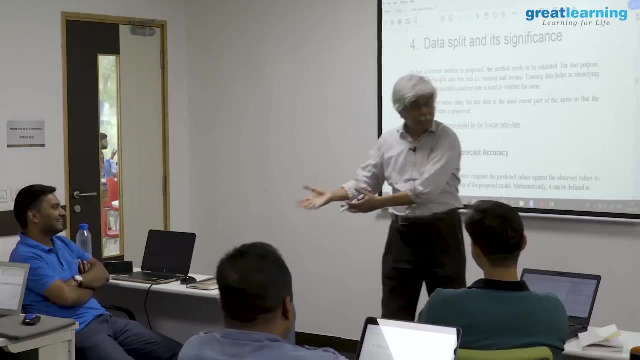 certain period of time. the only difference is that he doesn't expect to grow. well, he might. I don't know what he eats, but but, but, but but. so the difference is that in both cases you would expect the clothes to last for one year, but in one case 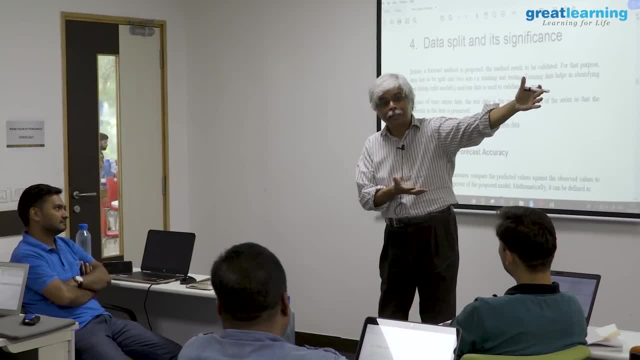 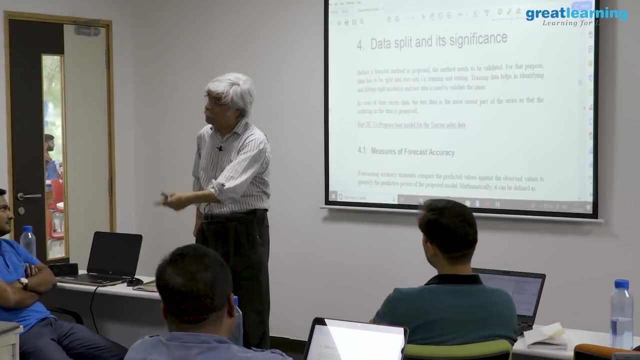 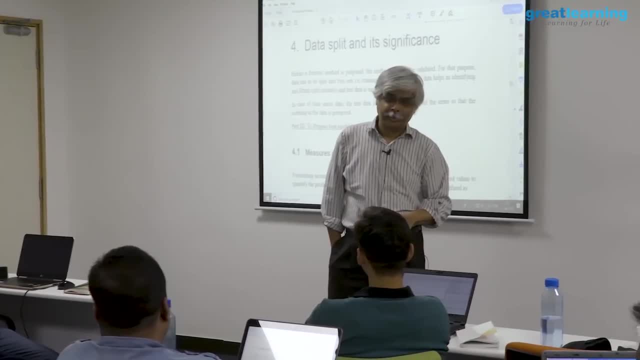 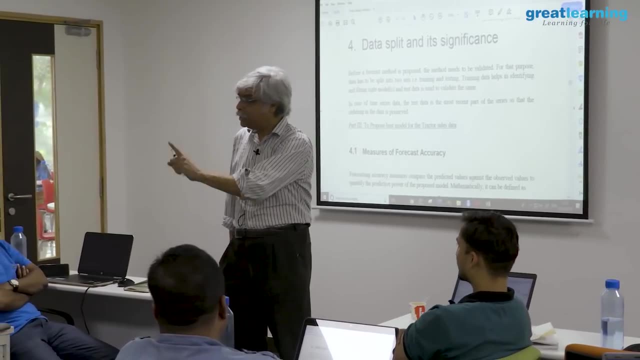 pretty good idea as to how she is growing. it was you know was. I can have a pretty good guess that a year from now how big she will be. so I'm not saying that there is no change in her height, but I'm saying I know something in her. 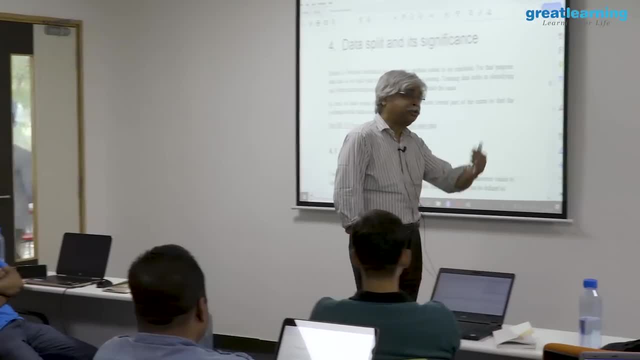 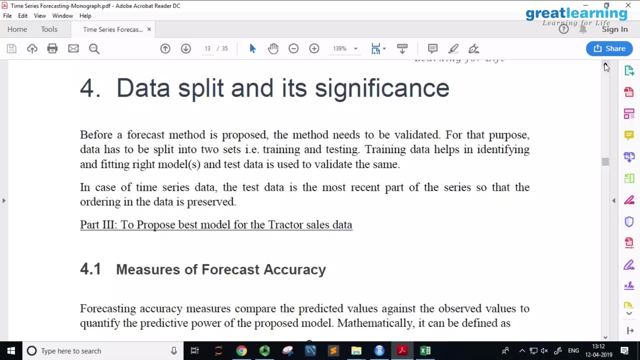 height is predictable. maybe she's going linearly, maybe she's going quadratically, I don't know. I don't do these things with my daughter, but you know so. but there is a systematic nature to her growth and that's all I need to be, that's all I need to be able to predict. yes, yes, so I'm trying to find. 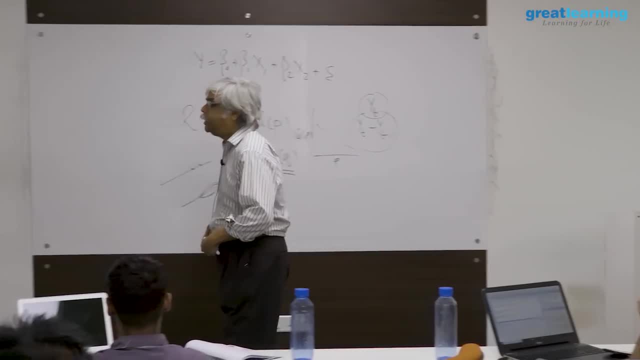 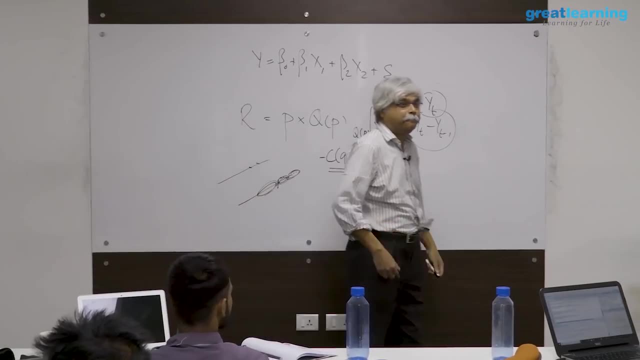 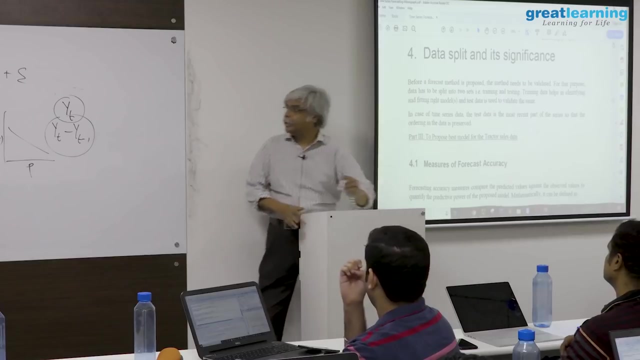 the change that I'm aware of, not aware of. I'm trying to find the change that I think will happen again. hmm, yes, yes, yes. so that's a very important question to us. so in a business, so in a business, let's say that something like uber comes in, etc. etc. 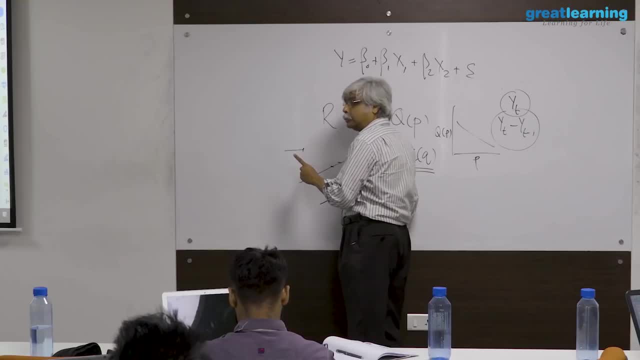 where would that go in a forecast? so there are two ways to do that. one way to do that is to say that I will anticipate someone like an uber will come in and I'll recognize for it. the other way of looking at it is that I do not know what. 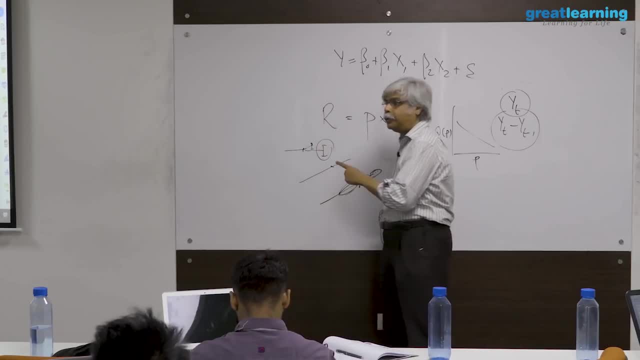 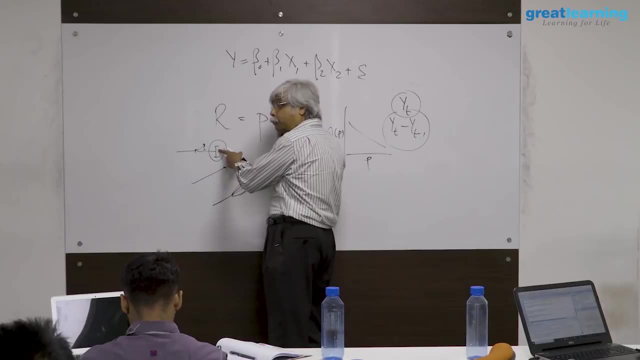 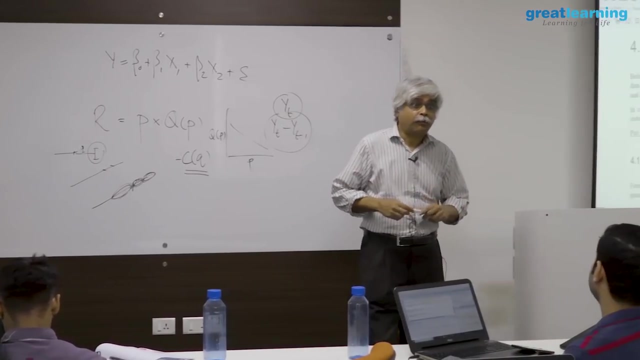 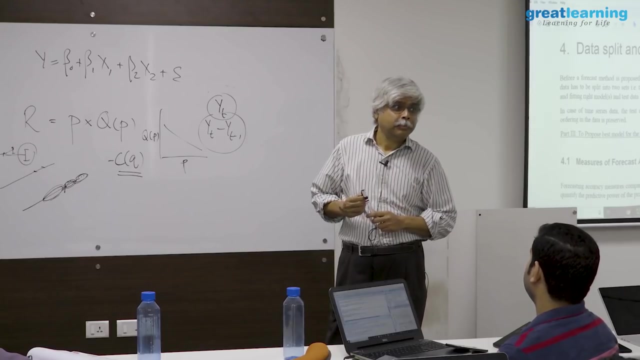 to anticipate, but I will run my business as if a change like that will happen. and now, what does that do to my business? what that does to my business is it doesn't change my forecast, but it does change the uncertainty around the forecast. yes, for example, what is jet situation doing to Indigo? so now what is? 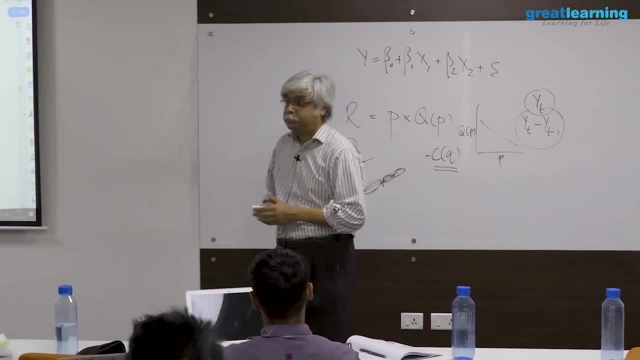 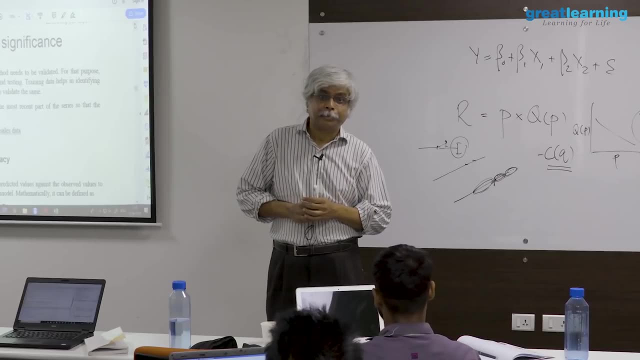 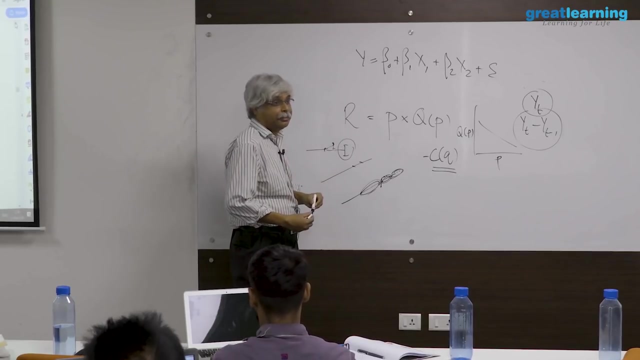 happening to Indigo sales forecasts? it's increasing right based on something that is not in their own time series. so, but Indigo's managers- or whoever would be capable of managing around that any good manager would be- they would have backlogs of planes. that backlog can. 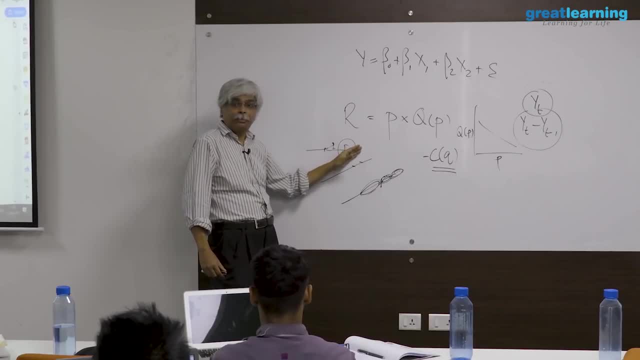 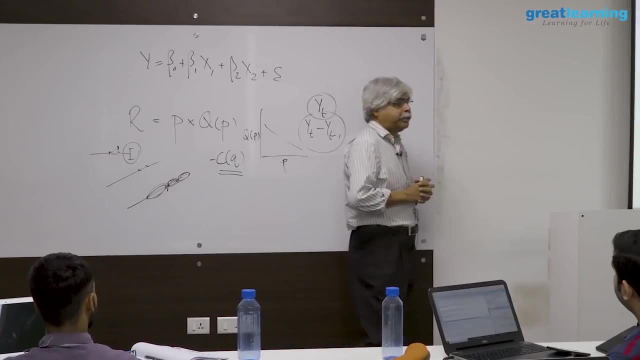 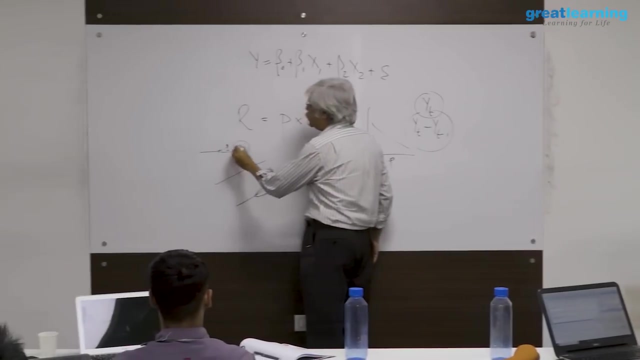 be shifted back, brought forward. many things can possibly potentially be done. that doesn't mean that people do not anticipate these situations. they do. right answer though these memes going around: yeah, you had some question you had, you had, you had some uncertainty to it. now, and that is a part of your to. 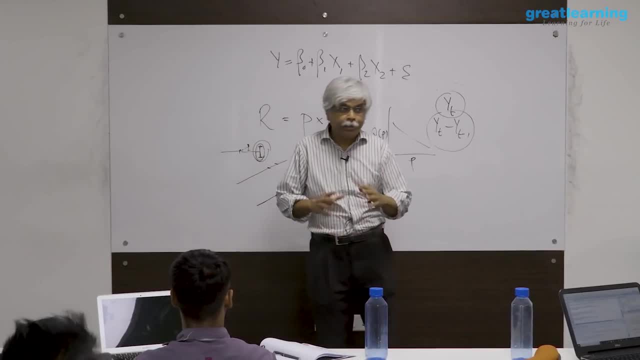 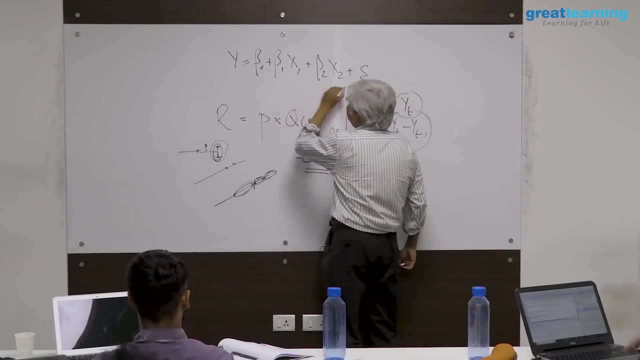 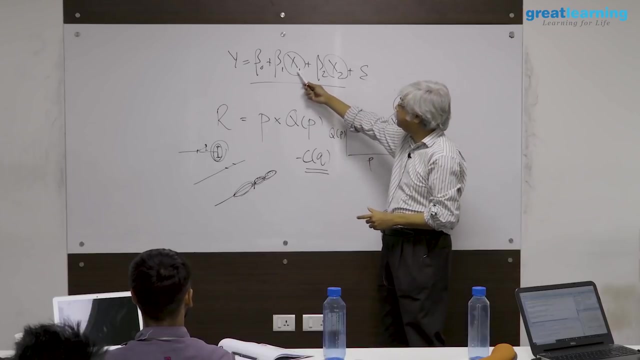 some extent, your management expertise? yes, the similar question is this. so, for example, you could have asked this question in time series as well. let's say that your model like, looks like this, and now you are going to put in a different text in a different way. now, when you put in a different text in a different way, 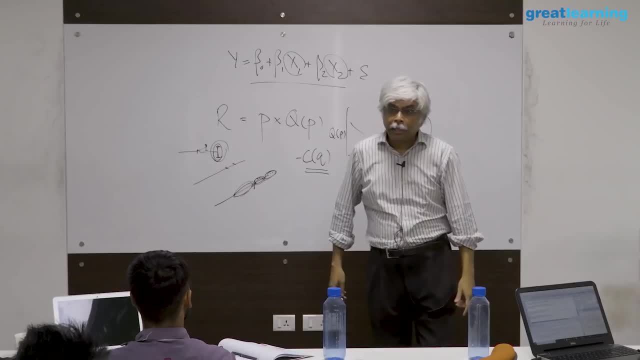 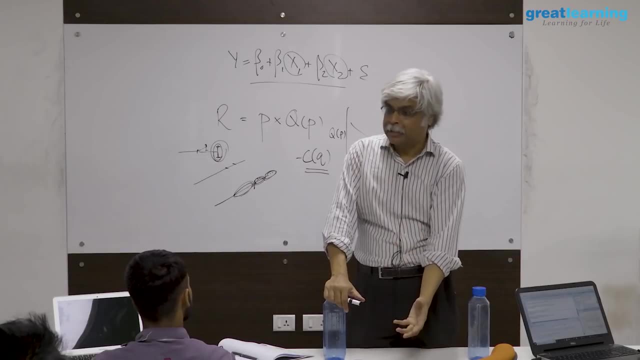 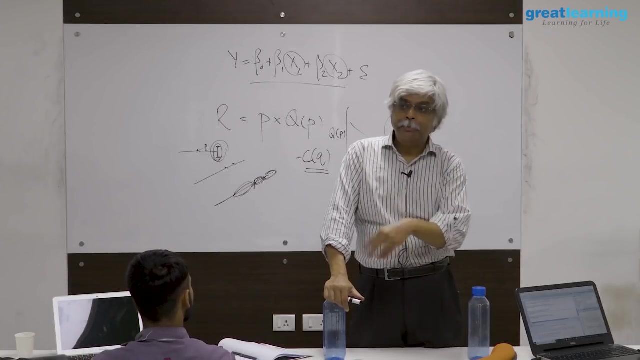 how do you know that? why is going to react the same way? in other words, let's say that I let's say that, in that that jet now drops prices, how does it know that at that drop price, at that change price, it will see so many increases in flyers, just like in time series when time changes, the 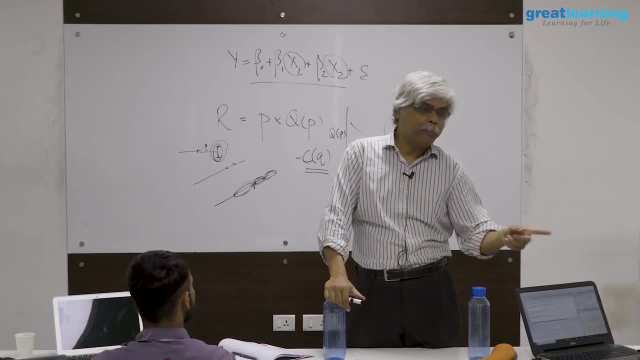 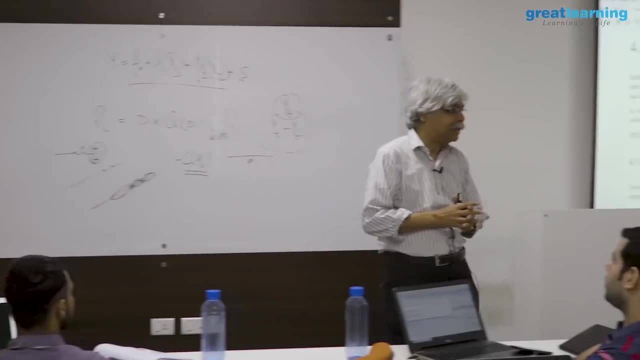 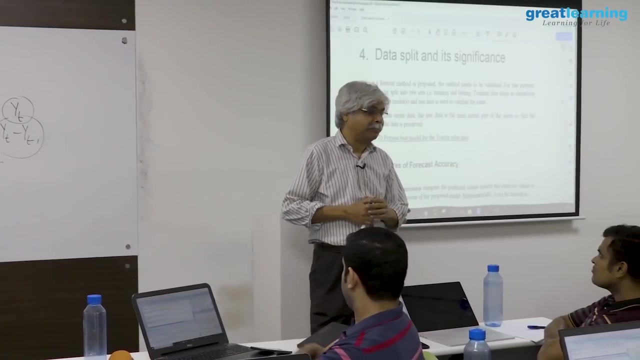 situation becomes unpredictable in regression. also, when your input changes, the output becomes unpredictable. it says that it's a little hidden there. it's not that that obvious, but but that problem exists everywhere. it's not just a time series problem or a statistical problem. it's a broad analytical problem. that how? 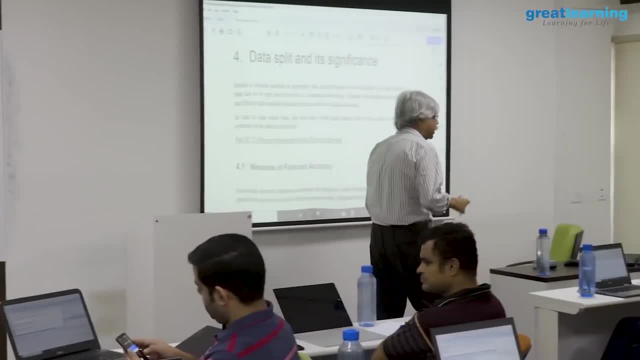 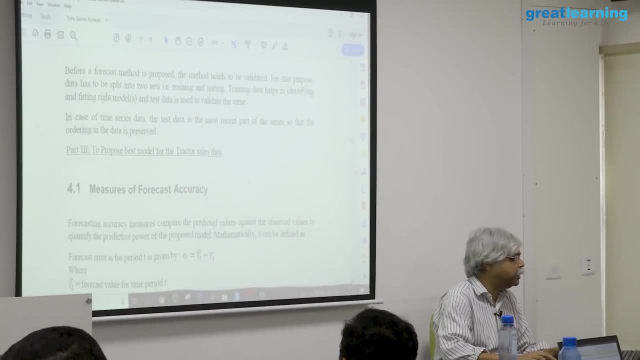 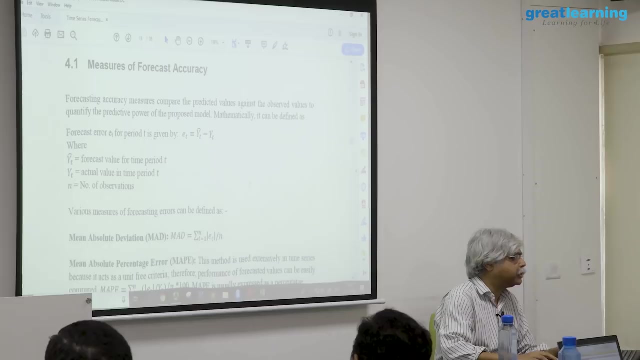 do you account for that uncertainty? and so one simple way of accounting for that uncertainty is as we had done, or as you had done, is to build models that allow you to explicitly measure it, so to speak, sort of measures of forecast accuracy. so, for example, let's suppose that YT is the object that you're trying to forecast. 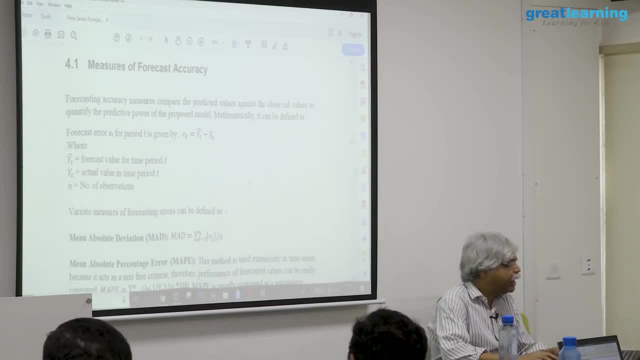 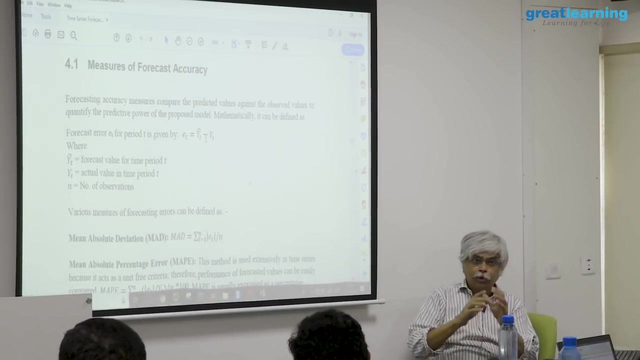 now, YT is the unknown value of the response and you forecast it or you've got a predicted value of it. as YT hat statisticians like putting hats on top of things- which is you know which is the estimated value or predicted value. this is therefore an error. ET is therefore the error in your forecast. what you forecast. 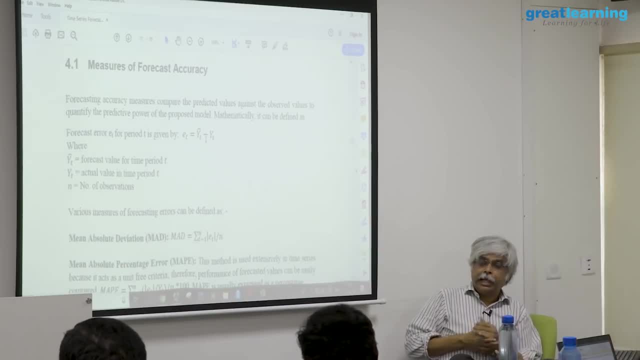 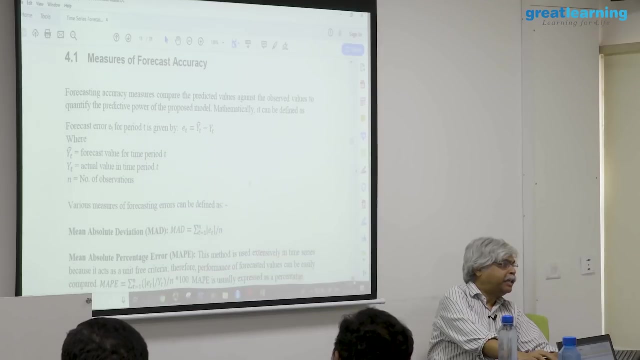 minus what the actuality is, and you want ET to be small. you want ET to be small in linear regression. you actually minimize some ET squared, which is what we'll be seeing again now. there are various measures that can happen here with. with respect to that one measure is you have what is called mean. 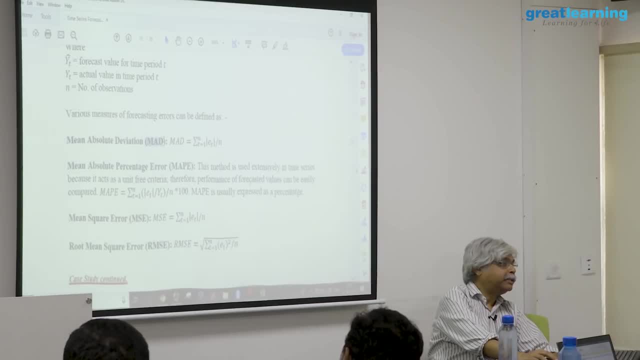 absolute deviation, who helpfully summarized as mad huh. so what is the mad measure? it is the absolute error that I make. so if I, if I am, if I am, say two units above and then I'm two units below the two units to use, don't cancel out, I'm wrong by two and then I'm wrong by two. 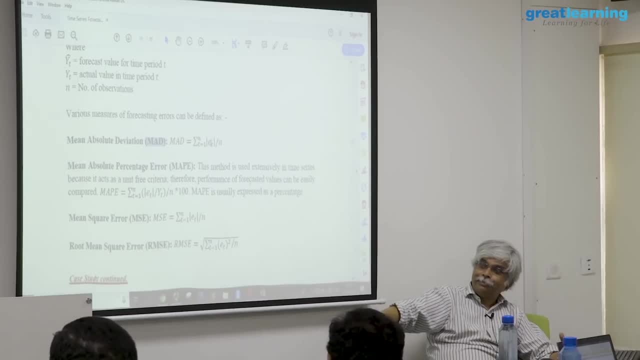 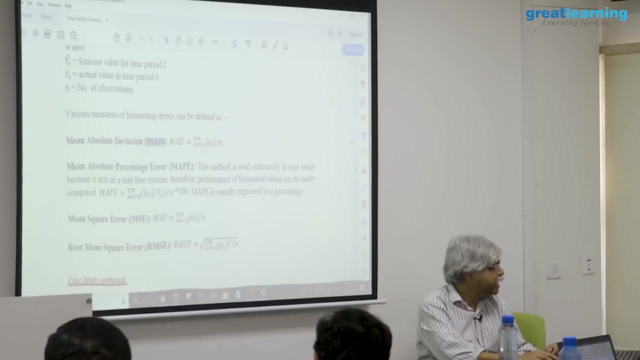 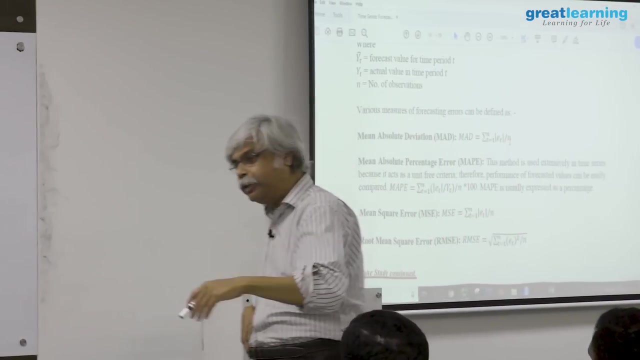 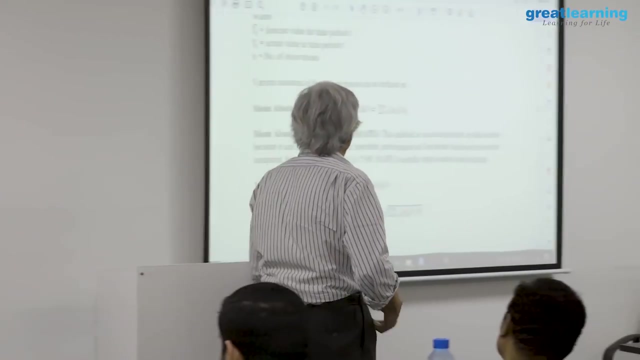 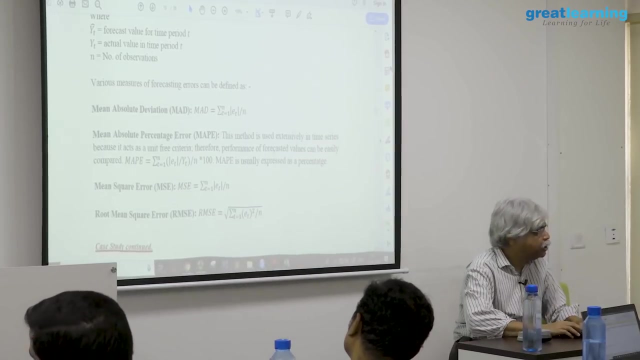 again, INQUIRY HereGuide MINOLA, INQUIRY of all factors. why is that absolutely INQUIRY, FINAL INQUIRY also 2 modulus. absolute value of minus 2 is also 2. so absolute deviation deviation is what? deviation from the actual YT is a deviation? ET is a deviation, a deviation. 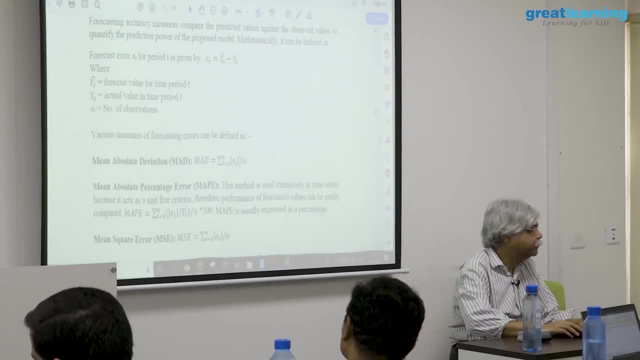 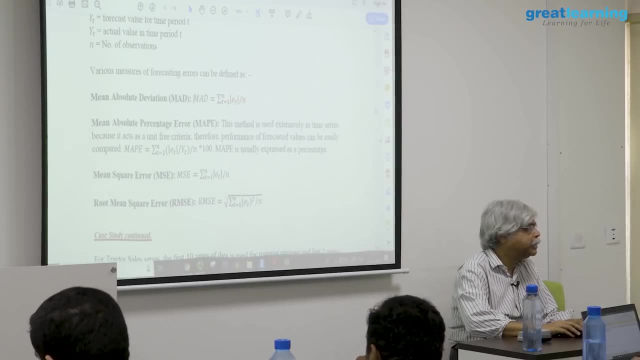 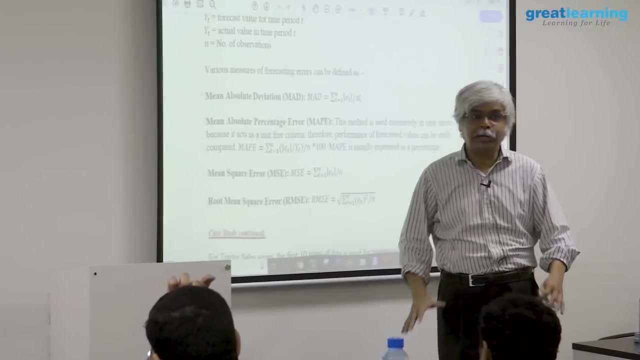 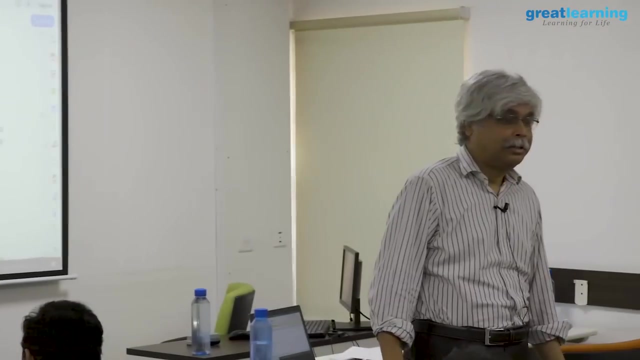 of what deviation of my forecast from my actual? there's a slight problem with this that makes it less useful than you think. is that? how do you know when this number is large or small? suppose I tell you that on the average you are off by 10 units. is that off? is that a lot? is that not a lot, or it's contextual right? 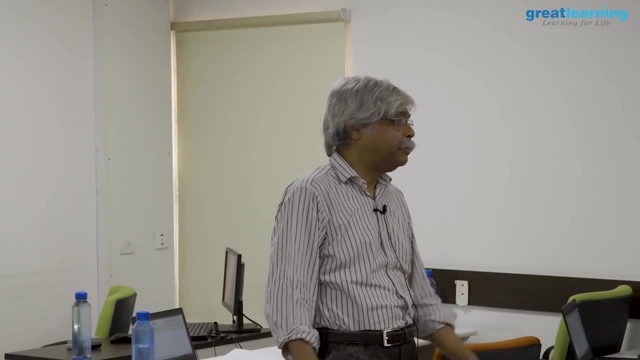 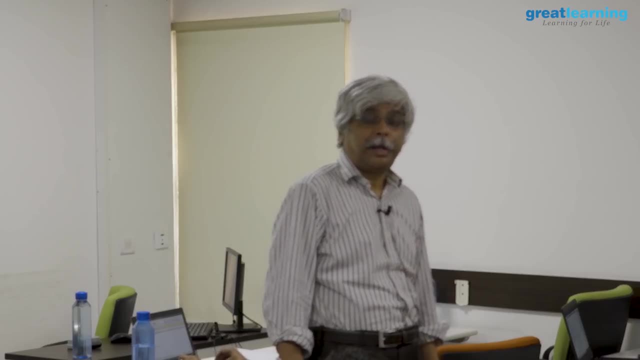 you don't know if you are buying. you know a plot of land and you're off by 10 rupees. you're very, very accurate in your forecasting, right, if you are trying to estimate the number of mosquitoes in your bedroom and you're off by 10? that's. 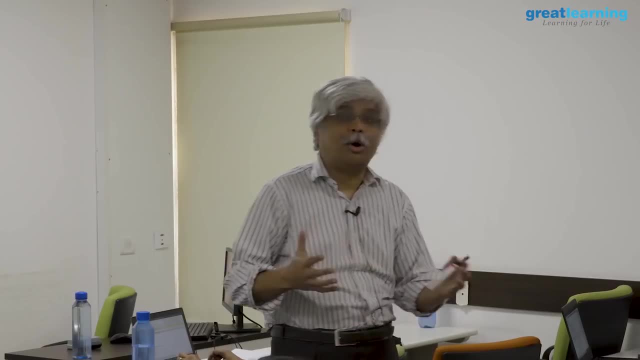 something that you are off by 10 units. you are off by 10 units. you are off by 10 units. a lot of pain. so you don't know. you don't know what plus plus 10 means. so what this is often done is: this is normalized by the actual. is written as a: 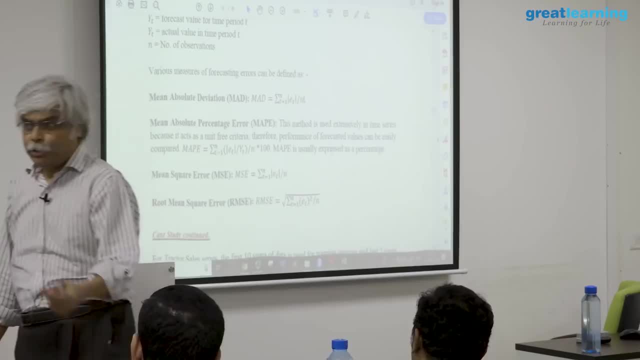 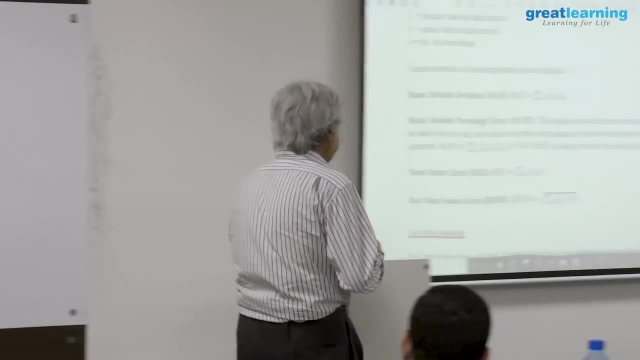 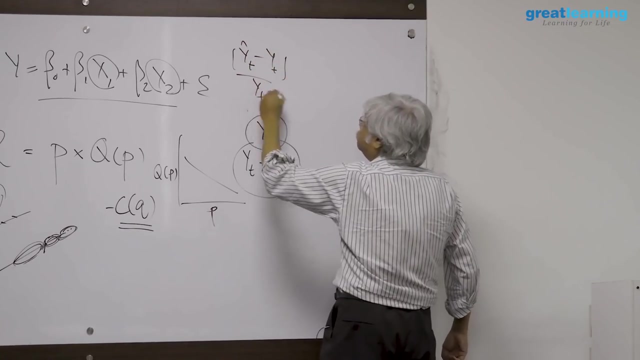 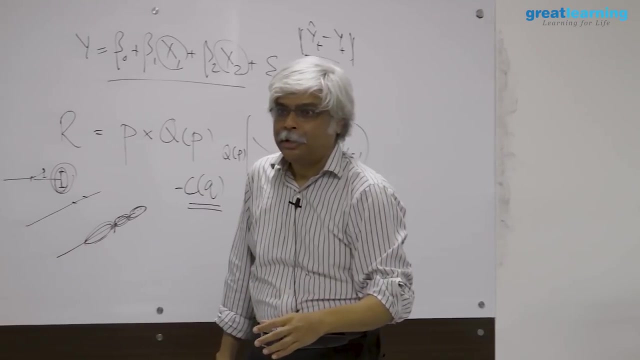 percentage. so 10 as a percentage of money or 10 as a percentage in number of mosquitoes. so now what you do is you look at the difference between this. so you look at essentially this. you look at YT hat minus YT divided by YT, so this will look like a percentage: 10% error, 20 percent error, 6 percent error, whatever. 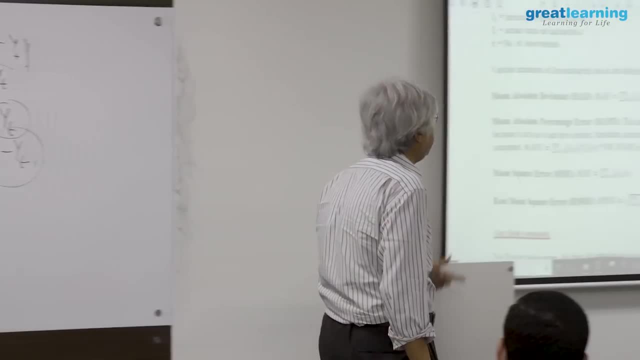 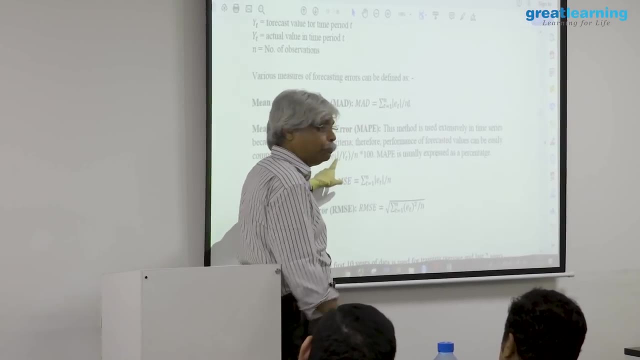 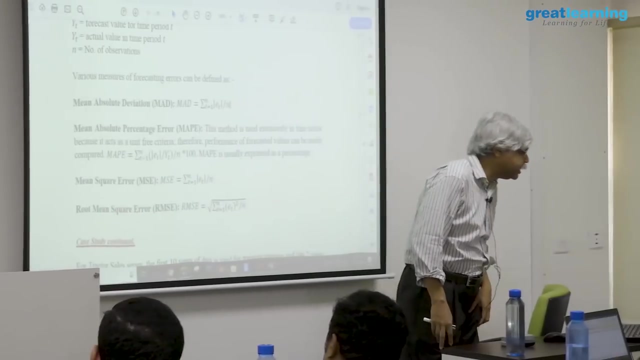 it is that should be. this is called mean, absolute percentage error. why is it a mean? again, it's an average of what of absolute percentage error. why absolute positive and negative are both errors: percentage because is written as a percentage and error because in this case it is used written as an error and 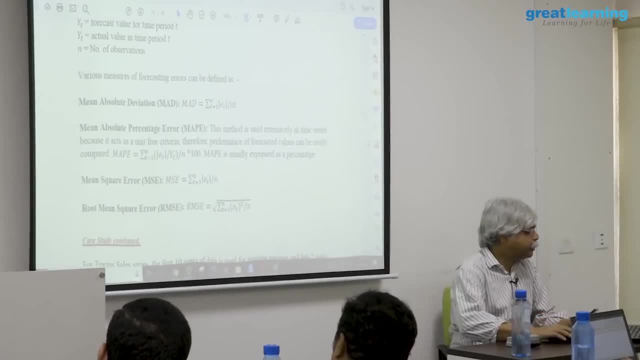 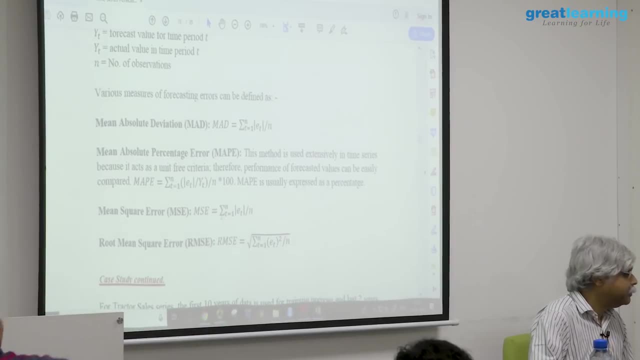 not a deviation. the third way is mean squared error. there's a, there's an error in the formula. this should be a square. so mean square error is exactly what you know. summation: ET squared by n and on the root mean squared version is the same thing with the square root. why the 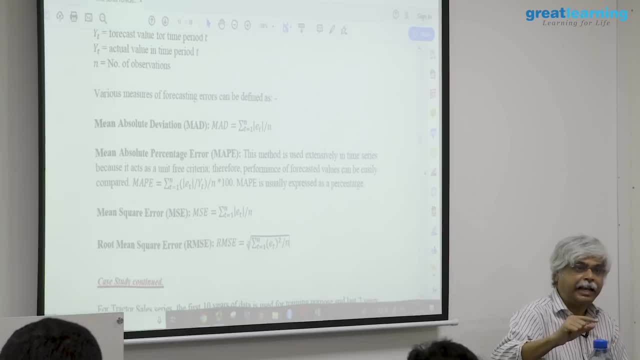 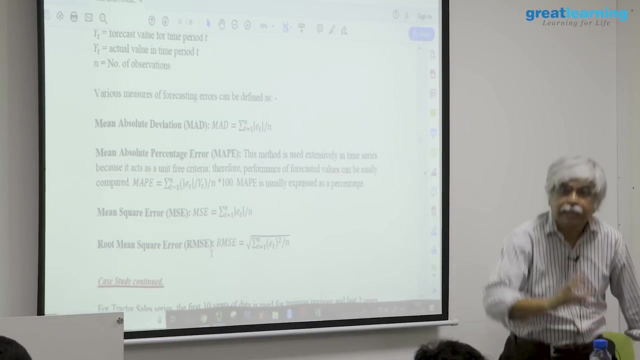 square root, because this square root is now on the same scale as my original value. so these are the two that we will mostly use. we'll look at the mean absolute percentage error. it will give us a number as a percentage. we'll also look at the root mean square error, which will give me my error like a standard. 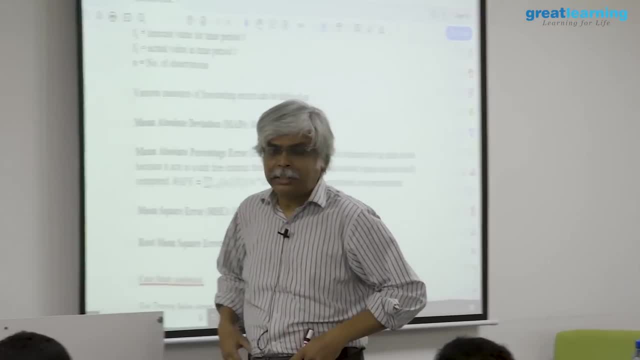 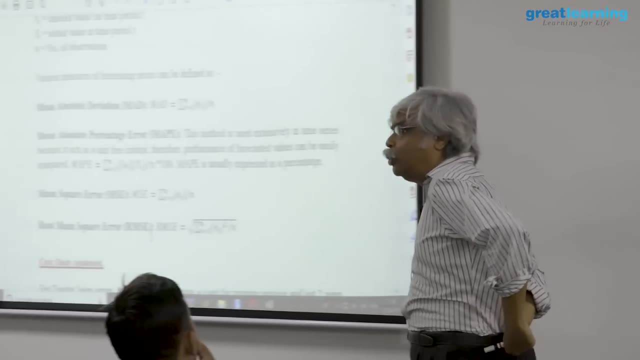 deviation. so if I give you a root mean square error, for example, let's say that I tell you that my forecast. as an example, let's say I'll give you that my forecast is 20 with the root mean square error of 2, that is roughly saying. 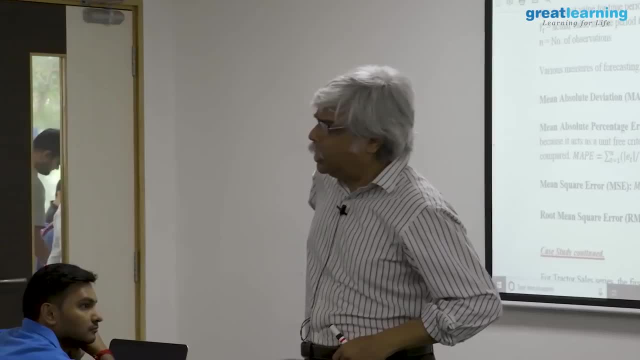 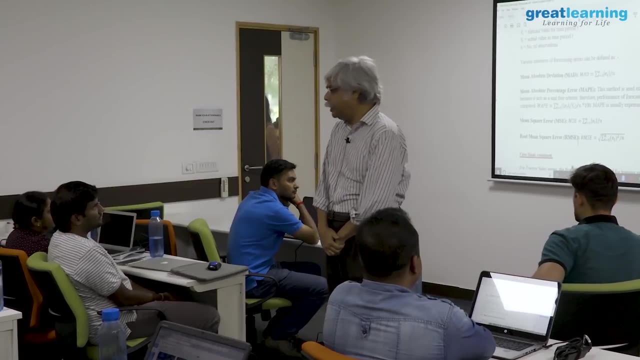 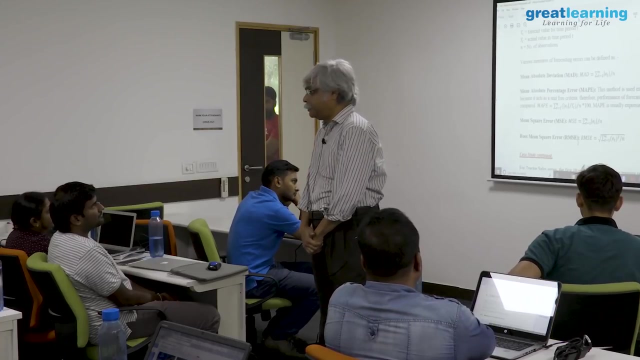 something vaguely like the following: I'm about 68% sure of being between 19 and 21, or not 19, 21, standard deviation of 2, so 18 and 22. I'm about 95 percent sure of being between 16 and 24. so the root mean square error often. 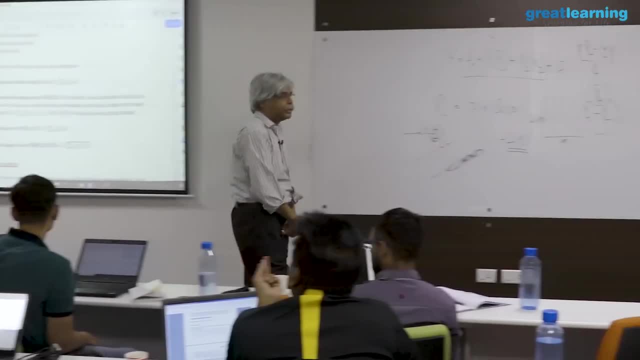 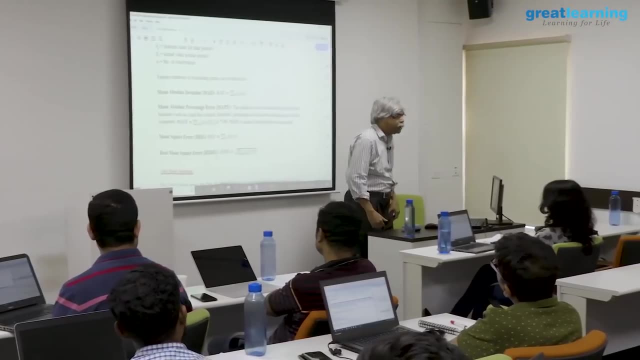 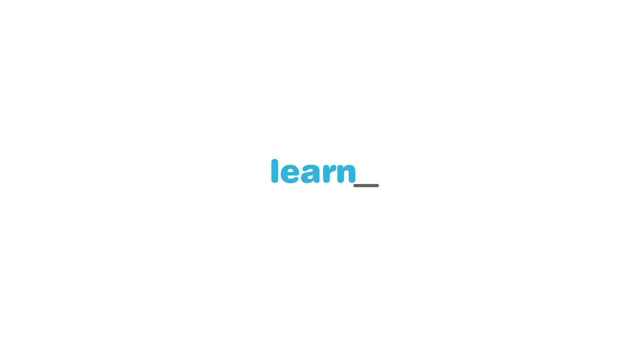 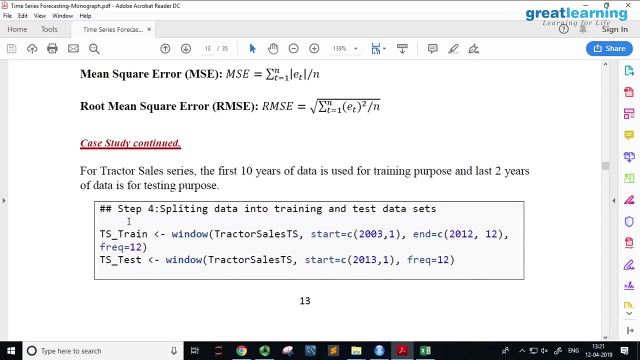 acts like a standard deviation around the forecast. so these are the numbers that we will tend to use in order to understand whether our forecasts are good, bad or ugly. you now to do that. you need to set this up, and here's an interesting way of setting. 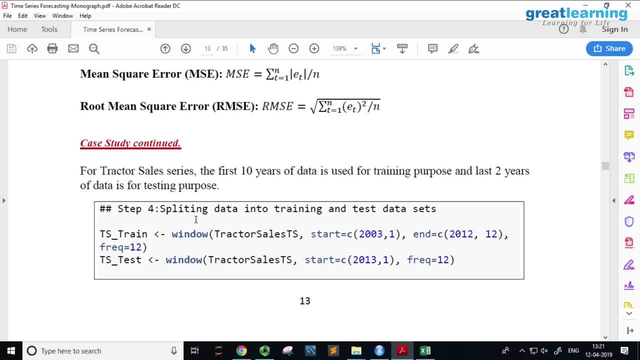 this up. so you're going to split the data into training and test sets. now how are we going to do that? this is a. this is the data set that now goes from 2003 to say 2014.. I want to divide this into two pieces. 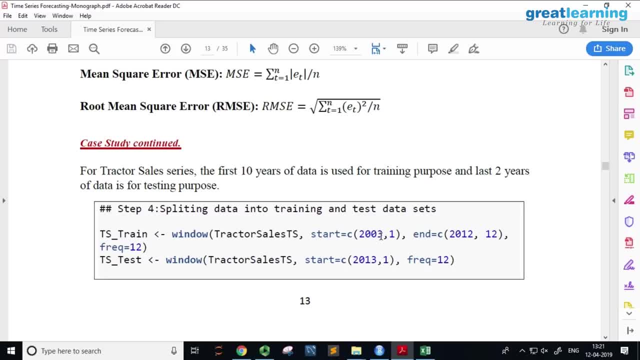 I want to divide this into two pieces: 2012 and then from 2012 onwards. now, this is a time series object. remember how I created this? how did I create it? I began with saying start equal to something. so we start has been identified with a certain label, which is 2003 to 1, which. 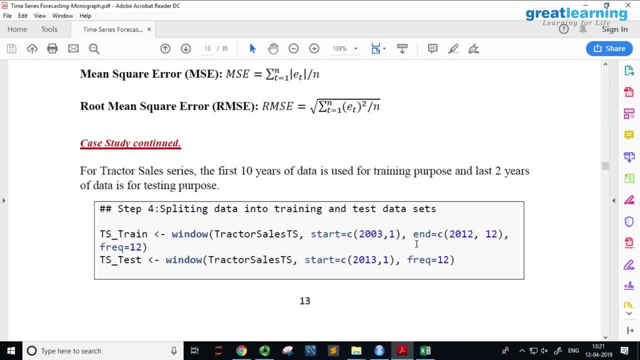 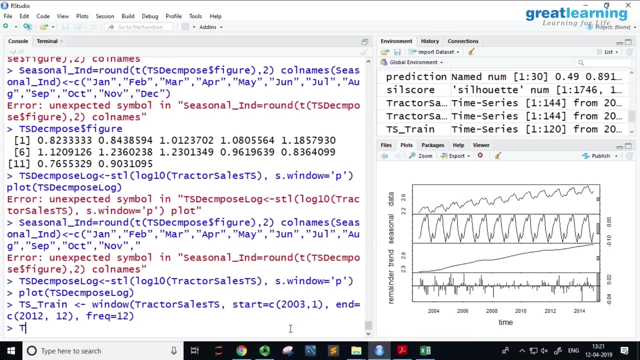 is how it was originally created, but now I am going to end it, and I'm going to end it at 2012, December frequency: again 12, because I'm going to create another time series object. so if I do this and then I see it, it looks exactly like my 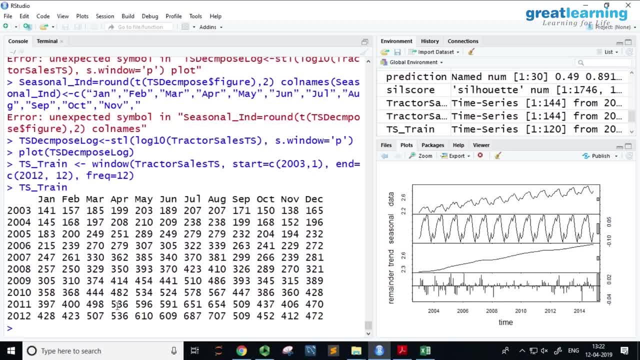 original object, except that it is now ending at 12. I could also actually done it manually. I could have gone from you, say 1, colon 120, and done that as well. that would have been my boring way of doing it, but this is not nicer. so what am I changing my problem into? I'm 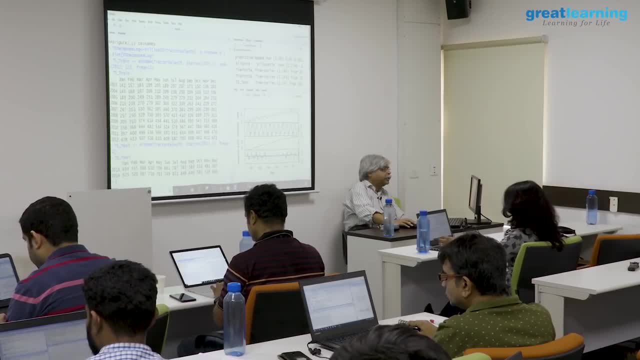 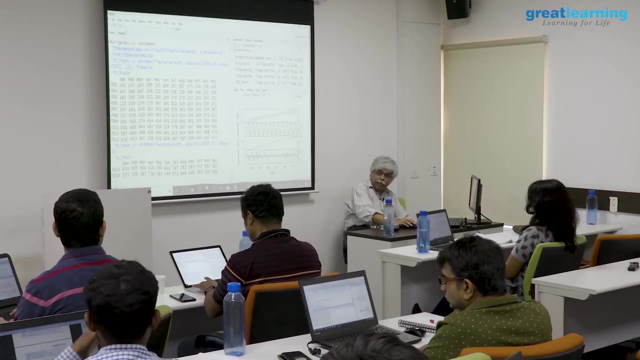 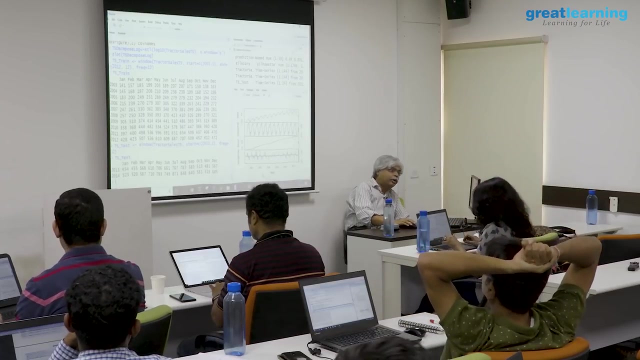 changing my problem into saying: do not work with tractor sales, TS, work with TS underscore train and then use that to forecast two years ahead. when you forecast two years ahead, compare your forecasts with these actual numbers and see how well you have done now. how do I compare the two numbers? by using either a mean absolute 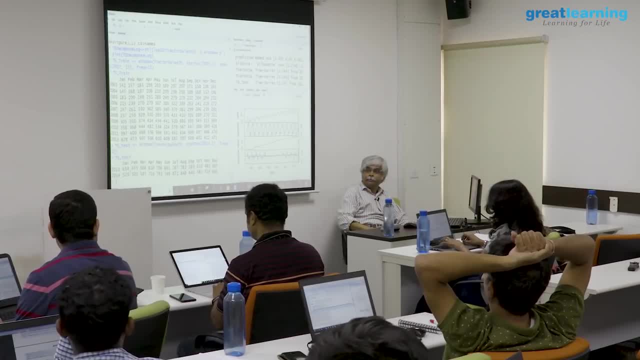 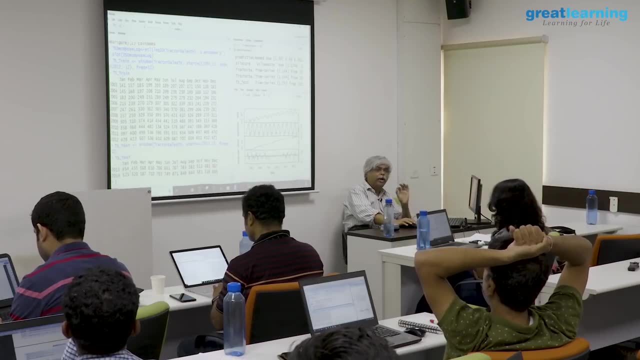 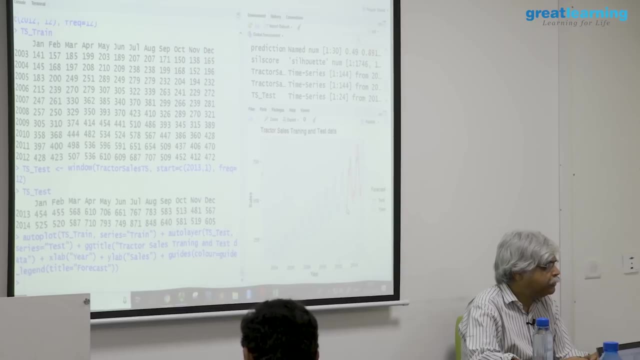 percentage error or a root mean square error, which will tell you how far off you are from your actual as a percentage or as a standard deviation. it's a visualization of it. there's a slight gap here, because the two data frames were different. there isn't a line that joins them out. but now the problem becomes. 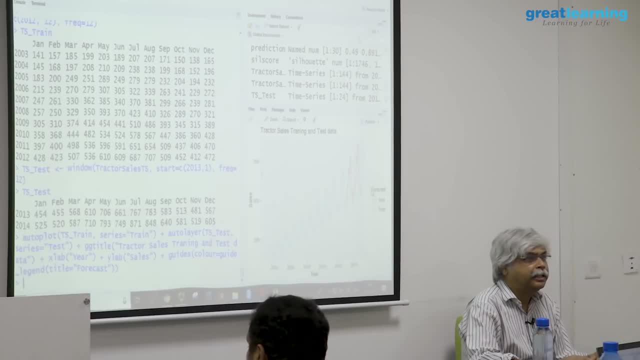 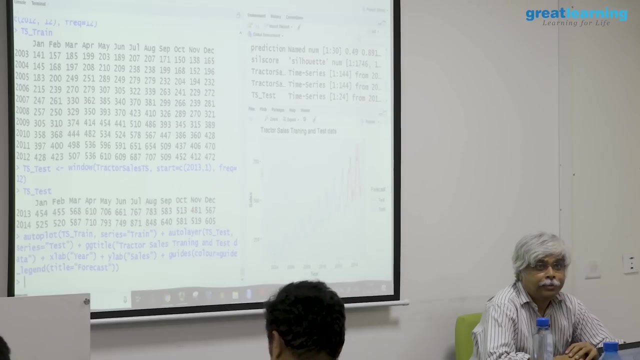 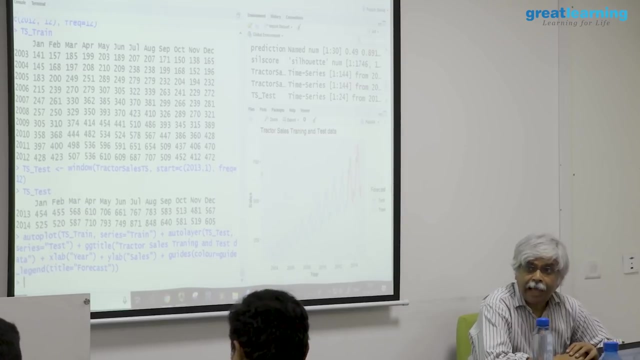 clear. can the green predict the red now? does the green or blue, whatever it does, it correspond to something that is constant? no, the business is changing. the business is growing, the business seasonal. there's a trend. this is. there is nothing in this that says that the past is like the future. I'm sorry, the 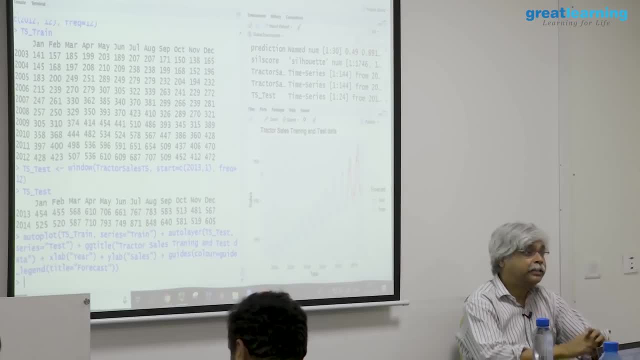 future is like the past. yes, certainly it. things are changing. certainly, it should not be the case, and what happened here is going to happen here. no, but you are saved by something. you are saved by the fact that what, if whatever, happened in these last two years is also different from what happened before. in other words, it 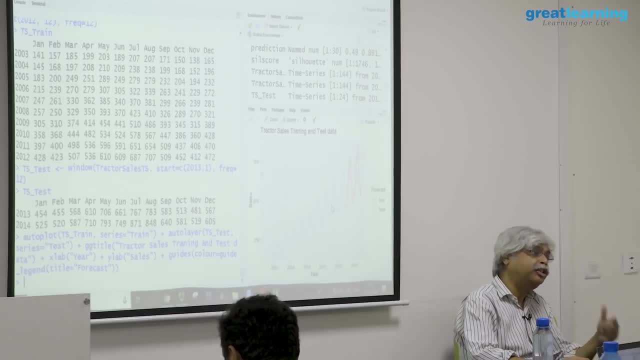 is changing, but it is changing in a way that it is changed before. it is not changing in a new way. if it is changing in a new way now, I'm in trouble. but if I'm allowed to assume that this September 2014 s adjustment is the same, 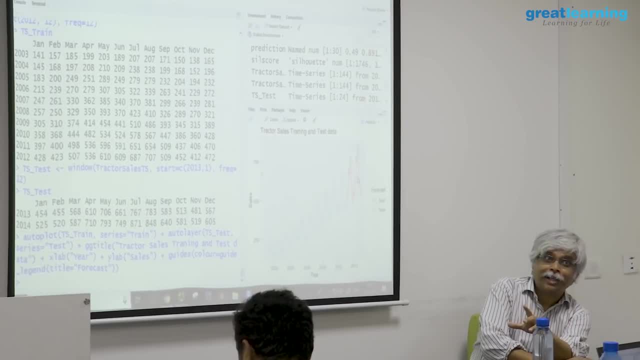 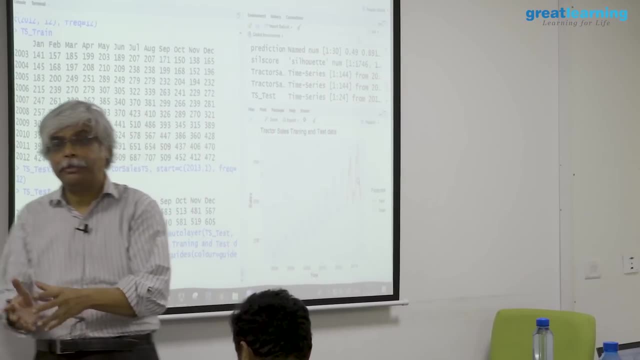 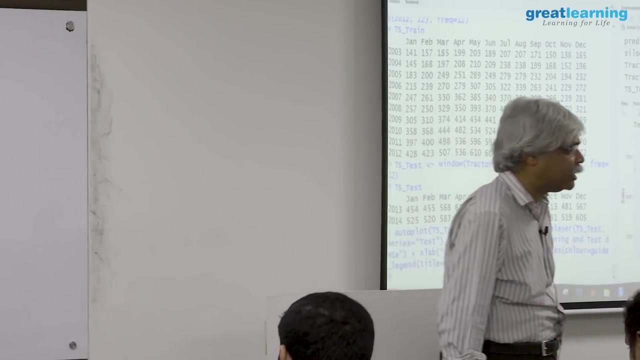 as previous September's, then I'm okay. I need to assume that there is an adjustment for September. September is not the same. but am I allowed to assume that this September is going to be like the previous September's in terms of raw sales? no, this September I will sell more than I sold last September. that's not. 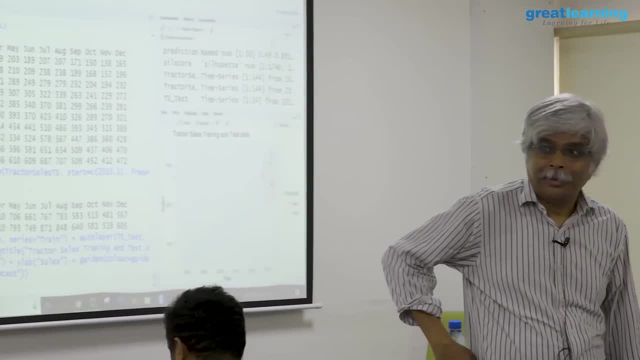 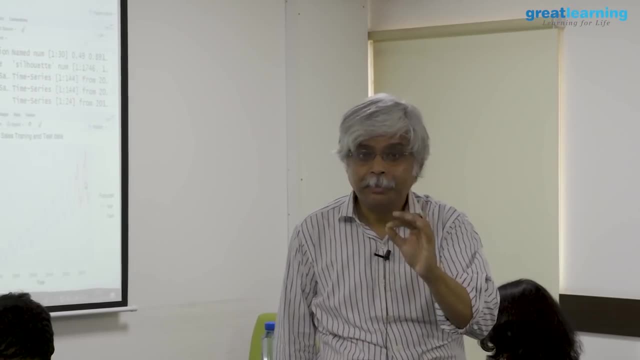 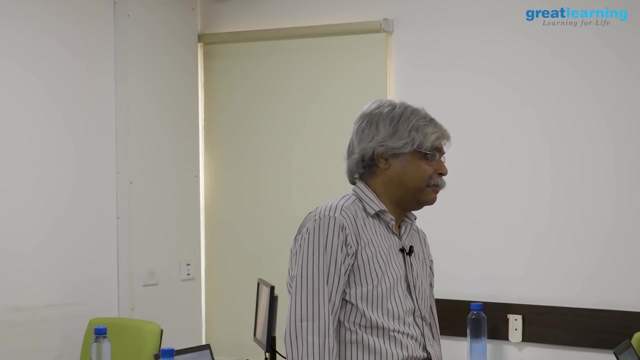 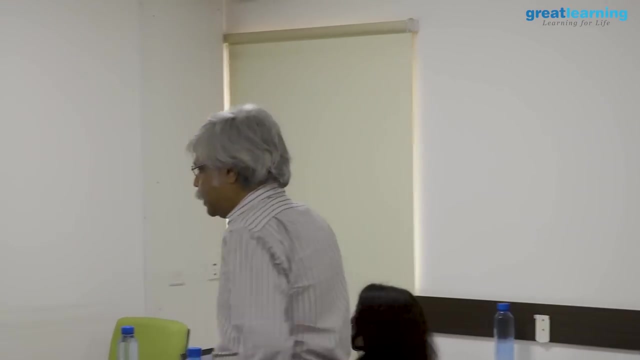 going to be the same, but what is going to be the same? something will be the same, and I'm assuming that the thing that will be the same is that the percentage lift that September will see over the same year's trend will be the same, and that's a complicated assumption to make, but that's the assumption that's. 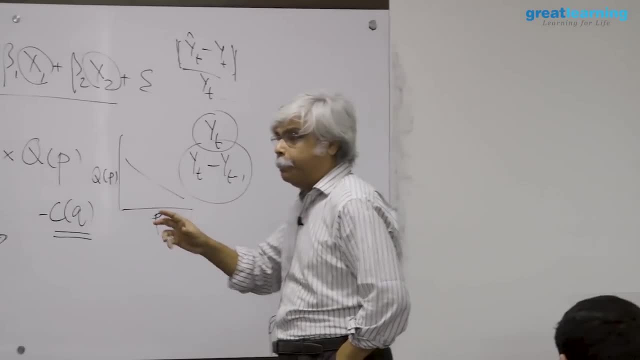 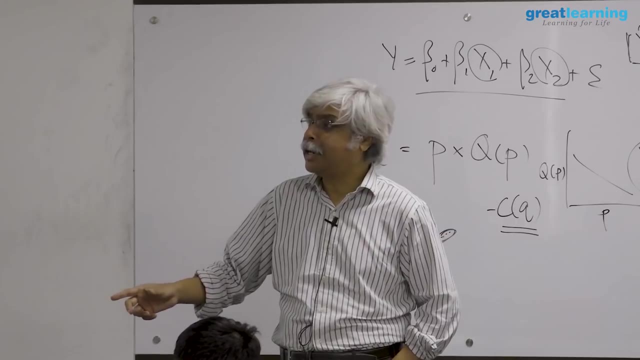 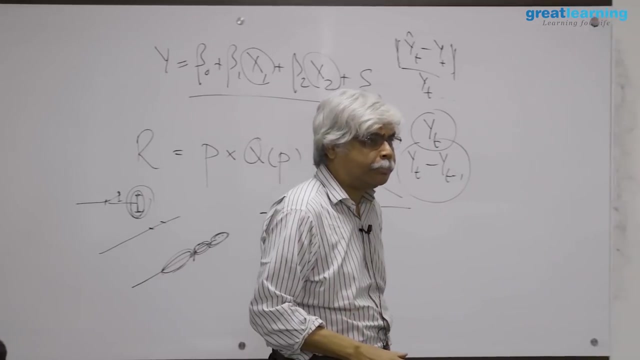 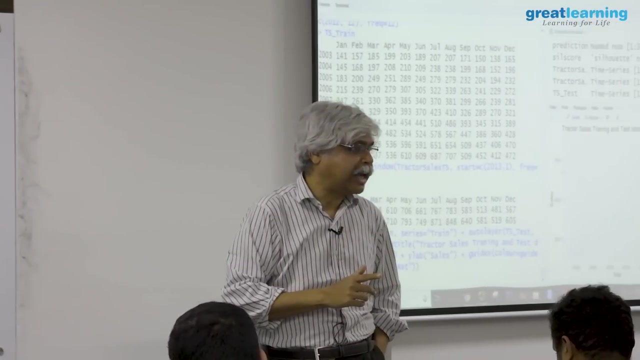 made this assumption. looks peculiar in time series, but you are making this assumption continuously. you made assumptions like this throughout the course. hypothesis testing is that assumption. as I said, with populations and the mu, that holds across everything in regression. you did this assumption. that line holds for a new data point, but will the new forecast be exactly that? 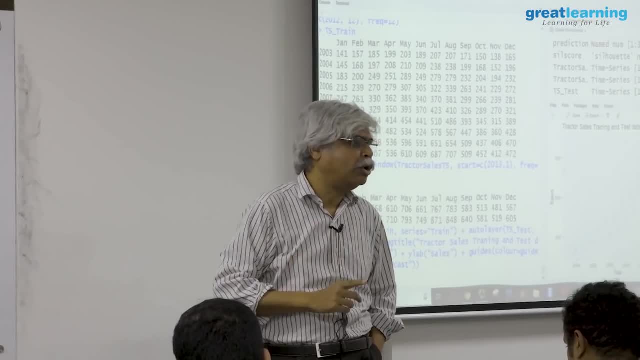 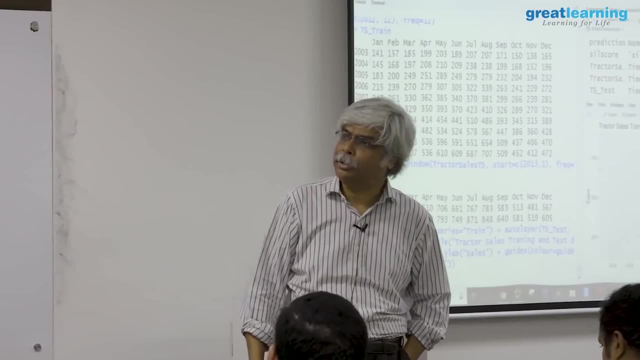 on that line? no, I'm sorry. will the new value be exactly be on that line? no, in fact, you know that it won't be. none of your points are on the line. if none of your points are on the line, how dare you assume that your future points will be? 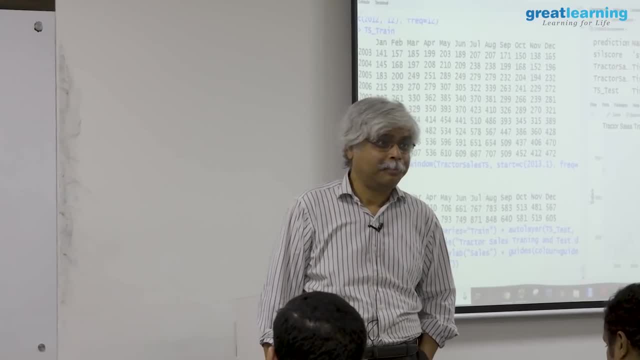 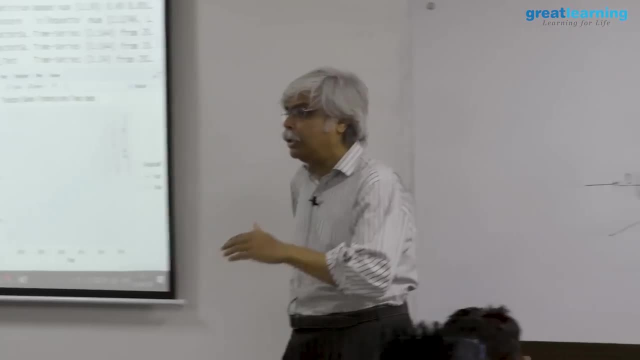 on the line. but the point is: no, you're not assuming that at all. you know that there is going to be an error, but in spite of that error, what about? it remains the same? and you say that straight line remains the same here. what about? it remains the. 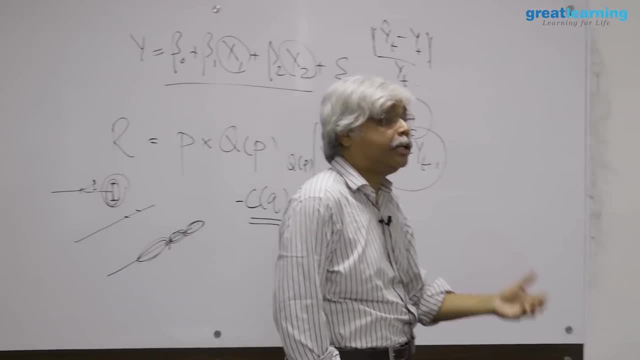 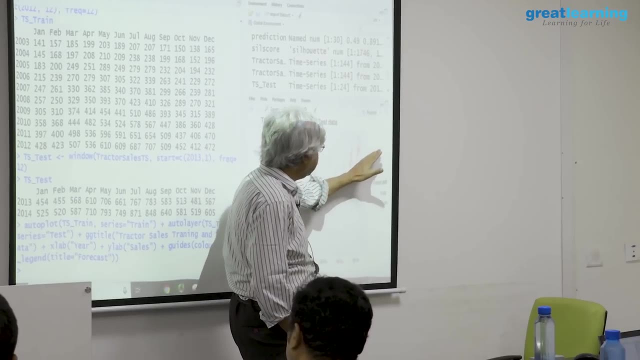 same and we're going to make assumptions. the trend remains the same, the seasonal corrections remain the same and if the trend remains the same, in other words, I'm going to, I'm now going to assume that it is going to increase, but how is it going to increase? the same way that it is increased before and as you will see, 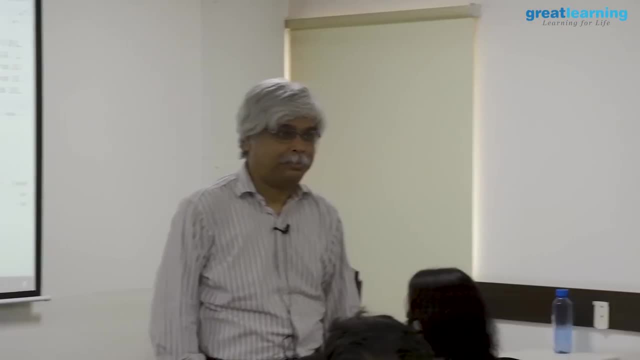 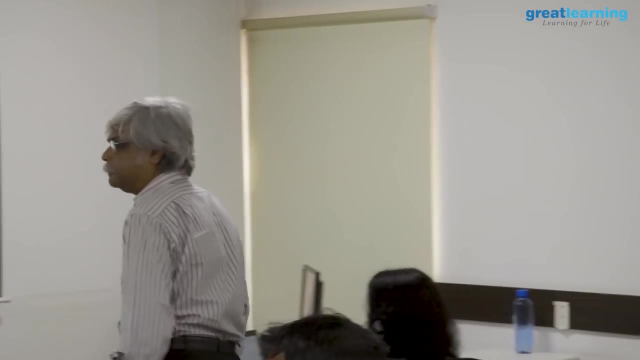 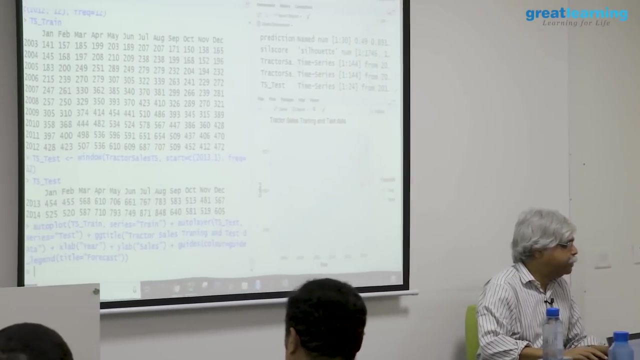 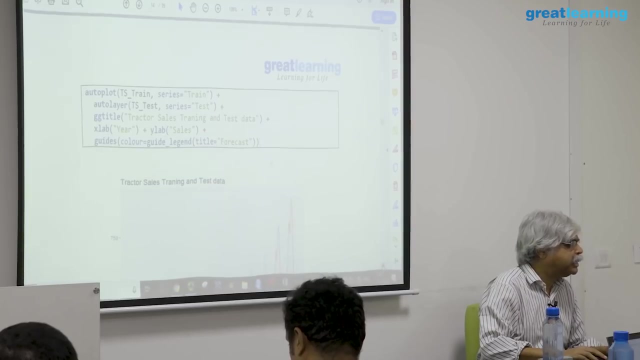 that assumption will be almost correct. it will not be fully correct, it will be almost correct. so that is clear. so that's going. that is our task, to say: build a model in which I can predict something like this: this: the ability to do this gives people a little more faith, otherwise you get. 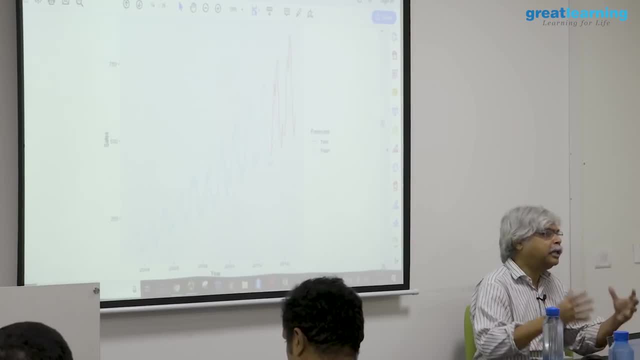 stuck in this time series question of saying: but you know the things are going to change and so there is no hope for the future. yes, yes, yes, I know things are not going to change, but that doesn't mean there's no hope for the future. let's figure out. what about any possibleugs? it's possible, nothing, right. now. this is very difficult and I hope that you'll try and look at this. kids also get right now common here, so this is very difficult, okay, so on listing the like you'll see at the Your Y of the Select, here is something like this: much into the: 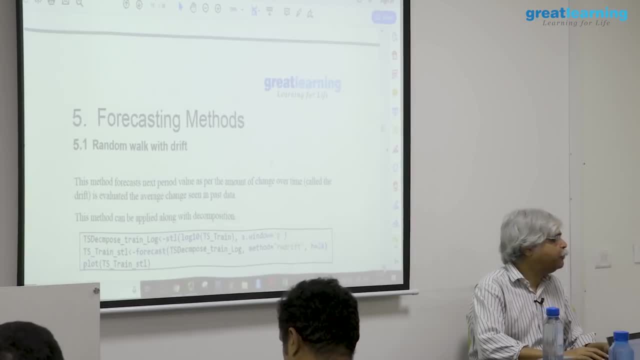 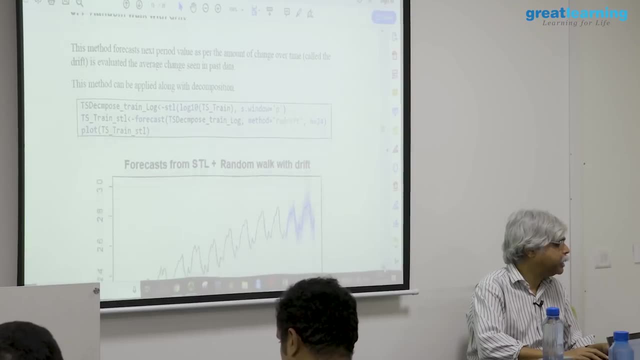 question, especially lately, which is not a solution. this is sort of thinking you did things right about this is going to. let me show you one forecasting method. so that is you do you have forecast a little bit and see what happened. so this is. this is an odd. 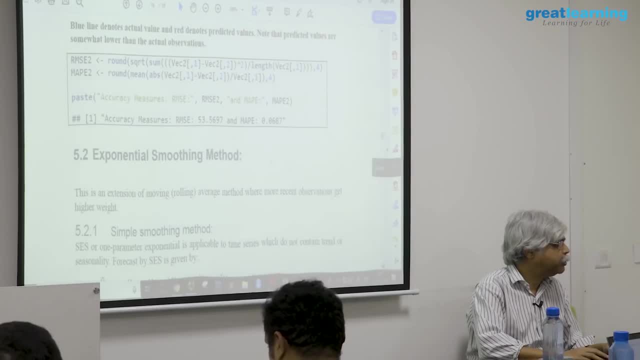 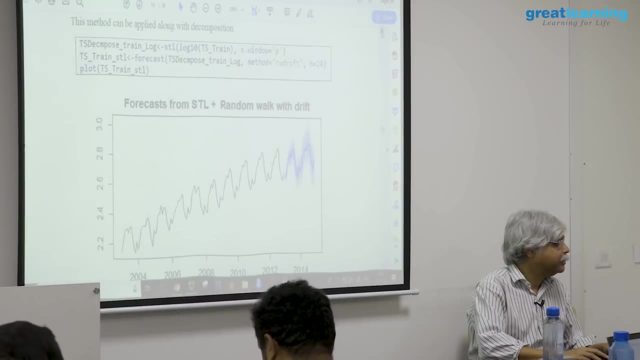 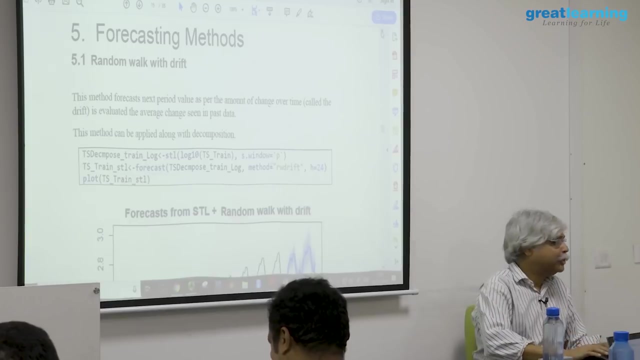 it's a strange forecasting method, but at least I want to show it. and then what we'll do is we'll begin again tomorrow. at this point I don't want to leave you without doing any forecasting whatsoever. the topic is time series forecasting- huh, not just fancy. so what we'll do is we'll do a forecast now. the forecast is: 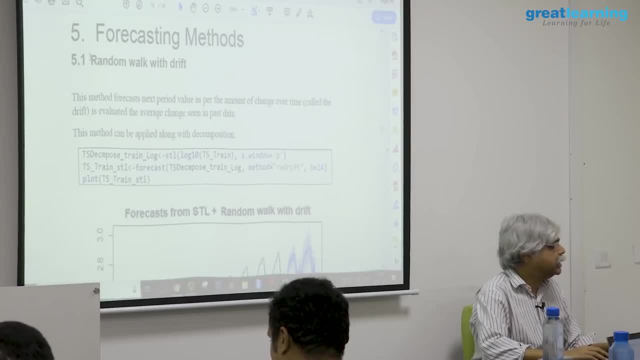 not an- not an easy forecast. we'll see easier forecast later. this is a forecast called random walk with drift. ignore the name. random walk means something is moving randomly. drift means inside that random drift there is the ability to pick up seasonality and trend, so there is a drift allowed within a random walk. 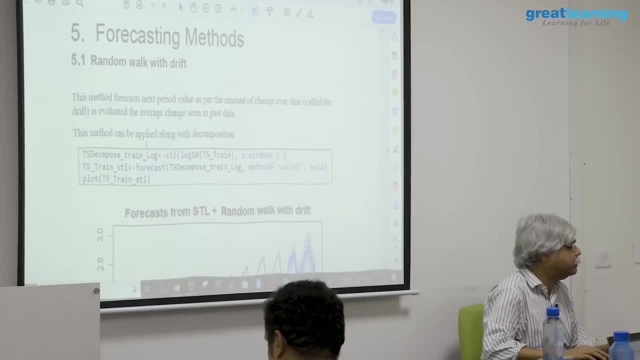 now to do that, as I said you will need, you'll need to use this STL function, which allows this. now to do the STL function. to run the STL function, remember that you have to run it within the log scale. so what we are going to do is we're going to predict, not sales, but we're going to 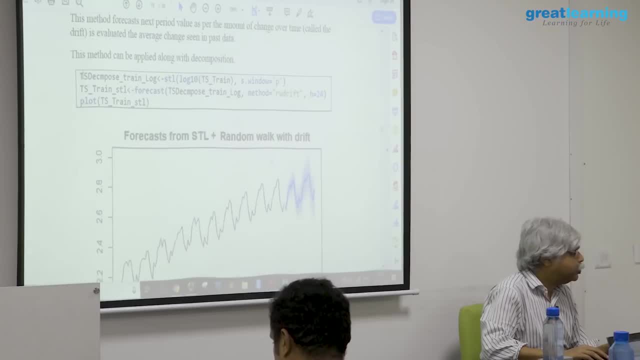 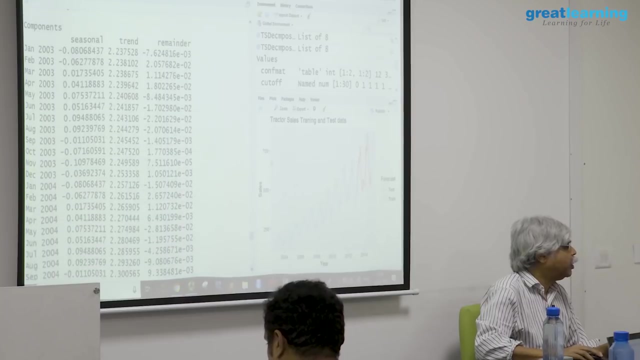 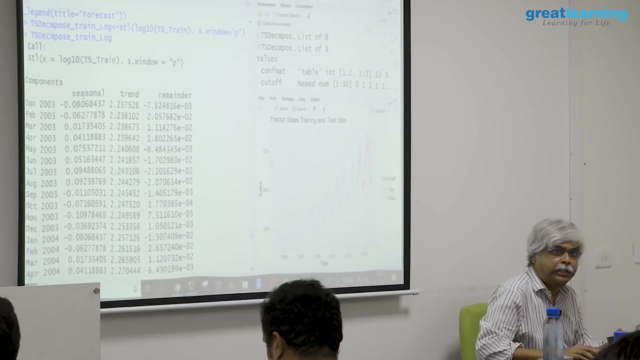 predict log sales. so first, is we're going to do the prediction, so to speak, or we're going to generate the time series object? generate the time series object through. let's say this: this is not forecasting, this is generating the time series here, components. what has it done on the log side? it has created a seasonal component. 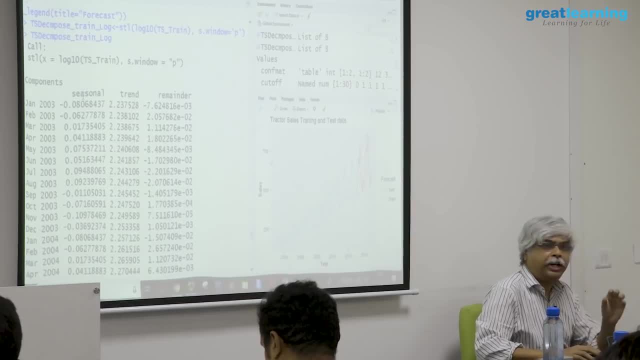 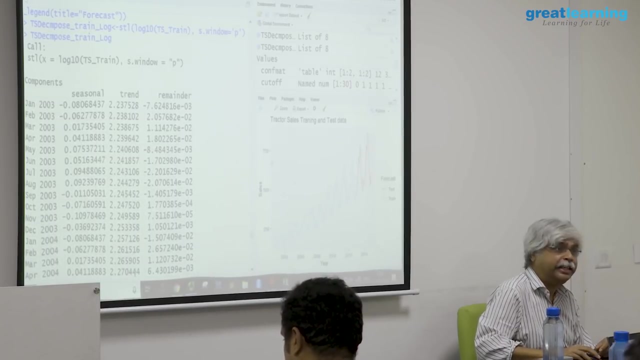 it has created a trend component and it has created a remainder. look at the seasonal component: minus 0.08, let's go to the next January. minus 0.086 is the same thing. the seasonal components are exactly the same. the trend, however, is increasing and the remainder remains unpredictable. we 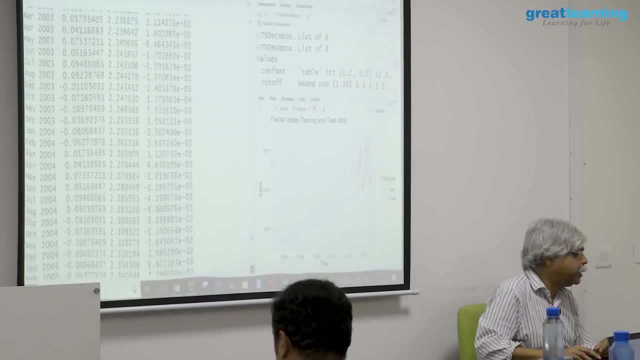 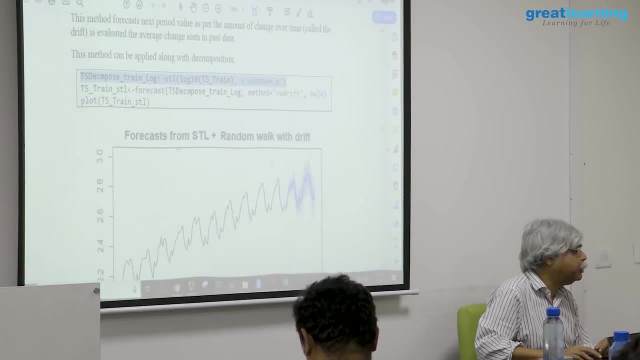 saw this plot before. this is simply is a simple year output of that of the same plot that we had seen before. this is a description of the time series. now, what we need to do is we need to check, you need to convert this into a forecast. now, when we forecast this, the function that we use is the function forecast. 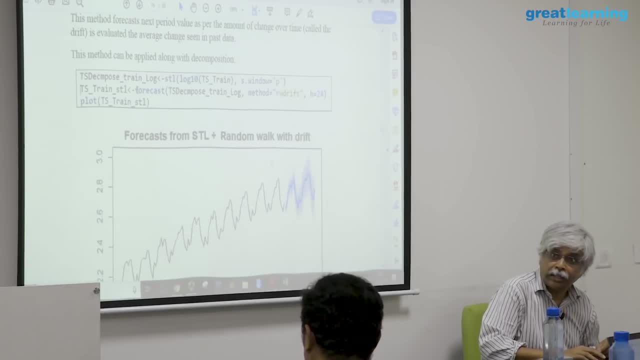 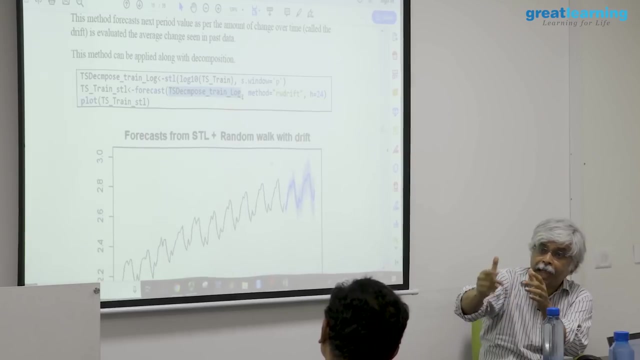 this comes prepackaged. there's a library forecast that does this. when it does a this, it takes this object, which is the decomposition. this is not a time series forecast, as a function in R doesn't act on the time series. it sorry, it doesn't act on the time series. it acts on the decomposition, so it needs to know what. 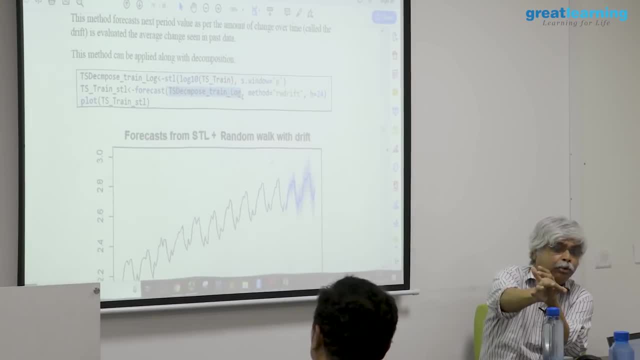 is the trend, what is the seasonality and what is the error, so that it knows what to ignore, because it will ignore the remainder part. so it needs to know what the remainder part is. so it needs that decomposition. so we'll get that recommendation. you need to know a method. in this particular case, the method is: 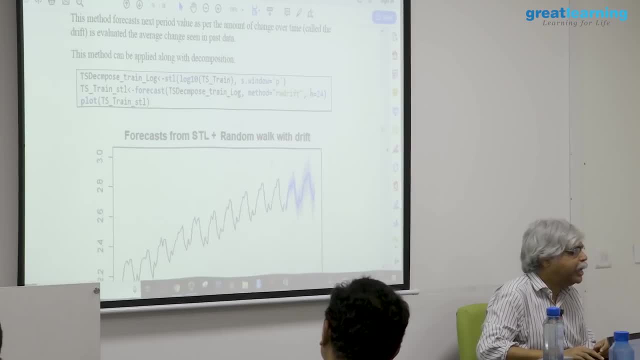 random work with drift. don't bother too much about the method. we can change it. H equal to 24 means: for how long do you want to forecast this for now? how long do I want to forecast this? for two years, which means 24 time units in this. 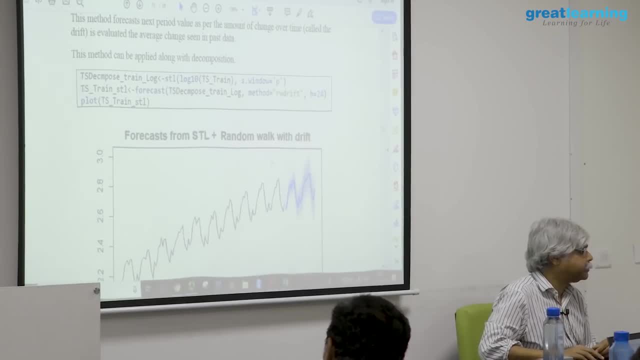 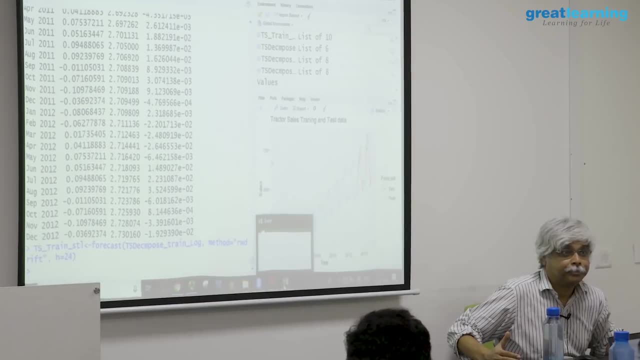 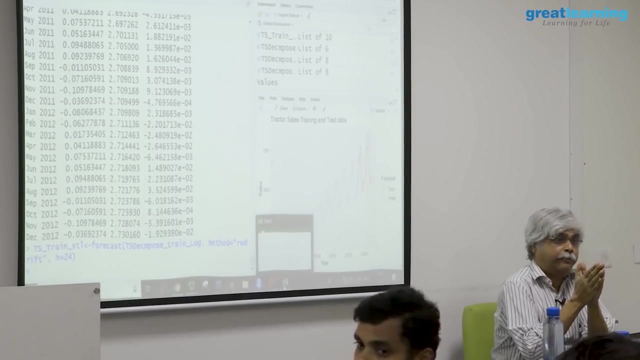 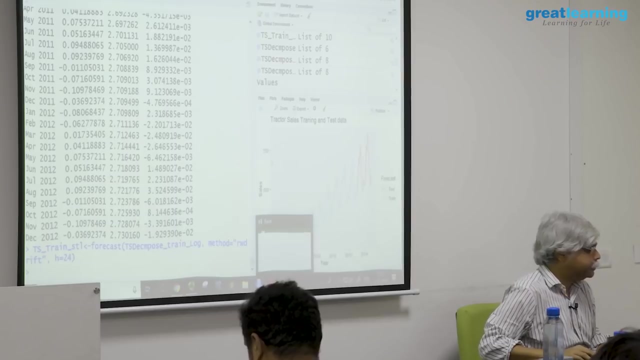 particular case. remember, this is being done on train because, using it, I want to forecast for two years. this is train, so train ends at 2012 and I'm going to forecast up to 2014 and then I'm going to compare, then I'm going to compare and now what I can do is: I can. 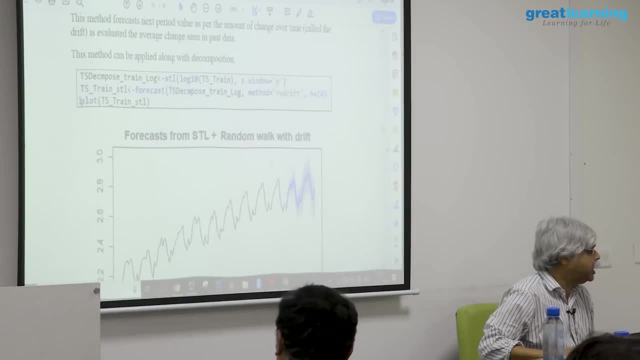 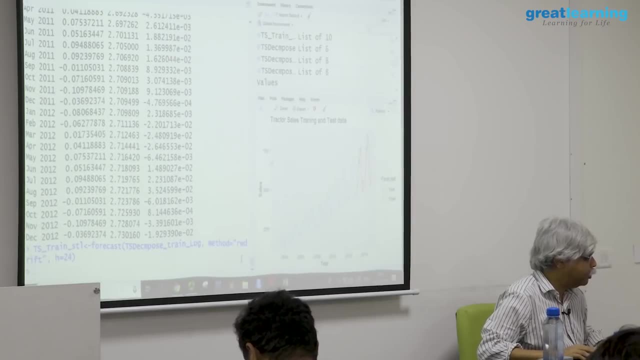 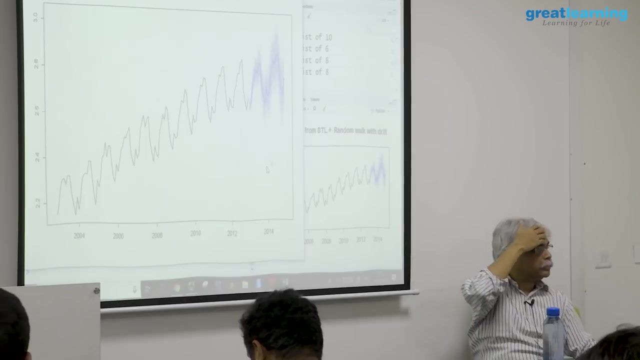 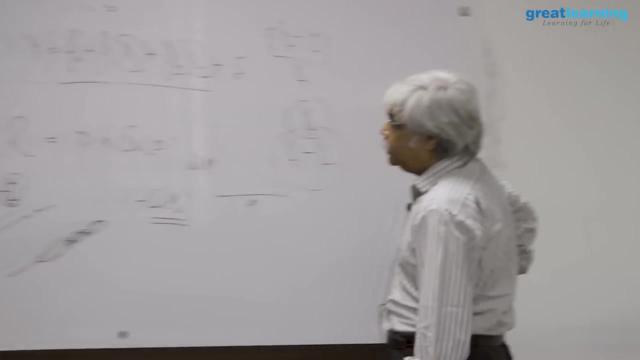 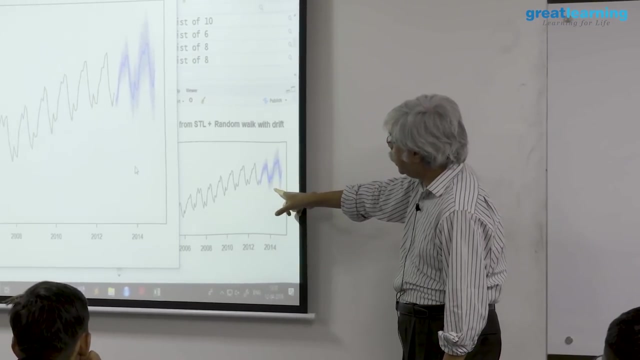 simply plot these. I can plot this. I can plot the forecast. when I plot the forecast, we'll see many more forecasts tomorrow. so when I plot the forecast, the forecast looks like this: this is my forecast on the log scale. this is how I forecast now. when I forecast this, I see certain things. number one: you can see. 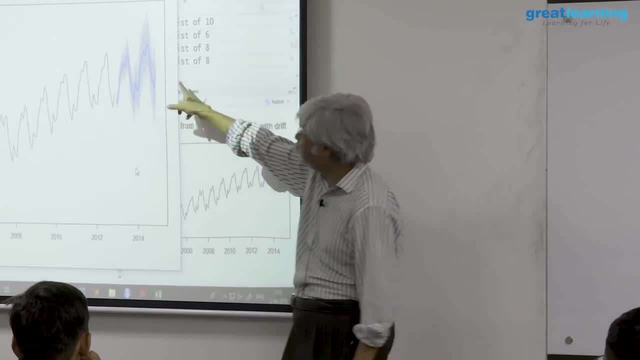 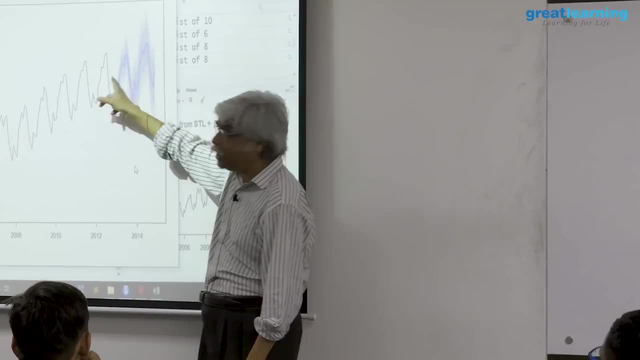 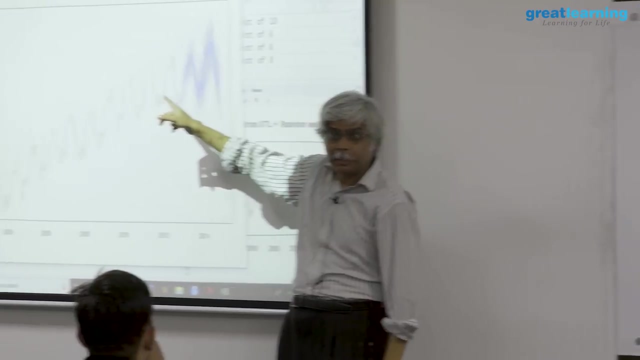 the forecast, and the forecast is not constant. the forecast has picked up the trend and has picked up the seasonality. in fact, how has it forecast? All it has done is it has extrapolated the trend and then multiplied back by the seasonality numbers, which you already saw in the output, and ignored the random part. and it has done. 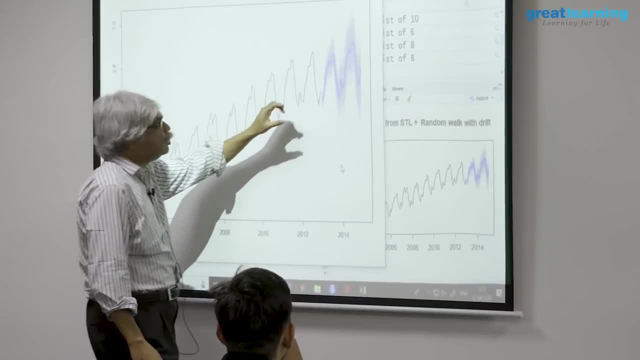 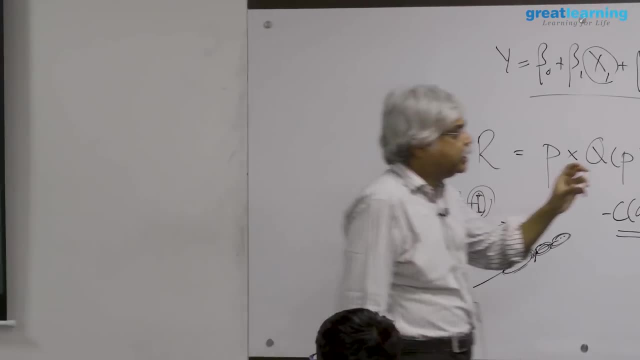 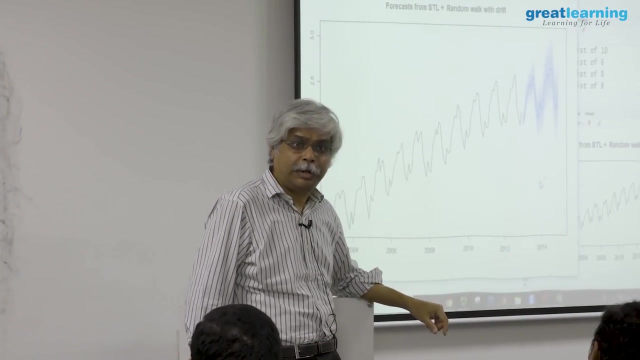 something a little more, in that what forecast has done is it has also calculated a standard error like thing, which is these grey parts, Very roughly speaking, that the dark grey is like a 95 percent and the light grey is like a 99 percent. but for now you do not need to ignore that. these are the error bars associated. 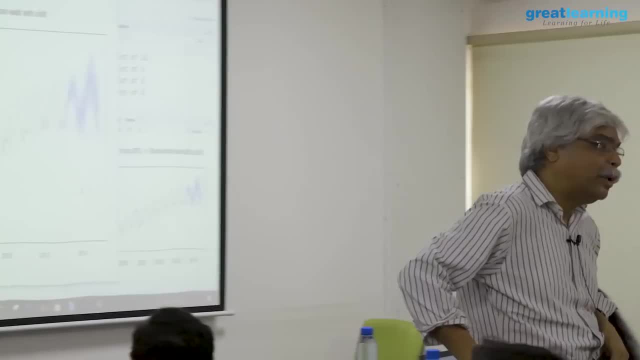 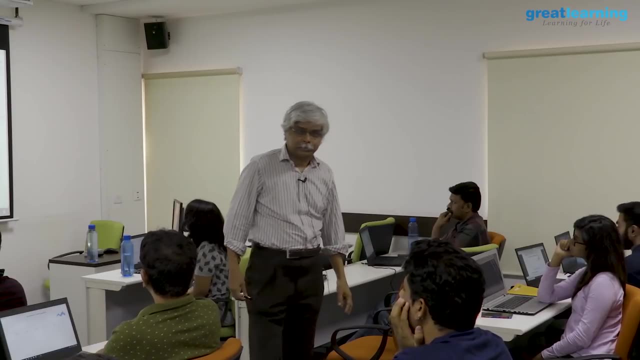 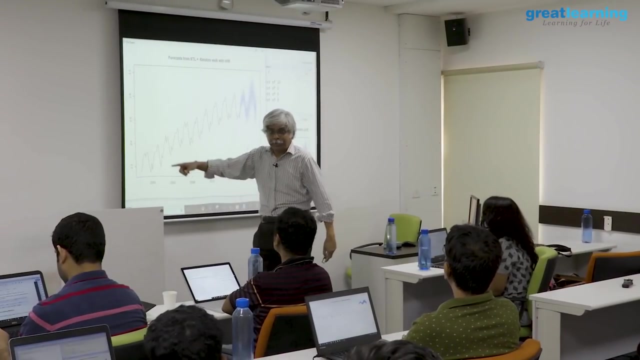 with my forecast, Which means I do not know where the forecast will be, but I am saying 95 percent confident that it is in that grey zone. So the actual line I do not know. I will see, I will calculate soon, but this is my forecast. 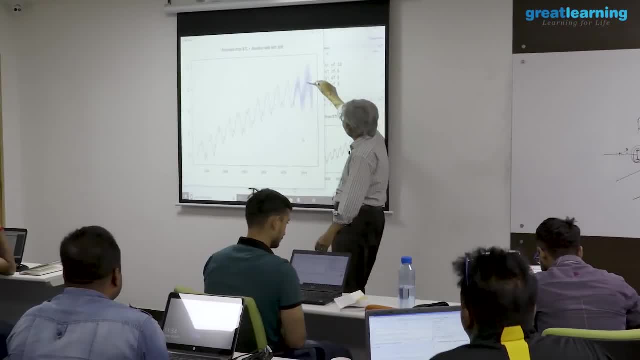 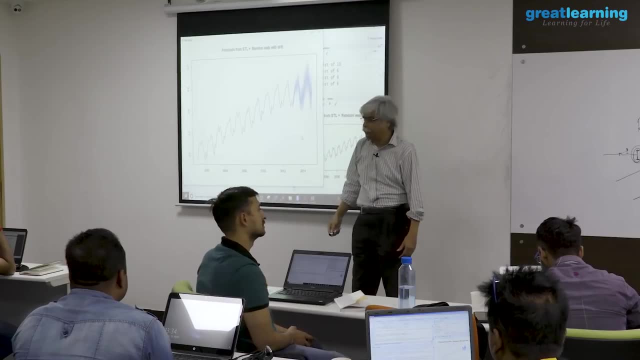 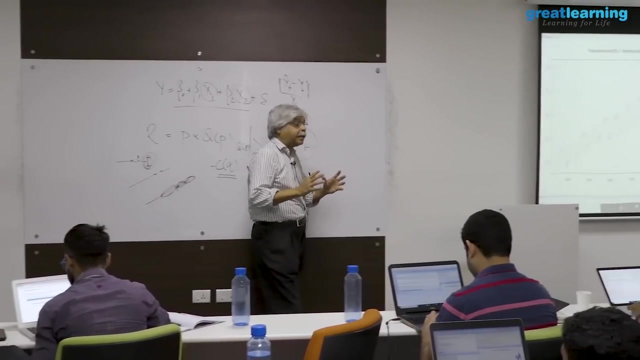 So it is saying that I do not know where the future will be, but the future will be somewhere in this grey zone. If you want a point, the point is here, but otherwise it is here that the general idea for confidence interval- I mean a confidence interval- is. you know, it is a, it is a technically, there is an acronym. 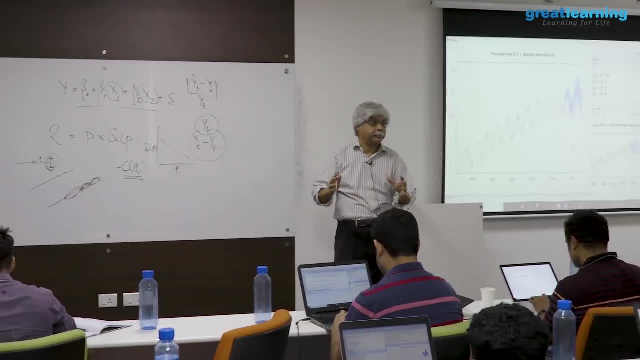 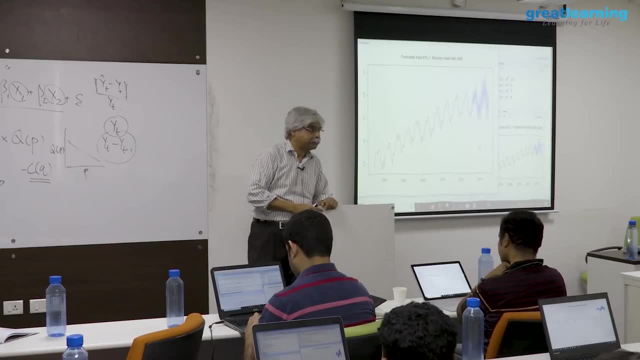 that is often used for it called CYA, which stands for cover your ass, which means I have no idea what the truth is going to be, but it is going to be somewhere here. So I do not know the exact number, but I am giving you error bars around that. 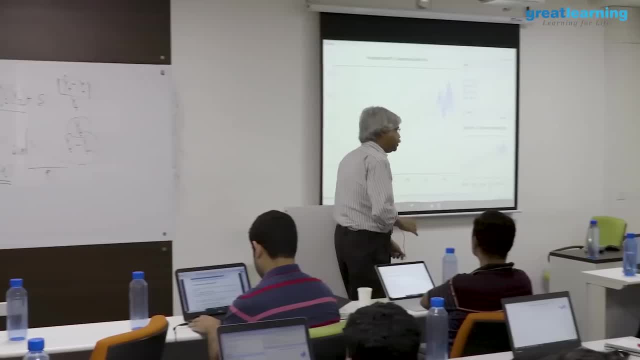 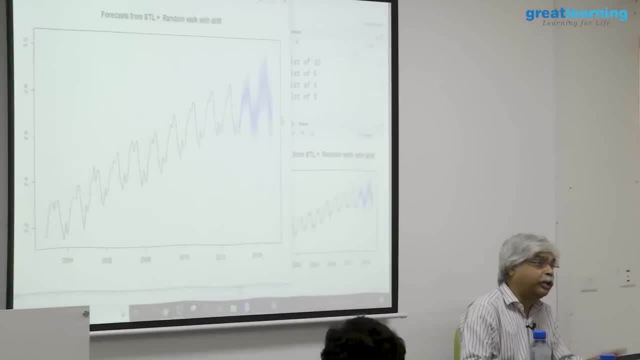 Now to calculate how much there is actually, which is the question that you are asking, I need to now do a little bit of fiddling around. Why? Because remember that this is a forecast of the logarithm. So to get to this, I need to go 10 to the power, this or something of that sort. 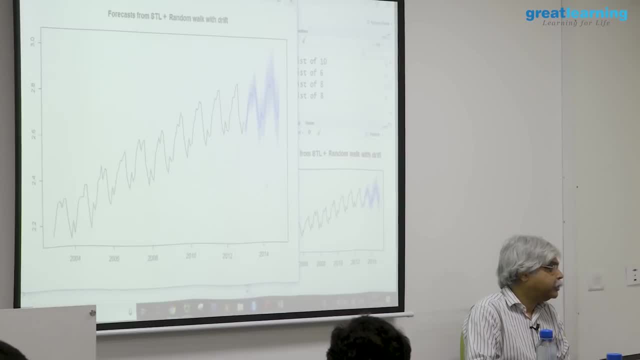 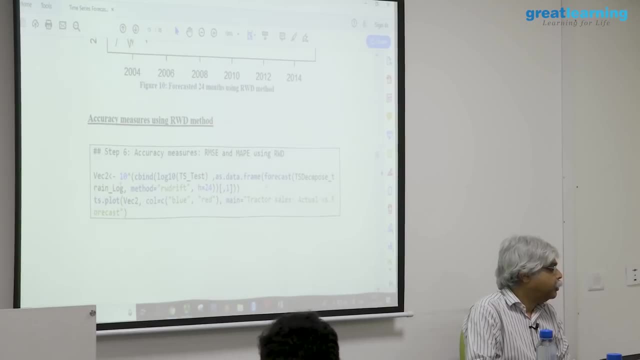 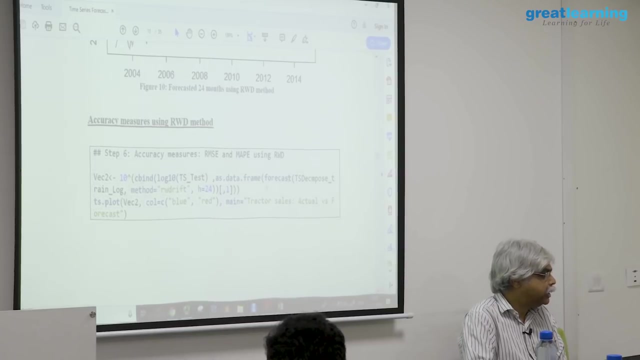 So I need to do a little bit of jugglery on that. So to do that, here is what I do Now. look at the next, look at the next piece of code here. What am I doing here? What is my forecast here? my, this is the forecast. decompose T and C bind and this is going to 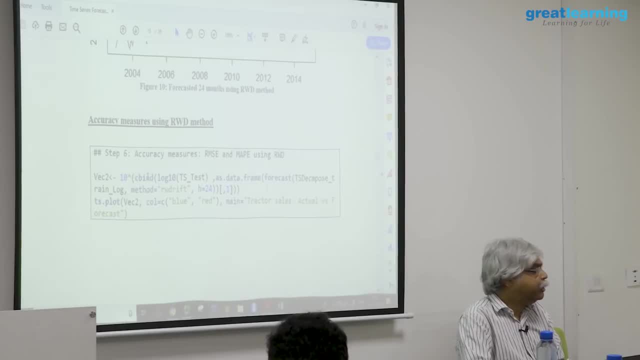 be 10 to the power. this, If you take 10 to the power, something, 10 to the power, what? 10 to the power of the logarithm? this is what this is, test compared with my forecast. So I am going to compare my forecast and compare my actual, but I am going to do it after taking 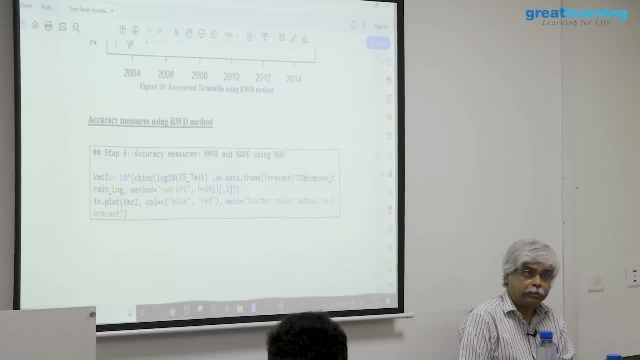 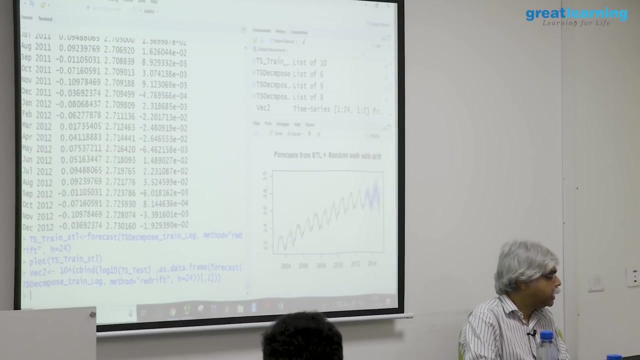 it 10 to the power. So you look at this code at your leisure, but what I have done is I am creating a vector in which I have got actuals and forecasts, But the scale of the actual sales, and now I want to plot it and see it, which is: 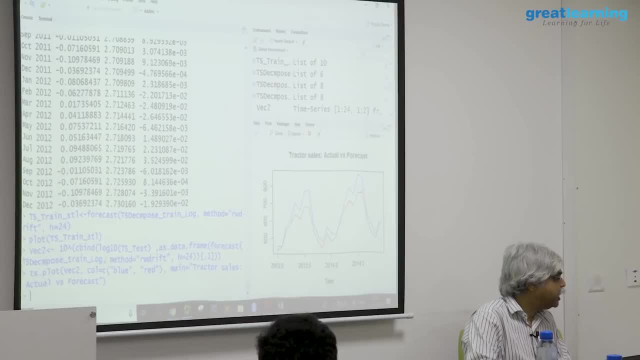 which back to what came in first. what came in first was my test, which is a blue, and my forecast is then my red. so my actuals is blue and my forecast is red and, as you can see, I've picked up the pattern, I've picked up the trend. 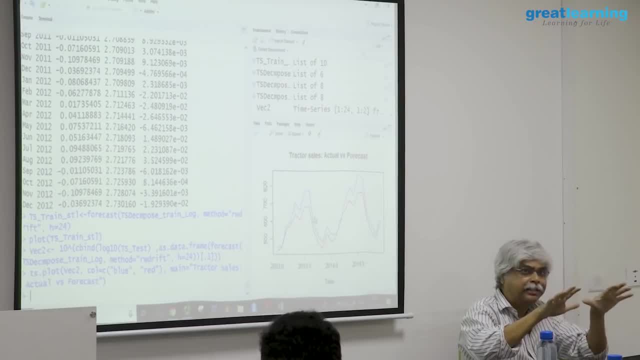 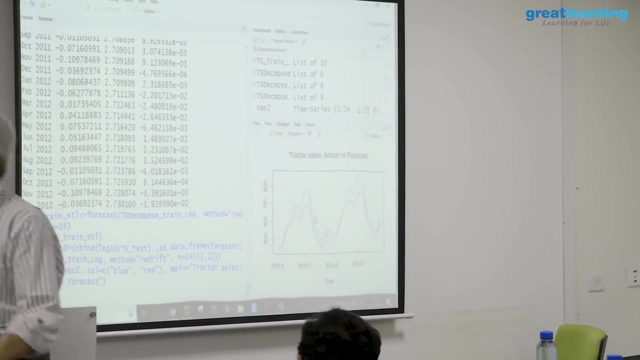 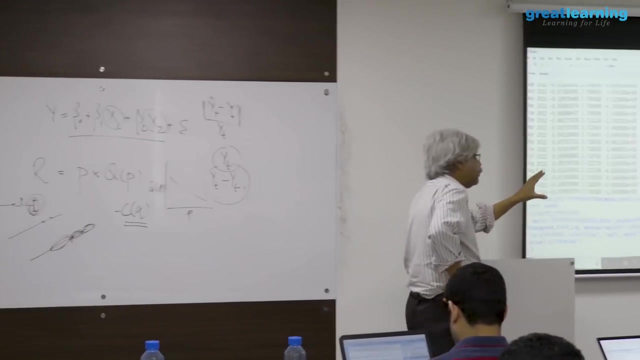 I've got a reasonable job, except that I have a slight under prediction, a systematic under prediction, which means that, in actuality, there was something that lifted my sales a little bit above the historical trend, something that is not explained by the trend of the past, but I'm not that far off. I'm not that far off, you know, if it's something. so 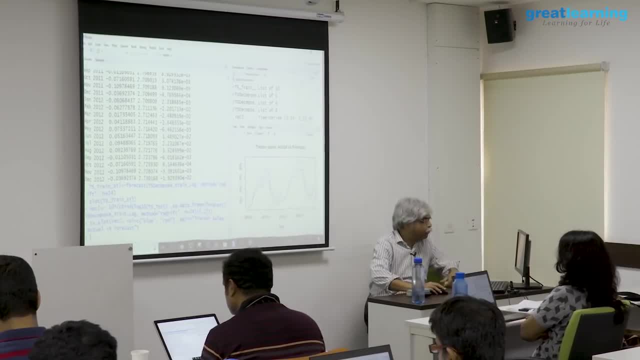 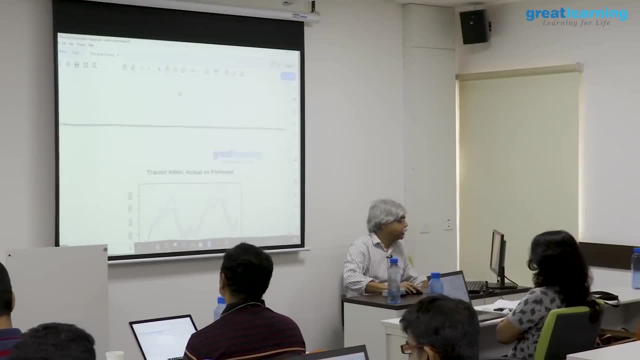 what percentage off am i? how do I calculate? how far off am I? well, to do that, I need to. I need to apply my MAPE and my RMSE formulas now. to apply my MAPE and RMSE formulas, I need to create formulas that do that. so this is. 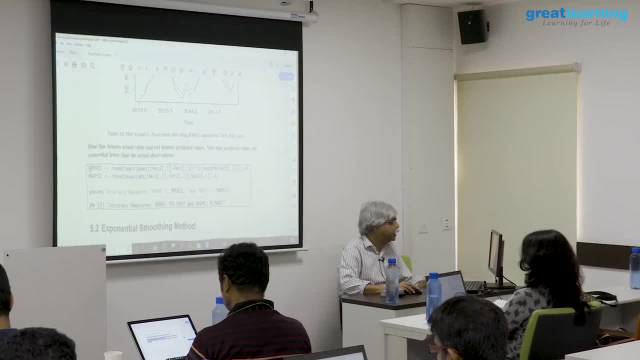 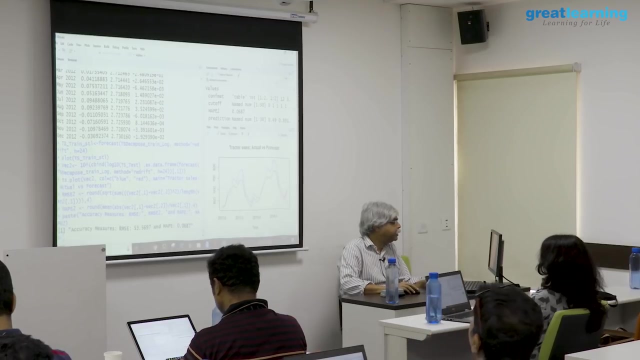 the RMSE formula implemented as a formula, and this is the mean absolute percentage error implemented as a formula. I know this is going quickly, we will repeat a lot of this também, pero vamos plantar para implementar essa formula e tomorrow RMSE is 53.56 and MAPE is 0.0687. as a percentage conclusion, I am 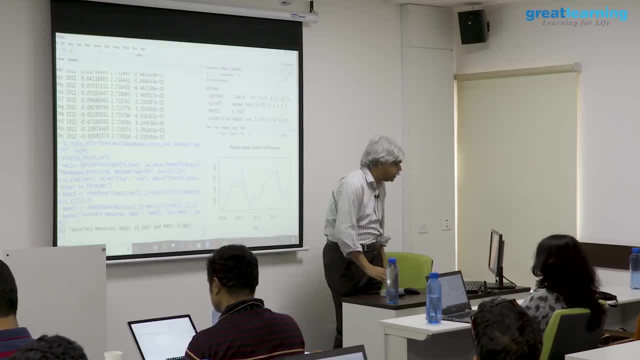 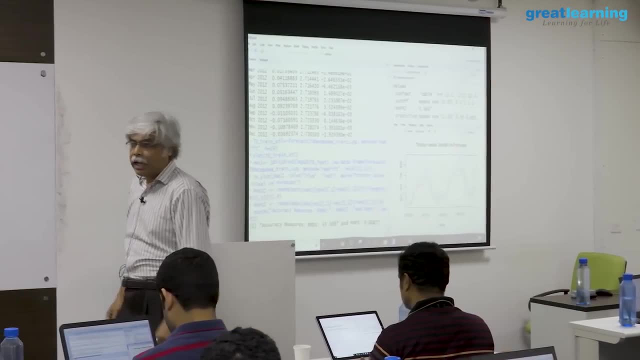 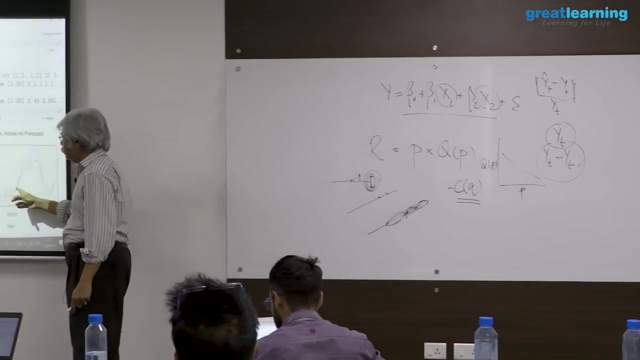 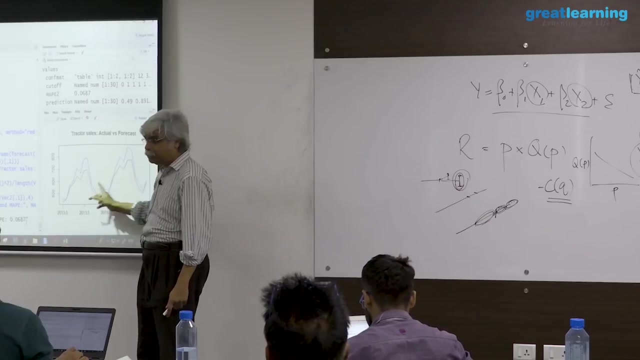 about six point on an average, I am about six point nine percent away from the truth. on an average, I'm about six point nine percent away from the truth. the actuality, because of this plot, most of this is coming from an under prediction. so about, say, six percent or six point eight percent under predicting in this? 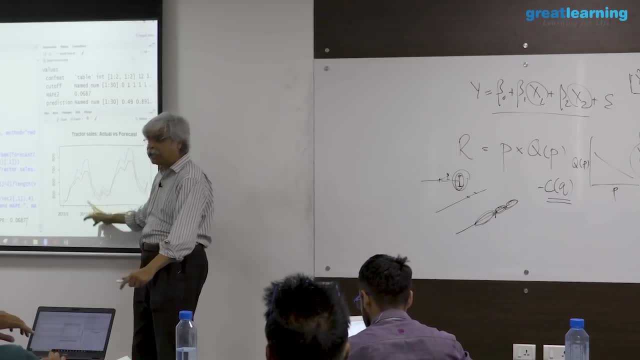 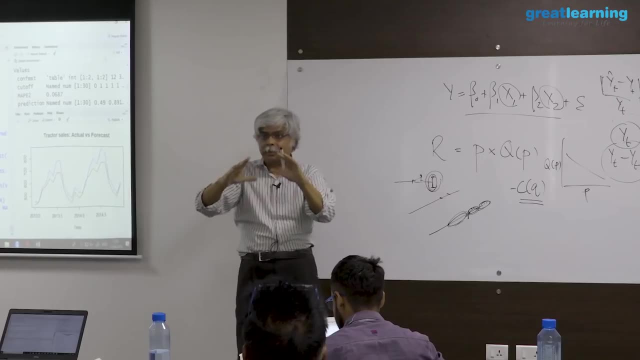 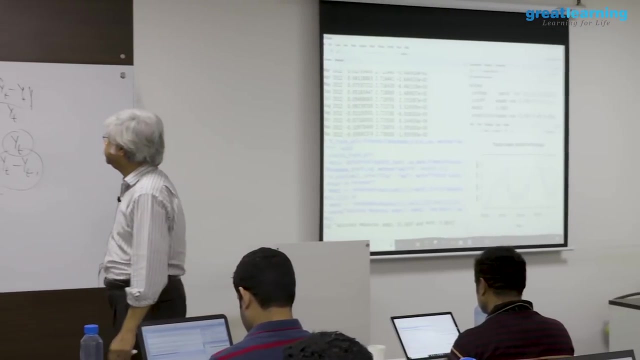 particular case I can say I'm under predicting because most of the time it is negative. in other words, that absolute value has the same sign for all of them. but in general this is sometimes we over, sometimes we under, but on the average I'm about six percent off. their term: is there the error term? the error term, is there this? 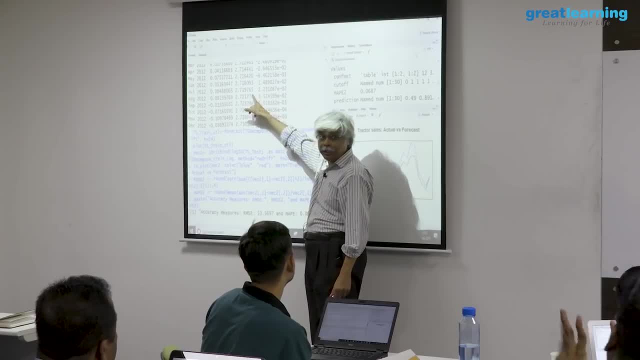 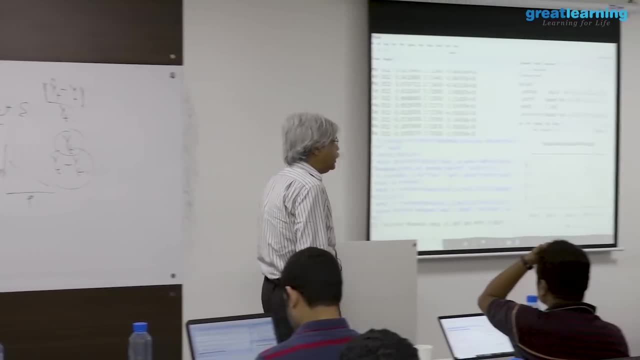 error term, but this error term was sometimes positive, sometimes negative, historically. historically it should have disappeared. so there's something else that is happening, something that is not in the historical data. RMSE is 53. RMSE 53 means something like roughly like the following: that whatever I 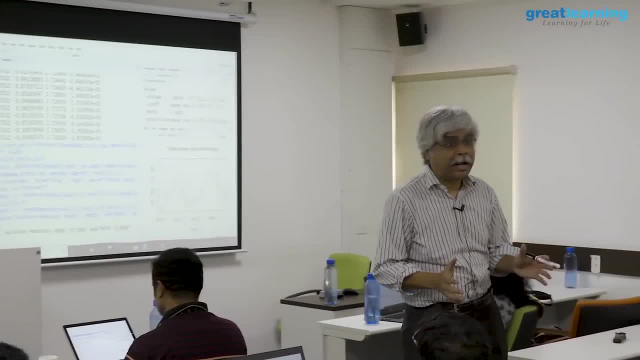 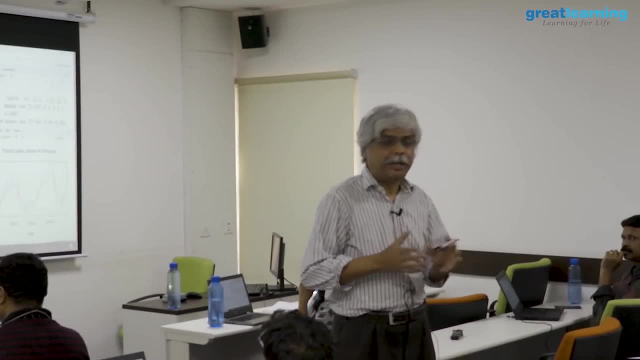 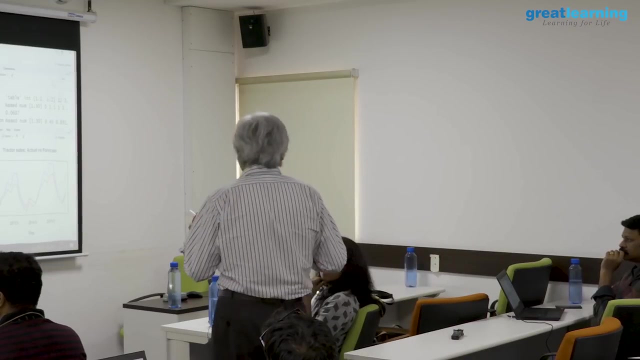 forecast. 53 of that is going to I'm about 68 percent sure of covering. if I want to be about 95 percent sure of my forecast, I should be over plus minus 106, which means I know my sales to about plus minus 100 roughly. number of factors: 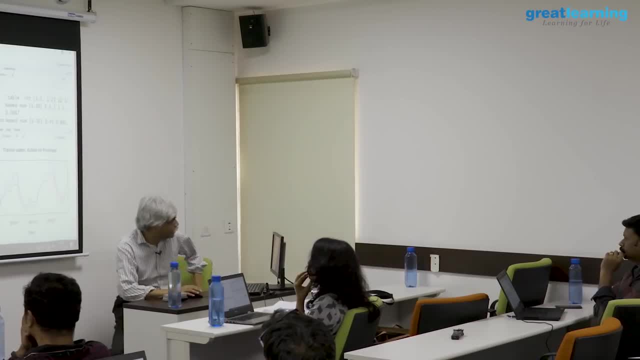 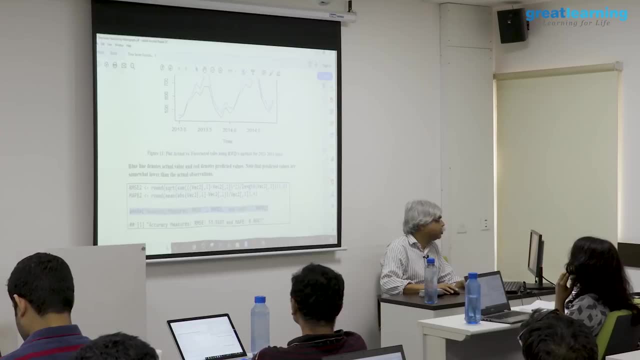 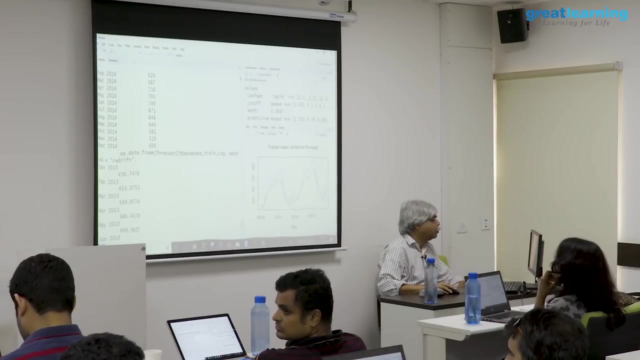 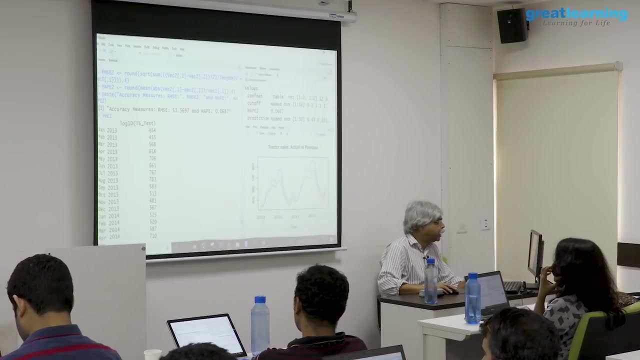 number of tractors. so I forecast right, so. so, for example, let's say here: but let's test, test- we do consider the actual actuality. now, based on this actuality, what they measure today they say that this value is what a number there is a purchase now counted Barker's that구두. 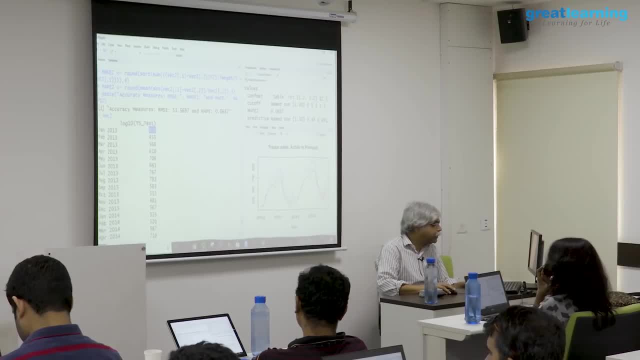 so let's look at so, following it when you have those two measurements here, as expected. so this is what a sales or net sales report is my number. what did this tell us in the test? this is the activity value. so my actual number, this, this is property. 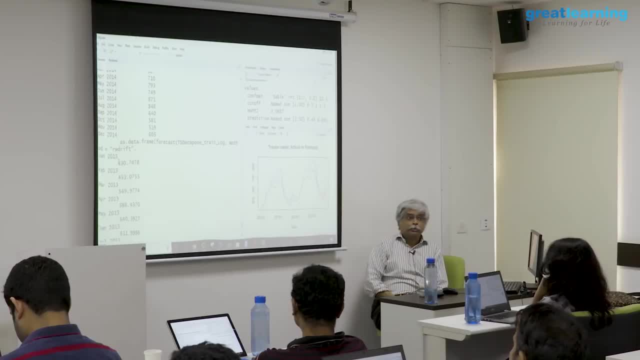 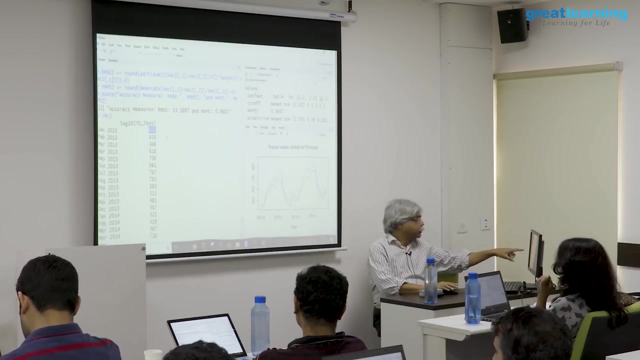 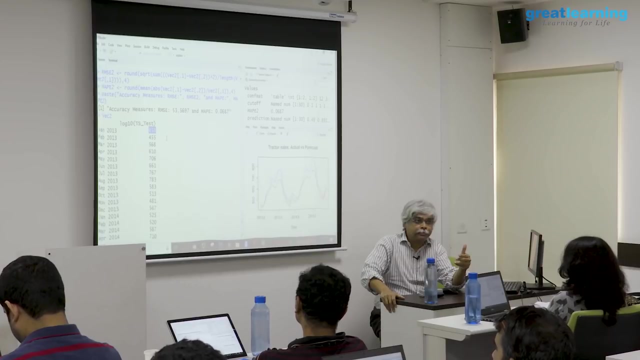 point seven. four. four hundred thirty point seven four was my forecast. what was my actual? four fifty four. I'm off by how much? by twenty four units convert that into percentage and that is about six point something. on the average over the years. how much of my forecast is from my actual now, if I choose to think? 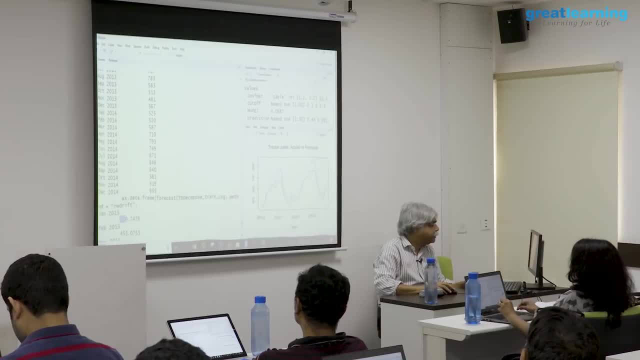 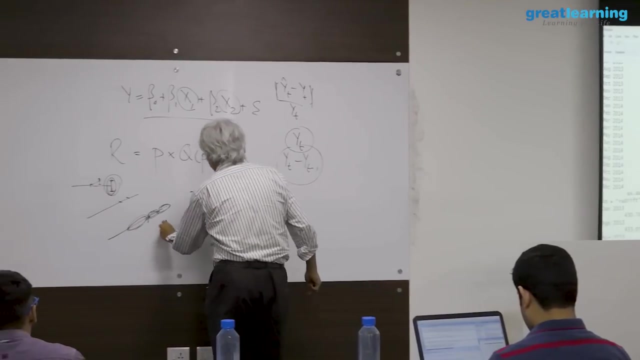 of it as an error. this has this as a point. estimate has a root mean square error of 53 right. that means if I want to give the forecast not as a number but as an interval, I should say what it should be is four hundred and thirty. 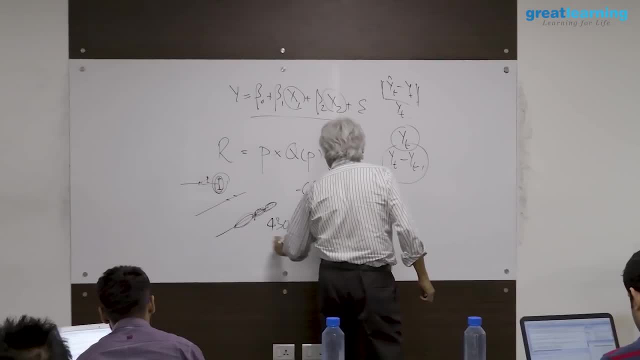 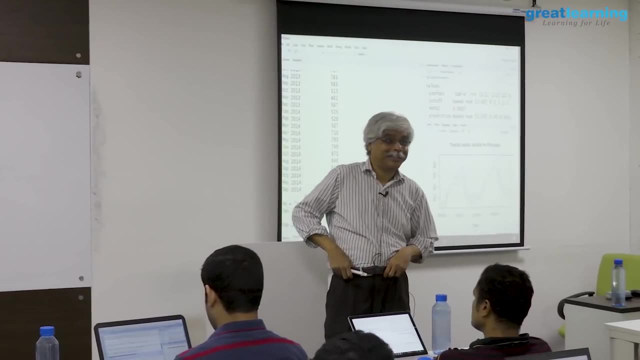 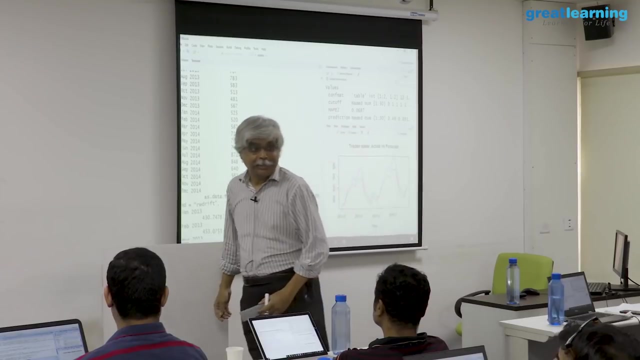 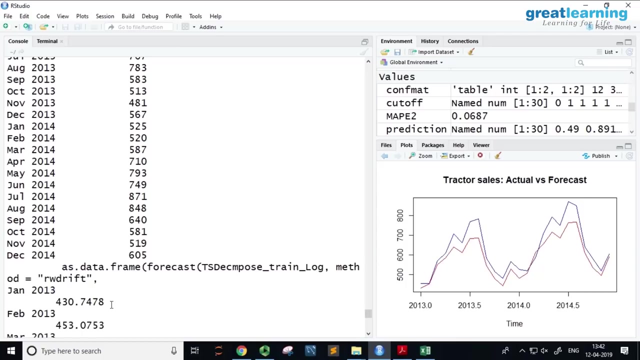 plus nine minus, say two, into fifty three. that's, that's huge for ninety five percent. or or, if he allows me, if he allows me the normality assumption, I will. I will make this one: point nine six. this error is point five, three in standard deviation terms compared to fifty three. this 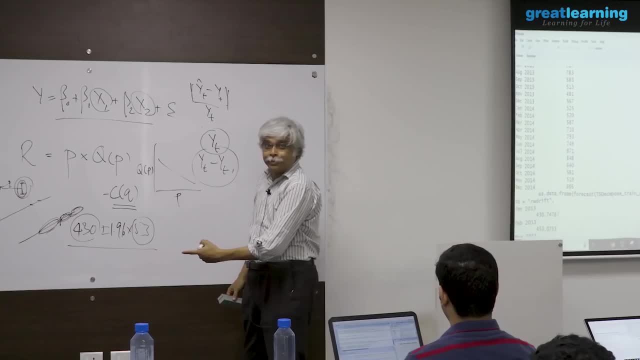 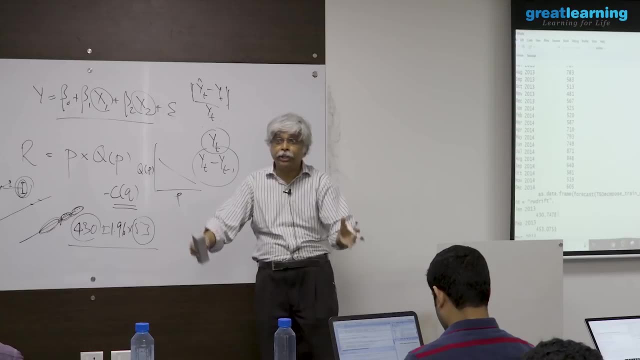 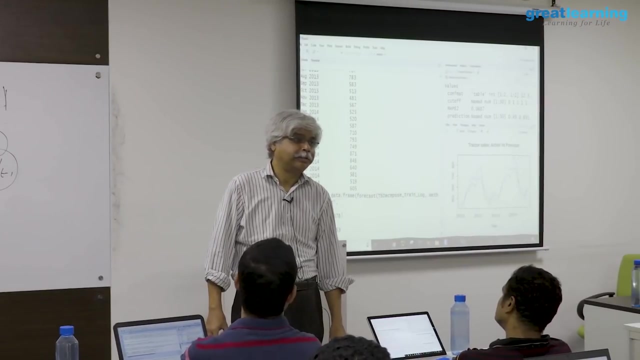 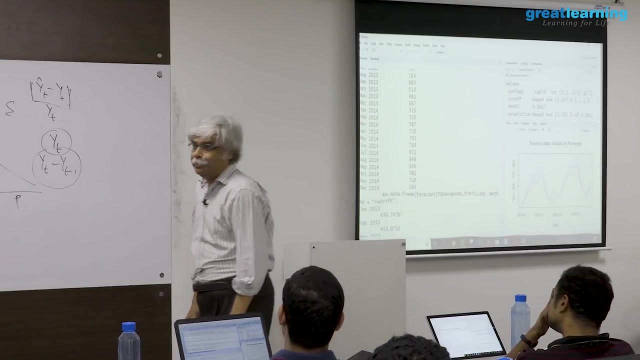 is at about ten percent of this as a percentage is not bad, but you're right and actual sense terms this gives you a fairly large interval. but what that means is that a plus-minus ten percent at a sales of 500 is a lot. true, if you know your error, if you know your salary to within plus-minus ten percent. 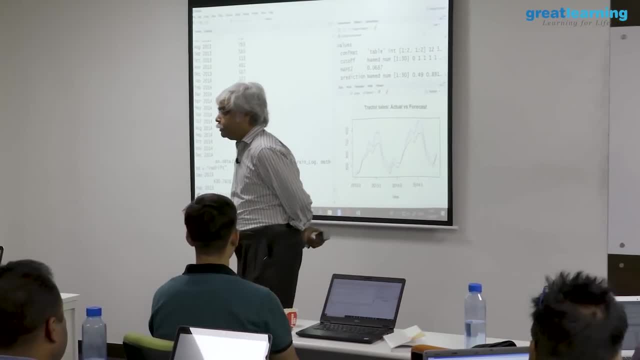 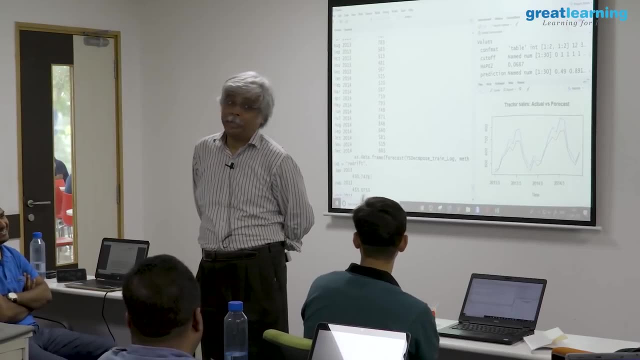 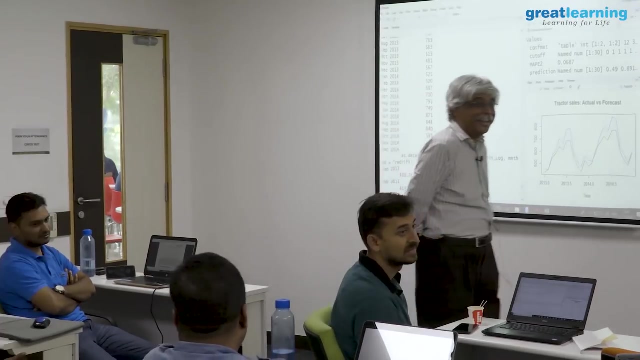 you may or may not know it very well, but if, let us say, Mr Rambali knows it to within plus minus 10%, that is many companies, right, that error is many, many companies. No, again, it is talking about sales. then it can be since the tractor sales per unit tractor. 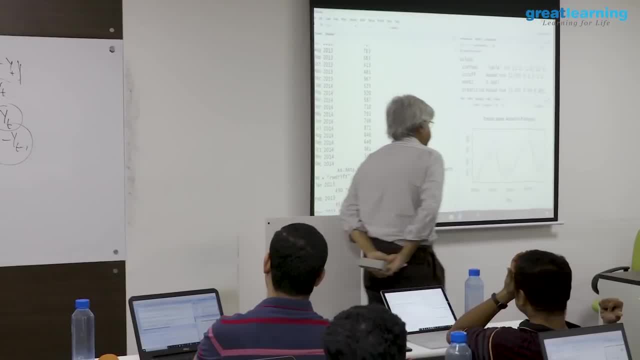 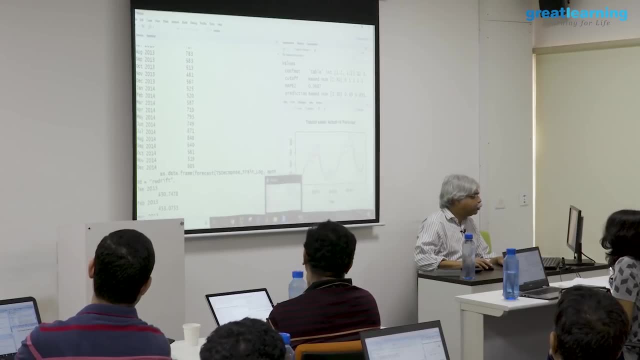 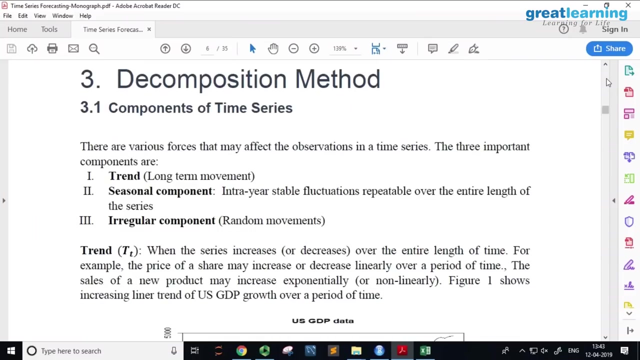 as a significant per unit tractors, but remember that that is the, so this is the variation, right? so let us say a plus minus of a 100, but let me go back and let me show you what plus minus of 100 actually means. So, if I go back to the original series, this is the series, right, this is the series. so 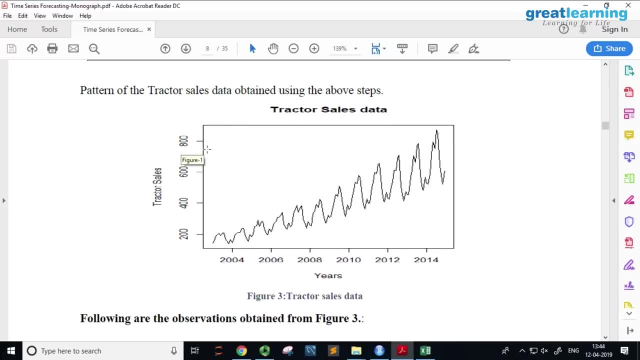 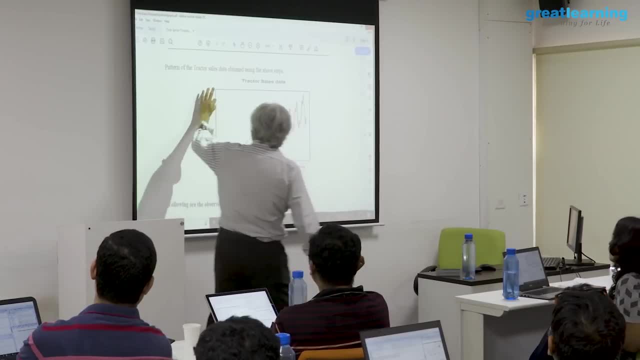 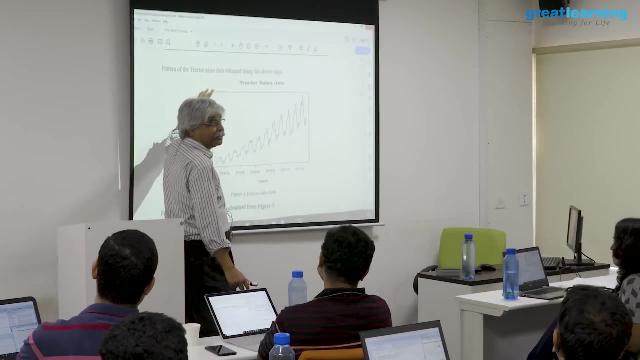 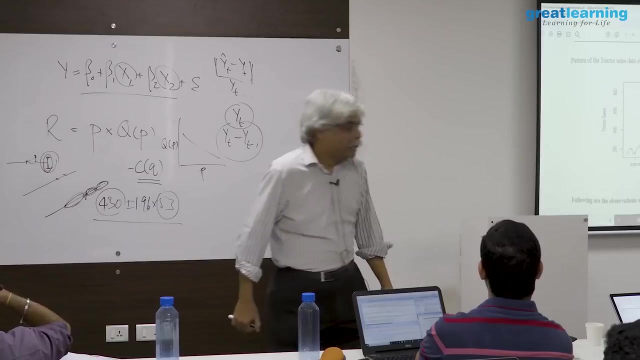 plus, minus of a 100 means what here, Plus minus of 100 on this plot is how much it is that much. So you know your forecast to that much, still not impressed. Where did I get that 1.9? say, as I said he, he should have kindly allowed me normality. 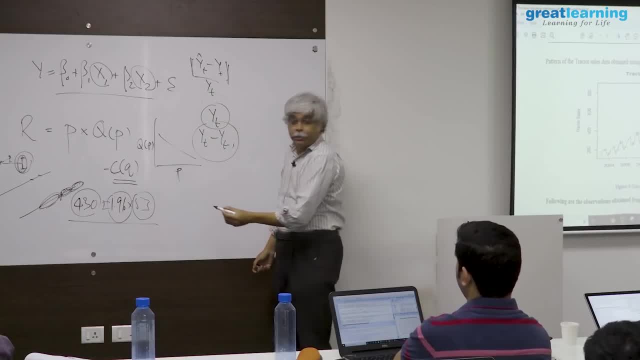 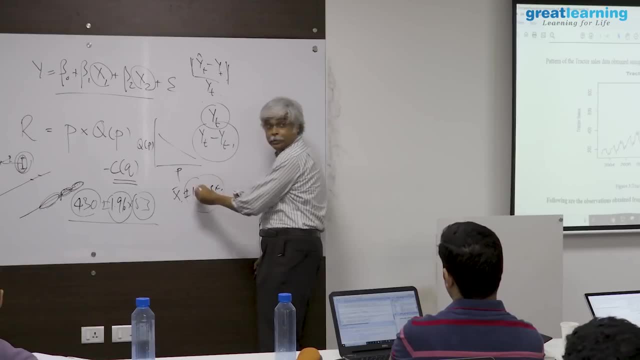 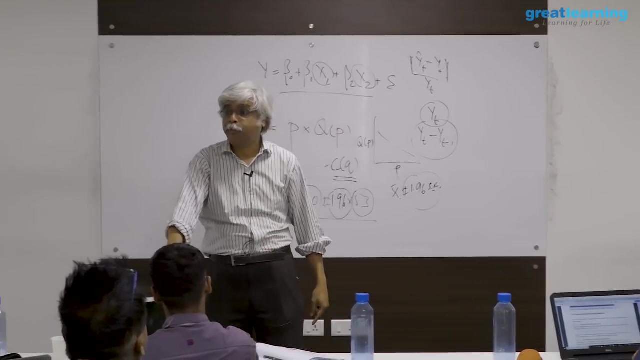 Your 2 sigma, your remember your confidence intervals. you use it as x bar plus minus 1.96 into into standard error or some such thing. use formulas like this same thing. Yes, If you want. this is an interpretation of what that root mean square error is. there is a. 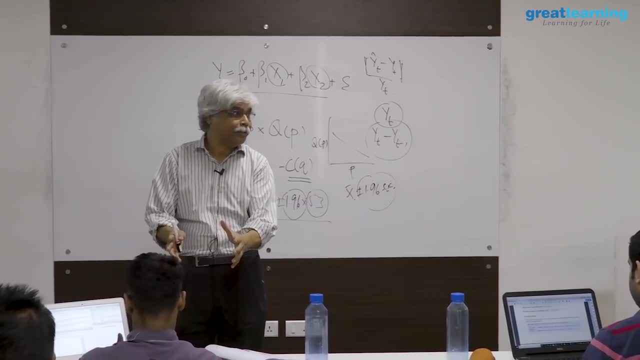 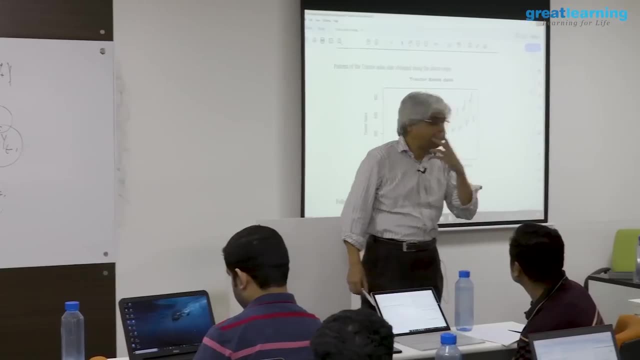 number 53 sitting there right, I am trying to give you an interpretation for it. Yes, so plus minus twice, that is going to be about 95% confident. If you want to standardize, you can look at your MAPE number and say that that should. 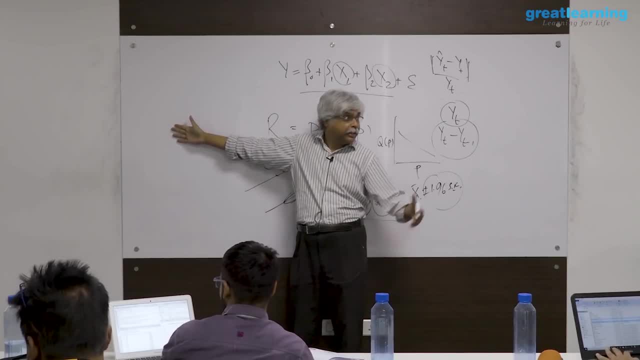 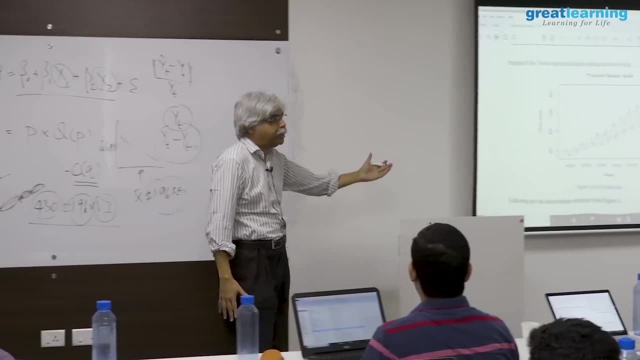 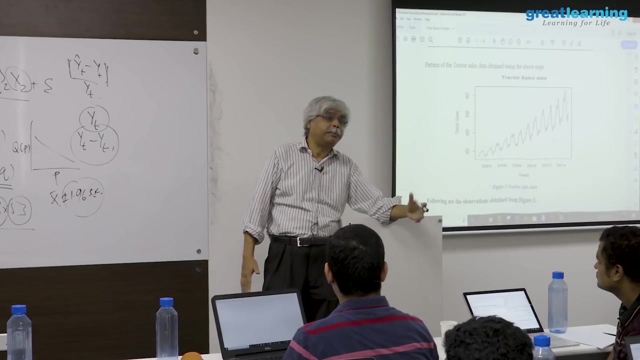 be less than some percentage. but what percentage that should be depends on business and how it is like. how square, how big should your R square be? how small should your MAPE be? RMA C: no, because RMA C is on the scale of the actuality, but MAPE yes, you can put a number. 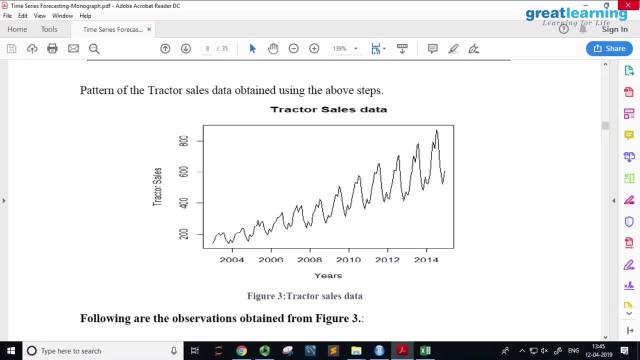 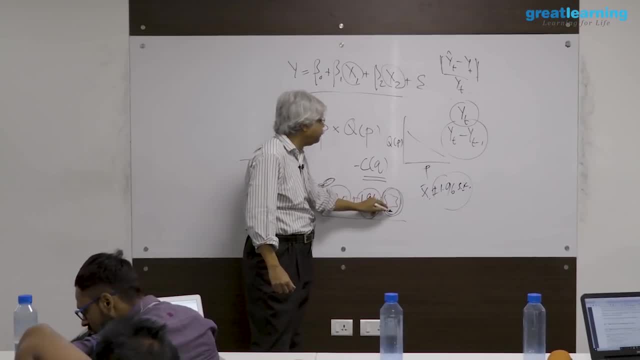 on it and say that I need to be at least 10 percent sure of my yes, which is the point I was making. that is a percentage sense. 53 as a permissible error or even 2 into 53 as a permissible error. around 430 does not look that bad, but you are also right that it means. 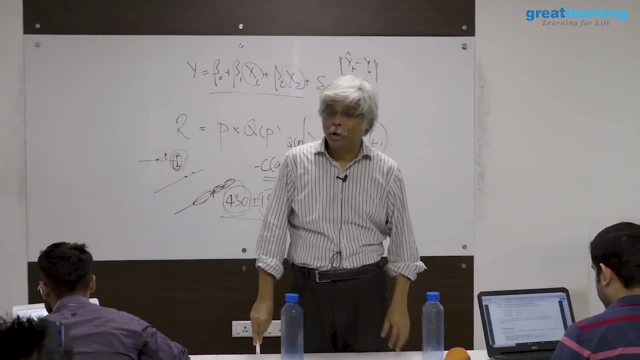 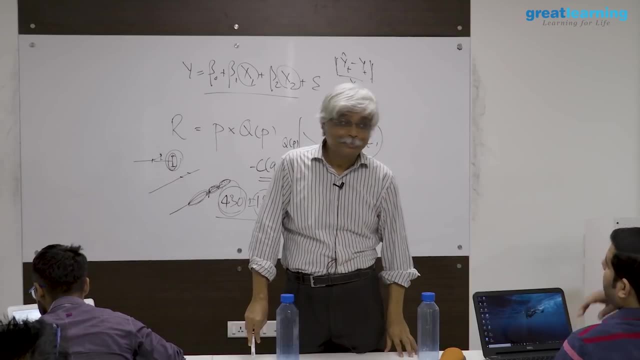 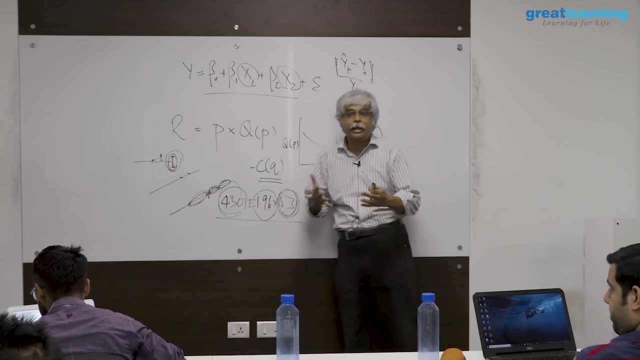 a 100 or more factor. 100 or more factors, So you are off by a 100 factors, which means that if you want to incorporate that risk, you are now playing around with 100 factors. yes, so you may say, from a practical perspective, that is not necessarily a workable range for me. if that is the case, then let us get better. 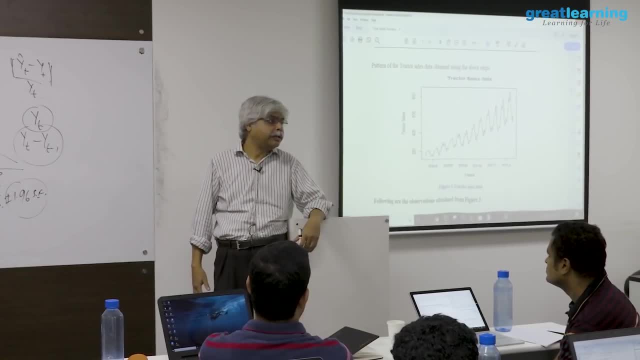 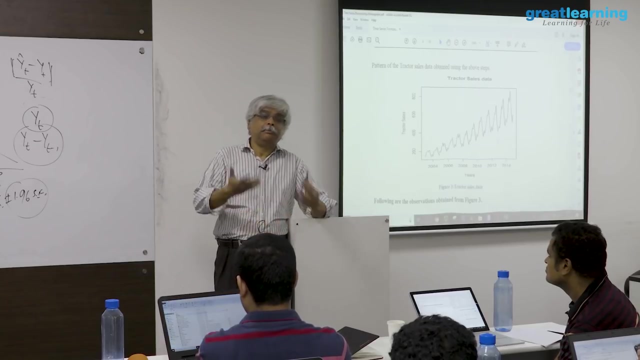 forecast out of it. let us use other data to get better forecast out of it, or maybe build a more sophisticated model. that is like saying: you have an, you have an R square, but that R square is not particularly good. what to do? one answer is: let us go wild and build. 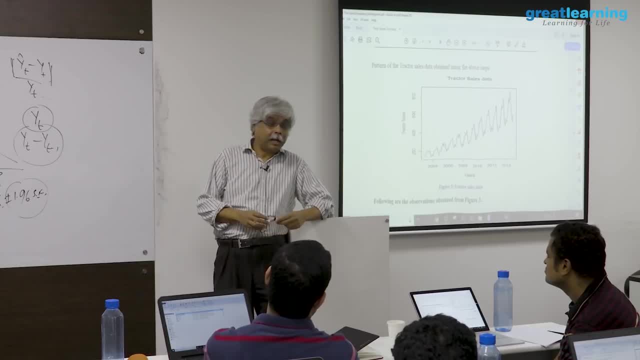 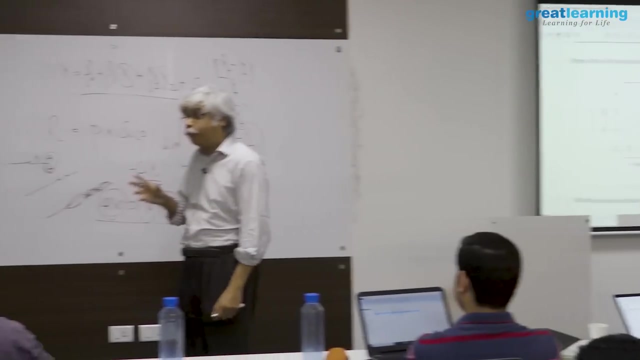 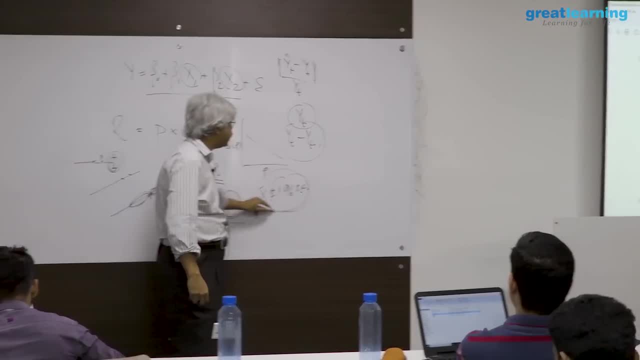 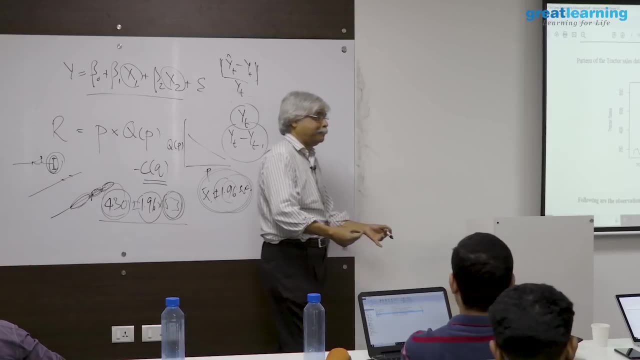 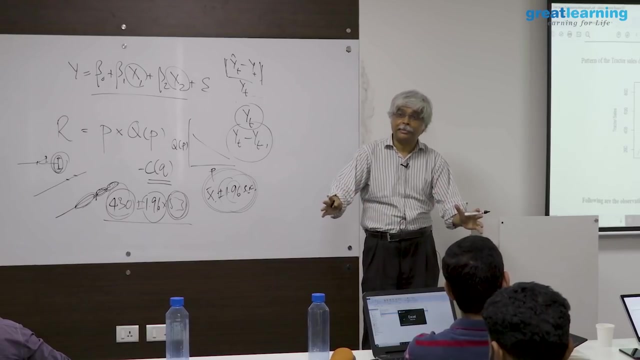 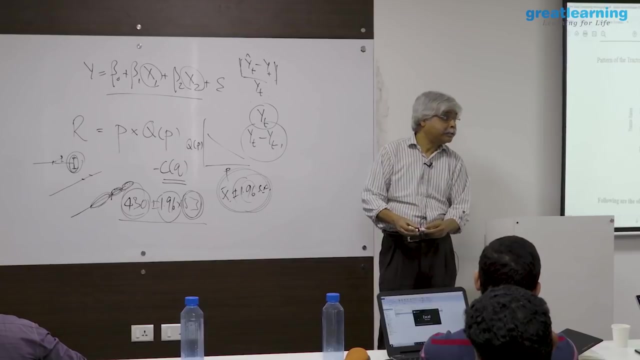 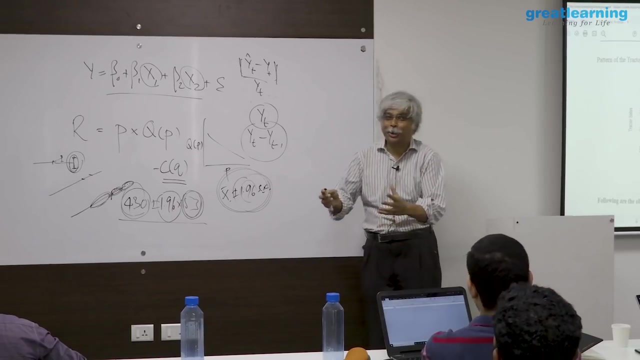 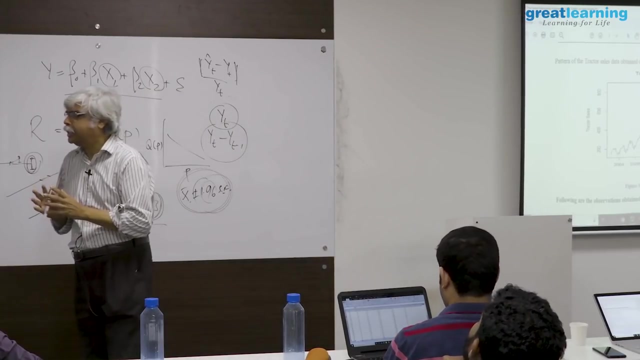 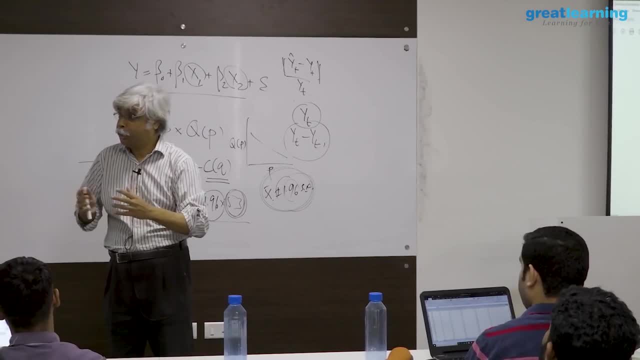 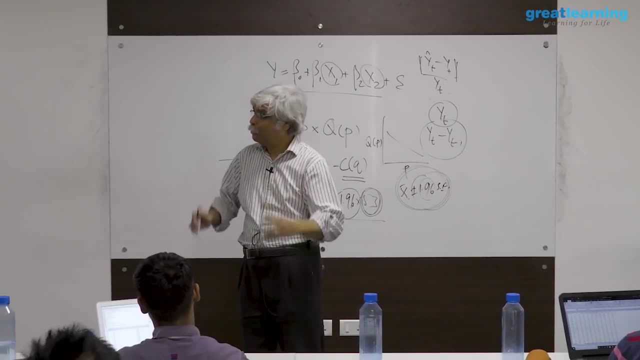 the right thing. I was like: let's say you're going deer hunting. I don't go deer hunting, but let's suppose you are going deer hunting, so there's a deer in front of you, right, you and your friend are both going there. you are all wonderful hunters. so your friend looks at it and shoots: miss ten feet behind. 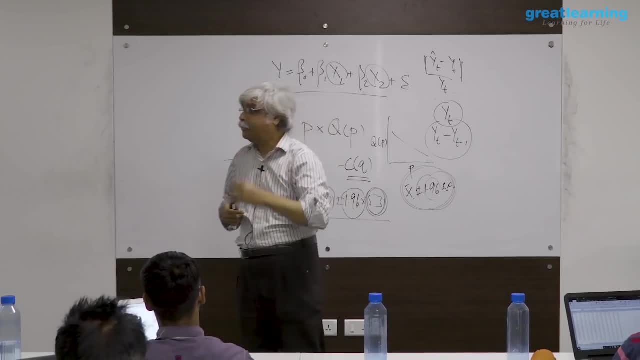 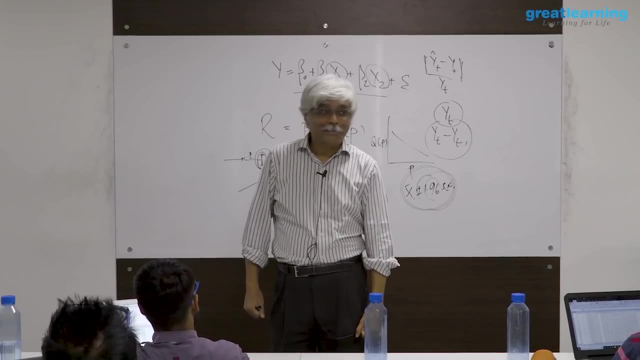 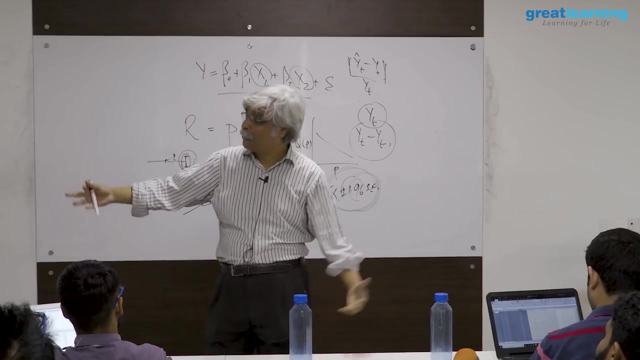 your other friend looks and says tough shoots, misses ten feet in front. you look at this and says, yeah, I jump up and down, we got him right. that's what a confidence interval. does you get the deer right by missing to the left and missing to the right? somewhere in the middle is the deer, somewhere in the 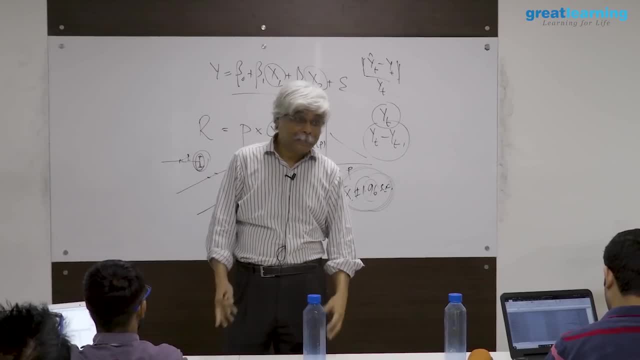 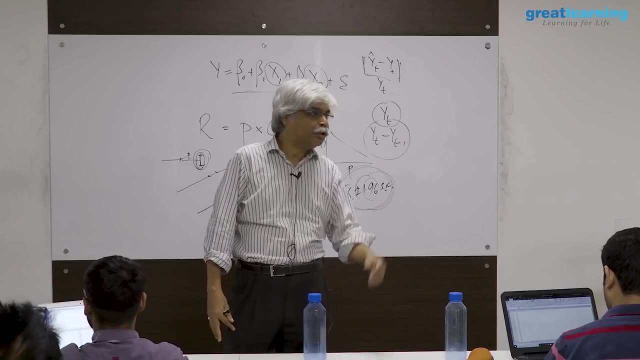 middle is your actual sales. but I'm telling you what's going to happen. if things go really, really well and everything that is uncertain, you're not going to be able to do anything. you're not going to be able to push your sales up. everything falls on your path. this is what will happen. your 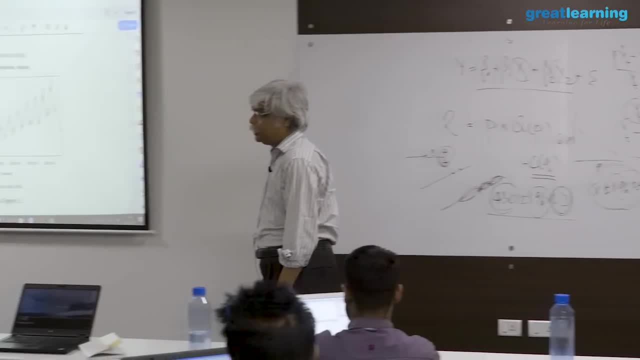 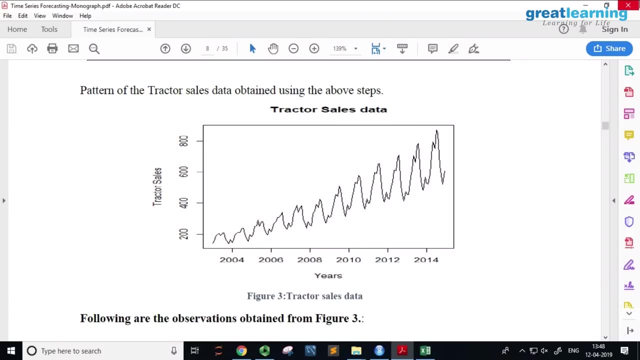 best case scenario. I'm also going to tell you what your worst case scenario is. shit happens, shit being defined by the past. and if every shit happens continuously, which means everything goes wrong, this is what's going to happen, and now somewhere in between is going to be. your state of affairs now depend on how 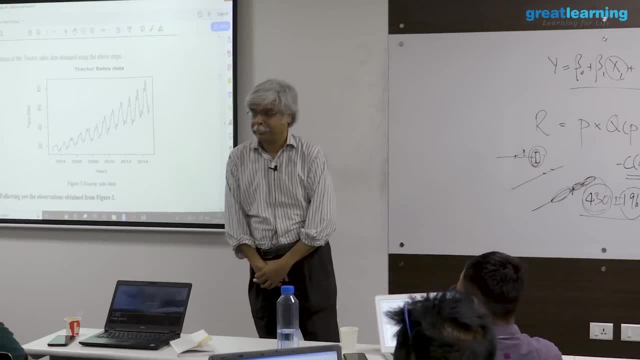 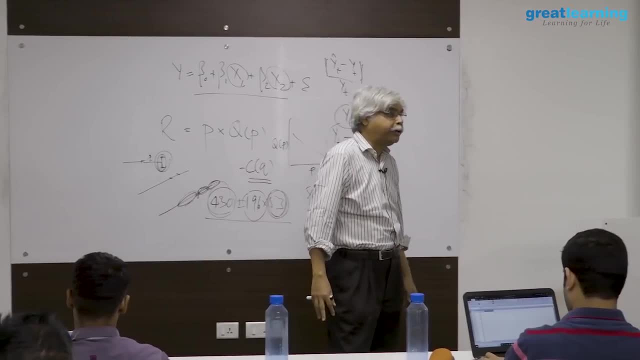 optimistic and how pessimistic you are, you deal with it. if somebody tells you that you know many good things will happen to you and you will end up with a salary of 1 crore, and somebody else tells you horrible things will happen to you and end up. 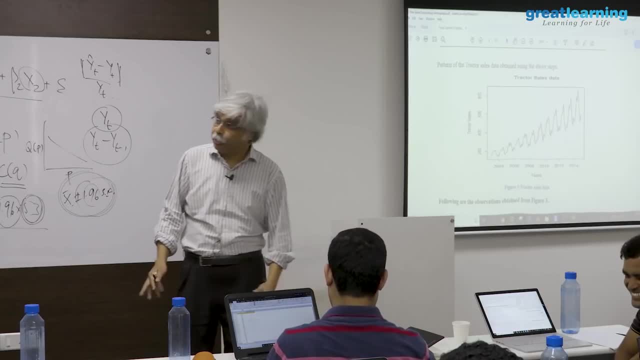 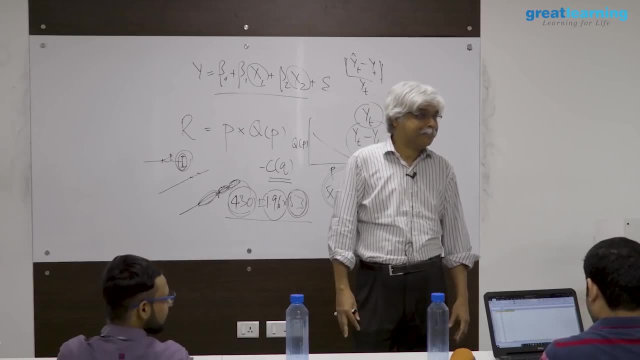 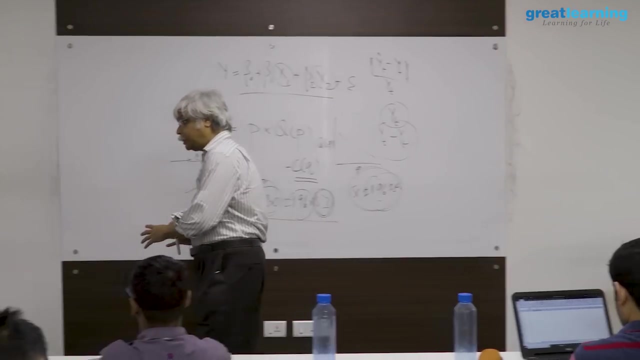 owing people 1 crore. now, based on this information, what will you do? different people, I think, will do different things, but that's not the analyst job. so what we have is: we have our first forecast, we have a, we have a model for it. how did we do it? we took the 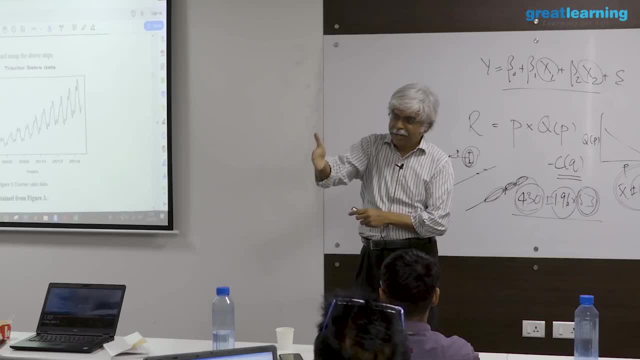 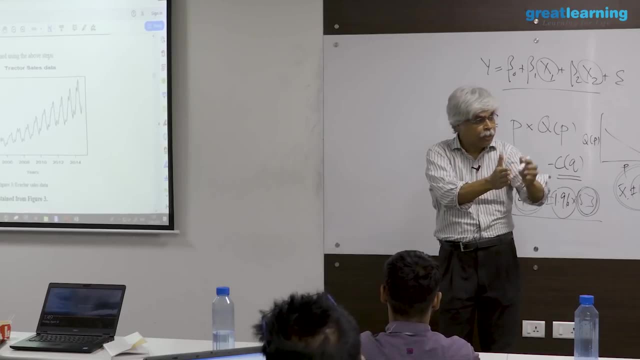 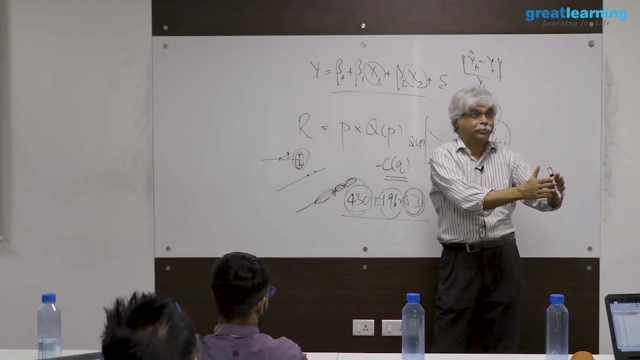 data. we convert it into a time series. we decompose that time series into trend, seasonality, etc. using that decomposition, we forecast it. that forecast we then compared with the actual on a test, in a test training way, to see how good that forecast was. we followed this process from the data to the forecasting. 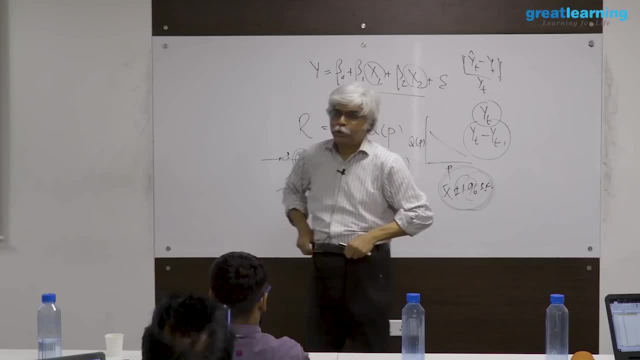 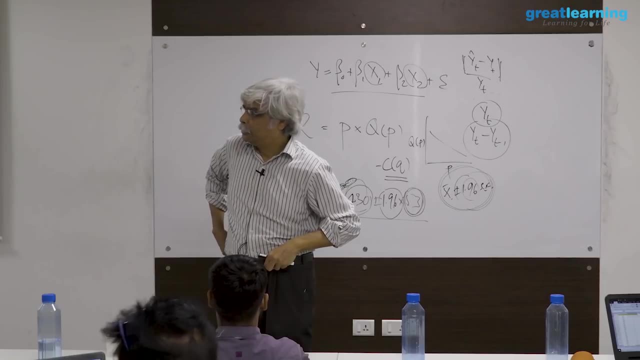 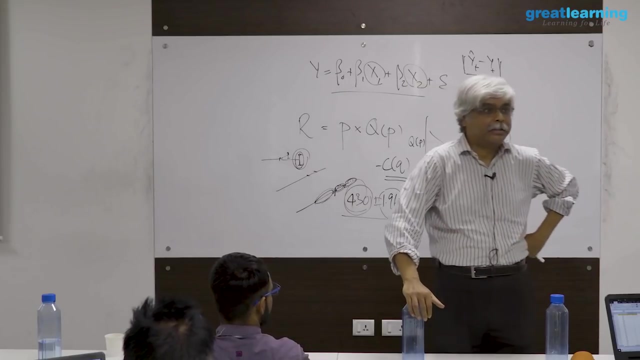 procedure, and this is a process that can be repeated. this is your first forecast. in the next two days, we'll maybe see about 10, 12, 15 more. I don't know. that's a random number, but my guess is we'll see about 12, 13 more methods and then at 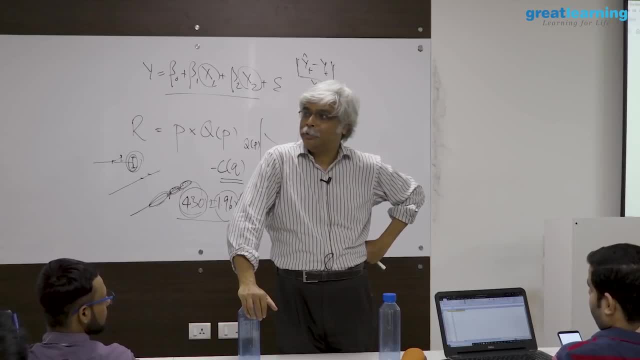 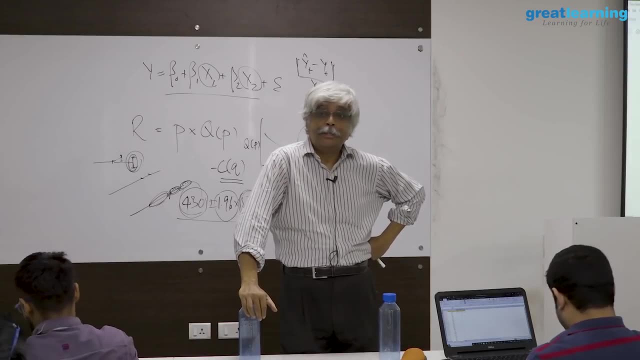 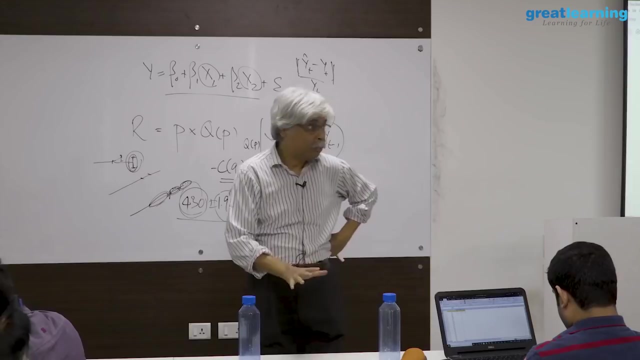 the end, or maybe I'll do very well, maybe I'll say: there is a homework, you come there. but yes, we will go through. we'll go through a number of methods- this is not the only one- and so we'll see what works and what doesn't work, and we'll see. try to understand why it works and why it. 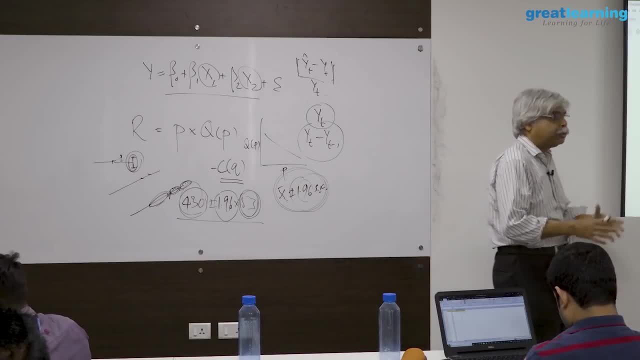 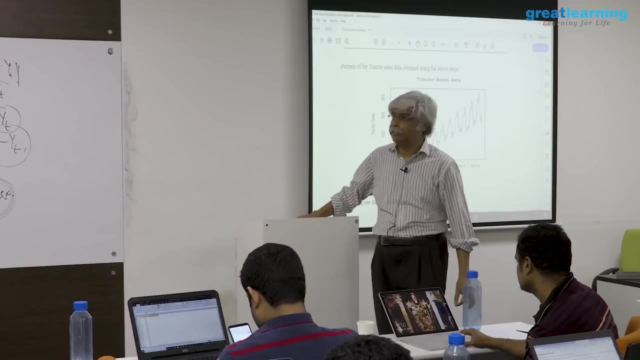 doesn't work and what one should do, what learnings there are, etc. I just wanted to end today with showing you one forecast. this is not the forecast, please. it is not what we will use at the end of the day, but the procedure. yes, data to time. 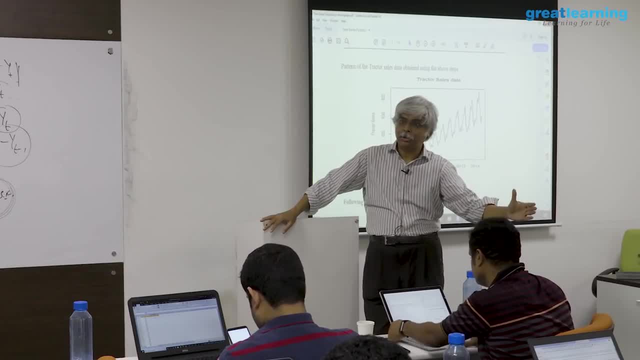 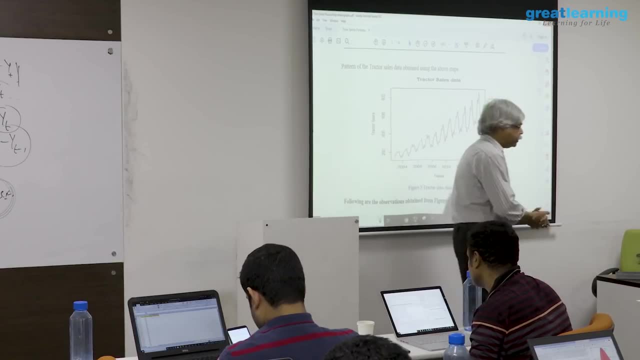 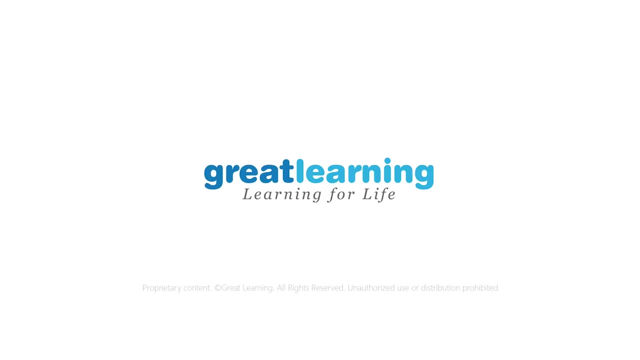 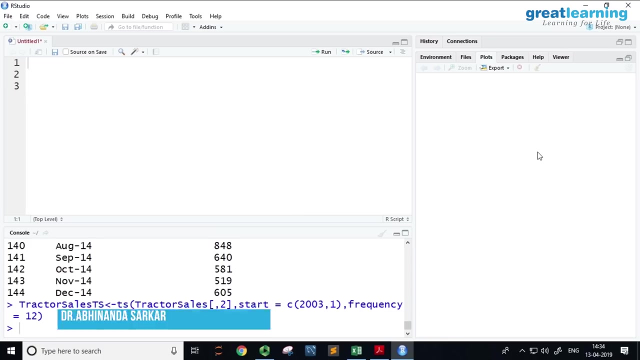 spreadsheet to time series object, to decomposition, to test training, to forecast, to RMSE and MAP. this is what we will repeat out. okay, see you tomorrow, you. so what we had done is we were studying time series analysis. to do that, we were using a data set as an exampler. we'll continue to do that today and tomorrow. 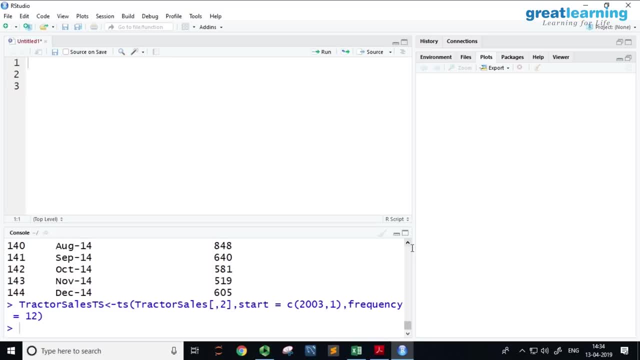 we might try our hands on a few other data sets, but the way we had loaded the data set, if you remember, is we had read a CSV file. the CSV file, when it was read, looked like this. in other words, it looked like a column of numbers: the number of tractors sold, and then a month, year. 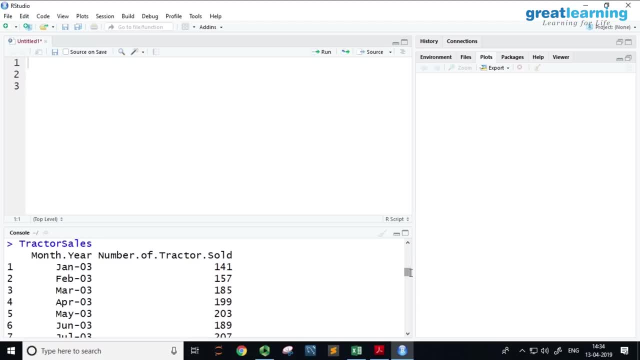 column which was not read by R in anything except for text. this needed to be converted into a time series, and the time series done by was by reading by a second column and then saying that I'm going to start this at 2003 and January with a frequency of 12. the frequency of 12, told, are that I'm looking for annual. 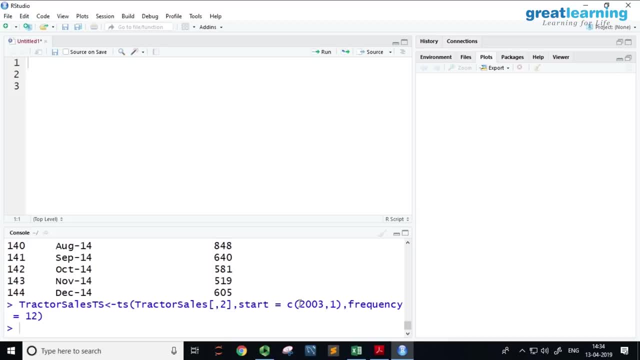 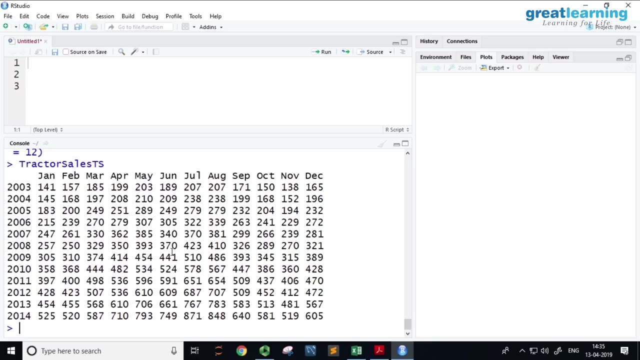 data, or data that is basically years and months, beginning from 2003, January and ending, in this particular case, in December 2015, which meant that you ended up with a data set that looked like this: then, what we had done is we have said that the problem that we were interested in was a forecasting problem, which meant: 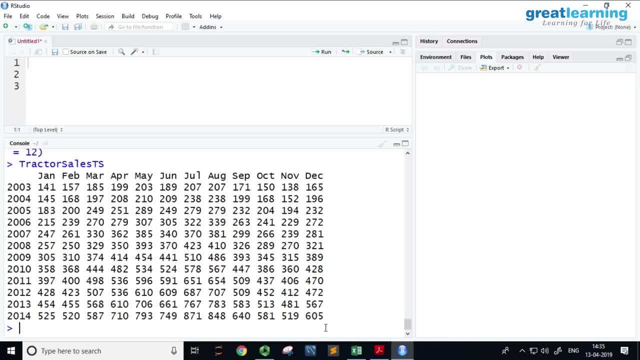 that, essentially, we were going to forecast beyond a certain period of time. to forecast beyond a series of period of time correctly. the philosophy that was being used was to say that if you want to forecast in the future, then see how good a job you are doing in. 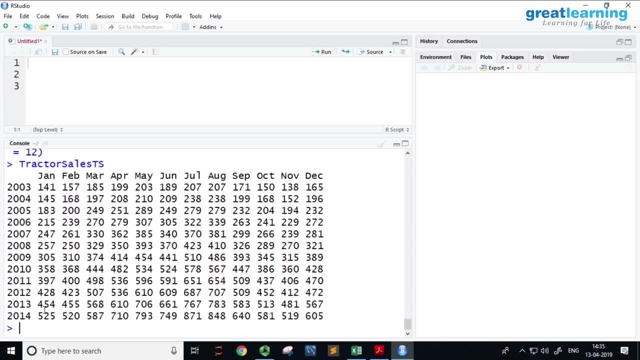 forecasting given the data that you have. so, if we are going to forecast, say, two years in the future, we needed to create a data set setting aside the last two years, defining this as a test set, and the purpose was to be able to forecast these last two years and see how good that forecast was. so the multiple 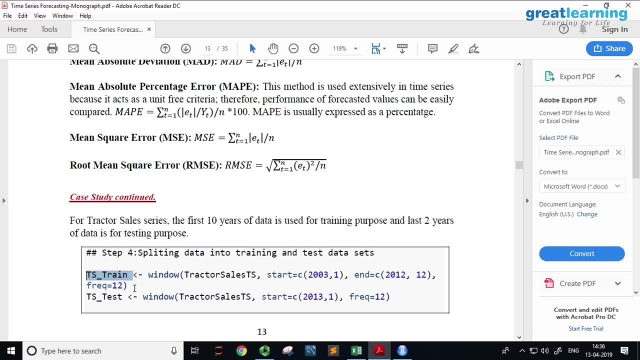 steps in that. one step, of course, was to was to set up the training and the test data sets. so setting that up. number one was to establish a training data set, and this is. you have done this before. if the code is there, is there for me, I think. 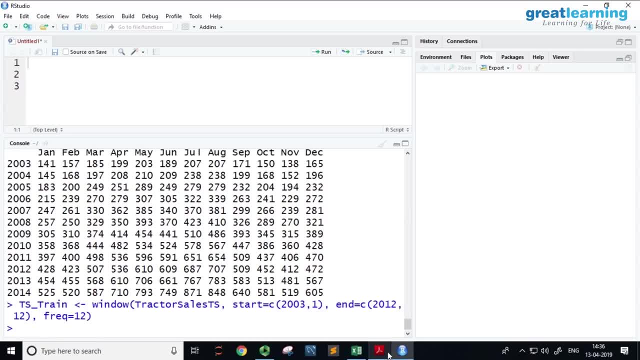 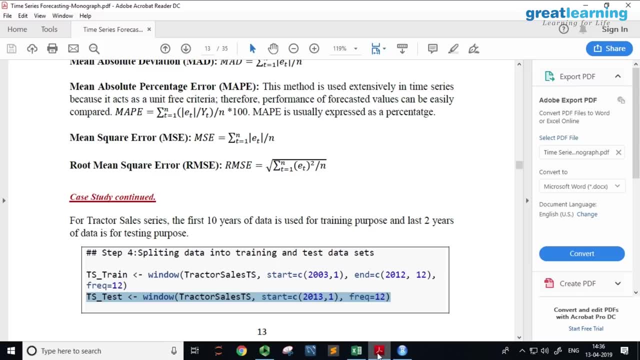 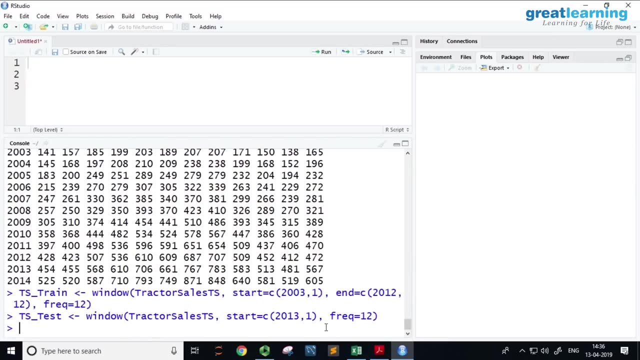 another activity happened on this computer, so we set up a training data set and we set up the corresponding test data set. if you have a start, then you may or may not need to specify an end, depending on how far the end goes. so because the second command has no end command, it basically goes to the end of 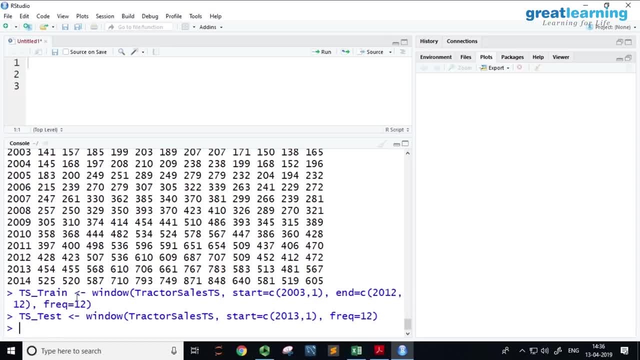 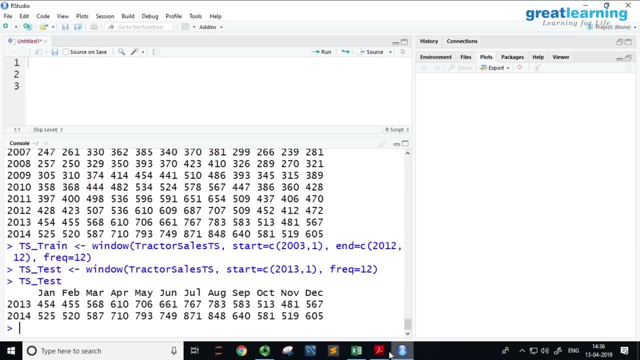 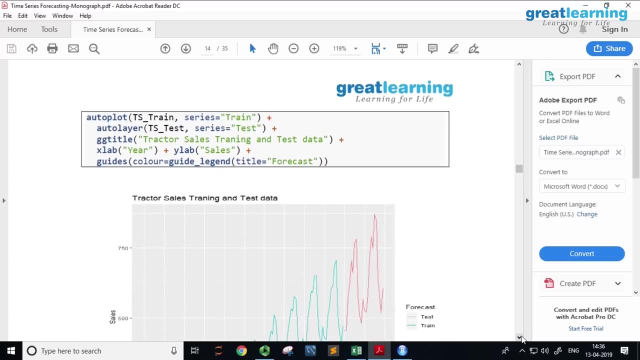 the data set. so now I've set up my training set and I've set up my test set. so, for example, my test set is of two years. I need to forecast using my training set. there are many forecasting methods that can be used. one particular method that we were doing was to try and use what's called a random walk with 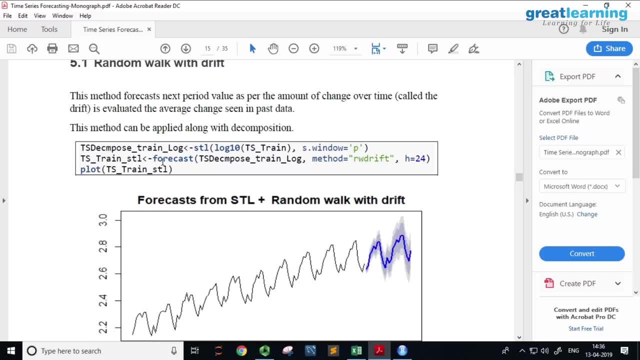 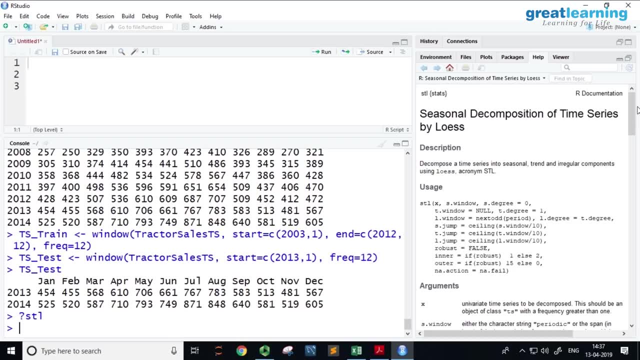 drift procedure including a function called say STL, now STL. while I didn't show this before, I can, I can do it now. I can, for example, say seasonal decomposition of time series is using lowest. lowest means sort of it's a local smoother. what lowest is is essentially 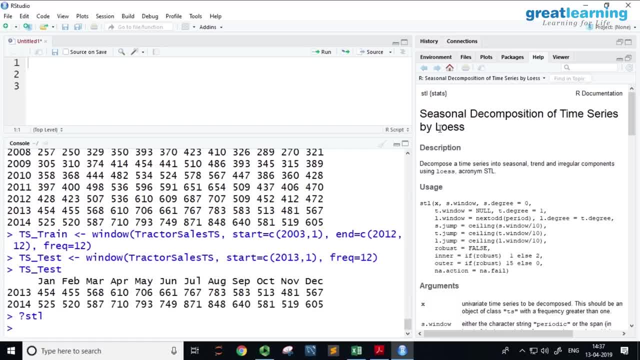 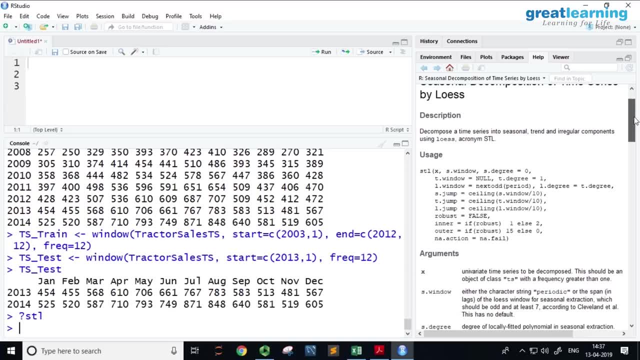 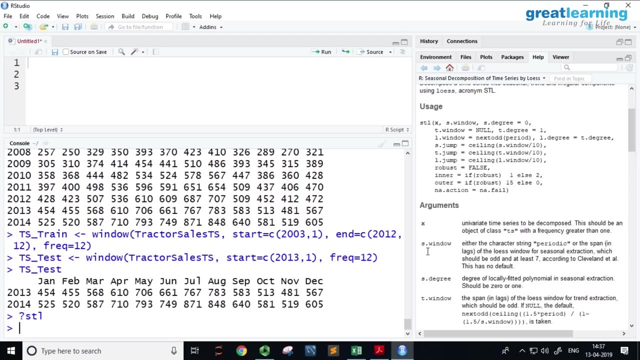 fits the kind of trend line that you were seeing, which is a smooth line. it's called a locally linear smoother. now, when STL is used as a function, it specifies a certain set of arguments to use, so, for example, one set of arguments that uses s, dot, window, character, string, periodic or the 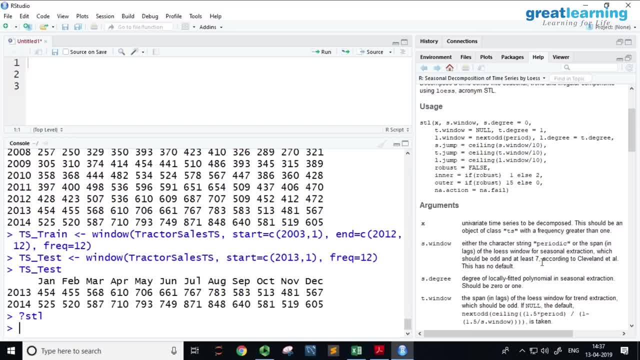 span and lags for the lowest window for seasonal extraction, which should be odd and at least seven. so what does this mean? it means that when I say lowest, I want to say how is this seasonality present in the data? if there is a seasonality present in the data, how long should my averaging be in this? 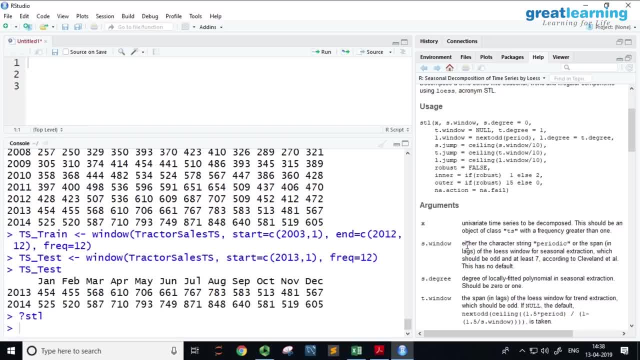 particular case, this was easy. all I said is that the periodic string is: I need things to be periodic, so I'm just going to specify that this is periodic and let the algorithm take care of a seasonal parameters. so a few things that you can play around with here if you want to. but since I would suggest that 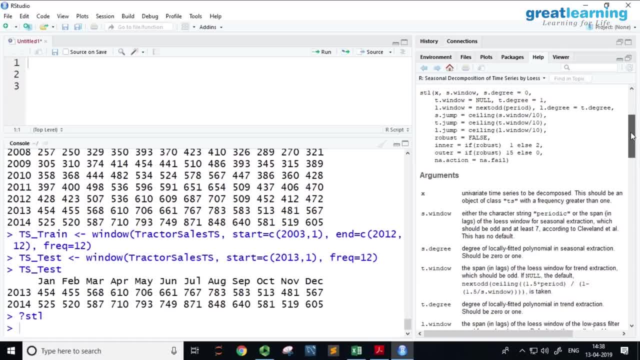 you haven't done too much training on how to fit these smoothers. just leave the default B, and if there is periodic data or seasonal data- and you're doing this- then you should say s dot window equal to periodic or some summary of that. if there isn't seasonal data, then you don't necessarily need to do that. so 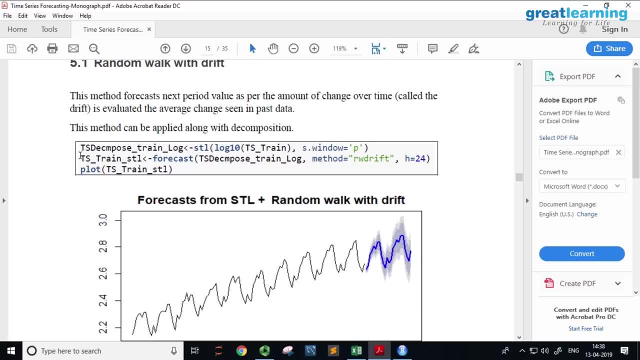 that's what this is. so how was this being done? first of all, because STL is something that looks at additive decompositions. this was done on the logarithm because this was done in the logarithm. so what is? what does the syntax mean? it means that work on the logarithm of the 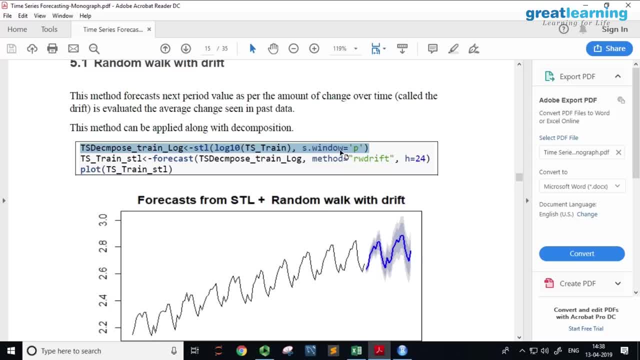 training data, assuming that there is a periodic component. periodic for this algorithm means seasonal for us, that there is a period of definition. it will pick that up from the time series. this, remember, is a time series object. so as soon as this sees s dot window equal to periodic, is going to inherit the 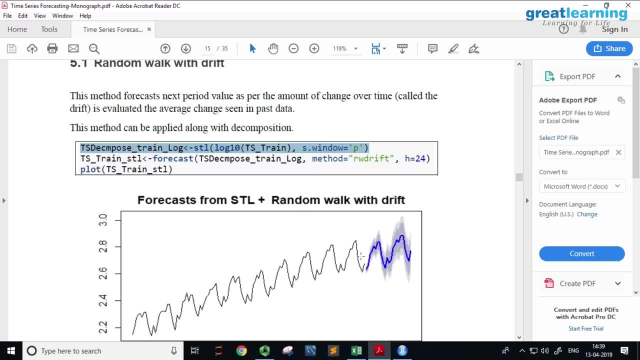 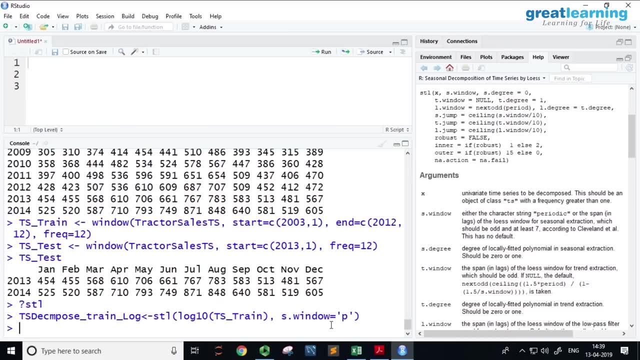 frequency of the series, which means is going to understand that there is a periodicity of 12 or 12 months cycle. that's present in this data, so decompose that again, as we've seen before, what a function like this does is it decomposes into different sets of. 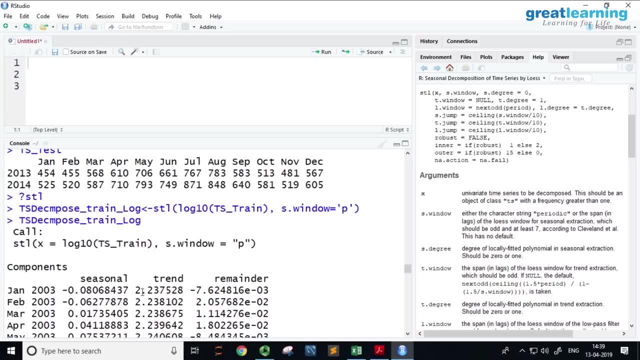 components. what are the different sets of components that it decomposes into a trend, a seasonal component and a remainder? in this particular case, it adds: what is my model? my model is logarithm of sales and is equal to this trend, plus this seasonal, plus this remainder. you 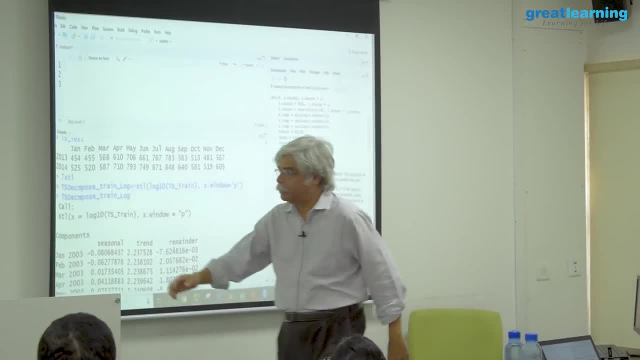 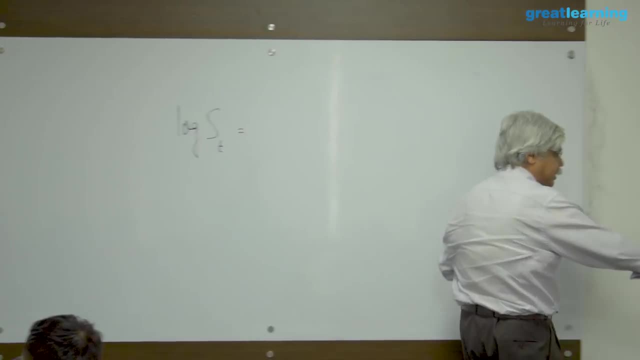 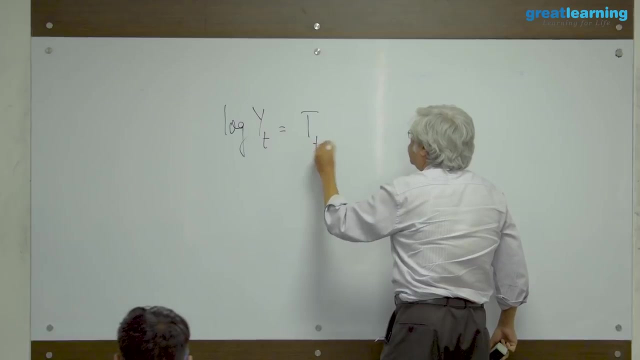 understand. so logarithm of trend is so in my particular case, my model is so I should probably drop this out. log of sales is equal to, let's say, trend. I shouldn't say sales, say YT, say trend, plus seasonal, plus my irregular compute, I think I'd call it I. 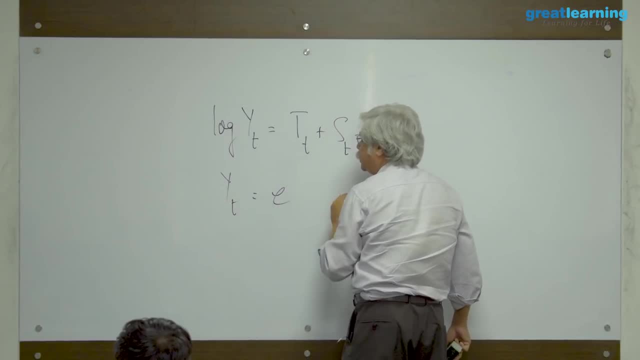 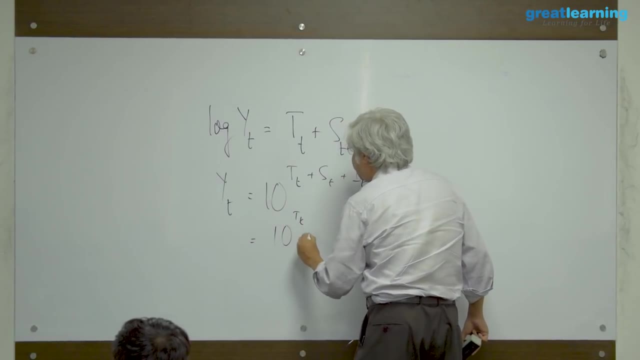 should probably drop this out log of trend. so YT, therefore, is equal to what, e to the power, sorry, not e 10, which is equal to 10 to the power trend multiplied by 10 to the power multiplied by 10 to the power, irregular multiplicative. so so. 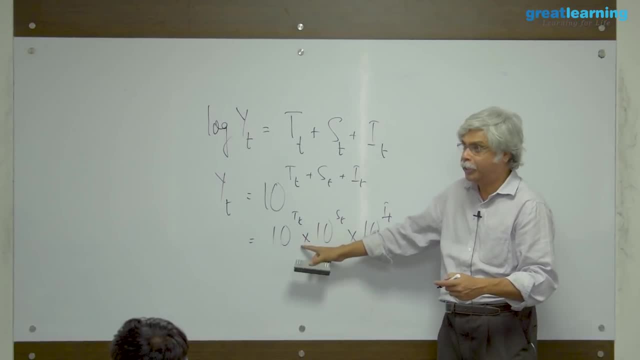 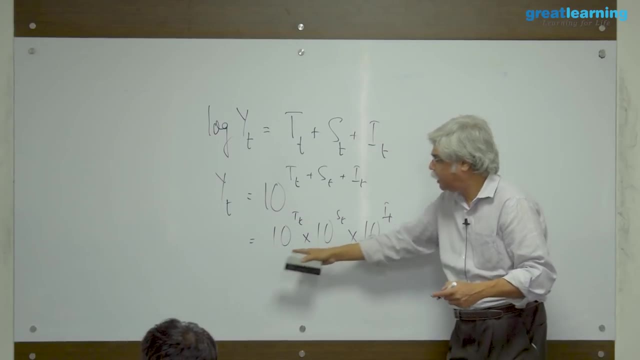 I've ended up with a multiplicative thing. I've ended up with a multiplicative thing of trend, a multiplicative thing of seasonality and a multiplicative thing of irregularity for YT itself. which means that when I want YT to look like this- a multiplication of something in trend and seasonality regular- I might as 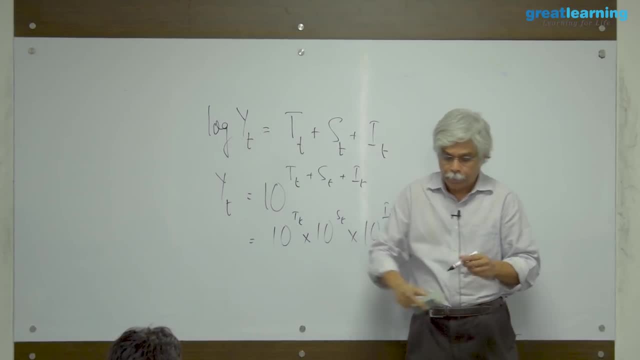 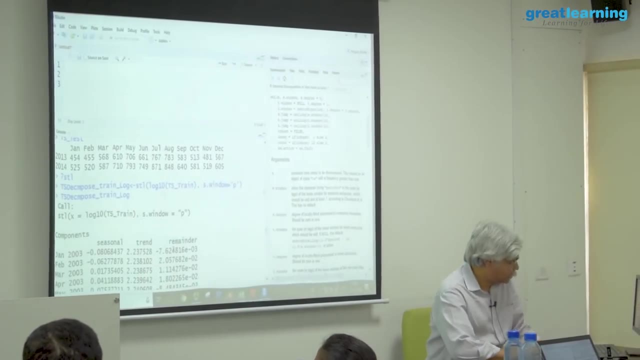 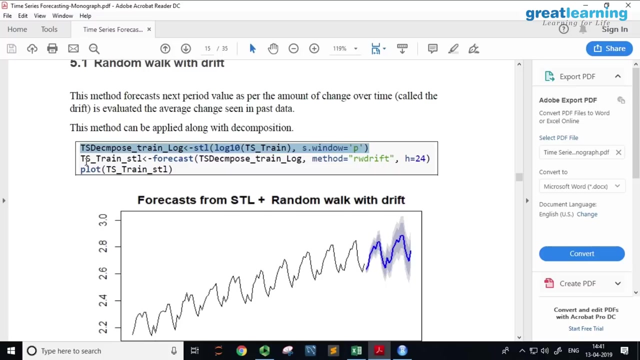 well work with logarithm and additively now, the land, the random walk function or any of these decomposition functions are much more naturally done on the logarithmic scale, which is why it's done this way. but the price that we have to pay is we now have to go back to the original scale later on. so now, what do I? 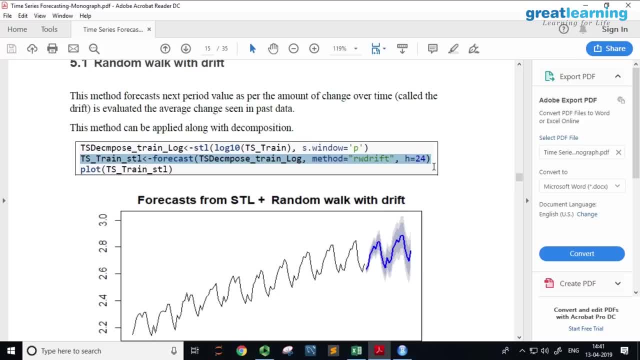 do now? I forecast. how do I forecast? well, what I do is I say: you've got this model on the logarithmic scale. I'm going to forecast 24 time periods ahead and I'm going to forecast using a random walk with drift. now, in this particular model, I've already incorporated the seasonal 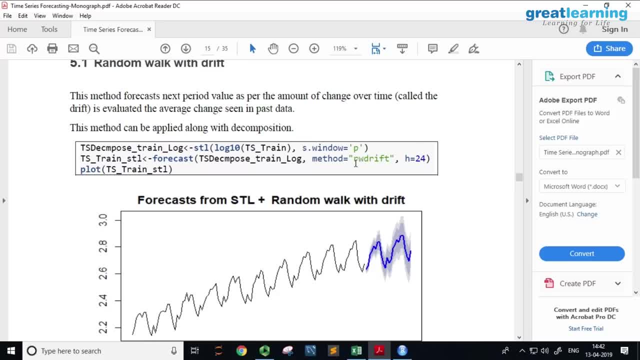 parameter because I've given s dot window is equal to P. so when this method is used- the forecast method with random walk with drift, it already knows that there is a seasonal component that I need to incorporate in my forecast. H equal to 24 means that I need to forecast for 24 time periods. 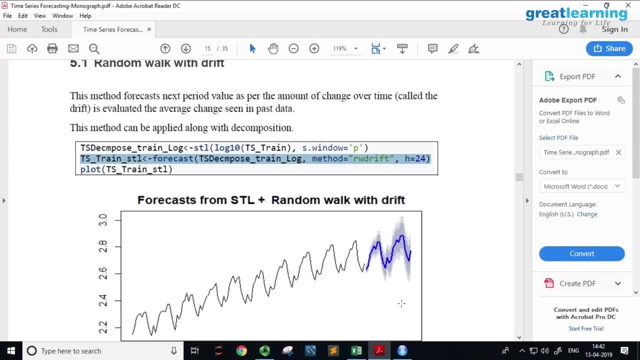 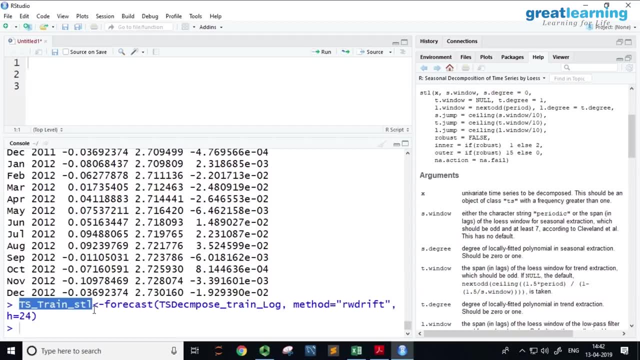 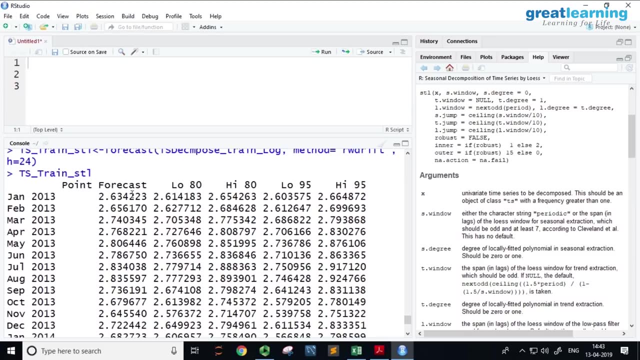 the the. the typical default for this, I think, appears to be 12, but just to be safe we can specify 24 in this case. this is my forecast for the training data, but it is forecasting 12 points. I'm sorry, I'm 24 points in addition to the forecast on. 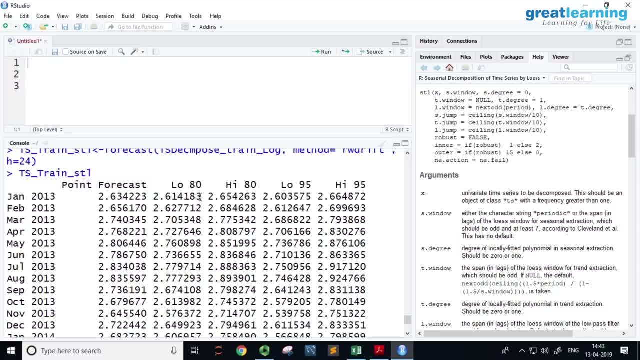 the logarithmic scale, it has also given me a lower 80% point in a higher 80% point and a lower 90% point in a higher 80% point and a lower 90% point in a 95% point in a higher 95% point. what does this mean? it means that I'm 95%. 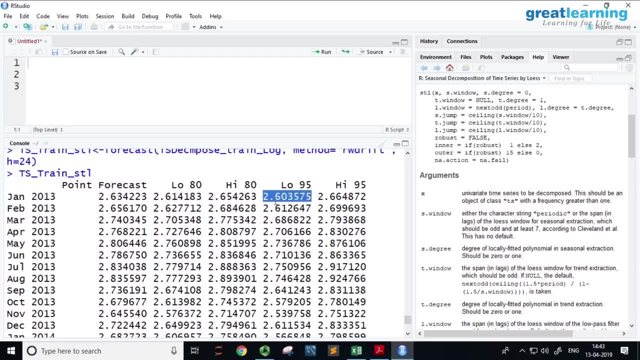 confident that, on the logarithm, my forecast is between 2.6 and 2.66. what does that mean from? what does that mean from an, from an actual perspective? let's say, for example: do this last one, so this is 2.77. so this is going to be the. 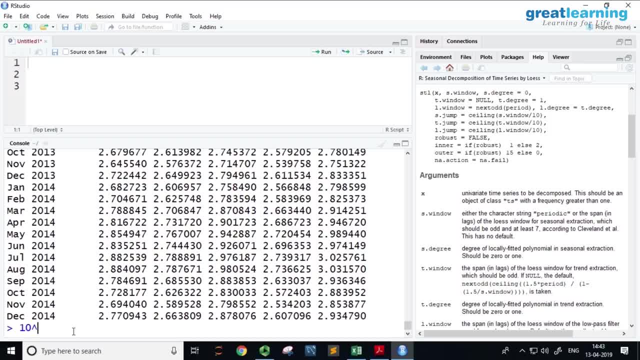 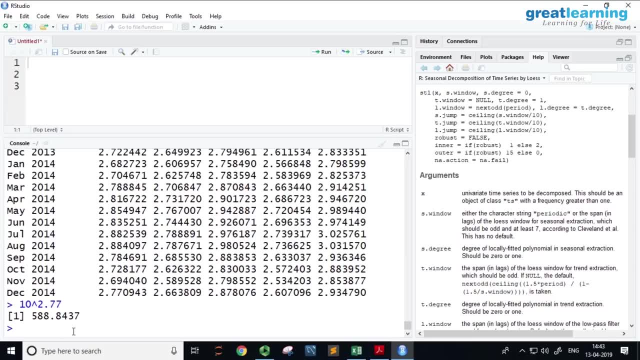 actual forecast is going to be 10 to the power. say 2.77, that's 588 and it's and it's, if you want the lower point in the upper point. the last two columns are my 95 and my 95, so I now know that this is say 10 to the. 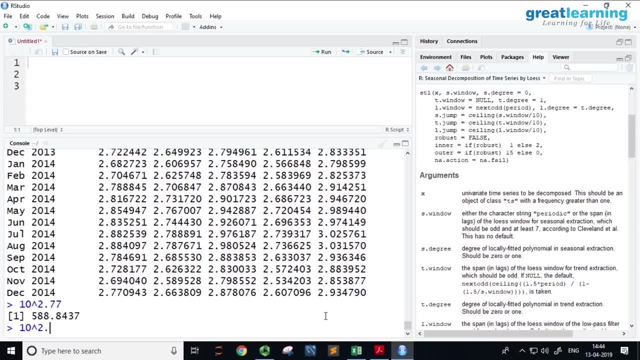 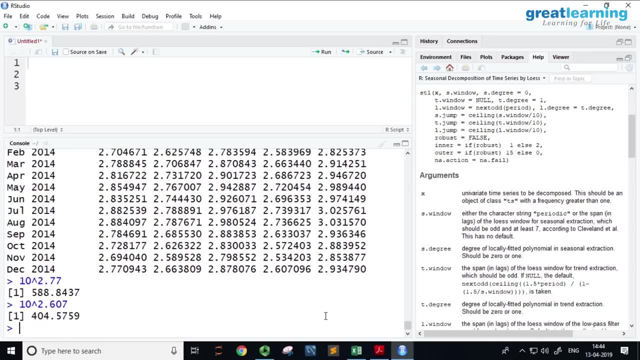 power 2, point 6: 1. so 6, 0, 7, let's say 6, 0, 7, 404 and 10 to the power 2 point 9: 3, 2 point 9, 3, 5, 860. now this is large and it is also asymmetric because the forecast is done. 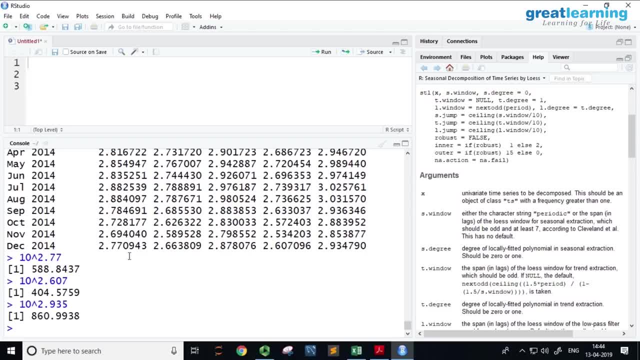 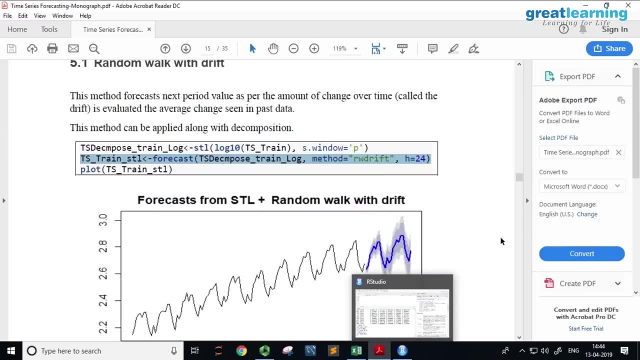 here. it's symmetric on the original scale, it is asymmetric on the logarithmic scale. so how do we take care of these forecasts and figure out whether these forecasts are any good or not? these are the forecast. so, plot train, if you plot this when you have plotted this, you have plotted this on the original origin, on. 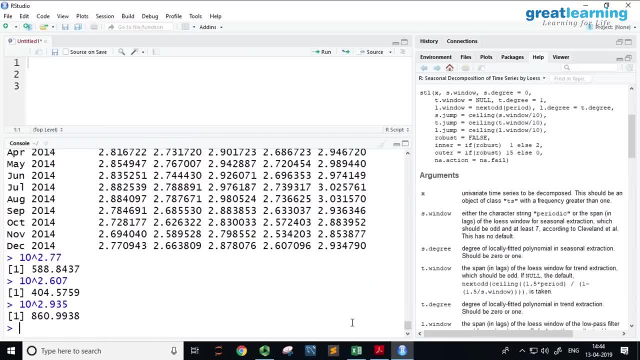 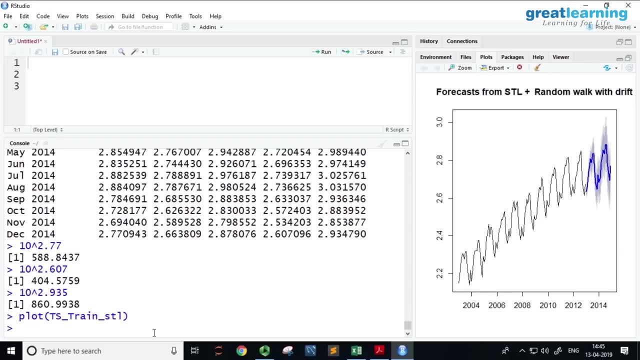 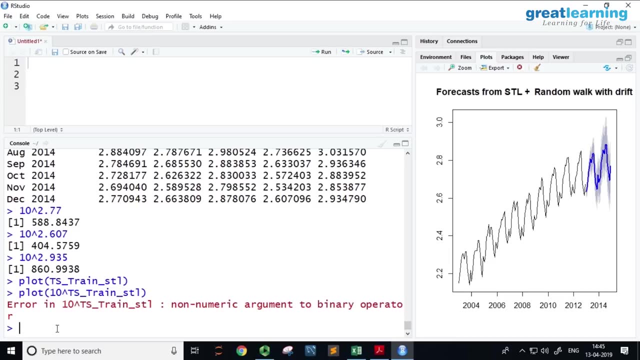 the original axis. let's say: plot off, this is on the original axis. let's try this out. for example, let's say that I do plot off and I do this instead. won't work directly, I'm going to have to go outside and figure out how to change this, but you can extract it and then you. 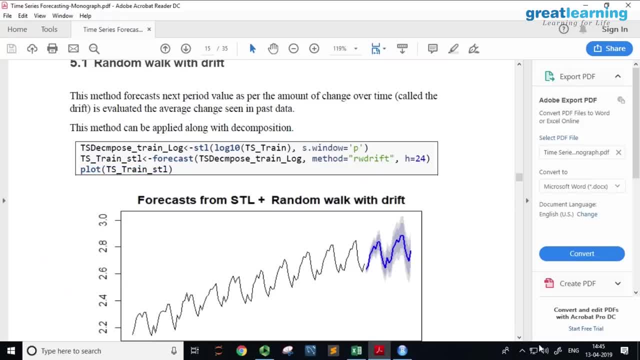 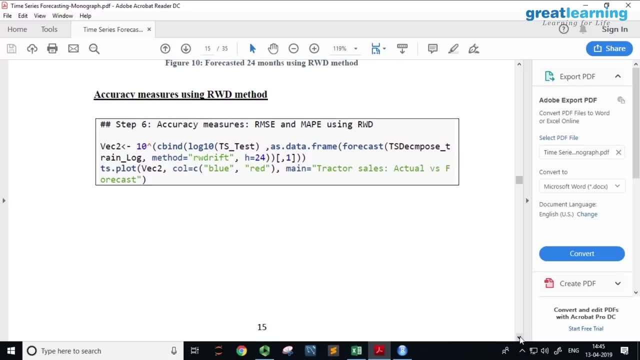 can go to e, to the power. we'll do that separately later on now. what are we going to do now? what we're going to do is we are going to measure how good my forecasts are. to measure how good my forecasts are, I will need to incorporate: 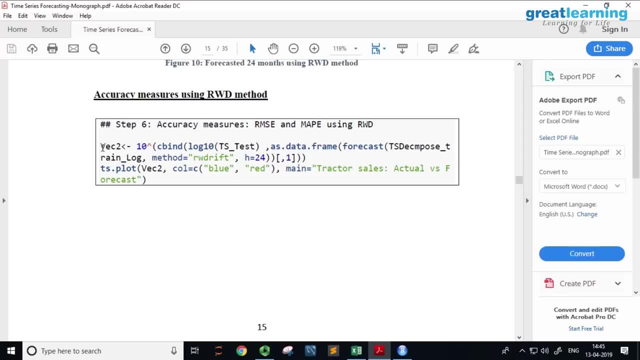 my uh forecast together with my original functions. So this function is being created. this function does what This function goes that 10 to the power, c bind the thing that I was trying to do. in other words, I need to c bind this and go log 10 to the 10 to the power, this. So 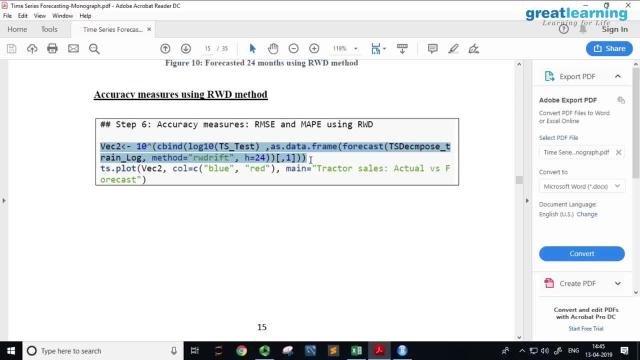 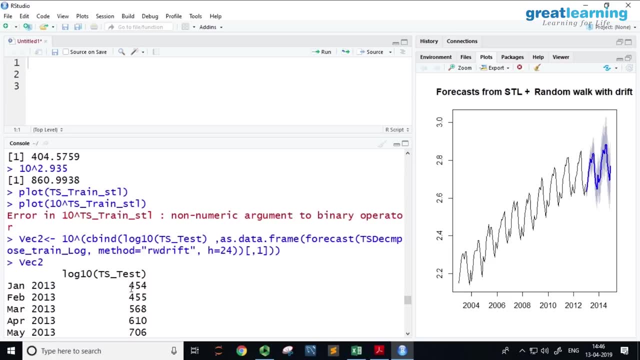 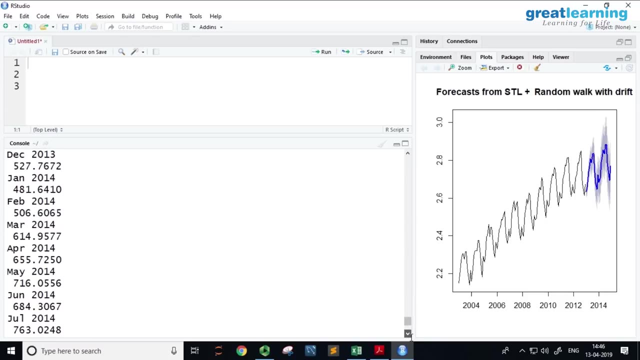 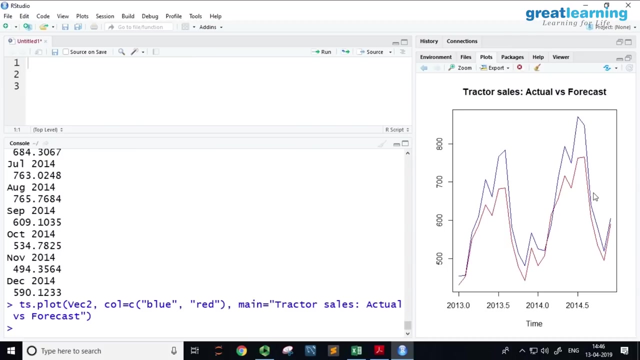 this is the forecast and this is being combined with the actual is being combined with the forecast to create this vector. The second set: this is my actuals and this is my forecast. second column is my forecast. I can plot both of these and see that I have. 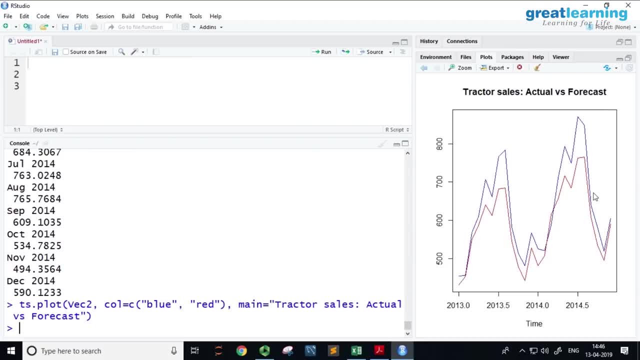 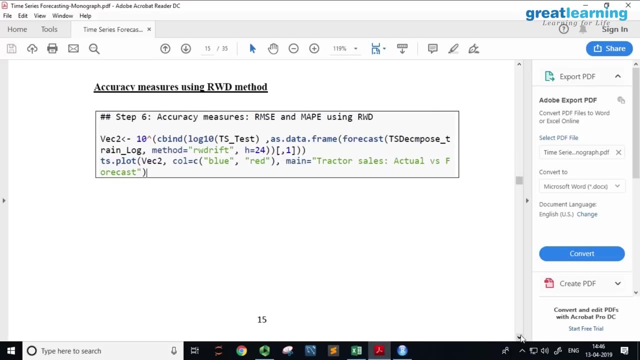 recovered most of it. I have recovered most of it, except that I have a slight under prediction, but, encouragingly, I have picked up a trend and I have picked up a seasonality, which is a good thing, which is a good thing. And now, in order to understand, 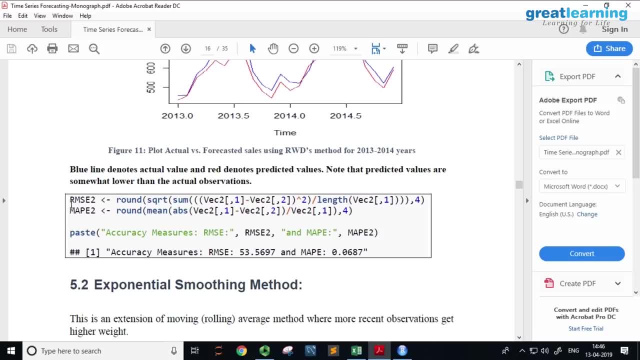 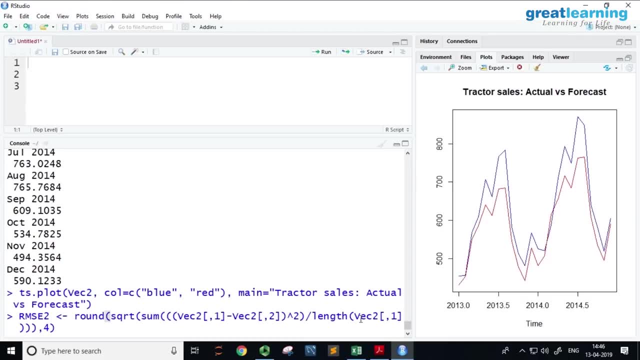 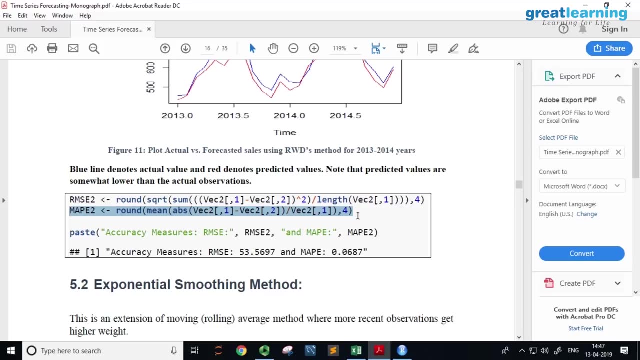 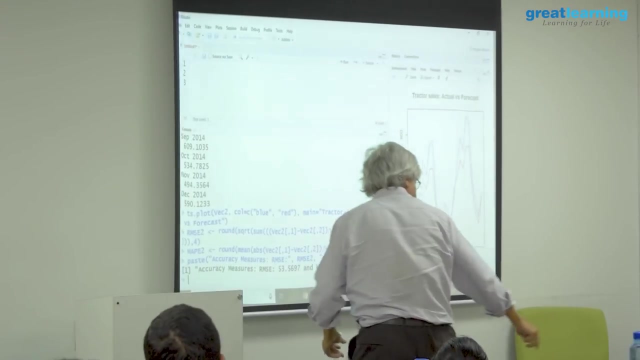 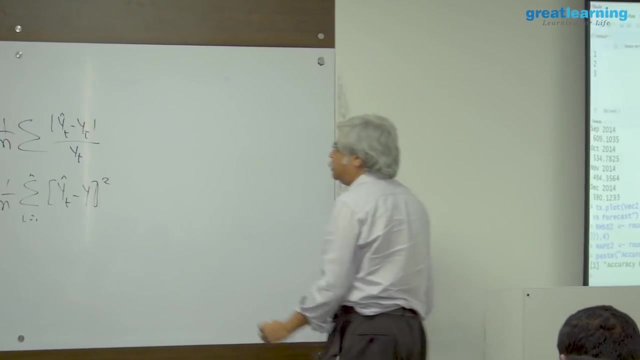 how good this forecast is. as I said, we can compute the the root mean square error and the mean absolute percentage error, And what it gets is a measure of. So what are these measures? Your, sometimes this is done with a n minus 1 here, if necessary. This is like a percentage error and this is like 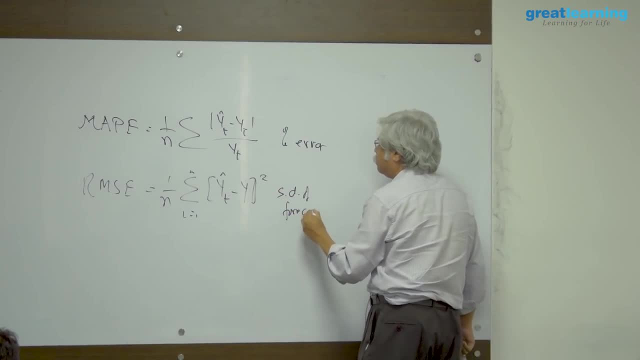 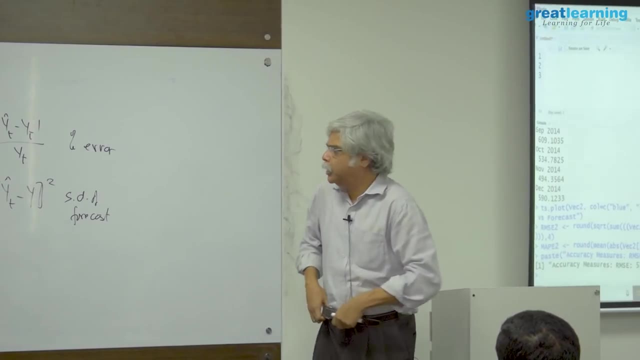 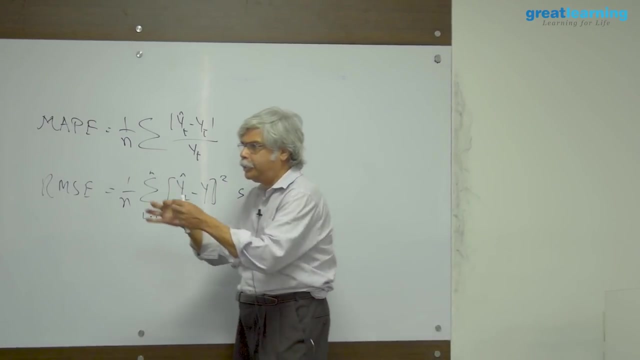 a standard deviation of forecast, if you want to interpret these things Ok. So this sometimes makes sense when comparing across different kinds of time series. This sometimes makes sense for a given time series on the scale of the original number. Sorry, root. 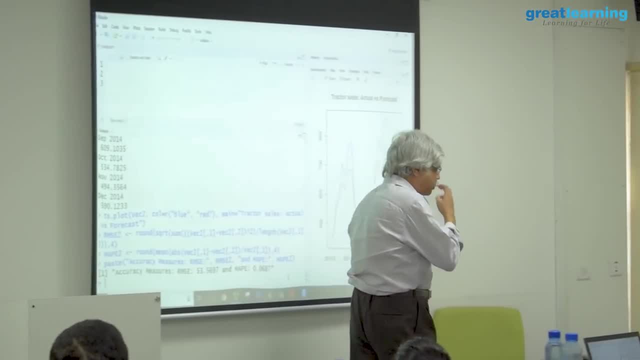 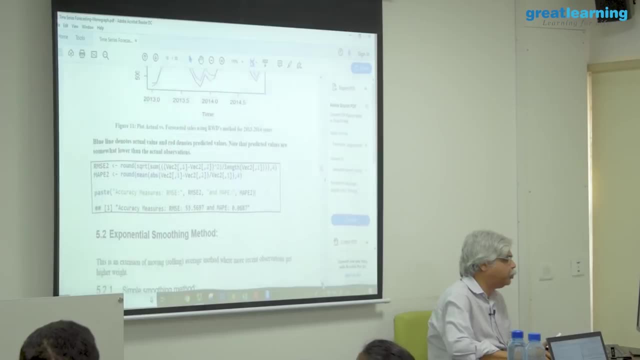 Ok, So what we want to do is we want to proceed in this direction and come up with, I think to some extent, what is the commonest way of doing this, and it is a method called exponential smoothing. 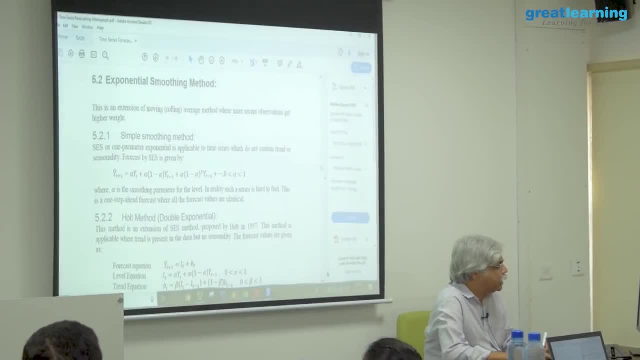 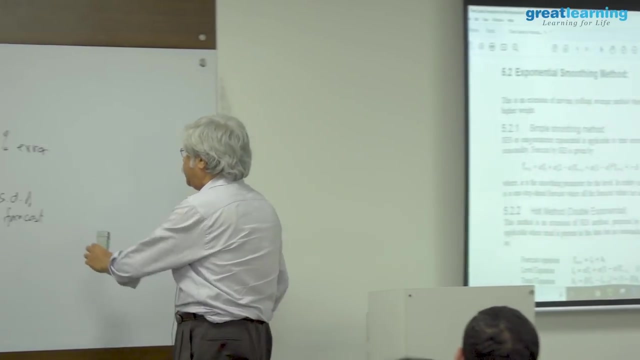 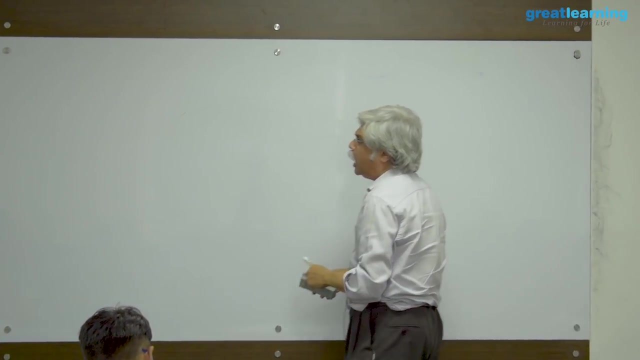 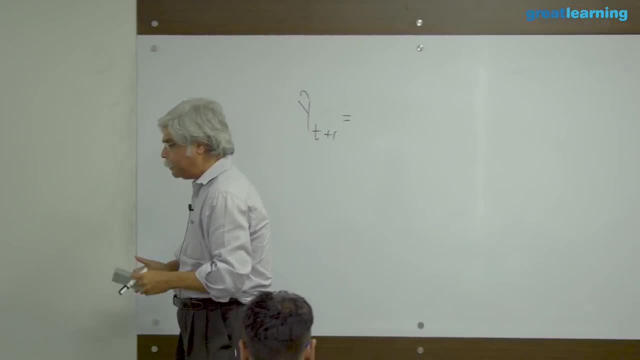 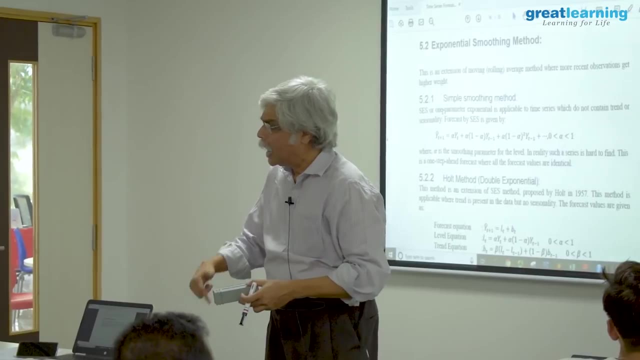 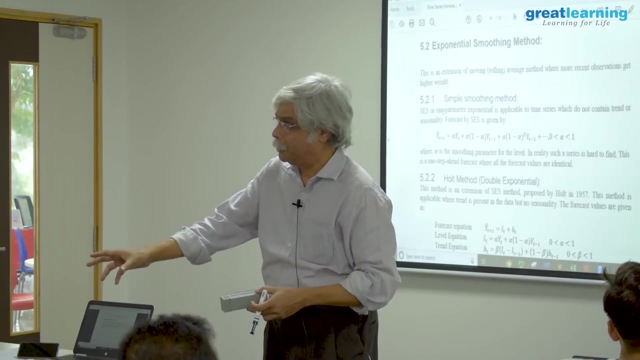 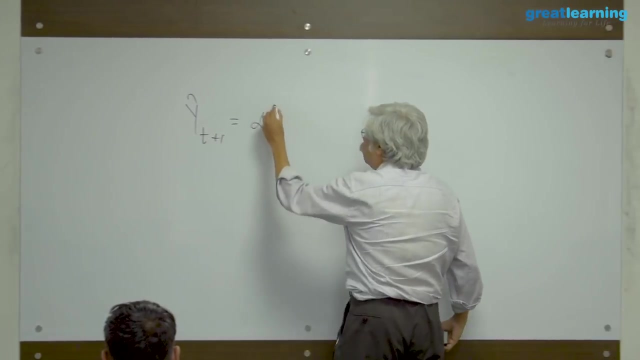 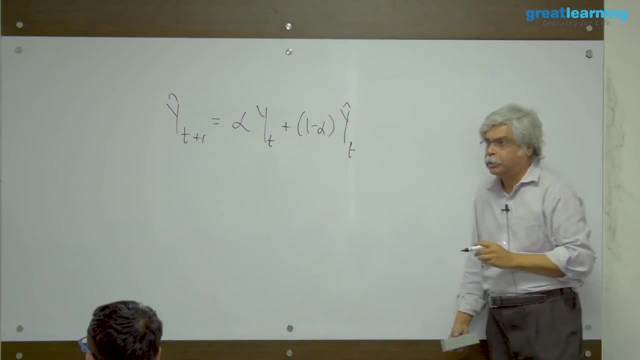 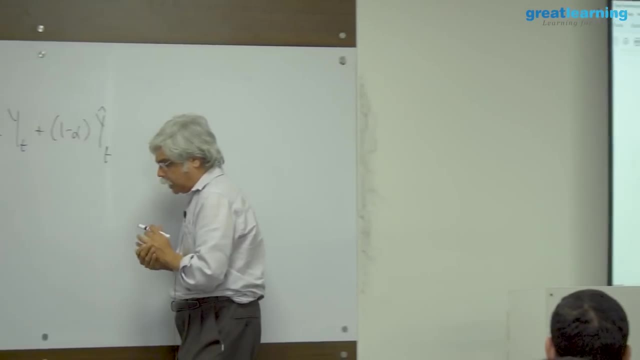 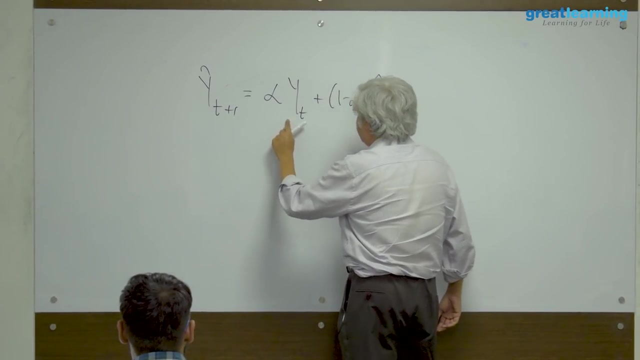 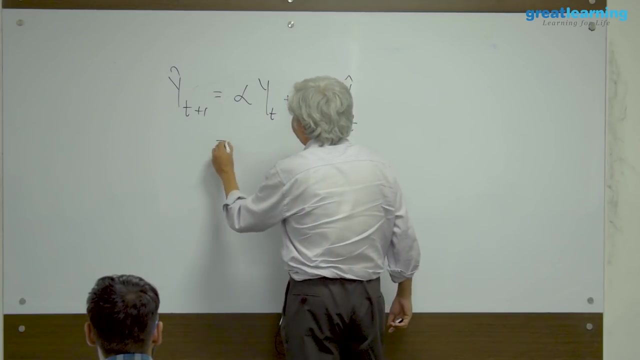 alpha of, let's say, yt hat. my forecast today is going to be that, so it's. it's, let's say, let's look at two particular extremes. so notation wise: forecast of today is a mixture of the actuality today and the forecast today. okay, or, or let, or i can write it this way: alpha of yt. 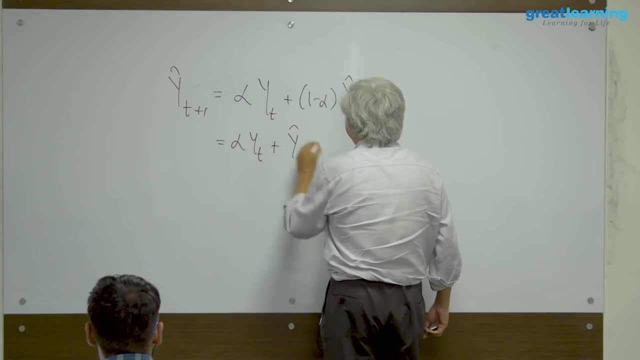 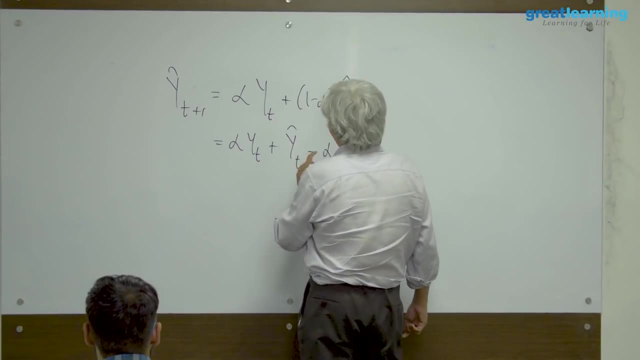 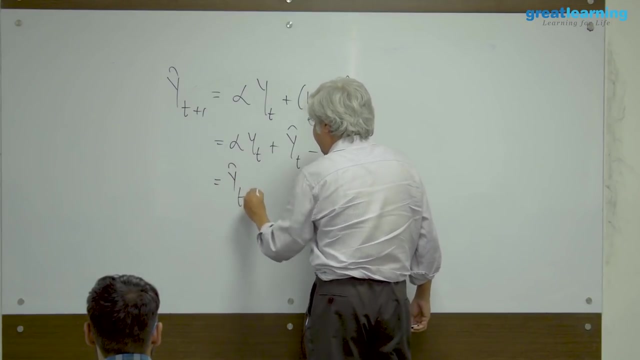 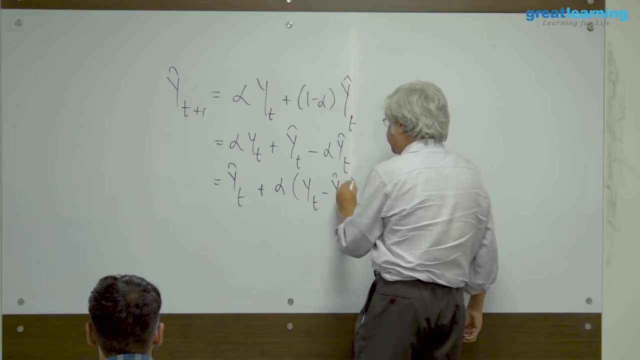 plus yt hat minus alpha of yt hat. sorry, um, is that right? that is correct, right? so now this is equal to yt hat plus alpha of yt minus yt hat. is that correct? i know i'm doing some high school algebra here, but i was never very good at it. 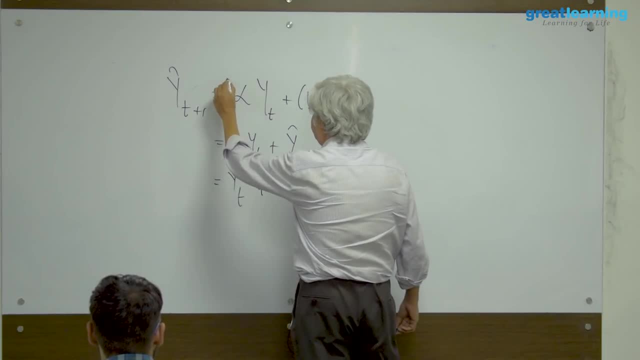 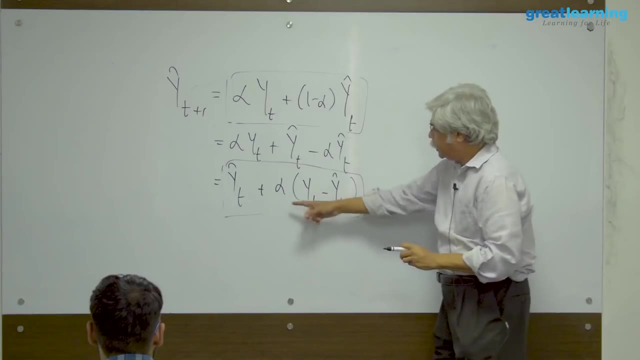 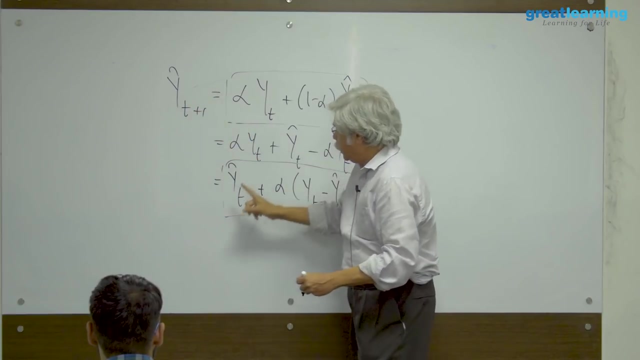 huh. so i want you to. so i want you to look at this expression. sometimes it's easy to see this way, and sometimes it's easy to see this way, i get confused. this version of it says the following: this version is what yt plus one forecast tomorrow is forecast today, modified by how wrong i was. 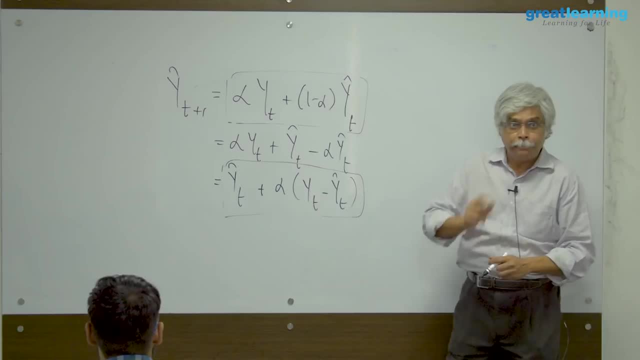 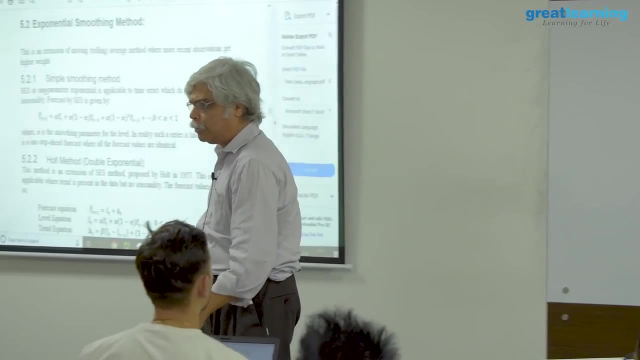 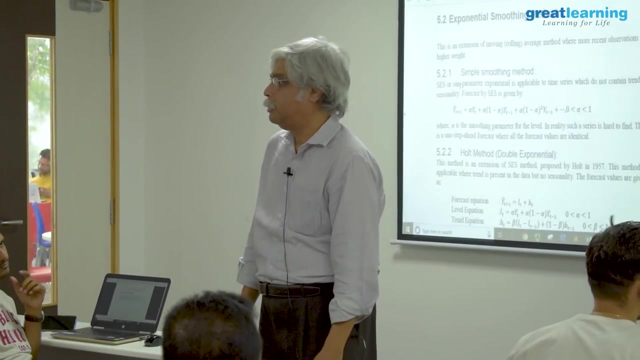 today, right? so in other words, let's suppose that tomorrow i, for i'm forecasting a hundred- i'm going to say: oh, you're forecasting a hundred. what did you forecast today? today i forecast 90. did, was it 90? no, it was 80.. so you over forecast. so assume that tomorrow also you're going to over. 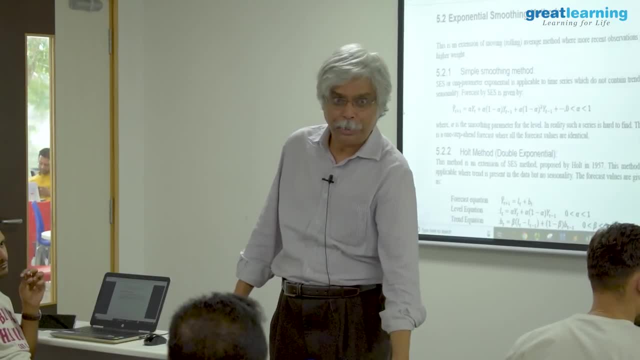 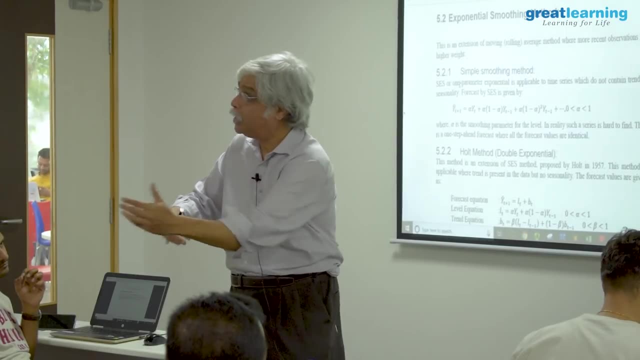 forecast correct tomorrow's forecast upwards. why? because today you were under forecast. by how much? by? not by the full amount, not by the full ten percent, but by some fraction of it, and that is what this alpha is. alpha is a fraction between 0 and x, and that is what this alpha is. alpha is a fraction between zero and y. when you add two youruing focus ratio to assistants passing out right now. that's correct. 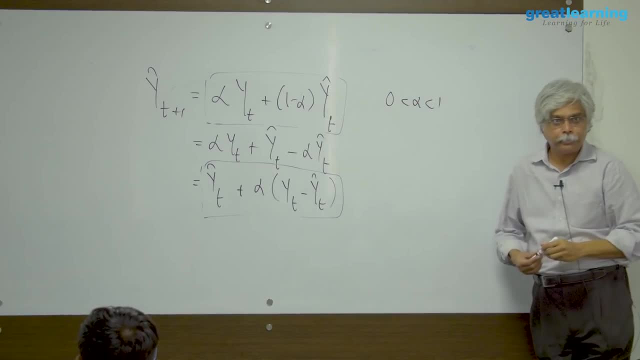 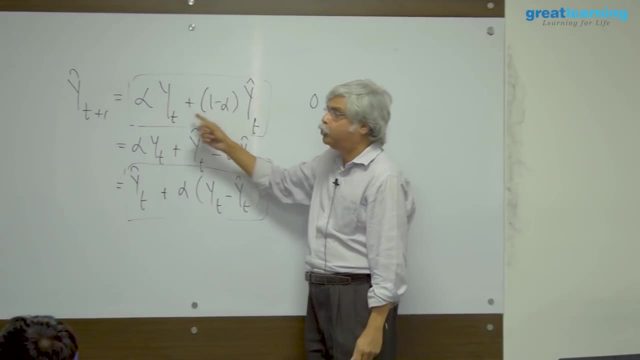 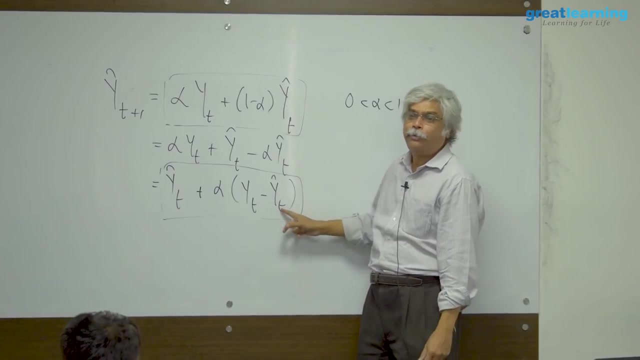 is a fraction between 0 and 1. alpha is a fraction between 0 and 1, so one way to see it is it's a mixture between today's actual and today's forecast, or it is today's forecast adjusted by how far off today's forecast was some people. 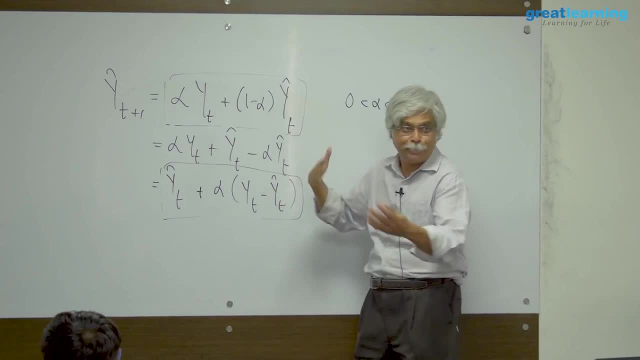 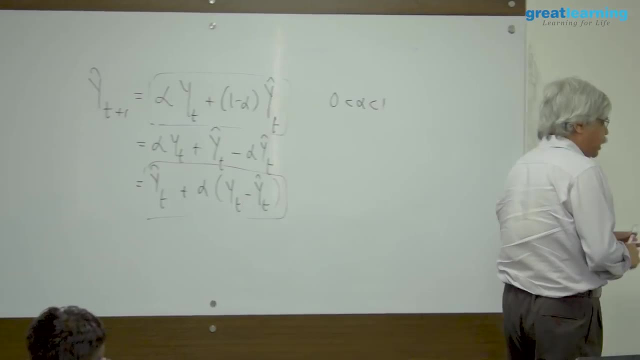 understand it better this way. some people understand it better this way. I apparently explained it by some combination of the two. but think of it this way or think of it, think of it this way. there's another way to think about it. that's often, that's often useful, and that is this and that's that's. 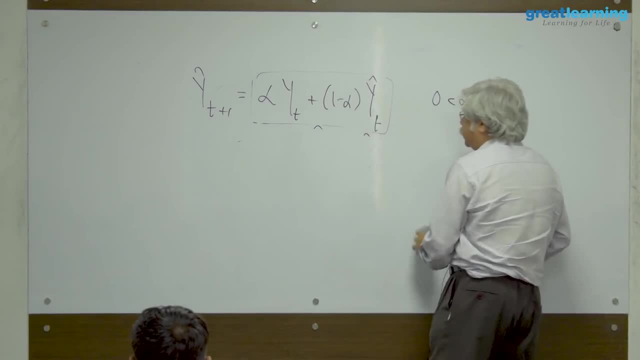 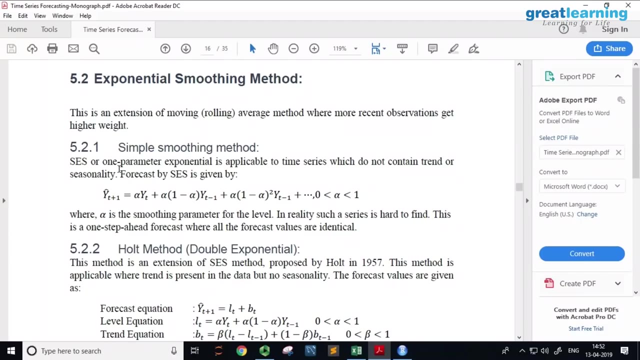 that's the way they've tried to write it out here. so a little more algebra. so now let's suppose that this is okay, let's. before I get there, let me take a look at a few extreme situations. let's look at the case. let's say alpha is very small. 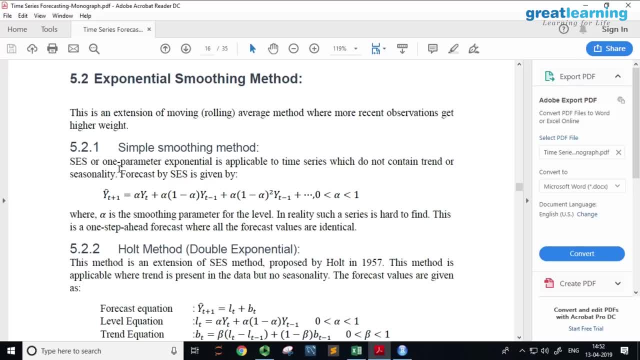 in fact, let's take the case alpha equal to 0. or let's take the case alpha equal to 1. if alpha is equal to 1, what happens you? if alpha is equal to 1, this corresponds to YT plus 1. hat is equal to YT. that 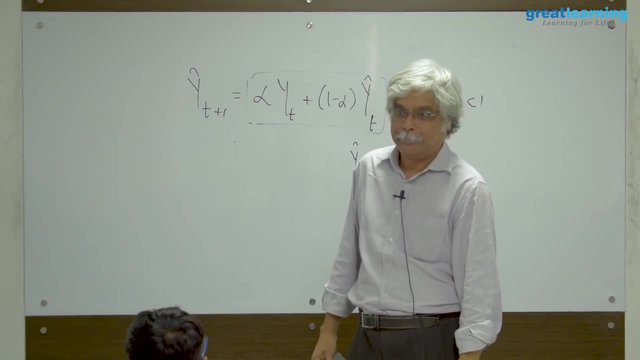 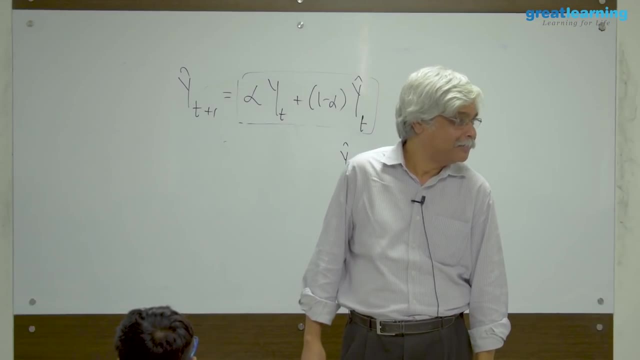 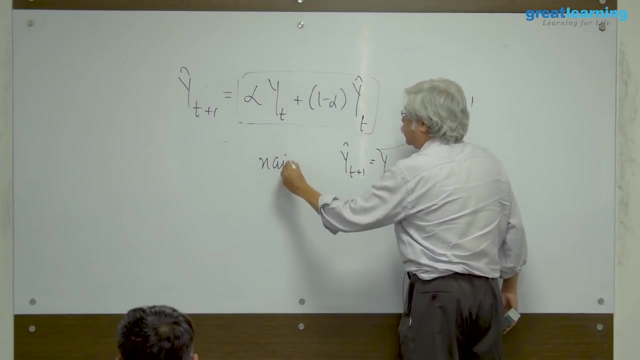 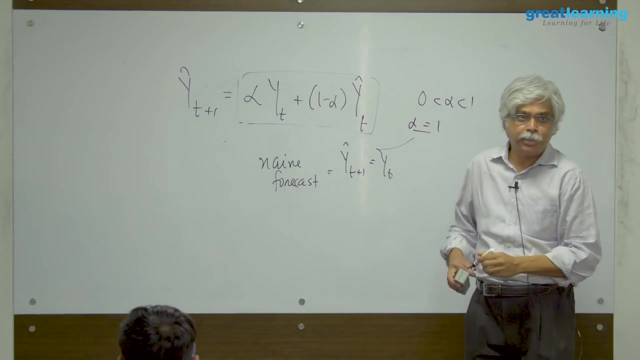 means what? tomorrow's forecast is what happened today. highly scientific and extremely simple. how much money will you make next year, how much money you made this year? this is called the naive forecast. have you done naive Bayes or any such thing? this is called the naive forecast. what naive means simple, so the simplest. 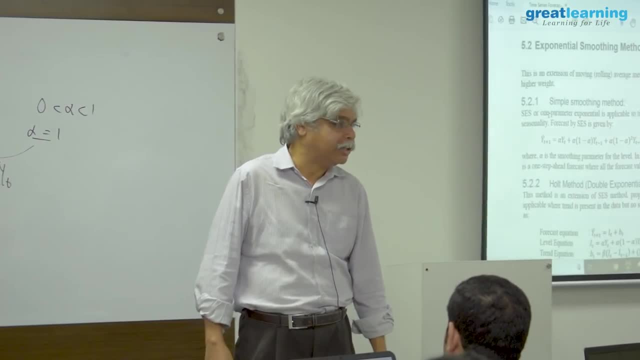 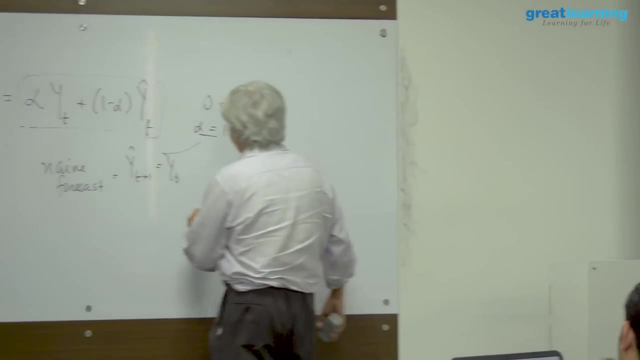 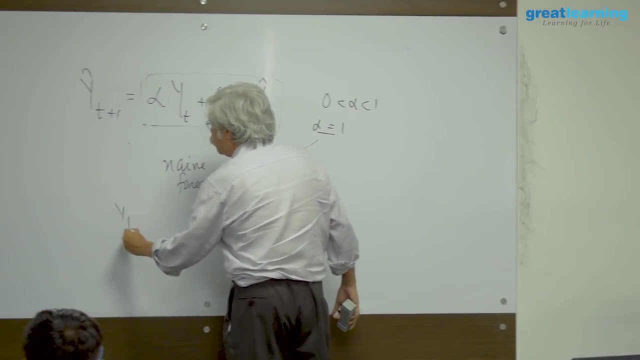 possible forecast is no forecast at all. essentially, which is today what it is today, not same. hold on to that thought. now look at the other situation, when alpha is equal to 0. if alpha is equal to zero, what happens if alpha is equal to 0? YT plus one hat is equal to YT hat that. 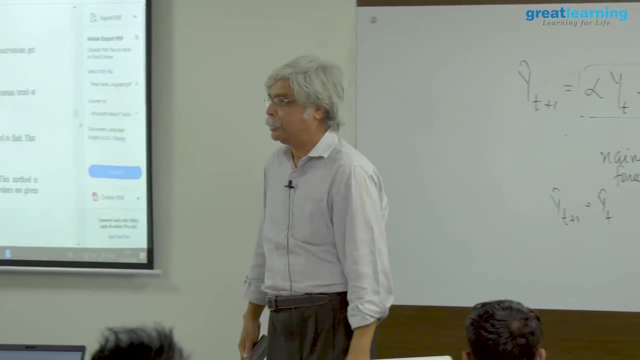 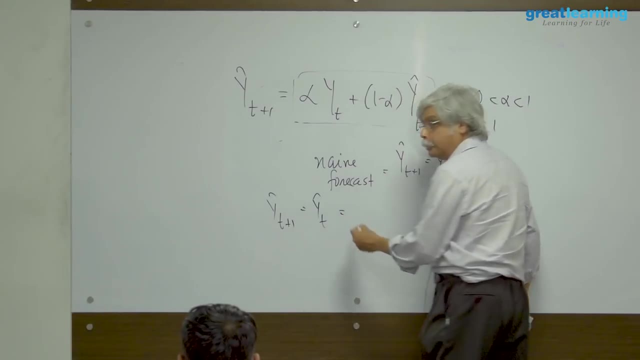 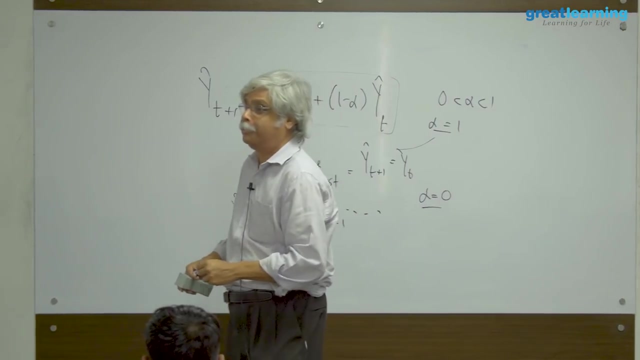 means: 2: tomorrow's forecast is today's forecast, but remember, this argument was for every time. point: what is today's forecast yesterday's forecast? that means what that means: the forecast doesn't change. irrespective of the data, your forecast is going to remain the same on one. 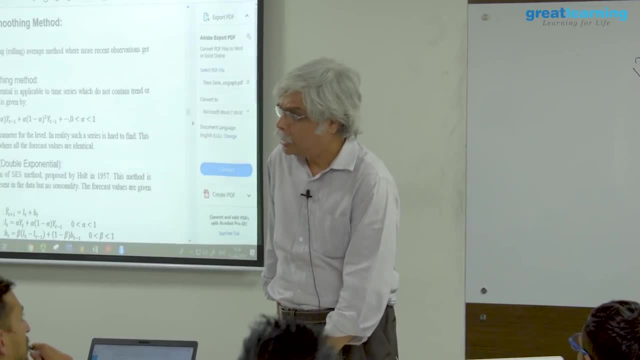 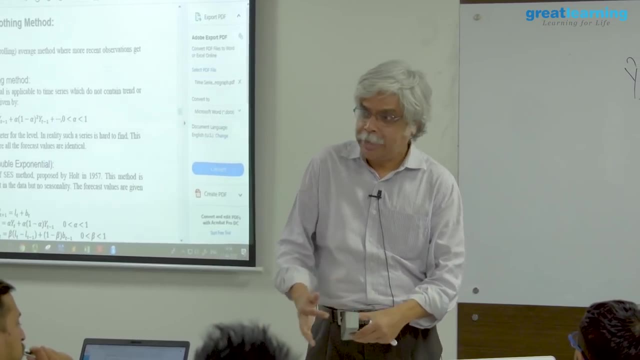 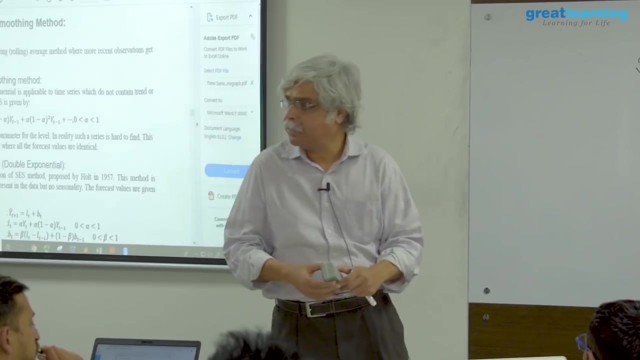 extreme, your forecast is what happened today. on the other extreme, your forecast is: what is the average of whatever has been happening so far? it doesn't change. so on one extreme, it's changing with today's data and the other extreme is not changing at all with today's data. it is the overall average. it's a constant. 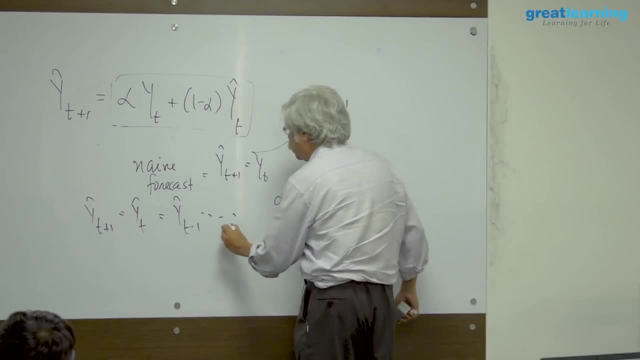 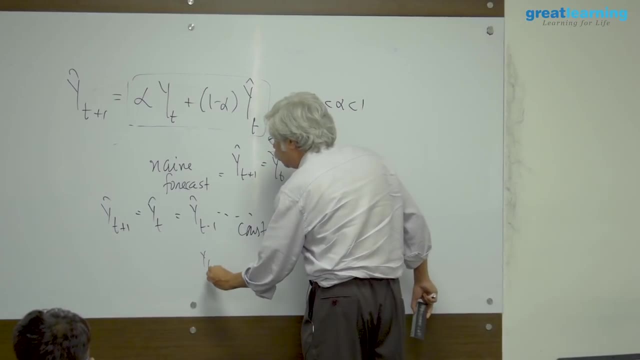 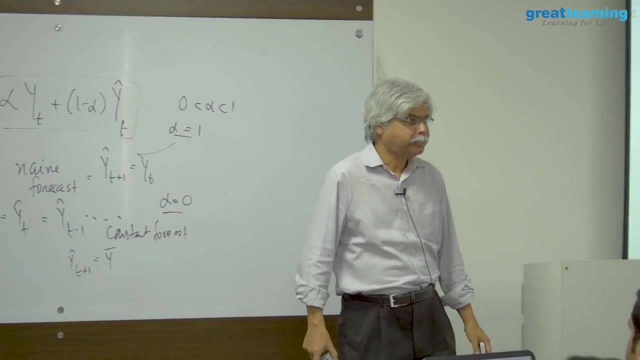 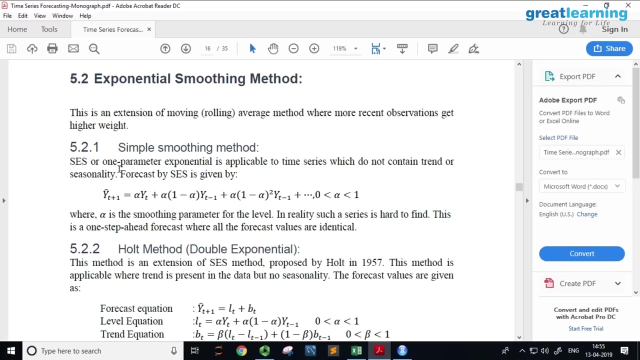 forecast. it is the same forecast as you were saying. it's a constant forecast. for example, one constant forecast is YT plus 1. hat is equal to Y bar. Y bar means average of all your observations. this forecast does not change but does. it may change a little bit, but the average is constant throughout. 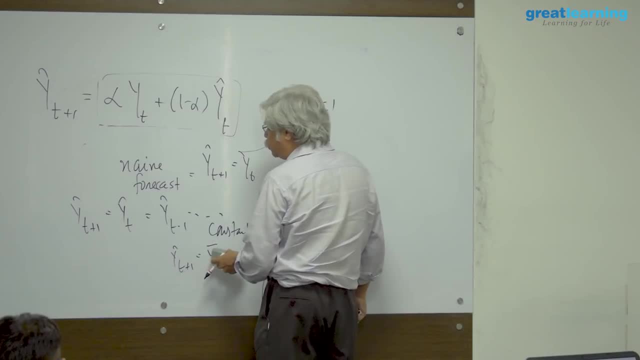 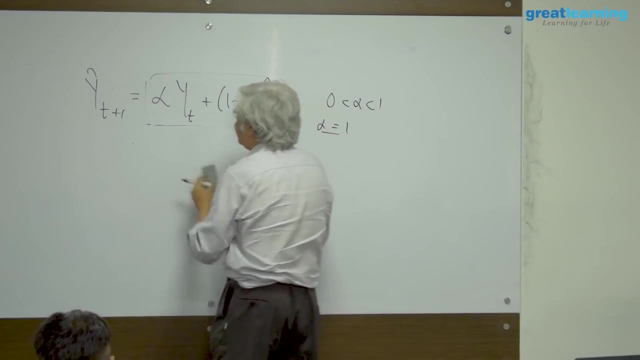 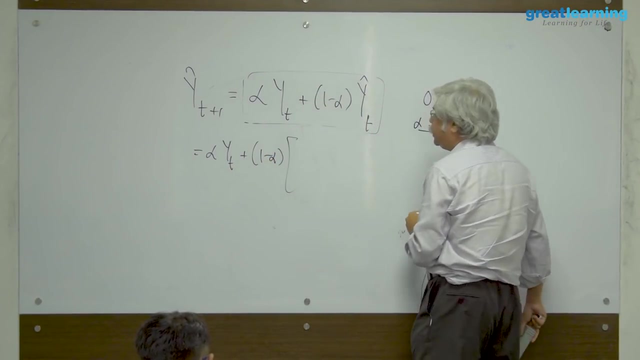 the data. so as alpha changes it moves between these two values. how does it move between these two values? so let's ride this out a little bit. so this I can write as alpha of YT plus 1, minus alpha off, but what is YT forecast? YT forecast is alpha of Tribi here, YT minus 1. 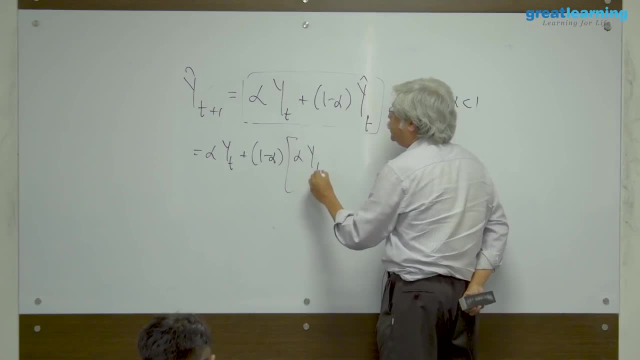 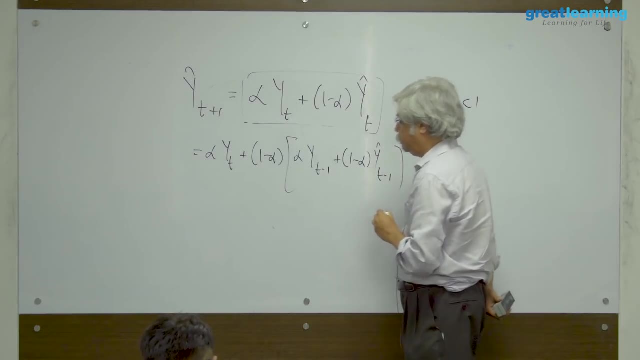 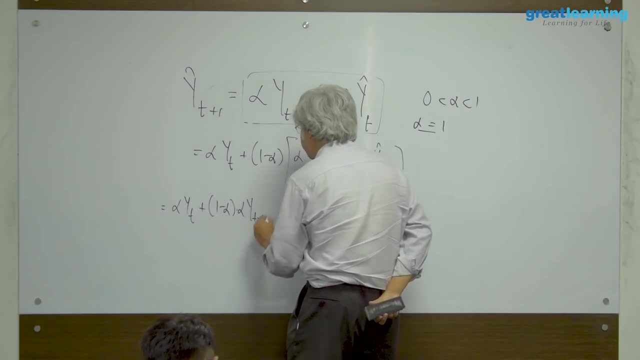 Y T Forkast is alpha of- help me hear- YT minus 1 plus 1, minus alpha of YT minus 1 hat correct. okay, one more step: alpha of YT plus 1 minus alpha of alpha YT minus 1 plus 1 minus alpha squared YT minus 1. 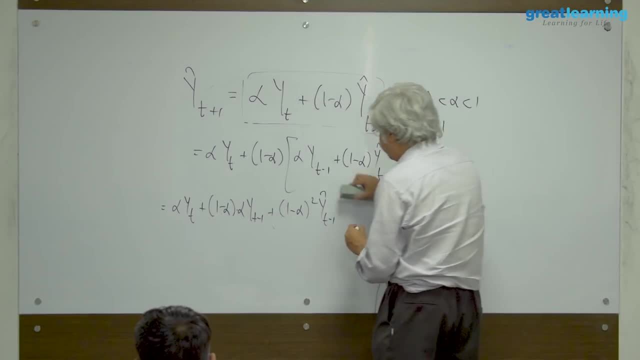 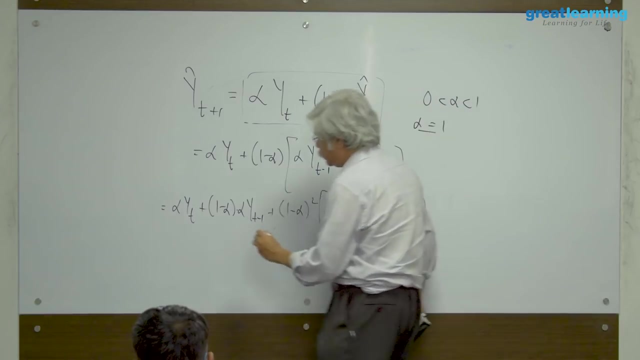 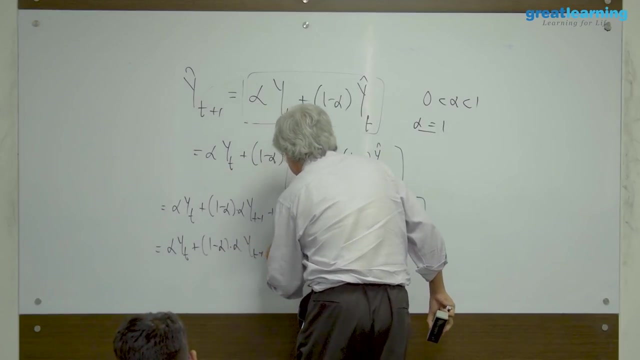 hat. okay, one more step. I'm going to replace this YT minus 1 hat by alpha of YT minus 2 plus 1 minus alpha of YT minus 2 hat, correct? I promised to end that here YT plus 1 minus alpha into alpha YT minus 1 plus 1 minus alpha. 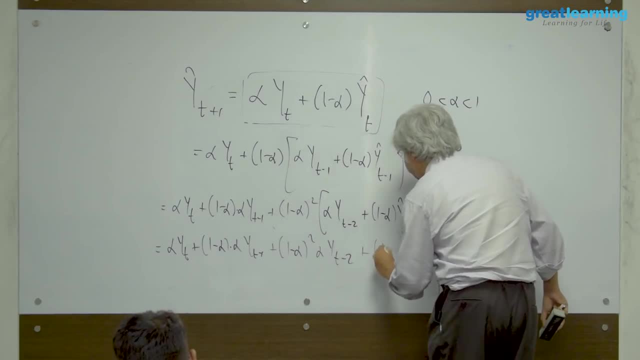 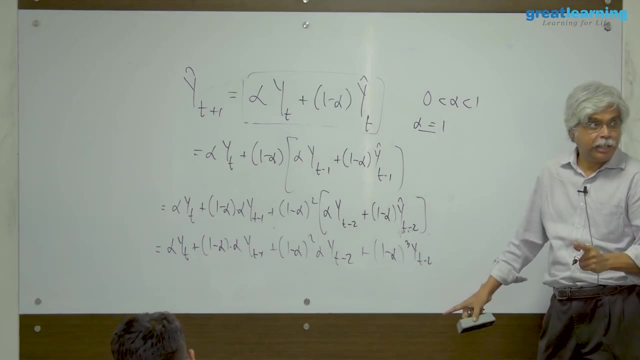 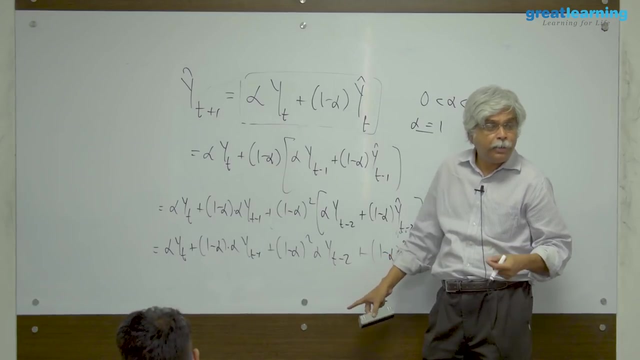 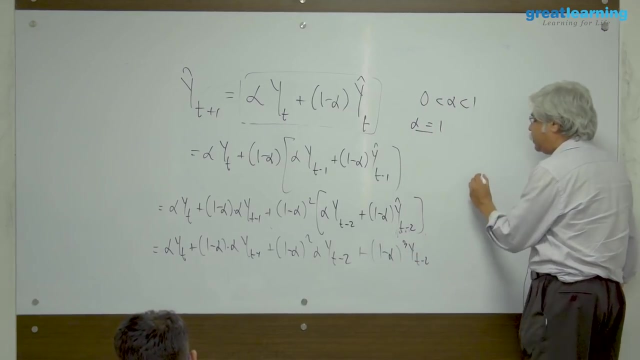 squared alpha YT minus 2 plus 1 minus alpha cubed YT minus 2 hat, you can see what is happening. you can see what is happening. the forecast is looking like a combination of my previous values. it's looking like a combination of previous values, but what kind of combination of previous values? exponential they're getting down. let's, for example, 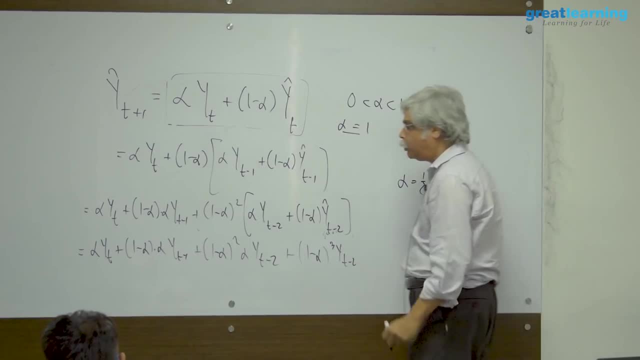 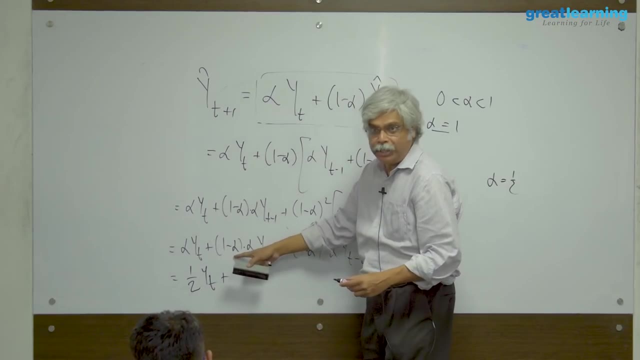 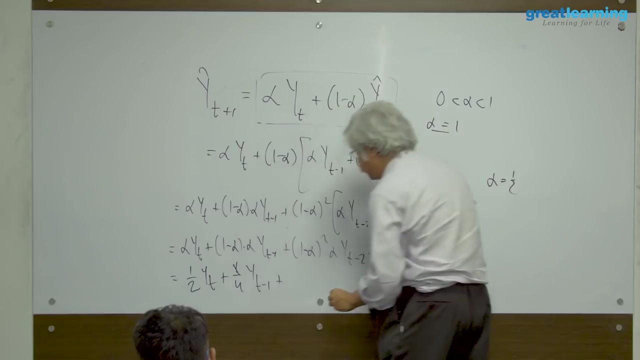 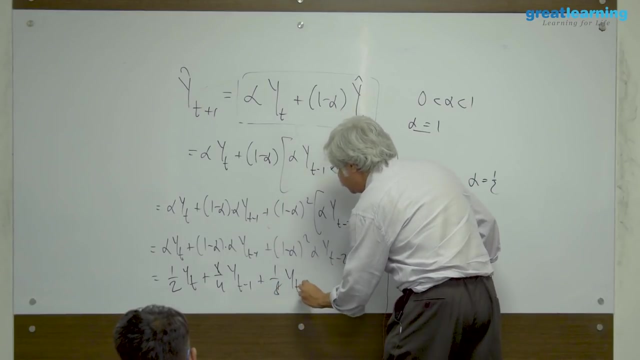 take the value alpha equal to half. if alpha is equal to half, what does this become? this becomes half yt plus 1 minus alpha is also, coincidentally, half. so half into half. 1 by 4 yt minus 1 plus half squared into 1 by 8 yt minus 2 squared into half, right, so what is my forecast tomorrow? 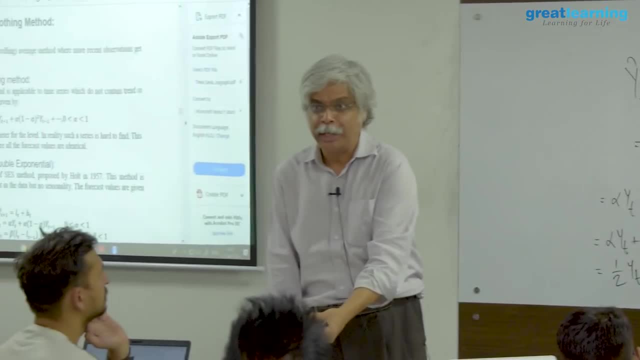 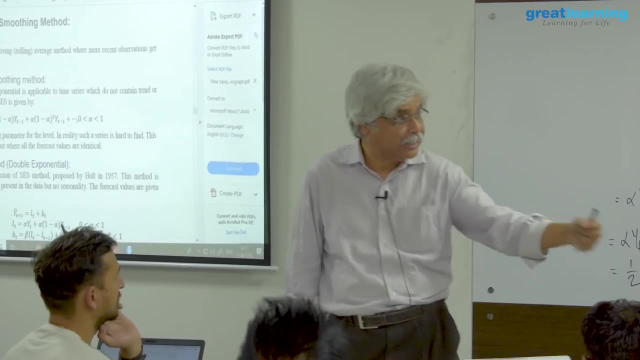 my forecast tomorrow is half of what it is today, plus a quarter of what it was yesterday, plus an eighth of what it was the day before yesterday, plus you can see what the next term will be: a sixteenth of what it was, and then 32. it keeps going. in other words, it is something between 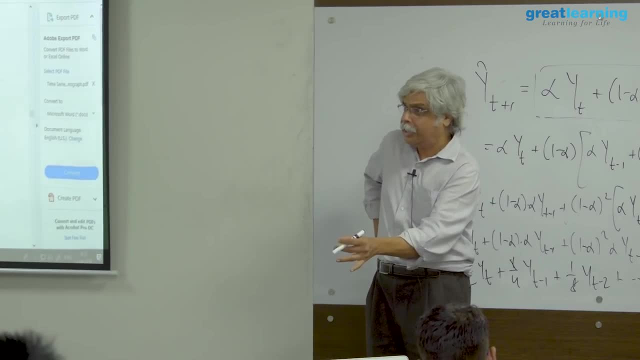 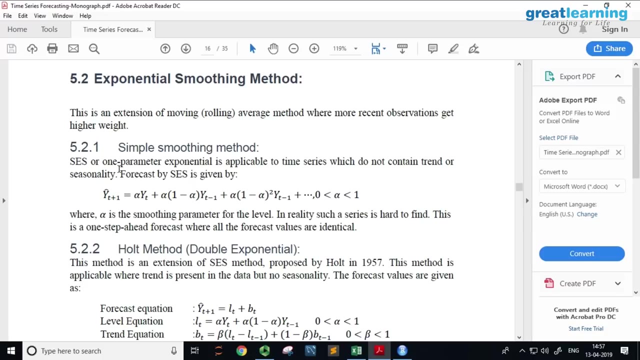 the most recent average of the previous values and the most recent average of the previous values, most recent observation and the average of all observations. it is an average of all observations, but with the weightage being much more towards the more recent ones. how much will you make next year? half of this year plus a quarter of the 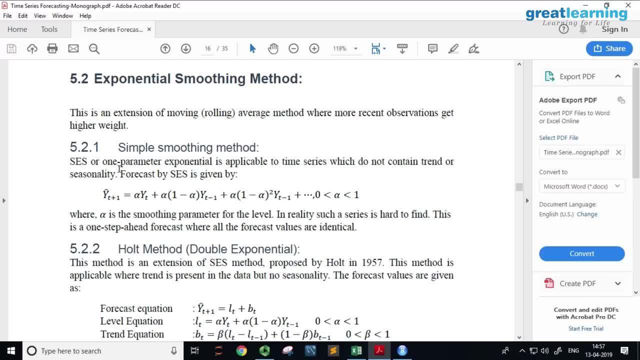 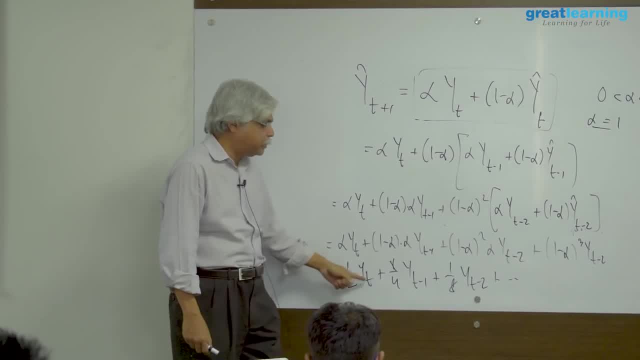 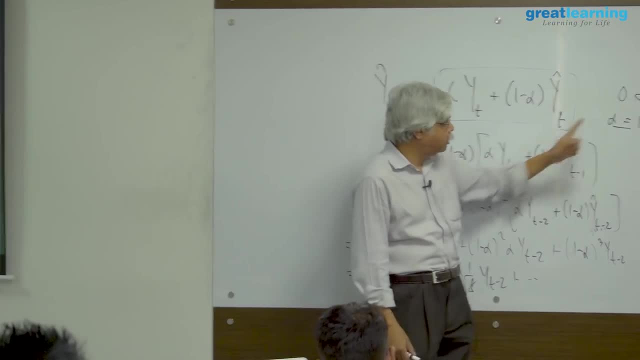 previous episode. so it's a, it's a way, it's an average of all that you've made next year, with more weights given to recent years. the, the extreme version of this. this becomes one which means there's no other year. the other extreme version: all these weights become equal, which is this: estimate of Y is equal to: 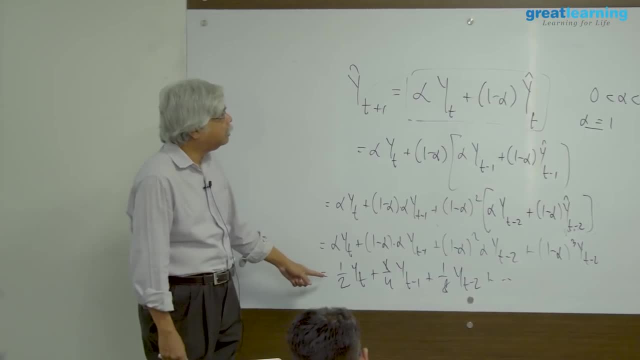 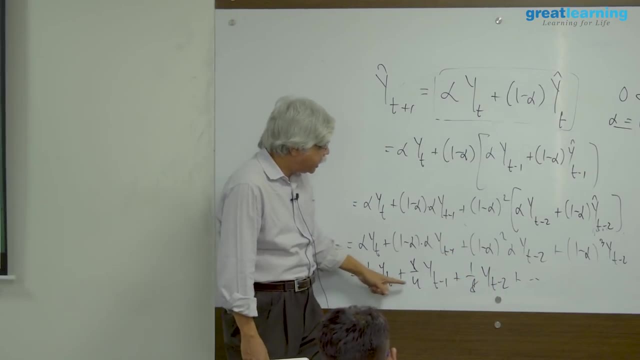 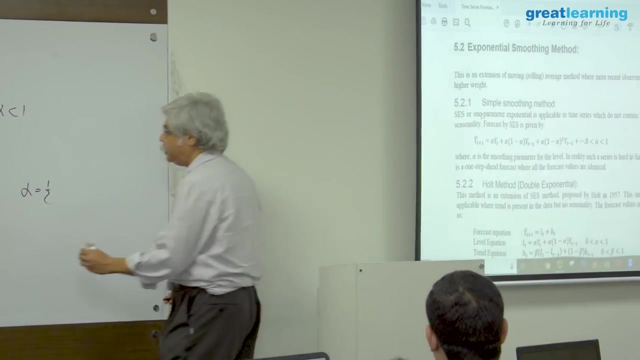 Y is equal to Y is equal to 1, alpha is equal to alpha is equal to 0, and you can work that limit out. so, therefore, what this is is a weighted average, a weighted average with exponential smooth. it's called an exponentially weighted moving average sometimes. sometimes this term is used exponentially weighted moving. 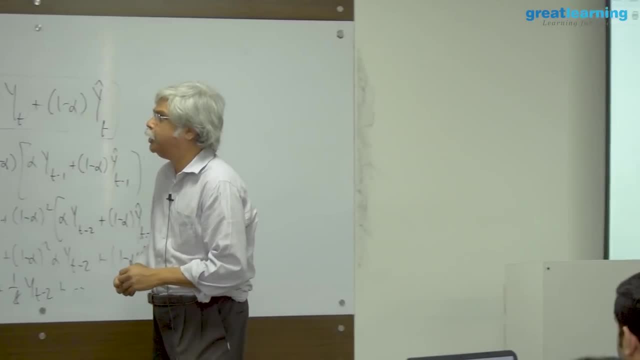 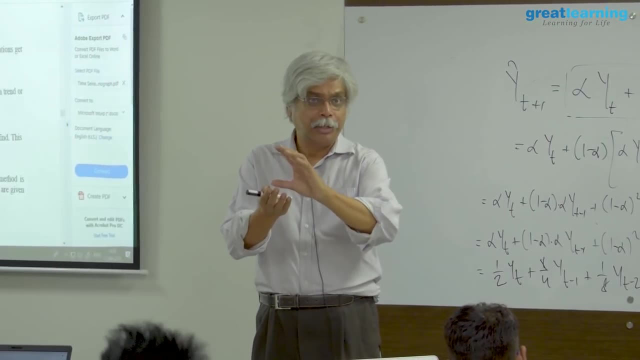 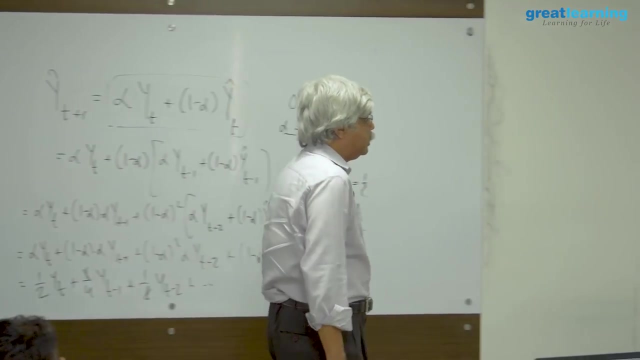 average, or sometimes very simply called exponential smoothing. it's a smoothing of the data. smoothing means averaging out. how is it being smooth? by averaging out the past observations. how? by exponentially decaying weights. this is also there, for example, in Excel. this is the simplest possible forecasting method. 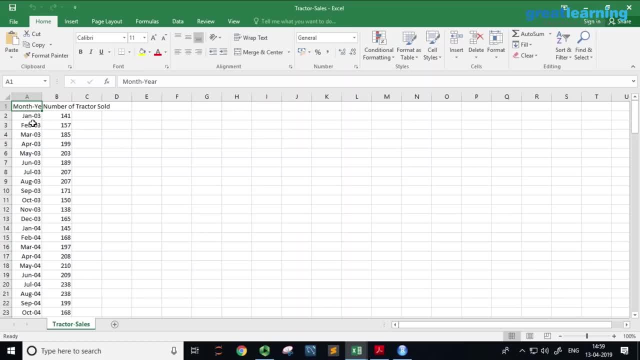 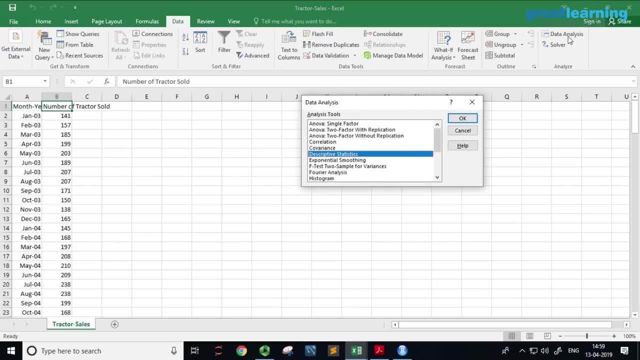 if you, if you go to Excel- so here, for example, you go to Excel data data analysis. there's something called exponential smoothing, so you can forecast in Excel if you want to, but this pretty much the only forecasting algorithm that's available in Excel. if you do that as an example. 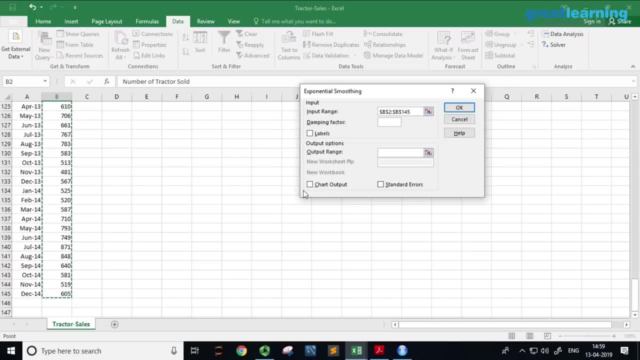 what you can do is you can take, for, say, the input range, something of that sort label is not there. the damping factor, so to speak, is this value of alpha, the value of alpha, that report here, and you can put in, say 0.5 or any of this, any of. 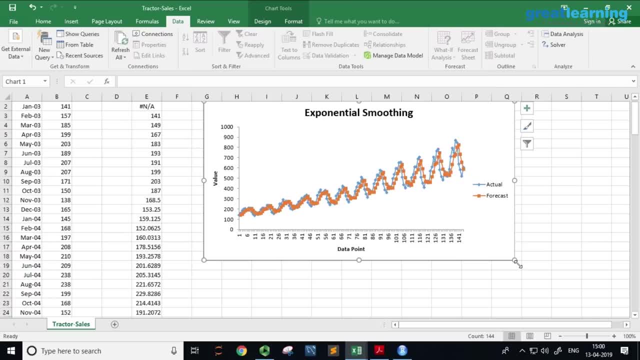 these values here, or you can say 0.5, maybe you can put in something like 0.0 and you, and then this is an excel version of it. you can model, you know, muddle around with it. what it has done is because I didn't set it up very well. it's actually. 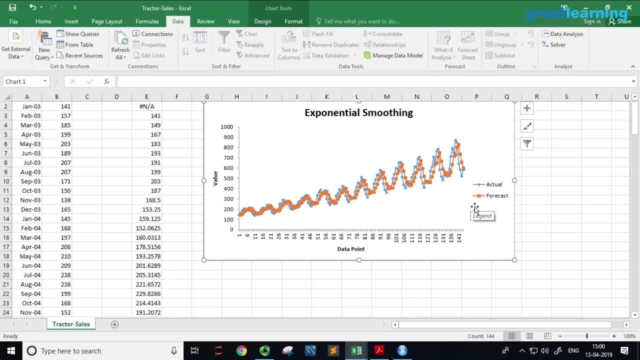 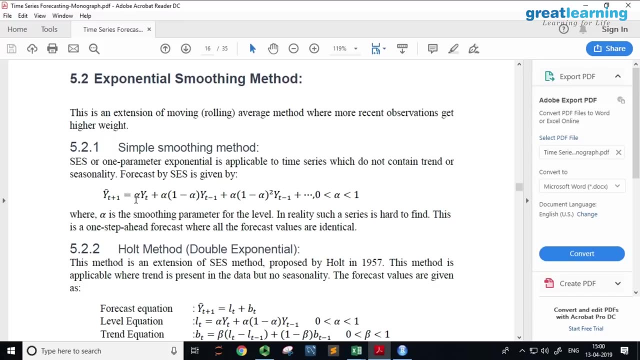 forecasting one period at a time going forward. this is just to show you that this kind of smoothing is available in other packages and it's in some way. it is the simplest form of smoothing that you can do now, but, as is, over a period of time, over longer periods of. 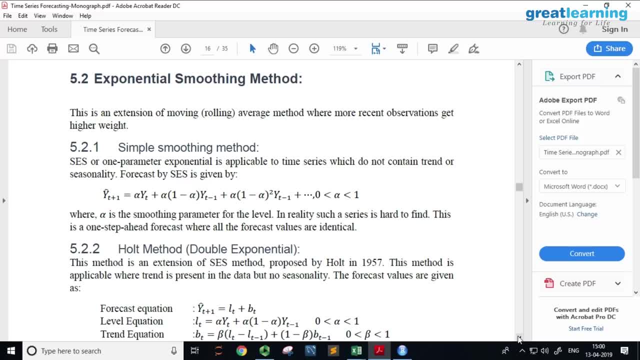 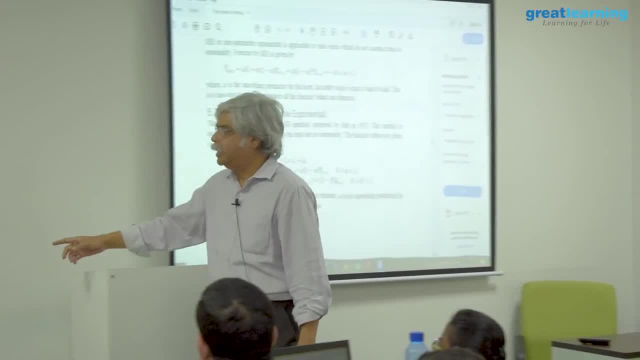 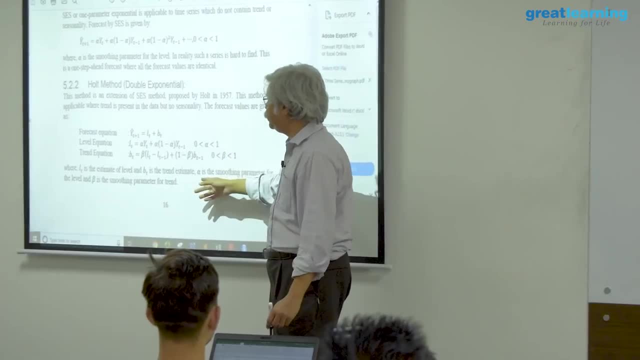 time. there is a problem with this forecast, and the problem with this forecast is that it takes- it doesn't take- any kind of seasonality into account. it doesn't take into account any kind of seasonality. so what people have done over the years is that they've modified this simple exponential. 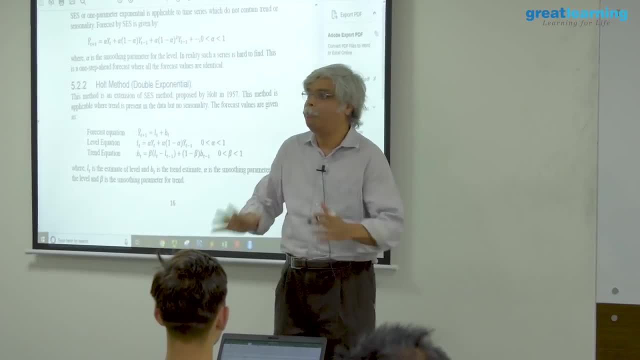 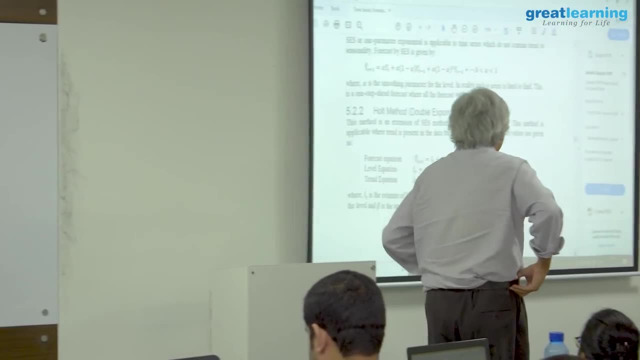 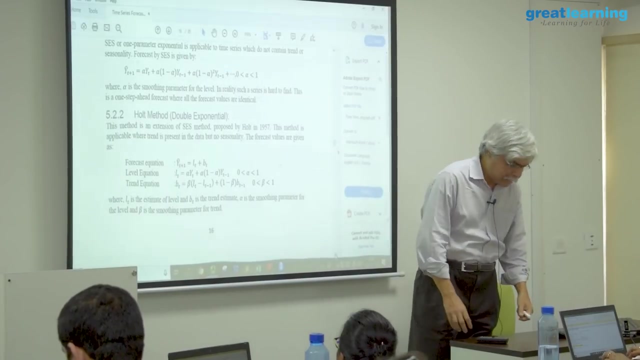 smoothing into various kinds of more complex things, say something called double exponential smoothing and then triple exponential smoothing, or what is called a hold winters. these are modifications of the same thing, and you can review the formulas at your leisure, but let me give you a rough sense of what these formulas are trying. 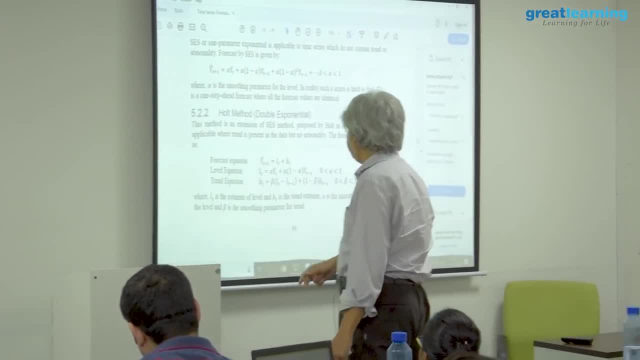 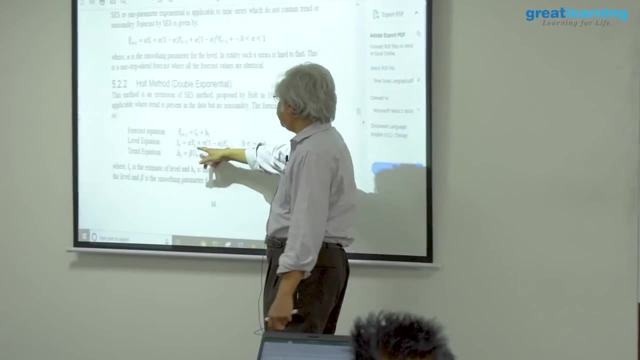 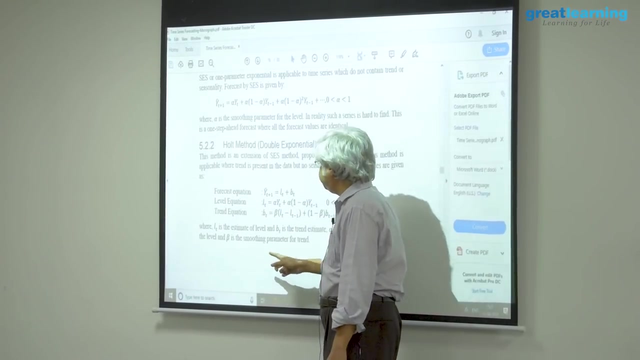 to do so, for example, here, let's say, double exponential smoothing. so here's the alpha. the alpha is the same kind of thing that you saw before, but what's more important is this: the forecast equation. the forecast equation is written as two terms. it's written as a level term and 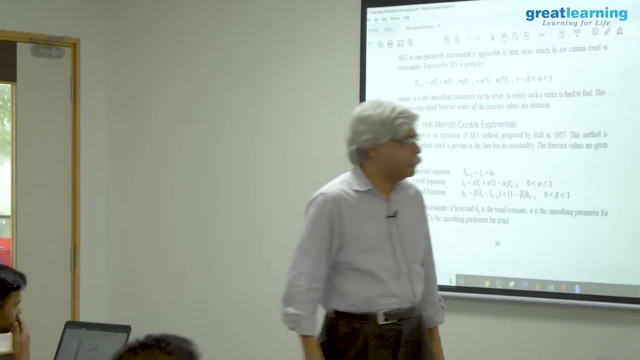 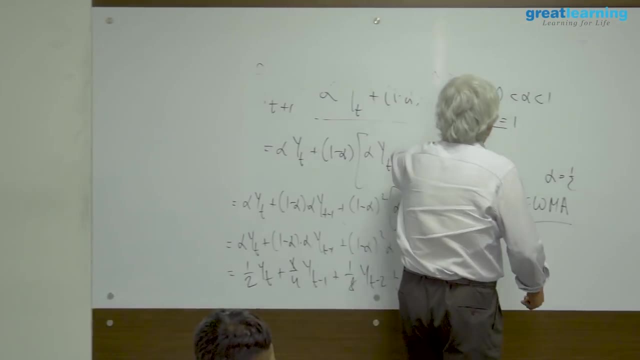 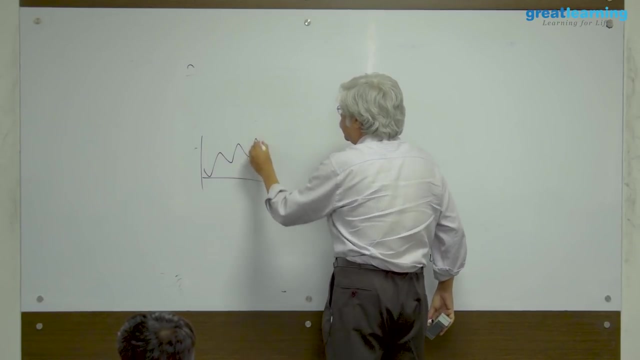 a is written as a trend term. what is the idea here? the idea here is to write my series. the idea here is to be able to write my series, not as a continuous series. so what a series that looks like this and I want to forecast it. I am at. 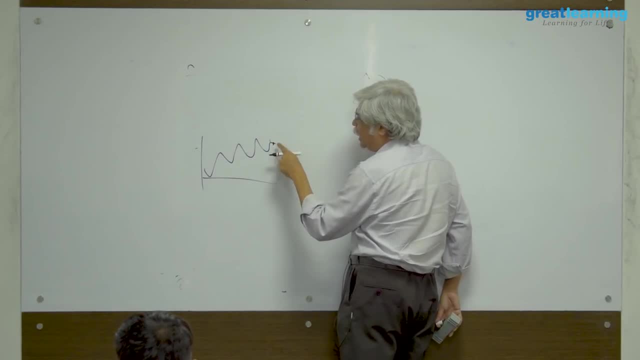 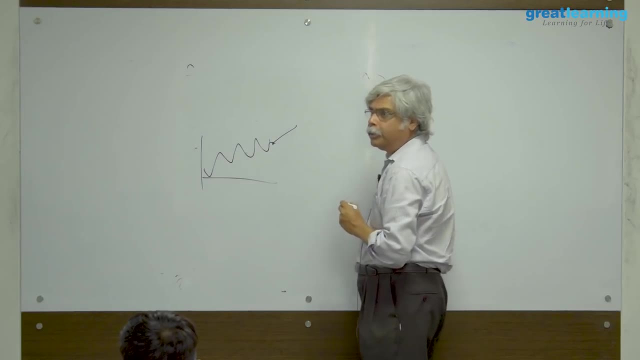 if I am at this point and I want to forecast, what I want to say is: I want to identify a level. the level is where I am starting the forecast. the trend is the line, the angle of the line with which I'm going to proceed. so my forecast is going. 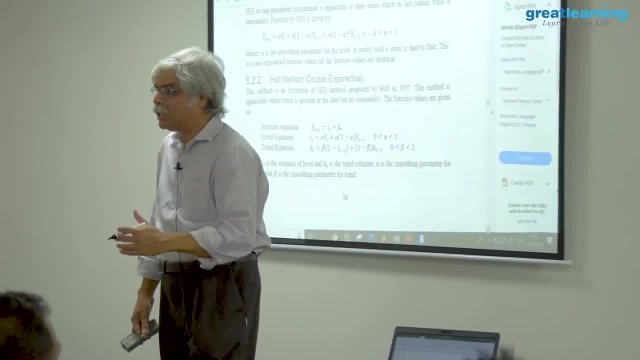 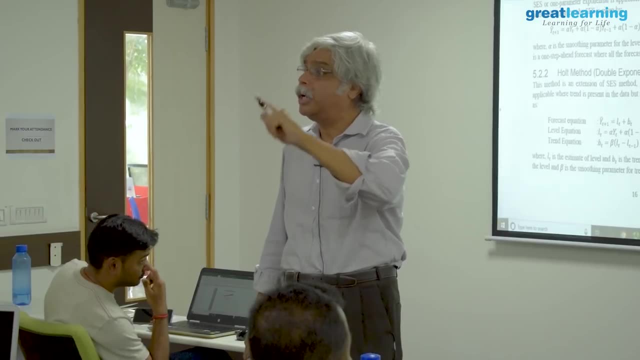 to be essentially something like an a plus B X. I want to know what that level is and I want to know what that trend is. in other words, I want to know what my LT is, where I'm beginning, and what my BT is, which is my per year correction. so I'm 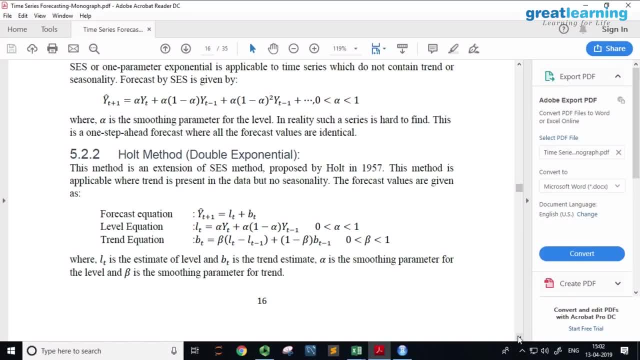 going to begin at one point and then I'm going to add a certain term every year. if I'm going to add a positive term, I'm going to go up. if I'm adding a negative term, I'm going to go down. now the question is: what should this level be? 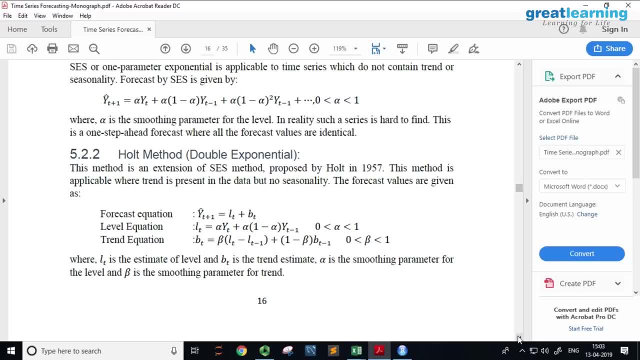 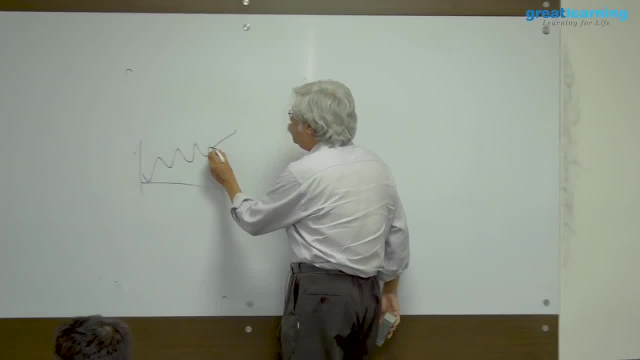 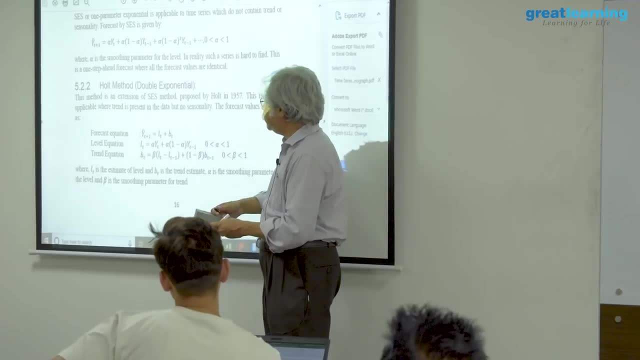 and what should this trend be now for the level? part of it it's saying: use a single exponential smoothing. like term you know was predict the level, predict where you start from, like you would use a simple exponential smoothing. the trend equation is slightly more complicated but you can see what the trend is it. 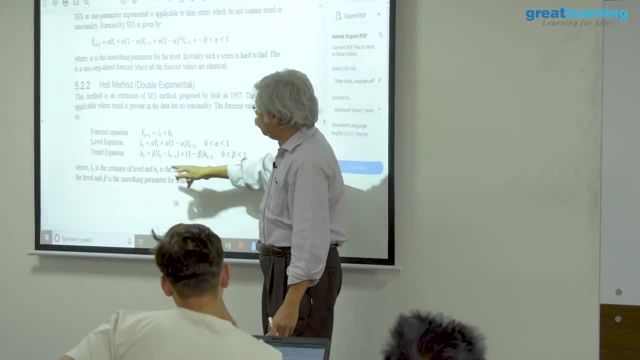 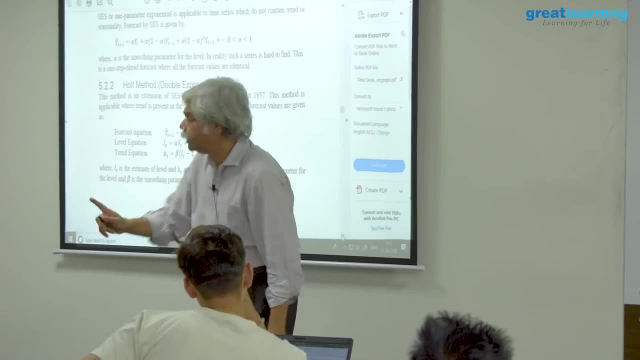 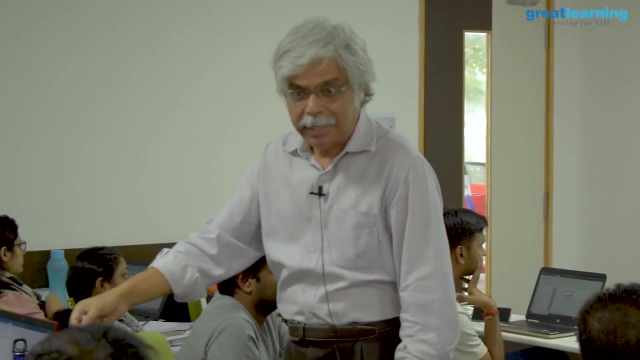 uses the same idea, but it uses it for a trend. it says: what is the trend? the trend is a combination of the change in the level and the previous trend. what is my current trend? my current trend is the change in the level, you, which is the trend I'm seeing right now and my previous estimate of trend. and so 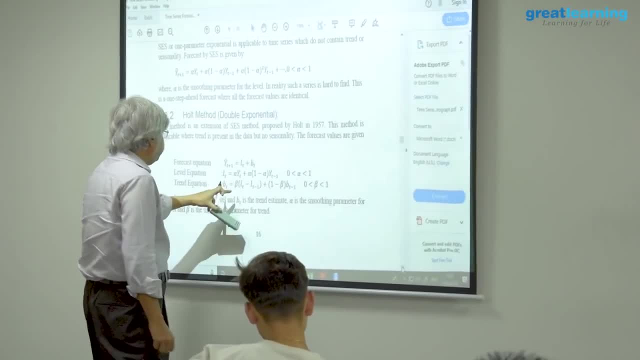 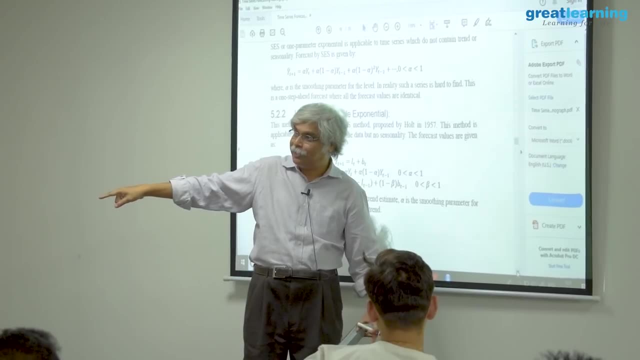 again. similarly, if my beta is very, if my beta is very close to one, then my estimate of trend is going to be simply the change in my level and has no memory of the previous trend. if my beta, for example is, is closer to zero, then my trend is going to be a constant. there's going to be a constant beta. that will. 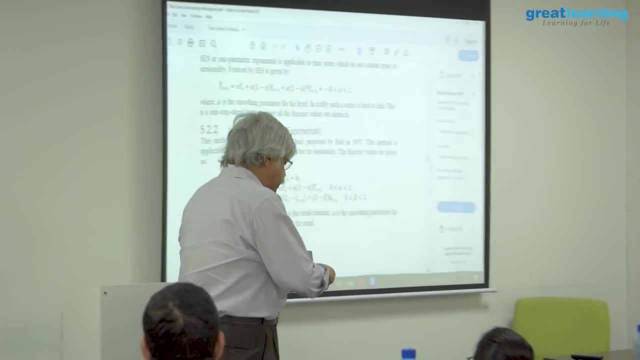 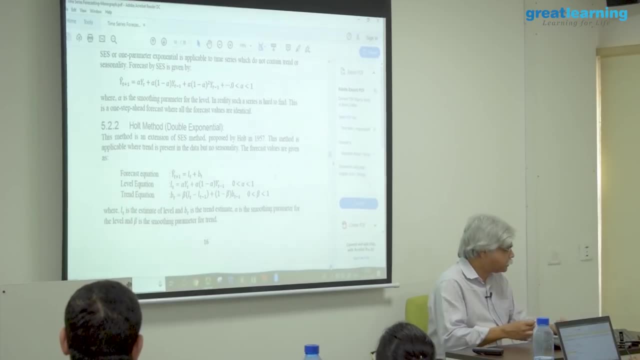 keep adding. it will not be modified by the data. so this is, this is the same kind of idea, except that what it has done is it has now incorporated the forecast and the, the level and the trend. seasonality complicates things even more, and the so-called triple exponential method, which is the one 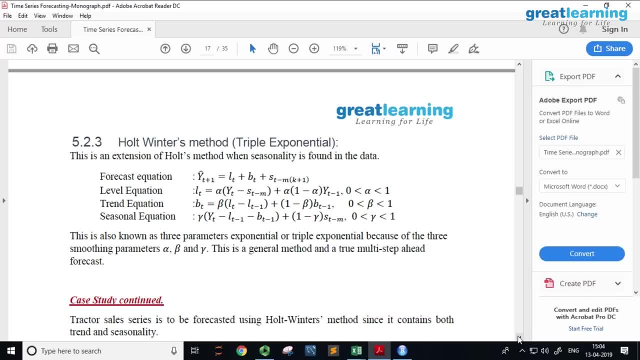 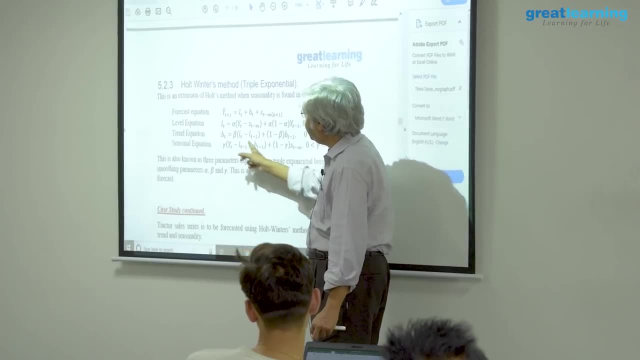 that's typically used, and here the problem becomes a little more complicated because the seasonal terms are terms that are included by saying what is the seasonal term? the seasonal term is a combination of whatever is left behind after the level and the trend has been taken care of and the previous seasonal 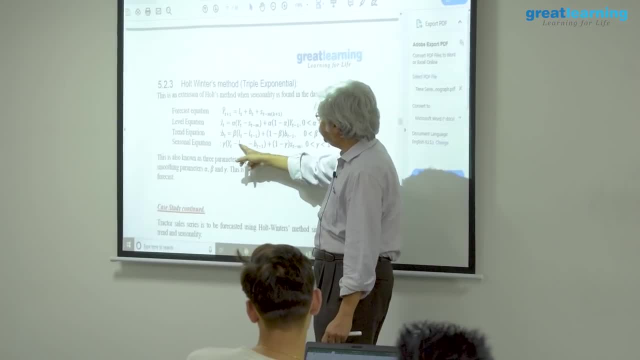 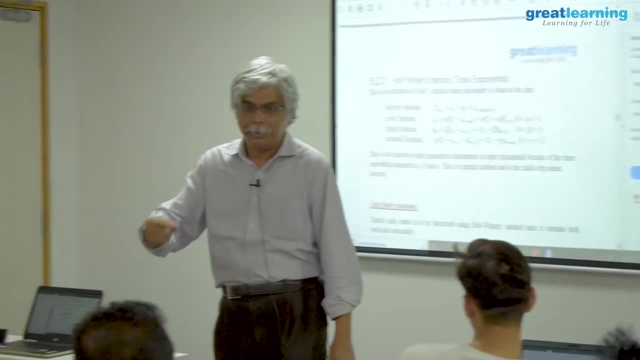 term. so every time I'm sort of using the same set of tricks in order to add a different component to this. now, the saving grace for you is that you don't need to know any of this. in other words, you can run the algorithm you may need. 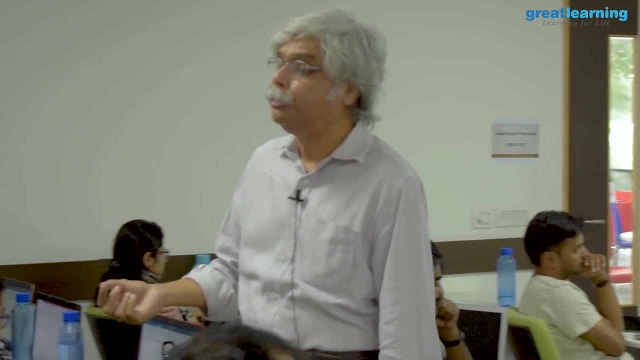 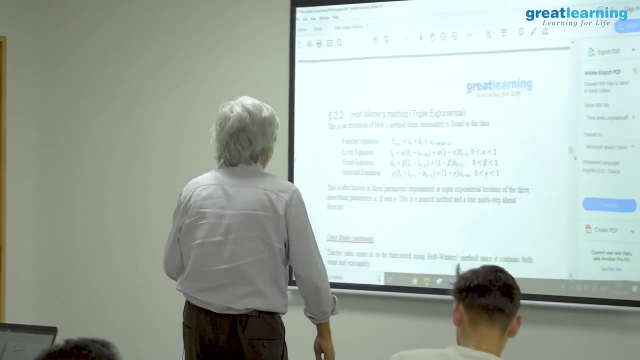 to specify what the alpha betas and gammas are, or you can let the algorithm choose for itself what the alpha betas and gammas are. so the usual way of doing this, executing on this, is to say fit the most common exponential smoothing kind of parameter, in other words, one with trend and one with season, it in one with 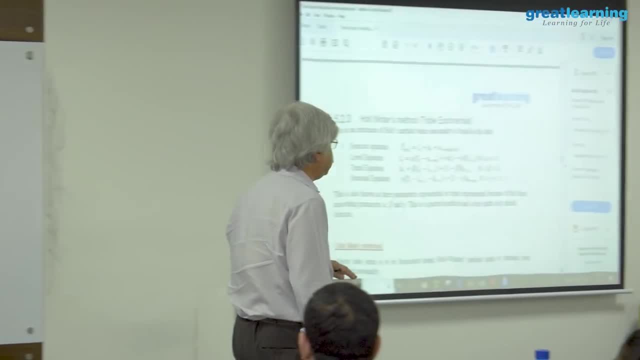 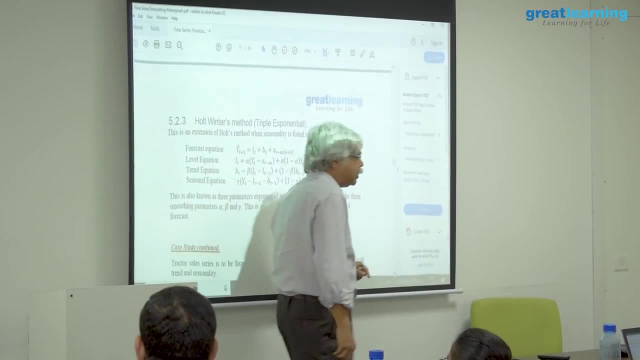 everything in it and then let the data say what the what the equations talk about. in other words, let the data decide as to whether there is a trend, whether there is a level, and what the level is and what the seasonality is, which is what we are going to try and do. hold on to this. we're going to come back and 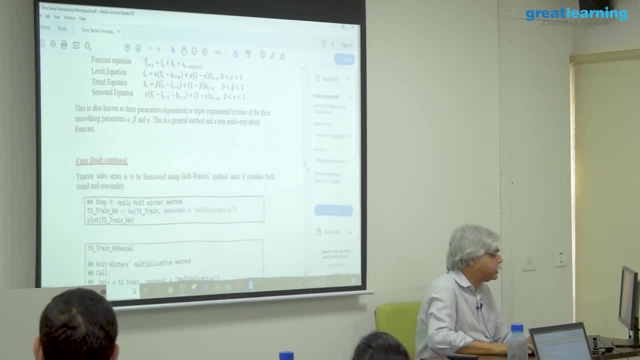 interpret these coefficients a little better. so, as I said, the, the, the object of this is easy, so apply Horst methods. now what are we going to do? we're again going to work this on the training set and going to work this on the training set for whole twins. 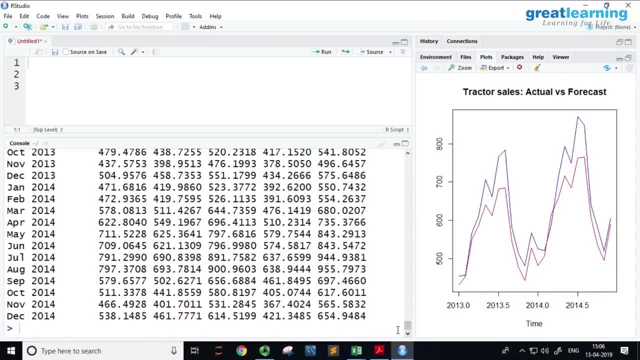 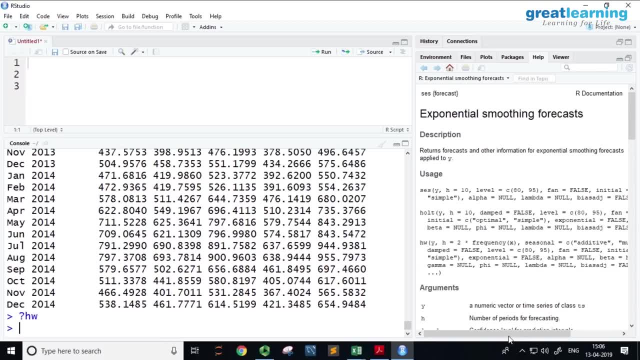 we'll see what it does. Now, one of the things that should be there is, say, holt winters. if I do holt winters and I just ask for the, the help on holt winters, here is the help on holt winters. So holt winters is the function, y is the time series, the forecast horizon, how long it will. 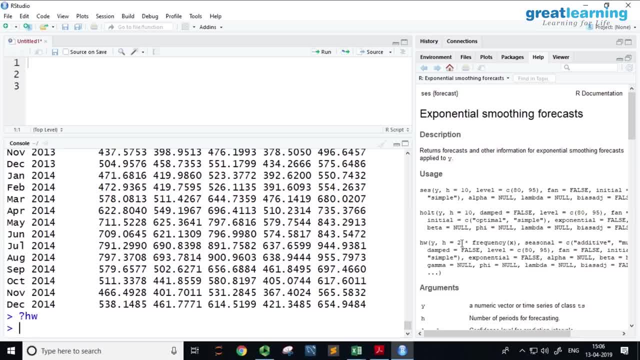 forecast for as a default is twice into the frequency of x. Now what for me? what is the frequency of my input time series 12.. 2 into 12 is 24.. So the default of h was here 24.. I could. 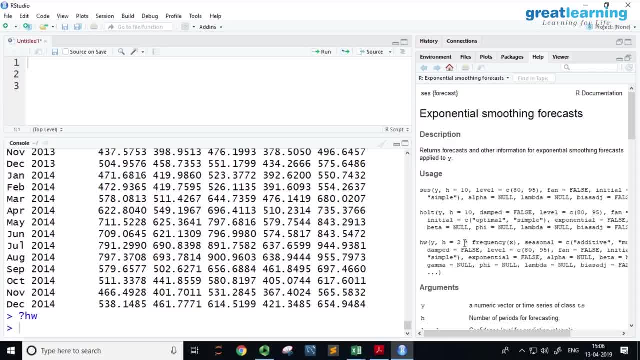 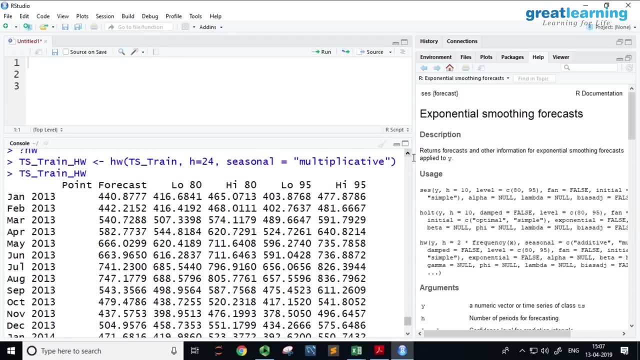 have said h equal to 24 and would have, would have given me the same answer, but the default here happens to be 24.. But you can, if you wish, write this as: but I didn't need to specify h equal to 24 here. So it's now given me. it's now given me this forecast, Just like the, the. the. 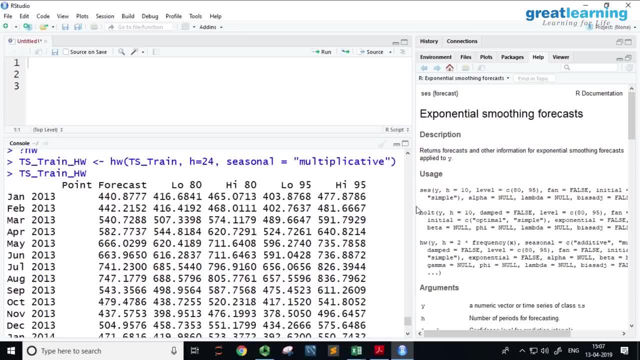 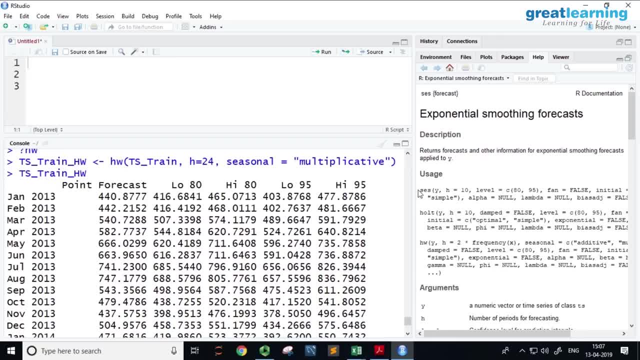 we'll try it out and we'll see what happens. So SES means simple, simple exponential smoothing. right Now, let me explain what simple exponential smoothing might do. So for simple exponential smoothing. why simple exponential smoothing? likely to be a likely to be a bad idea. Let's see what. 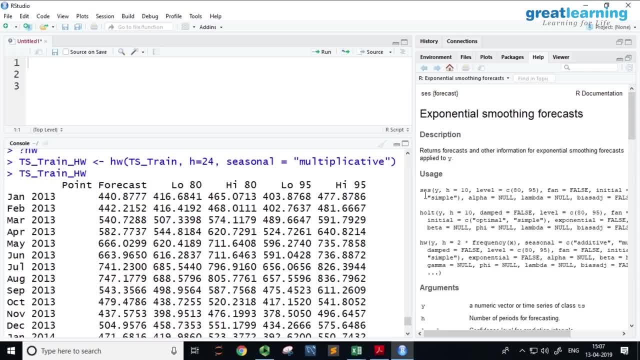 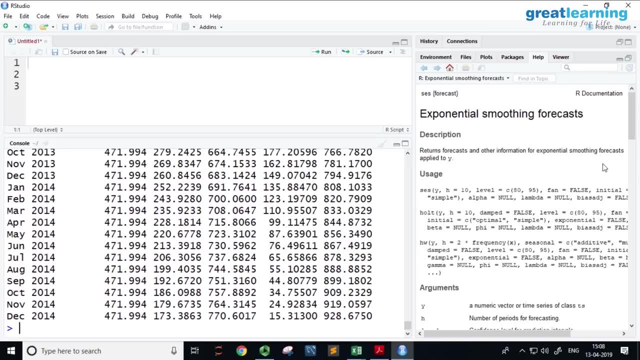 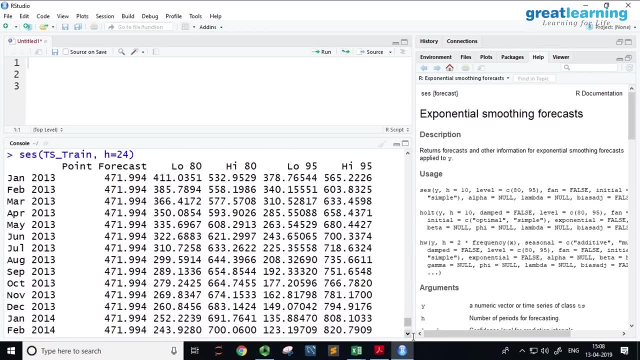 happens if I do simple exponential smoothing. So let's suppose I do this. I say: remember, there is no seasonality here. Here is my holt winters. This is my simple exponential smoothing. Do you see anything interesting about this? What are the forecasts Same? No, it's not an average. This is 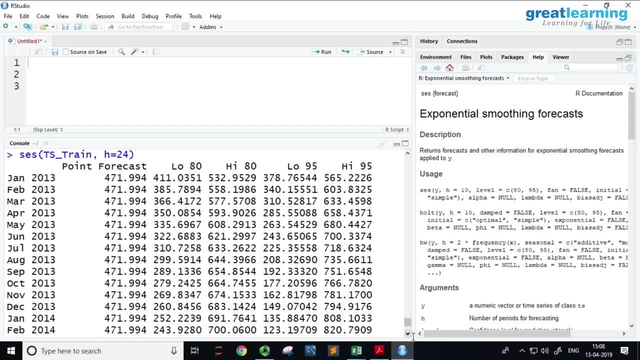 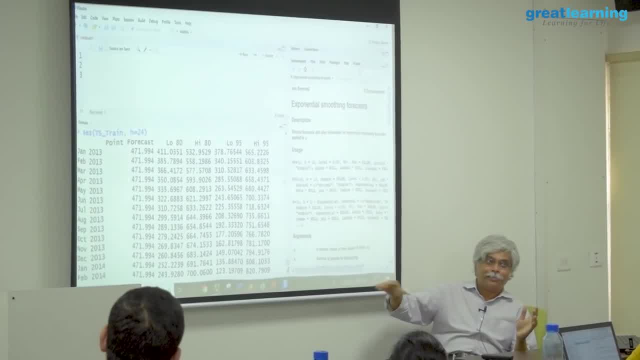 not an average. I'll see what. I'll tell you what this is. But point number one: the forecast is the same. There's no seasonality, There's no trend. There's nothing. There's no seasonality. There's nothing. There's a flat line. It's a flat line, which is why we didn't do this. But why does it? 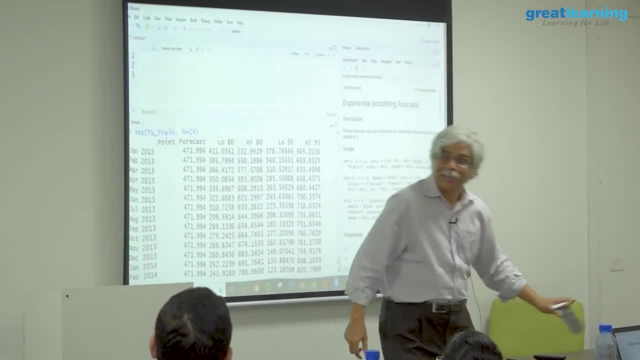 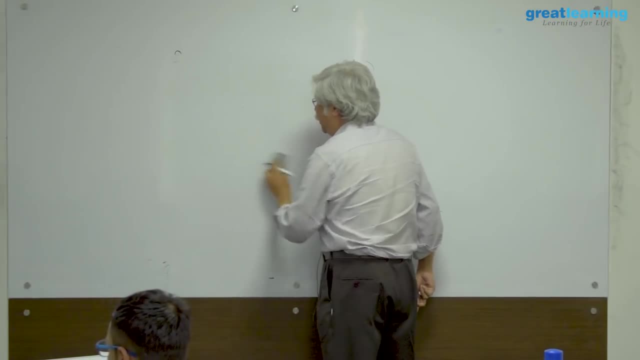 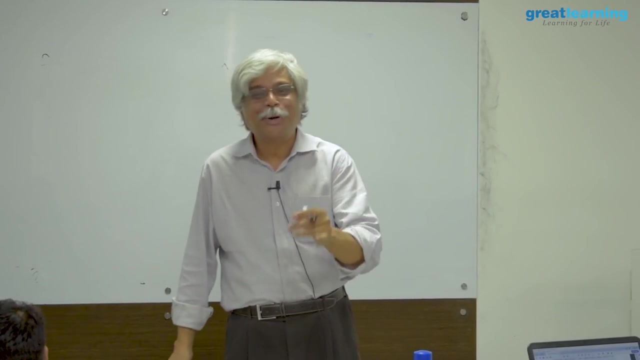 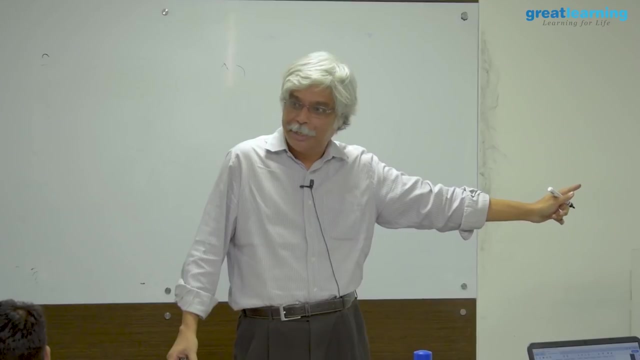 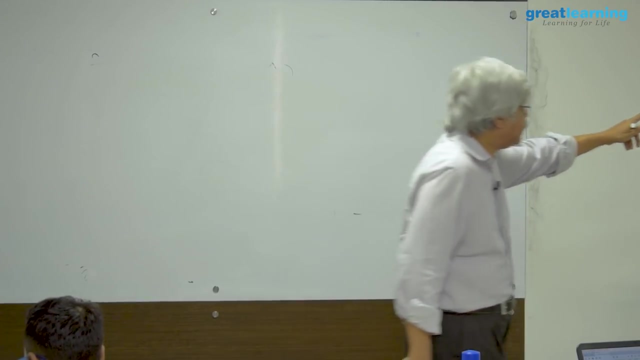 look like this. You're cynical, aren't you? So it does forecast, but it forecasts only one time point ahead, Which is what Excel's version did? It forecast one time point ahead. It took the most recent data and forecasted using that. Here, my syntax said: you must forecast 24 times ahead. You must forecast. 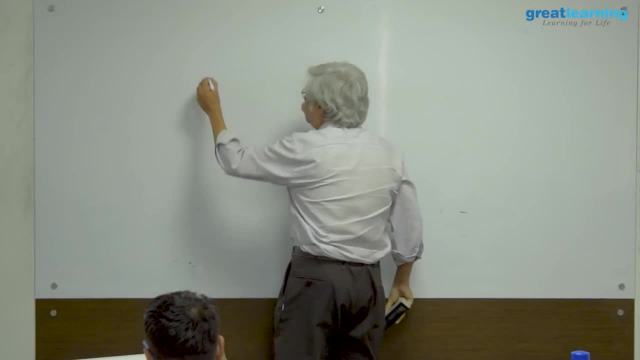 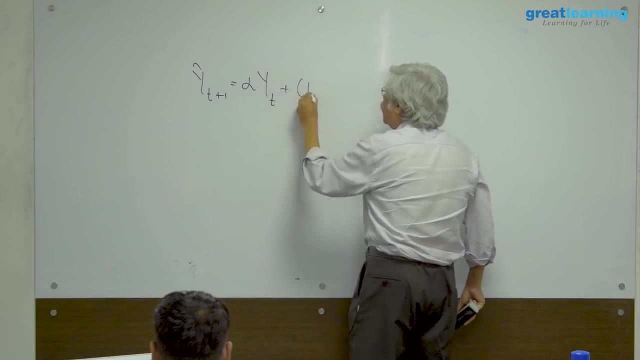 24 times ahead. Now, why does it look like this? Remember what my original, what my forecast formula was: Y t plus 1 hat is equal to what was it? Remind me of the formula 1 minus alpha y t hat. Okay. 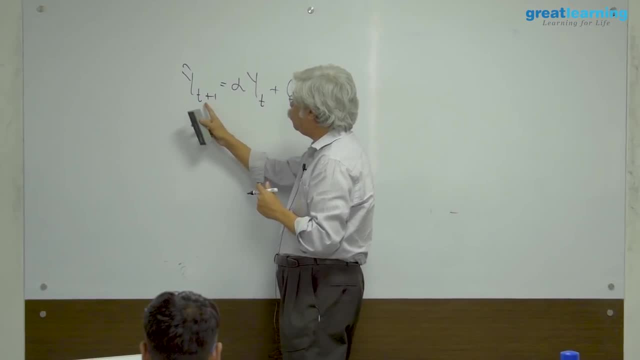 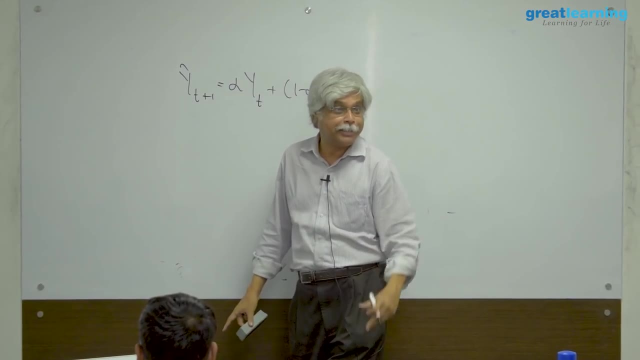 Excellent. Now let's suppose that I have my data and I forecasted y t plus 1 hat. I've got one forecast So far. he can't complain because I've given only one number. He can't say it's the same because he hasn't seen any other number. But now we have to see the next one. Now what? but what is? 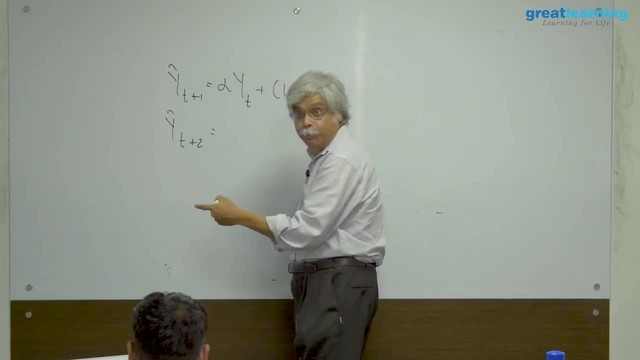 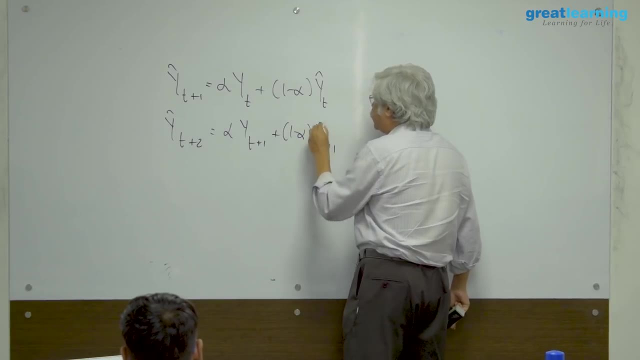 y t plus 2 hat. The next time point: Alpha y t plus 1 plus 1 minus alpha y t plus 1 hat. Excellent. Now y t plus 1 hat I already have. But what is y t plus 1?? 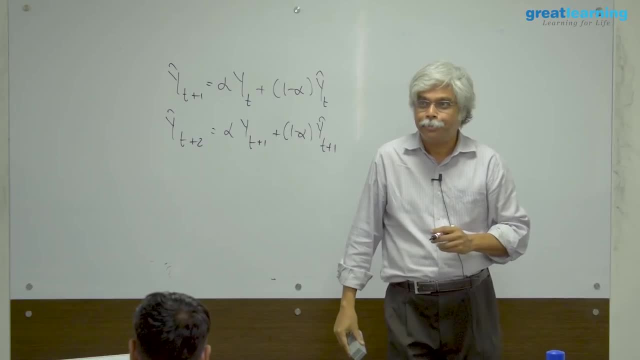 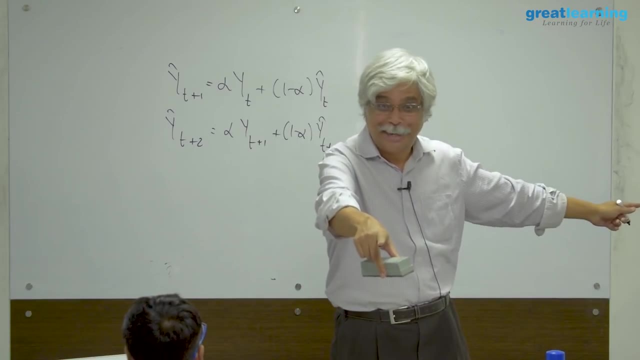 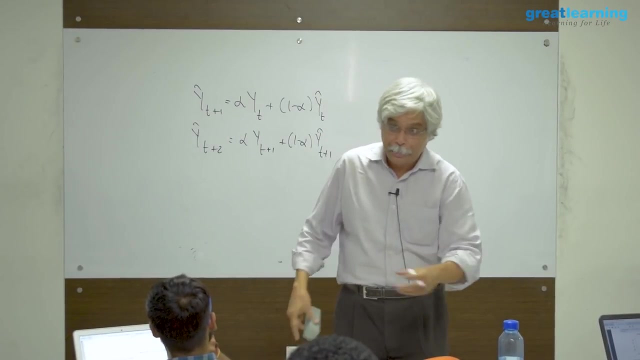 Yes, But I don't have y t plus 1.. Correct, Wait, Wait till tomorrow, Which is what Excel did. Which is what Excel did Every day: use the previous data, predict. So I can't wait for tomorrow, But I'm sitting here and I'm going to predict two years in two, two months in advance. 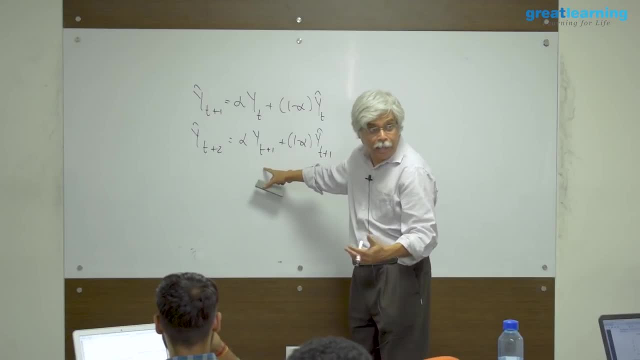 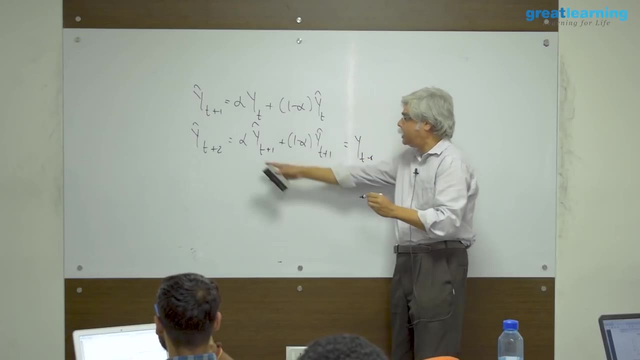 So the best that I can do is, whenever I see y t plus 1, I use its forecast. But as soon as I do this, this is what Not cancels out. This is the same number Alpha into y t plus 1.. So this is y hat t plus 1.. 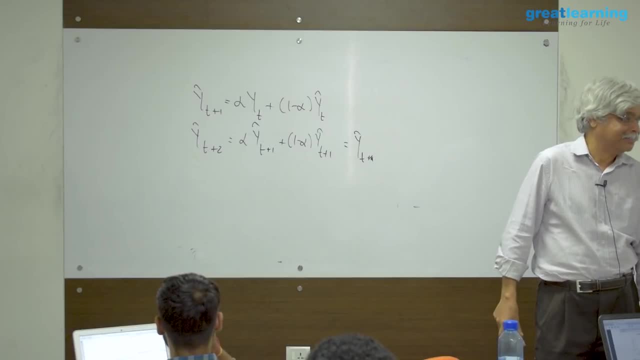 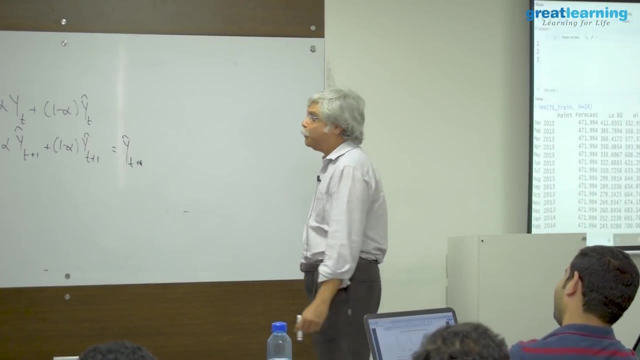 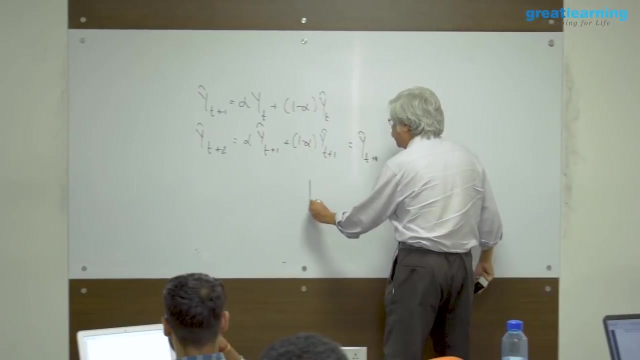 And you get the same number again And the same game plays. Hence, simple exponentials. So therefore, beyond one point, this is not helpful. Or, if you want to think of it pictorially, what it does is it sees a data of this kind and it says: 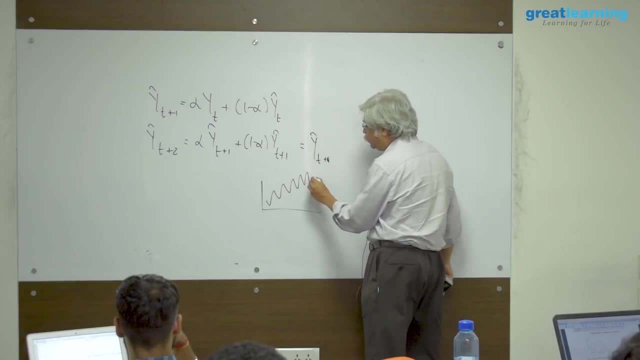 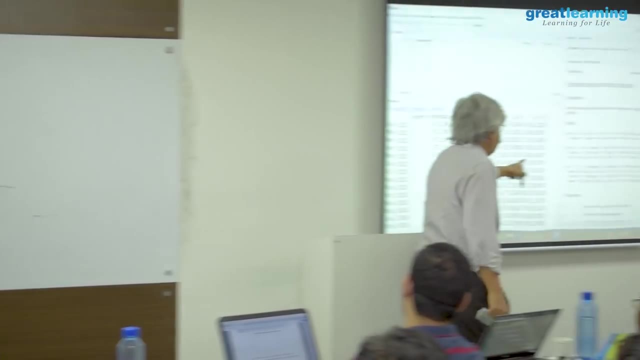 fit only a trend, Sorry, fit only a level, Which means it fits only this. What, what, hold this? what the second forecast will do is the second forecast will do is: I'm going to fix that problem by adding a trend feature to it. So in other words, it's going to allow to do that. 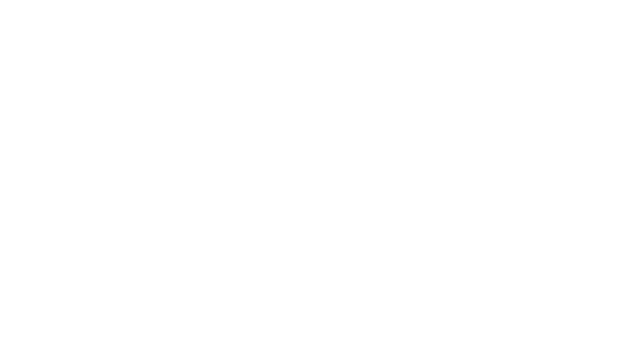 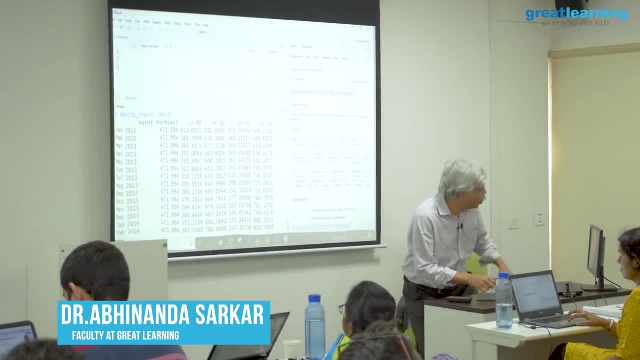 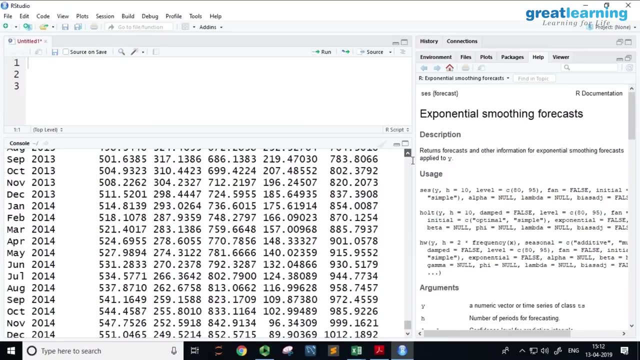 now, if I, if I change this to, let's say, hold, in other words, I do exactly the same thing, but I fix it now, I'll get a forecast. now, the numbers are not going to be the same. now, the numbers are not going to be the same. 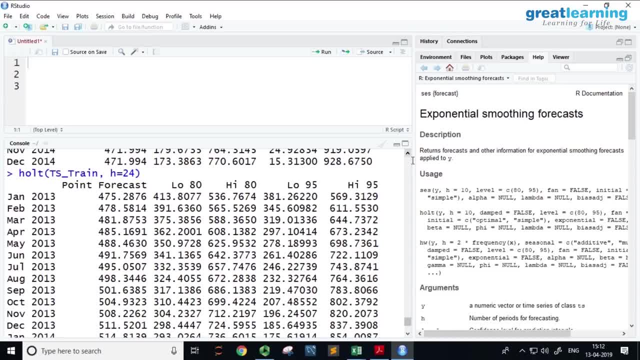 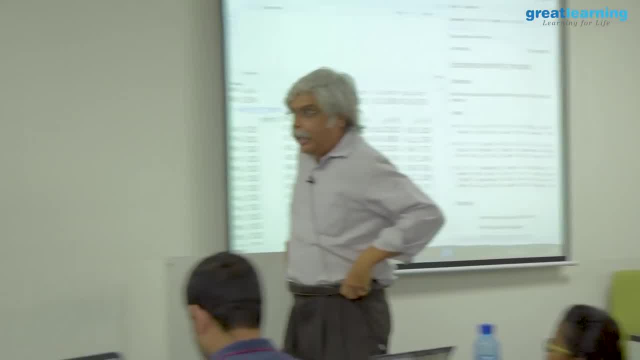 it's increasing by about 3 or a little more than 3 every month. it's getting, it's recovering that trend. it's recovering that trend. it's not necessarily exactly a straight line line. it would have been exactly a straight line if the beta had been one. 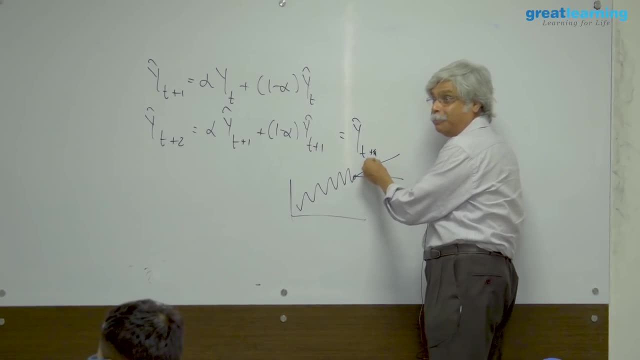 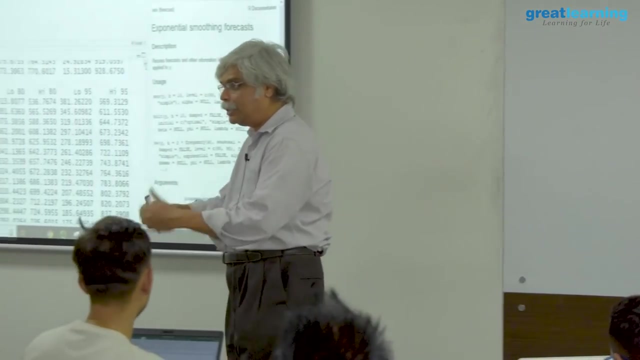 but remember, it's also learning a little bit by the changes in the levels, but the changes is level one, in this case a constant. so effectively, what it is doing is is approximating this by a straight line. so the forecasts are increasing, but they're increasing in a lockstep. they're increasing by the same amount every time. 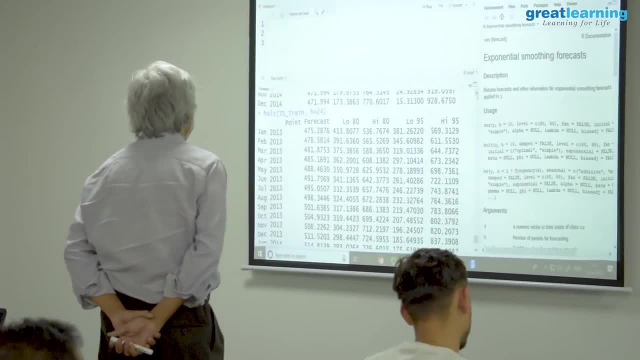 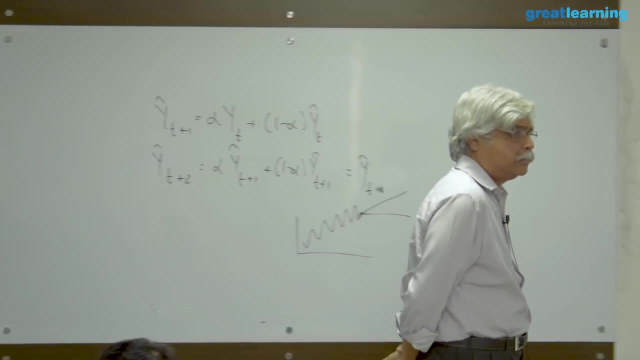 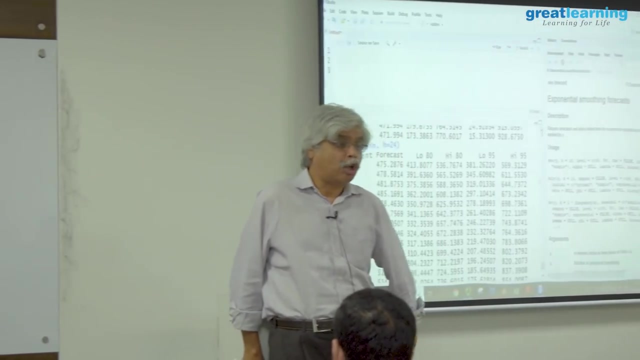 January to February is the same increase. yeah, February to March the same increase. every watch me, same easy. there is no sense of seasonality in this. you can see the same jumps. so this solves the problem a little bit. now what I need to do is I say, okay, the, my series is not constant and I fix that problem by 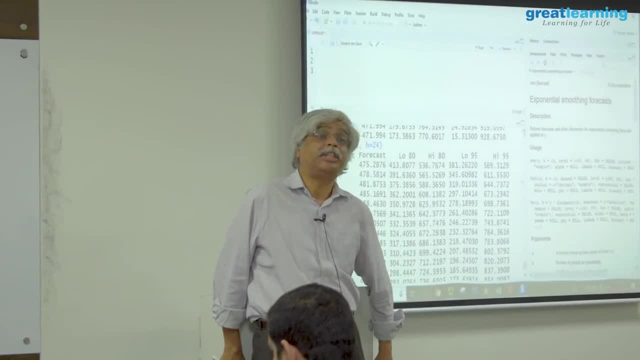 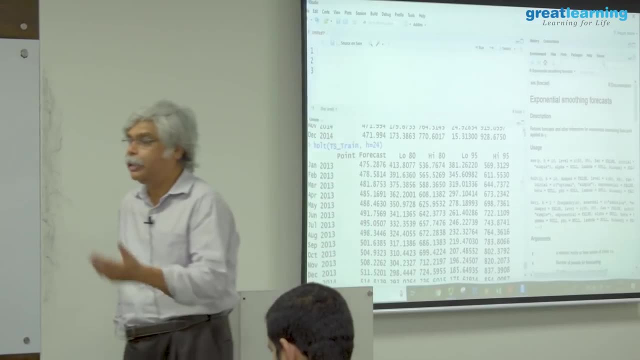 saying my series is allowed to increase. now I have to say my series is not stationed not, is not non seasonal. there is a seasonal correction that I need to be able to add. that correction is added by the triple exponential smoothing, which is what they called whole twin test here, which now 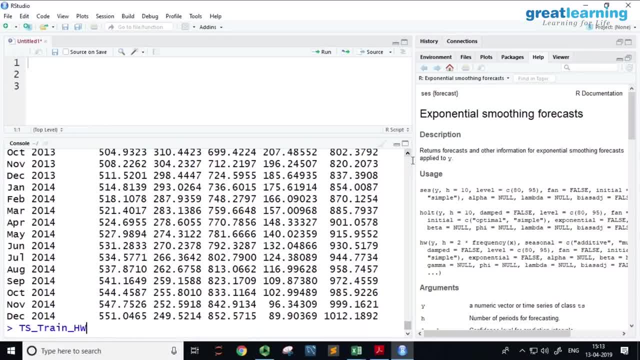 incorporates the linear combination of spines and the linear combination of the linear combination of spines and the linear combination of spines and is the seasonal correction to this. but now, if you do this, you, you should argue, so i can do the, i can do the same command, so it is whole twinters. but for seasonal i have an additive model i also have. 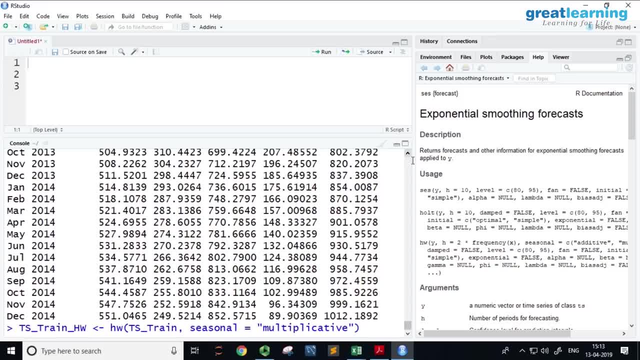 a multiplicative model. in this particular case, i want the multiplicative model because i know that the trend and the seasonal irregularity multiply with each other. i don't know that. to some extent i'm guessing it by looking at the picture, but this i can specify. this is why i end up with this, and 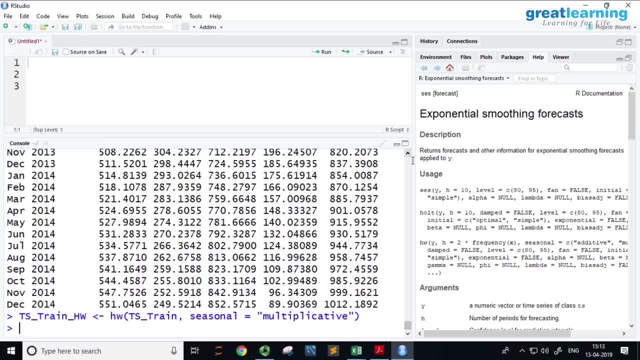 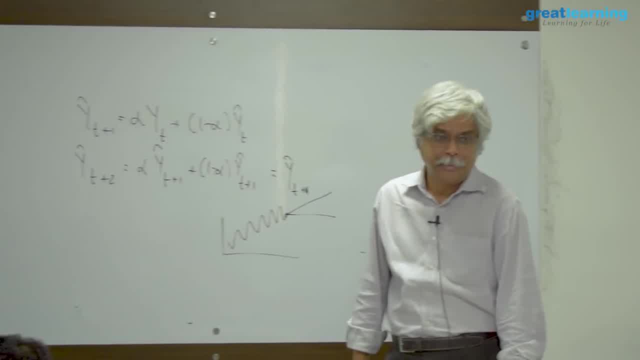 and what you? what you can argue is that if you have a series in which you do not think there is any seasonality, then you can stop at this at the second one. the third one will add a layer of complexity that might be picking up just noise, because if you think there is nothing called 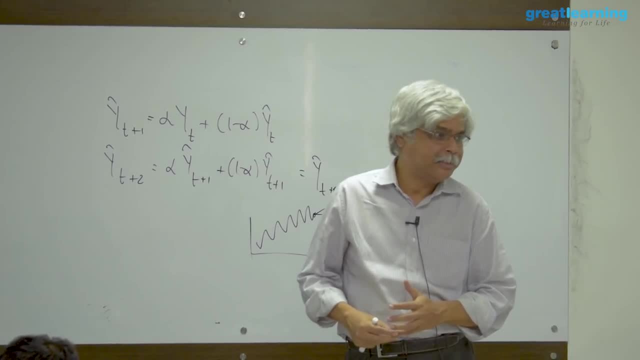 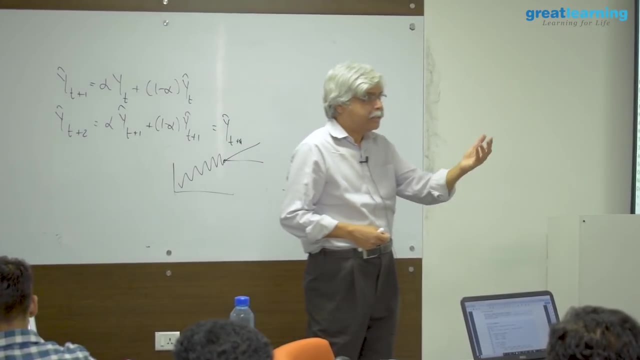 seasonality. it's said with, let's say, you're looking like at a stock price, looking at daily closing at a stock price, and you don't believe that there's a. there's a monthly or a seasonal effect. there is a trend, the stock price is increasing, but that's. 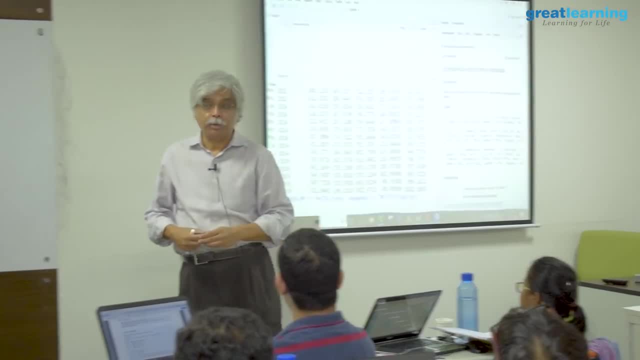 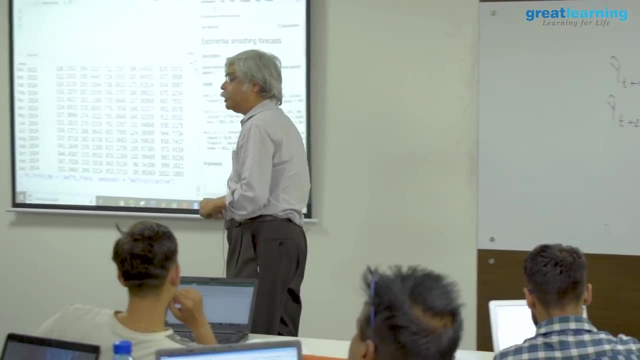 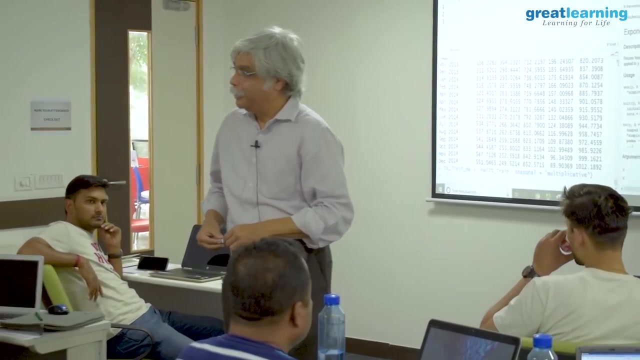 about it if you believe it to be so. similarly, if you believe that there is no trend, for example, if you believe that you know what my stock price is is constant, is not constant, but my returns are constant. so what i can do is i can calculate the returns and then do a simple, simple forecast. 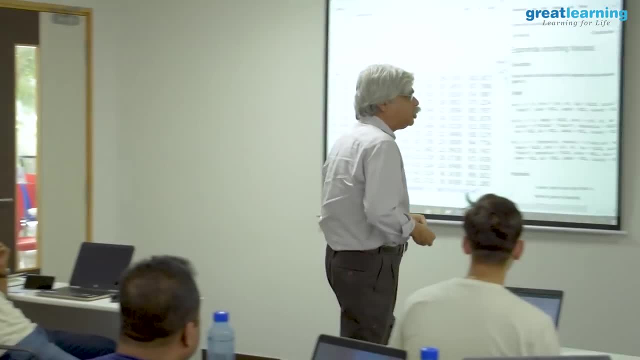 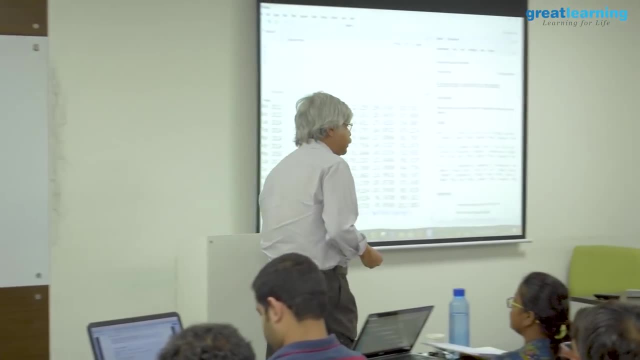 if you want to, although, as you said, the forecast will be flat. but then you're assuming that it will be flat, you're assuming that the returns are not going to be changing. there's nothing else to understand from those returns. so simple, exponential smoothing. but just to just to warn you. 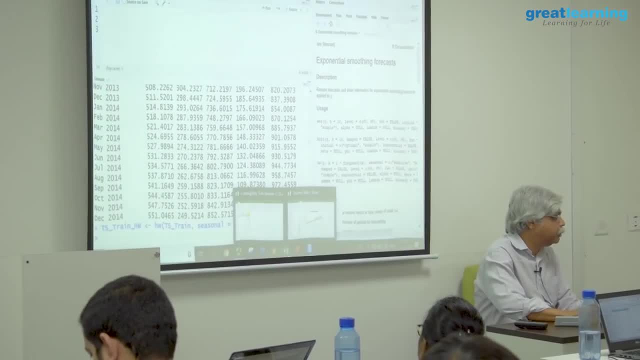 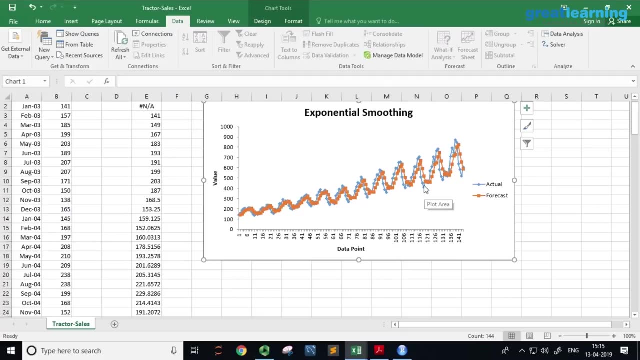 in excel. we got a very good fit. where is that excel spreadsheet? what is this then? this exponential smoothing? this is ses. this is ses, but what is this point? so there's a forecast. right, this is my forecast. why is the forecast this good? because this forecast is based on every point, just to the 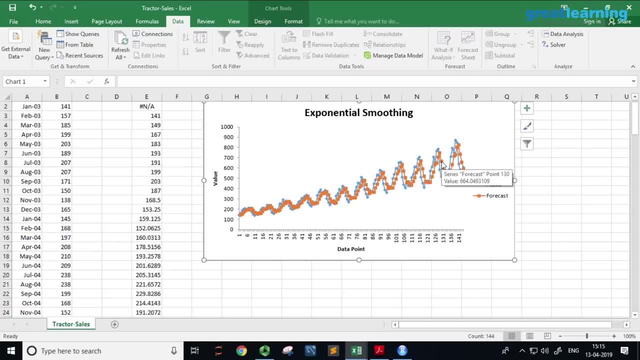 every point is a one point forecast every day is using the entire data set up to that point in time. so essentially, what is doing is is trending with the data. it's not forecasting 24 months in advance or 12 months in advance. it's only forecasting one month in advance every time. 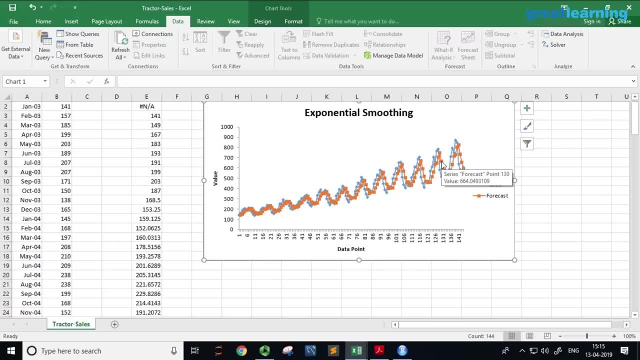 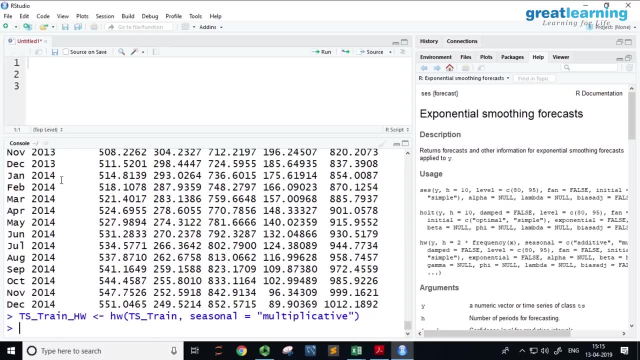 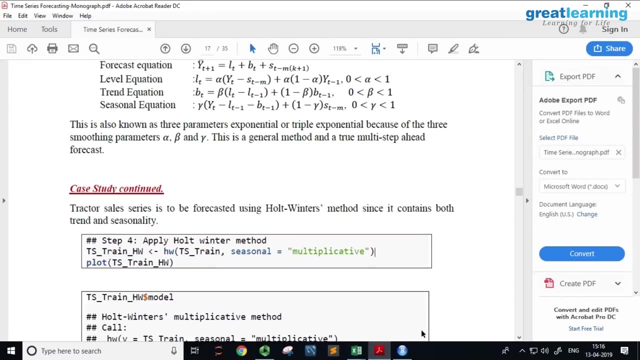 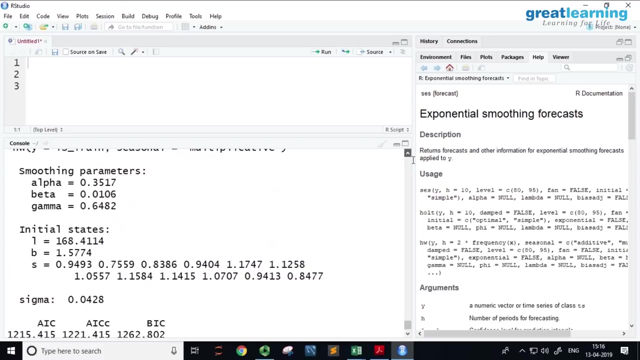 and you can fix that, filling around with excel if you want to. here we've asked a hard problem, mind you. we've asked to predict two years. we've asked to predict two years. that's not an easy thing. now the model itself. what does it say? here is the output of the model: smoothing parameters. 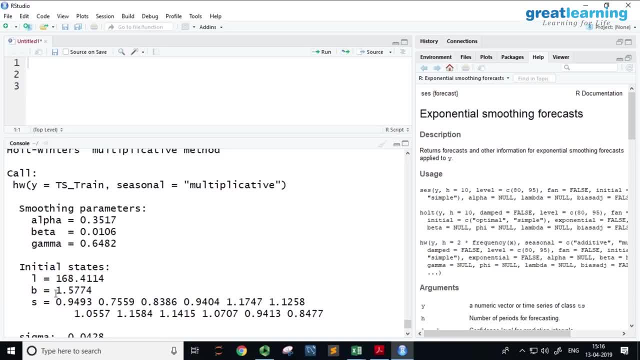 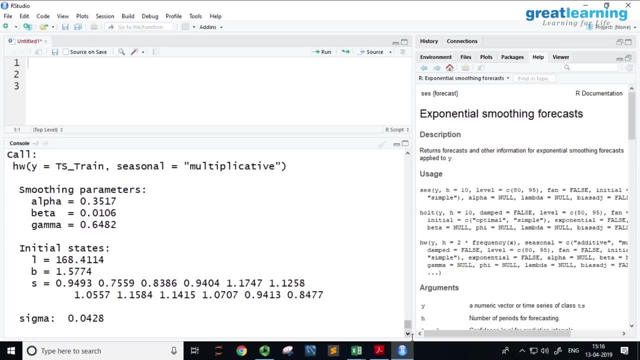 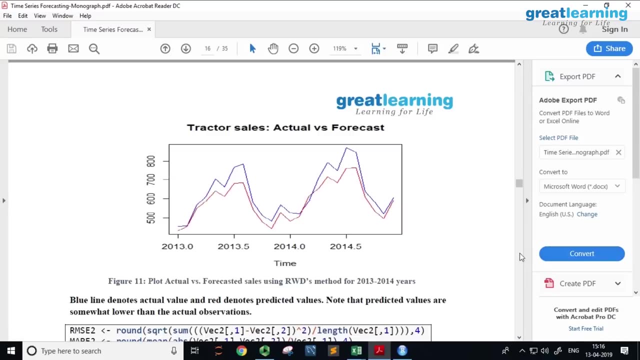 the time series began with. this is what the time series began with: forecasting with. it said: I'm going to begin with 168, correct? where is the one? where is the 168 coming from? where is the? where is the 168 coming from? not at the beginning of the forecasting window, but where is the original data? 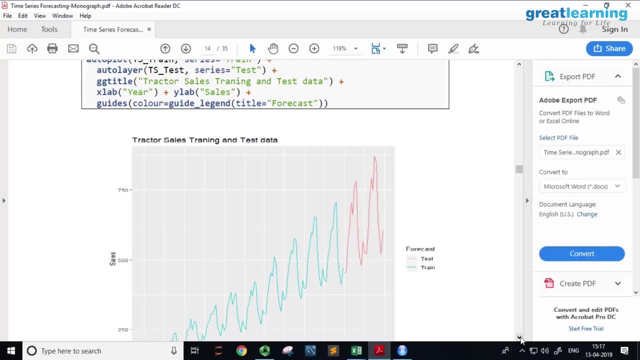 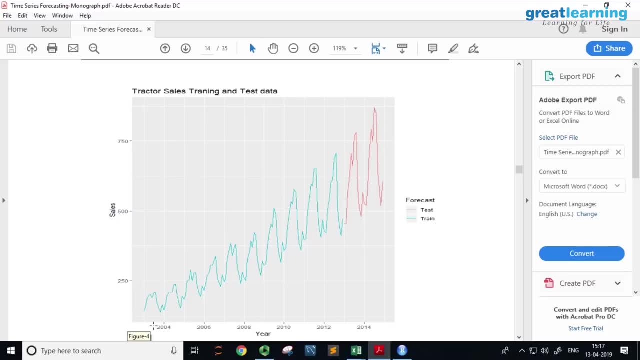 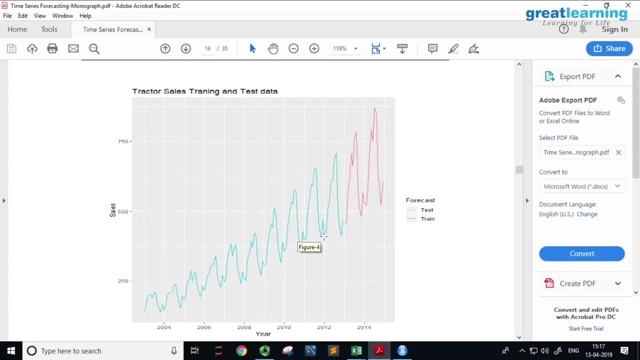 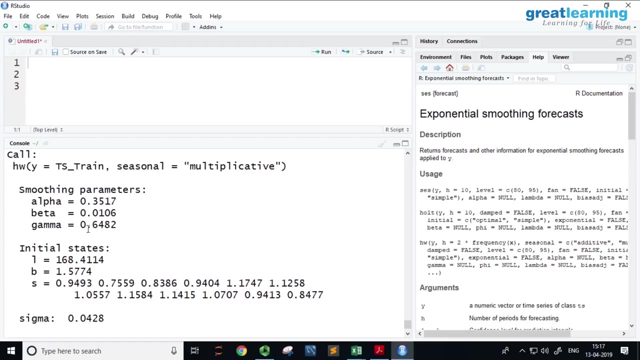 the new level. how do I get to the level after that? the current level that I have and the current point new level, and I keep building up the level. similarly, I keep building up the trend, beginning with a certain value of the trend, which is point zero, one, six, and this is the seasonality fix. now these 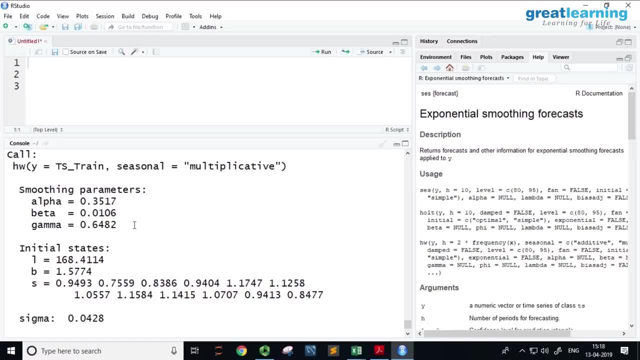 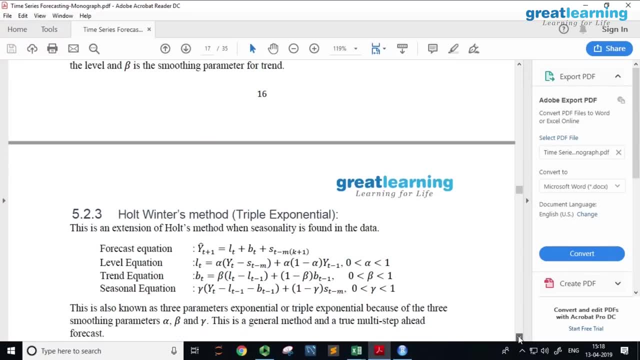 values means what? point zero one, three, four. point zero zero one, three, six and point zero one. so let's go back and understand this and it gives us a little bit of interpretation as to what is going on. so beta, for example, so alpha, here is the smoothing, is the smoothing of the smoothing of the level. this is 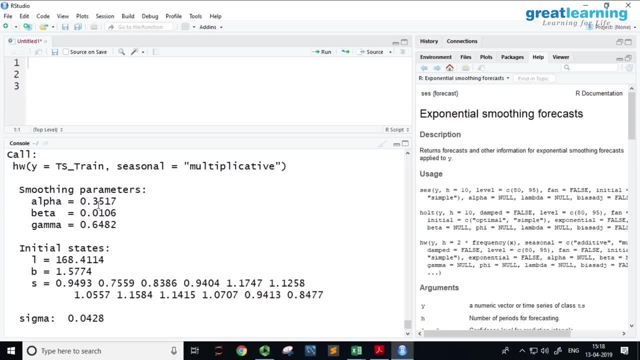 our point three, five, not very close to zero, not very close to one, which means the level is an average or a combination of my, of my current value and my pass level. but this beta is very close to point zero. point Z is close to zero. beta being close to zero means that the current value, of my current value is. 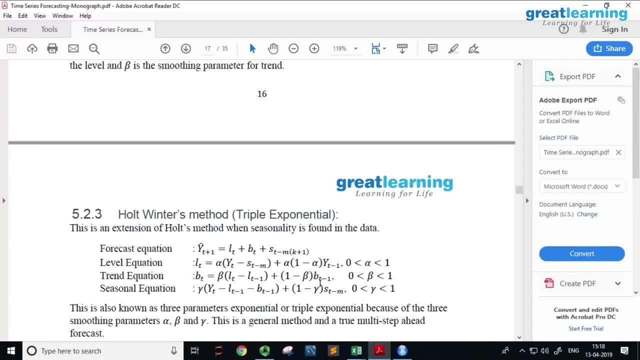 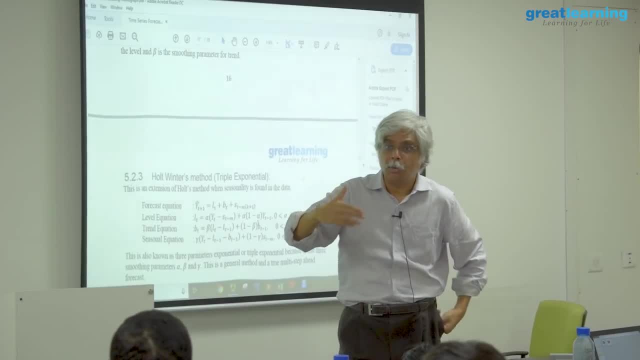 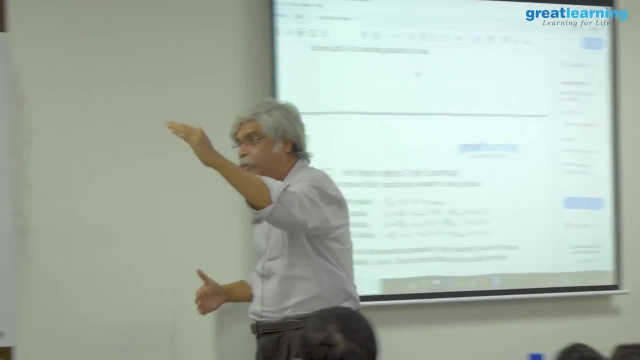 zero means what it means. beta is almost this, which means beta is very close to the previous beta. that means my trend is not changing much. my trend is remaining the same. what that means is my series is fairly constantly increasing. if my series was not constantly increasing, what would have happened? what would have? 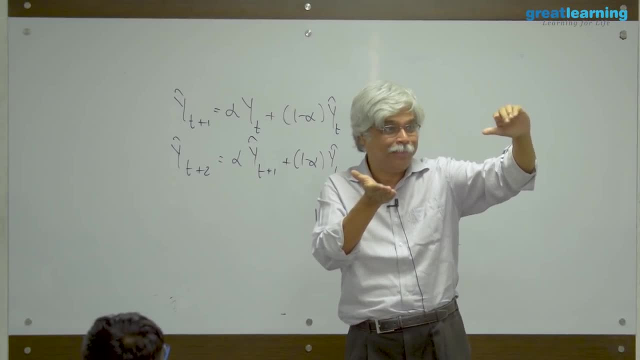 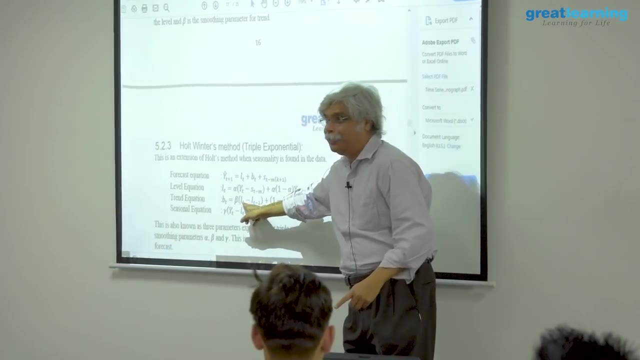 happened is that the trend would have wanted to change every time. every time, the trend would have said: please update me, please update me. based on what? based on the current change in level, the time series was doing this, then LT minus, LT minus one would be changing and 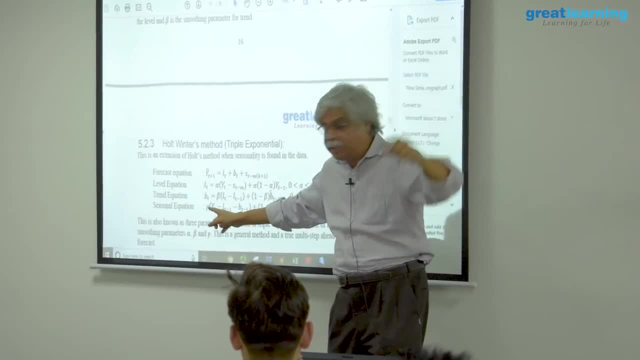 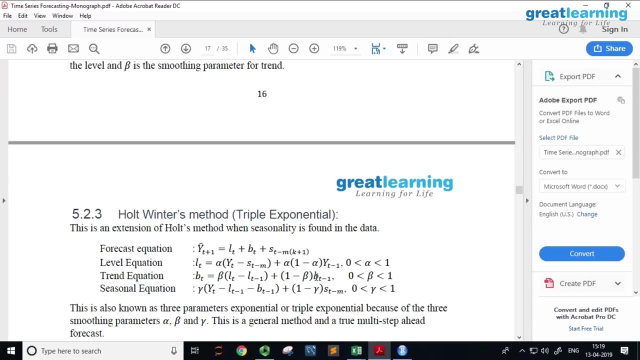 the trend will want to adjust for that. but here beta is very small, which means this term is very small. so the adjustment due to the change in the level is very small and the old trend stays. that's why it's very close to a straight line. but if it wasn't a straight line the model would had the 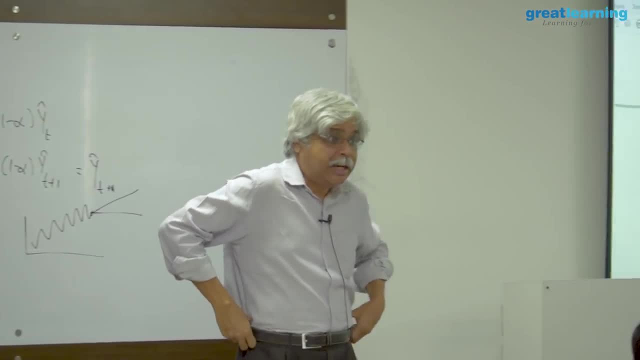 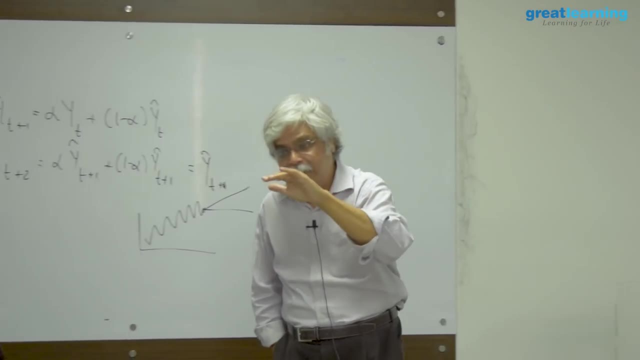 power to add, adjust to it. it doesn't need to be a straight line, it just needs to keep refitting the straight line and the slope of that refit can change, and that's all right. Abg, it can simply. appreciative is so if the level is. 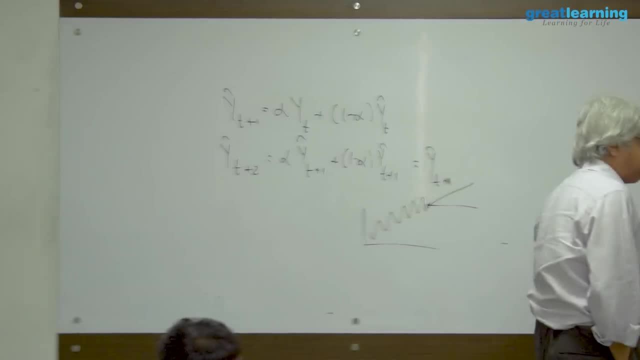 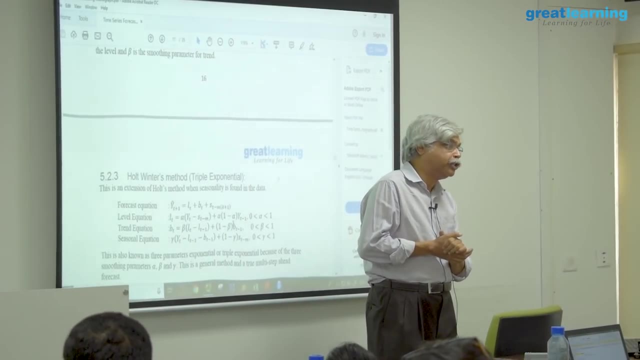 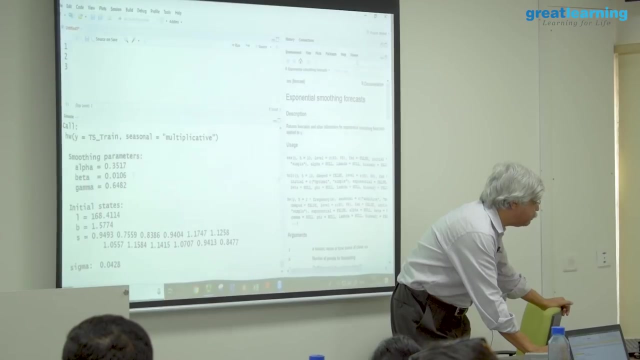 changing. it has the ability to change the value of beta or change the value of B. so my estimator beta is telling me the fact that it is a low number is telling me that the trend is nearly a straight line. my slope does not need to change much. if, for example, my alpha was very, very low, what would have that? what would 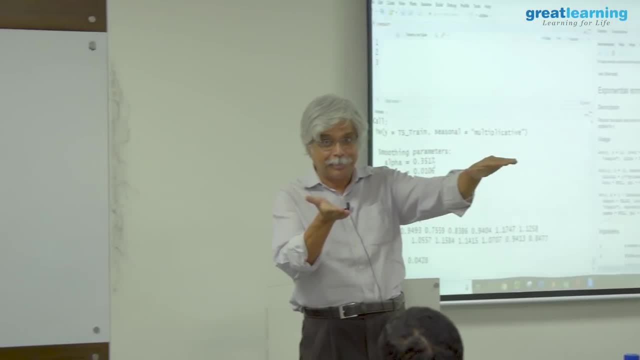 have that told me. if my alpha was a very low number, I would have concluded that'mime level is not changing, which is my series is doing. this introduction telling me that my level is not changing, which is my series is doing. series is not flat. my series is increasing, so my alpha has to stay away. 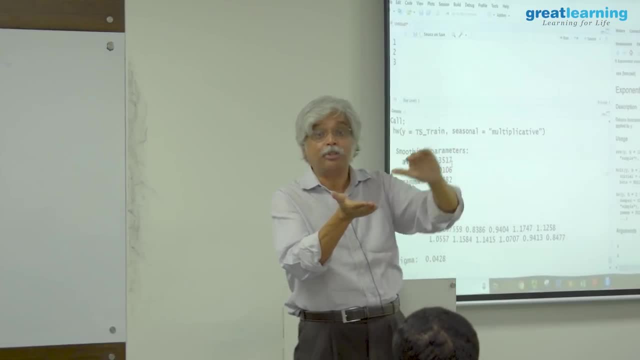 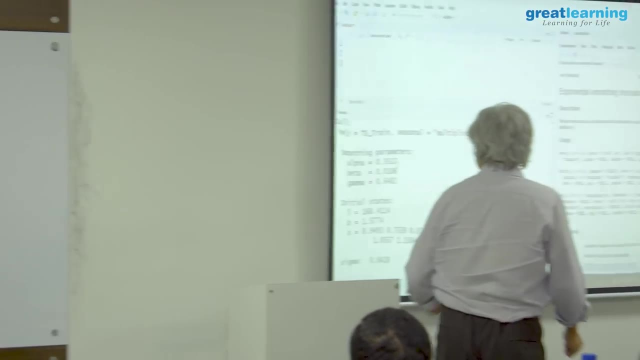 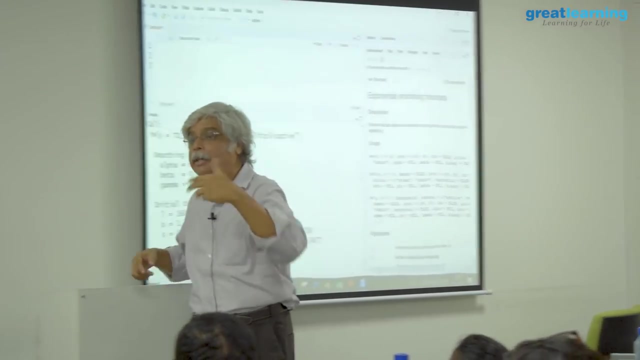 from zero to be able to increase. but my trend does not need to increase. my trend can remain the same. seasonality, seasonality is, is this: this number is high. this number being high means what this number being high means: he has a seasonal, there is seasonal fluctuation, and is trying to adapt to the seasonal. 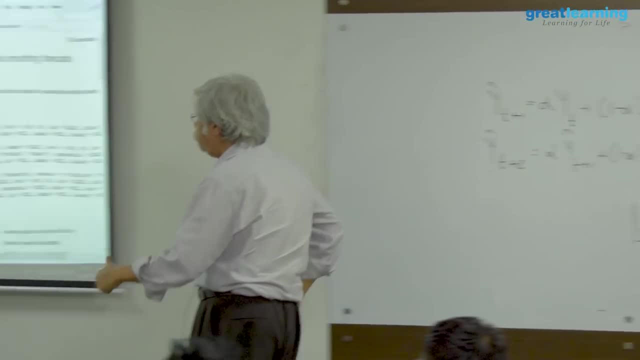 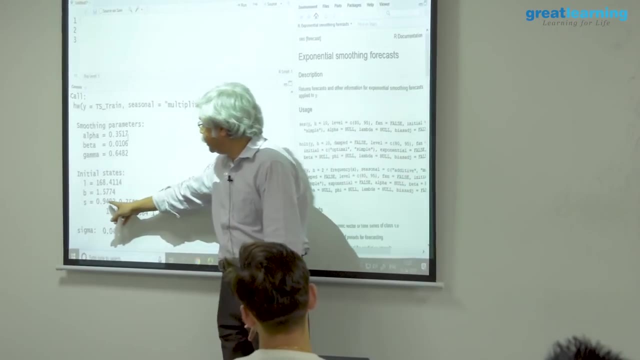 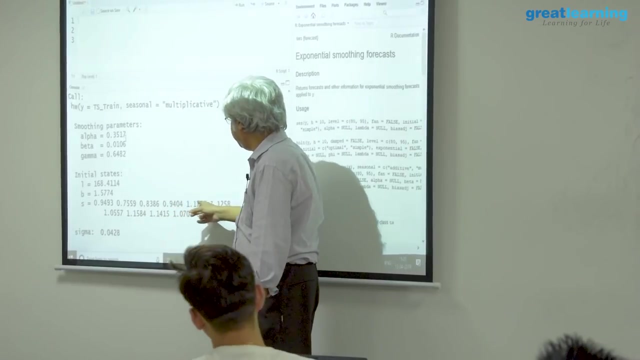 fluctuation as it goes along. so what that means is going to begin with these corrections. this is the initial correction factor for the seasonality and it begins by saying: January is about ninety four percent, February is at about seventy five percent, wherever it is, if every March, April, May, June, July, this is 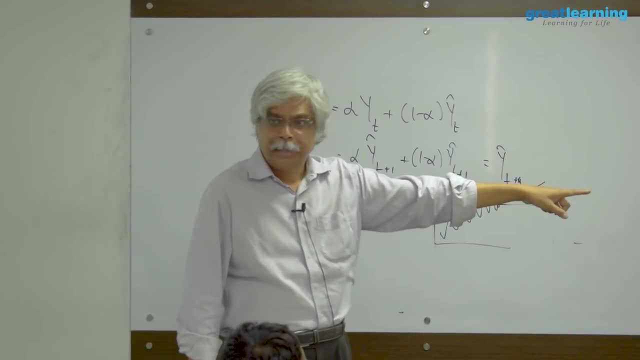 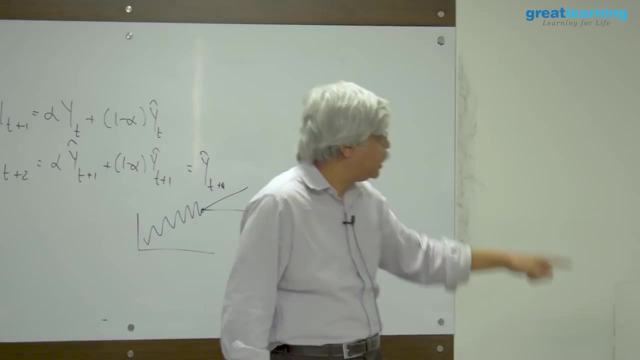 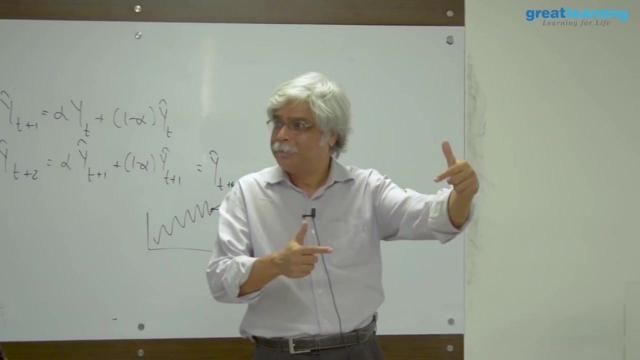 every month. there are twelve of those every month, and it begins at that. it begins at that and it updates it. it updates it because that gamma is close to point six. so as the years go by, it keeps adjusting that number. if gamma was very, very close to zero, that number would not have been adjusted. so it's so, it's. 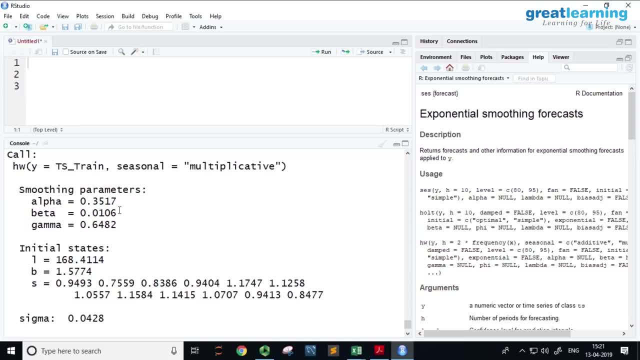 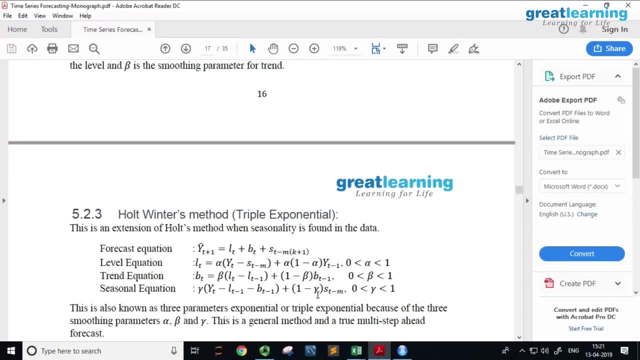 capable of changing the seasonality correction. if the seasonality correction is changing. you know, see, see the gamma here. if gamma is, say, very close to zero, then this is going to be almost like STM minus one, which means S of T is going to equal S of T minus one, which means S of T is going to equal S of T minus one, which 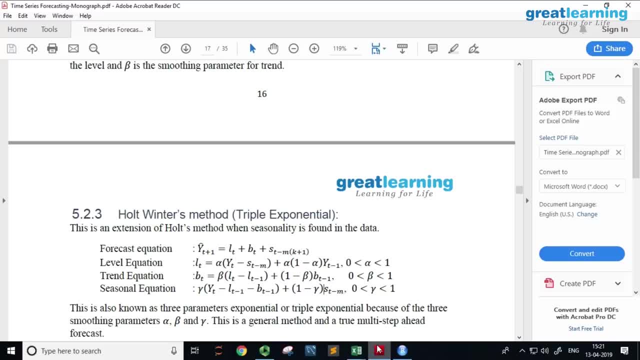 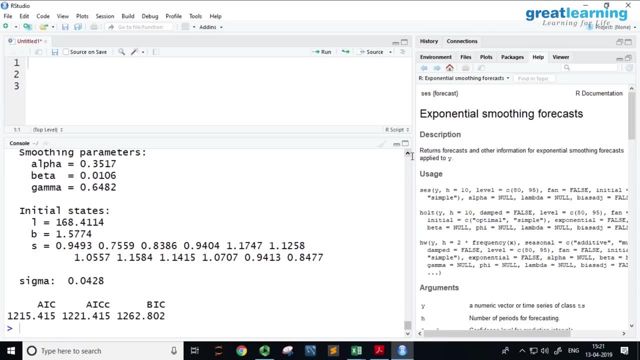 means the seasonal term does not change at all. so therefore, what this model does is really hard to interpret. but what this model does is it sort of tells you how what this fit is actually trying to do. if you don't want to hack into this model, that's okay. the forecast is there for you in any case, it's got certain. 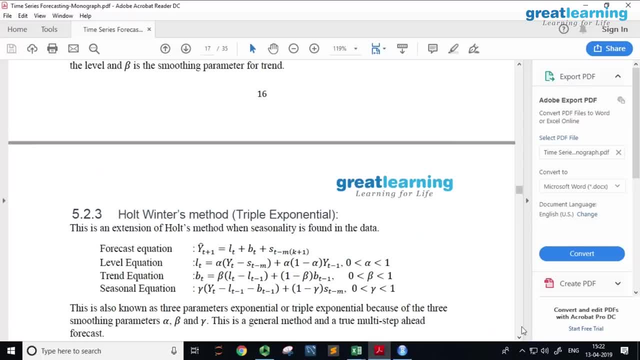 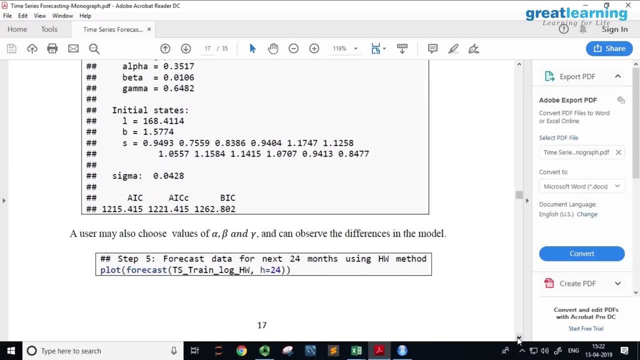 things here called the AIC, BIC etc. which are model fits, which are an interpretation as to how well the model fits. but you don't need to do that because we are going to look at models that way. we're going to look at models by comparing test and training anyway, so that part you don't necessarily need to. 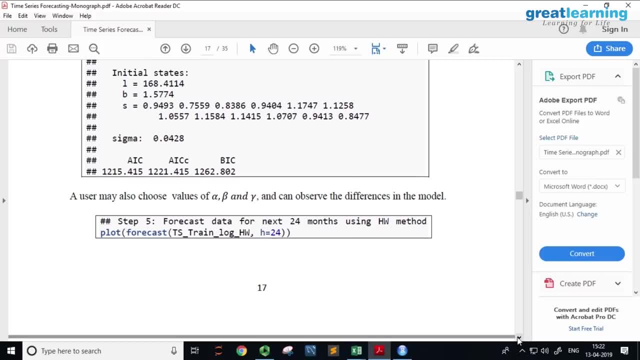 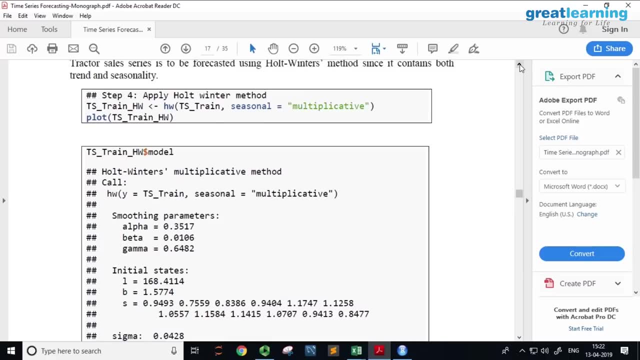 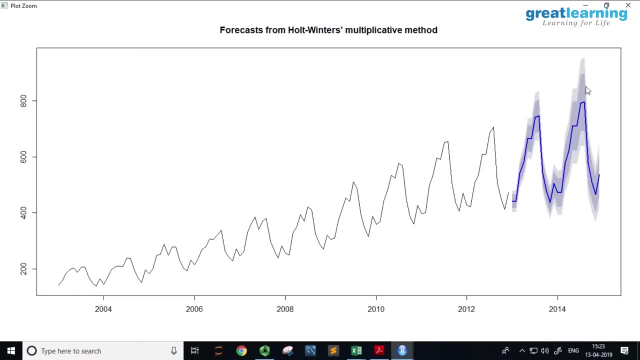 look at so we can forecast. in this particular case, this is just a plot of the forecast. yeah, log shouldn't be there, right, because we did not. we worked on a multiplicative without the log, correct? this doesn't look right. so this is my forecast. and again, these little boxes, in this particular case, weeks- my default. 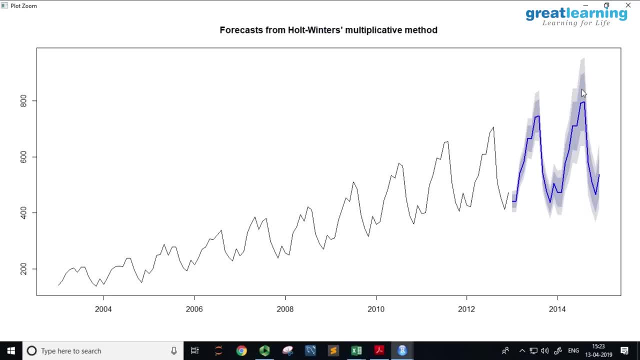 had been set at 80 to 95. I think this is your 80 and your, which means that you're 95% sure that I am between these two and, as some of you was, some of you were yesterday pointing out, at the end of all this sophistication, that seems way too large. 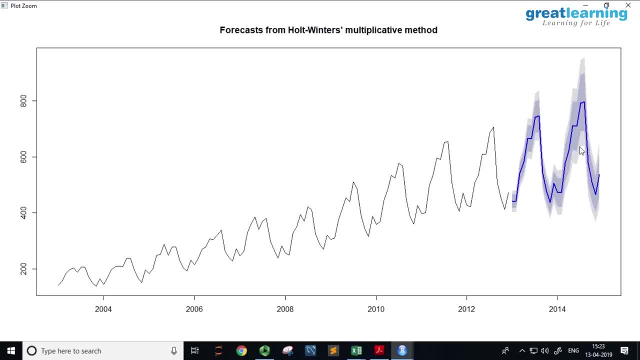 that seems like a waste of effort, but that's the kind of uncertainty that this data is carrying. so this is the point estimate and this is the forecast. so if you want an upper estimate of sales, for example, you should plan possibly for this happening, possibly for this a lower estimate, a pessimistic estimate. 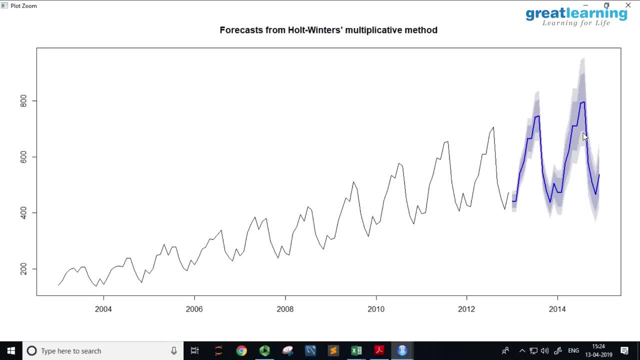 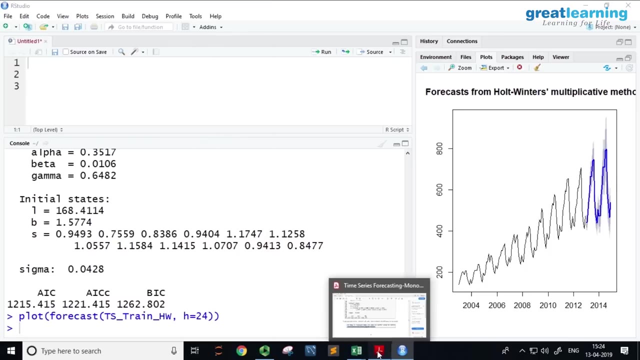 possibly could be this. no, no, this is only the forecast. we don't know that. we'll see that. we don't know that. we'll see that. we'll see how well it actually fits, as you were saying. we have a lot of data. we haven't seen that, but we can compare that, which is what we, which is what. 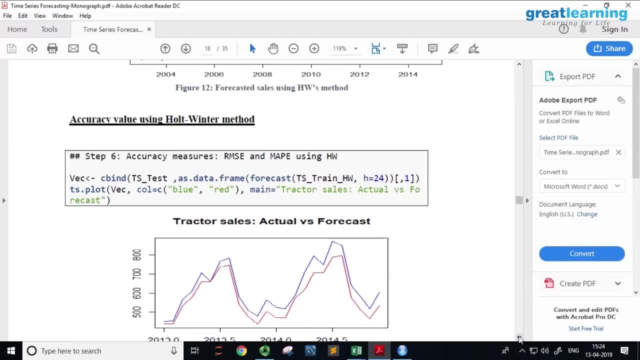 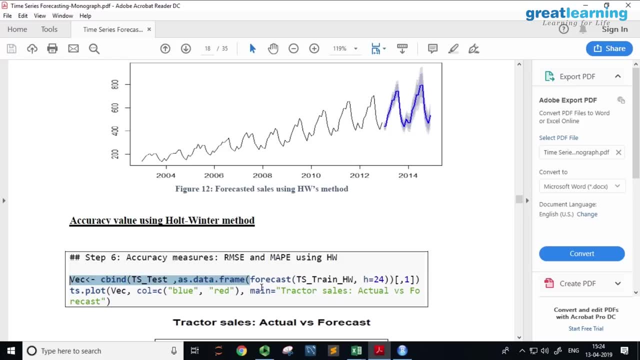 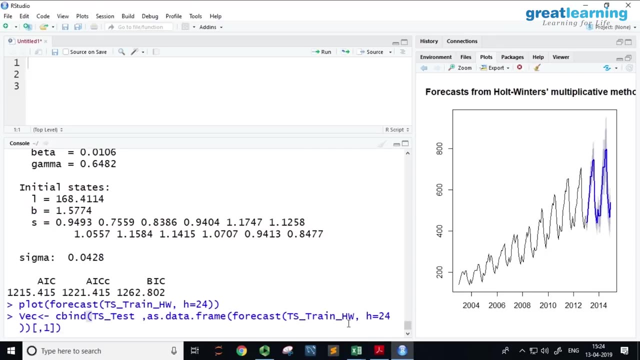 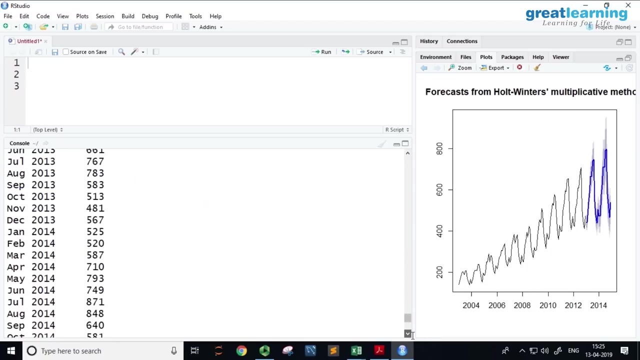 we're going to see here, which is the accuracy. so that's this. so what we're now going to do is we're going to combine the forecast and the actuals from this model into, again, a vector. this is my, this is my 2013 actual test: 454- and my forecast is here: 440.. 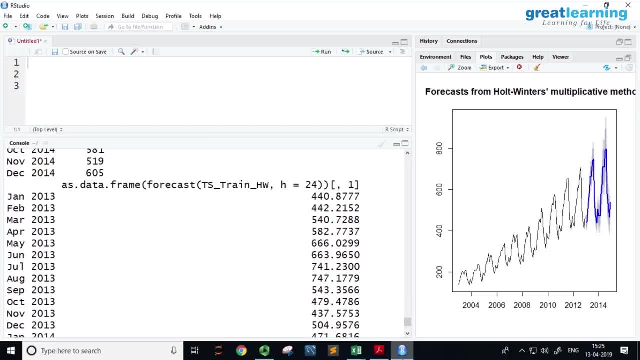 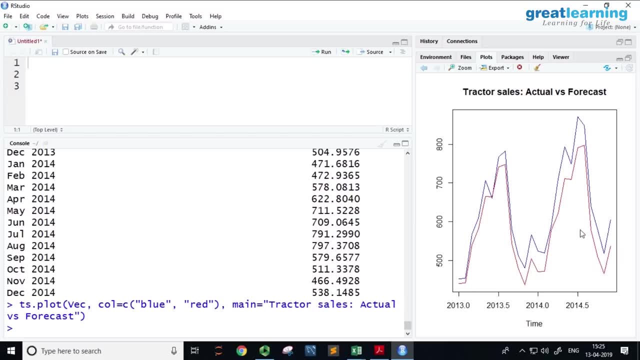 point eight, seven, seven, close, but perhaps not quite good enough. almost there, still little under predicted. still little under predicted. what does that mean? it means that the trend was increasing faster than historically. the last two years have seen an increase in trend. that is a little more than what the historical evidence of the increase in trend suggests. 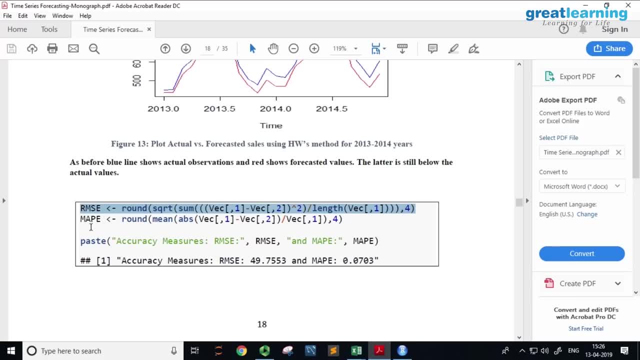 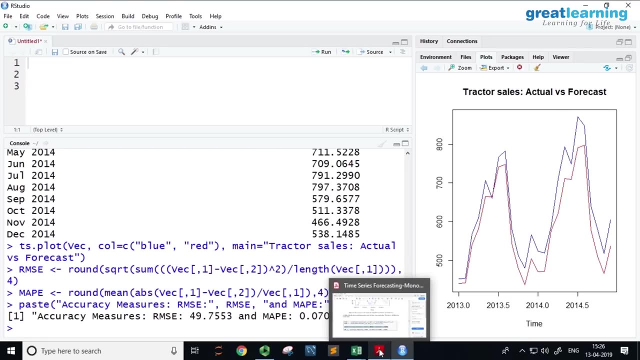 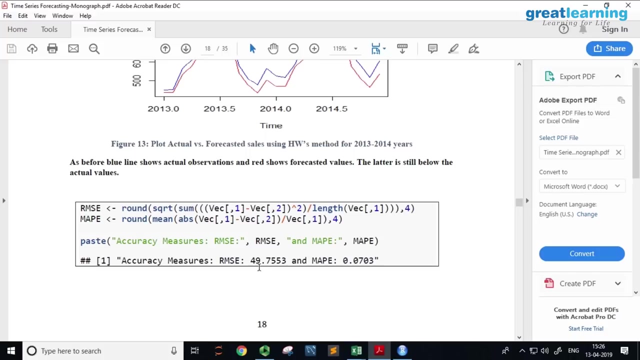 my, I'm doing exactly the same thing as before. the RMSE and the mean absolute predicted error, RMSE of 49 and MAPE of point seven zero three. since this is the second forecast that we are doing, is useful to compare this with the first one. this root mean square is about 49 and this: 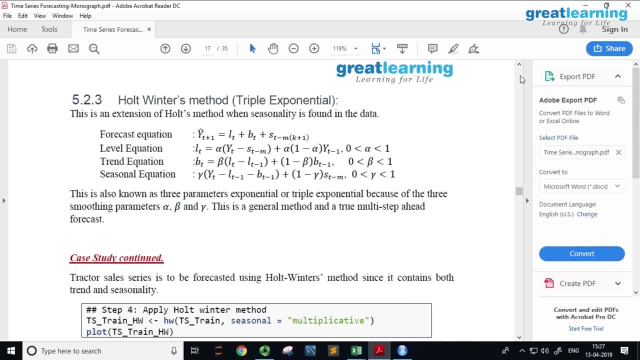 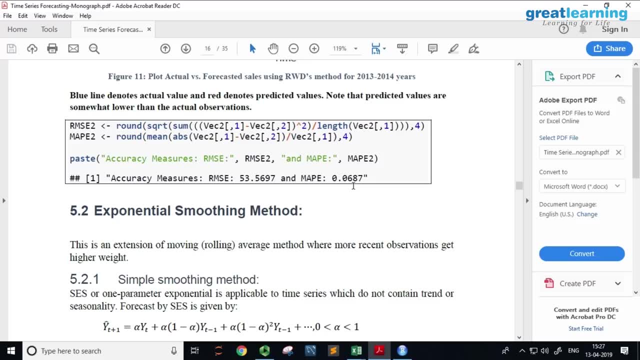 absolute percentage error is about seven, seven percent in my previous model. so the random walk model, this is 53 and this is point zero six. so in a root mean square error sense my exponential smoothing model is better, but in an in a percentage error sense it's a little worse. in a percentage error sense this is a little worse. this is. 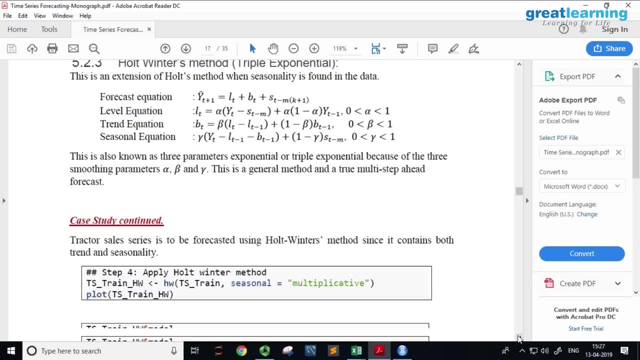 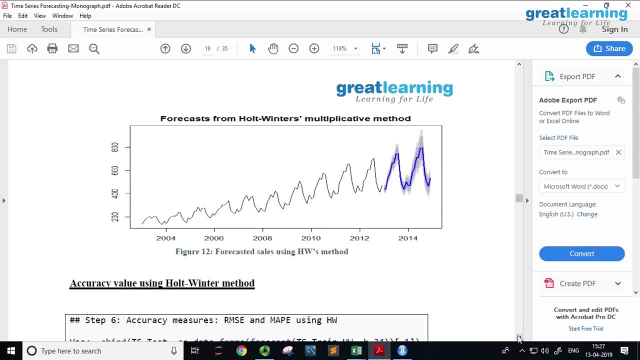 not surprising, because remember what these models are trying to do. these models are trying to fit outside the data set. Now, when you look at the data set, Now when you look at the data set, When you fit outside the data set, what are the things that could potentially go wrong? 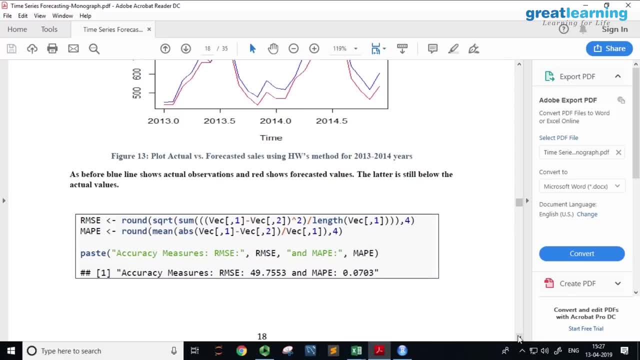 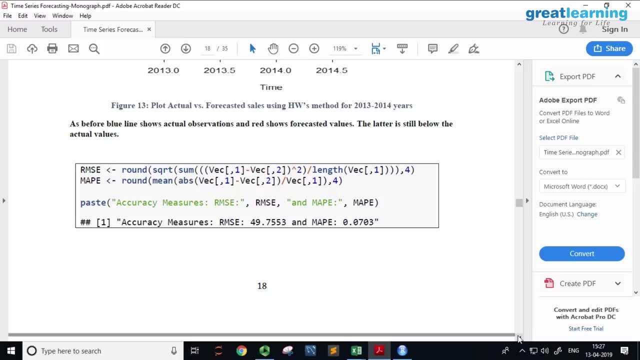 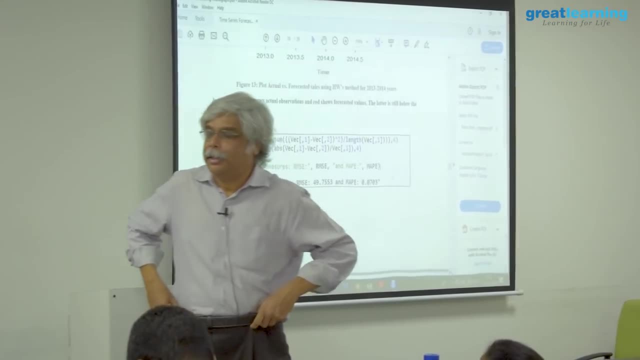 have you done a bias variance trade-off thing somewhere in some course? not, not, not yet, not in detail, etc. so it's not a neural network idea. neural networks are often used for it. it optimizes bias, but the bias variance trade-off is this idea, the bias you have done. regression. 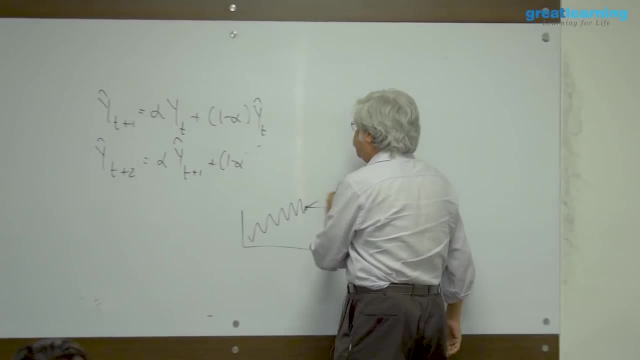 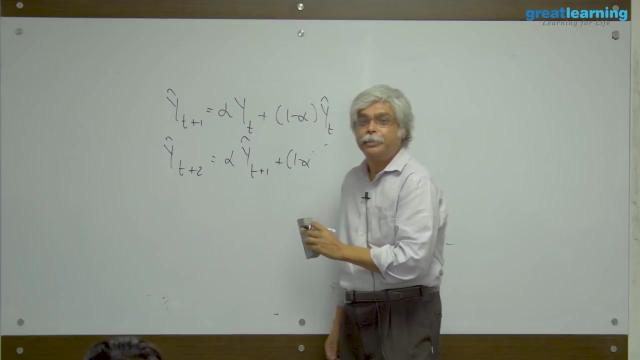 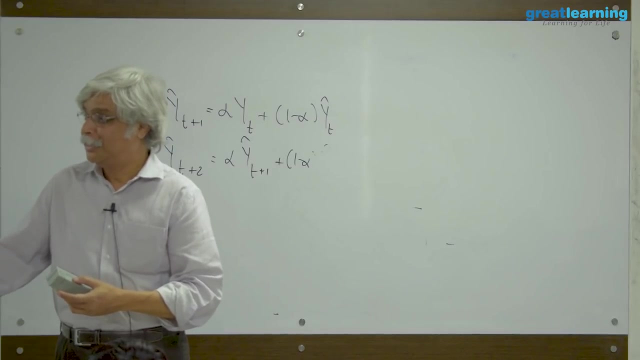 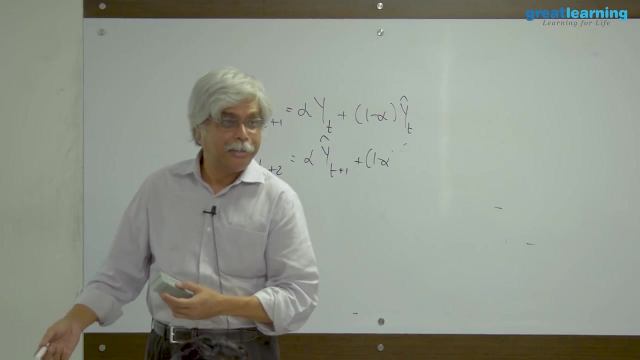 so the idea is a little like this, so suppose I want to. well, today you are building model, logistic regression models, very nice. so what were your Xs, your Y was what default or marketing right- positive things churn. and what was your X in income if you received an rfm right? so 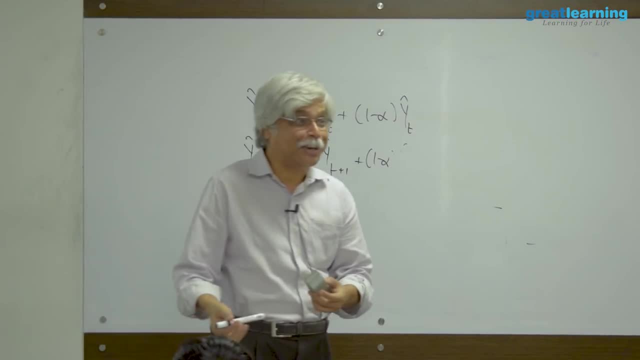 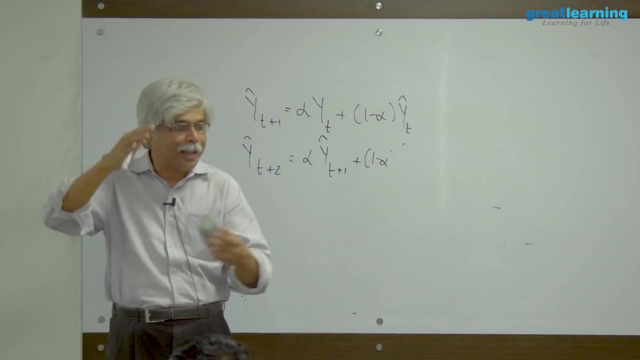 what's your what's your RRFM is yes. second, negative logistic regression models three: Recency can't be yesterday, so whatever. so there would be. let's say, okay, I'm not going to get in. you know your marketing teacher space. 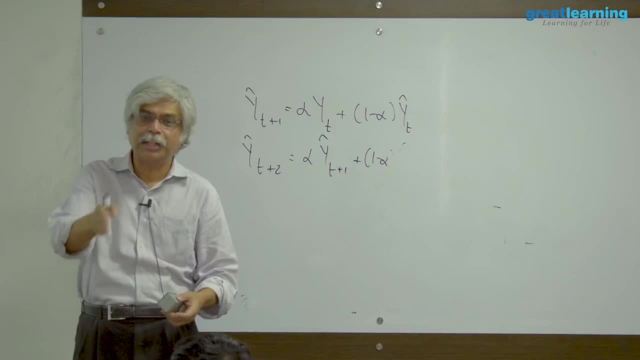 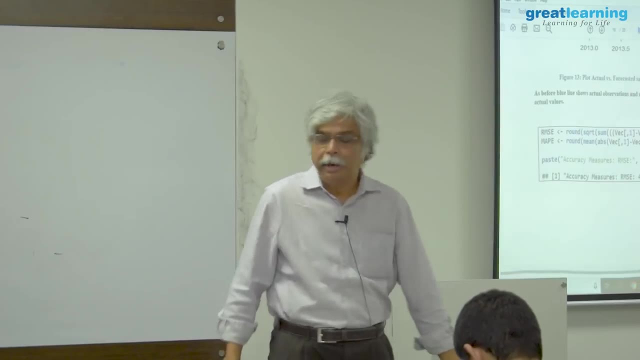 So there will be a recency value vector and there will be a frequency vector and let's say, there's a monetary value vector. So you're trying to predict churn based on, say, three predictors. Now let's suppose that it's going to cost you money to get those predictors. 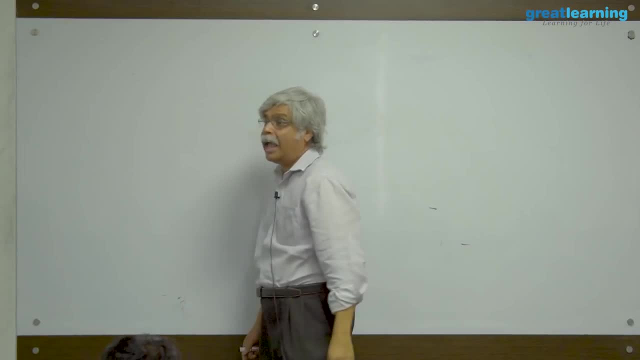 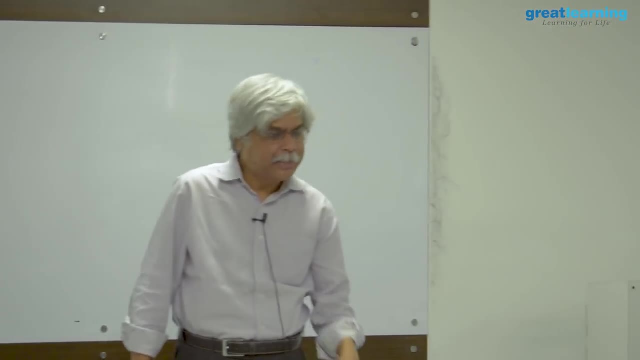 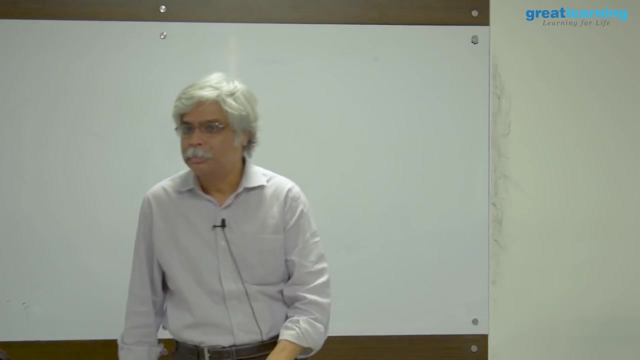 And you're asking yourself the question: what will happen if I use one less predictor? So I know that my right model has three predictors, But I'm asking the question: can I get away with only two? What will go wrong, What will go right and what will go wrong? 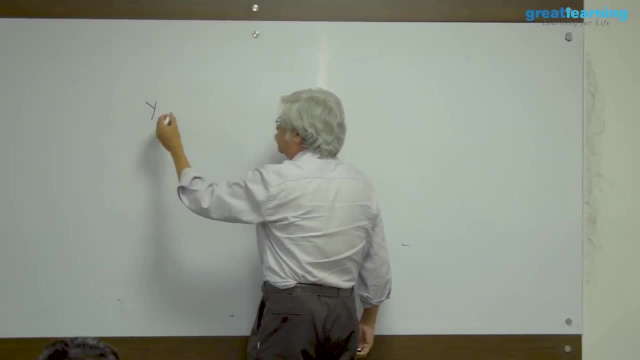 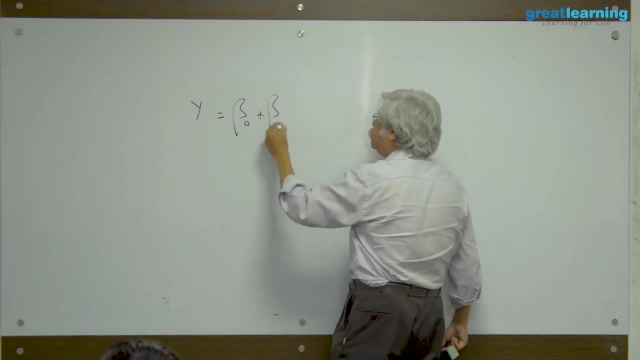 So okay, So now I have a model. Now this is in regression terms, not in your logit terms, Or I can do it in the logit. No, I confuse things. So beta naught plus beta 1 x1 plus. 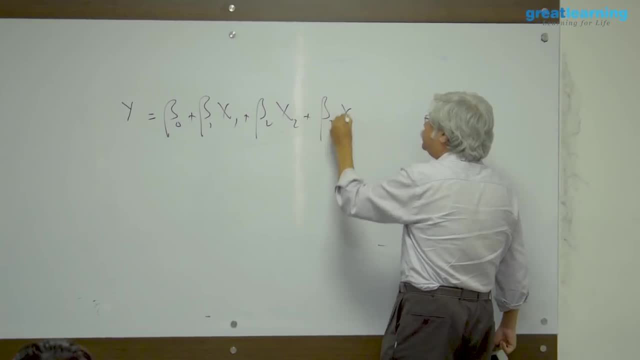 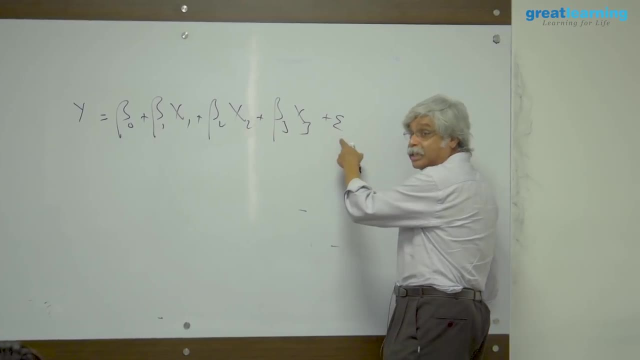 Let's say beta 2, x2, plus say beta 3, x3.. Correct, This is an equation. Where did this equation come from? This equation came from? Well, originally you began with this. There was an error, And then you said: let me minimize this error. 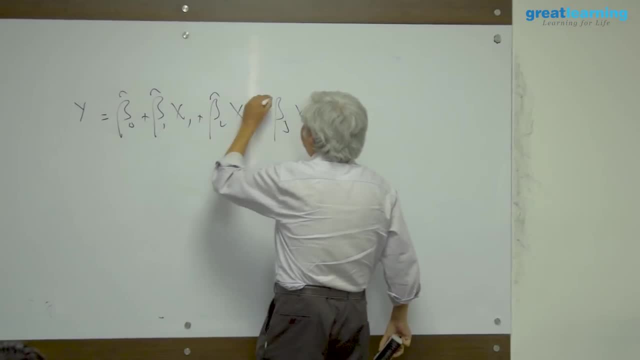 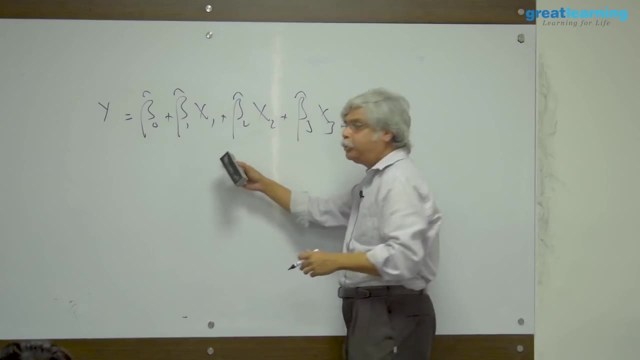 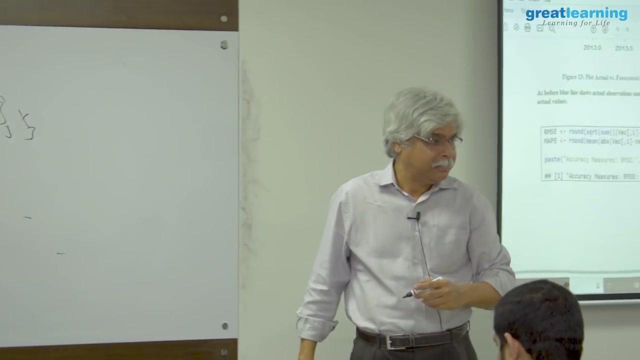 Okay, Subtract of the epsilon and put a hat in. This is my forecast formula. This is my forecast formula. Now, what I'm asking is what happens to this forecast formula if I ignore the third term? Is that a good thing or a bad thing? 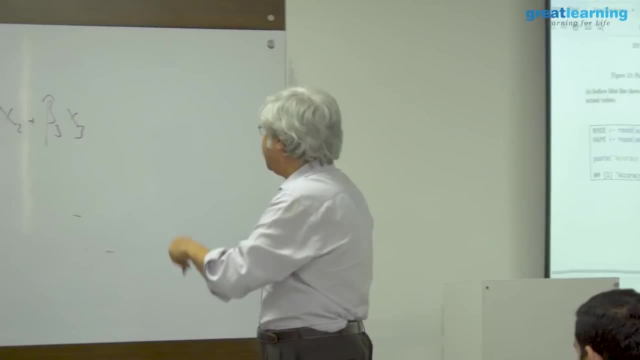 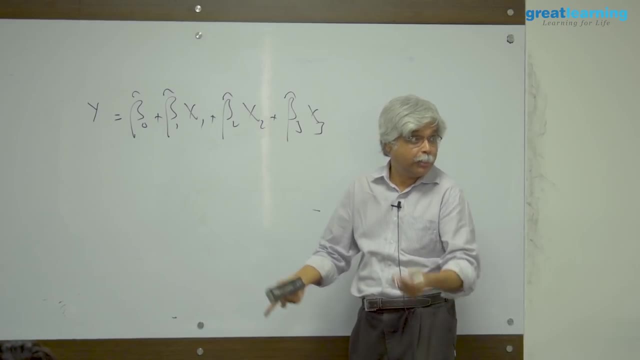 Depends on Ah depends on how significant it is. So if beta 3,, for example, is 0, I can throw it away No loss. That's variable selection. Why you do hypothesis testing, Why that whole p-value stuff exists in logistic regression. 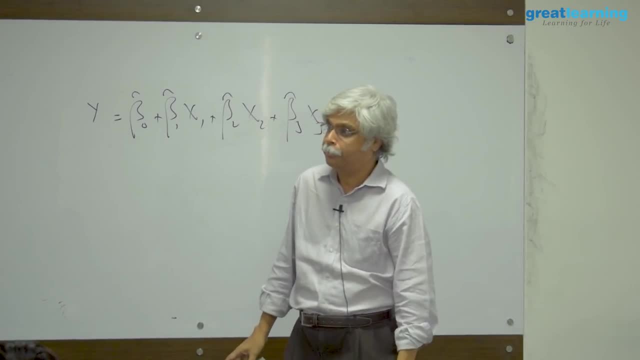 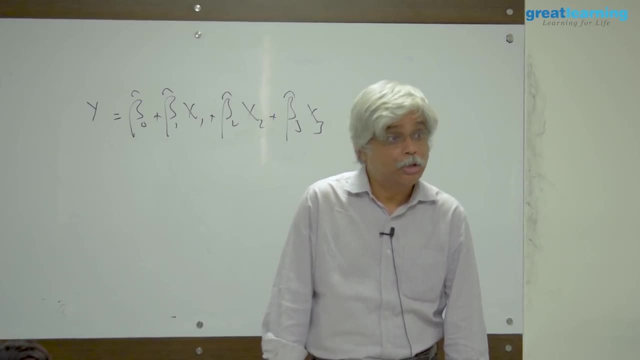 If it's 0, you can throw it away in a consequence-free way, But let's suppose it is not 0.. Let's suppose it is not 0.. If it is not 0, what's going to happen is you're going to generate an incorrect forecast, shall we say. 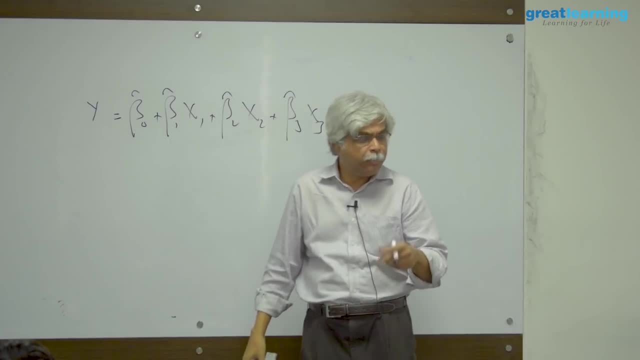 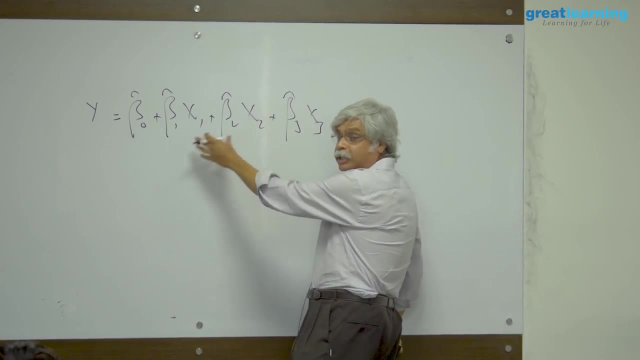 In other words, you're going to generate bias. Your forecast will be biased Because you removed this. If it was correct with this term, then without this term it is going to be, let's say, incorrect, Either large or small, depending on the sign of this beta 3.. 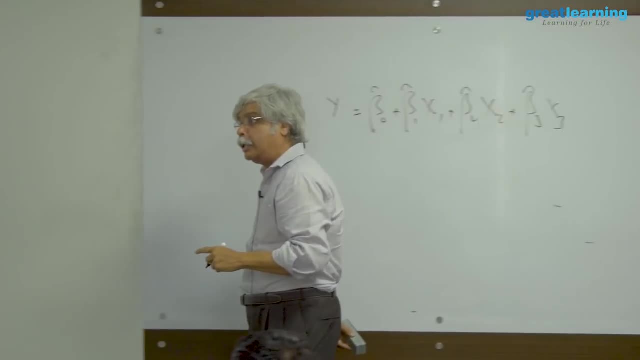 However, now I'm going to make things a little complicated. I'm going to say that this is all bakwa statistics anyway, So I'm not going to allow you to give a forecast. I'm going to force you to give a forecast plus minus an error. 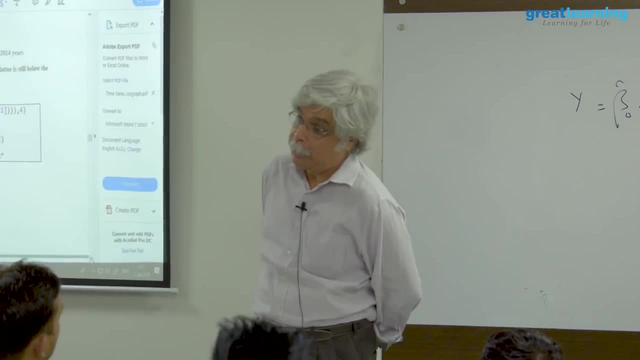 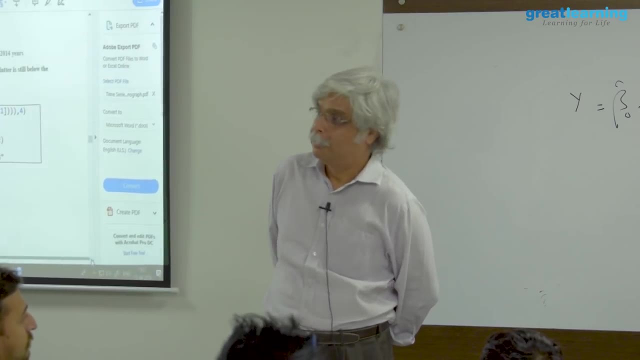 You're not allowed to give me a number. Your number is wrong anyway. Whatever you do, your number is wrong. So don't give me a number. please Give me a number plus an error. So now what I need to do is I need to calculate what the variance of, let's say, y-hat is. 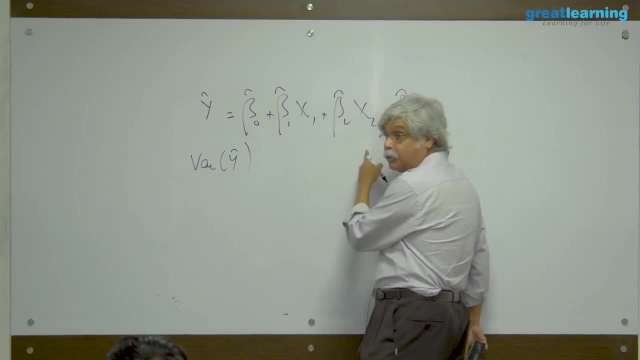 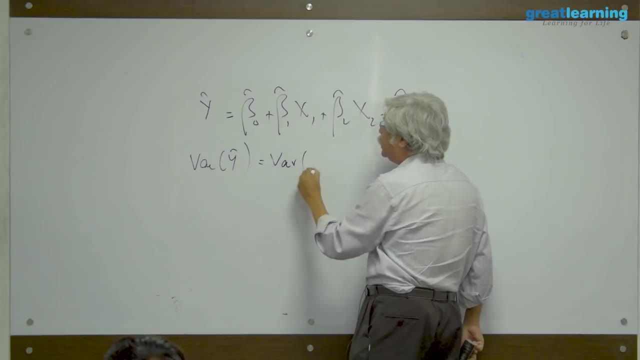 Now the variance of y-hat is going to come from where The variance of y-hat is going to come from. the variance of this thing Now. where is the variability of this thing? The variability is here Now. so now I'm going to calculate the variance of all these things. 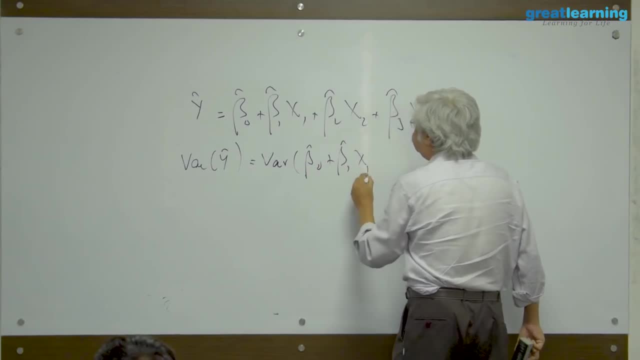 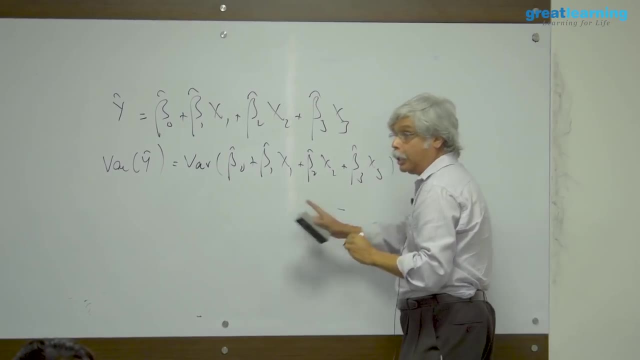 Let's say the variance of beta naught hat plus beta 1 hat x1 plus beta 2 hat x2, plus, say, beta 3 hat x3.. I'm making a very simplified assumption. Now suppose I ignore this, What will happen to the variance? 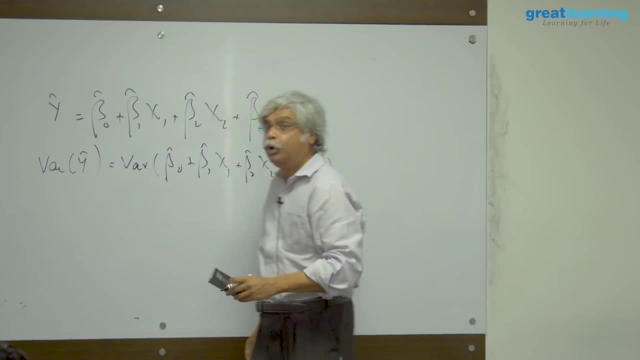 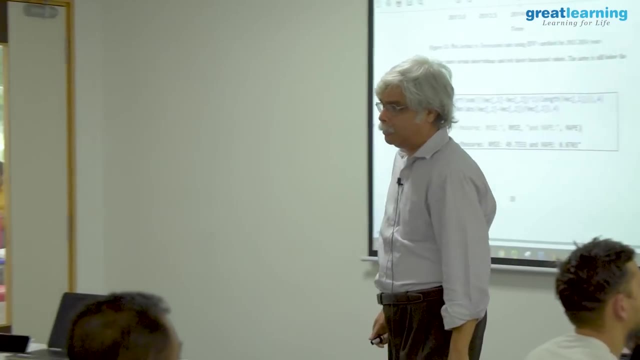 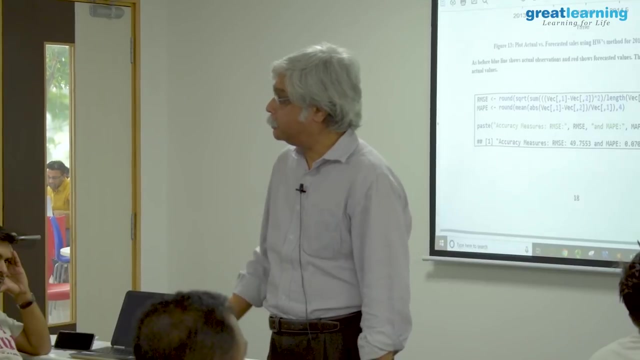 The variance will. unless it is very peculiar, the variance is going to come down. Yes, Y is going to come down. Why? Because there is less uncertainty in the prediction. So when I use fewer terms, I predict the wrong thing, but I predict it better. 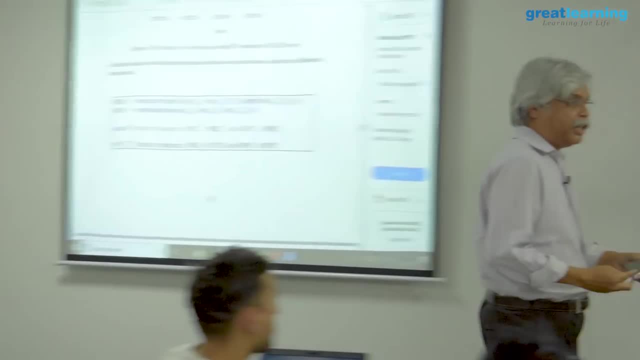 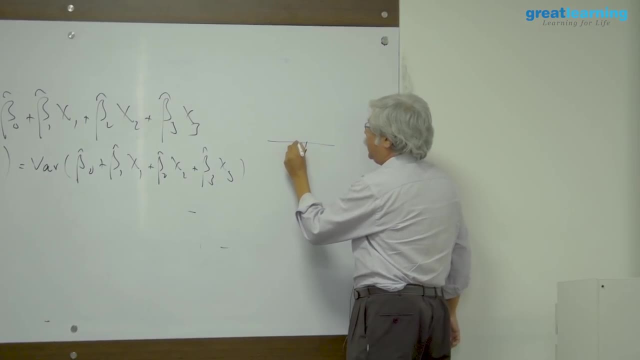 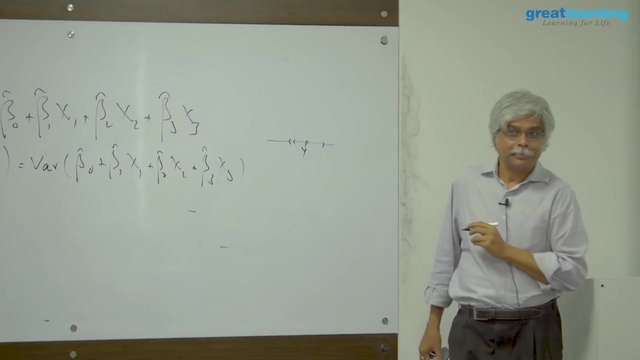 So I'm left with a solution that when I do a prediction- and this is my actual point- let's say my y, which is a better forecast. Is this a better forecast Or is this a better forecast? The second one is a better forecast. 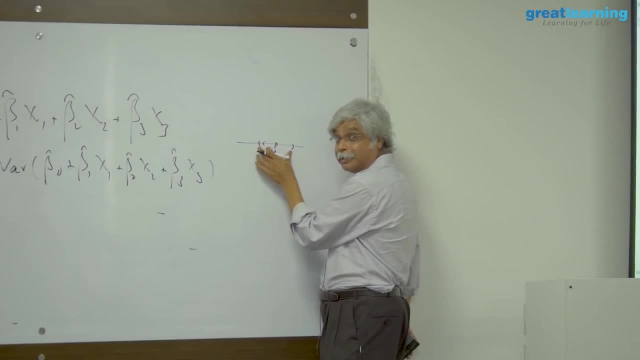 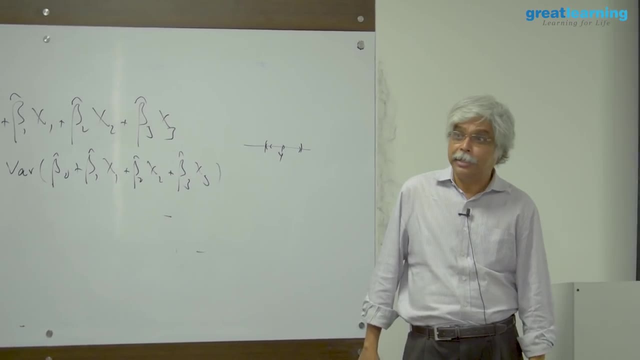 Because the y is inside it. but the second one is a much bigger number. It's a bigger range. He's going to be even unhappier, And he's right. We want a small range for the forecast to be useful, which means we want smaller variance. 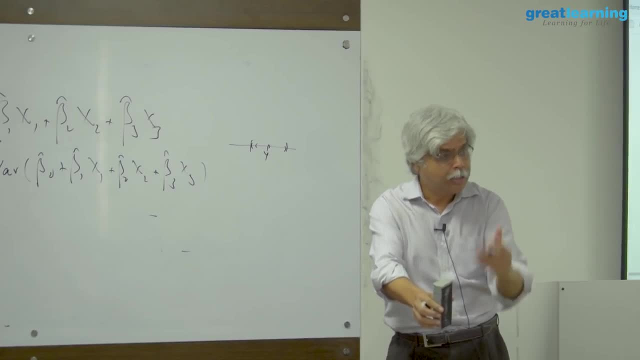 But the way to have a smaller variance is to have less uncertainty in the model. And the way to have less uncertainty in the model is to have less things. So you have less things estimated. but as soon as you have less things estimated, you're not estimating correctly anymore. 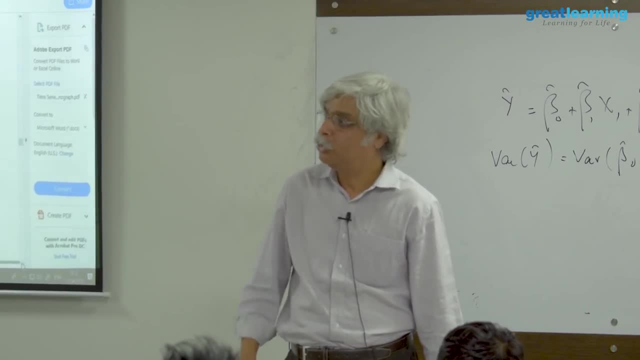 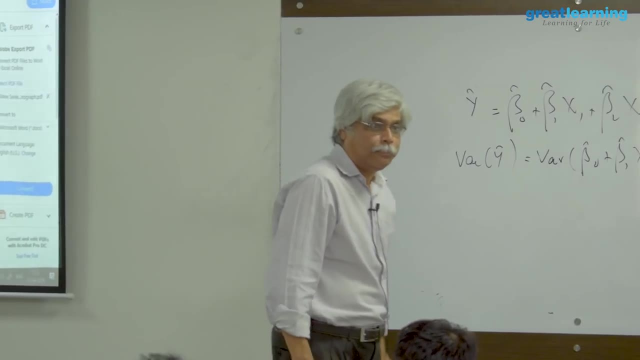 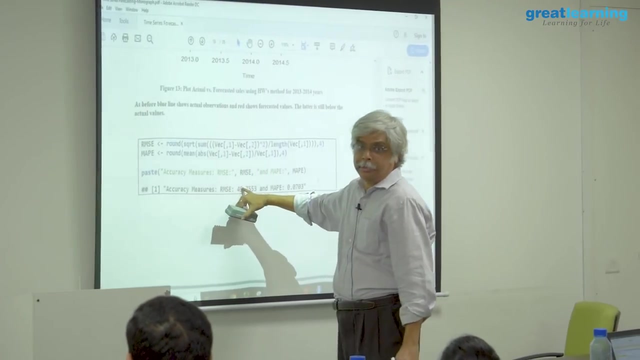 You must have seen this before in some course, somewhere, in some capacity. It shows up everywhere, Right? So this is the bias variance trade-off. Now, to some extent, this RMSE tracks variance and this MEP tracks variance. So this is the bias from purely analytical perspective. 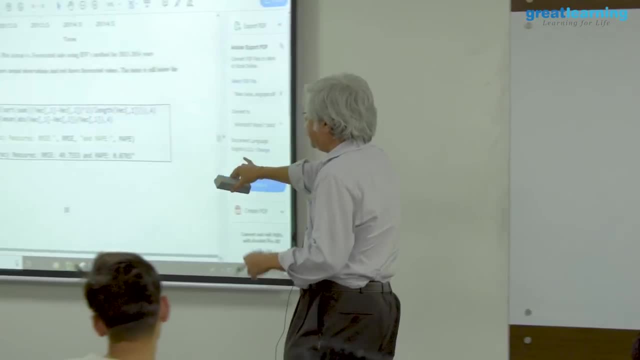 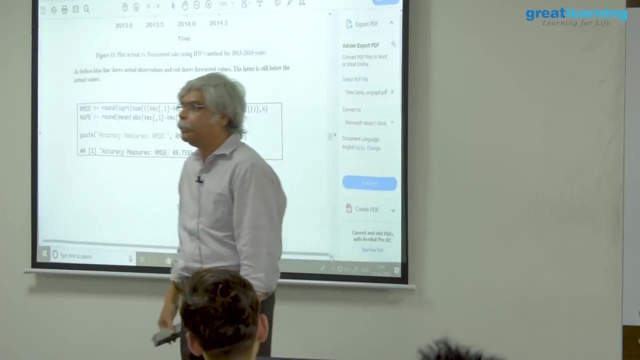 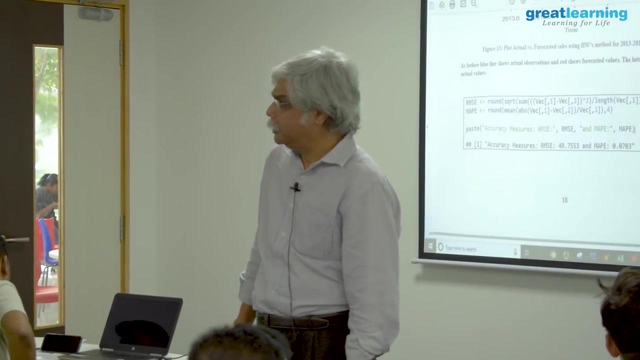 So this model is better than the random walk with drift model in a variance sense, But it's slightly worse in a bias sense. That doesn't mean it's worse. There's a trade-off. There's absolutely a trade-off. In fact, this trade-off has a formula. 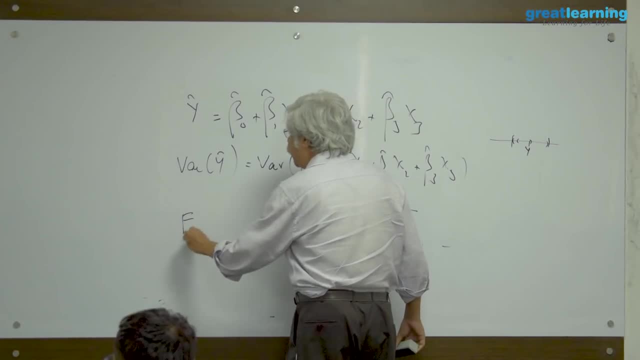 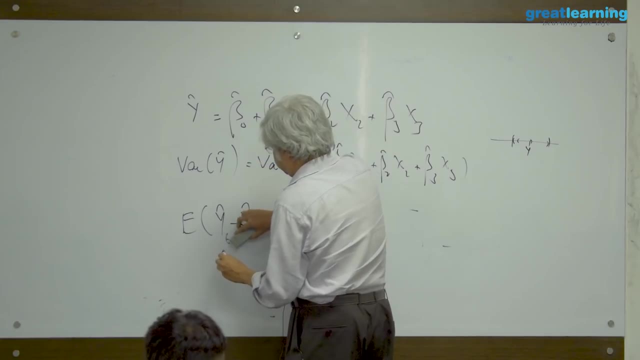 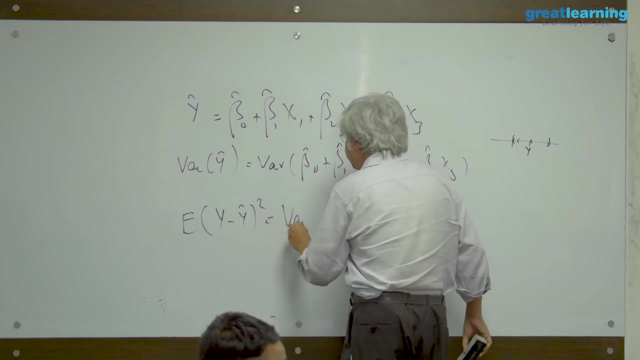 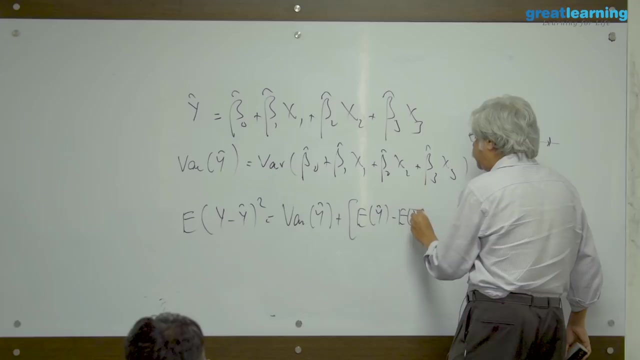 The formula looks a little like this: Expected value of the actual minus the forecast. Say y minus y hat, Y minus whole squared is equal to the variance of y hat plus the expectation of y hat minus the expectation of y. In other words, this is variance and this thing is bias squared. 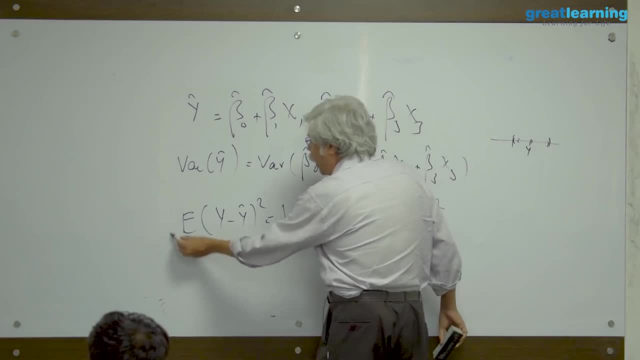 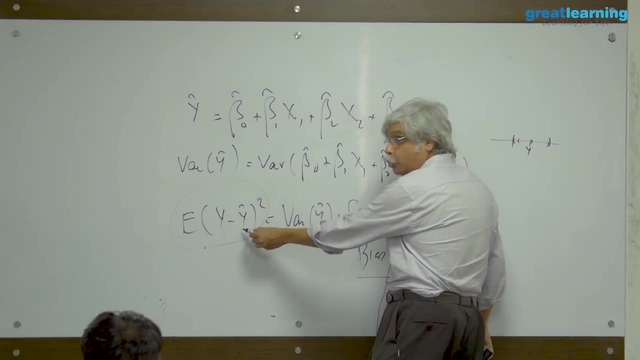 Variance plus bias squared, How far off I am from where I want to be is a sum of the variance and the square of the bias, And you can be close to where you want to be by either having small variance or by having small bias. 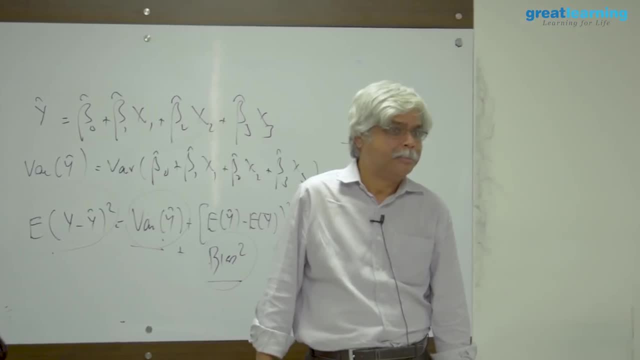 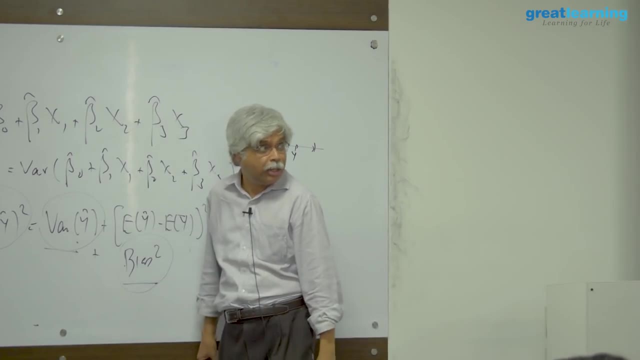 And it's very hard to have a model that does both. A big, complicated model tends to have a low bias and a high variance because of the complications in the model and the many parameters that it's estimating. Right, Right, Right Right. 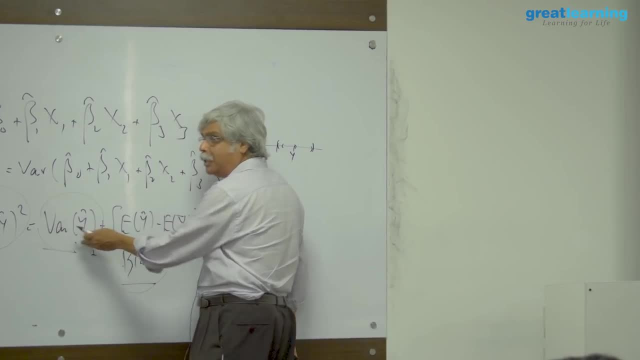 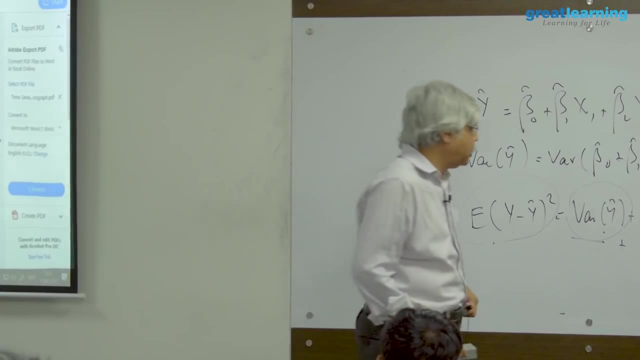 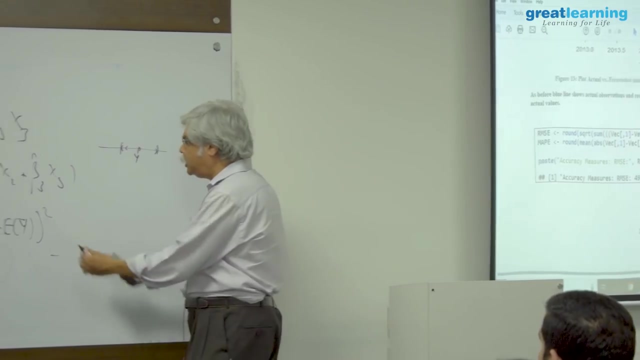 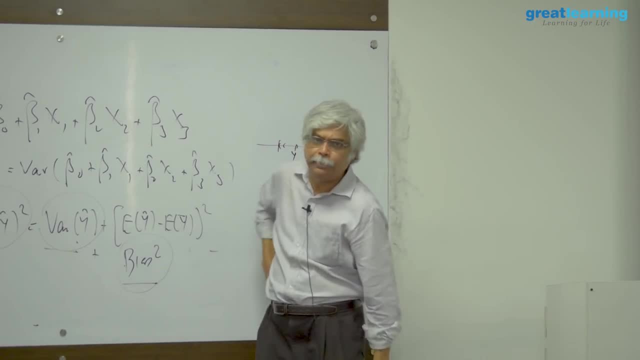 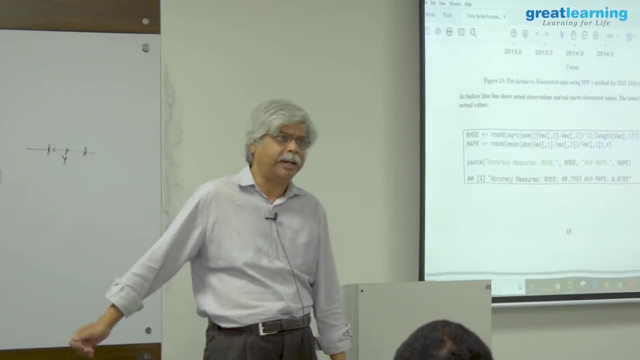 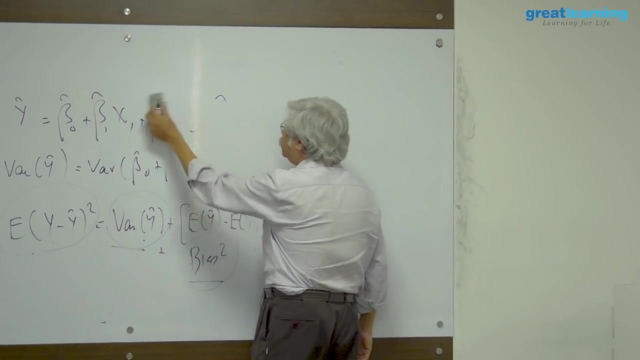 But this is just one illustration of it. There's nothing peculiar in this about time series. This phenomena exists in any kind of machine learning or analytical circumstance, Like regression, Like logistic regression. It's not a time series kind of phenomena. Yes, 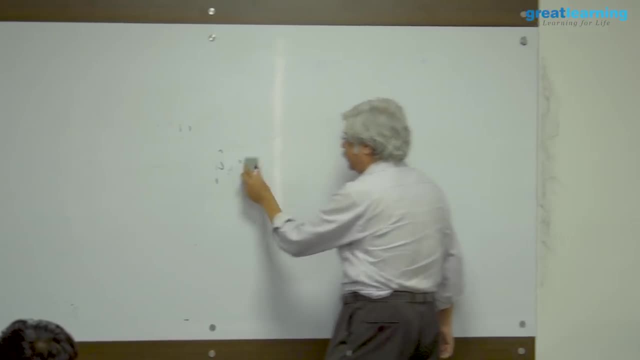 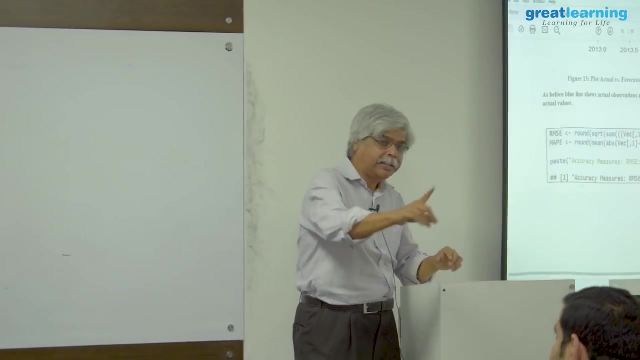 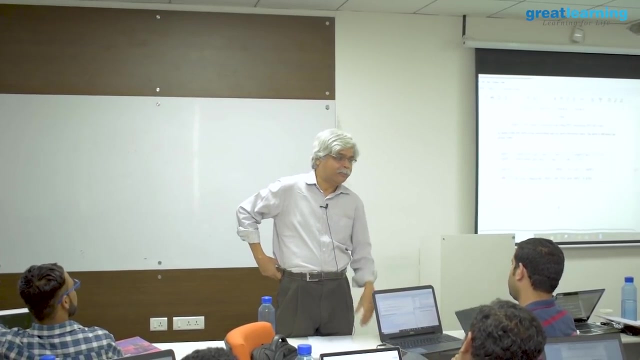 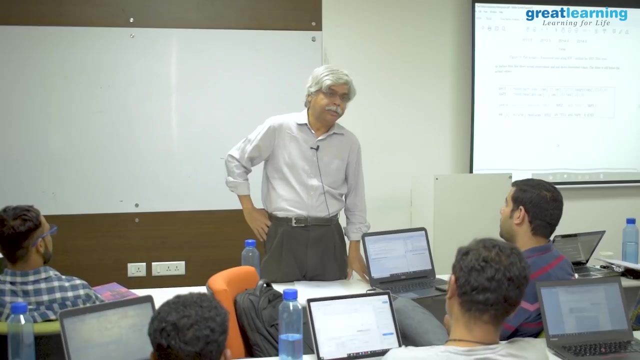 Every model handles both In a correct way, Not affecting this. So he asked an interesting question. He asked the question: why should I use simple exponential smoothing at all, Since the forecast is not doing anything? But how many parameters is the simple exponential smoothing using? 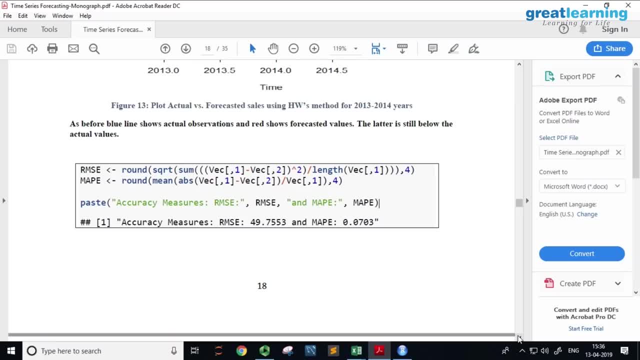 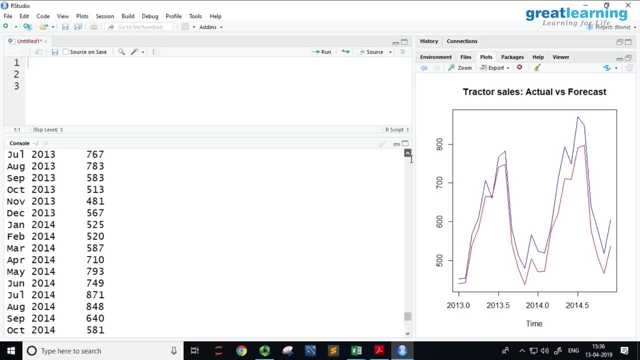 How broad is it? So let's go back here. So look at this number. So look at where am I. So let's go back and see the output of this. Here is my output of Holt Right. 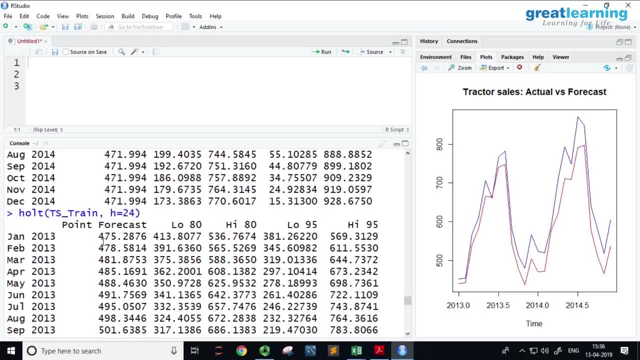 Now look at the forecast: 475.. Correct. Now look at the 95.. This goes from 381 to 569.. 381 to 569.. Now let's go back. This is my simple exponential smoothing: 471.. 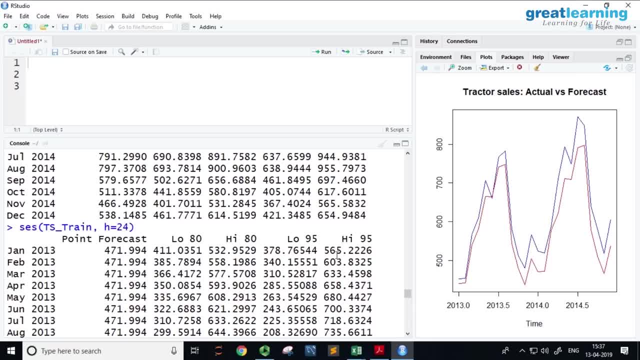 This goes from 378 to 5.. The simple exponential smoothing forecast is going to be better Almost always and invariably, from the more complicated model, Because the Holt model is doing better than the simple exponential smoothing model by adding complexity. As soon as it adds complexity, it adds uncertainty. 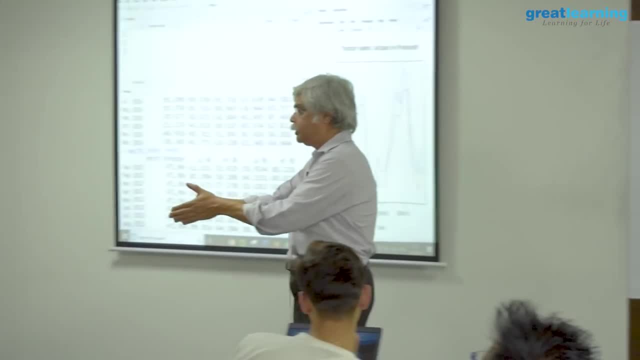 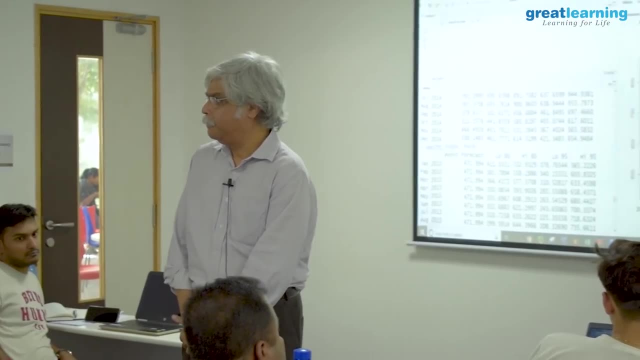 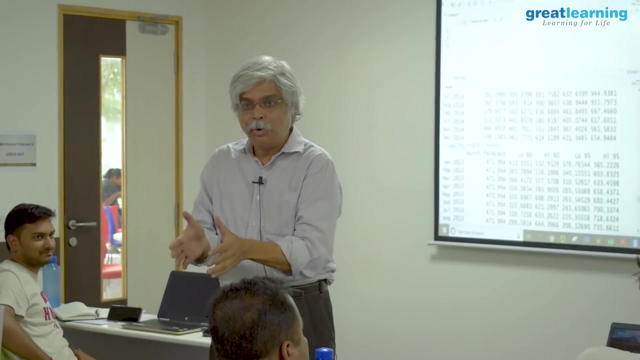 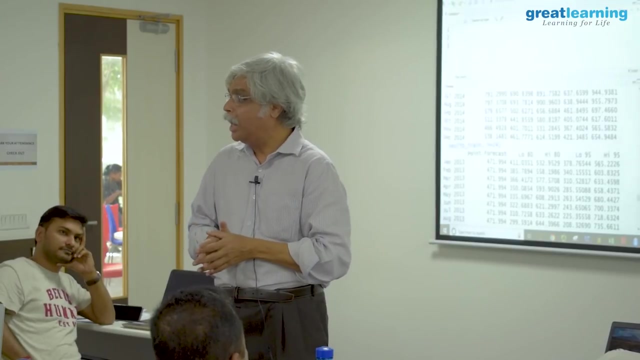 So As soon as you want a better forecast, you also get a more uncertain forecast. So the trade-off that you were asking for is a trade-off between seeing: do I want a narrow forecast or do I want a correct forecast? Do I want to do the wrong thing well or the right thing badly? 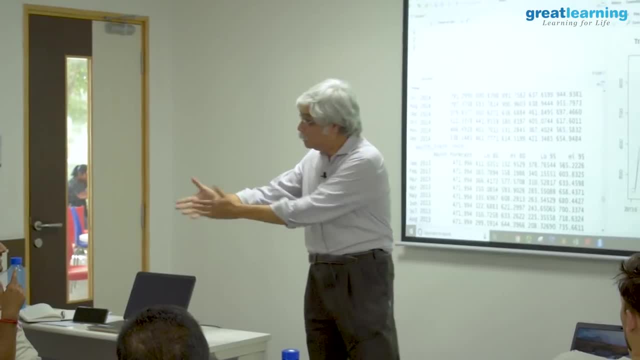 That's true. He is saying this is too much. I mean, you know, But in the middle there is a whole model sitting out there. in the middle there's a whole model sitting on there with the same problem you're going to see. 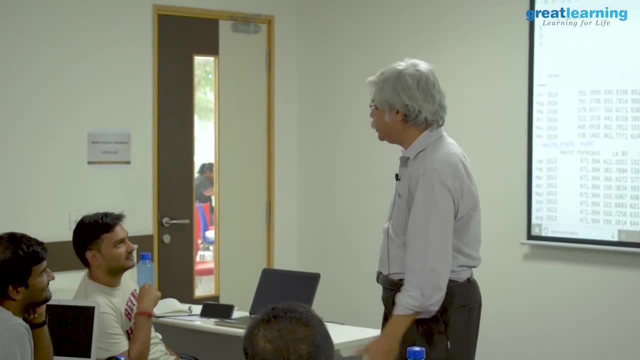 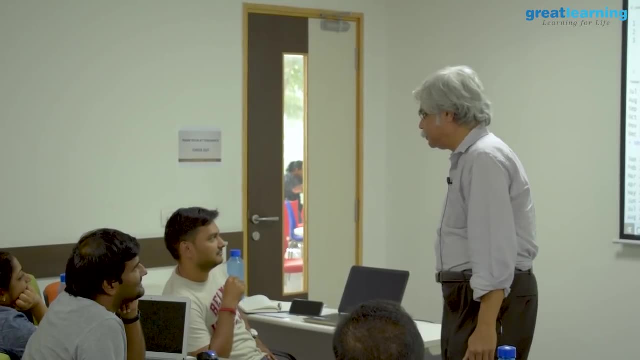 that is going to be a little better than whole. two enters from a variance perspective because it's not trying to estimate seasonality parameters. so it's going to be a little narrower, it's going to be a little more, you know, precise, if you want to put it that way. 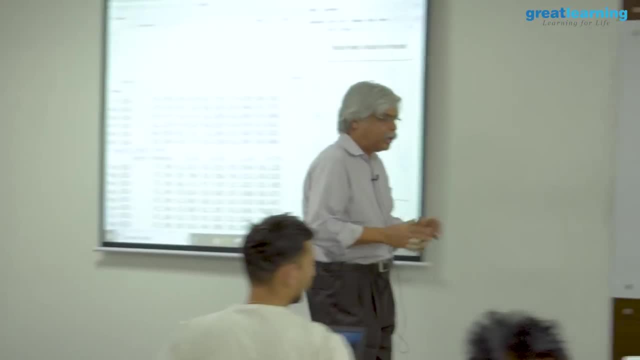 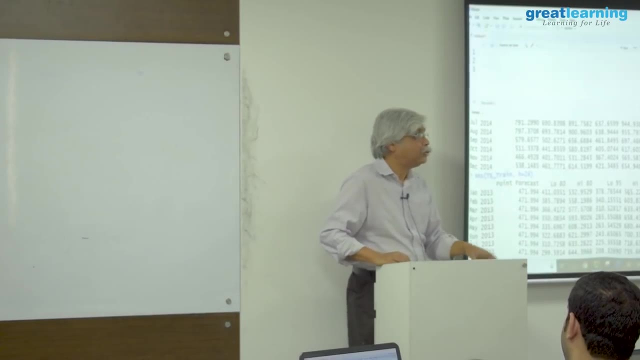 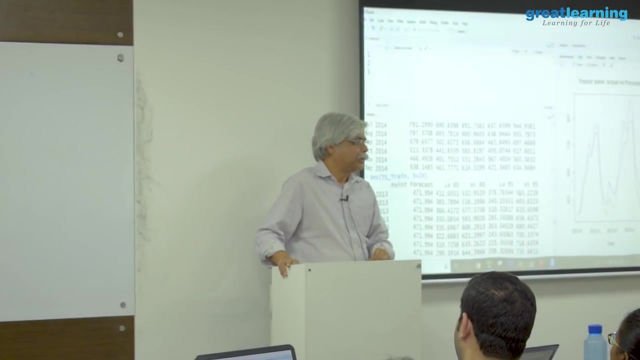 so in all these models, so now, in statistics, this is a hard thing to do, but in machine learning or the machine learning approach, this is an easy thing to solve. because what do i need to solve? i simply need to solve the, whether it fits well or not, and very often, therefore, what people do. 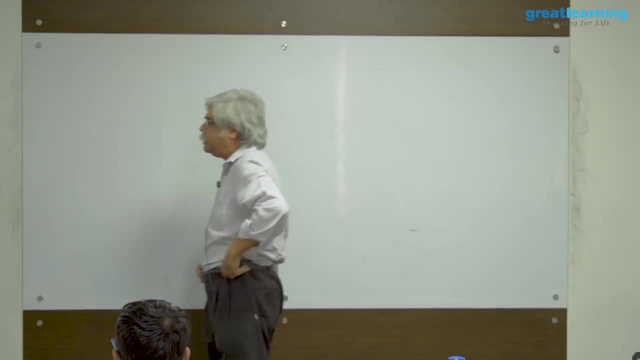 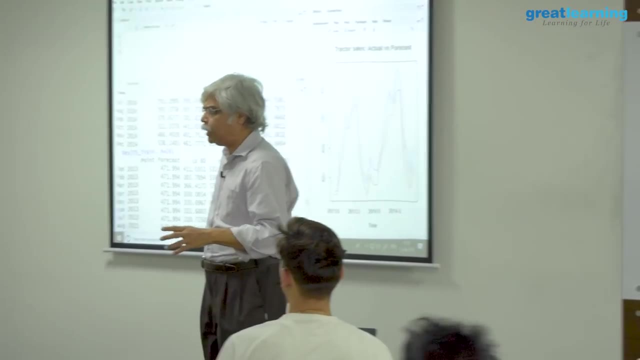 is people look at their criteria and say i'm going to look at mac, i'm going to look at map, and then i'm going to say i'm going to use one of these two things. both map and rmsc have elements of bias and variance. it says that rmsc tends to be a little more sensitive to variance. it's like 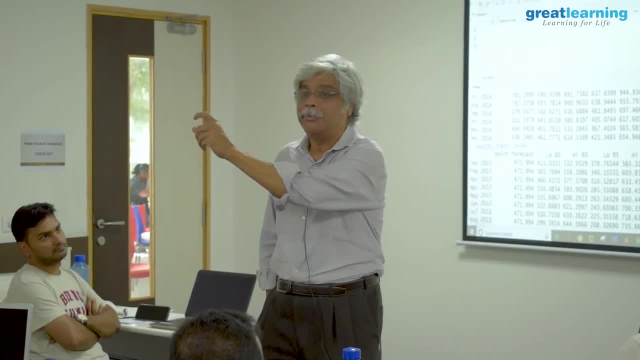 an error measure and map because it's like an a mistake in the forecast kind of measure it's like an error measure and map because it's like an a mistake in the forecast kind of measure tends to be a little more sympathetic to bias, but both of them carry the same thing and they say: 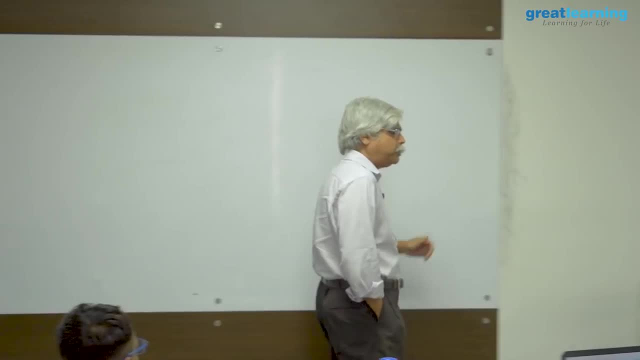 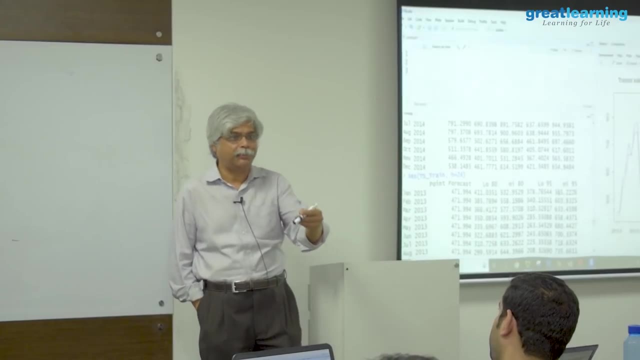 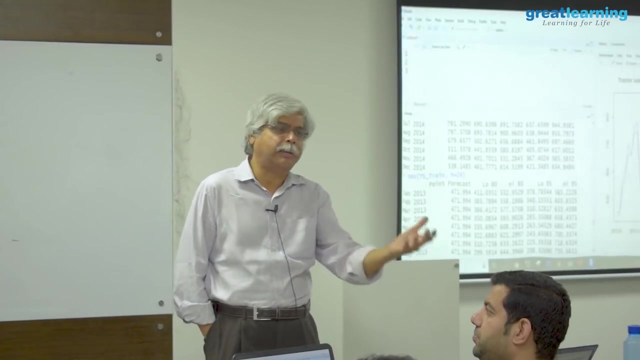 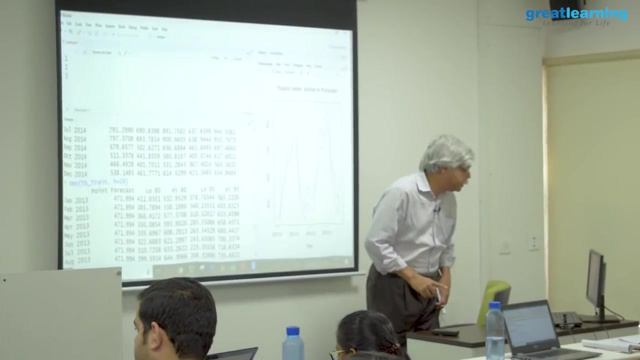 you figure out why the measure is right or wrong. just compare with the actuals. so the machine learning answer to this question is: figure out the right loss function, figure out the right measure of properness that you are comfortable with, what is acceptable. if rmsc is okay, then rmsc is okay, and not to worry about this too much in the statistical perspective. 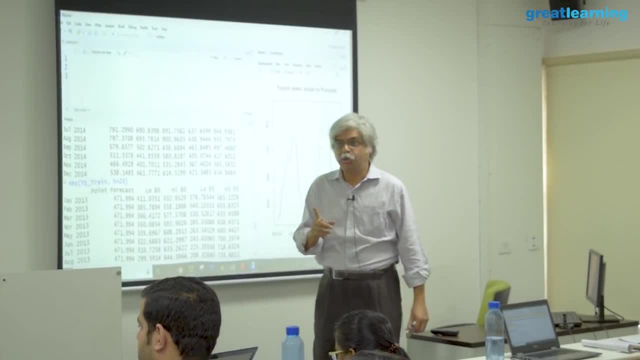 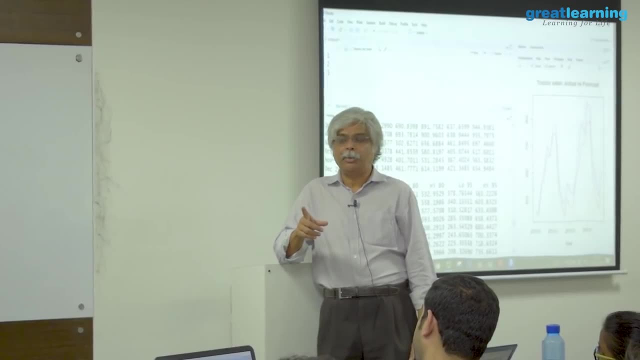 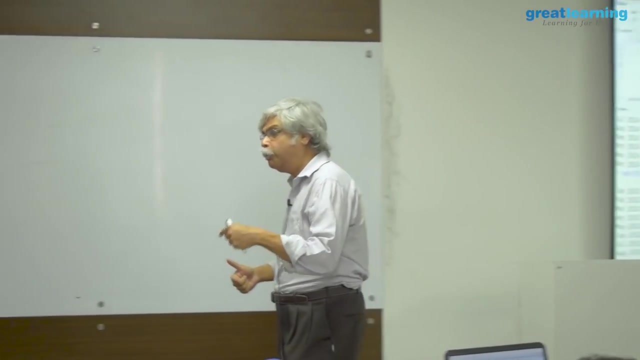 this is a hard question. for example, in regression you struggled with this and you used a notion called adjusted r square. adjusted r square does what adjusted r squares adjusts for too many parameters. now, why does it adjust for too many parameters? it says that if there are too many 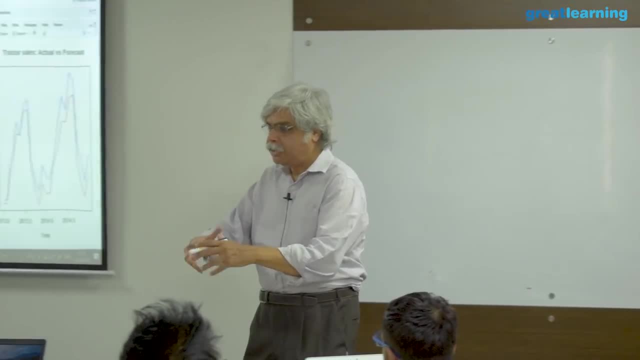 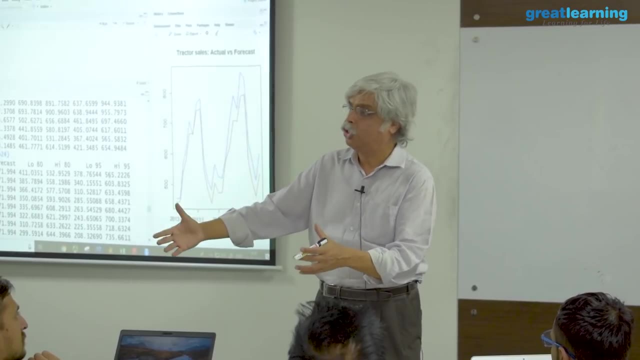 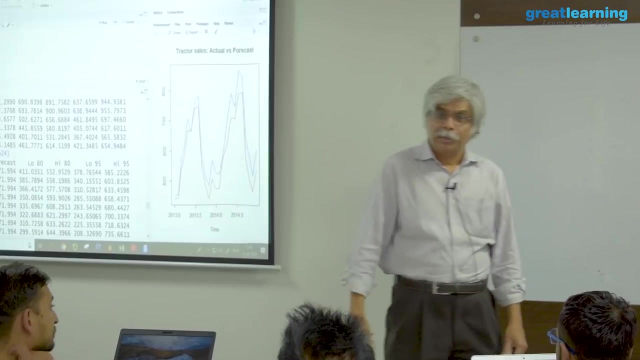 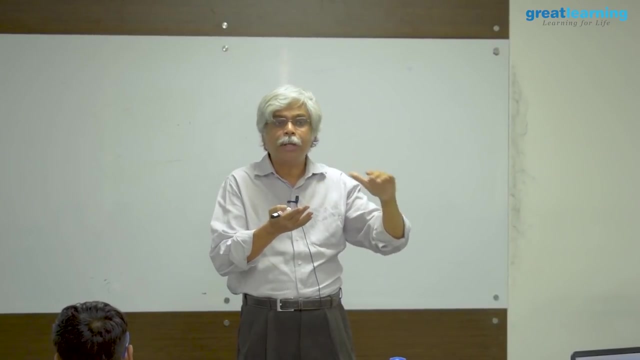 parameters i might over fit. in other words i'm the extra parameter is getting me more fit, but not enough compared to what one more parameter should do. in other words, it's a adding more variance but not reducing bias enough. so the criteria of maximum, maximum, adjusted r square sort of, is a comp, is a bias, variance, trade-off kind of compromise. 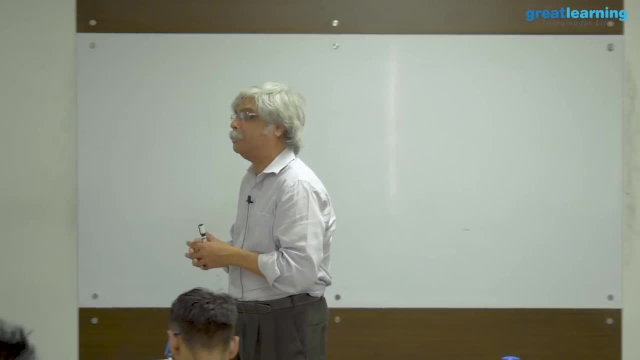 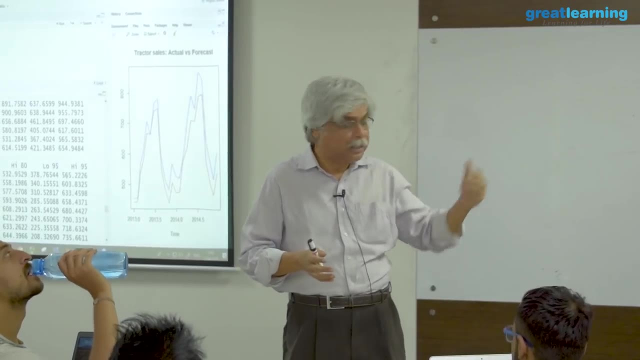 and statisticians do that because they do not have the test training principle to guide them. the guiding principle is a population sample kind of principle, but if you have a test training principle like this etc. then you don't need to worry about it so much. it's still there if you want this. criteria of aic is that? 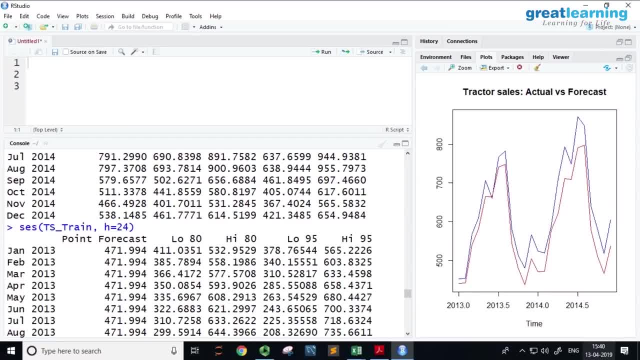 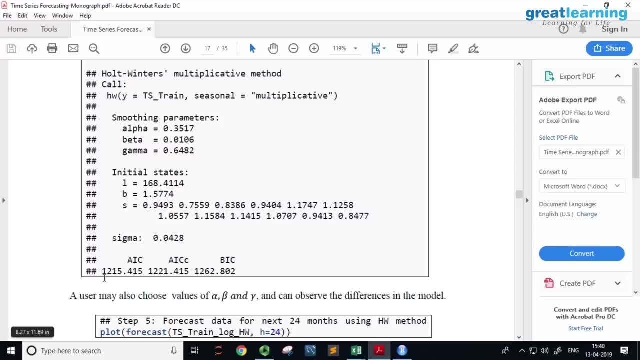 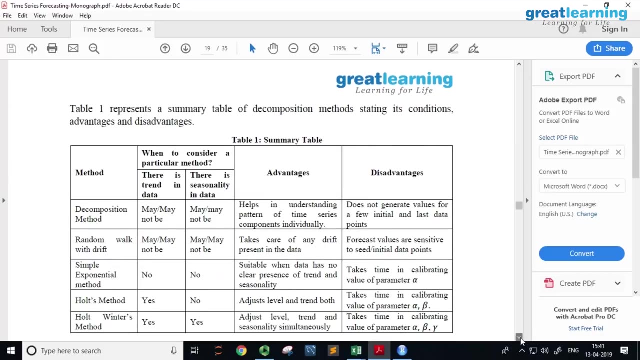 the aic criteria, that is, there is a criteria that is comparable to adjusted r square. this criteria is: is comparable- i'd comparable criteria to adjusted r square minus twice log likelihood. so the so lower values of aic are good. so here's a little table that kind of says that base of aic is that. 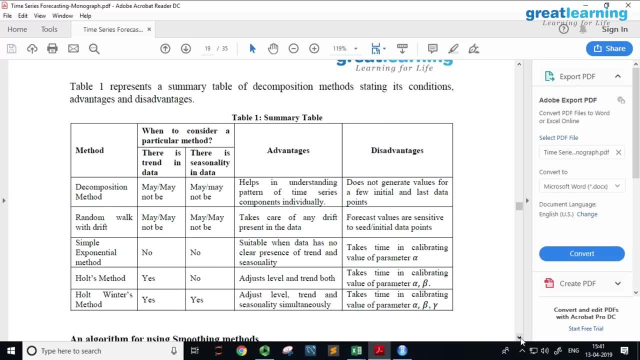 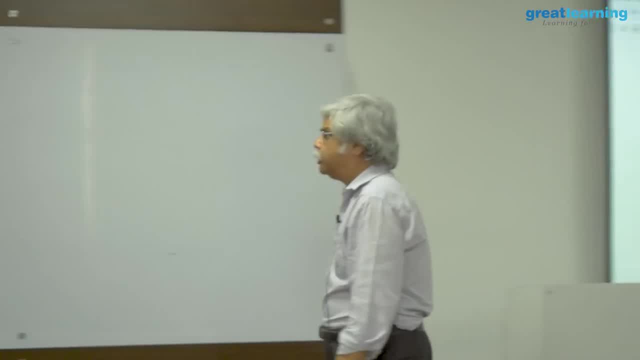 says that, based on all of these, what kind of forecast method can I use And use this table at your at your discretion if you want to? So you have got certain. you can use a simple straight forward decomposition and forecast. from that. You can use a random walk. 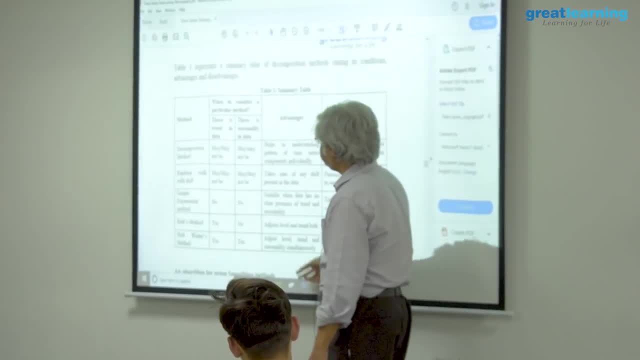 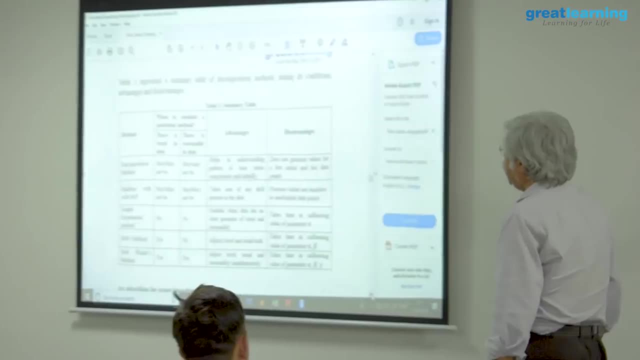 with a periodic drift, You can use simple exponential smoothing. Ask the question: is there trend? is there seasonality? Would you ever use simple exponential smoothing? Yes, if there is no trend, no trend Advantages suitable. when the data has no clear presence of trend and seasonality, There are some disadvantages. 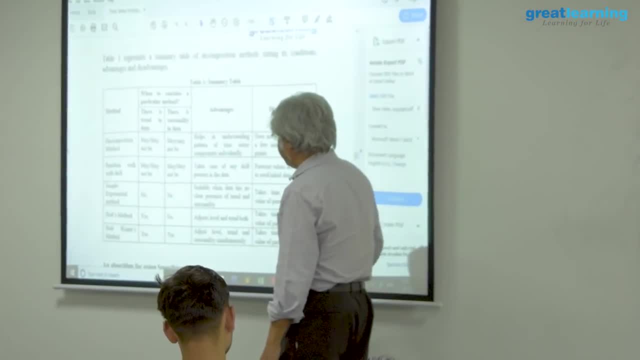 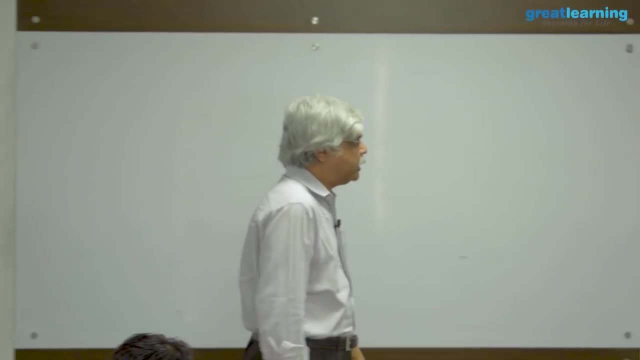 it takes time calibrating the value of parameter. In other words, it needs a certain amount of data to get this. well, So you can take a look at this and it gives a theoretical sense as to which of these methods would work. But the simplest proof of a proof. 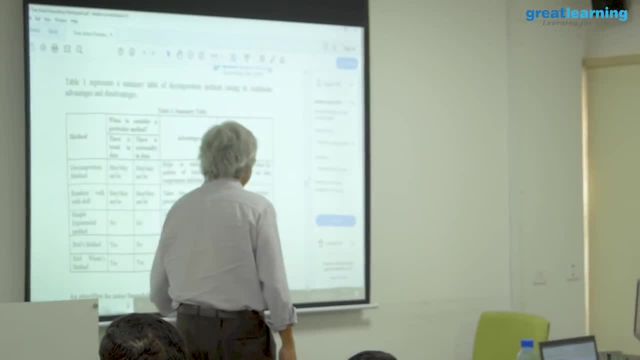 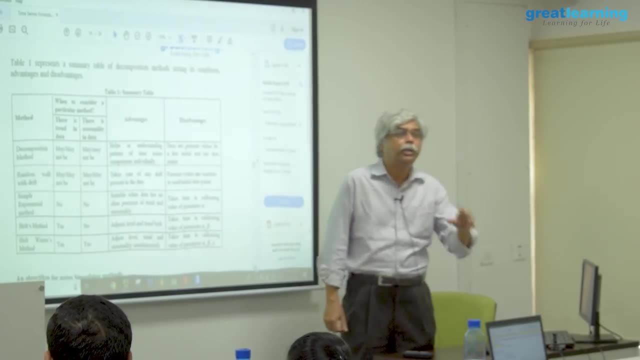 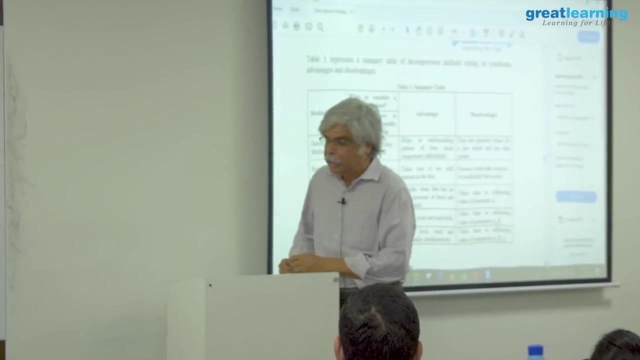 is in, just in doing it out. Run all these models and see, whether the from an RMSE sense or from an MAP sense. whichever one you choose, which of these models gives the best, which is which is true, which is true, That there is no real prediction required, So very. 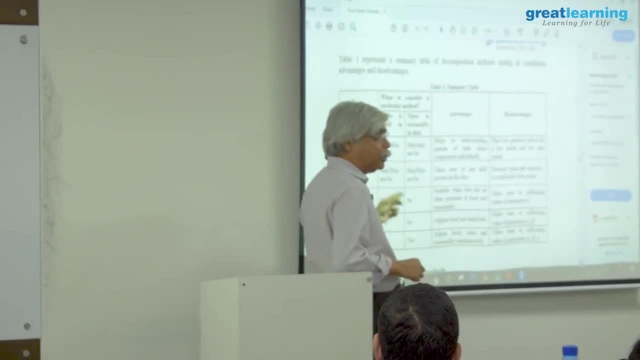 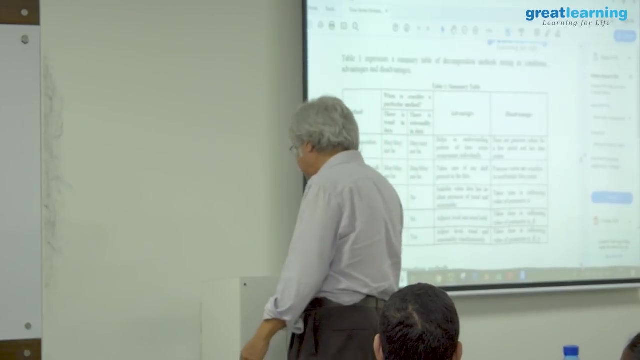 often this without a drift, in other words, random walk, for example, without that seasonality parameter or periodic parameter set, is something that does something very similar to simple exponential smoothing, In fact, a very crude version of that. Now, whether you should forecast such a series or not is something that is up to you. In other words, if you are seeing a series, 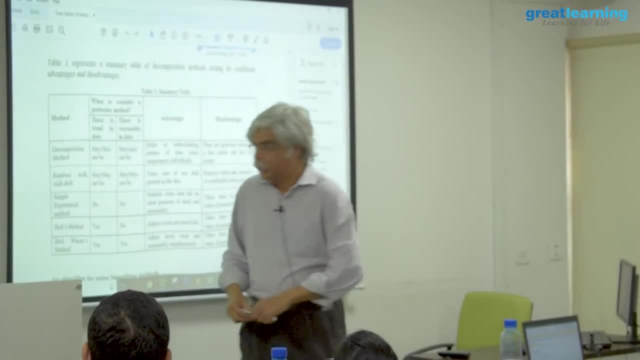 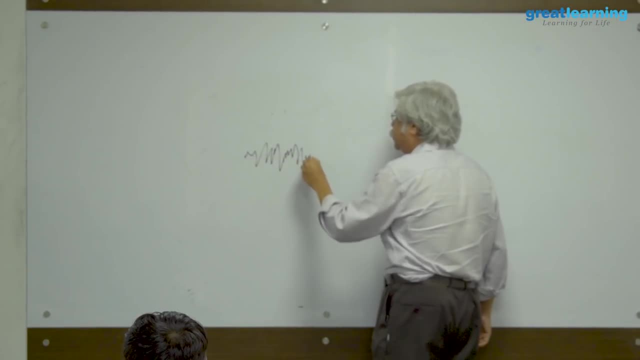 that is essentially random noise, In other words, a series that isn't showing much in it, Like we had done yesterday. So you know, something that just randomly moves up and down at different points in time. No seasonality- nothing I can't do. no seasonality- Humans when they do. 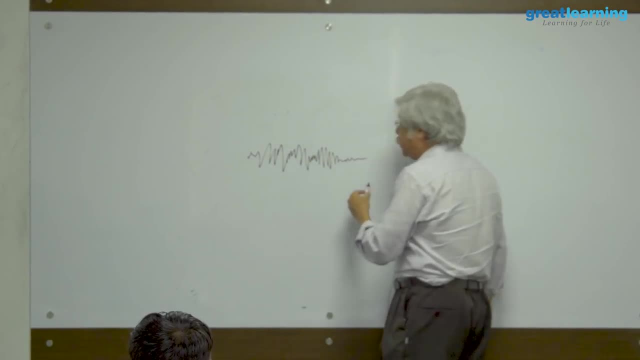 such signal, the hand goes up and down, which means seasonality. That's what seasonality is right: Something going up and down. So when you draw things, hand goes up and down, What to do? Seasonality happens. So, but if you have something, 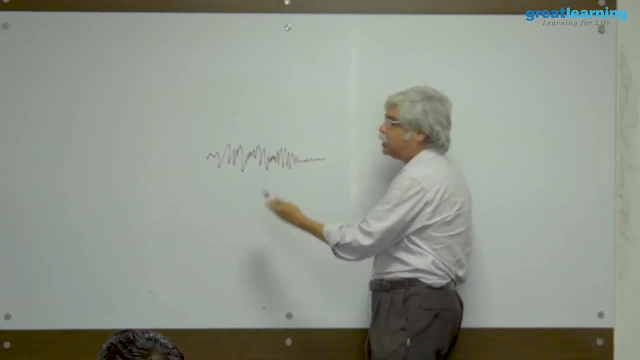 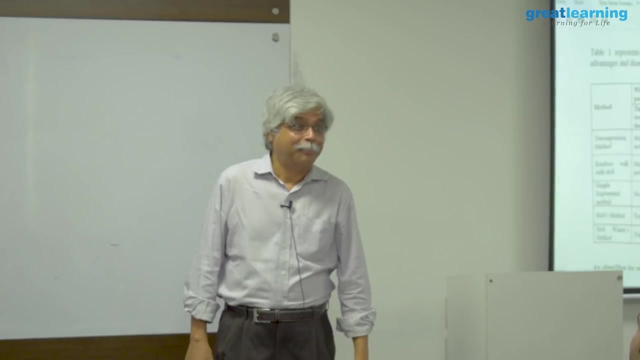 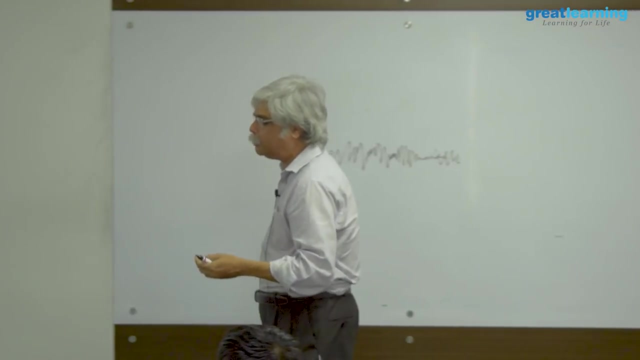 that looks like this and you want to forecast. Now, what would you forecast such a thing to be? Not Noise, But how do you forecast noise? But do you forecast noise or not? This is actually a very difficult thing to understand and it's not an easy problem. There's a 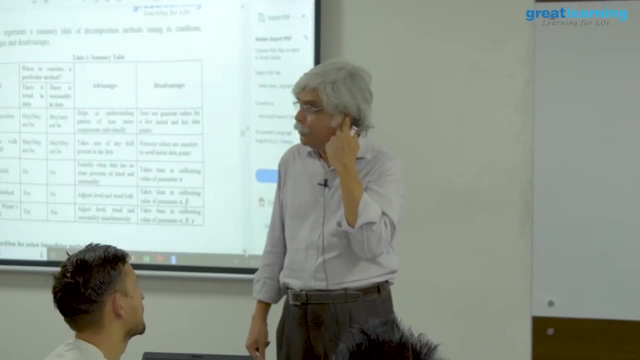 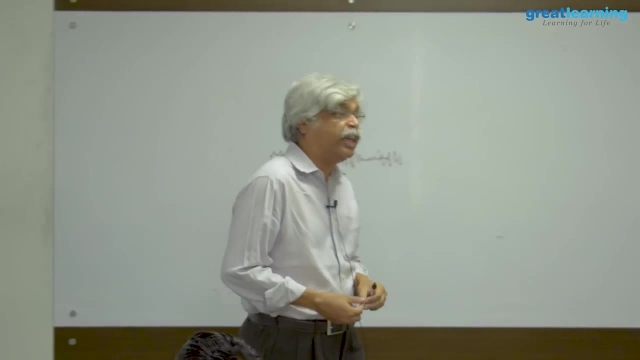 famous finance professor- He died many years ago, called Fisher Black. So if you do Black-Scholes pricing and things like that. So Black once wrote a paper, a very famous paper. He got awards for it. The title of the paper was just noise. 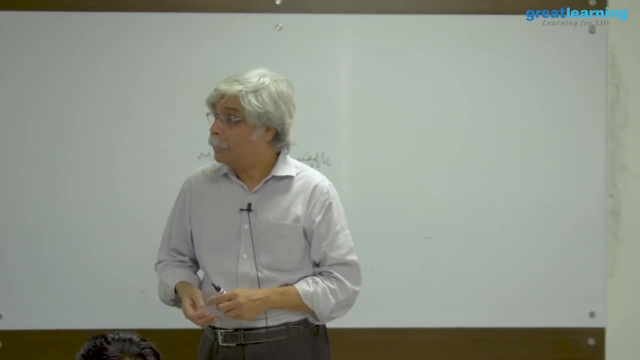 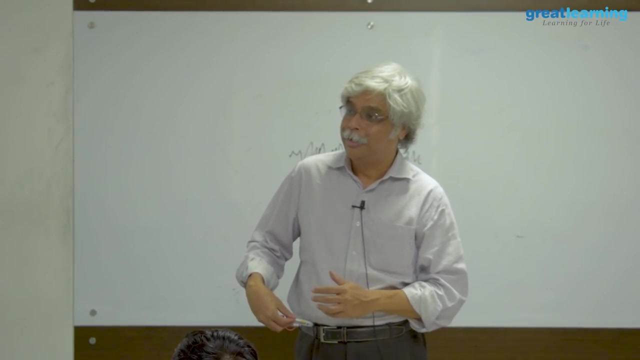 Noise. But in that paper he was talking about this. He said that when we do forecast we know we have to take noise into account, But do we forecast noise at all, Or do we say that noise is unpredictable? If anything is unpredictable, by definition. I cannot forecast it, Which means you are ending up with something that's pretty much flat, Which means the forecast is: There is no real forecast there at all, Which means why you are doing forecasting. So the question becomes increasingly trivial. 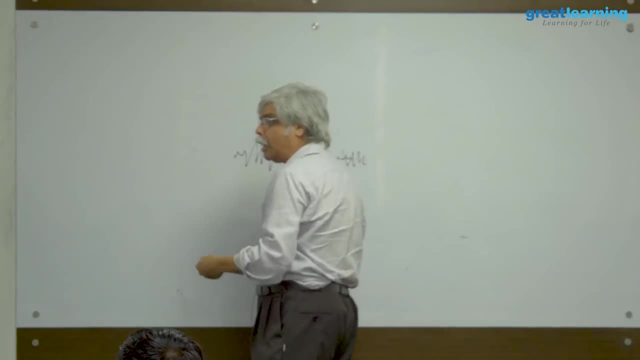 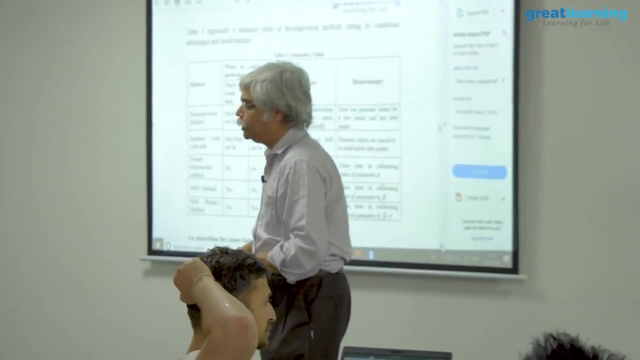 But you still left with this uneasy feeling that this is a series that is going up and down and that has you know that's things are happening to it and my forecast is that it's constant. that's. there's something disturbing about that. it's as if you are throwing. 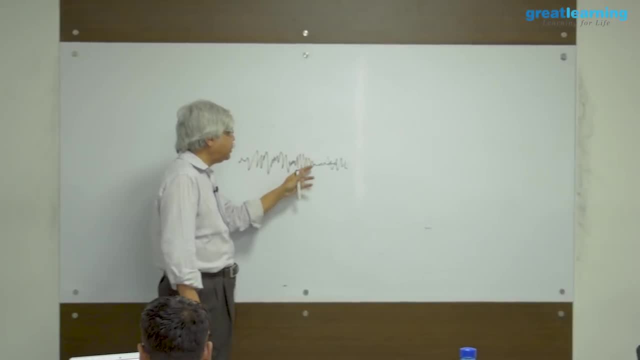 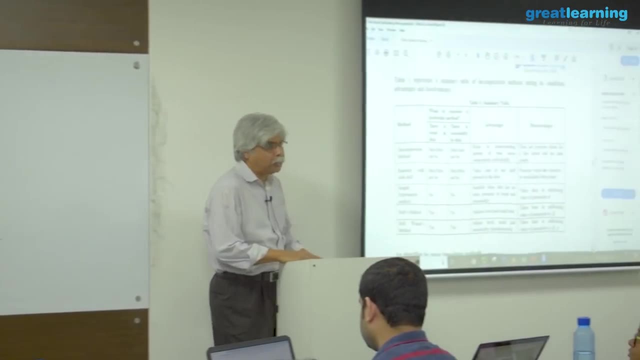 data away. it's as if you are not taking any advantage of the information that is present in this, and people do sort of do struggle with that idea a lot. many, many years ago, I collaborated in a paper in which what what we were trying to do was: 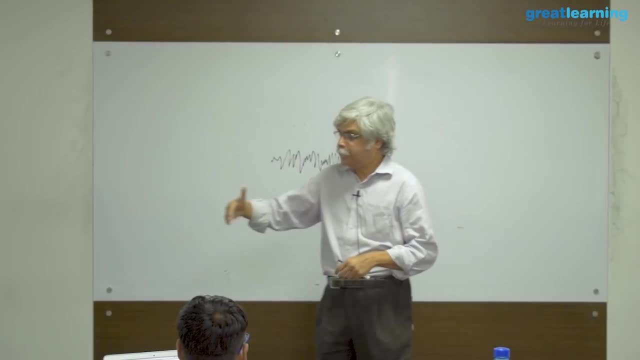 we were looking at stock prices data and we realized that the sort of the first difference in the logarithm, stock prices or log returns, they were stationary, but there was a, there was a pattern in the noise and we did that is, we found frequency diagrams of the noise. is it blue noise? is it high frequency? is it? 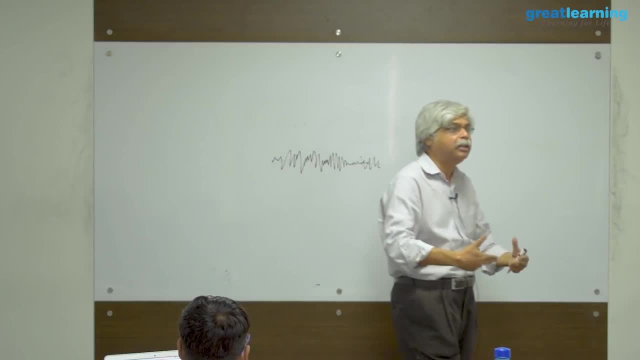 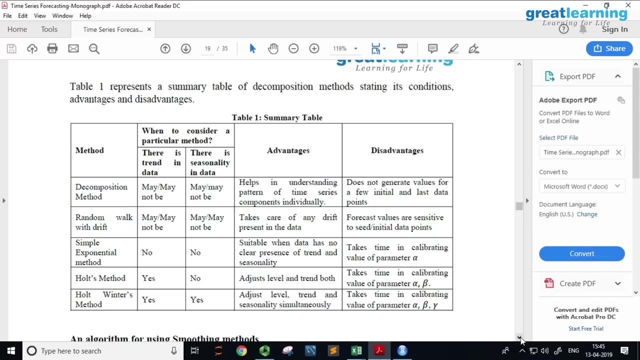 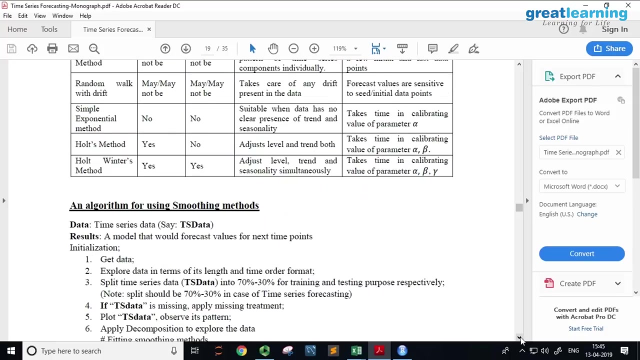 low frequency and we were trying to do noise mining. we're trying to find patterns in the noise, so it's possible to do that, but it's a. it's a far more sophisticated set of methods and people disagree about it as to whether you should do that or not. anyway, yes, yes, no, what this weight will. 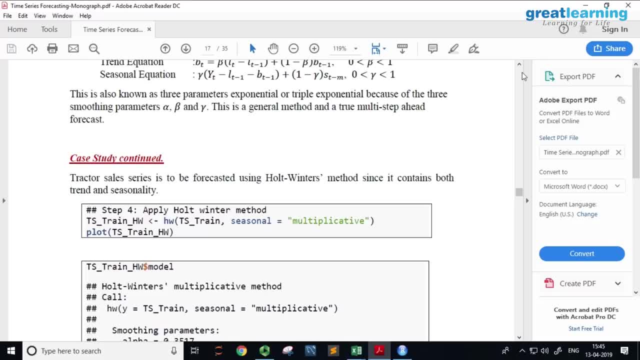 do is you can. by the way, when you fit these models, you can always take your value of alpha and beta and gamma in this. so if you believe that, for example, you should give more weight is to the recent past, then what you can do is you can artificially change this gamma so this gamma is taken to be 0.64 over the. 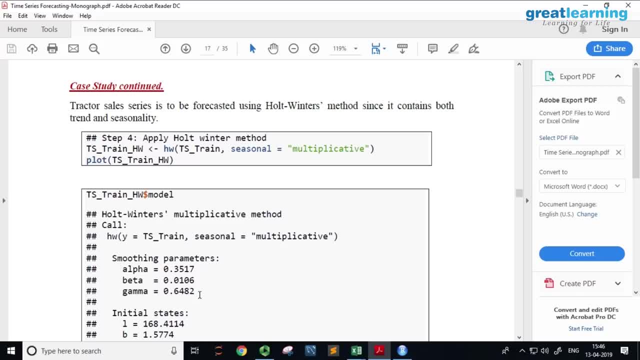 2003 to 2013 period, but you might say that's not exactly true. I want to give more importance to recent weights based on recent events that make the 2003- 2007 irrelevant. so you might want to bump up this gamma to about 0.9, 0.8 or 9 or 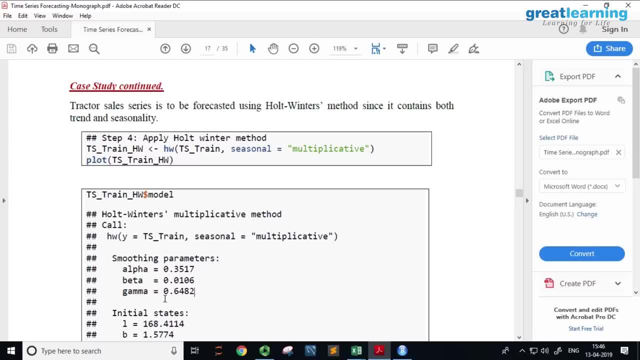 something of that sort which will adjust seasonality a lot more to the recent happenings in the seasonality. I don't know. I can try that out, but it's a dangerous thing to do because what the model will do is the model will learn a lot more from the recent past. 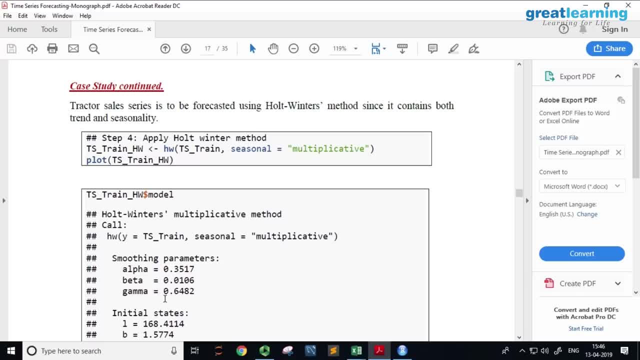 but in learning from the recent past, it will then adapt a lot more to what is happening right now, but it is good estilo. it's going to want to tend to ignore what had happened in the past of. that may be a good thing, that may be a bad thing. not in the recent past, in the 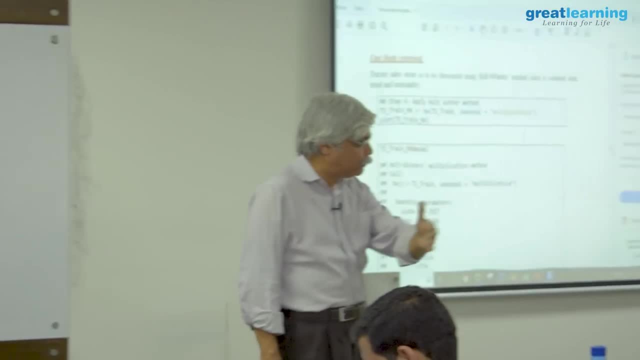 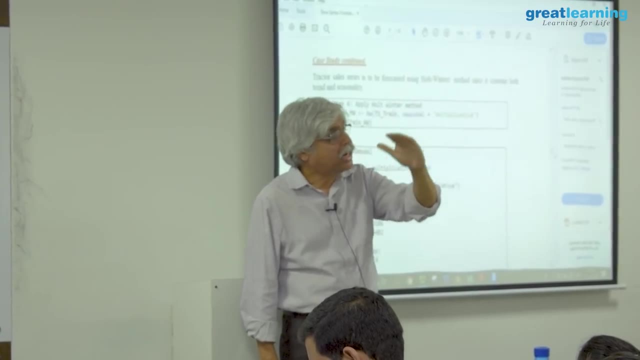 forecast window, because I am forecasting 13 and 14. so the actual sales in 13 and 14 was a little higher systemically, a little higher than the previous sales, because if then it will come a little higher, so you might not get really high. but that's the stuff is. 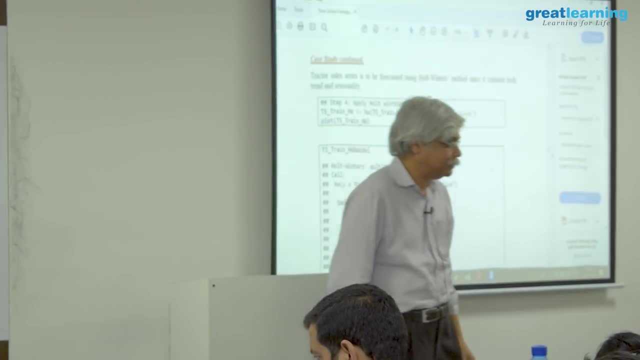 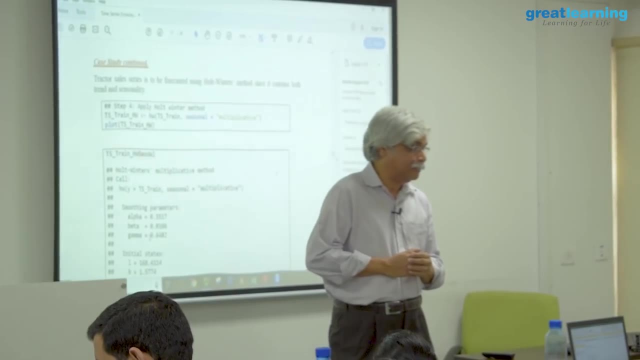 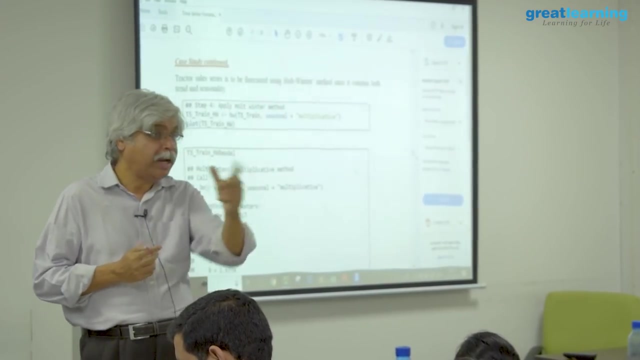 than what was forecast from 2012 onwards. So if I simply looked at 2003 to 2012,, the forecast that I got was slightly under, So 2013 and 2014 were a little higher than expected. Now his point is that. can I somehow interpret that? 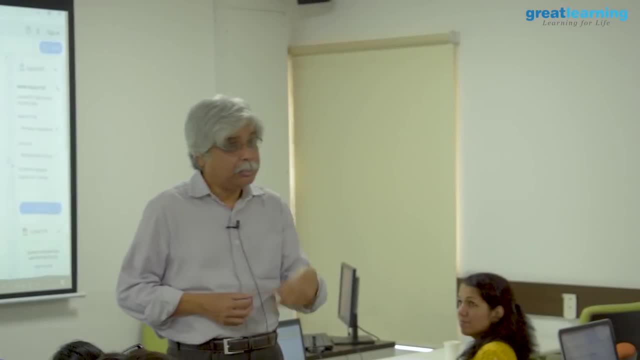 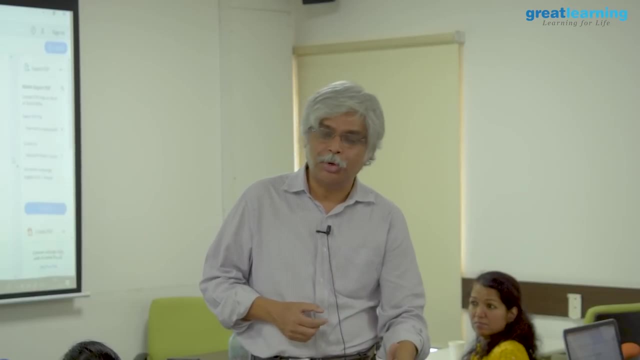 to be a drift, a change, and that change was already present in, let's say, 2012 and 13.. So by biasing the model towards the more recent past. can I pick that up? And the answer is possibly, but in biasing the model. 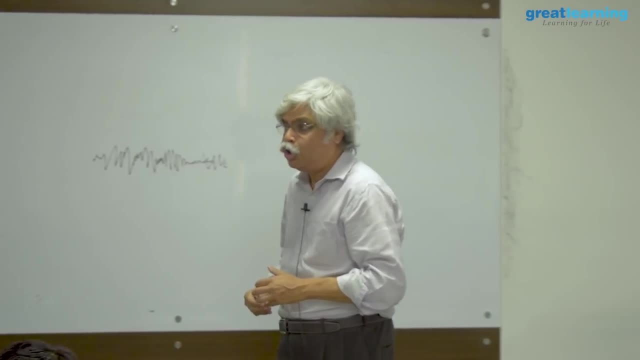 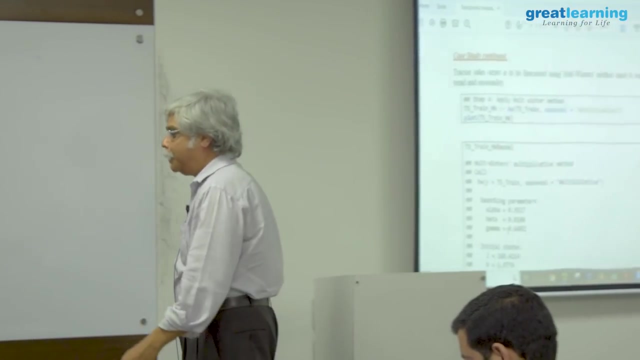 you're also making the model use less data, And so I'm not sure which way the answer would go, but you're welcome to try it out. Yes, that's a much more complicated problem, as I said So, and that model- you may do that, for example. 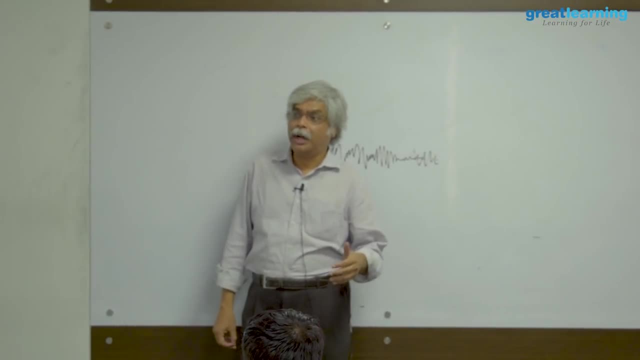 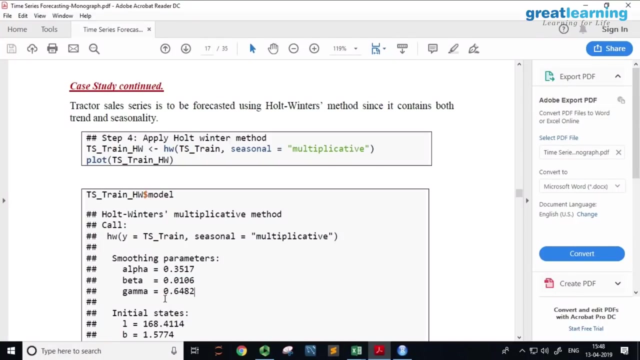 like share, right. so when you grow a market- I don't know whether you're doing that in marketing, but when you grow a market, how do you grow a market? Or how do you grow a product base? One way is that you take market share away from someone. 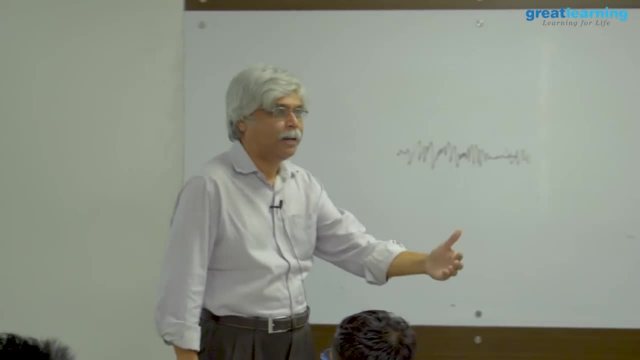 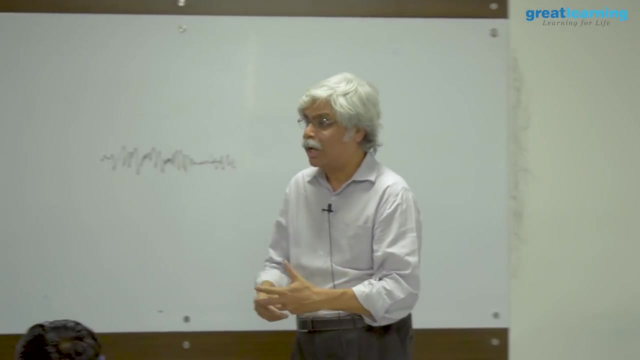 The other is you get new share. In other words, you get new people come in, And these often require different kinds of strategies. Sometimes, as I said, you're cannibalizing your own product line. You're essentially saying that I'm not going to do this. 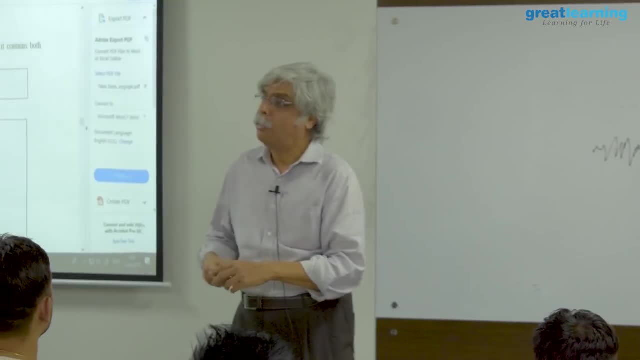 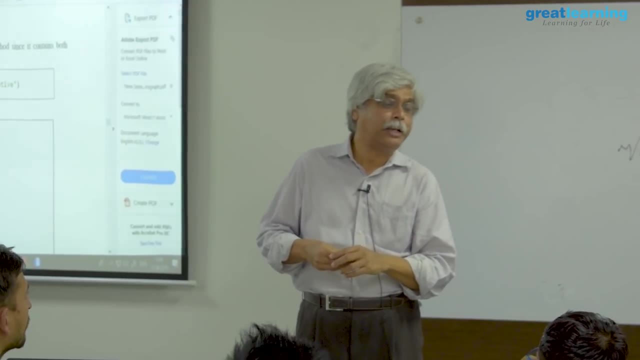 So I remember many years ago one of the more commonly used- in fact a very popular- car was the Innova, the Toyota Innova. Everybody had an Innova, more or less, And then suddenly Toyota said we're not going to do any Innovas. 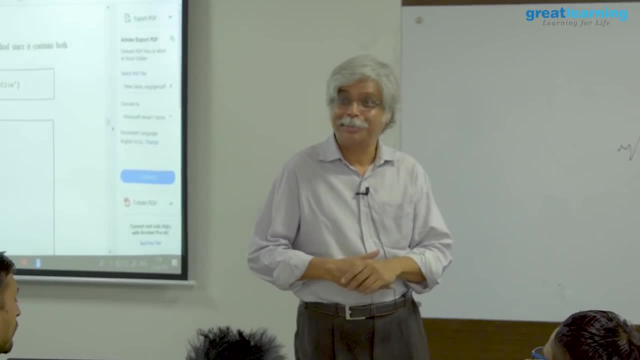 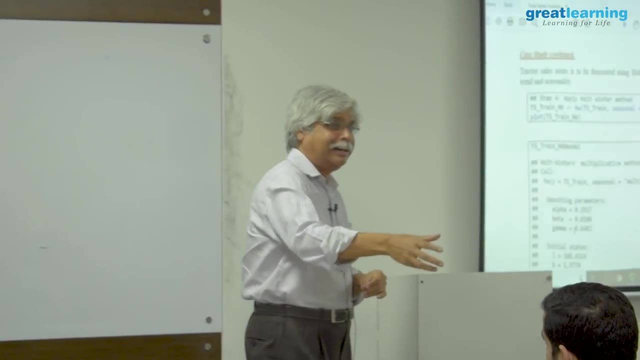 Everybody said why Everyone likes Innova. Why is the Innova, you know, disappearing? But Toyota essentially said that we want that Innova market and we want another car in that market, which is, in some long-term way, a fairly sensible way to think. 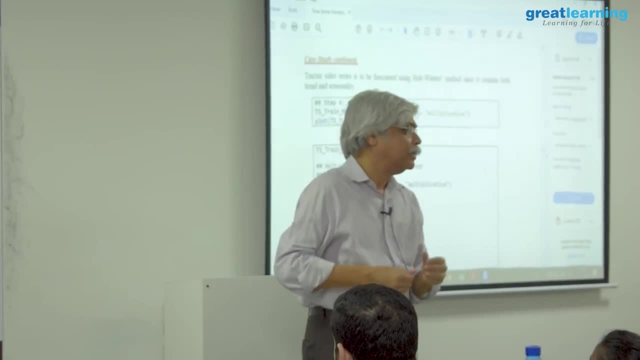 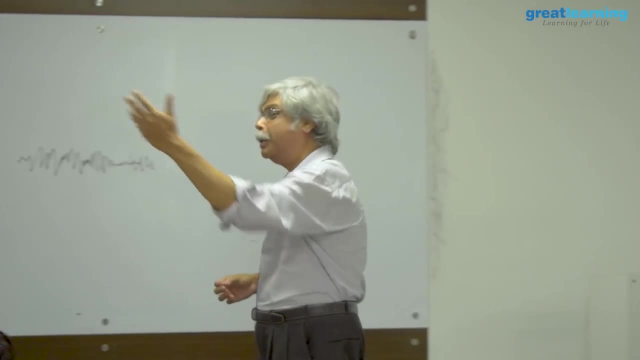 That if I have that Innova market, that Innova market is where I should be launching my new product. So they cannibalize their own market in order to be able to get an easier ride into a bigger market share. now what? what that happens from a time series perspective is so, for example, what would 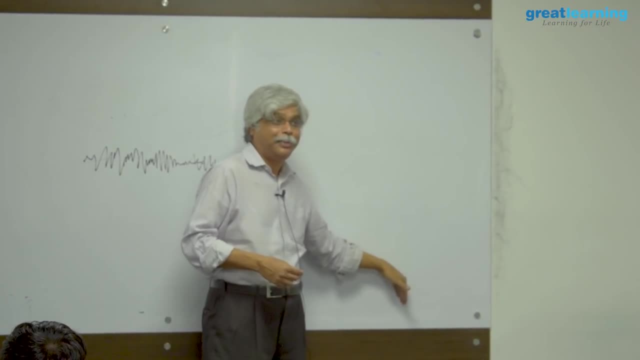 happen to the share of Innova? now, by definition, the Innova share would just drop. it was, you know what- to some extent stopped, but the other markets shared, but the other products that was coming in to replace it would get an artificial boost up which would be less than what a typical time series or any market. 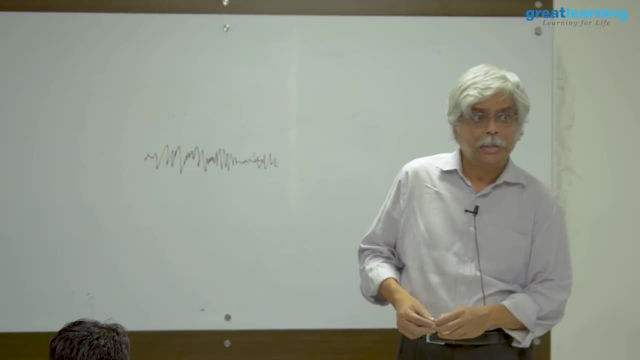 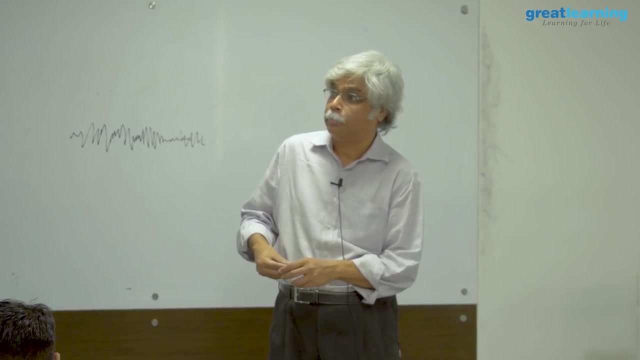 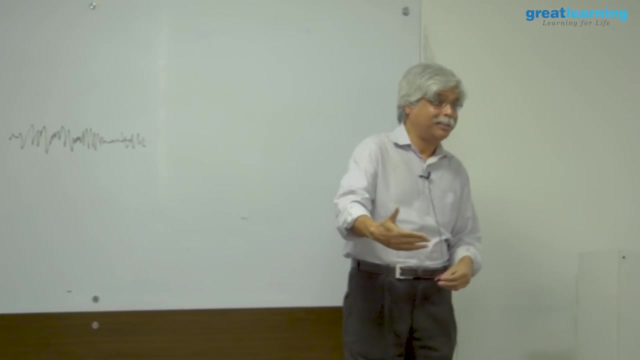 projection forecast would do, and so can you conceivably do that? yes, I mean, it's the business equivalent of a politician setting aside and leaving the seat to his son. I mean, the seat is being cannibalized, so to speak, but the son is getting that, you know- a boost from the, from the, from the boot bank. that was. 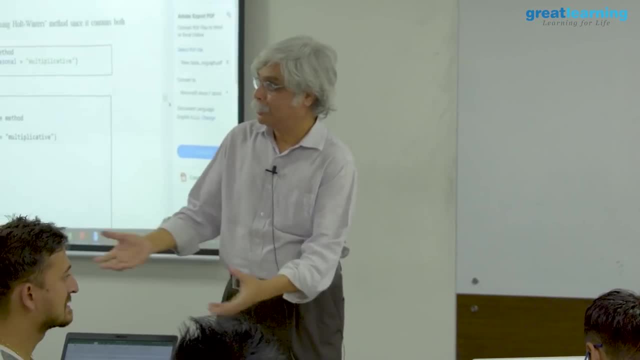 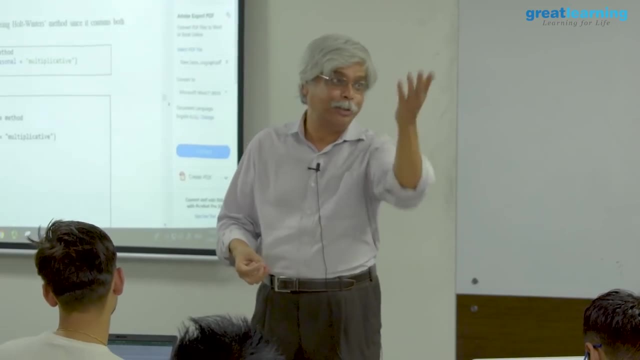 there but the father is not getting any boost. the father's vote share is forecast to be something and suddenly it becomes low, the son's forecast with no credibility whatever. you would expect it to be low, but he is going to get a very cannibalized share of that vote. that 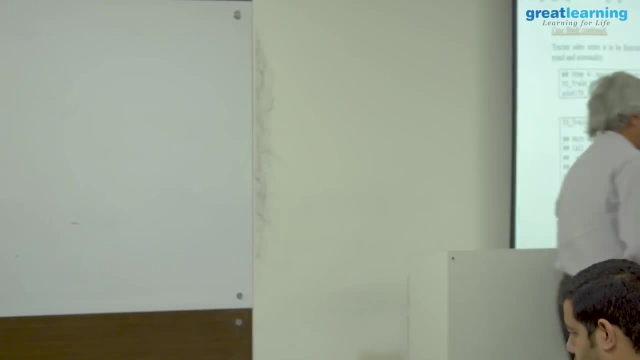 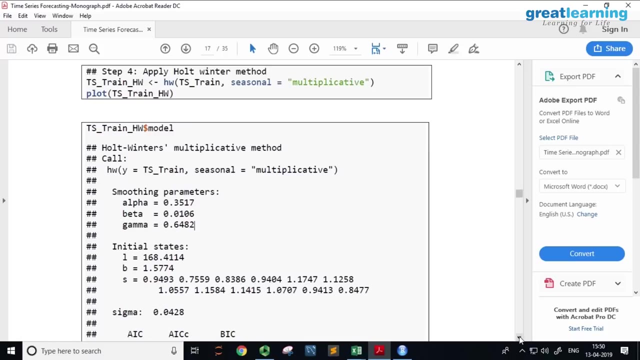 makes forecasting very difficult. you're right, but, yes, what you can do is this: what you can do is in data sets of this trend or your kind. the better way to do that is not to do this. the better way to do that is to forecast using a smaller. 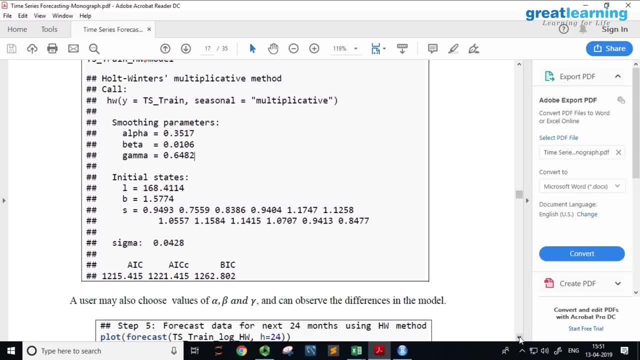 series. repeat this, but don't use all of 2003 to 2012. use this, let's say, from 2009 to 2000, 2012, and see what happens. don't let the data feel around too much in the past, and that is. that is always the. that is a standard way of doing it. it leads to its. 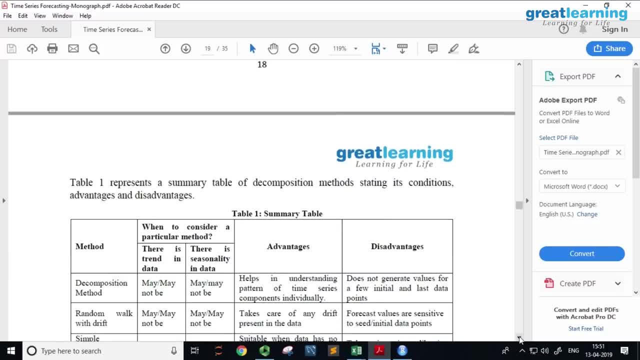 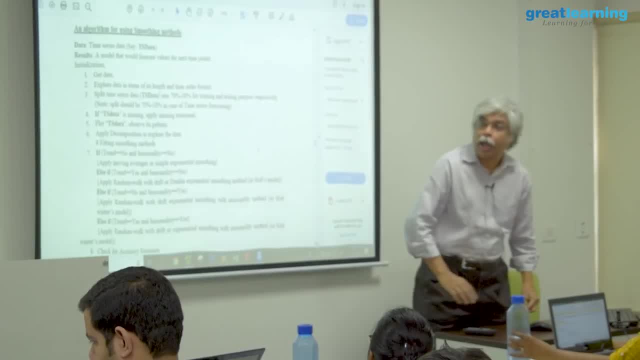 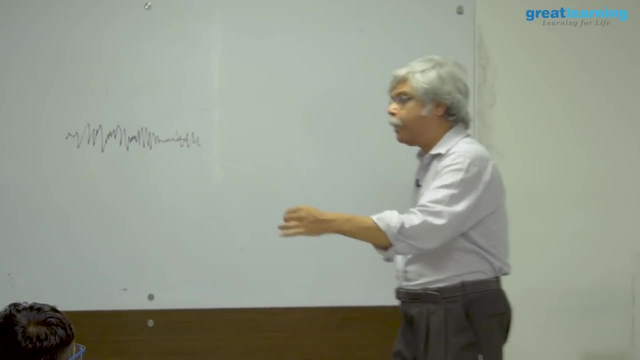 own problems, should you do that? so, for example, let's suppose that I'm trying to understand how much raise you will get next year, correct? and I'm going to ask yourself the question. I'm going to say I'm going to forecast your annual raises and I'm going to forecast is, as an average of a. your previous years raises. your choice is: how many years should I take? should it be one? should it be two? should it be three? should be four? now you see the problem. if I take one, then my entire data is going to be driven by how much raise you got this year. but if I take, let's say, five or six, then I'll get a. 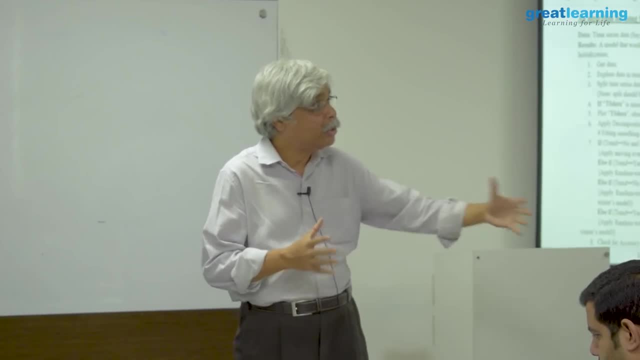 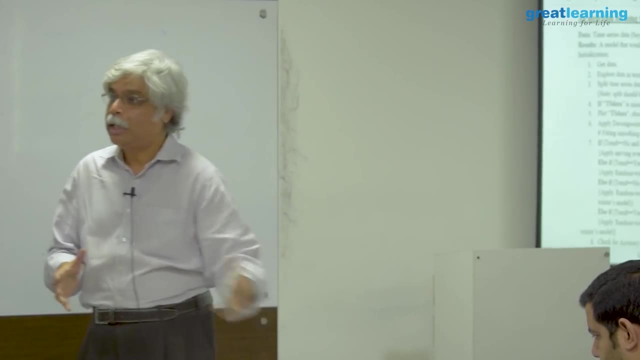 far. I'll get an average picture of what you are like and where your career is going. but maybe that represents too much of what is happening three or four years ago and you may say, no, forget about that. I'm a lot better now, so it's a bias. 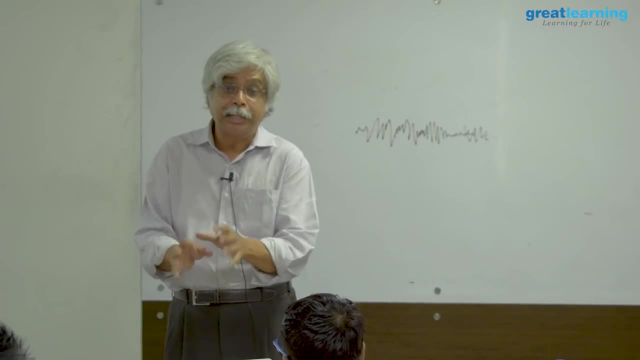 between saying: do I use a little bit of correct information, but one that is not validated by long-term performance, or should I use long-term experience and say that's that's. is there an easy answer to that? no, as you yourself are probably figuring out in your head. 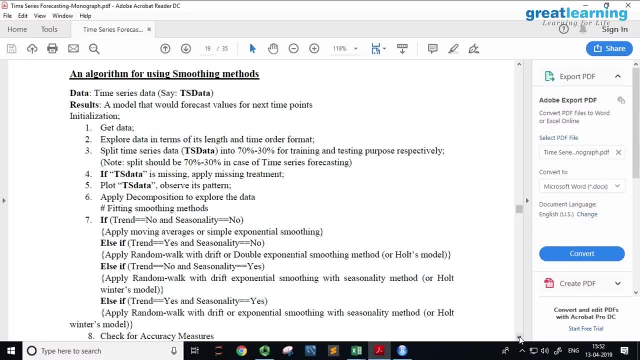 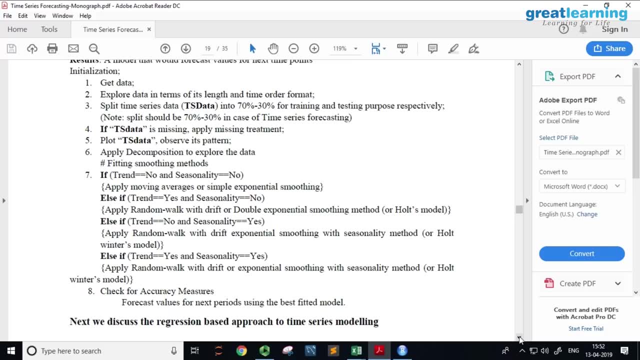 there's an algorithm here. if you're doing this, it's simply a inverse version of what they're talking about, saying: which algorithm should you use? if we have the time and we might, we might try this kind of algorithmic approach to a new data set and see what happens, or you might try it and I might help you out. 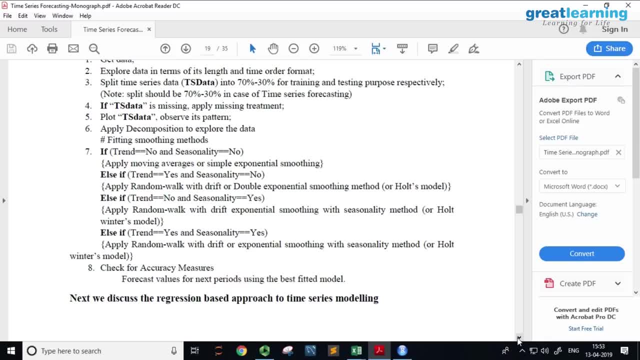 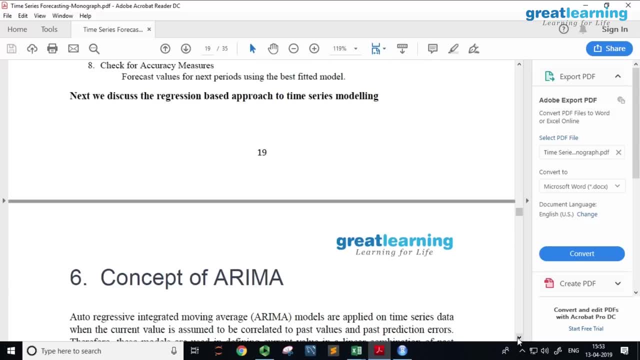 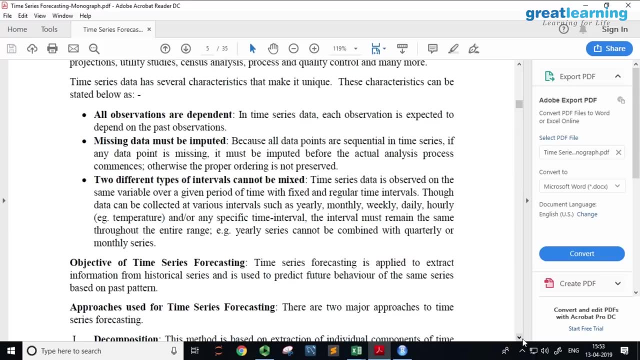 so this is one approach. now, if you remember, we are talked about two different approaches to time series analysis. when did we begin this? class 230, right? so the second way of doing it, let me go back. so the second. so the first way of doing it was here: decomposition. decomposition means I'm taking a series 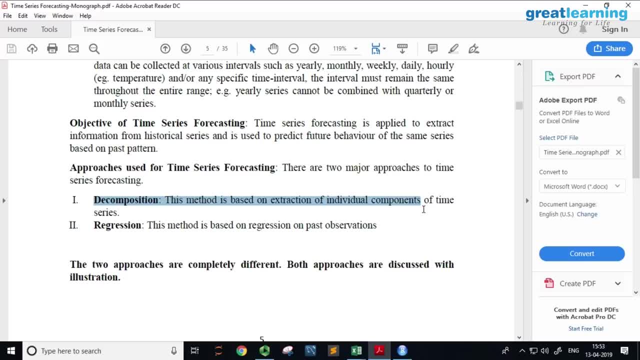 and I'm splitting it up into seasonality- sorry, level trend and seasonality- and I'm forecasting based on that. the other way of doing things is to look at the problem as a regression problem and see my problem is: I want to predict YT and I'm going to write it as a function of my